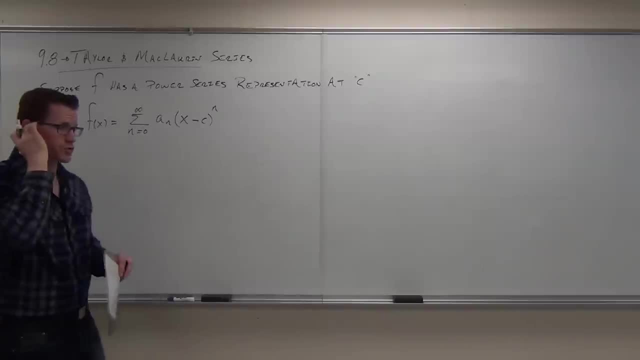 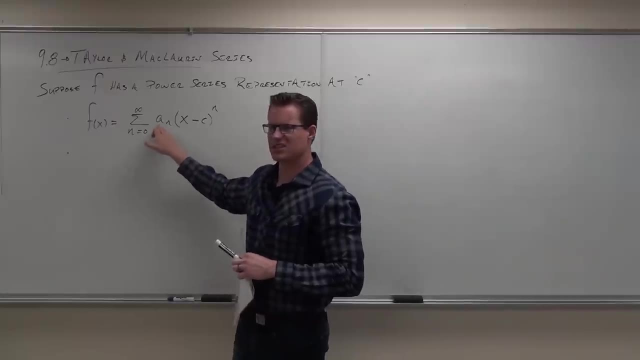 going to state next is this: If this is true, if we have a power series representation because we have these terms, the sequence of terms where we get our series from, all of these a sub n's are going to be constants, true or false? 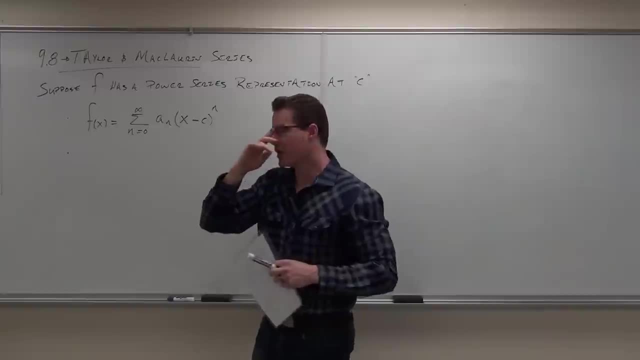 Which means that x is coefficients. yeah, as n goes from zero to infinity, Then we're going to have x, basically x to the zero, x to the one, x to the two, x to the three, x to the n, correct? What that means is that, for sure, if this makes a power series, we're 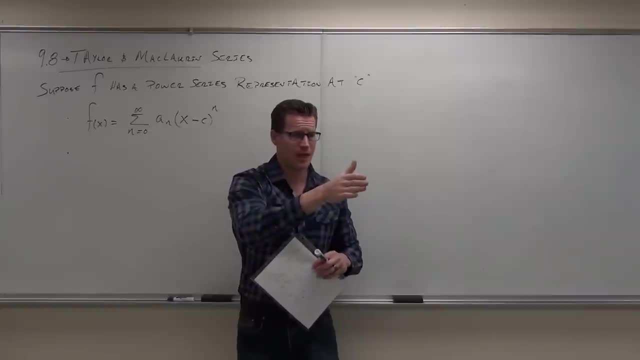 going to have a whole bunch of terms right Wherever we stop is going to be the nth term. Does that make sense to you? That's going to be x to the n. What that means is that the f to the n derivative must exist. It's got to be there, Because what we're going 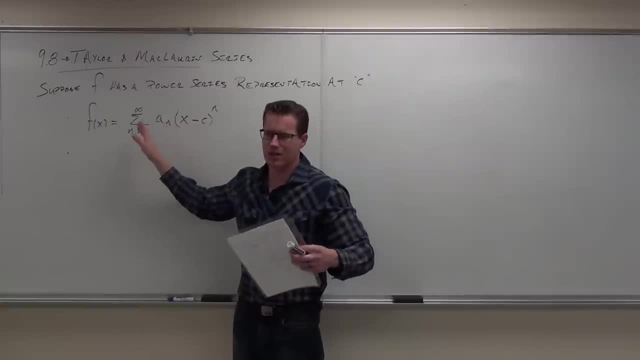 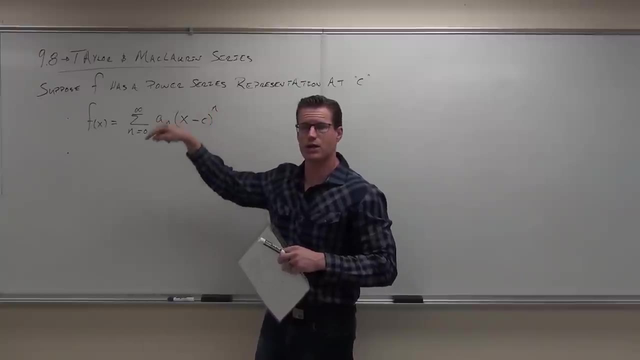 to end up getting is a whole bunch of coefficients. These are constants, fractions, I don't care what they are, It's going to be something. times x to the blank power. That nth power means that you could take a whole bunch of derivatives, couldn't you? Hello, yes, no. 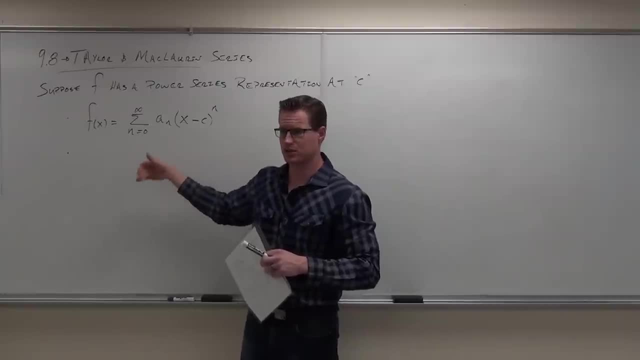 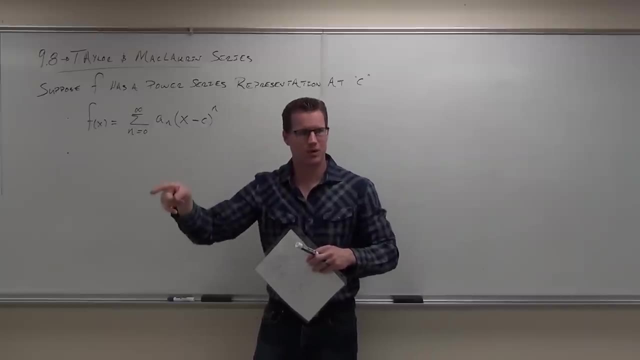 If I had three terms I could take up to a third derivative, and it's going to be there. It's going to be a constant. actually, That's what it's going to be. Just say: okay, bring down the power, subtract one from it. That's the first derivative. Bring down the power. 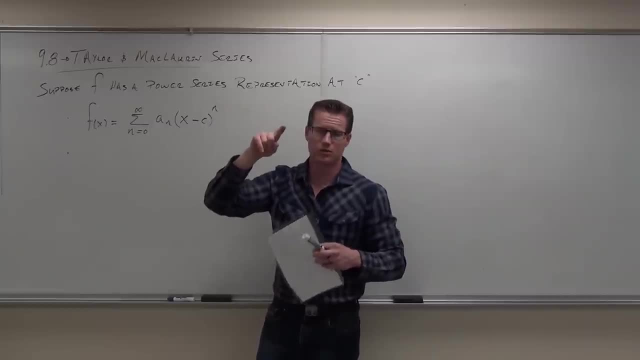 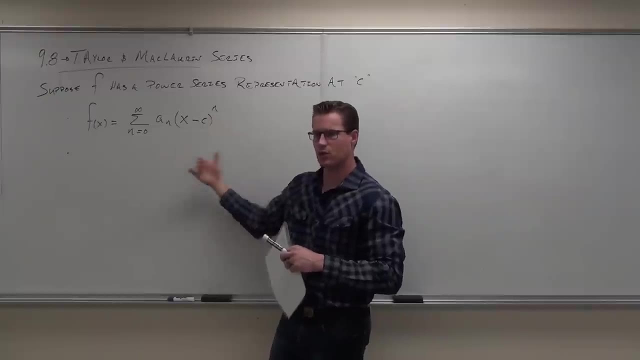 subtract one from it, That's the second derivative. Bring down the third power. subtract one from it, That's the third derivative, and so on. Bring it up to the nth derivative, because there's going to be a power n somewhere in. 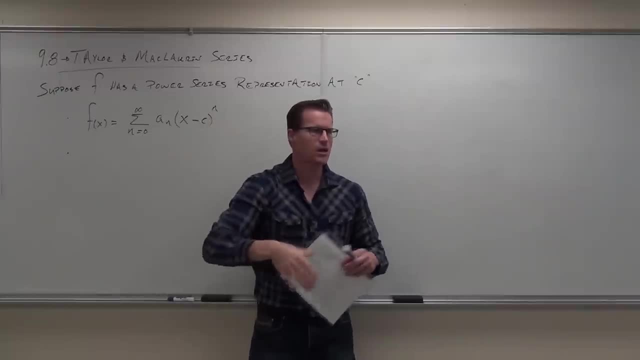 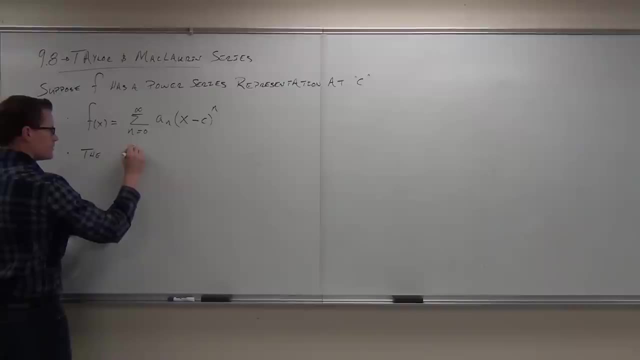 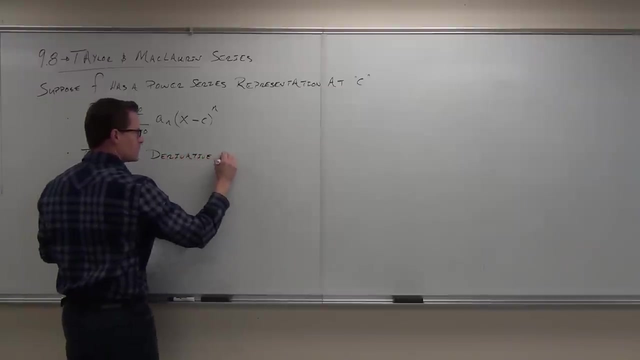 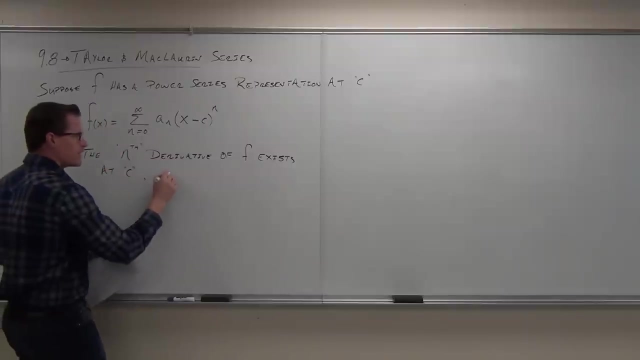 your power series in your list of terms. Does that make sense? Then we say, all right. well then, the nth derivative of f exists At c, And the way we write that is f to the. well, not f to the, I'm sorry. the nth derivative. 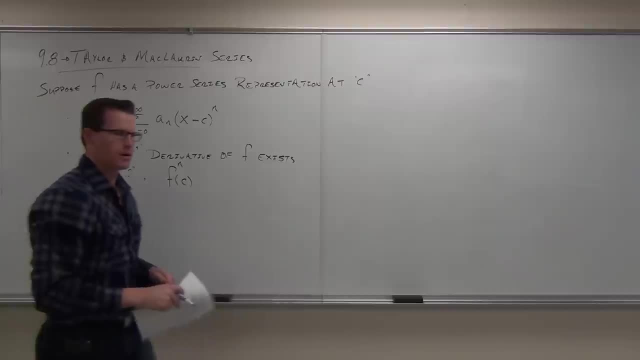 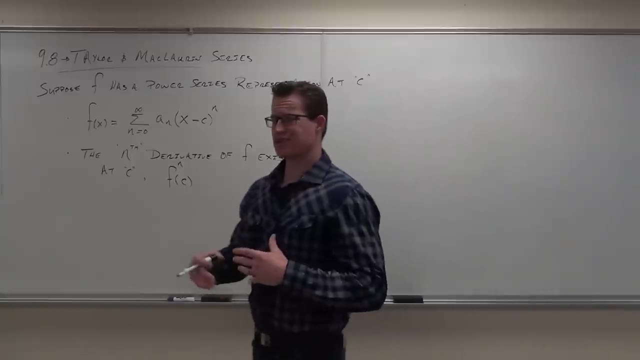 of f at c. That's what that says. I'll go through it one more time just so that makes sense to you, and then I'm going to show you what we can do with this thing. This is going to be interesting. This is where we're going to get our Taylor series from, So here's the 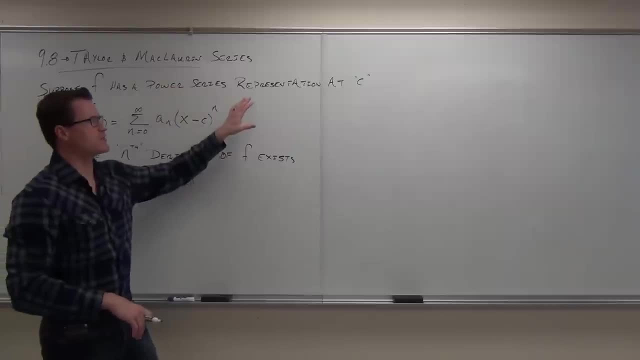 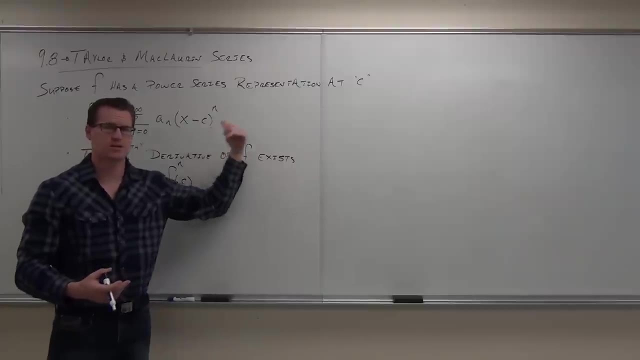 idea one more time. If f has a power series, or if it's a power series it's going to have a representation at c, then this is for sure true. Then f can be represented by a power series. Not a problem. A power series is x to some power. If we have x to some power, 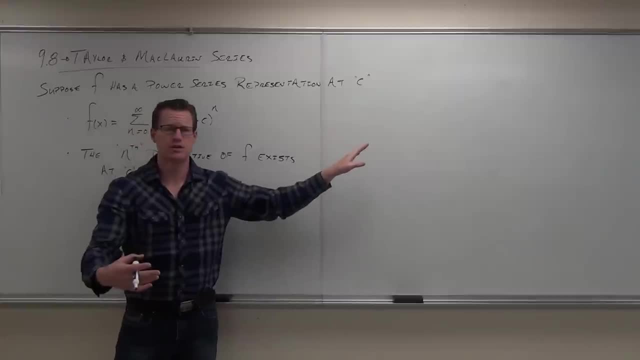 n and we list out all of these terms and we start taking derivatives. then the first derivative is going to exist, and the second one, and the third one, and the fourth one, all the way up into the nth derivative, because what's going to happen is that our first term? 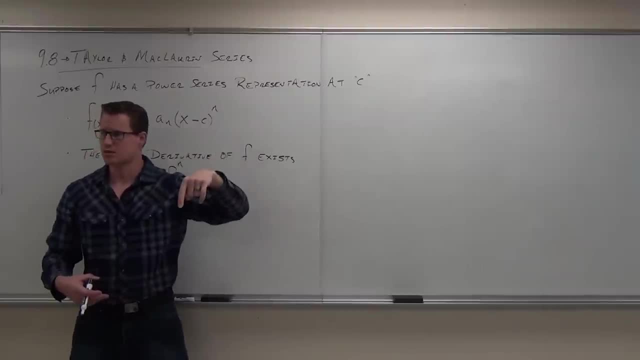 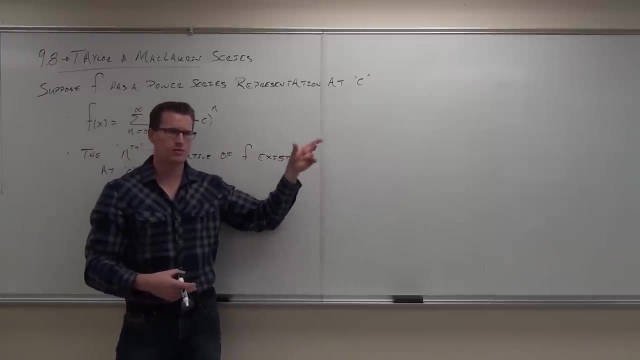 is going to go to zero. It's a constant. Our second term becomes a constant. Therefore, when I take my next derivative, that term goes to zero. That's going to happen until we get down to our nth derivative. Our nth term ends up turning into a constant at our 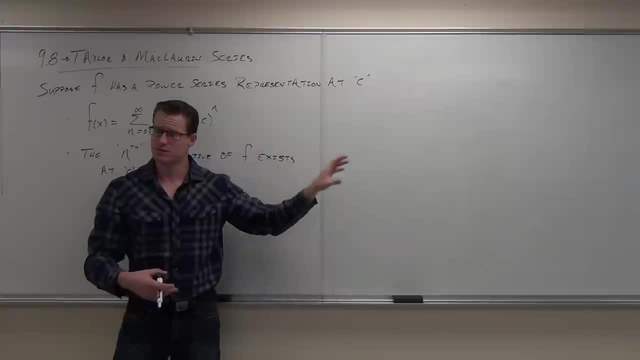 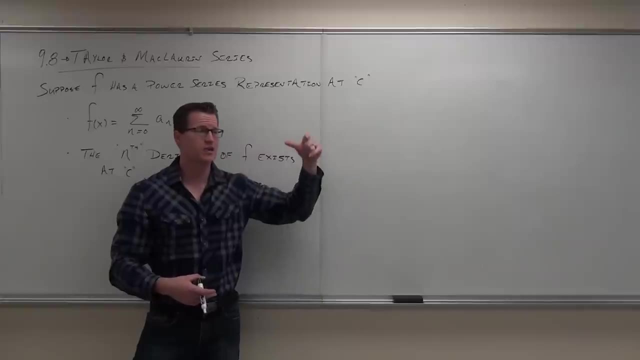 nth derivative. Does that make sense to you? All the rest of them are going to be something like x minus c to the, whatever the next term after the nth one, n plus one. That's going to be x minus c to the first and then to the second, then to the third, then to the. 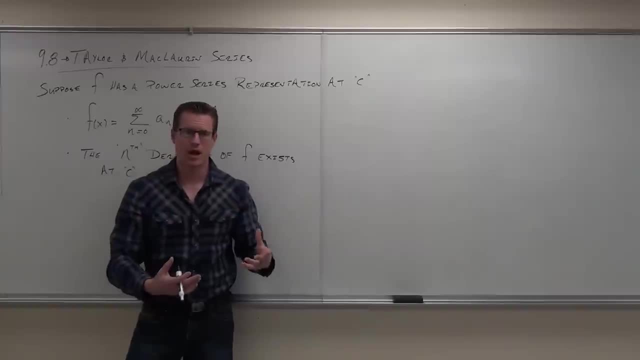 fourth, But we can take up to the nth derivative and it's going to exist somewhere At c just means hey, plug in c, Not a problem, Show fans, you feel okay, that this is going to exist. This is going to make a little bit more sense when we go through the next term. 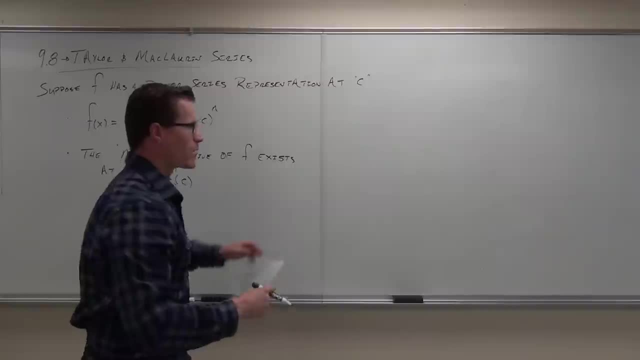 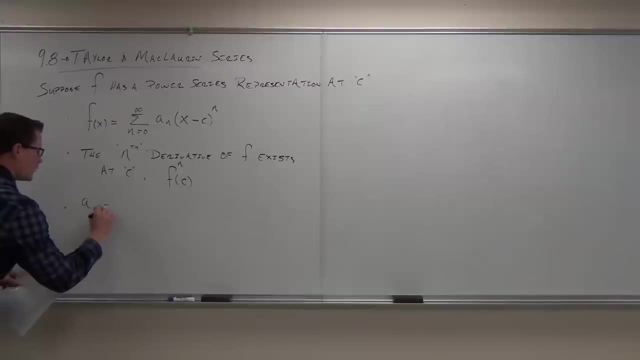 The next thing I want to find out- and I'm going to write stuff up here, I'm going to erase it in just a minute- This is just to show you what this is. The last thing is: I want to find out what a sub n is in terms of my derivative. in terms of that, We're. 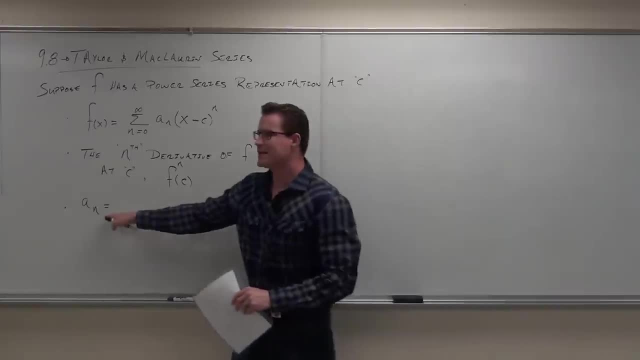 going to do it this way. You guys ready for it? We're going to come up with what a sub n is. The idea is, what I'm trying to do is figure out basically a formula that's based on my function that I can put right here, If I can. 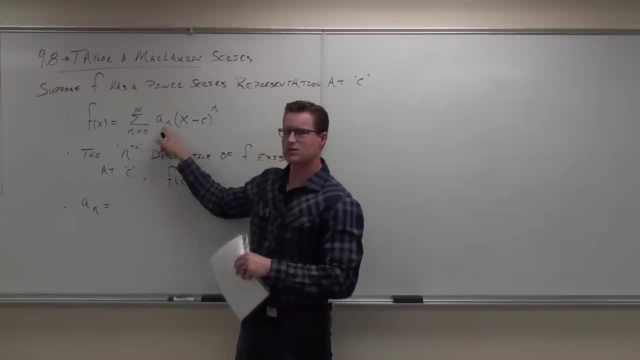 do that, I'm going to be able to figure out what a sub n is. I'm going to be able to figure out a formula that's based on my function that I can put right here. If I can do that, if I can base this on my function, well then I can start building a power series from. 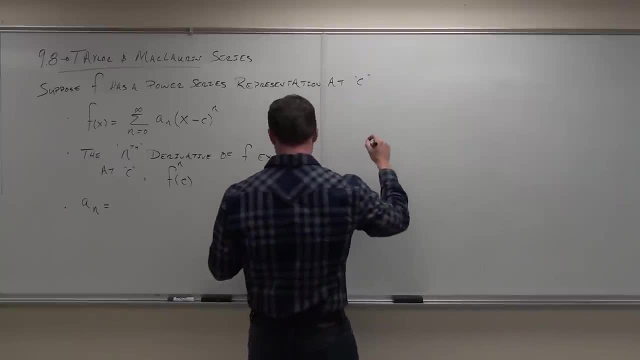 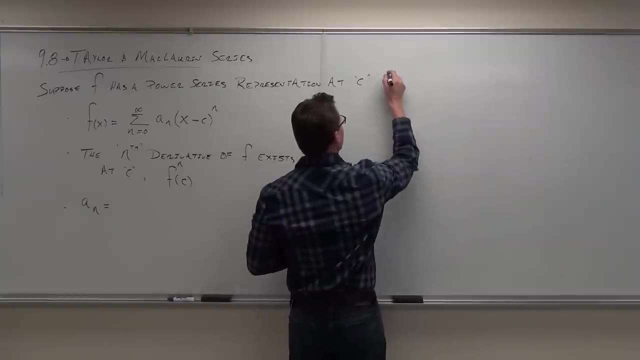 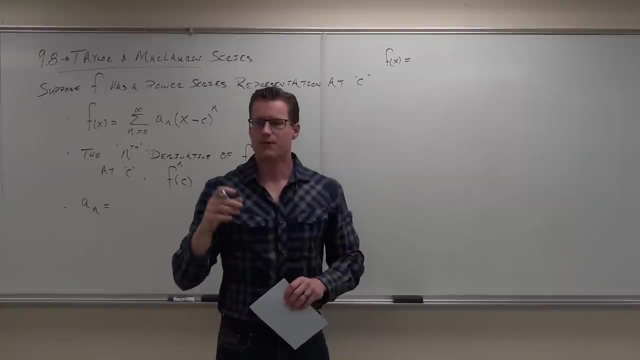 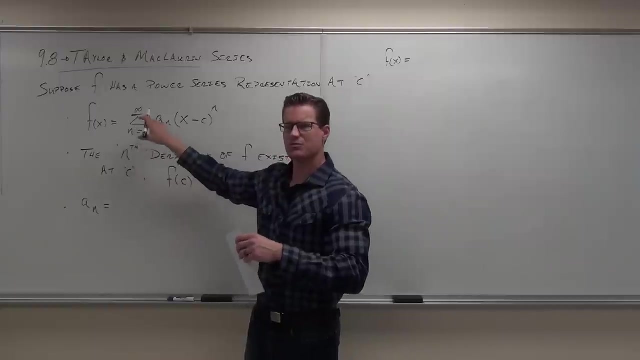 a specific function. Here's the idea on this. Let's start with f of x. If f of x has a power series representation, then it's going to be represented by this thing. In general, it's going to be represented by this Give. 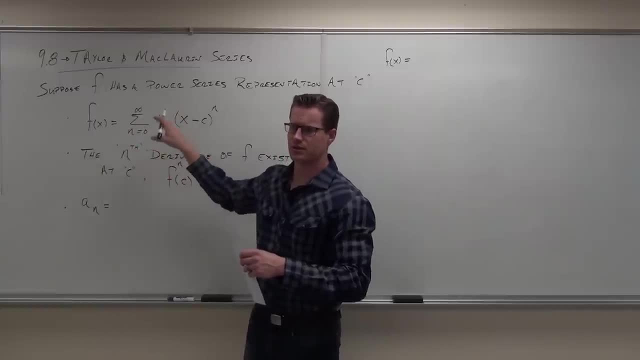 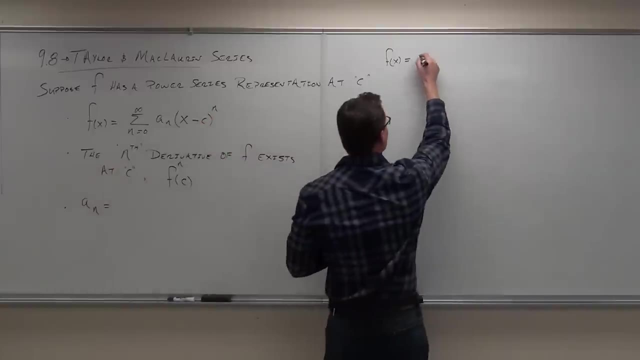 me the first term, The first term of this power series: a sub n, a sub zero, Zero. And it would be this to the zero. It would give me one, It would be a sub zero. Then I would get what's the next term. 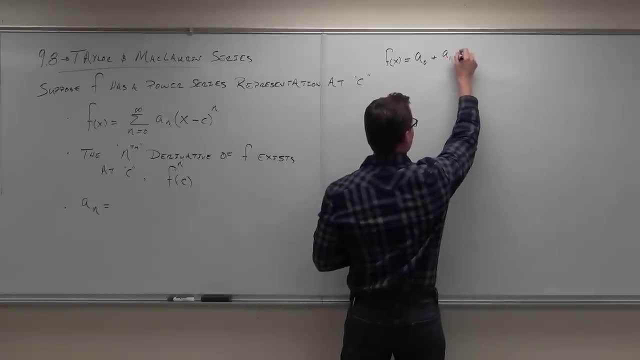 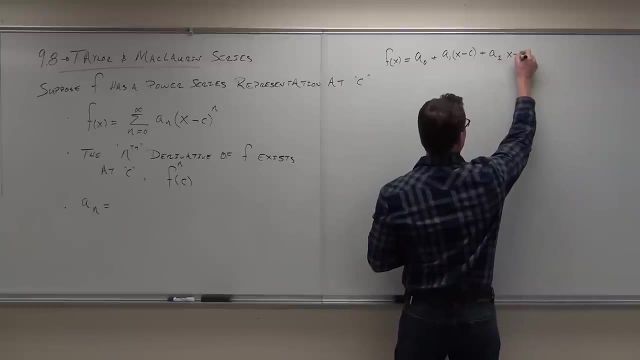 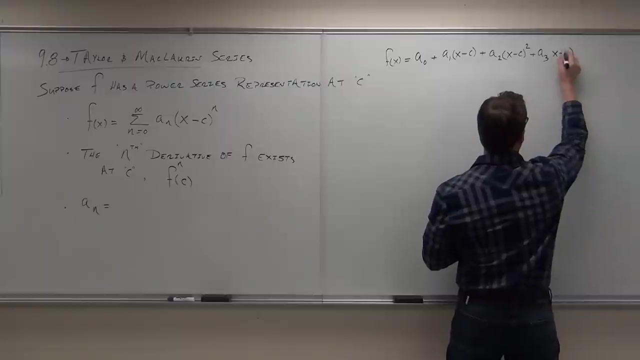 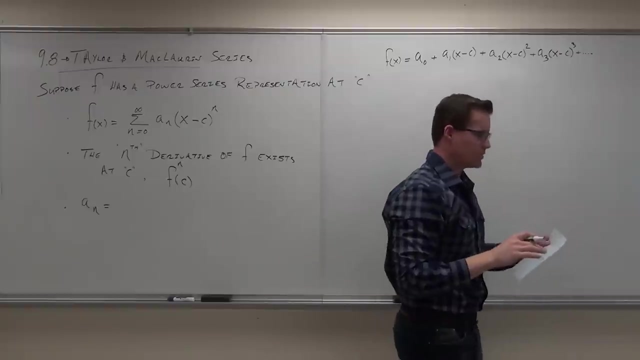 a sub 1 x to the second minus c To the Tell us a sub 2 x minus c squared Plus a sub 3.. x minus c squared Plus blah, blah, blah, blah, blah all the way down until we get to. 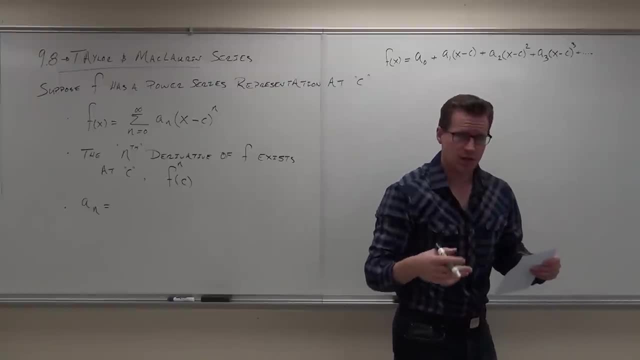 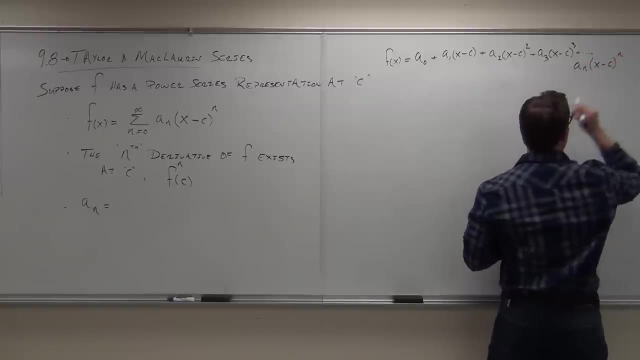 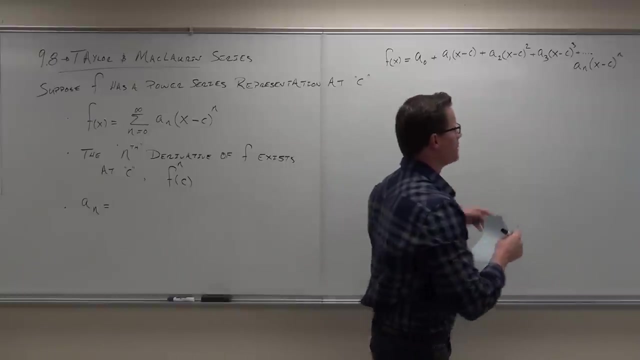 n a sub n. a sub n x minus c to the n. Good You guys. okay with that one. Now, this says we stop at n, but in reality this thing would keep on going until we get to the. 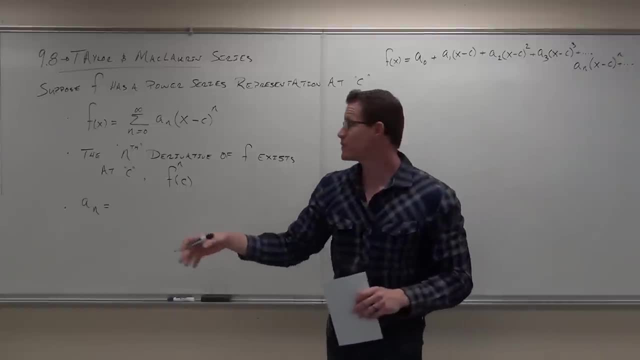 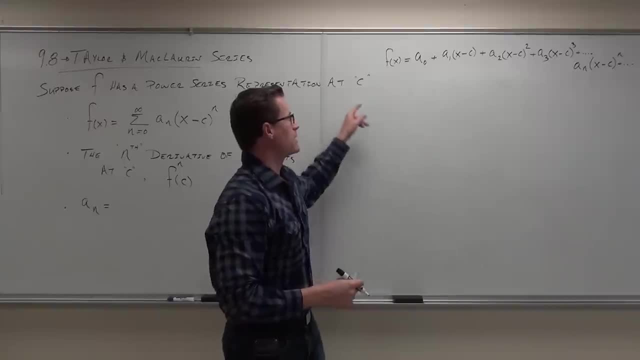 Are you with me so far? So here's the point I was trying to make earlier. Maybe you can see it a little bit better now. Do you understand that? if this is my power series representation, it basically acts like a polynomial here. 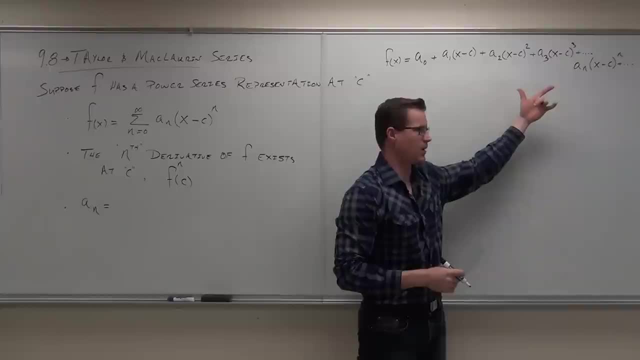 It's going to be x to some power. These are all constants. They're coefficients of whatever x term we have. What that means is: could I take a first derivative? Sure, Could I take a second derivative. Could I take up to an nth derivative? 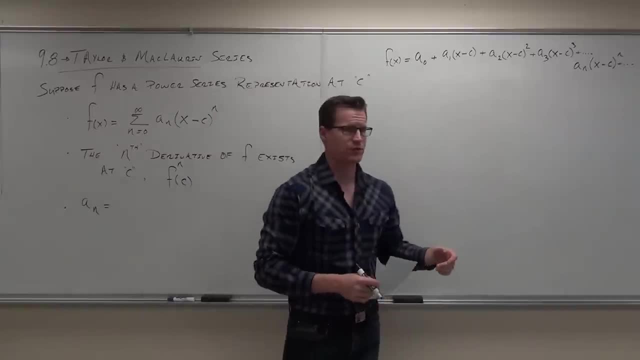 Absolutely. All that's going to happen is I take a second derivative. means is: could I take a first derivative? Sure, Could I take a second derivative? Could I take up to an nth derivative? Absolutely, All that's going to happen is I take a derivative. 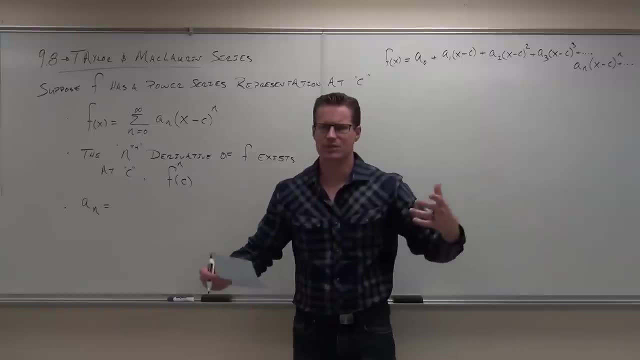 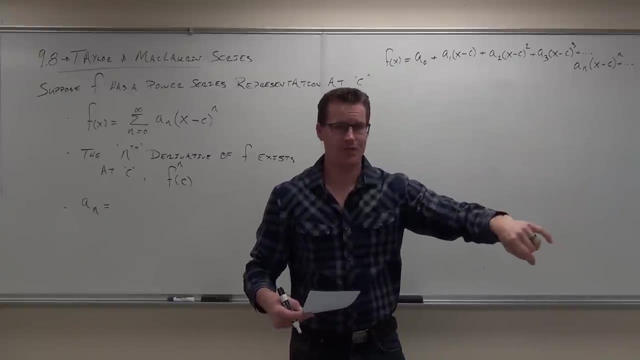 of all these things, n times or whatever. n is five times, seven times, a million times, who cares? If I have a millionth term, then I can take a millionth derivative and then I can plug c in. Does that make sense? Now this is going to get kind of interesting, for 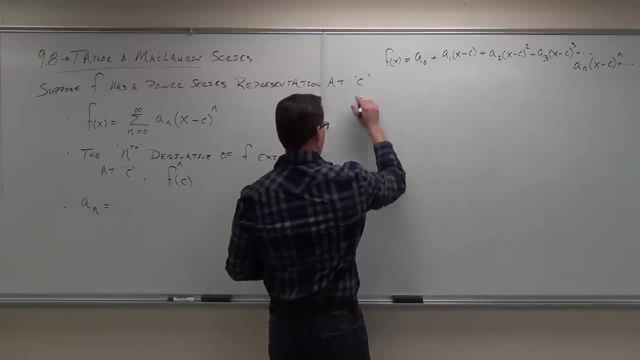 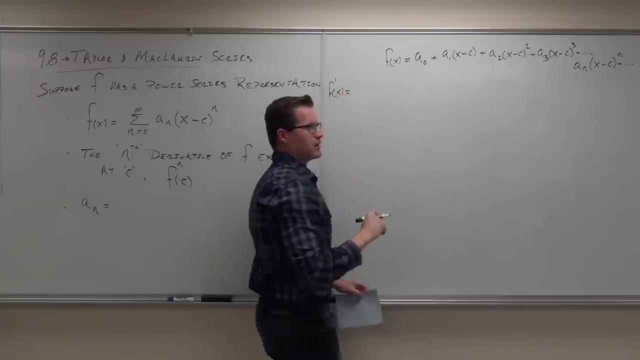 us. Let's start taking derivatives. If I take the first derivative, I don't want to erase that- If I take the first derivative, f, prime of x. help me out with this- What do I get? Remember, we did this in the last section. This is why we just did that is so that you. 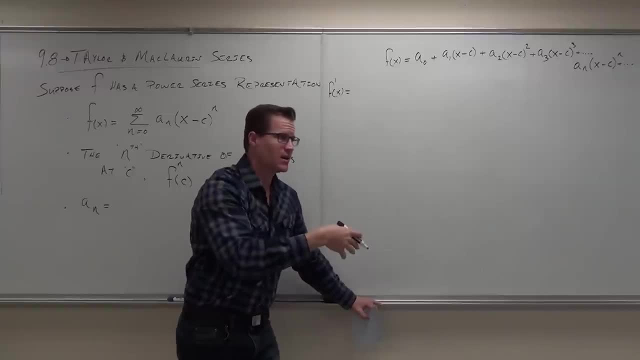 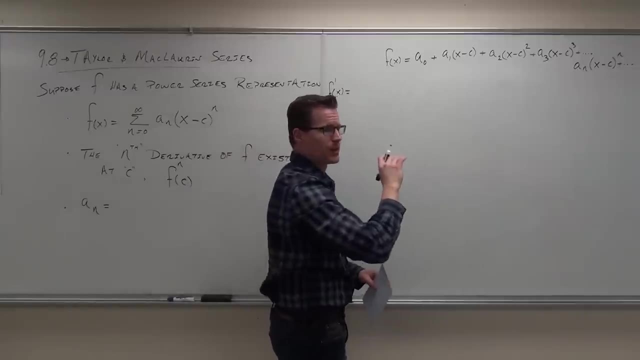 understand that you can take a derivative of a power series. That's why we did it, because now we're going to use the last idea that we had in the previous section right now. So take your derivative. What happens to a sub zero? Zero, That's gone. What happens? 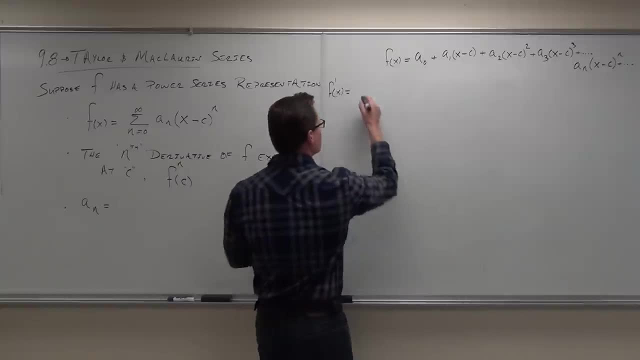 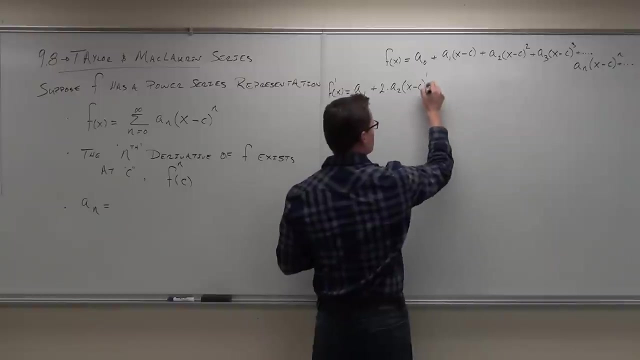 to a sub one x minus c. What's that become? A sub one, Very good, Plus what? Two? a sub two, Oh good, Why the two? What are we going to get Change? So two times a sub two x minus c To the first power- Very good, Plus Three: a sub three. A sub three. 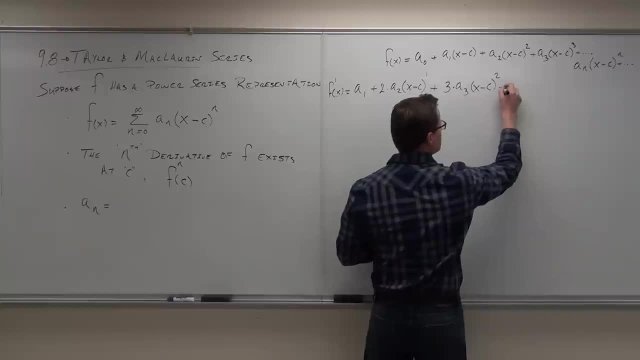 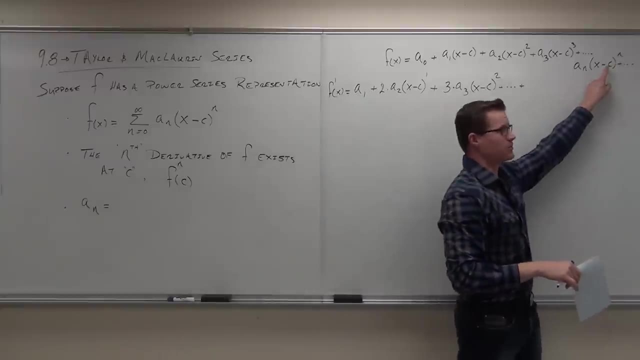 x minus c to the Second power. Now, this is the one that I really want to focus on, This one. You see, here's why I want to focus on what we got from the nth term. What I want to focus on that one is because, when we get down to the nth term, we're going to have 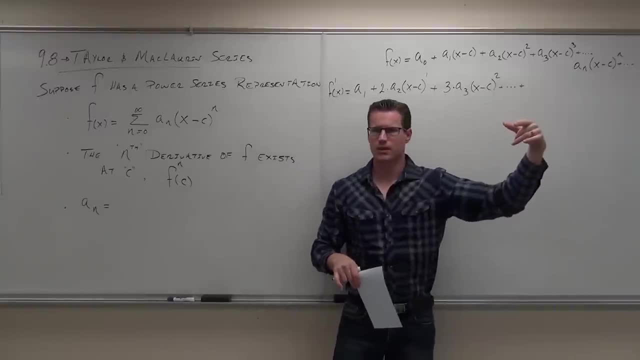 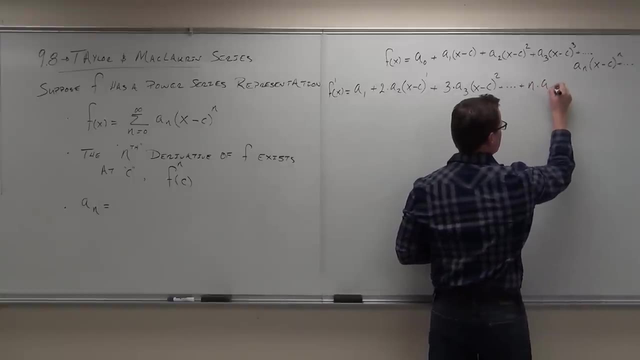 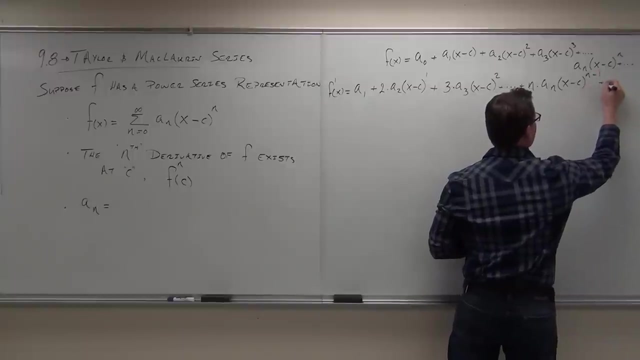 to get down to the nth derivative, Do you understand? all these things are ultimately going to go to zero. They're all going to become constants. So I'm really focused on this guy. So what happens here? And then we would continue. You all okay with that one? 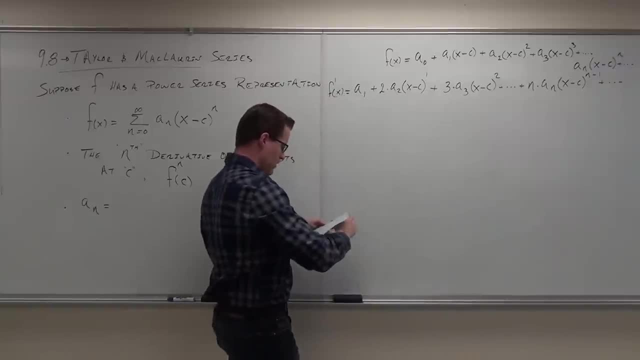 That's the one I want you to focus on, to see what happens with this. Okay, let's continue. We're going to do like four derivatives, Three or four derivatives, So just to get a really strong pattern here. So let's do f double prime of x. Okay, tell me what happens. Come on, you guys got it. 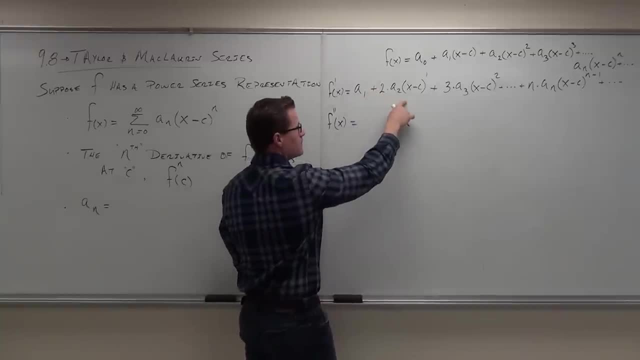 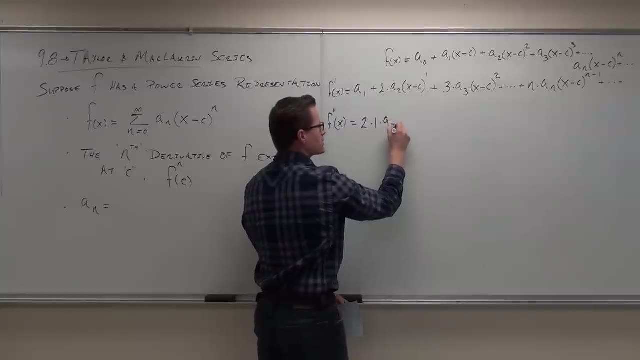 What happens here? What happens here, Really? what happens is you bring down the one, don't you? You really get two times one, Do you see it? A to the second, I'm sorry, a sub two x minus c to the zero, but that's going to go away. So you get two times one times. 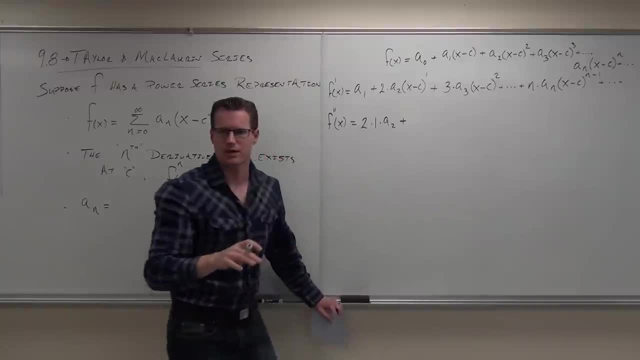 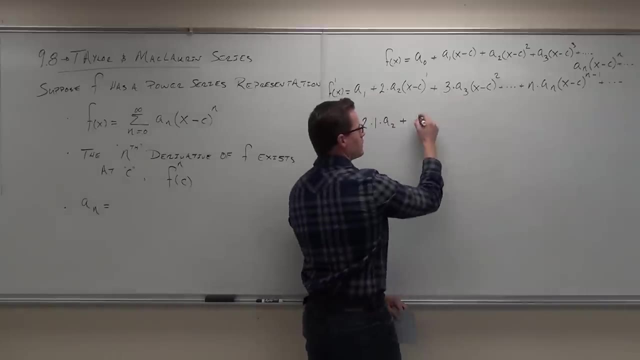 a sub two, Two a sub two. Yep, Now I don't want you to simplify it, because we're going to be looking for a pattern here. Does that make sense? Looking for a pattern? Okay, next up It's three times. don't give me six. I don't want six With this stuff, we're really 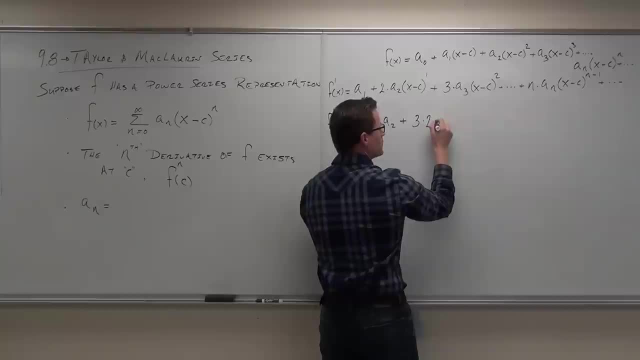 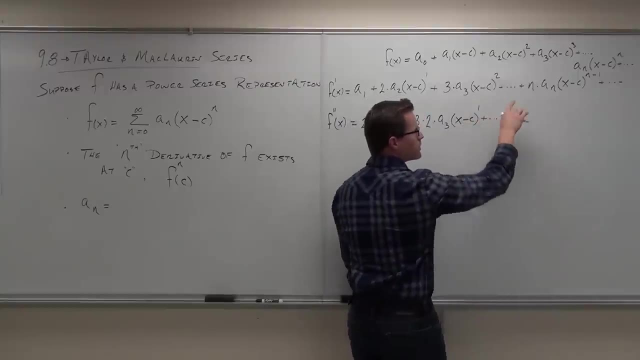 looking for a pattern here. So it's three times two times a, sub three x minus c to the first plus. Okay, now remember, this is the one I want to focus on right here. What's going to happen? N times n minus one. 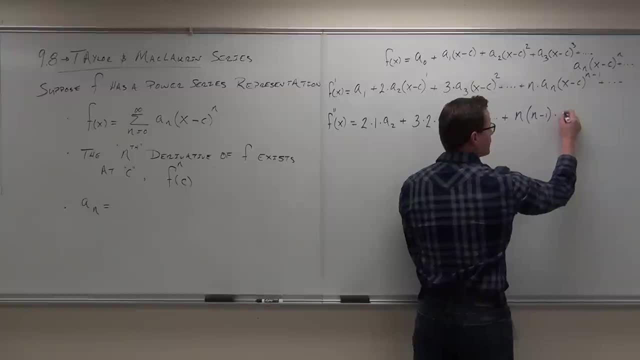 Good, You'll bring down the n minus one Times n minus one, Times n minus one. Then you multiply by X minus c, X minus c Minus one Minus two. Very good, Minus two. Are we okay with that so far? 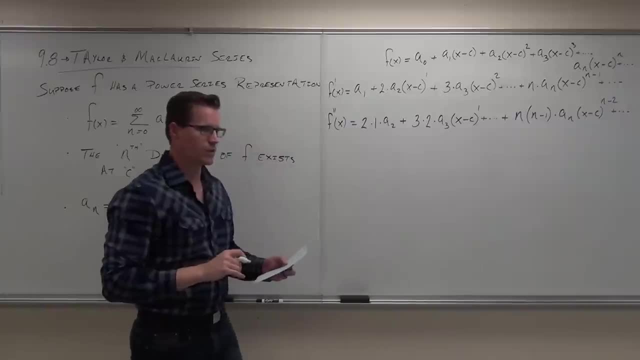 Mm-hmm. Okay, it's going to keep on going. Let's do. this is the last one that we'll do, because the pattern's going to be apparent after this. If we did a third derivative, what happens to this term? Where does it go? 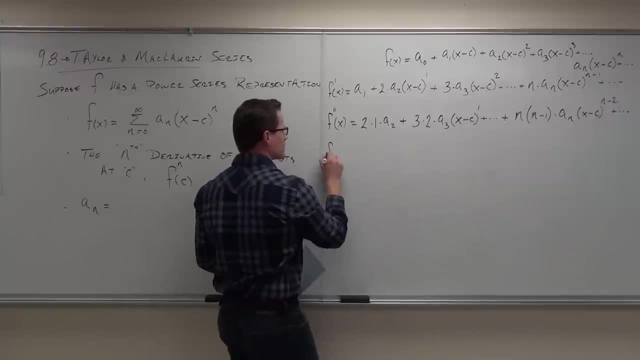 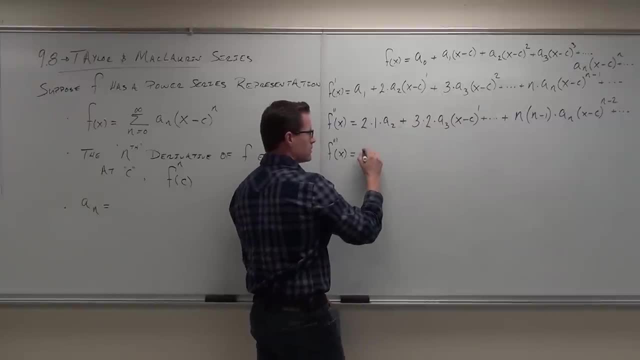 Z, Z, Z, Z Z Z Z. The second term we'll be doing will be Three times two, Three, Three times two times one A sub three x minus c to the Zero. Zero. that's going to go away, that's going to be one. Are you with me? 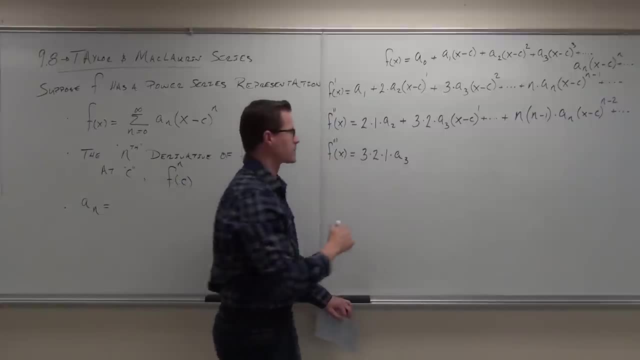 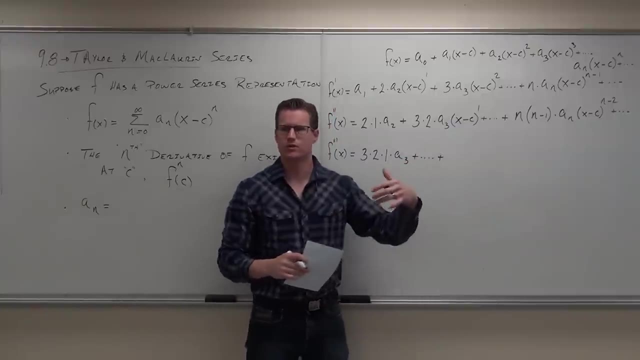 I'm sure you're with me. I'm sure you're with me, okay? Plus, blah, blah, blah. Do you notice that? what happens is that we're going to end up getting a constant for every single term that we have. Are you with me? So check this out. 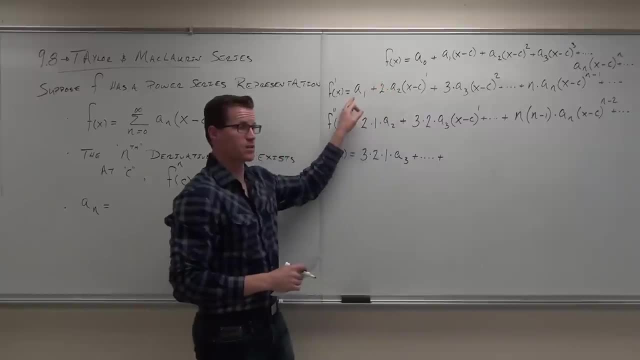 when we did a first derivative…. What I ended with was a sub 1 term as a constant. Are you listening? When I did my second derivative, I ended with my a sub 2 term as a constant. Do you see it? a sub 3 had an x with it. 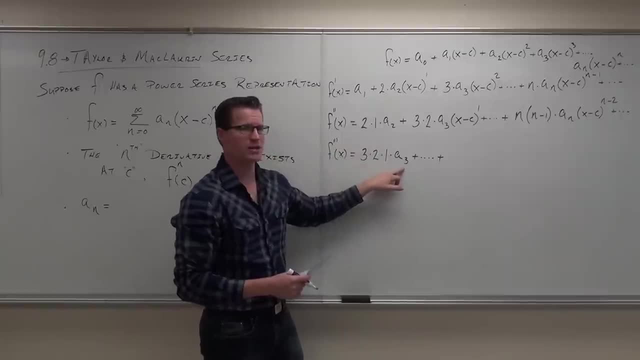 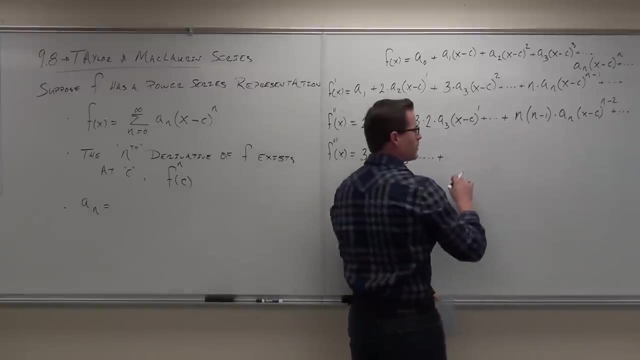 When I did my third derivative, I ended with my a sub 3 term as a constant. My a sub 4 term would have an x to some power. Does that make sense? Now let's do our next derivative. What am I going to get from this term as a derivative? 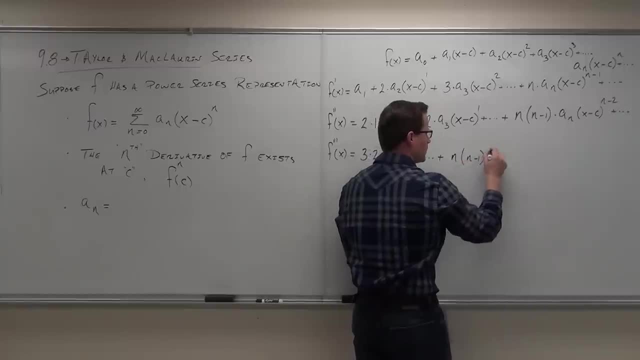 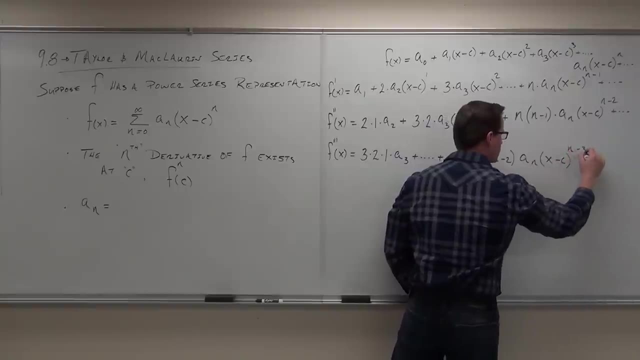 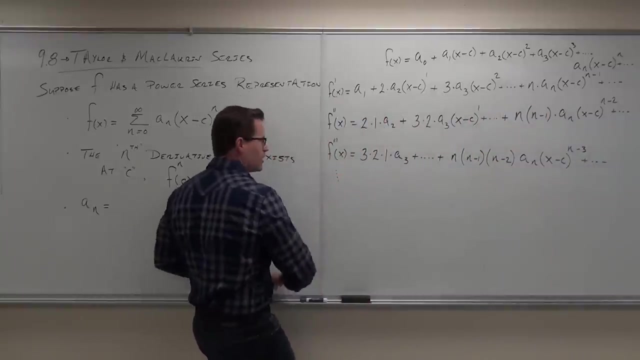 a sub n. very good: x minus c to the n minus 3 plus blah, blah, blah, blah. forever, never, ever. Now we're going to make a big jump. We're going to go down here and do the nth derivative. 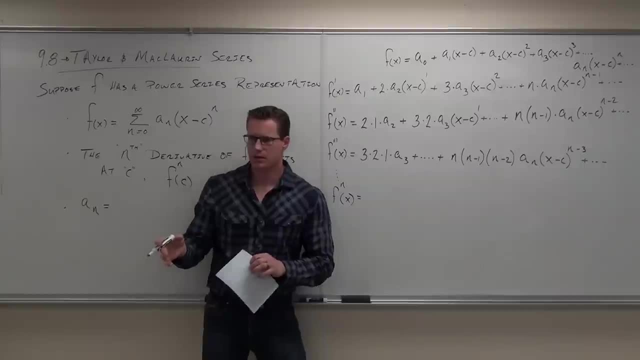 Firstly, does this make sense to you where all these things are coming from? Hello, yes, no, Are you sure? Yes, We're just doing derivatives, We're doing chain rule, no problem. Derivative on the inside is always 1, so we got it easy here. 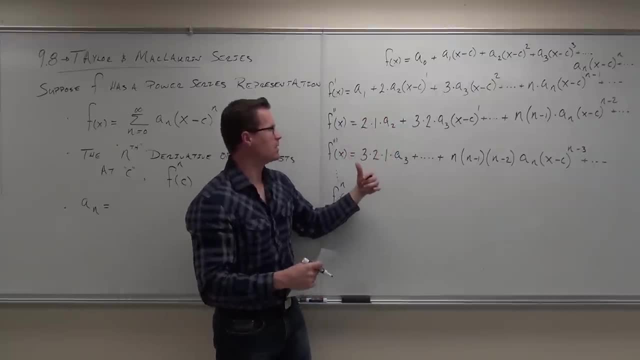 What I'm trying to get you to see is the pattern that's taking place. What we saw is that, okay, well, when we work this down, we got 2, 1.. We got 3, 2, 1.. 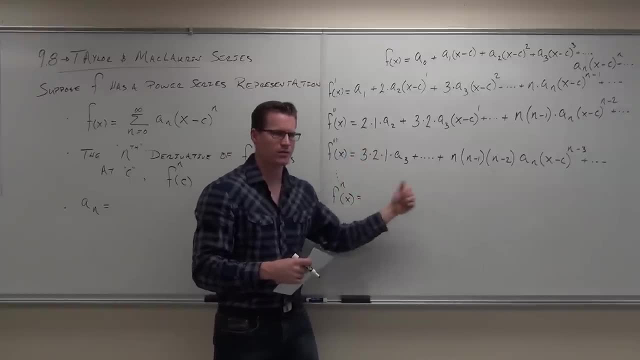 We're going to have 4, 3,, 2, 1.. We're going to have 5, 4,, 3,, 2, 1.. We're going to have 6, 5,, 4,, 3,, 2, 1.. 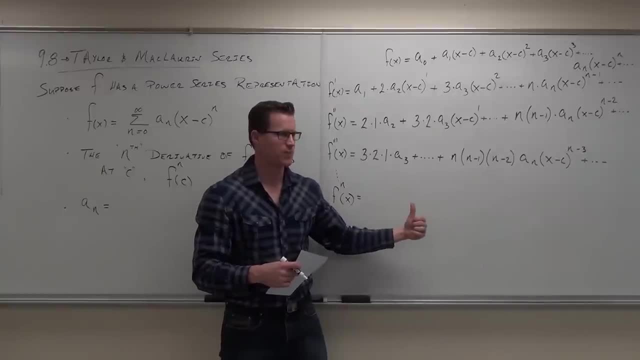 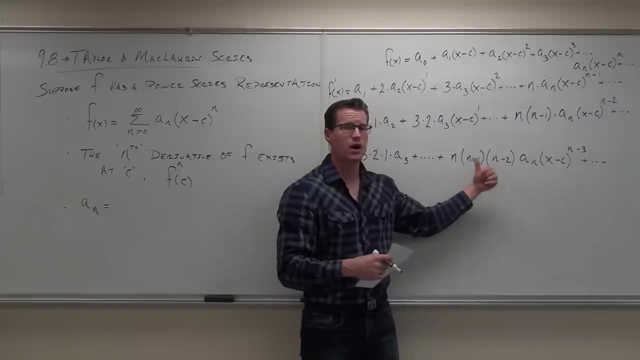 We're going to have n factorial somewhere in this problem. Do you see it? Also? it says right here we have n. We have n times n minus 1, n times n minus 1, times n minus 2.. That's a factorial idea. 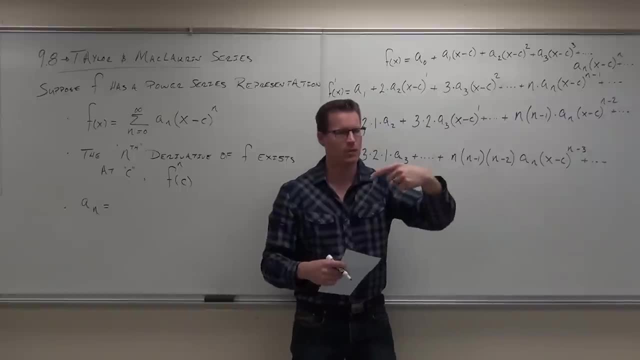 Start with 7,, multiply by 6,, multiply by 5,, multiply by 5.. Start with n, multiply by n minus 1, n minus 2, and all the way down until you get to 1.. Are you with me? 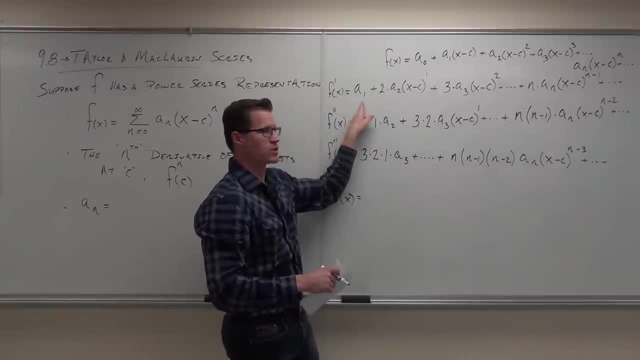 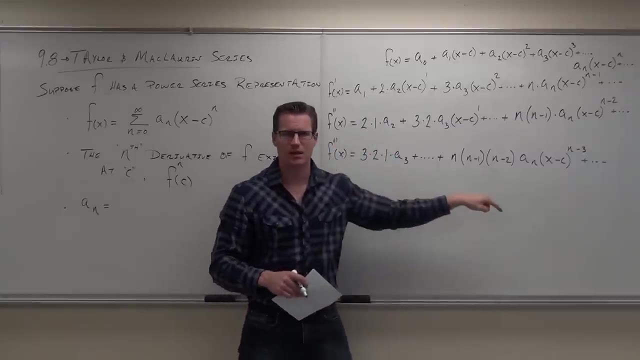 Also what's happening. I wanted you to see this. First derivative says: a sub 1 is your constant term. Second derivative: a sub 2 is your constant term. Third derivative: a sub 3 is your constant term. Nth derivative: a sub n is your constant term. 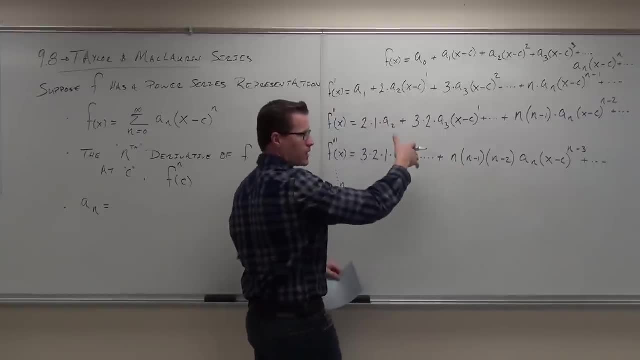 So, ultimately, what we're going to get down to is every term before it is going to go to 0.. The a sub 1 term Going to go to 0.. A sub 2 term goes to 0.. A sub 3 term goes to 0.. 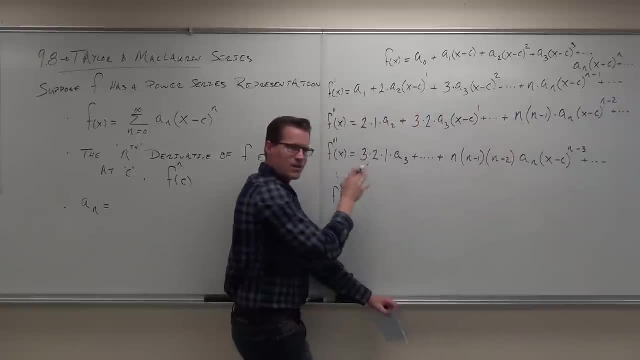 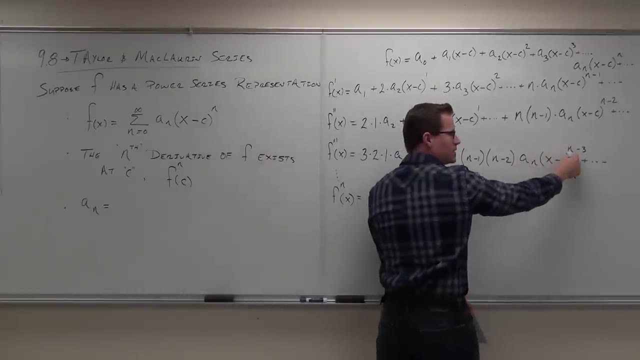 A sub n minus 1 term is going to go to 0 if we take the nth derivative. Do you get that At the nth derivative? what's going to happen here is: you've subtracted n minus n. You'll have n minus n there. 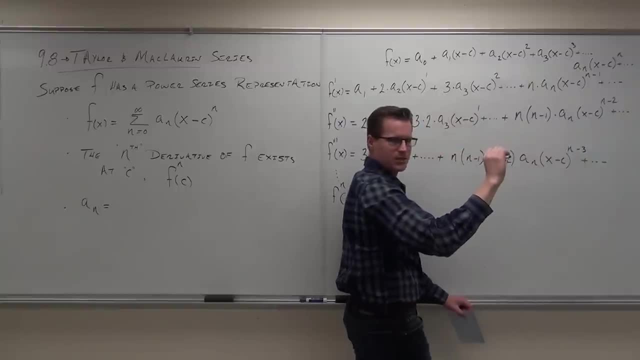 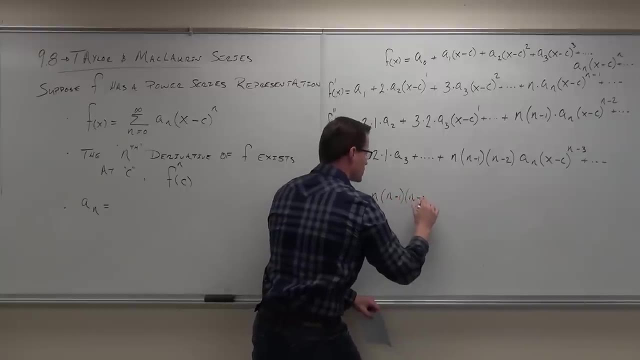 That would give you the 0. Does that make sense? So we bring it down. We have an n, Then we have an n minus 1.. Then we have an n minus 2. Then we have multiplied All of that. 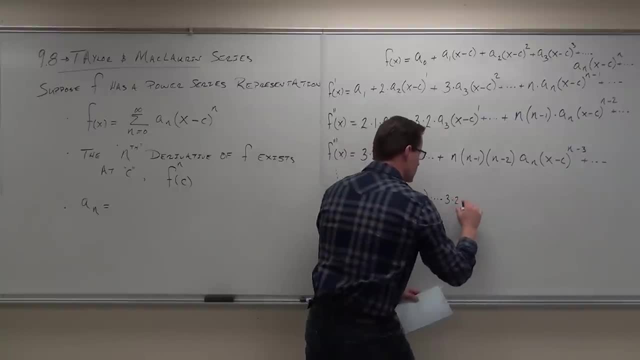 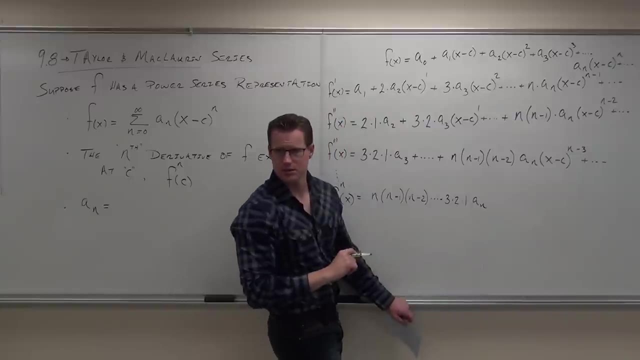 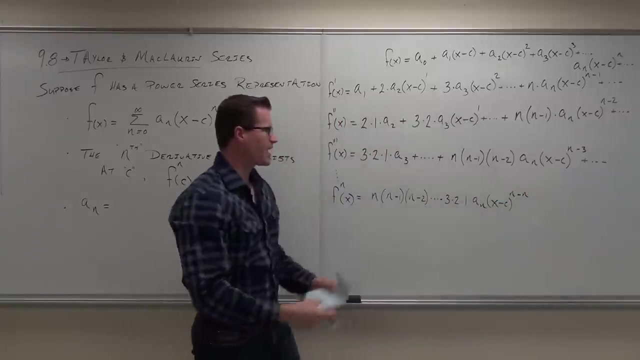 All the way down until you get 3,, 2,, 1.. And then you'd have an, a sub n. Does that make sense? Are you sure it makes sense? We would have x minus c to the n minus n, And then we'd keep on going. 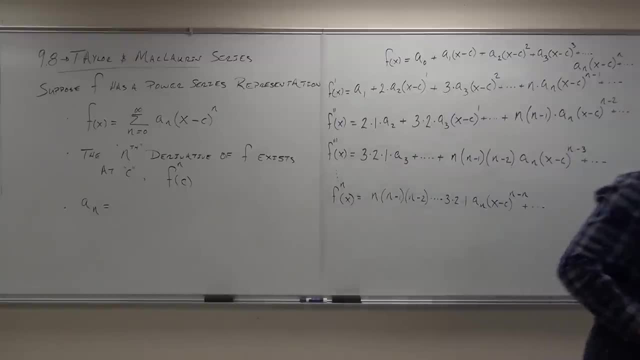 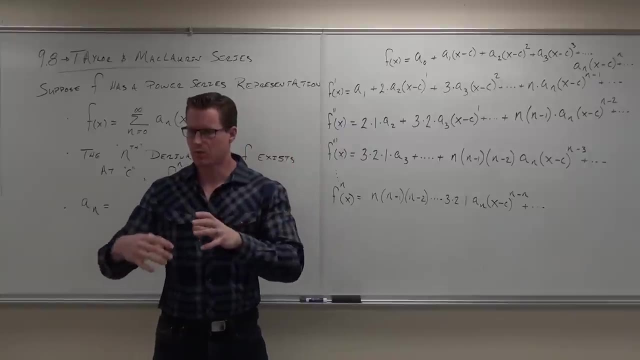 This would be a blah blah, blah, blah blah, But I want to talk about this for a bit. I'll try to have this be really stuck in your head, because this is what this is what we're going to get: our Taylor series. 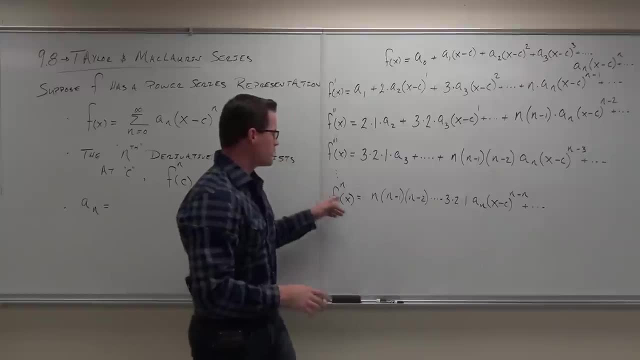 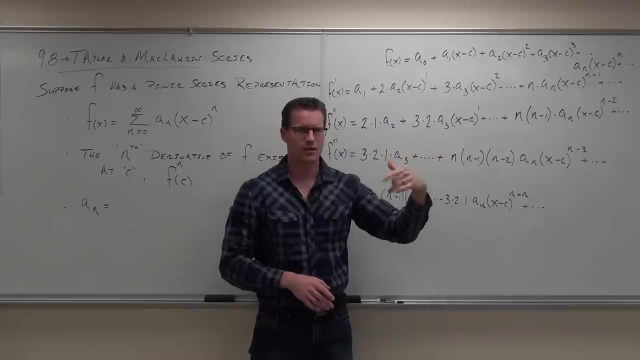 from in just a moment, okay, So bear with me for just a second. If you were to take the nth derivative of a function like this one, if you were to do that, an nth derivative means not the first, not the second. 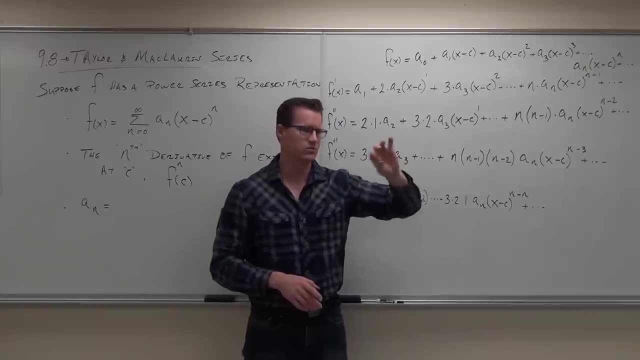 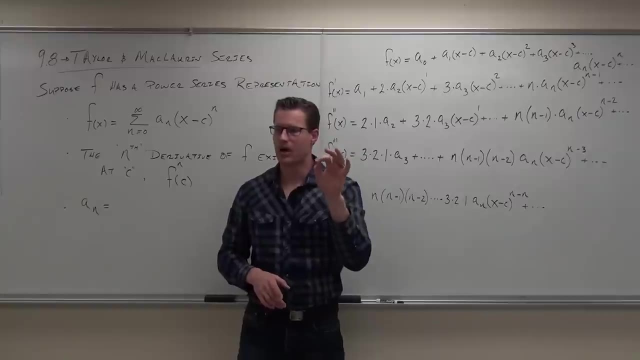 not the third, not the fourth, not the fifth, not the sixth, but do it forever. and then go up, not forever, but do it to a certain point. n What's going to happen is that every power, every term, with a power less than n. 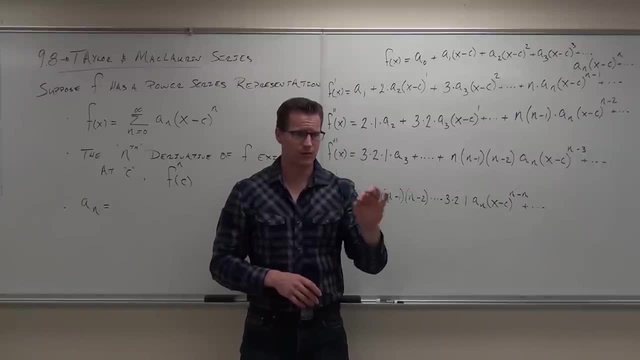 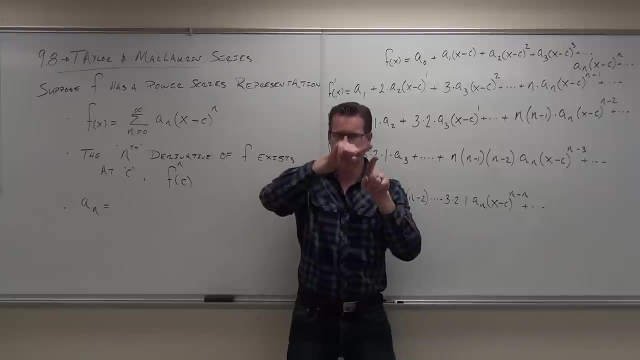 it's a polynomial that's going to go to 0.. Do you get that? Every term is going to go to 0, except for the nth term. At the nth term you will have done so many derivatives. The first thing you do is the n. 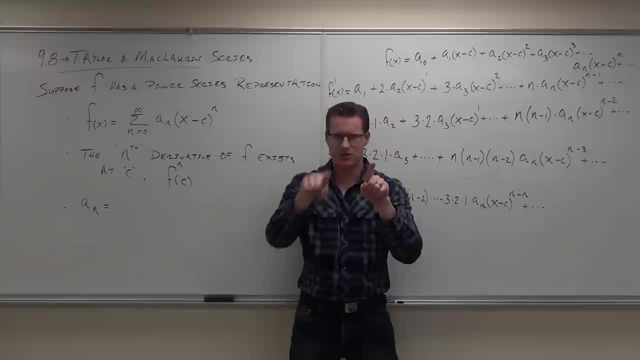 Then you multiply by n minus 1, then n minus 2, then n minus 3, all the way down until you get to 1.. Does that make sense? Now, the n minus n, that's going to give you 0.. 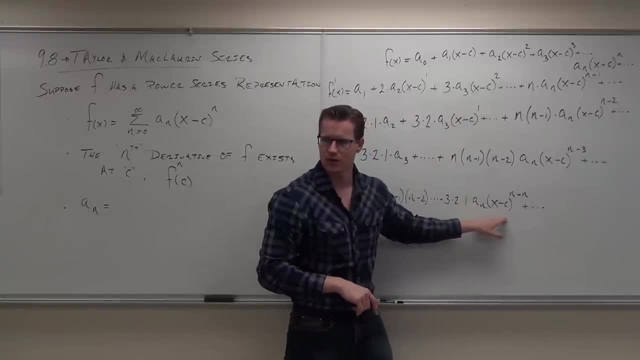 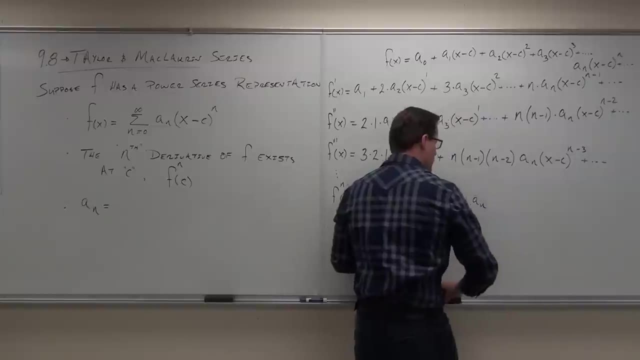 What happens to this final little piece here? Where does that go? This goes to 1.. Anything to the 0 power is 1.. So this is going to be gone. So what we know is that if I take an n. 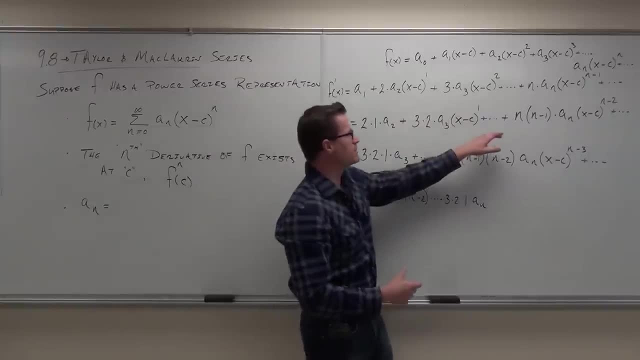 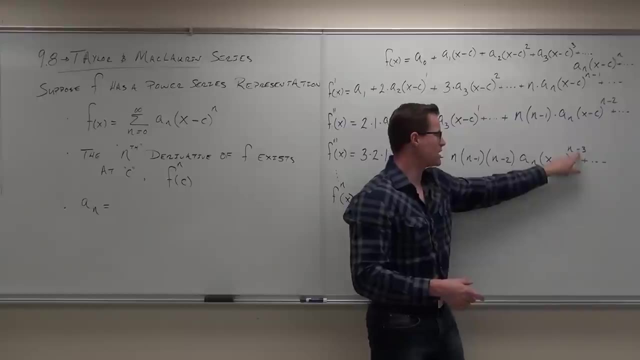 derivative. what's going to happen here is because I'm taking this down every time and saying, hey, one more derivative, I bring down the n minus 2.. Hey, look at that, One more derivative. look at this, My next derivative. I bring down the n minus 3.. 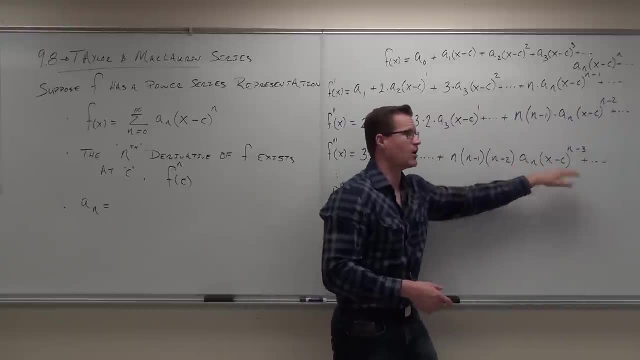 Do you get it? My next derivative: I bring down the n minus 4,, n minus 5, all the way until I get to n minus n minus 1, and that would give me my 2 and then my 1,. 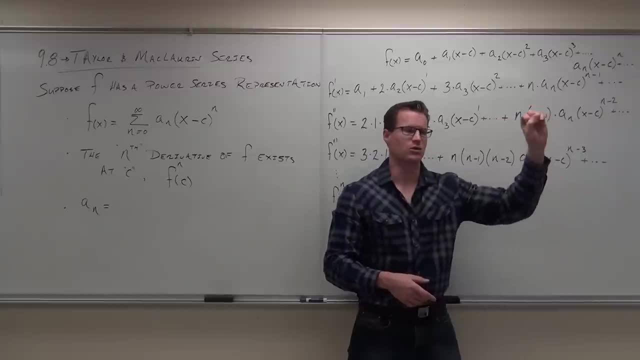 and then I'd have a sub n, but then I'd have x minus c to the 0, because at my nth derivative it'd be n minus n and my n minus n would give me 0. Anything to the 0.. 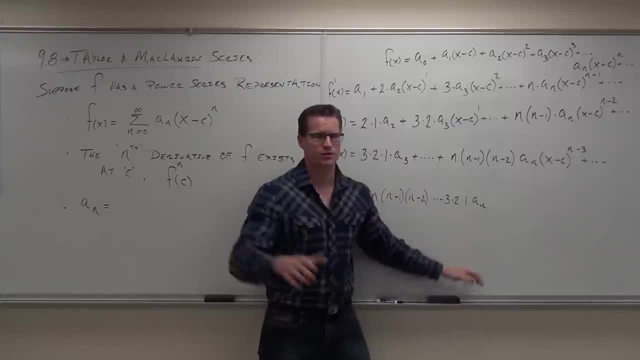 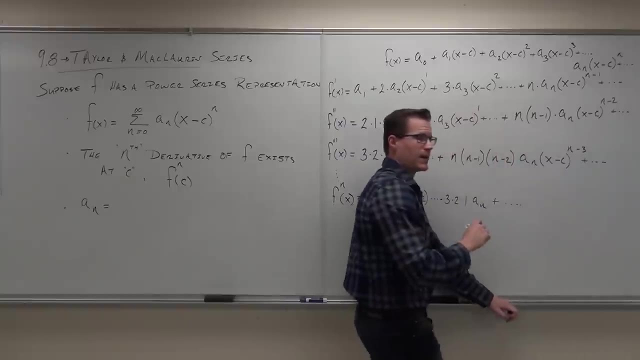 Anything to the 0 power gives me 1.. This would be my very first term, So if you guys feel okay with that, Now this doesn't stop. but when I keep going every term past, this is going to have some bunch of crap. 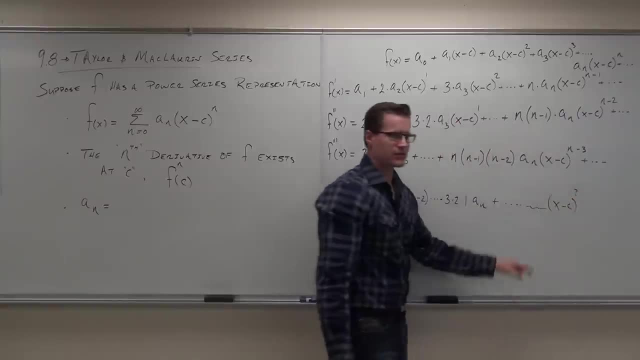 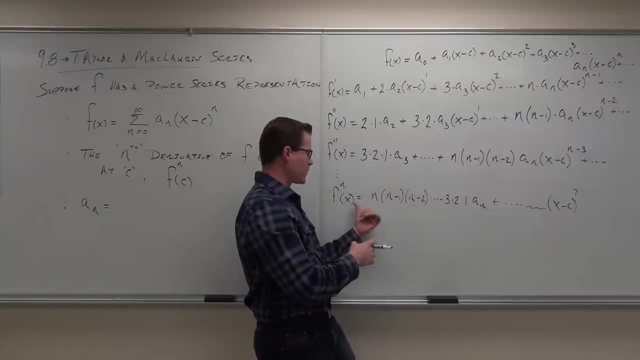 x minus c to some power. That's very unmathematical, but I'm trying to get you the idea here. Does that make sense to you, Are you sure? So my nth derivative, my very first term, is going to be n times all this junk, and then a sub n. 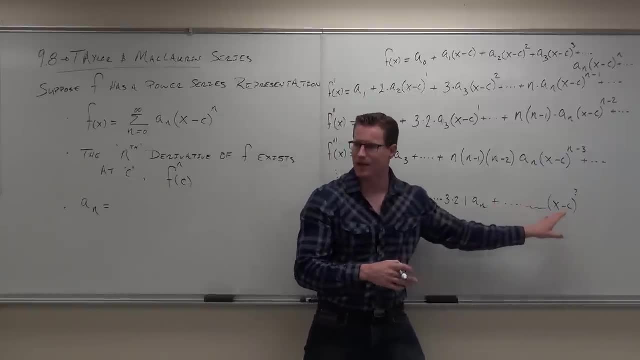 with no x minus 3.. So I'm going to have x minus c, but every term after that is going to have an x minus c. Do you understand why this does not have an x minus c? Yes, Do you understand what all these ones do? 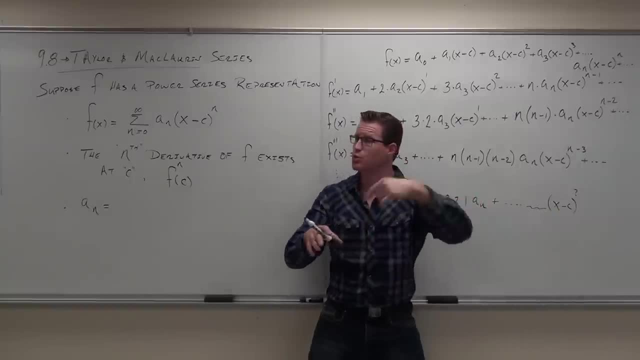 Anything past the nth term is going to have an x minus 1 to 1 more power. So when I take an nth derivative, I still have a power there. that's not 0.. Does that make sense? Now let's write this better. 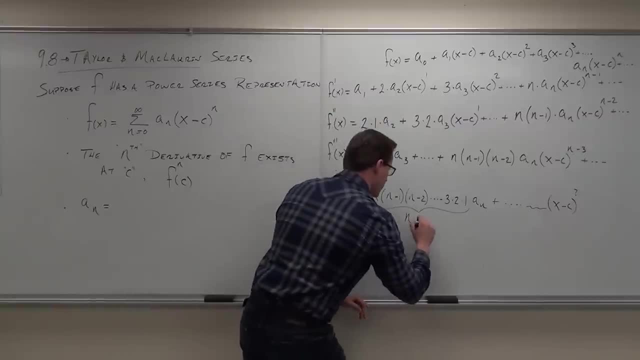 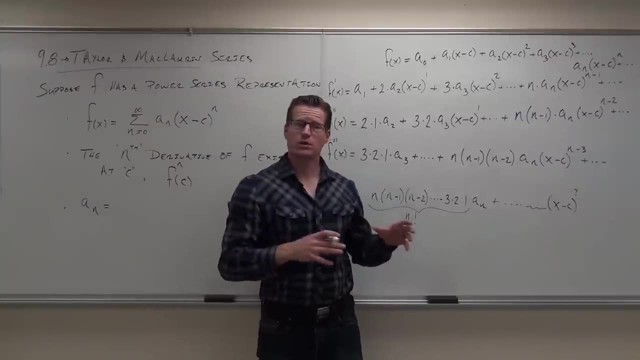 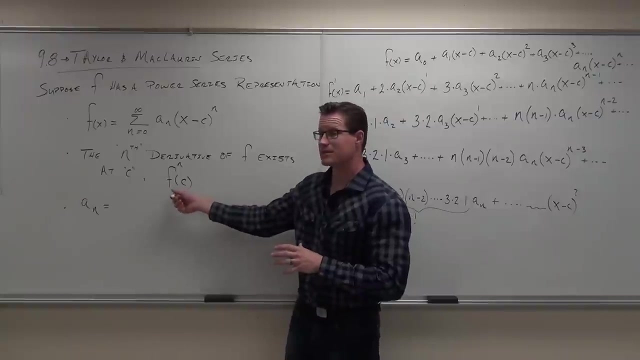 What is all that Number? Number Very good. Now what I get is what I care about, what I don't care about. I don't care about f, the nth derivative of f at the x. What I want to do is this, at c: 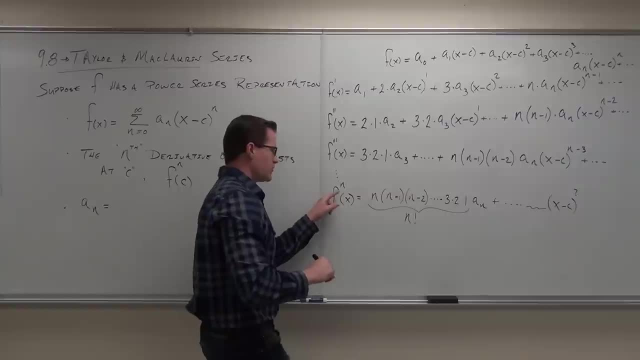 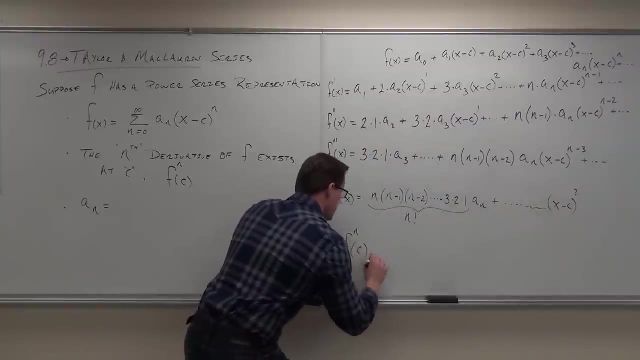 So we're going to make one little jump. If this is true, if the nth derivative of f of x is all this junk, then if I want to find the nth derivative of f at c, let's think about what's going to happen. 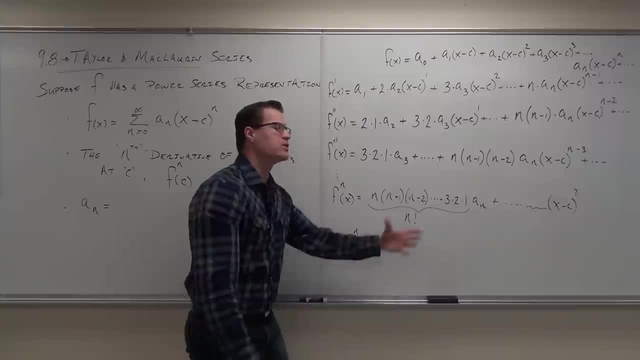 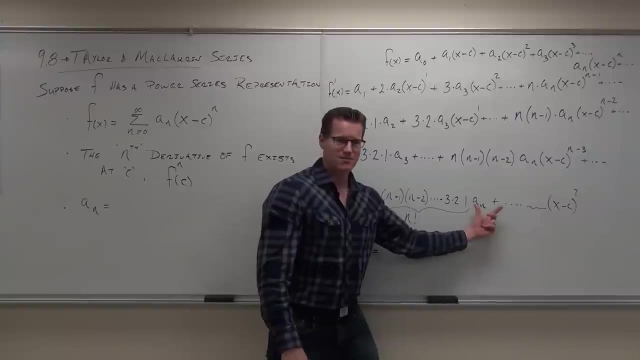 Please bear in mind. this is why I just asked the question. do you understand that there's no x minus n here? Or, sorry, x minus, what is that? C, C, C. There's no x minus c here, but every other term is going to have an x minus c. 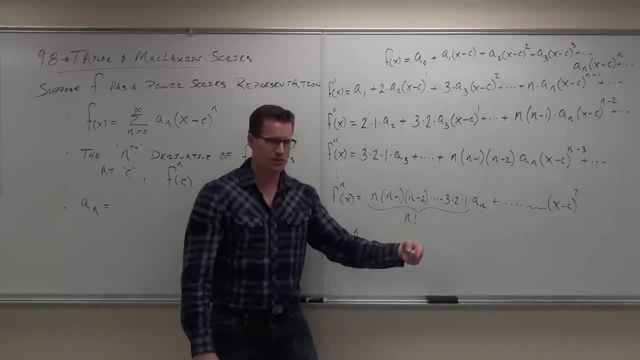 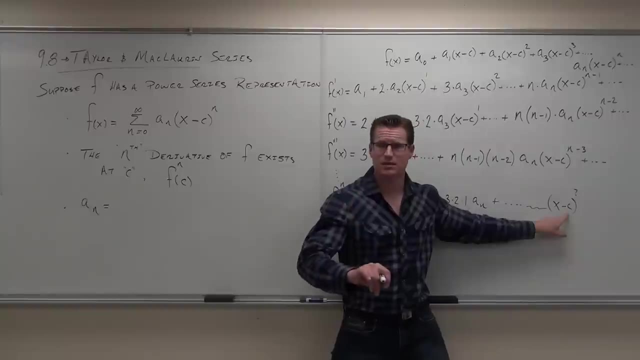 Do you get that? Yes, Do you understand that f of c means I plug in c for x? Yeah, So if every one of these terms has an x minus c with it and I plug in c for my x, what's c minus c? 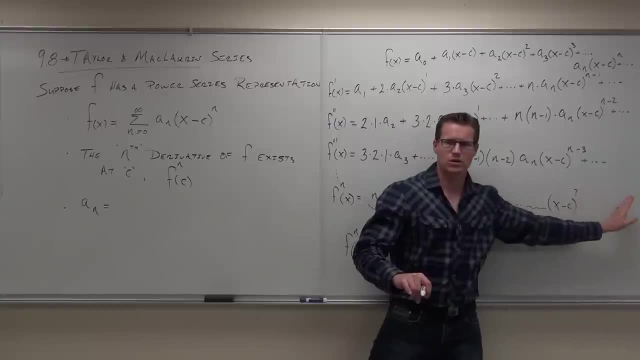 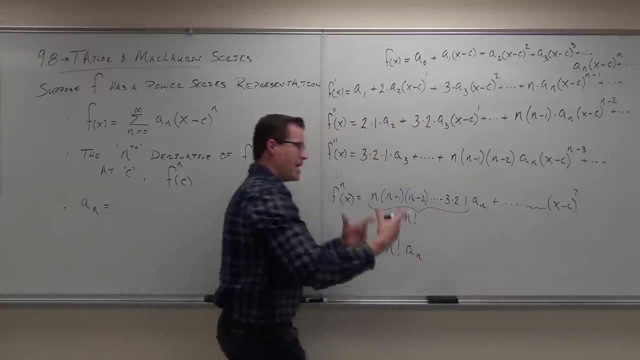 Zero. Everything else is going to go to Zero, Zero, And the only thing I'm left with is this guy And that's Zero, And that's a factorial times a to the n and that's it. Did that make sense to you? 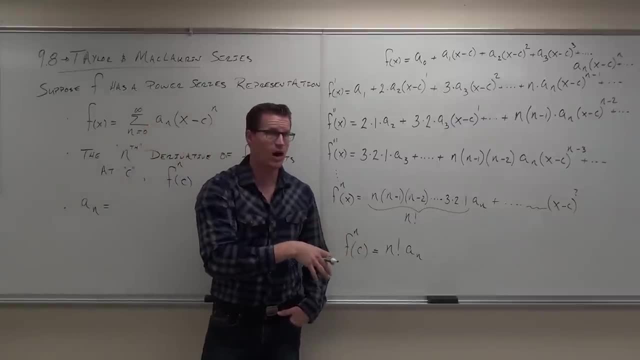 It's kind of weird, right, But this is the idea. Now here's what's awesome about this. Can you solve for a to the n Very easily? This is where we're going to make the jump, so I hope you caught on to this. 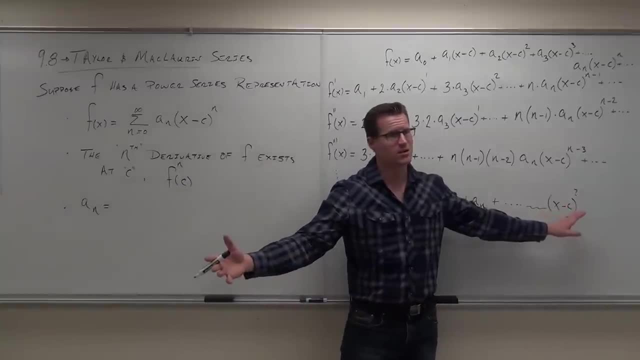 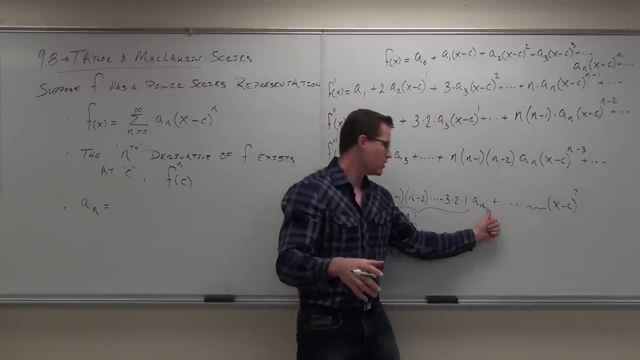 If every other term has x minus c, when I plug in c, c minus c is zero. all these things are gone. This does not have any x's at all, It's just a constant. This is the first constant. When I plug in c, everything else is gone except for that constant. 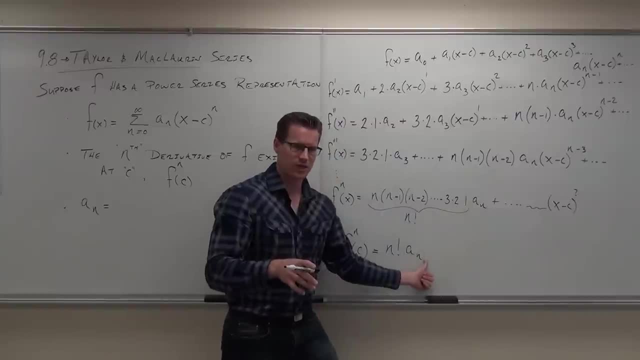 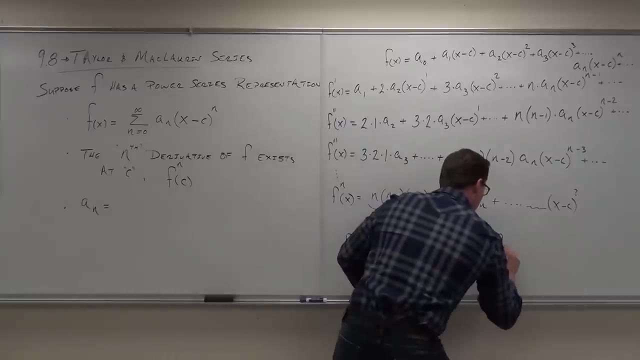 This is n factorial. This is still a sub n. Let's solve for a sub n. If I solve for a sub n, I get a sub n equals. let's just divide both sides. f, the nth root of f, at c. 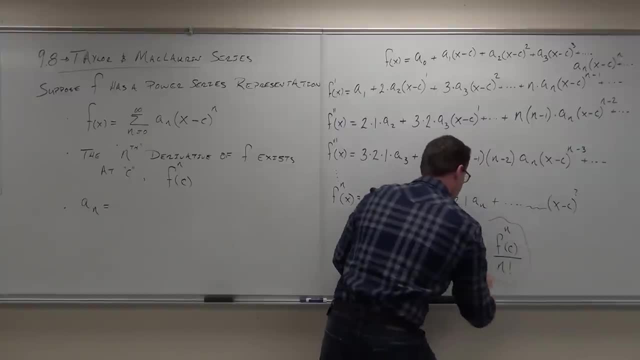 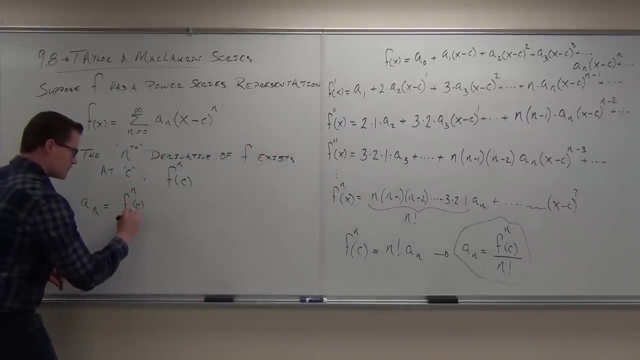 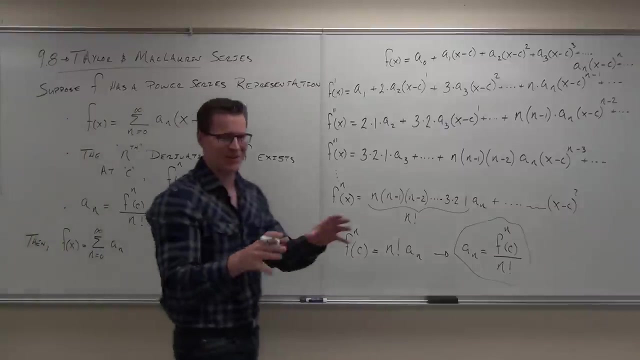 divided by n factorial. That, ladies and gentlemen, is what I was looking for over here. Well, what that means is that, if I have just solved for the a sub n term, this is really kind of a neat idea. Do you understand that? this is all in general, right? 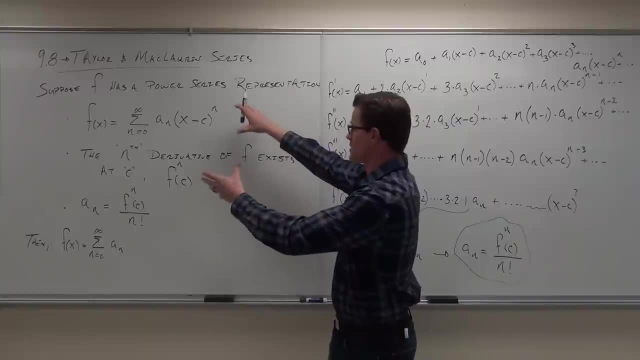 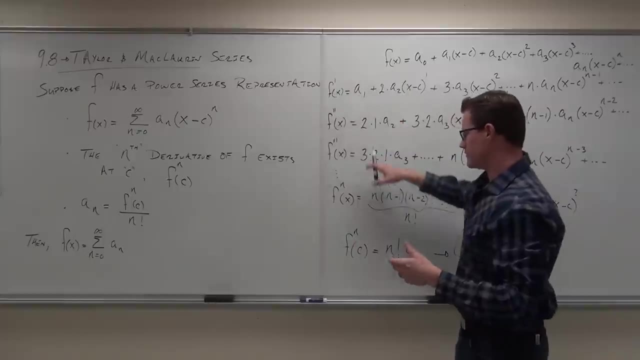 I make no specific case about this whatsoever. I said, if this has a power series representation, we have this. We can take derivatives. We can take derivatives of it, no problem, Of course we can. Let's do derivatives. This right here would be the nth derivative of f at x. 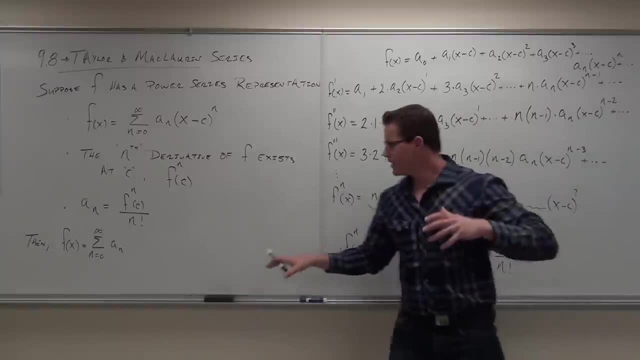 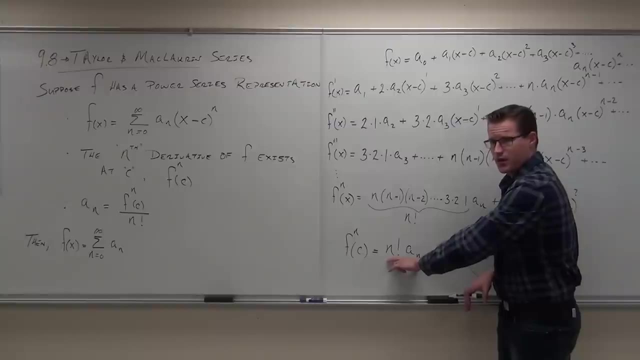 If I plug in c- which, wherever my power series is centered, I can do that- If I plug in c, everything's going to disappear, except for this very last term. This very last term, It has a sub n in it. So if I want to solve for a sub n, I just divide. 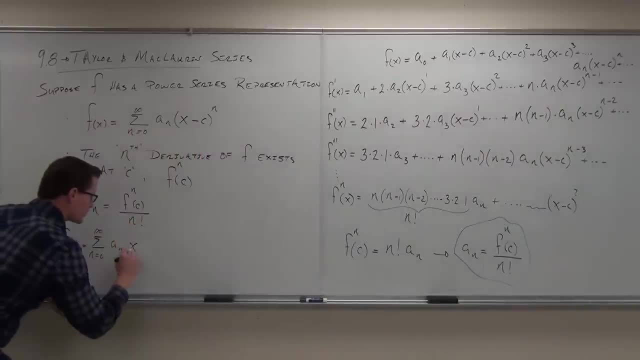 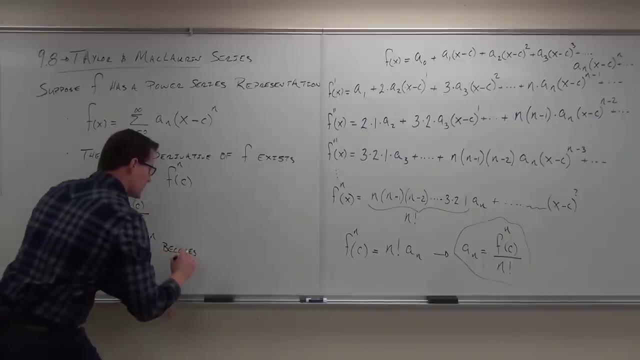 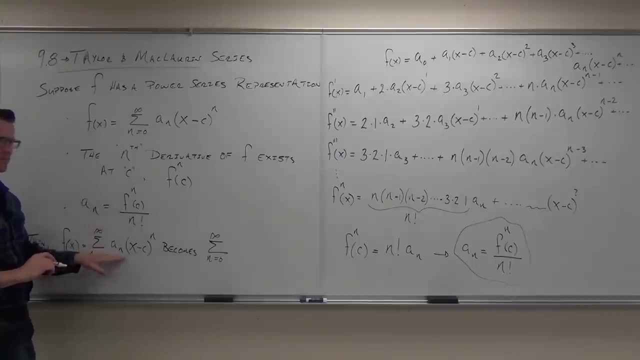 What that means is that what we can do is change this power series. It becomes this power series. Why don't you tell me, Instead of having a sub n here, what am I going to put? What am I going to put f of f and cd? 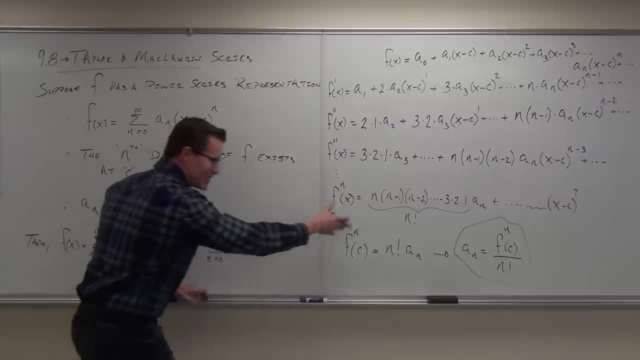 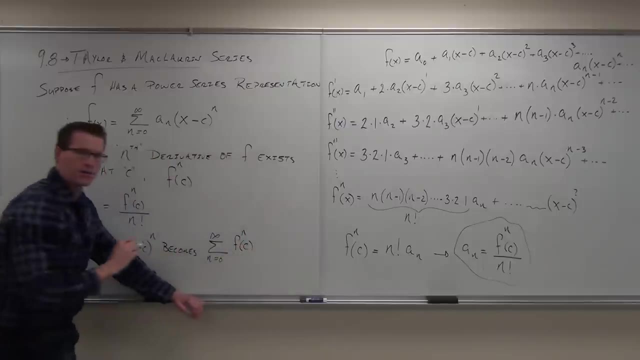 The nth derivative of f at c. It's hard to, it looks weird, It's weird to say, but the nth derivative of f at c, The nth derivative of f at c. And then what? Over n factorial, Over n factorial. 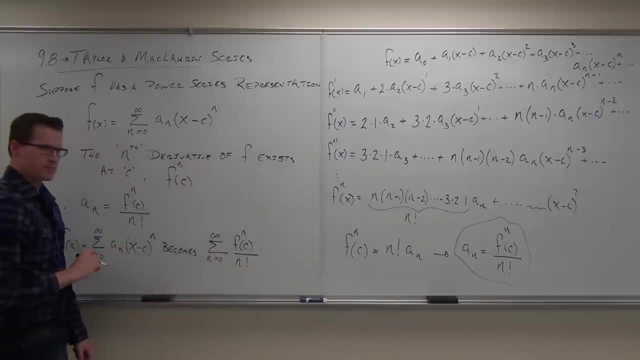 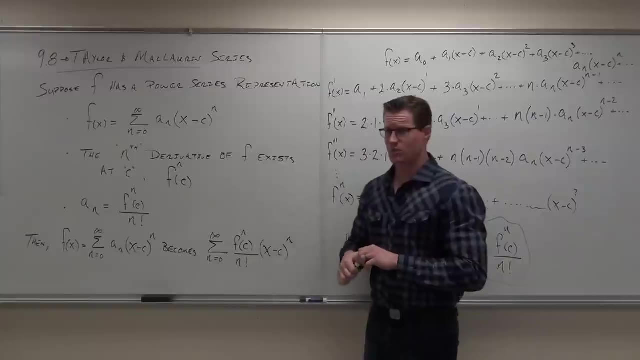 Very good. And then what? 10 to the nth, 10 to the nth, 10 to the c to the n? Okay, I want to make sure that if there's any questions, I answer them right now. Do you all see what I'm talking about? 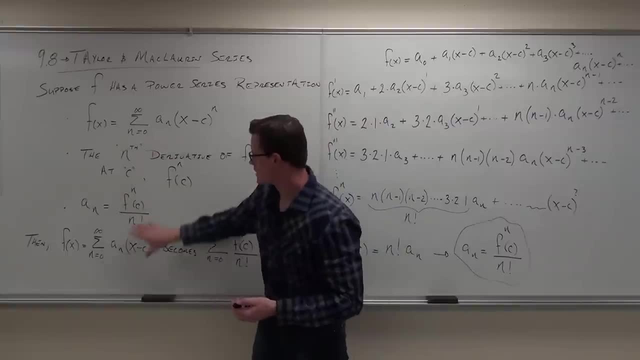 Do you see that what this thing becomes, this is the same. okay, What this thing becomes is: if I know this is true, which I just proved it that it is- If I know this is true, instead of a sub n, I can have the nth derivative of f at c divided by n- factorial. 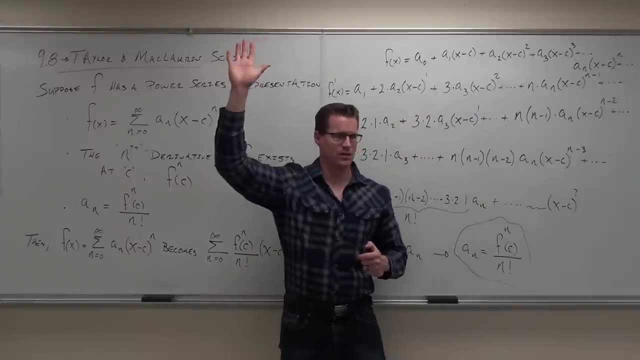 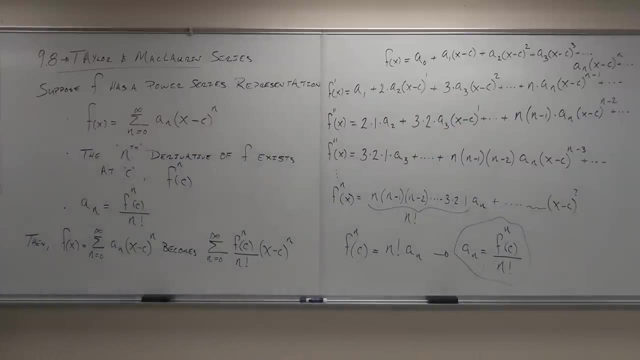 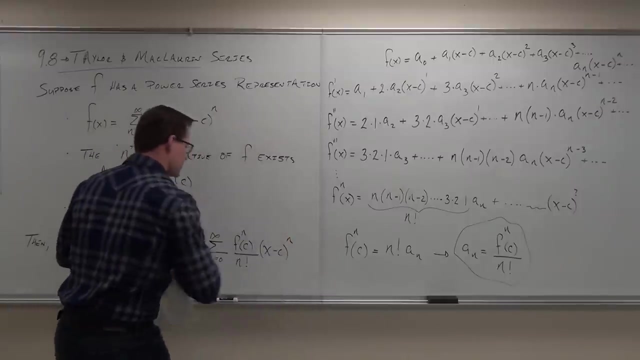 And that is what goes right there. It depends if that one made it. It doesn't make a little bit of sense to you. Okay, What this is is a Taylor series. This right here is the Taylor series. Any questions on this at all? 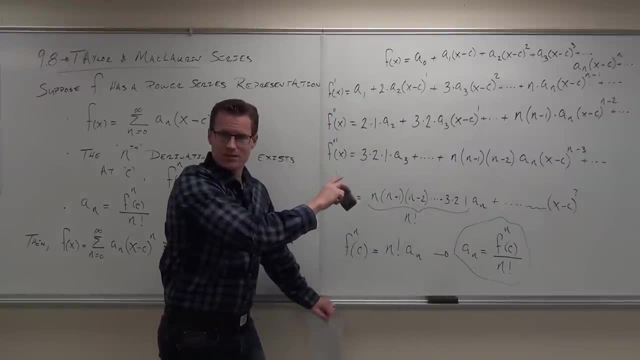 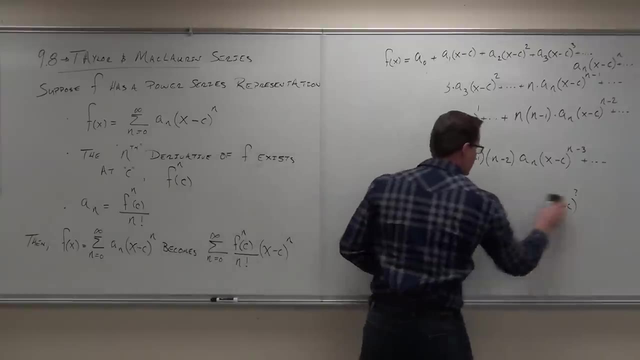 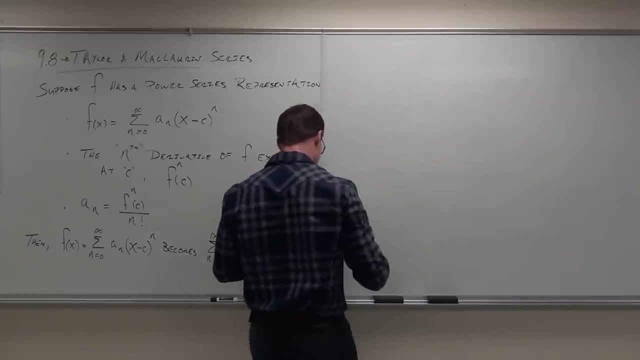 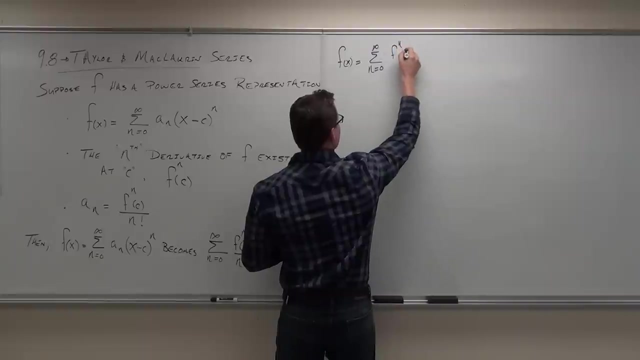 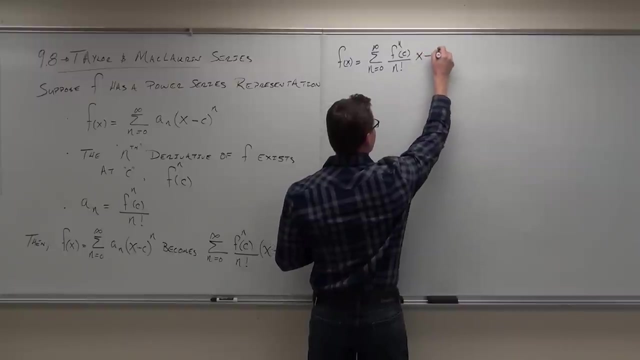 Because I'm going to erase this whole side. You sure Did it make sense to you. Some basic derivatives, Maybe not so basic, Okay, So this thing, this series from 0 to infinity of the nth derivative of f at c, over n, factorial minus, n minus, sometimes x minus c to the n. 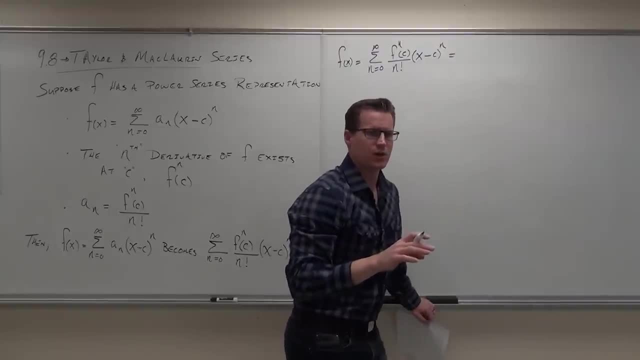 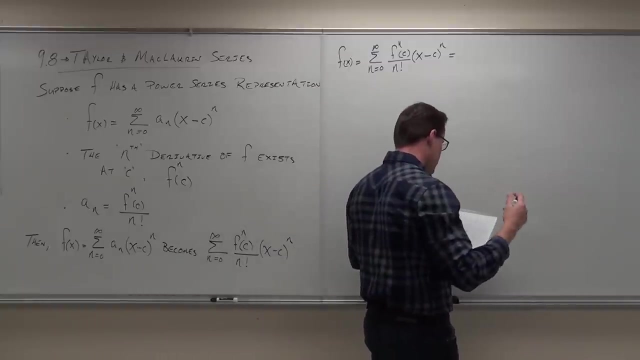 Let's look at how this would look. okay, Just like the first few terms. What's the first term? Let's plug what would you plug in to find the first term: Plug in 0.. Okay, So if you plugged in 0. 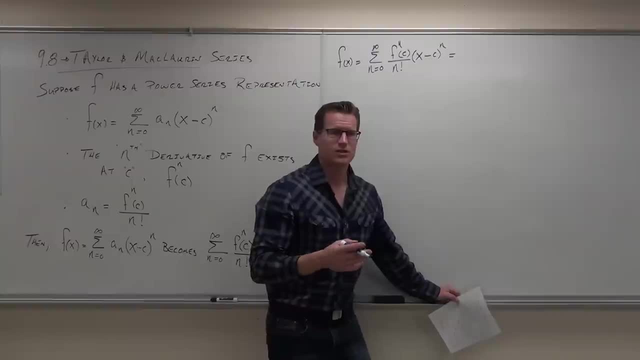 What is f to the 0?? It's not f to the 0. It's the. you don't take a derivative of f, yet You don't have it. You take 0 derivatives. That's what that little n means. Okay. 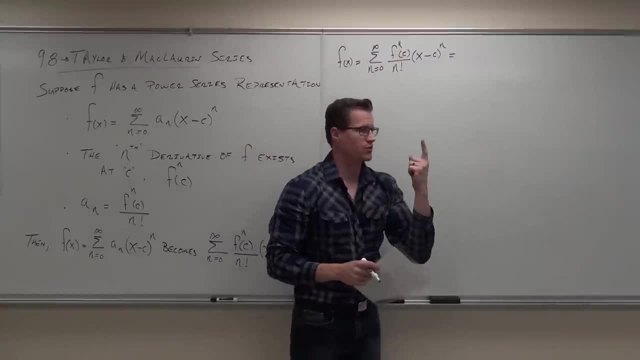 So you plug in 0. It means, if that was a 1, you take the first derivative. If that was a 2, you take the second derivative. If that's a 0, you don't take the derivative. Does that make sense? 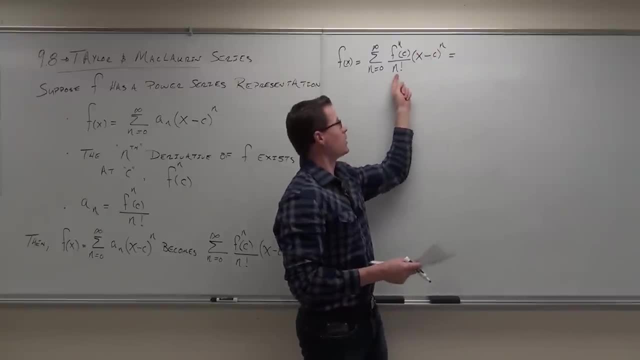 x minus c to the, what would that become? 0.. That would be 1.. All over: 0 factorial: 0 factorial. If you don't remember, it's defined as 1.. So this would simply be f of c. 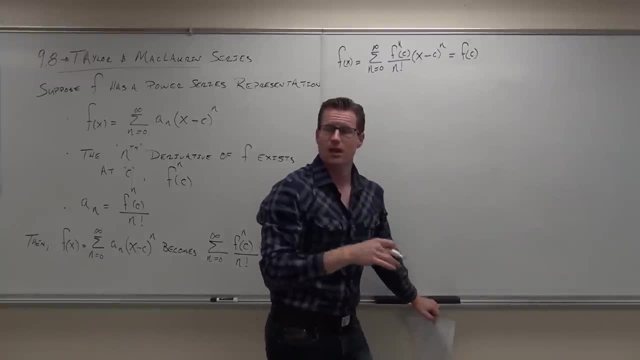 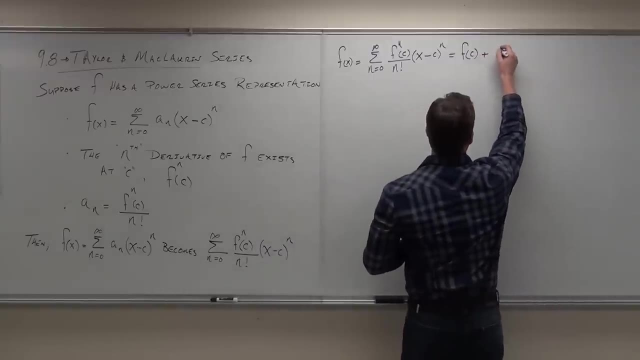 You don't take the derivative of f, You plug in c. That's the very first term here. Does that make sense to you? The next term says: okay, add to it now. Now take the first derivative, plug in c. have x minus c to the first power, all over 1 factorial. 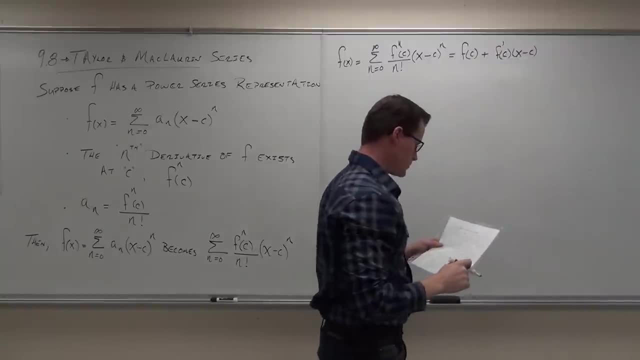 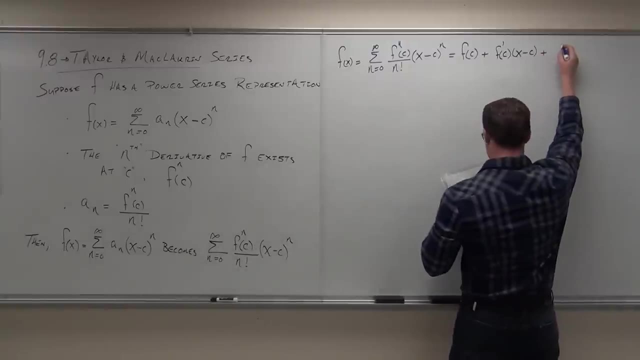 We don't need that 1 factorial, It's just 1.. Does that make sense to you? Make sure I'm going to do one more term and see if you can hang with me. Plus what's the next one? Take two derivatives. 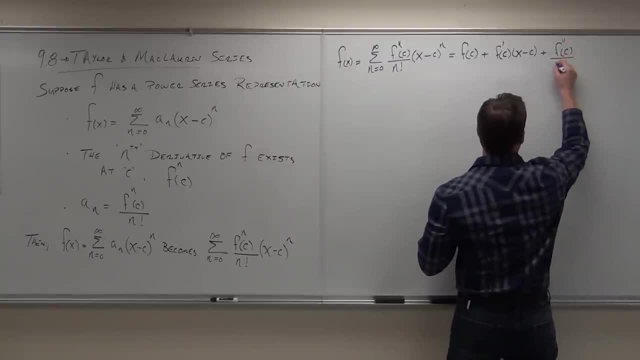 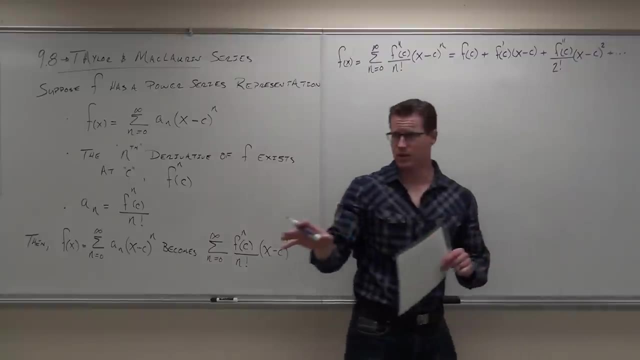 Plug in c. Divide by 2. factorial multiply by x minus c to the. do you see the pattern? Are you all okay with that pattern? for sure, for real, Yes, no, Yes, This series. did you guys see that we get a series? 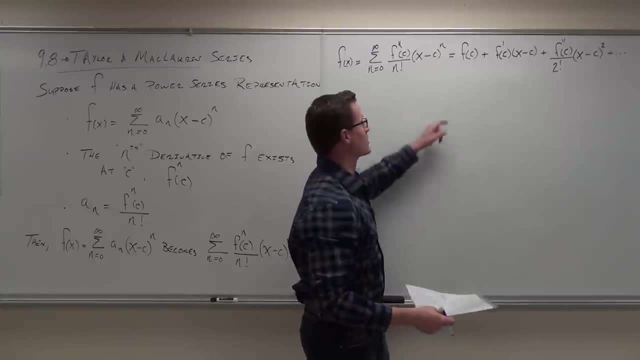 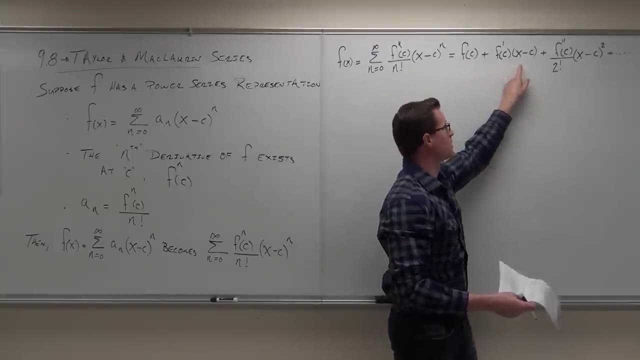 Seriously, do you see that we get a series. We get a series here. We get: hey, take the function plug in c, No problem. Take the first derivative plug in c. Okay, no problem. Multiply by x minus c to the first. 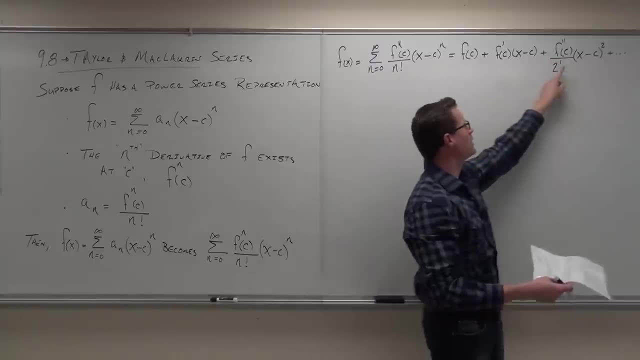 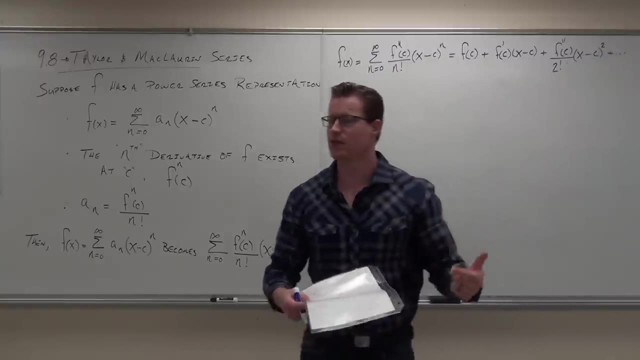 Take the second derivative plug in: c Divide by 2 factorial- That's where this is coming from- times x minus c to the second power. That's how your factorial and your power always match up. You keep on going, going and going and going and going for infinity. 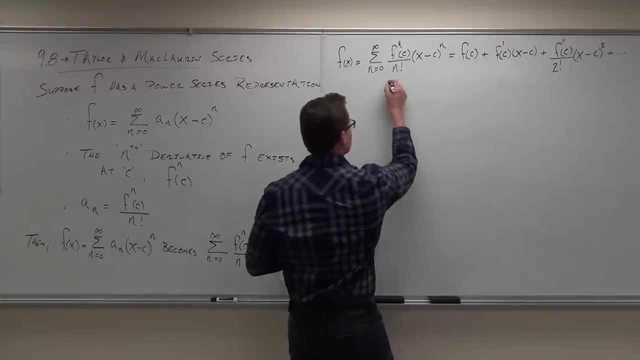 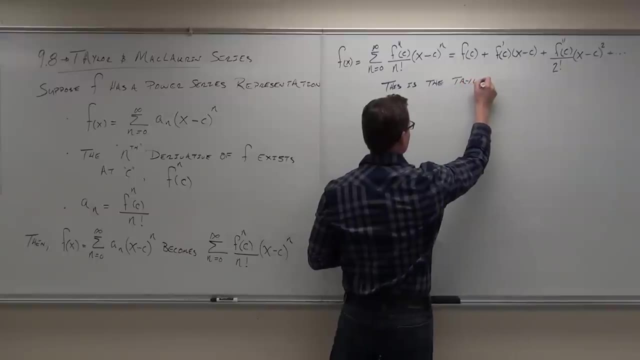 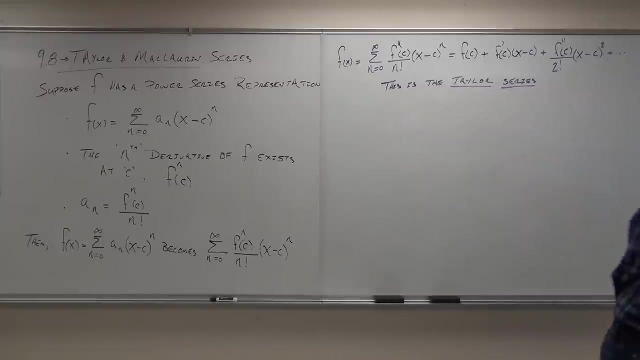 This right here. this is called the Taylor series. Now it's going to be a real pain in the rear, but we're going to go ahead and do the McClure series right now. okay, It's a lot of work, Okay. 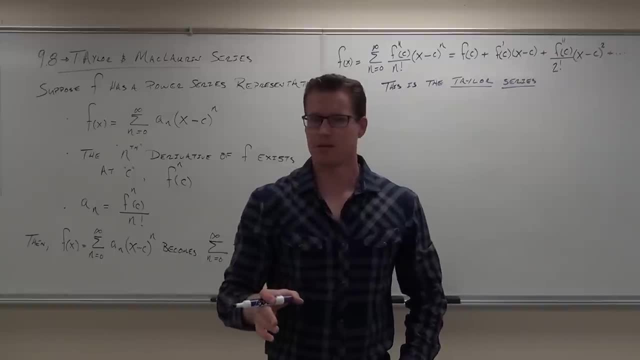 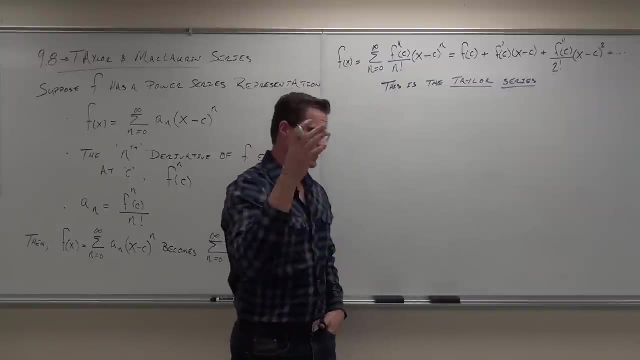 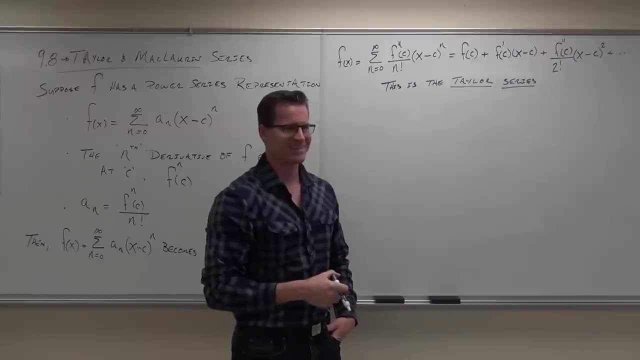 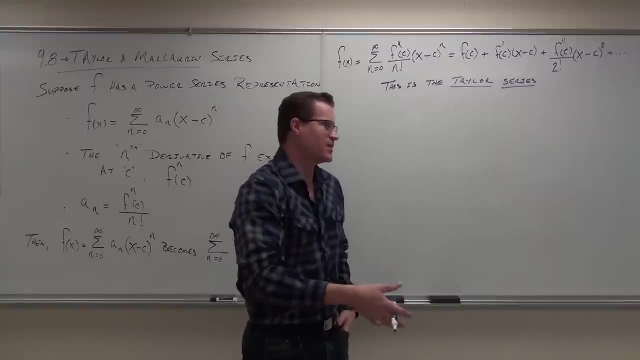 Super hard: 30 seconds, But it's a harder one. It's going to take about 30.. There's always a catch, There's no catch. It's easy, It's not easy. I mean, it's the same thing. 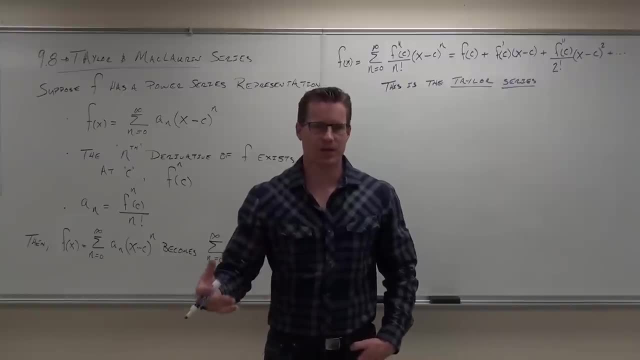 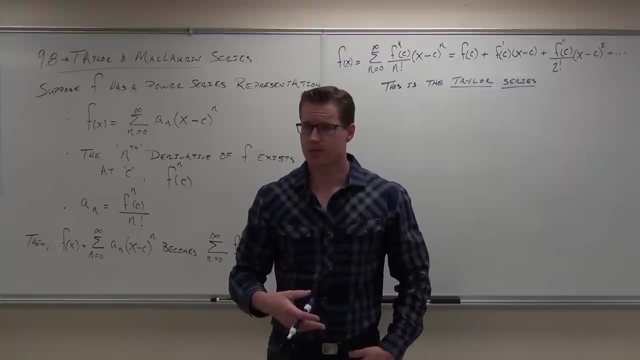 Listen, do you know how? like every square is a rectangle, but not every rectangle is a square. Yeah, It's kind of like that. Okay, that's analogous to what we're doing here. Every Maclaurin series is inherently a Taylor series. 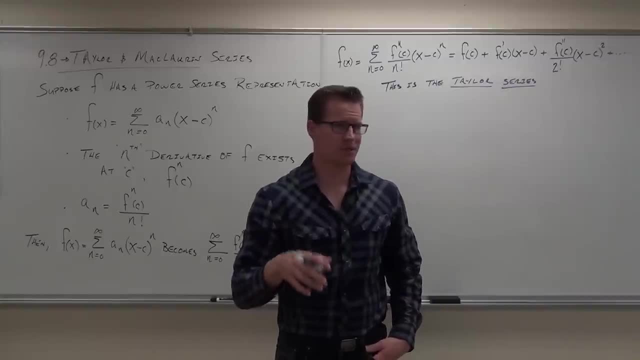 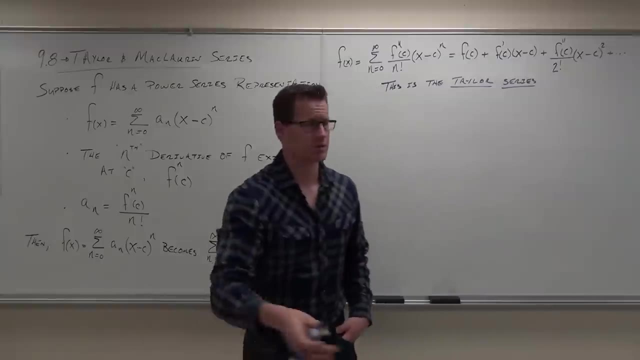 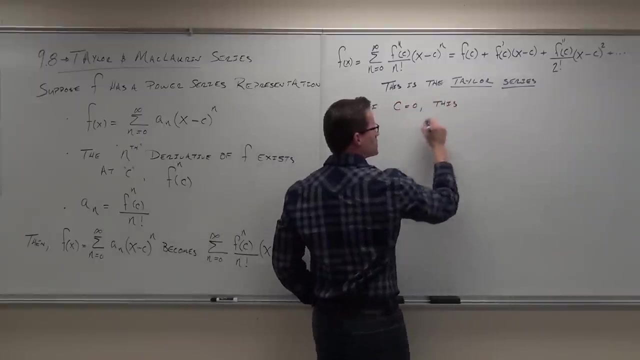 Every Taylor series is not a Maclaurin series. A Maclaurin series is simply a Taylor series. with C equals 0. You with me. So if C equals 0, you have yourself a Maclaurin series. If C equals 0, this becomes the Maclaurin series. 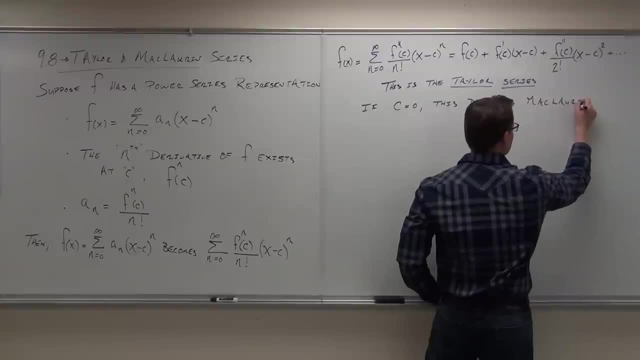 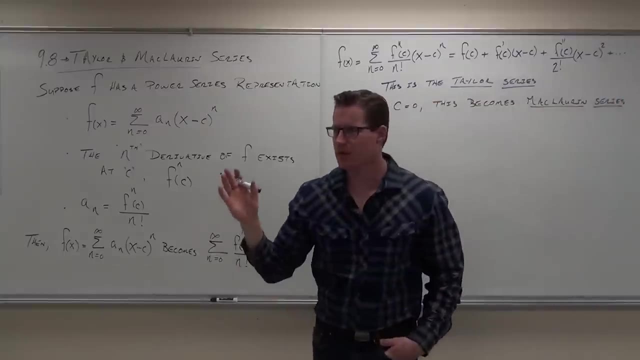 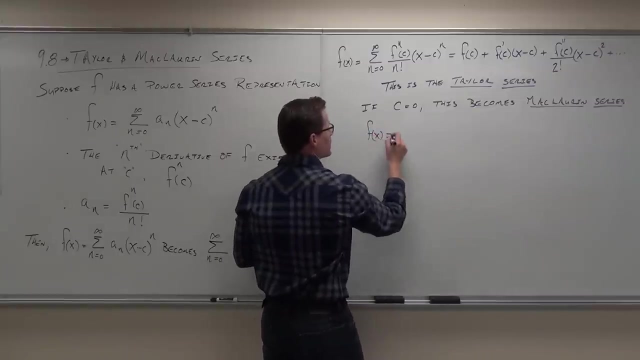 Are they different? No, You do exactly the same thing. it's just C is 0.. Well, it makes it a little bit nicer. Our notation becomes nicer. So F of X would now become for a Maclaurin series. 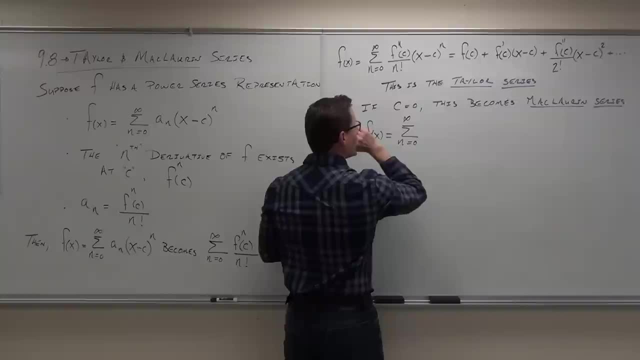 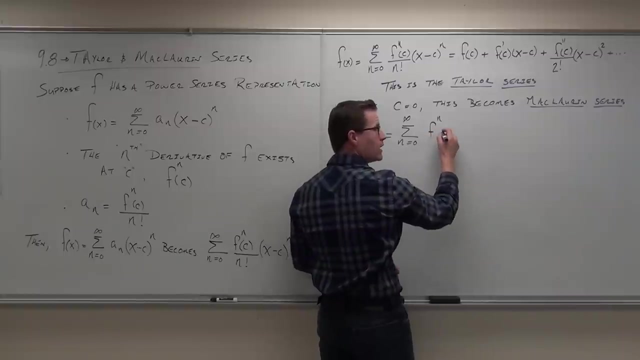 a series from N equals 0 to infinity. It would just be this. It would be the Nth derivative. Notice how the N does not become 0. It's the C. It's the C that becomes 0. So what it becomes is F, the derivative of F. at what? 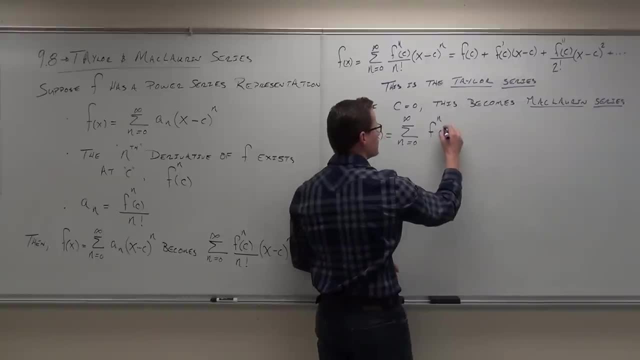 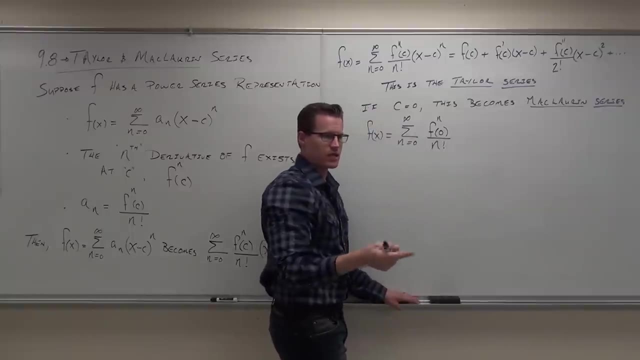 Zero, Zero. That's a Maclaurin series All over N factorial. And then what happens here? X minus Zero, So we just have X to the N. Do you see how it cleans it up a little bit? 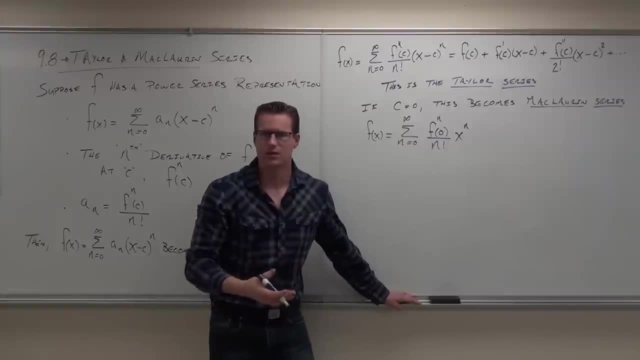 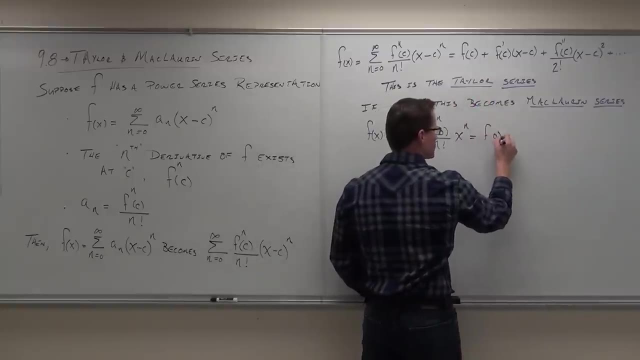 A little bit nicer looking, Because you don't have that minus C, You don't have the C, You just have 0 because we're putting the 0.. It's going to look exactly the same. It's going to be. It's going to be F of 0.. 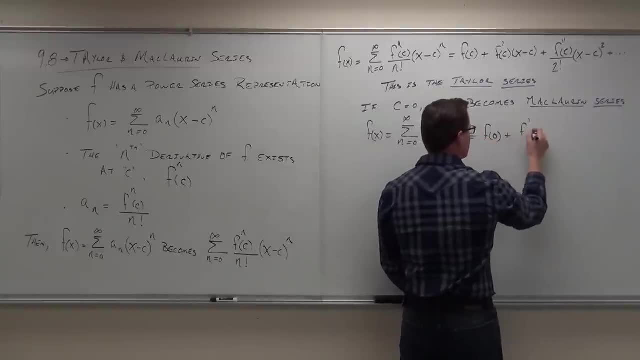 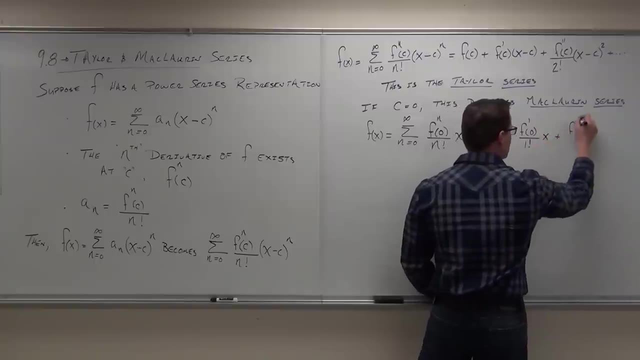 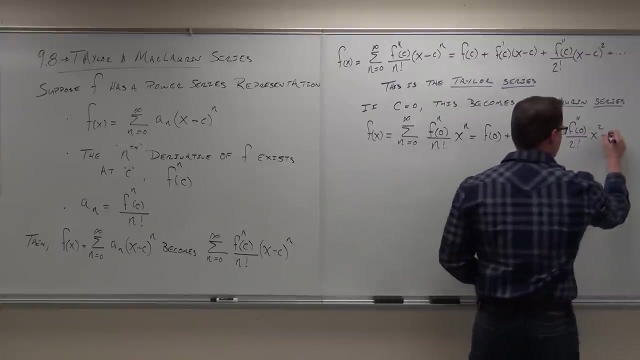 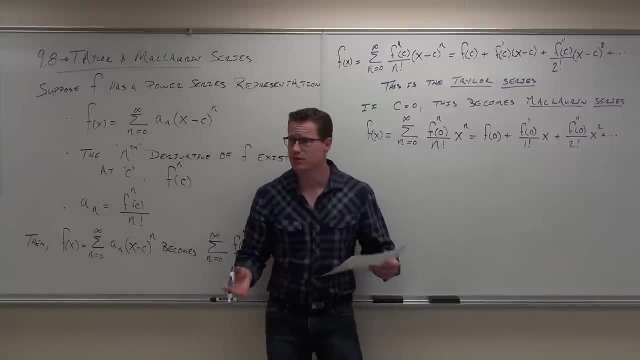 Okay, quick show of hands. if you understand the notation and the verbiage, the idea of the Maclaurin series and the idea of the Taylor series and how they differ, Do you understand how they differ? Yes, So on a test, when I ask you for hey, find the Maclaurin series. 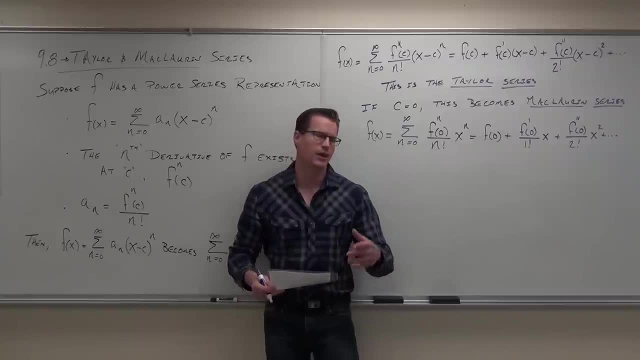 that represents this function. would you be able to do it? Well, not right now, Not right now, But would you understand what I'm talking about? Yeah, It's a Taylor series with C equals Zero Done. Now here's a couple. I'm not going to write these down. 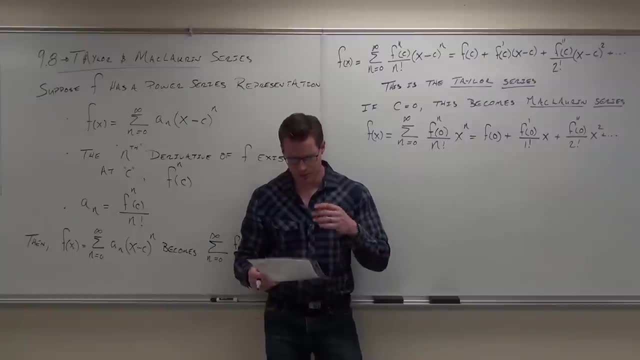 but a couple of pieces of information that are quite important. Firstly, a function that has a power series representation will be Represented by a Taylor series. It will be represented by a Taylor series. The converse is not necessarily true, but we kind of assume it to be true. 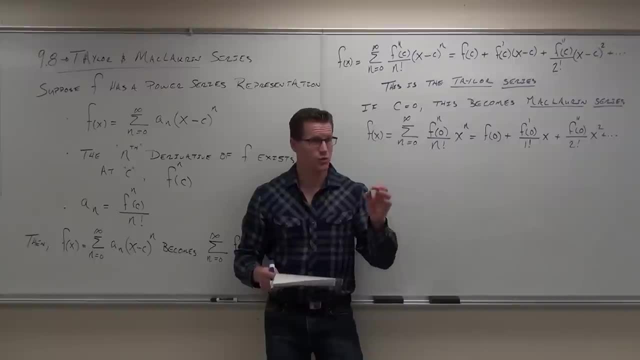 If we find a Taylor series based on the derivatives of some function, that function that we get from that series usually represents our function very well. We assume that to be true for this case. There are cases where it doesn't, but we assume it to be true for us. Does that make sense? So what that means is that if you've got a function that's not represented by a Taylor series, it's not represented by a Taylor series. It's represented by a Taylor series. It's represented by a Taylor series. 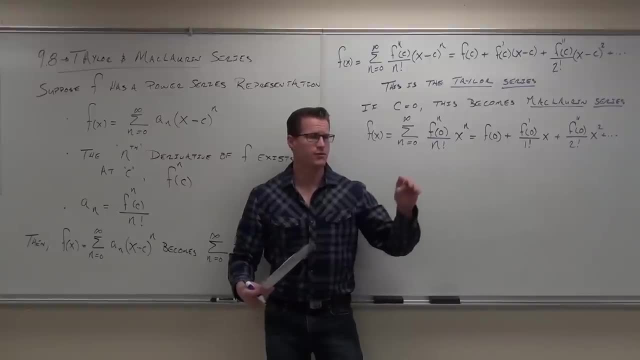 If you've got a function and you represent it with a power series, it's going to be a Taylor series. If you find some Taylor series, a function that you didn't know, that series that you get usually represents the function If you base it on the derivatives of the function that you're looking for. 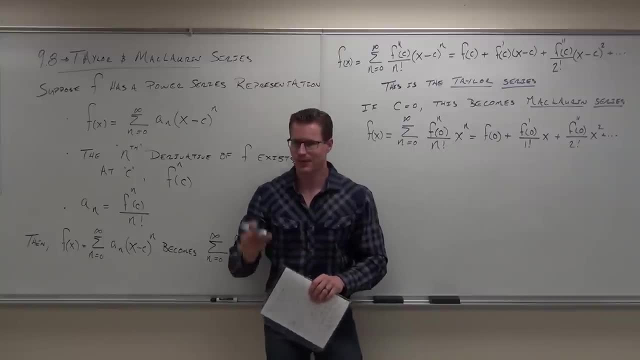 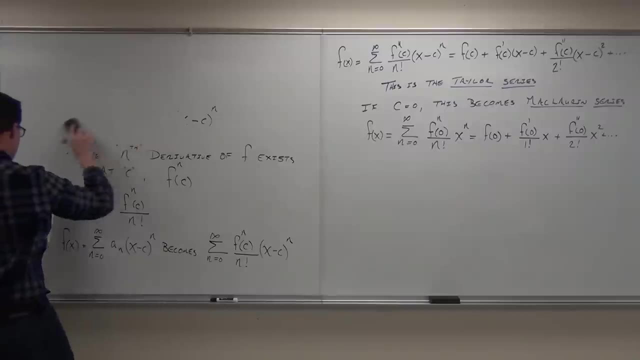 That's what I'm trying to say. Can we please do an example to clear all this stuff up? Yes, I'd like you to do at least two of them. The first one's really quick, really nice and easy. So here's how your question on a test will motivate you. 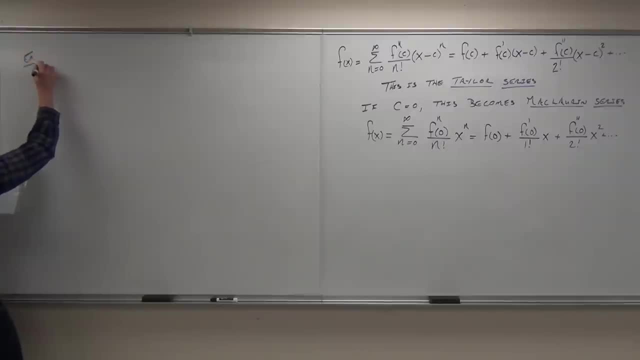 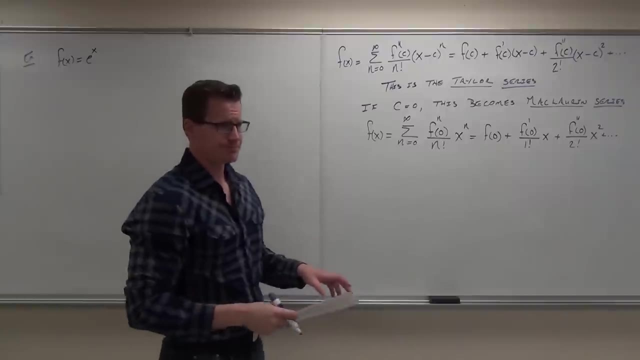 Most likely look. no matter what class you're ever taking calculus, this is typically how it looks. So if we have a function like this and I say what I want you to do, I want you to find the Taylor series that represents this function at a certain point. 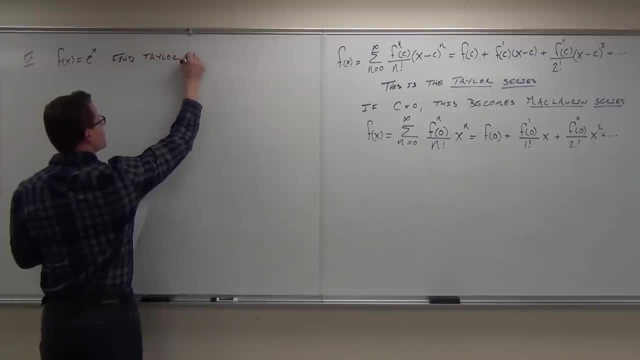 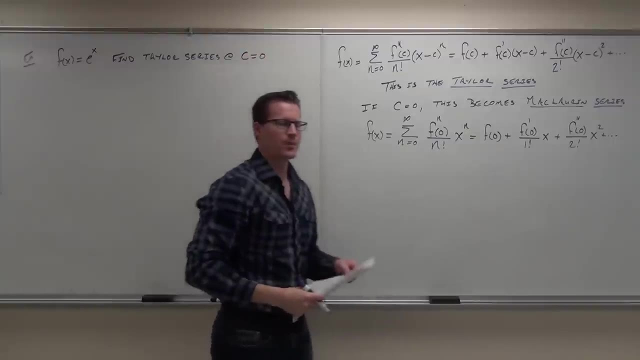 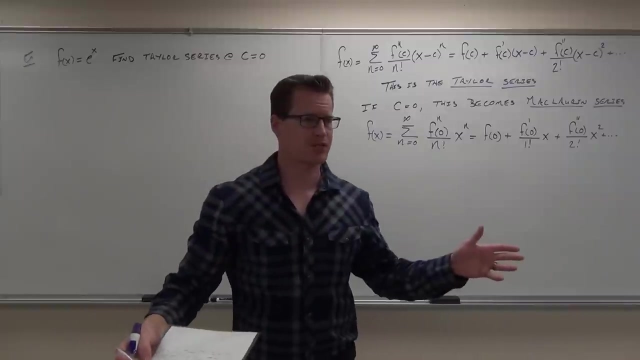 Find the Taylor series that represents this function at the point c equals zero. Can you please explain to me another way that I could have worded this? that would mean the same thing: Find the Maclaurin series. Bam, Do I have to say find the Maclaurin series at c equals zero? 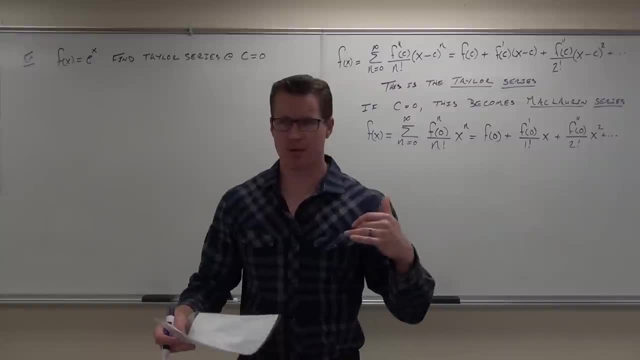 No, No, just say find the Maclaurin series, And that would be exactly the same thing as what I just said right here. So if I say find a Taylor series, that's equal zero. this means find the Maclaurin series. 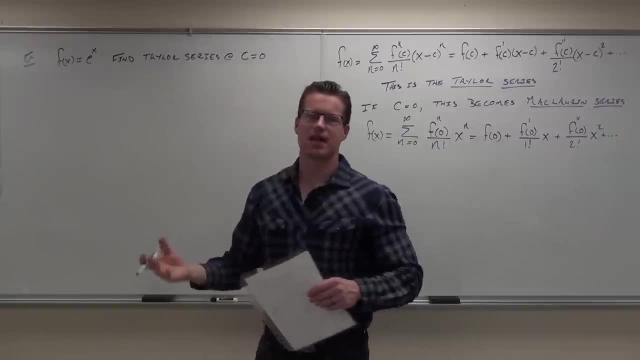 That's all it means. You okay with that? Mm-hmm, I'm going to give you the steps on how to do this. If you follow these steps every time, this is going to make your life a lot easier. So here's the steps. 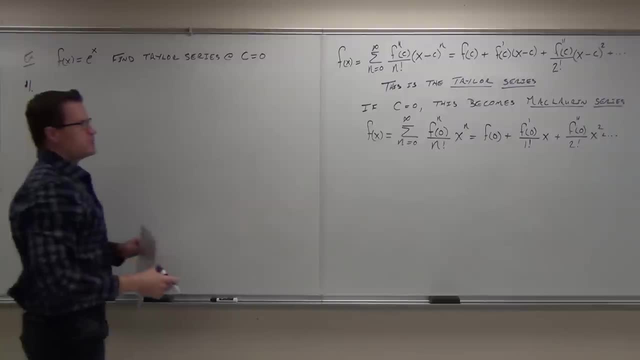 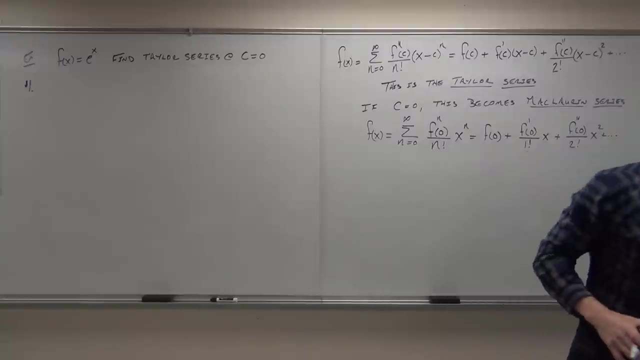 Step number one, Because our Taylor series are based all on derivatives, what you're looking for here, and it's not that hard to actually do, but it's hard to find the pattern. so I said: find the patterns, the hard part, okay. 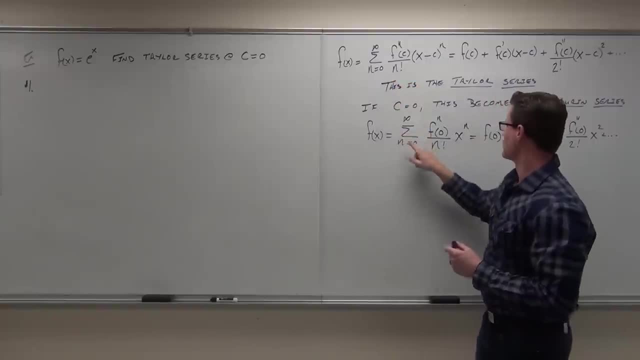 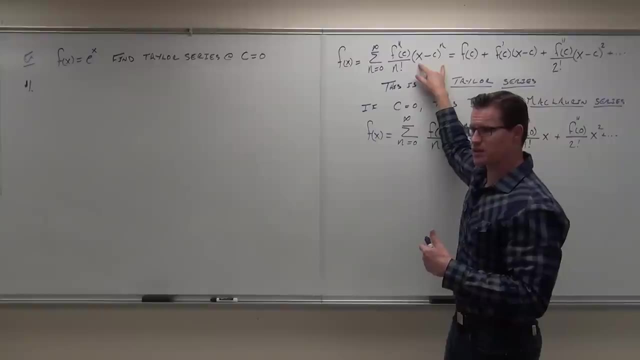 Check it. This part- or rather where am I at This part- never changes. That's going to be n factorial. This part never changes. That's going to be x minus c to the nth or x to the nth, No problem. 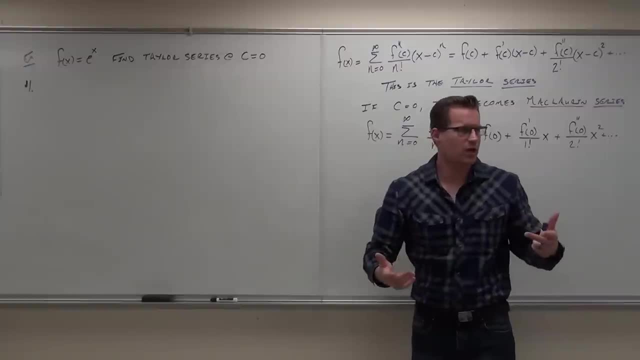 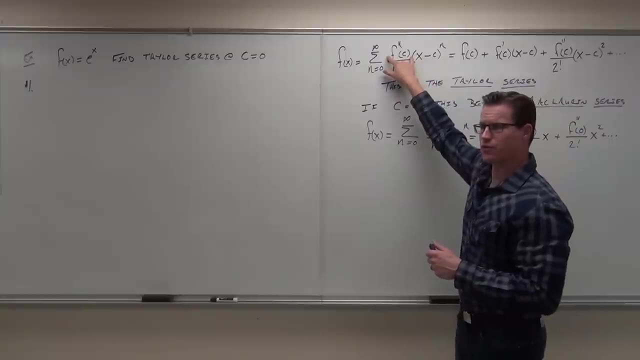 Whether you're dealing with Maclaurin Or a Taylor series, Okay, All you're looking for. all you're looking for is this guy or this guy. That's what you're looking for. Does that make sense? And if you have a c, then it's not just going to be c. 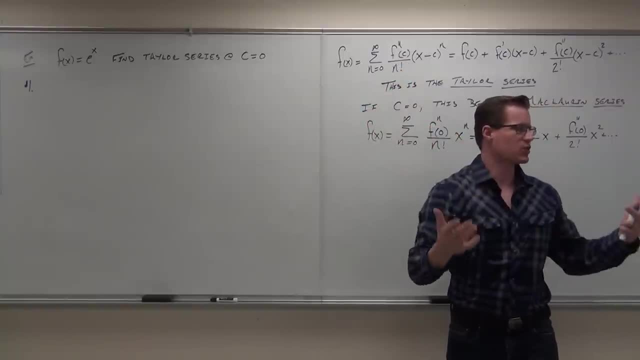 It's going to be like centered at 1, or at negative 3, or whatever you have it at. It's going to be around that one point, So you're going to have an actual number. What you're trying to find out is find a pattern that represents the nth derivative of f. 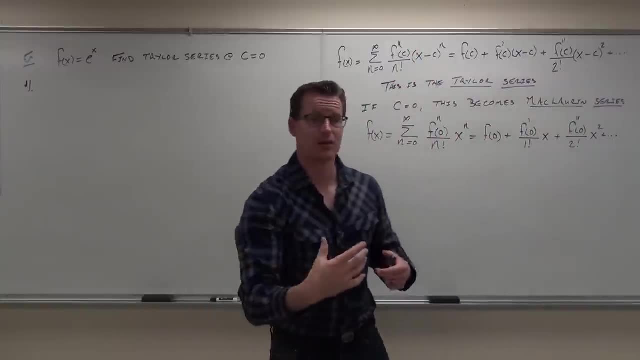 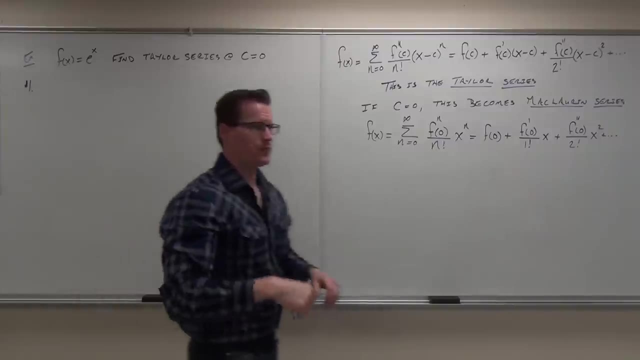 So, in order to find a pattern that represents the nth derivative of f at a certain point, like 0, or whatever number I give you- in this case I gave you 0,- you need to start with the derivatives. So step number one is find several derivatives of your function. 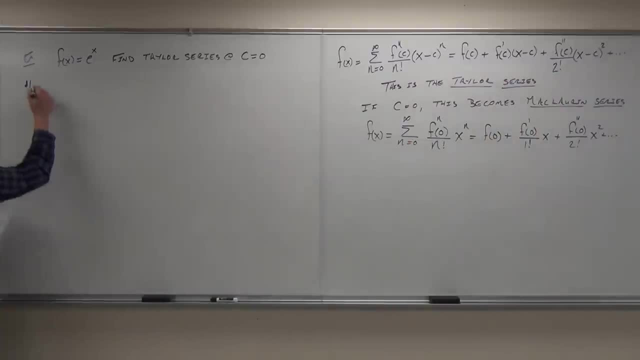 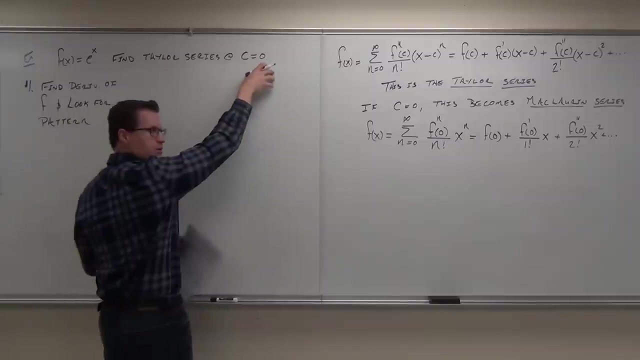 Start with several derivatives of your function. So find derivatives of f, and I want you to start looking for a pattern. So I'm going to do that right here and we're going to do another column right next to it, so leave yourself some space. 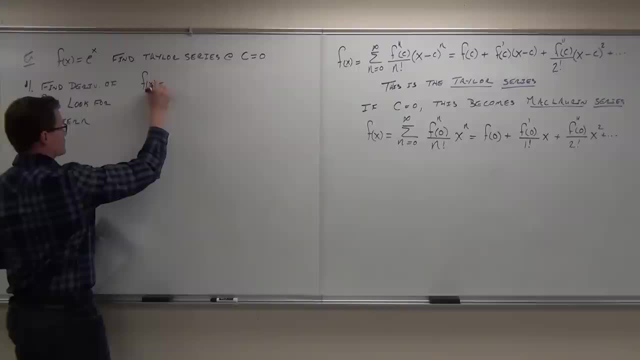 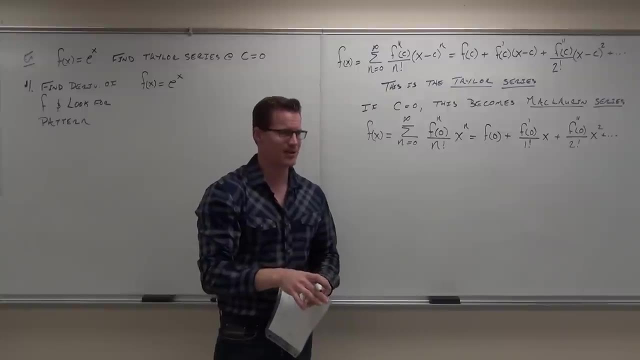 So we start with the function itself. f of x equals what please, E to the negative 2.. Now I think I gave you probably the easiest example in the world right now. Okay, What's the derivative of E to the x? 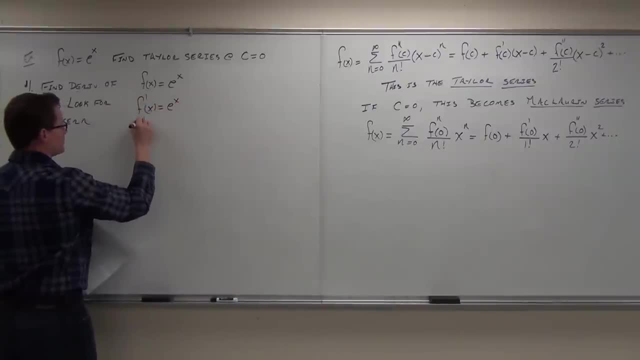 E to the x. Oh, oh, but wait, What's the next derivative? E to the x. E to the x. E to the x. Okay, Well, wait a minute. How about the next one? E to the x. 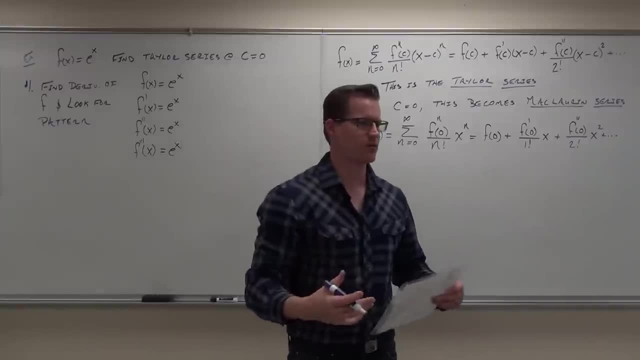 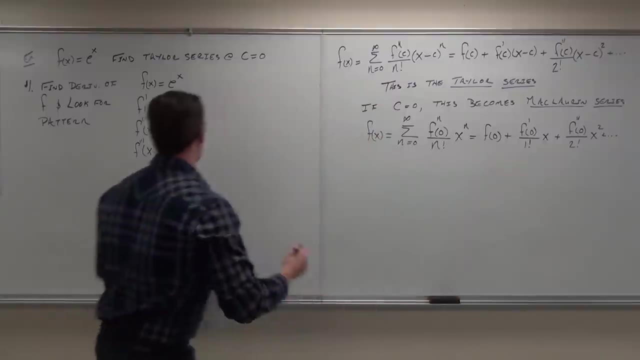 Go ahead, Do it a lot. okay, Do like. typically I do three or four derivatives. In this case, this is pretty straightforward, so we're not going to do that, but you usually do like three or four derivatives. What you're looking for is the pattern, so that you can go down to here and say, all right. 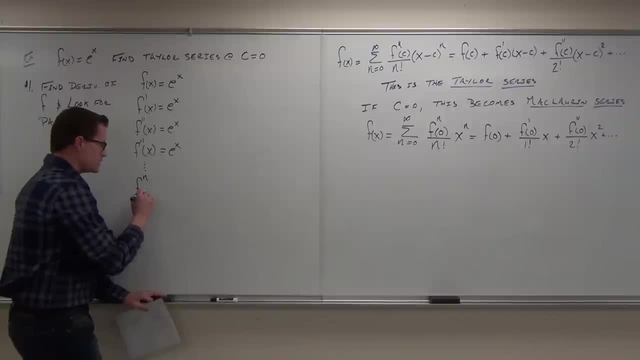 now I know what the nth derivative of f is. You see, you want a pattern so that you can plug in a number to that. So if you know the nth derivative of x, you can find the nth derivative of c- 0, or 1, or 2, or whatever. 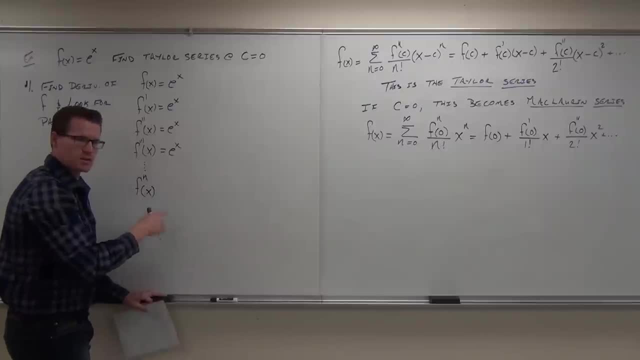 Sometimes it's not this easy. I'll give you another way to do it in a minute, but sometimes it is So you're looking for a pattern on your derivative, if you can find one. So what is it? Pretty good, You guys are geniuses. 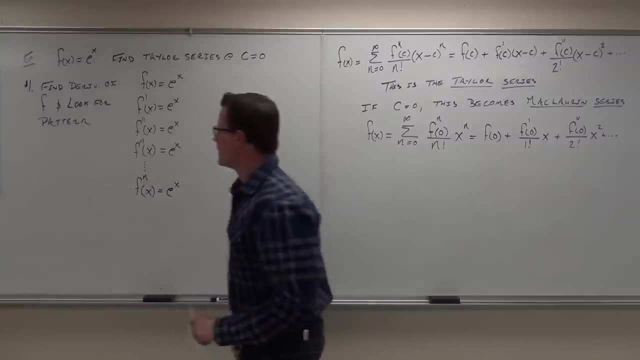 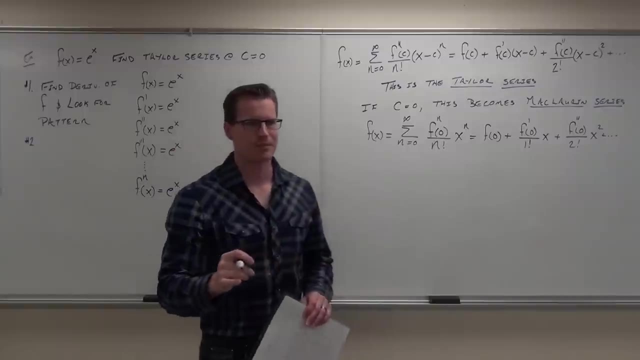 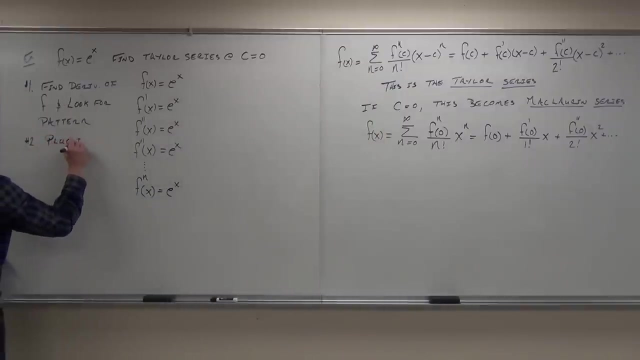 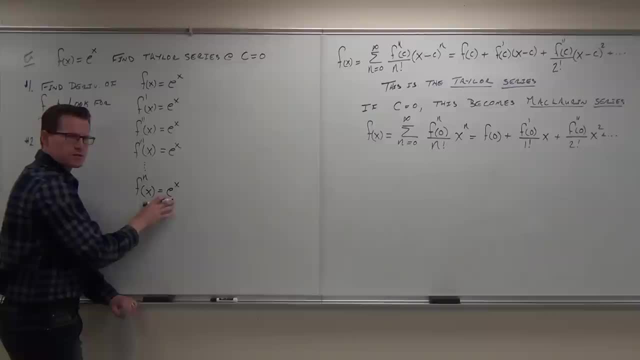 It's going to be apparent to you, but we're not really looking for this. This is x, the nth derivative of f, at x, I'm looking for at c. So our next step is: plug in: x equals c. Make sure you find the pattern here. 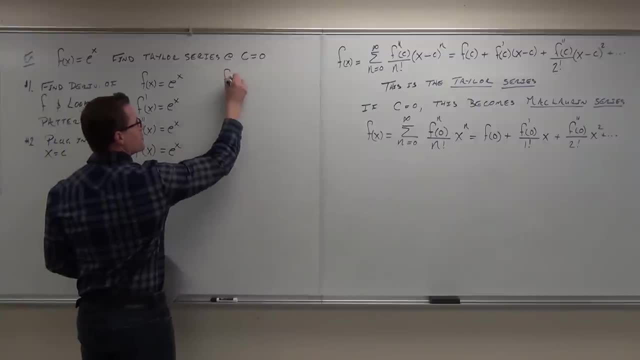 This is the big one. So here's what I do. over here I find I find f of c. I want f prime of c. I want f double prime of c. Only in our case we know what our c is. 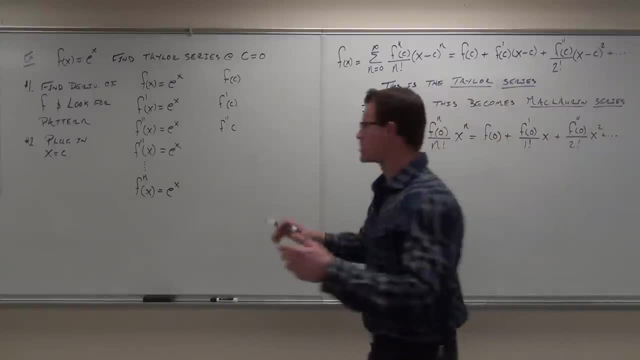 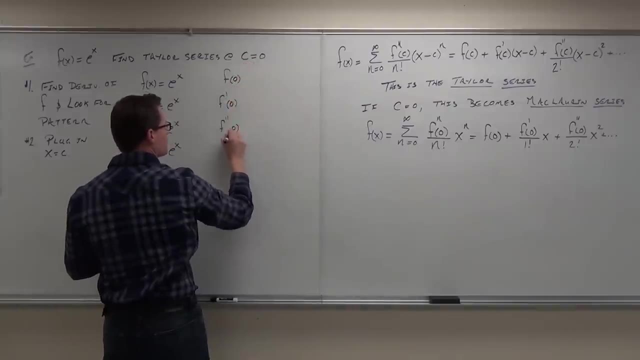 You're always going to know what your c is. What is our c here? Zero. So I don't want just f of c, I'm really looking for f of zero And f prime of zero And f double prime of zero. 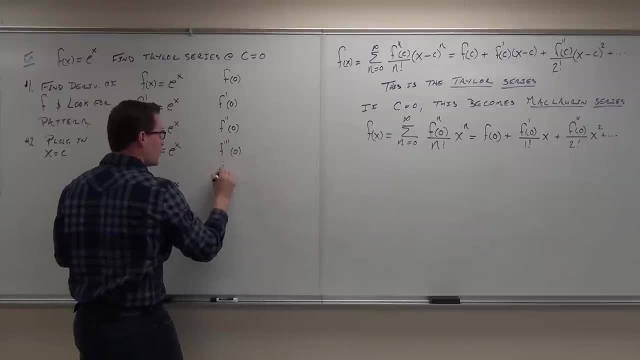 And f, triple prime of zero, And ultimately, this is what I want. I want f, And that's an nth derivative of zero. Let's see if we can do this. You see what we're doing here: we're trying to find a pattern based on n for this thing. 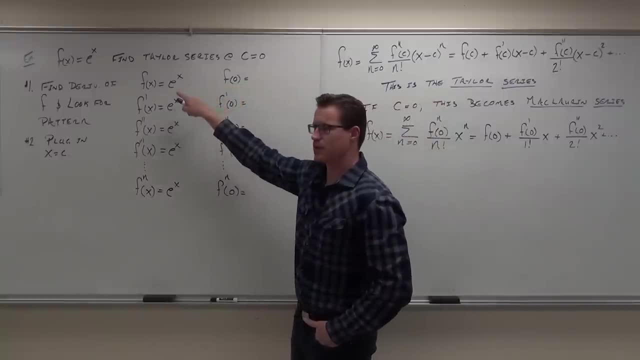 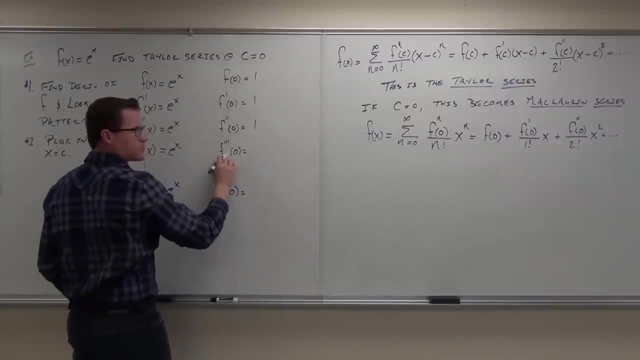 So what's f of zero? when I plug in What's f prime of zero One? What's f double prime of zero One? What's f triple prime of zero One? Do you see a pattern here? Yes, What's f. 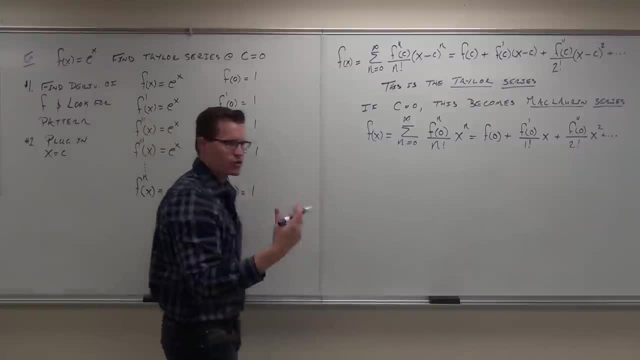 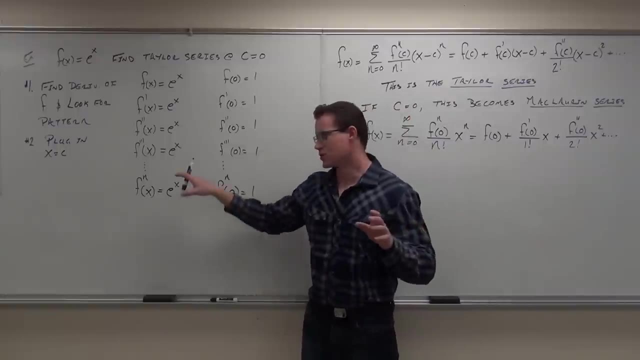 What's an nth derivative of f? at zero, One, One, One. If it never changes, you're just going to get one or two, one Show of hands, if that makes sense to you. So if you can find a legit power, sorry. 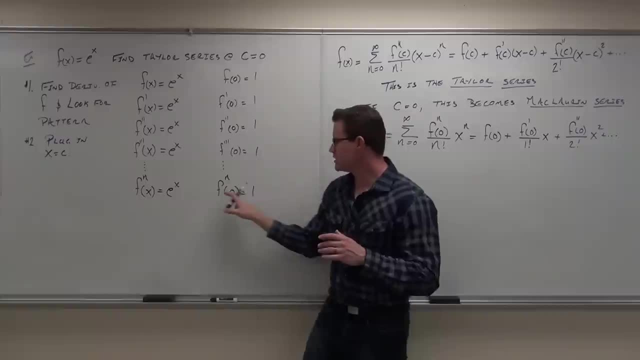 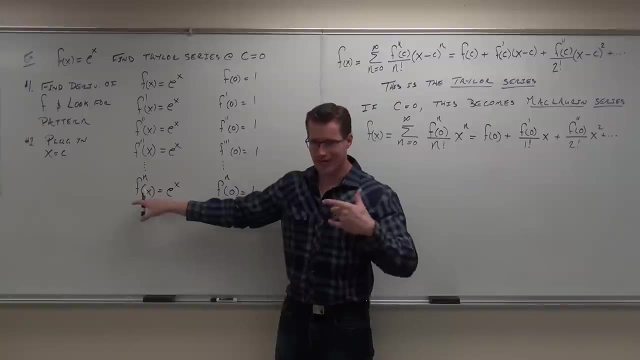 legit pattern for the nth derivative of f of x. all you got to do is plug in zero to right. here It's going to work for you. Does that make sense to you? Sometimes this is really hard. So besides doing just that, we try to look for a pattern amongst these terms. 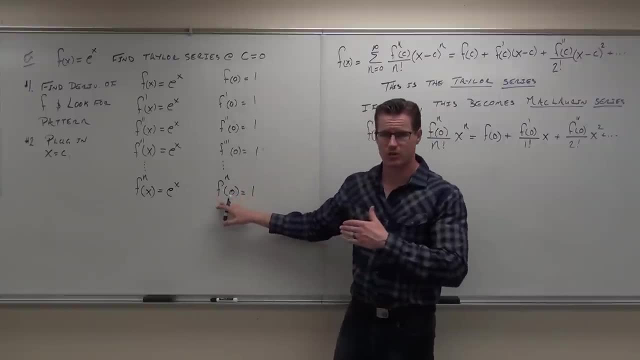 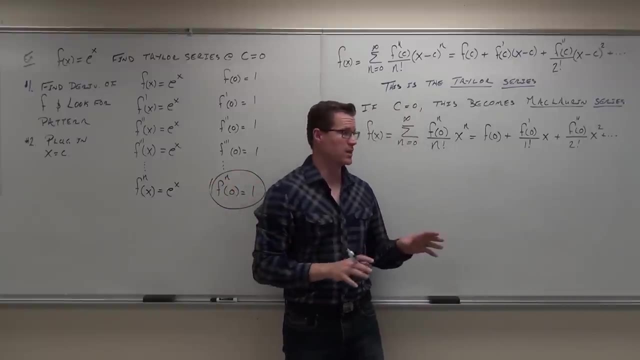 and we try to work this down to get the nth derivative of f at whatever point we're trying to find. As soon as you find this, everything else is easier. Everything else becomes really really easy. Are you ready for it to get really really easy, Are you sure? So here we go. 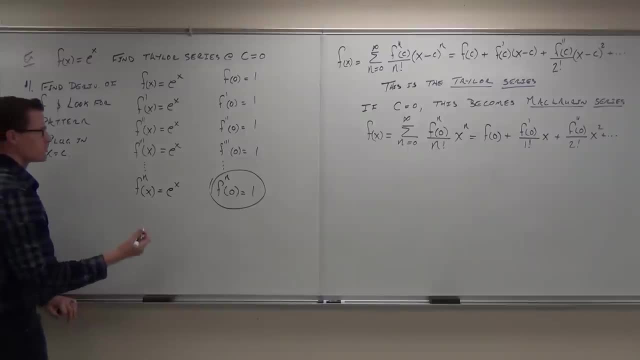 So if we want to find a Taylor series at c equals zero- that's a Maclaurin series- then what we know is that our function is going to equal a series that looks like this: It's going to be f as the nth derivative of f at zero, over n, factorial x minus c to the nth. 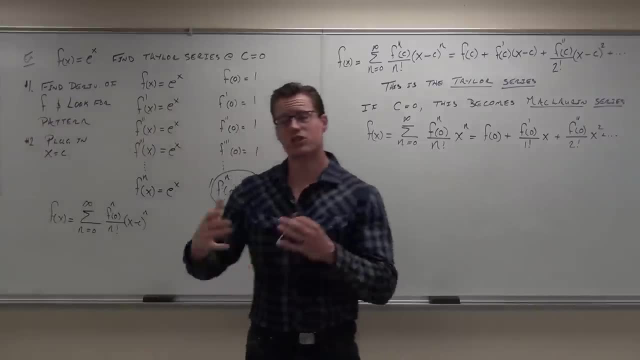 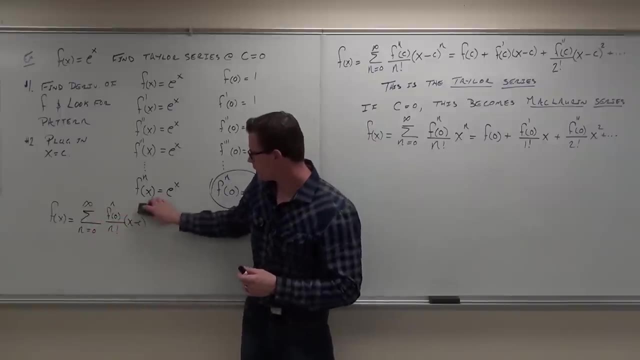 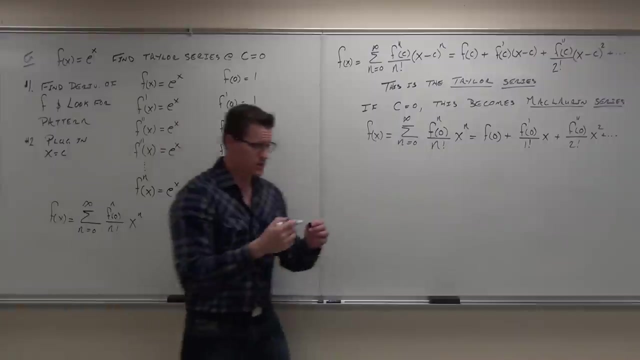 derivative of f at the nth. OK, by definition, by what we just proved, this is the Maclaurin series. This is a Taylor series at. actually I'm a little wrong. This is the Maclaurin series. if I just do x to the nth, It's a Taylor series at zero, because when I do zero I'd. 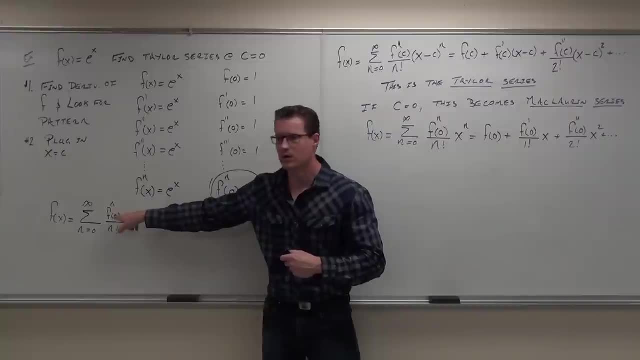 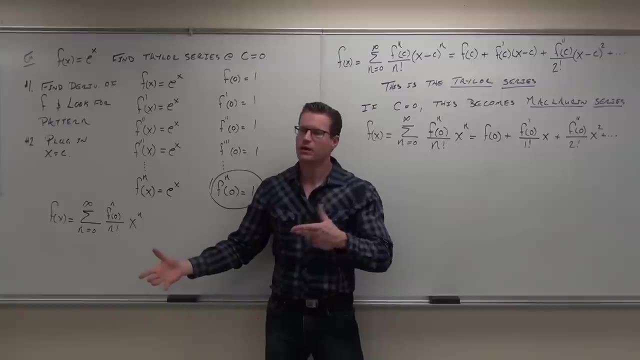 have x minus zero to the nth, I would have a zero for my c Show of hands, if you feel OK with that one. That is a Maclaurin series, That's a Taylor series at c equals zero. They're Now all we've got to do is. did you notice why we only have 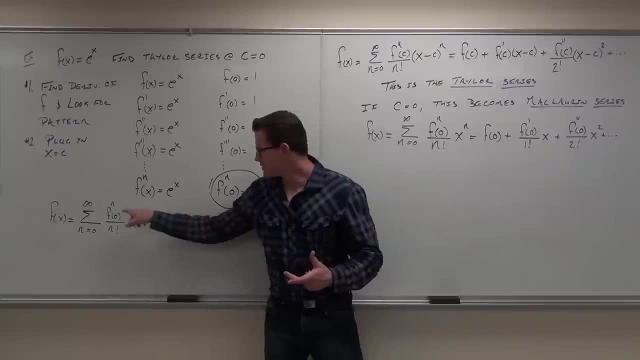 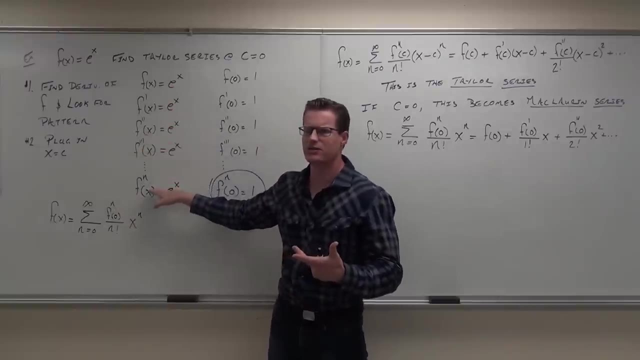 to find one little piece of information. All we're looking for here is that guy. That's it. This stays the same. that stays the same. it's that guy. So we find our derivatives Cool. Find a pattern, if you can. 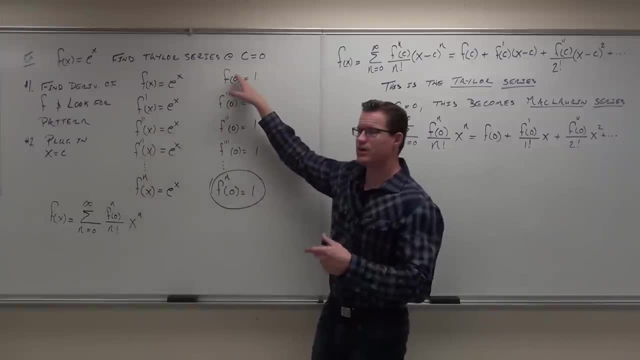 Sometimes you can't Find a pattern. if you can't Plug in the number C, Find a pattern, definitely This is where you have to do it. Whatever you get as the at C, this, whatever this is, it's usually this is the most basic example. 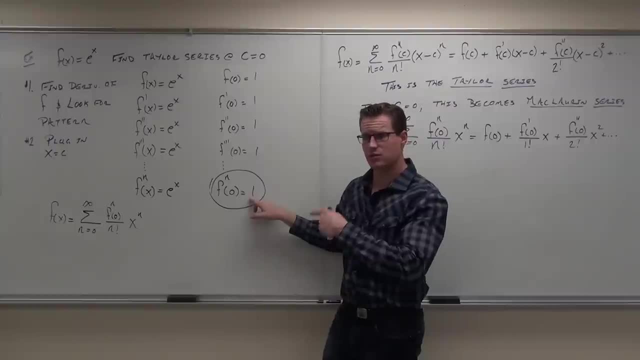 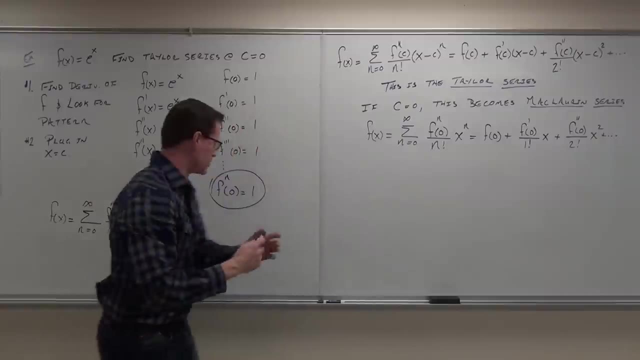 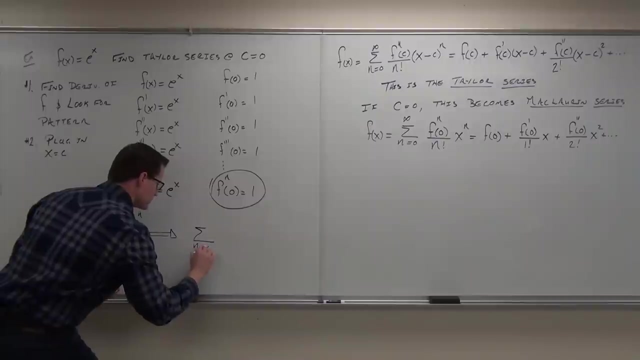 I can even think of. It's usually based in terms of N. So base this in terms of N and put it right there. You catch that. So all you do is a little substitution. So this thing changes to You. tell me what's it change to? 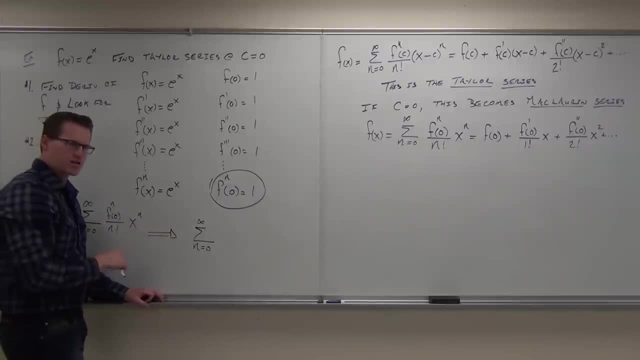 What's the Nth derivative of F at zero? What is it? One One, It's always one. Over what? F at zero, Over what F at zero, And then F at zero, F at zero, Perfect. 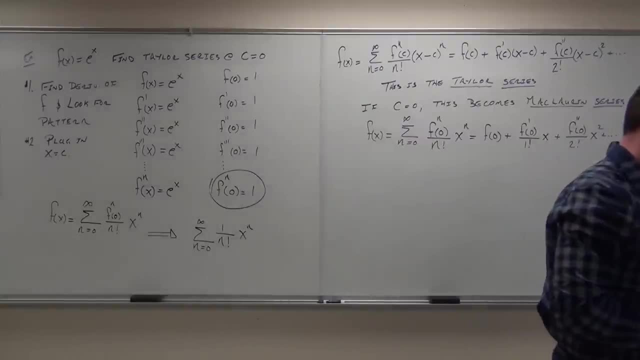 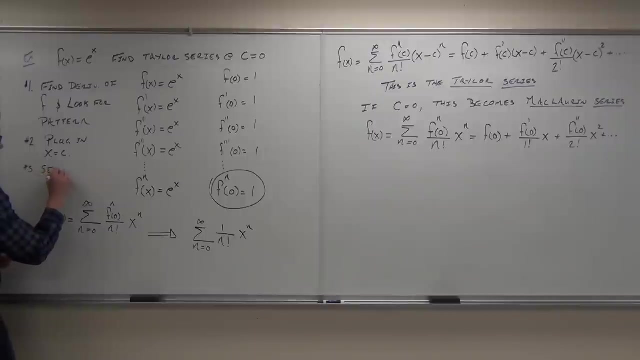 That's exactly right, Exactly, exactly right. So, step number one: find your derivative. Step number two, plug in: X equals D. Step number three: as soon as you have this thing set up, your series. Now step number four is where the figure is. 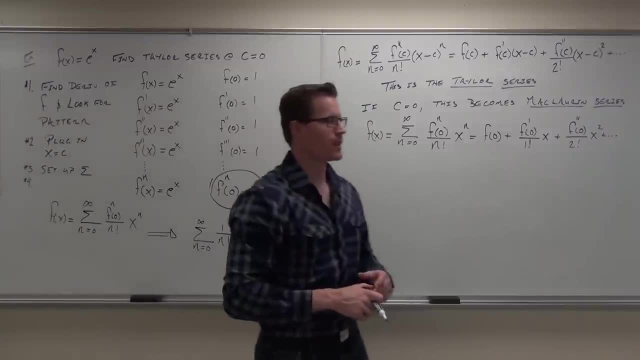 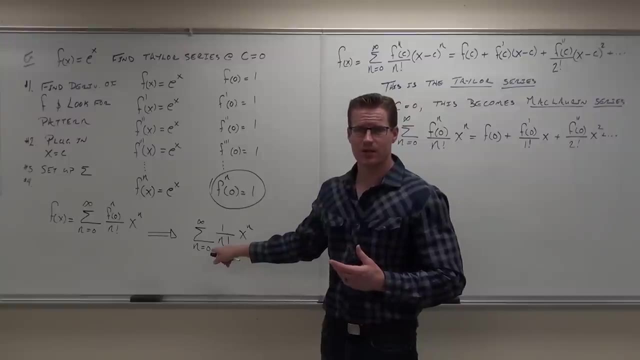 the fun begins. Step number four: well, hey, does that look like something we have dealt with before in this class? Could you find me the interval of convergence? Ah, does that sound familiar? Did you just do homework on that, Or should you have? 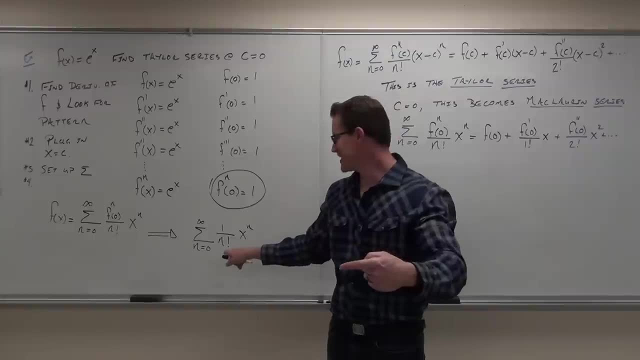 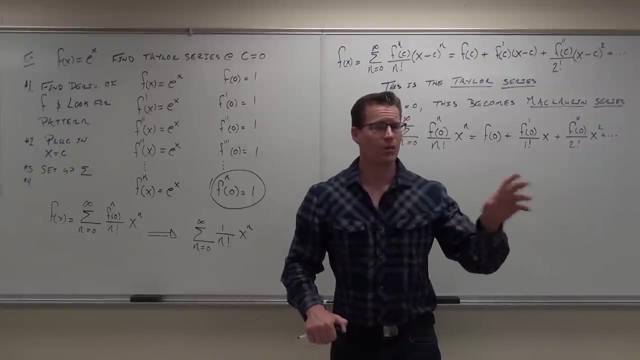 just done homework on that. Now you go through the ratio test or the root test or something that will give you the interval of convergence. You see what we've just done here is, you said, cool. this is awesome. you know what that's. that function has a power series. 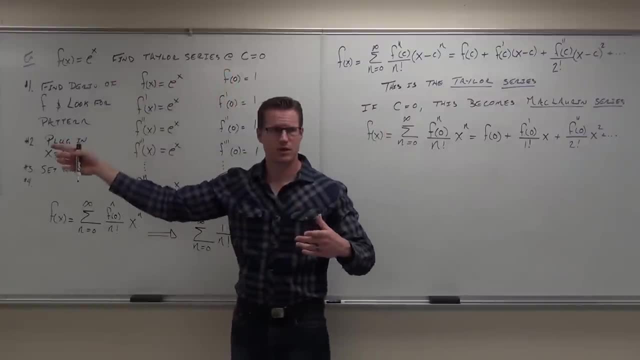 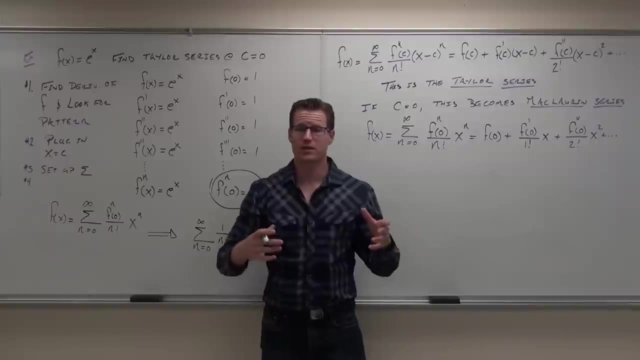 representation that's equal to zero. that's a Maclaurin series. Well, we've just found the Maclaurin series, but you need to tell me where it's good for. The where it's good for is the domain. The where it's good for is the X's that make 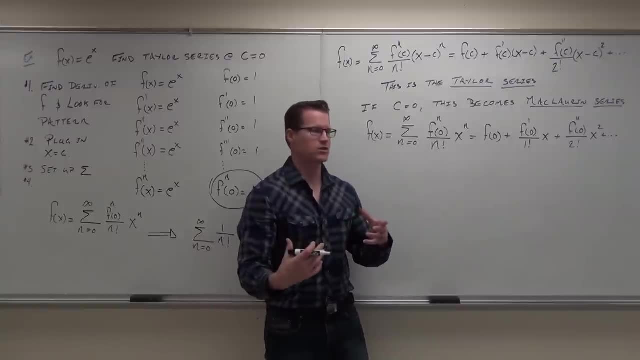 the series convergent. Remember that a function is only represented by a power series when that power series is convergent, when we actually have a sum. Do you remember talking about that? So we're looking for the interval of convergence, the domain. 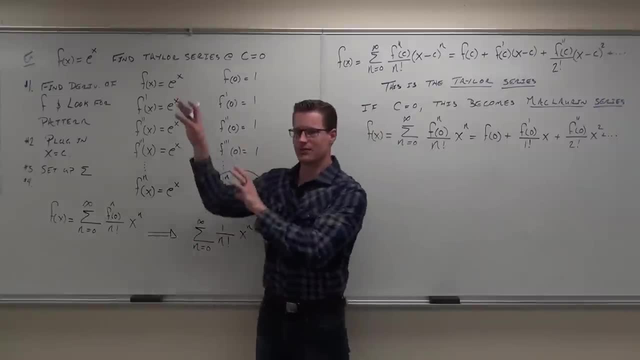 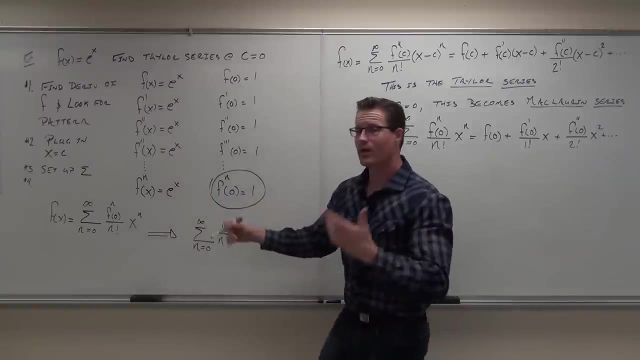 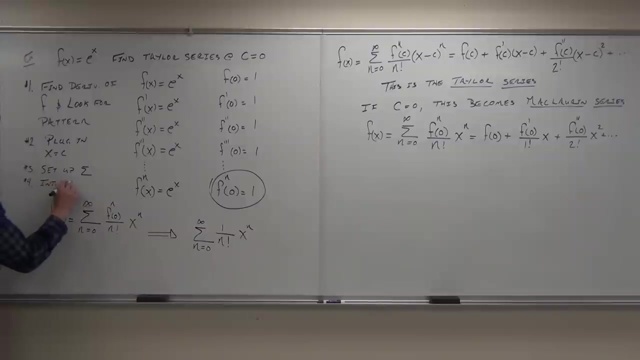 We're looking for the X's which make this power series convergent. that will represent that function. Did you catch all that? It's in the previous section, if you want to review back on the power series idea. So last little thing. step number four is find interval of. 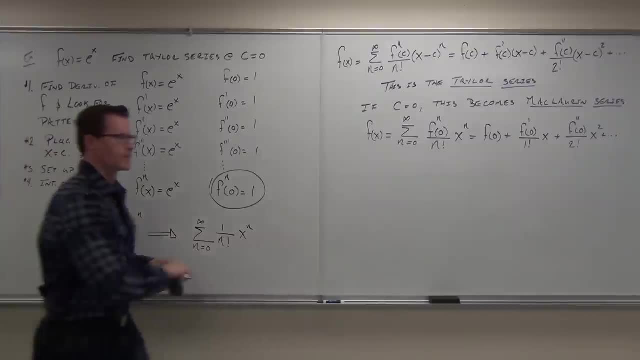 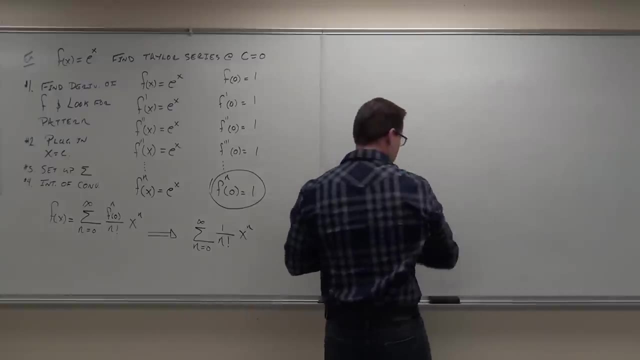 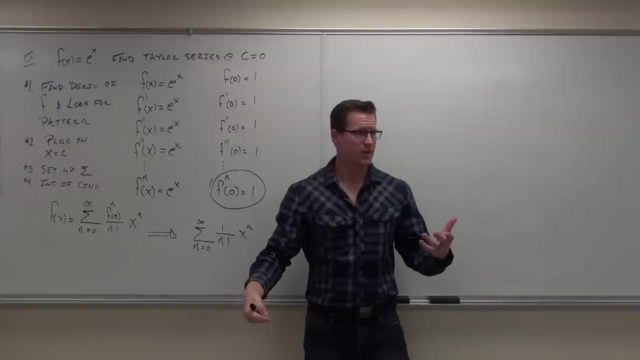 convergence. That is all the stuff that we've just done. Are you starting to see how this chapter before it's like this? what does this even build at all? Are you starting to see now how this builds? Why we did all that junk? We did all the convergence tess. 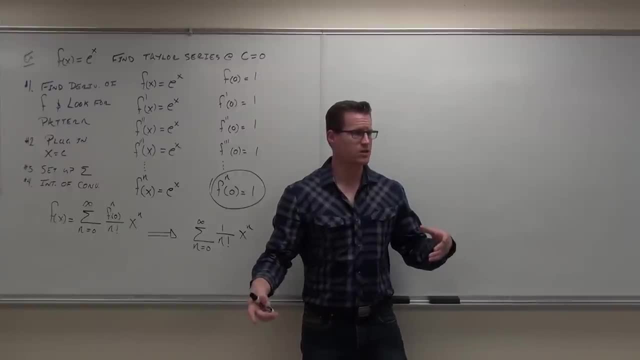 because of the endpoints For power series. We did the power serie, the ratio test for the power series and root test for the power series. We did power series for Taylor series and Maclaurin series and we did those for approximation of by Taylor polynomials, Which we will do in the next section. So here's our last thing. 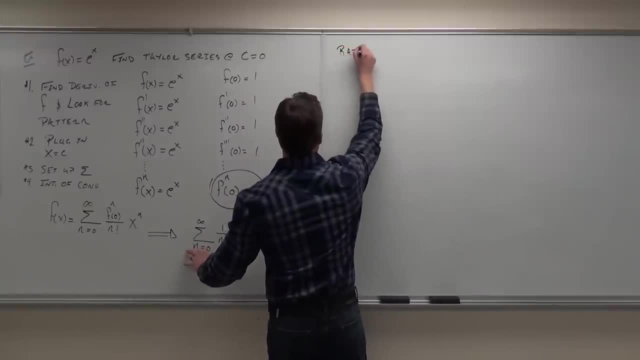 find the interval of convergence. You will all say almost always. you'll oftentimes use the ratio test for this. So I will not say always, but always. So cover it for me, and if you don't know, then you could do this. We'll go ahead and 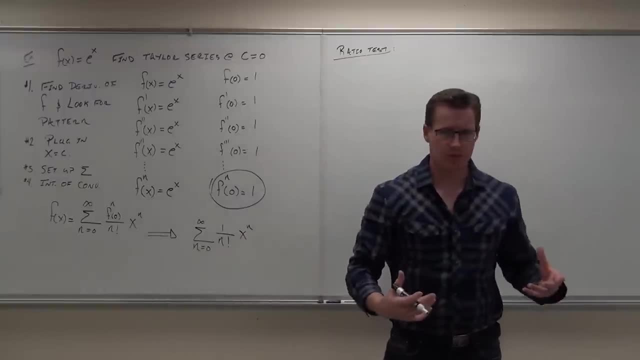 I'm going to speed through this really fast. This is not the section on learning the ratio test. This is the section on just using it. now This is not a problem anymore. This is part of our problem. The problem really is right here. 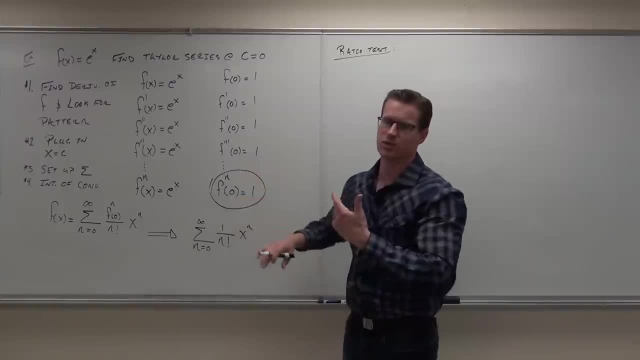 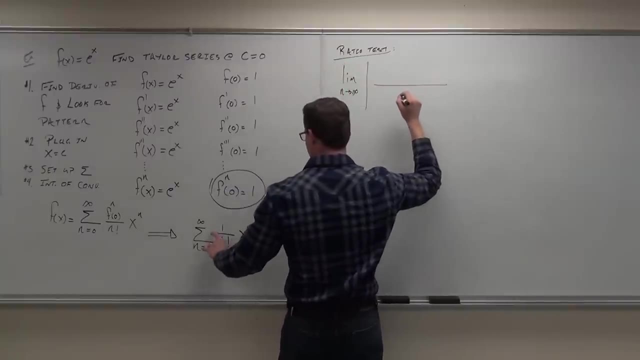 As soon as you do this, you've solved the problem. The rest of this old stuff. So we're going to do a ratio test Limit. as n approaches infinity, Absolute value. This would become, by the way- you can simplify this- 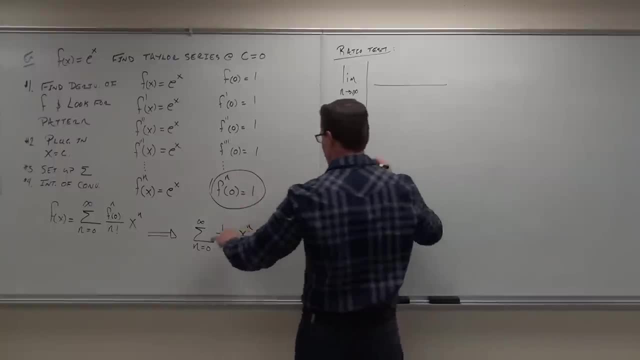 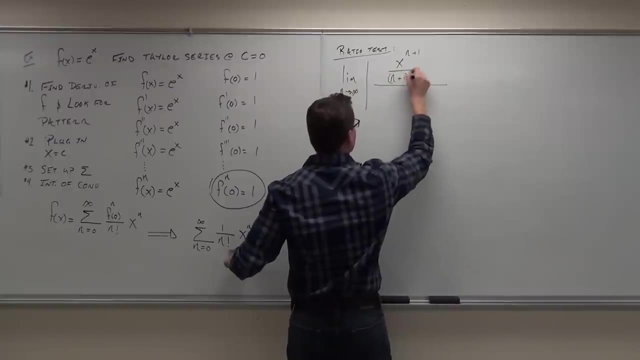 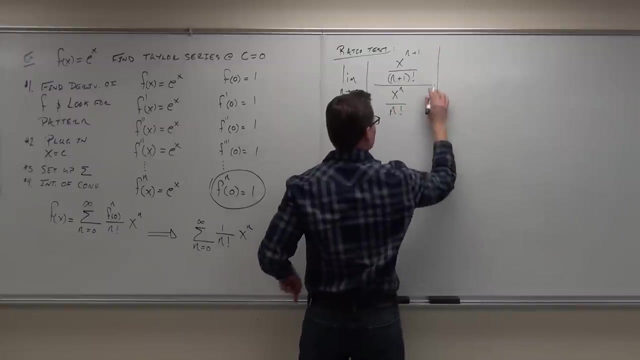 Make this x to the n over n factorial instead of 1.. Make it a little easier for yourself. So x to the n plus 1 over n plus 1, factorial. All over x to the n over n factorial. So far, so good. 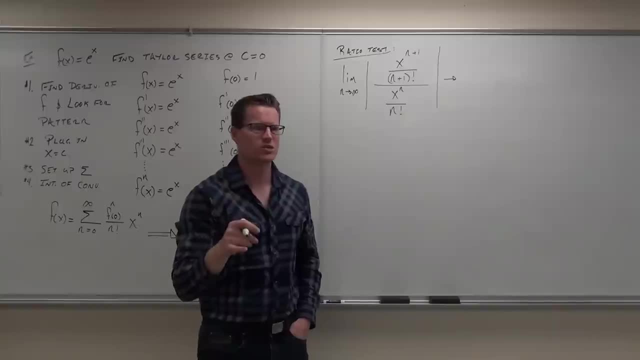 Do you see where all that comes from? It's just our ratio test. Tell me when the ratio test says convergence, When this limit is. That's why we're doing this: To find the interval of convergence. So we keep on going. 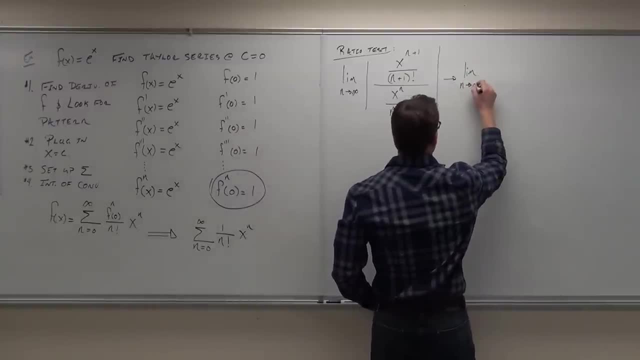 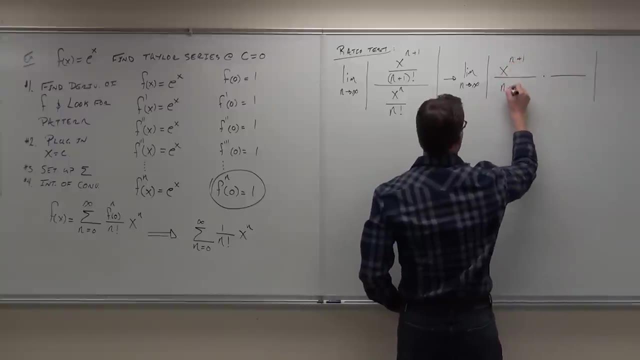 That's a limit. Should I drop the actual value right now? No, Oh, please don't do that. Very good, So we have x to the n plus 1 over n plus 1 factorial, Not a problem. And then n- factorial over x to the n. 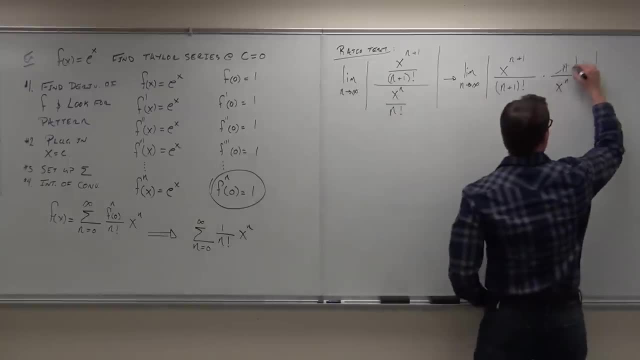 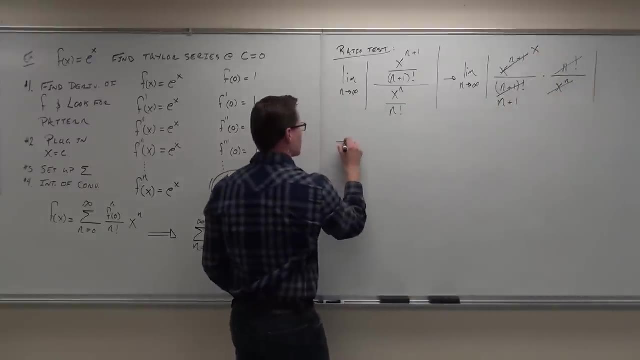 What now? Simplify, Let's do it. We're going to do it fast. This is gone. We have n plus 1.. This is gone. We have x. That gives us a limit as n approaches infinity of. Remember what I told you. 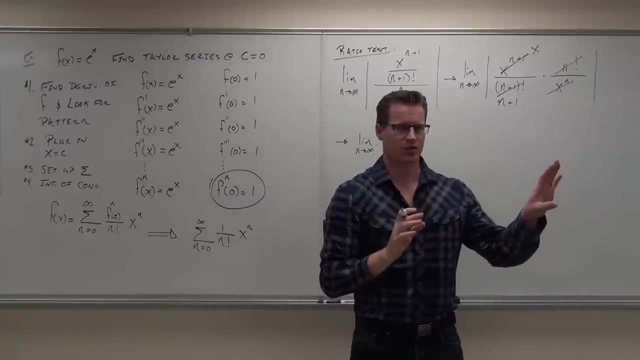 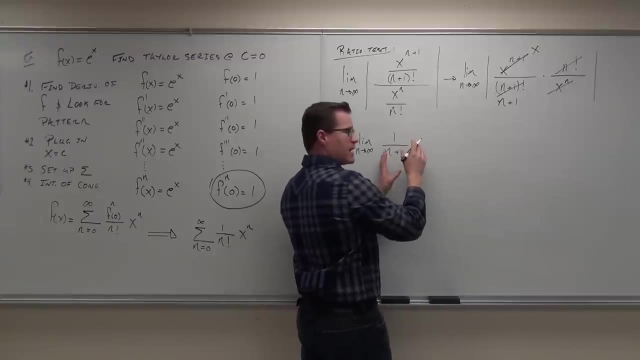 We're going to talk about this. collect your n terms, separate off your x term, So your n terms become 1 over n plus 1.. Absolute value of x. Yeah, that doesn't have to be an absolute value, because this n is always going to be positive. 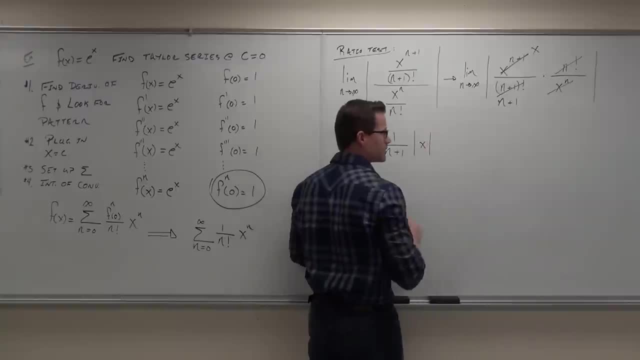 We start at 1.. But the absolute value of x of that is important. Should we be okay with that so far? Now be careful on this. You've got to be really good at this: Be able to determine what this limit is going to be. 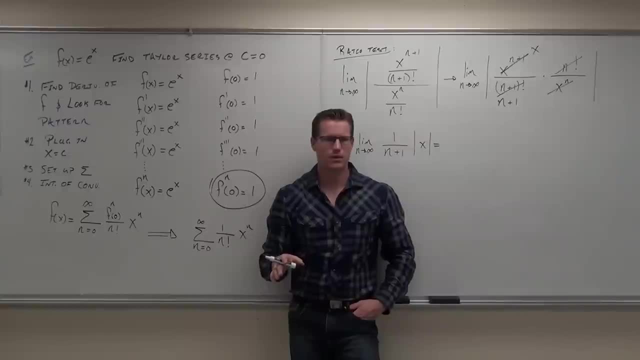 What is this limit going to be? 0. All the time For anything that you plug in for x. remember, x has to be an actual number. it can't be infinity. For anything you plug in for x, is this going to be 0?? 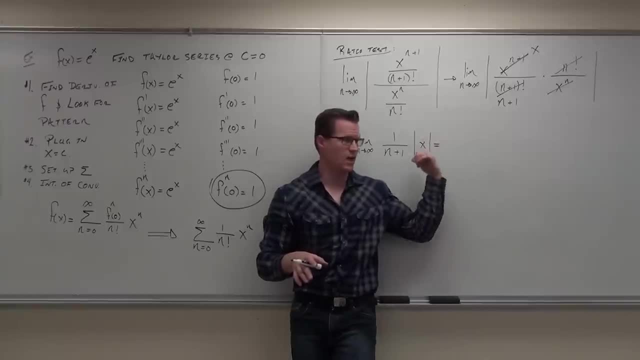 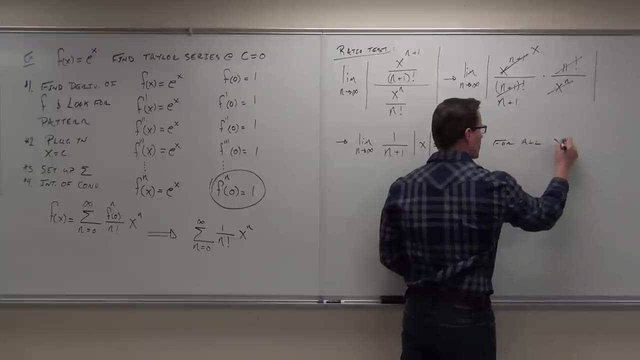 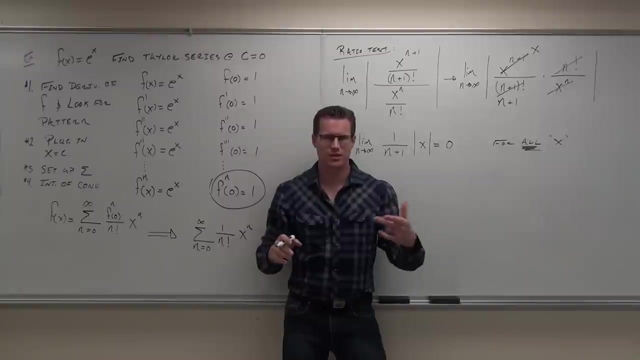 Yeah, it's something over infinity that gives you 0 times whatever I got. I don't care what that is. this is going to be equal to 0 for all x for all x. Are you with me? Okay, Now why is it important that we've got a 0 here? 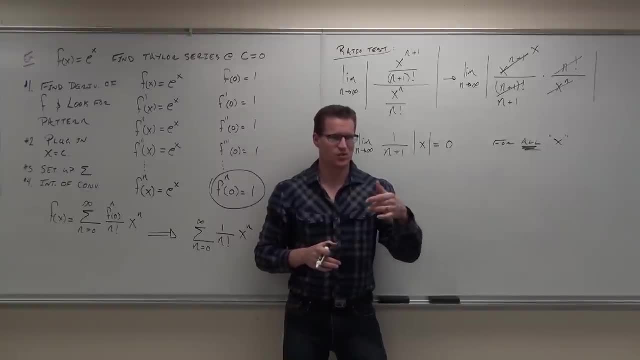 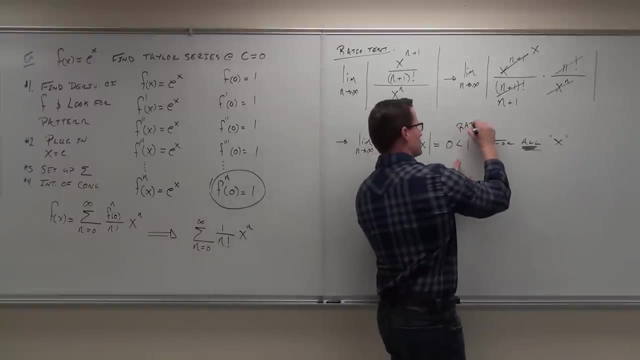 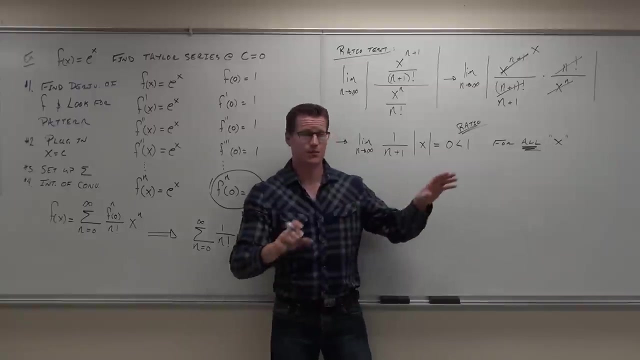 Does that help us at all? So that's not 1?? No, Ah, this is the ratio test, Since 0 is always less than 1, ratio test for all x. can you tell me what my interval of convergence is if I can plug in any x and I get 0?? 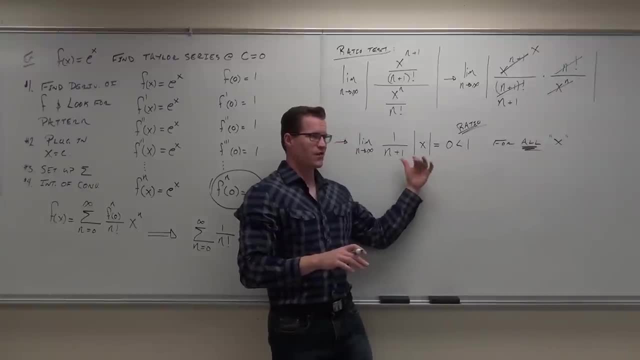 0 is always less than 1, right Negative, 1.. Good, So if I can plug in anything that says my interval of convergence is any number, this series- listen carefully, this series converges for any x. Do you get that? 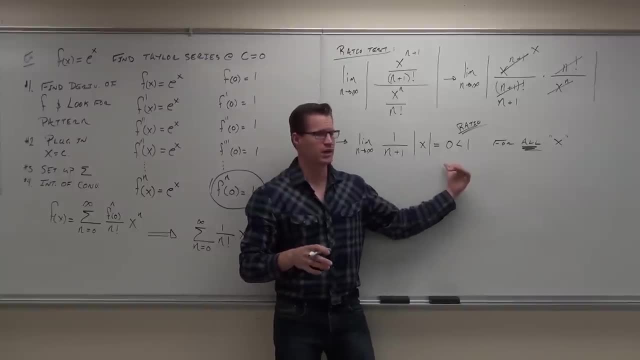 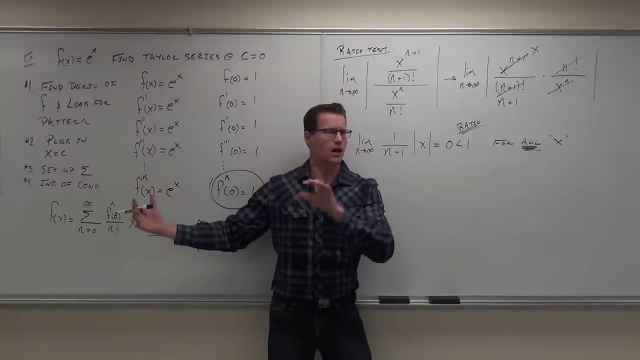 Anything, but just prove it right there. It's always 0 less than 1 by ratio test that converges for any x. What that means is that this function is represented by our Maclaurin series for any x- Any x you plug in. I can represent it with this series. 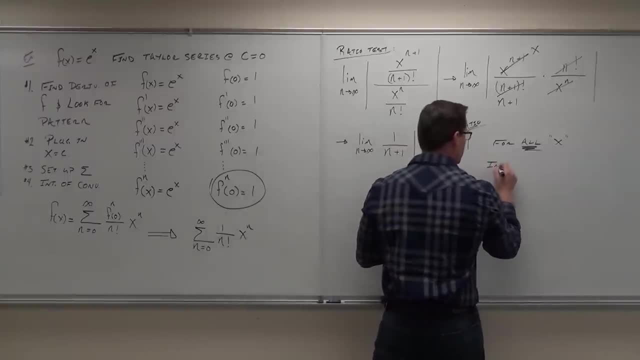 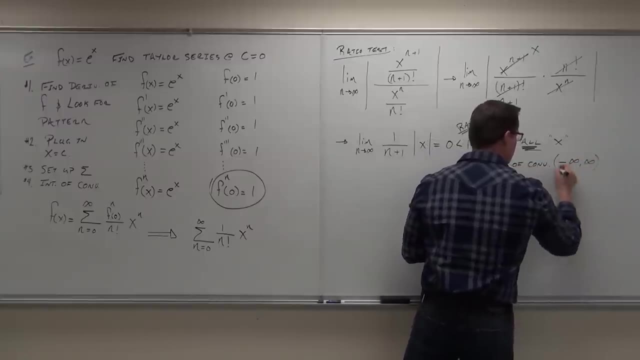 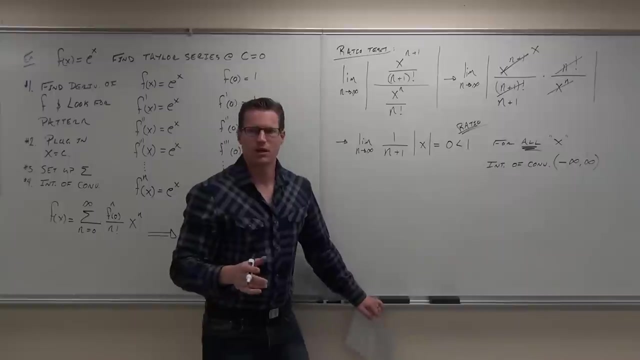 So, for all, x means our interval of convergence would be: interval of convergence is negative: infinity to infinity. Now, if you're wondering, why in the world are we doing this? what's the point? Here's the point. What's kind of cool, and here's what we would say. by the way, 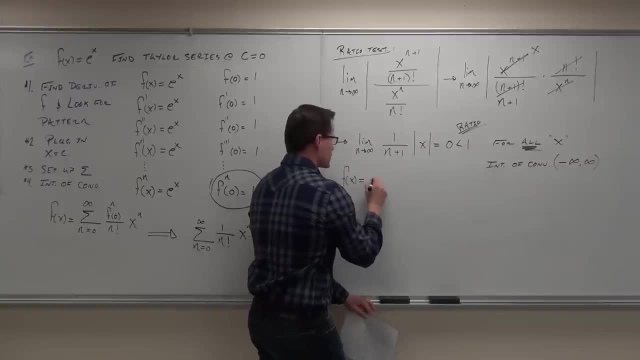 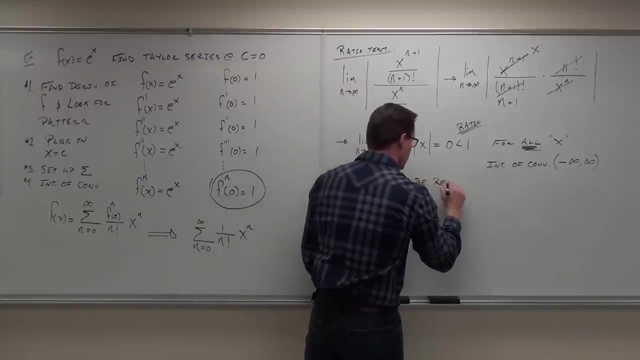 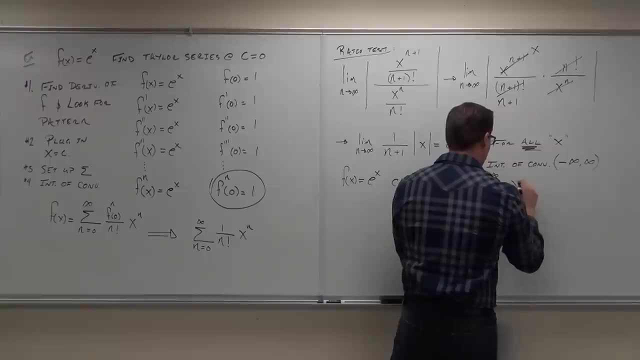 We would say that f of x equals e to the x. here's the point. can be represented by the series power series. n equals 0 to infinity, of x to the n over n, factorial. That's just right here. That's what we found. 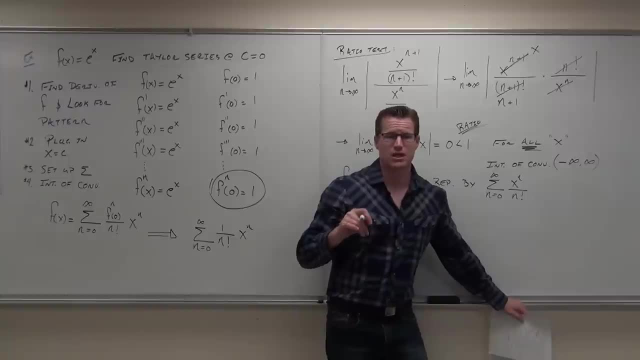 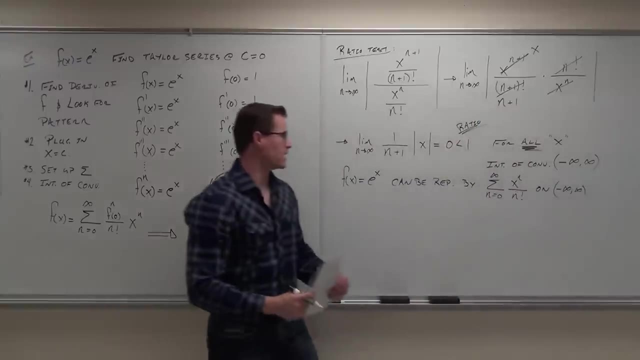 And then you state the interval for which this, this thing converges, which is the interval for which our power series works for a function. On the interval negative infinity to infinity. That's the appropriate way that you write out your answer. You say: hey, the function that we started with. don't forget what we're doing here. 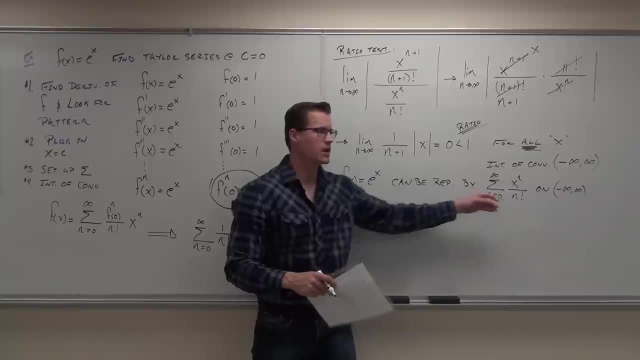 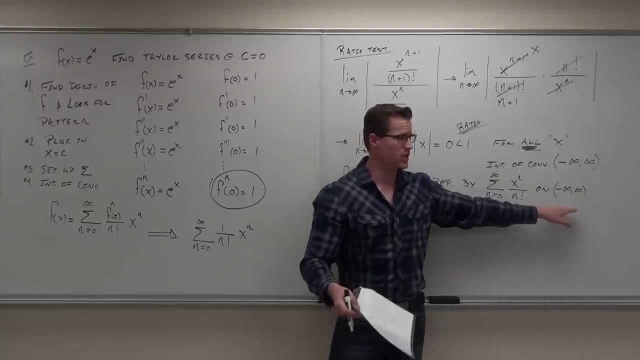 What we're doing here is we're actually representing this function with this series. It says this function can be represented by this series on some given interval. If this had been different, we would have had to check endpoints. Remember checking endpoints? Yes. 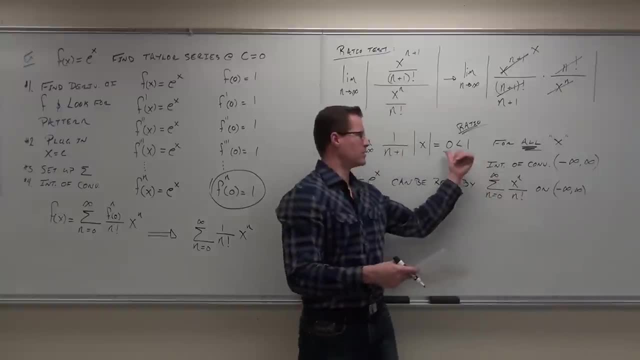 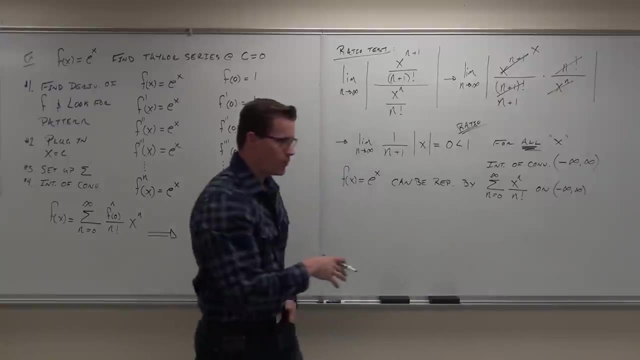 All that junk. Now, since it's infinity- well, since our limit's 0, we get negative infinity to infinity. We've got to check all that stuff. But here's the point. What you can do now is use this to approximate this. 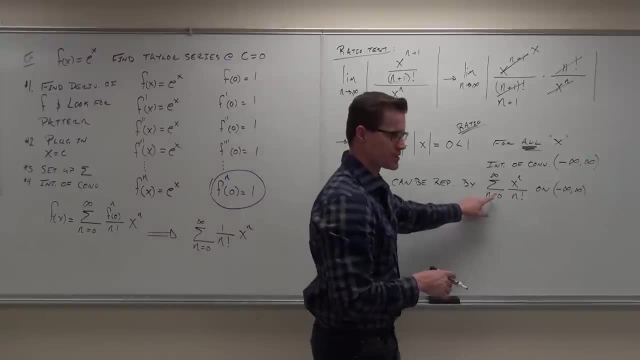 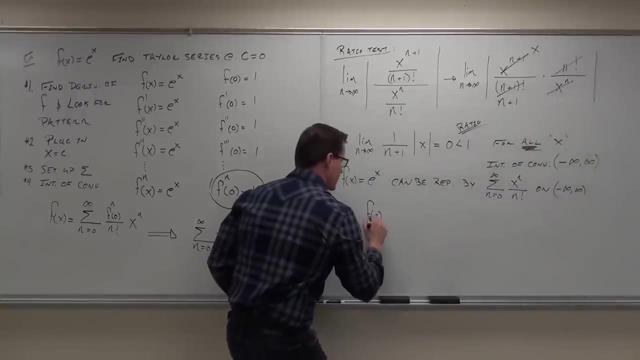 For instance, understand that this, what this is, this is. oh, what is that? Well, we could actually do it If I wanted to find f of 2, that would be e to the second power. If I wanted to be as accurate as possible, I didn't need a calculator or whatever. 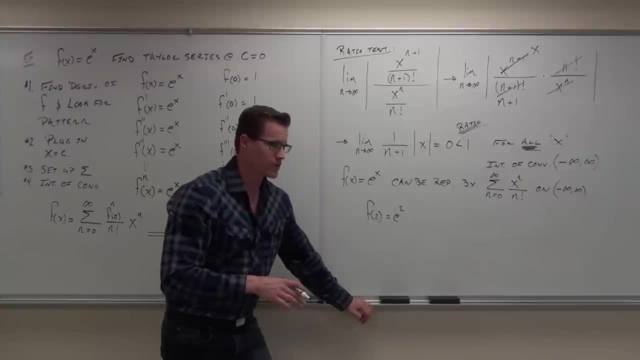 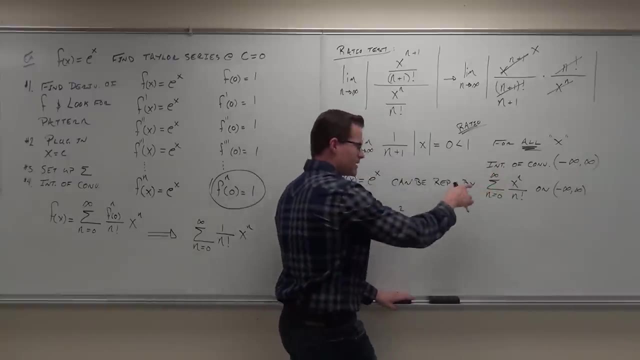 here's what I could do with that. It's really cool. I have an e here. Does this have an e in it? No, Yet when I do my series, if we did this, if I plug in 0, I would get x to the 0.. 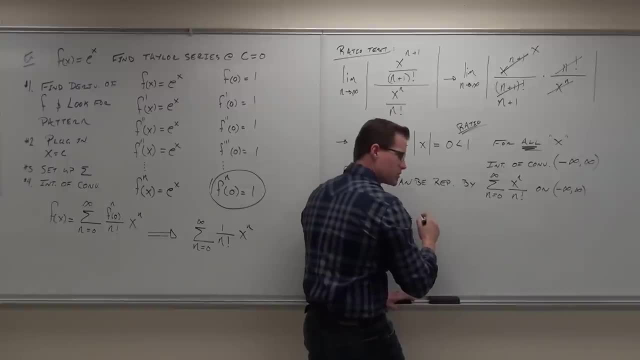 So I'd get 2 to the 0 over 0 factorial, I would get 1. 1. Plus, I plug in: remember, my x is 2 in this case. Are you with me on this? My x would be you know what? maybe it would be easier if I did this. 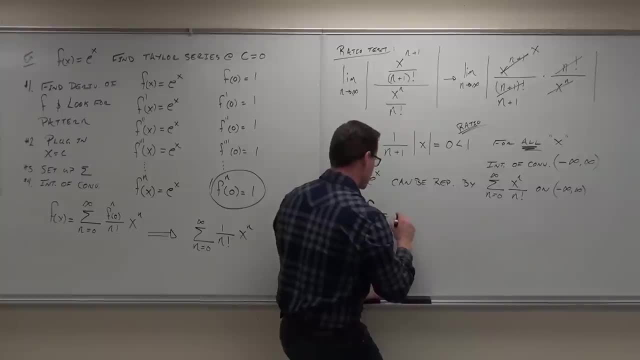 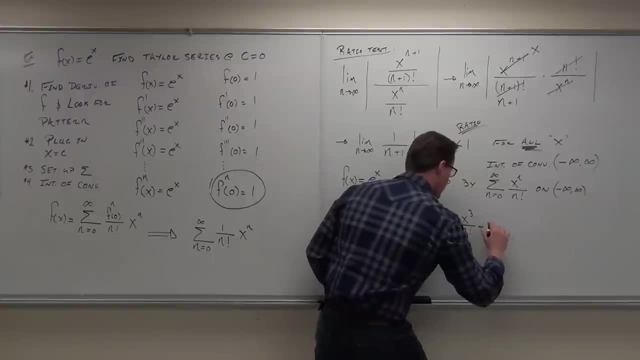 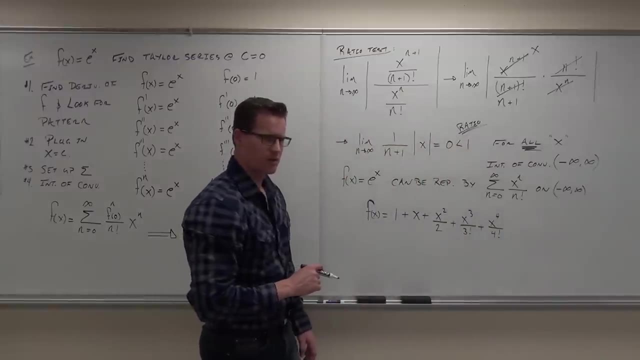 Then x to the third over 3 factorial. Then x to the fourth over 4 factorial. Do I have that right? Can you double check me on that one? Make sure I'm good, Am I? Yes, No, Okay, So if I want, 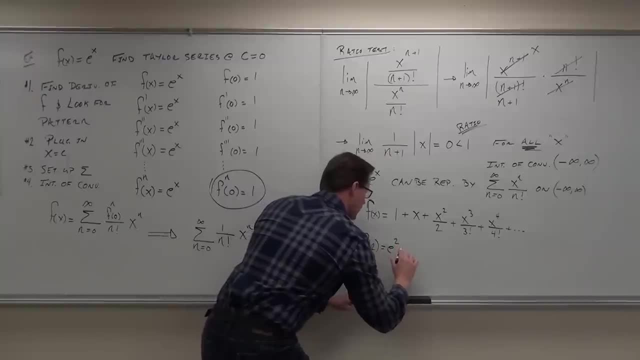 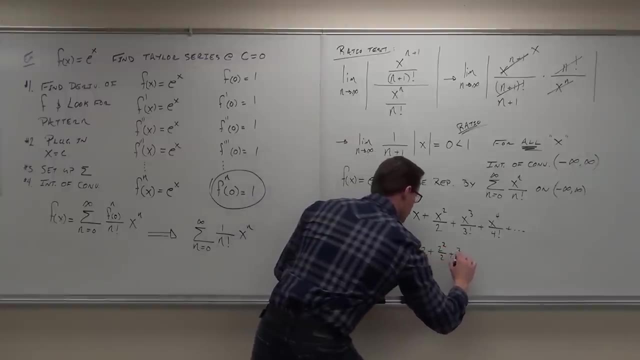 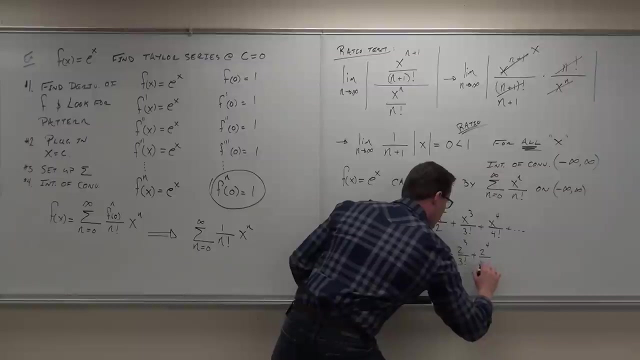 f of 2, basically, if I want e squared, well, I have 1 plus 2 plus 2 squared over 2, plus 2 to the third over 3 factorial, plus 2 to the fourth over 4 factorial. And if I do that forever and add them all up, I will find out exactly what e to the 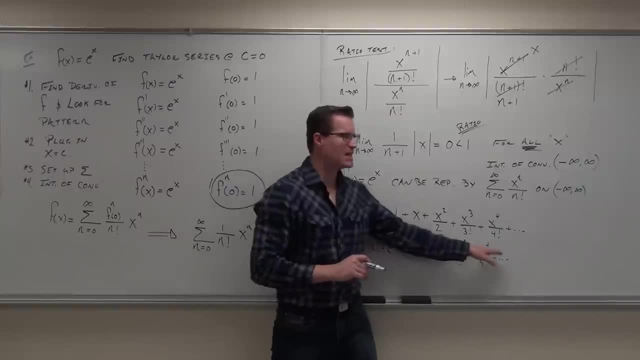 second power is: Is that interesting to you? This doesn't even have an e in it, But when I add them all up, I get e squared. You could do e to the first if you wanted to. You could find out how much e is based on just this polynomial. 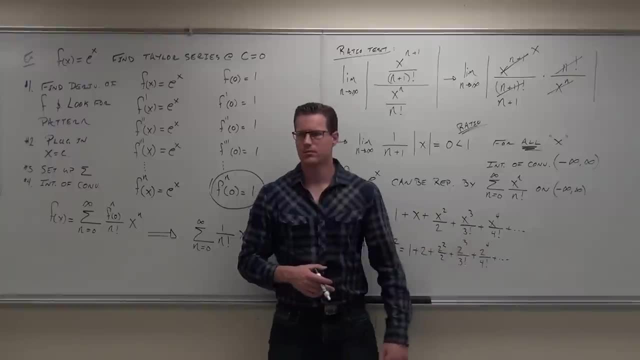 That's crazy. So if you want a good approximation, do it to the fifth term. Add them all up. You're going to have a pretty darn good approximation for what e to the second is Or e to the first, whatever you want to plug in. 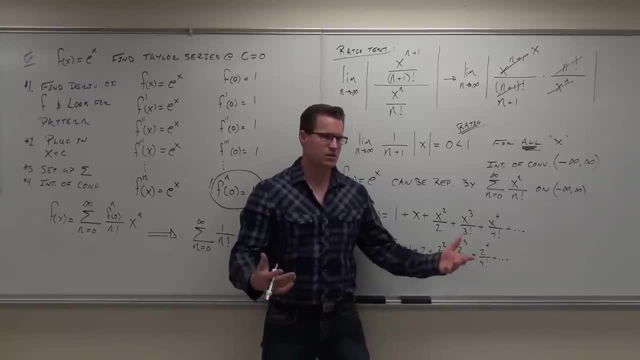 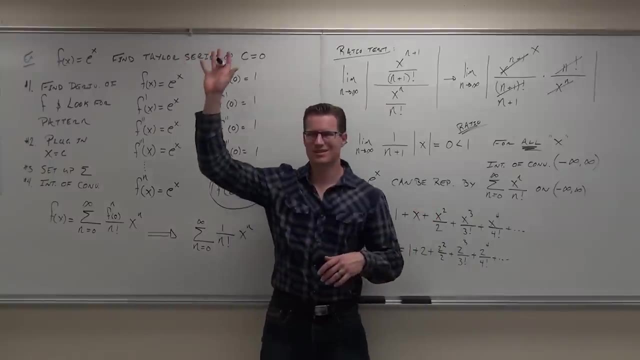 If I want to e to the first, I just plug in 1.. e to the seventh, just plug in 7.. And then add them up And you can get as accurate as you want to on that approximation Show of hands. if that one made sense. 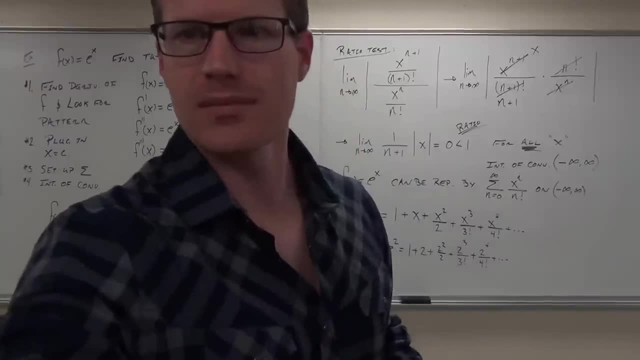 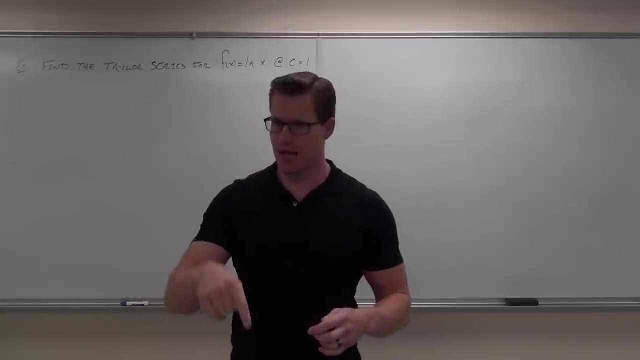 Kind of cool, right, That's the idea. All right, Let's continue our example. It's on how to find Taylor and Maclaurin series. Now, if you remember from last time, I gave you some steps on how to do this. 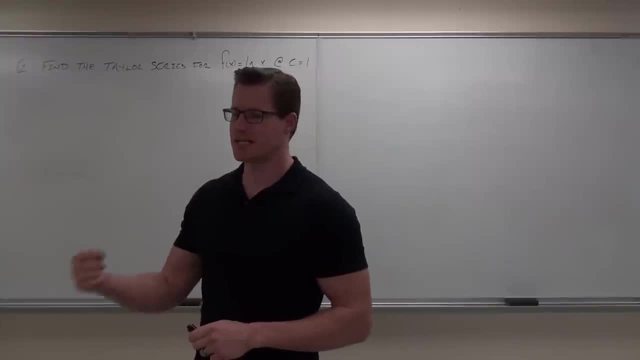 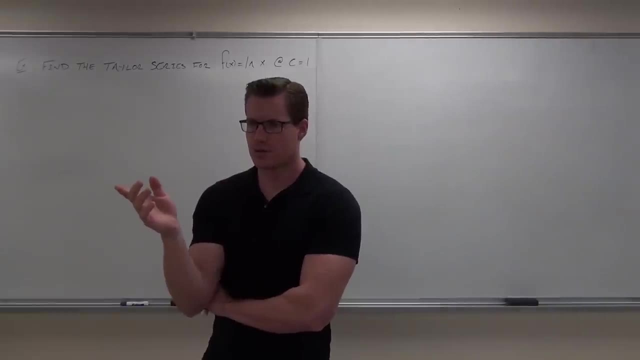 I want you to read those steps to me. What's the first step in finding a Taylor or Maclaurin series? What should we do first? How many derivatives, You know what? As many as it takes for you to find the pattern. 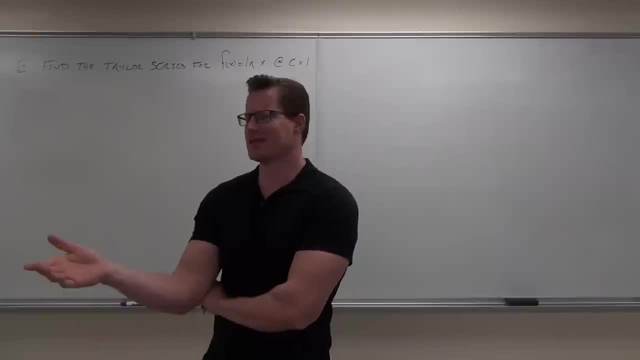 If you can find a pattern on the first derivative, fine, Like e to the x. It was really easy On some of them. you can't do that, So do 3,, 4,, 5, however many it takes to actually find the pattern. 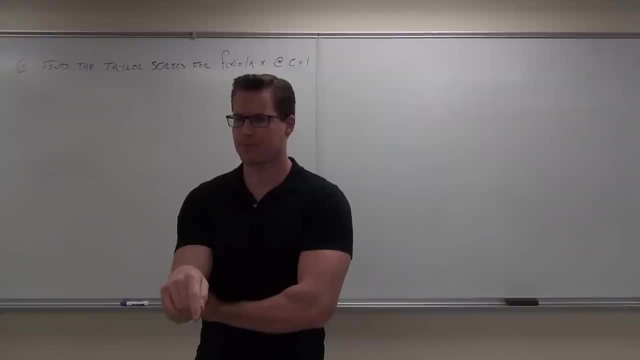 Do derivatives. What's the step after that? Plug in: x equals 1.. Very good, In our case, x equals well, c equals 1.. That's going to be our c, So we're going to be plugging in 1.. 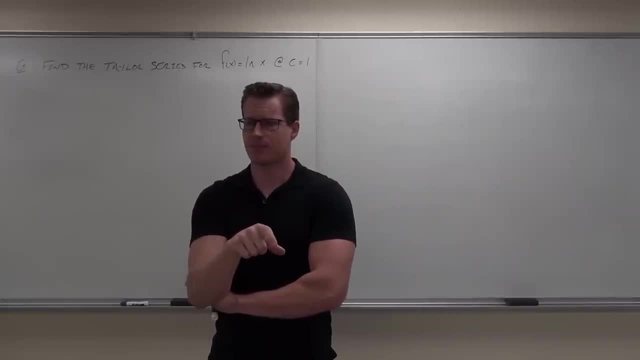 And then we find a pattern for that. After that, Set up your series- Good. And after we set up our series, we're looking for Interval- Very good, It's going to be a function, right? We've got to find out the domain of our function. 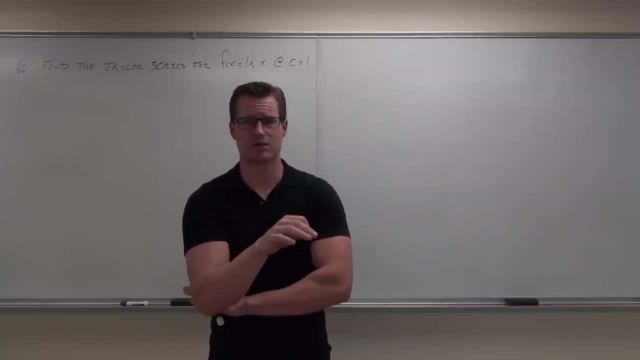 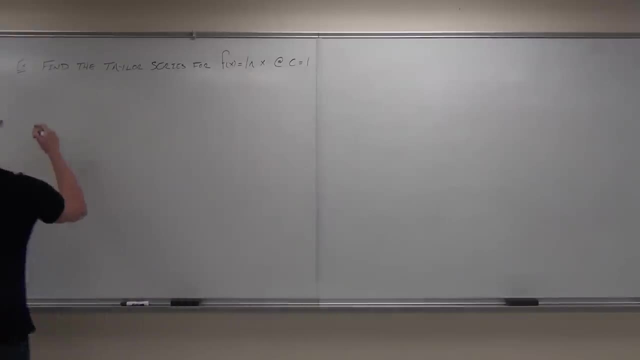 That is the interval for which our series converges, which our power series converges. All right, All right. So, step one, let's go ahead and let's find some derivatives. We always start with the function itself, like ln of x. 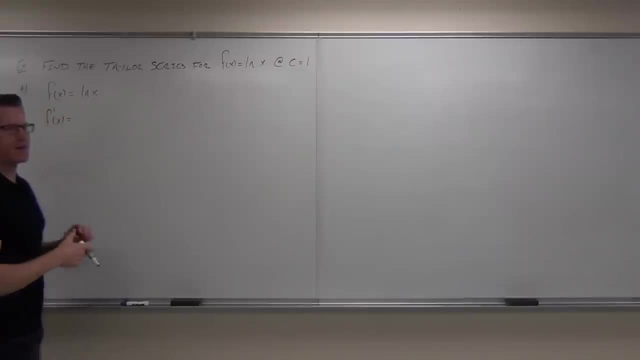 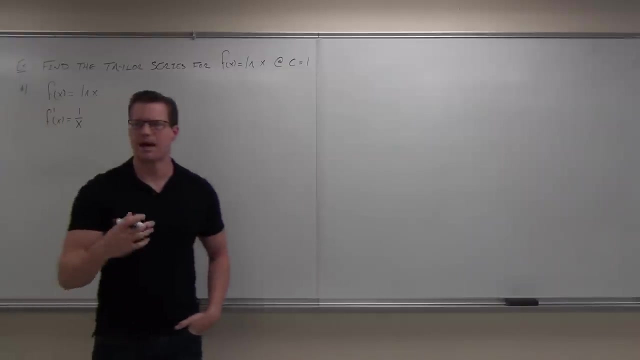 After that, Well, we start taking first derivative. second derivative: Hey everybody, What's the derivative of ln? x, please, 1 over x. Good, Now, I'm going to write that differently because we're going to be looking for a pattern here. 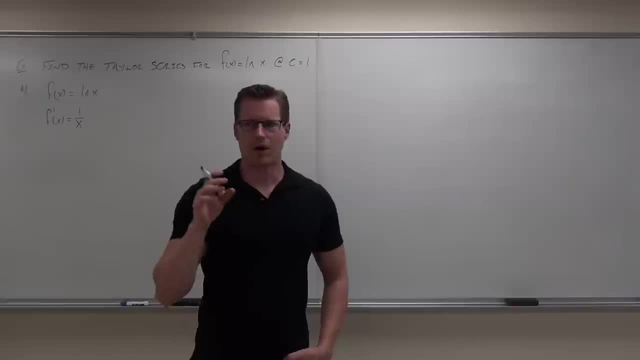 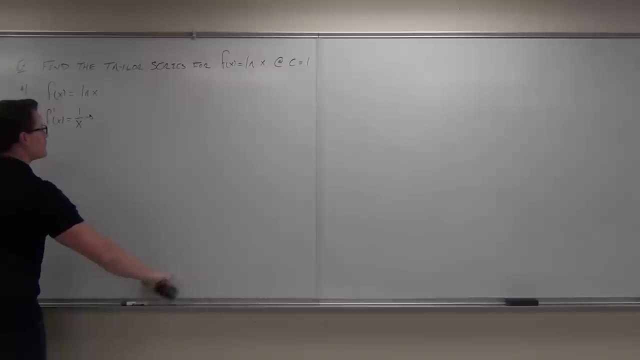 So when I do 1 over x, usually I want x to some power, not 1 over x. So I'm going to write this instead: x minus x to the power of 1.. Yeah, x to the negative 1 power. 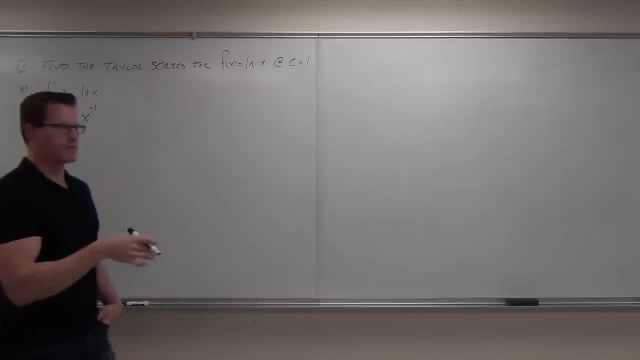 So let's write this as x to the negative 1.. That's going to make our derivatives a little bit easier if we go down the way, And it's going to make us find a pattern pretty quickly. Are you with me? Yeah? 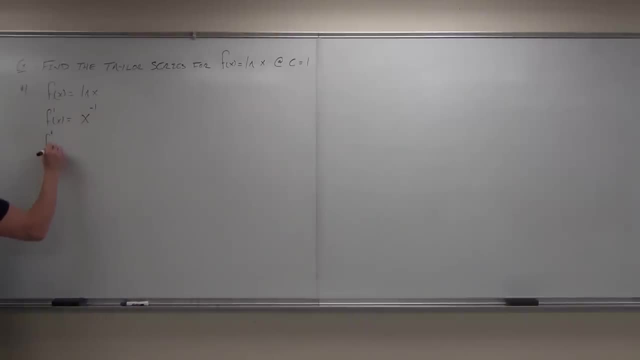 OK, so we're going to go fast through this stuff. Hang on to your hats here. What's the second derivative, please? Negative x to the negative 2.. OK, I'm going to write negative 1 x to the negative 2.. 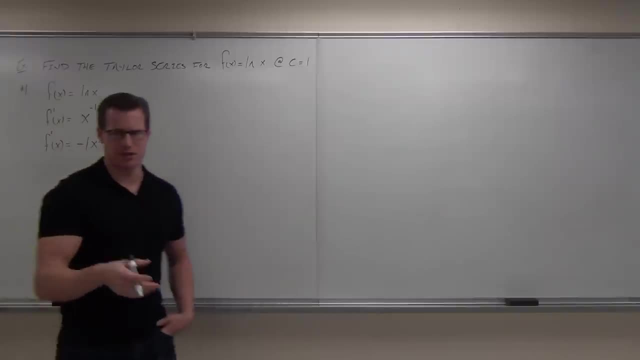 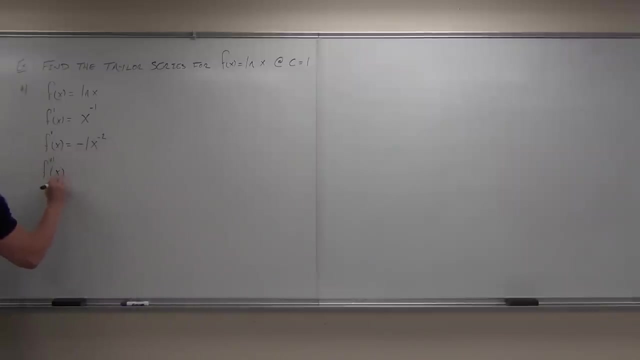 Is that OK with you? Yeah, And here's why we're going to do that. When you're doing this, when you're doing your derivatives, do not do things like this. When you do a third derivative, I don't want you to multiply the negative 1 times the negative 2. 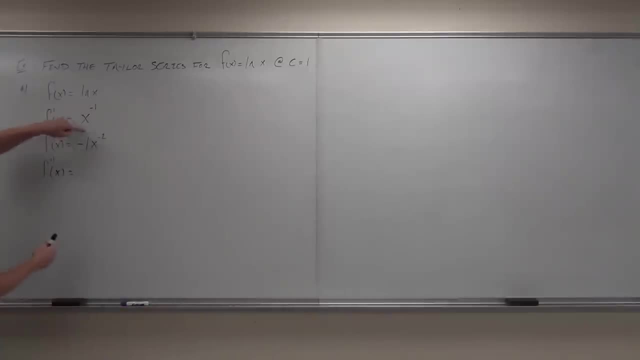 and get 2.. I want you to look for a pattern. Yeah, a negative times negative is a positive, But really we're going to get 2 times 1, x to the negative 3.. Does that make sense to you? 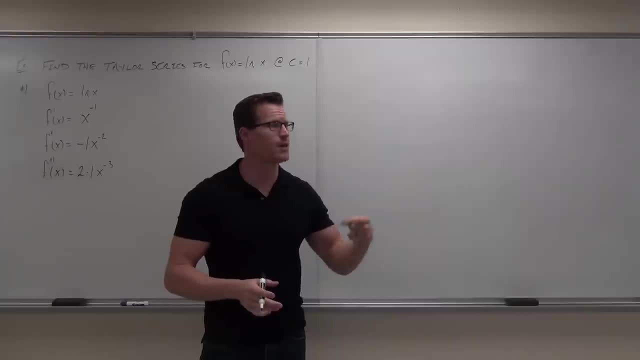 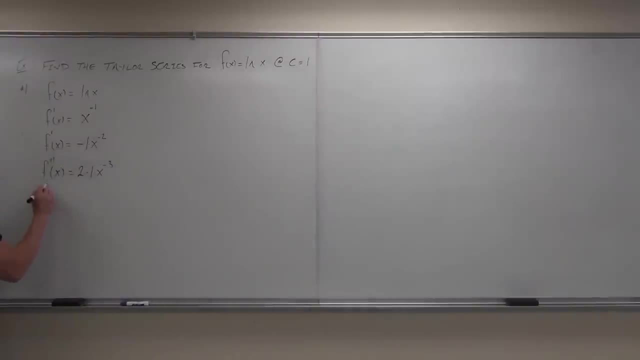 Are you with me? Remember, you're looking for patterns here. You're looking to make a pattern out of this guy, not to get the number. to get a pattern, Let's do a fourth derivative and a fifth derivative And then we'll find it. 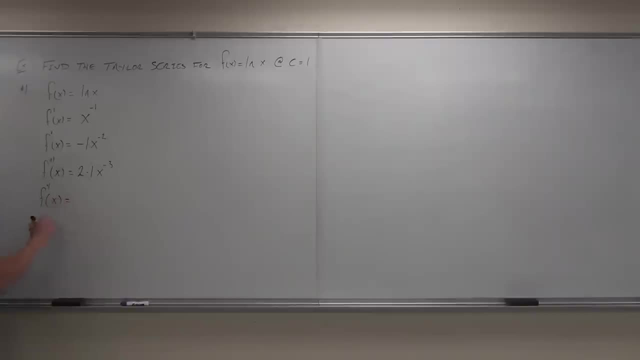 So the fourth derivative of x, we write a little 4 up there. What's going to happen? It's going to be negative, Very good, And it's going to be 3 times 2 times 1 times x to the negative 4.. 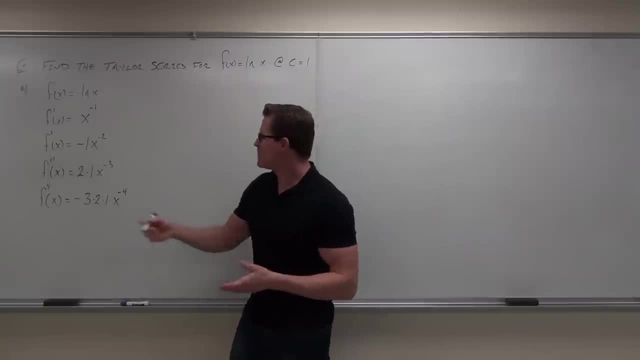 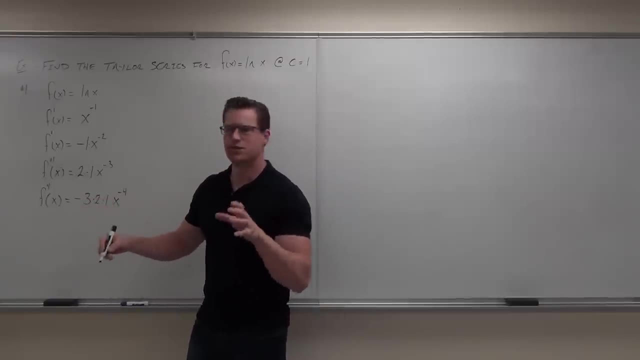 Does that make sense to you? Do you see what's happening? Had I put 1,, 1,, 2,, 6, you would not have seen a pattern here. Does that make sense? So when you're doing this, don't do that. 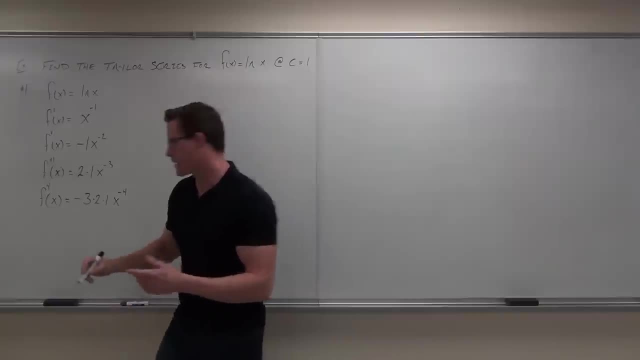 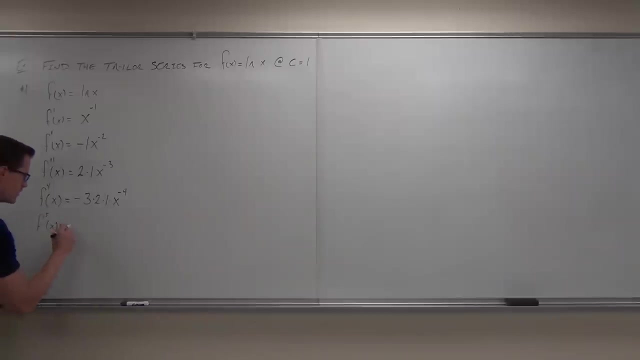 Don't do 1, 1,, 2,, 6,, 20, whatever you're getting OK. So let's do one more, The fifth derivative of x we're going to get. is it positive or negative? Positive: 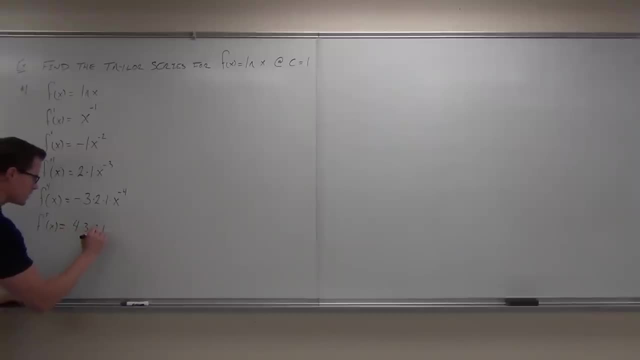 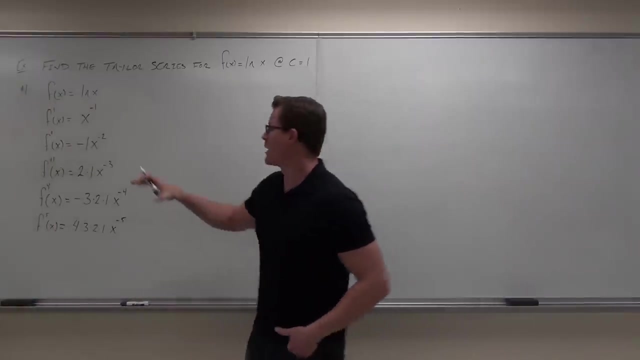 So we're going to get positive and then 4 times, 3 times, 2 times, 1 times x to the negative. Very good, Do you see your pattern? Yes, Tell me something about your pattern right now as far as the sign goes. 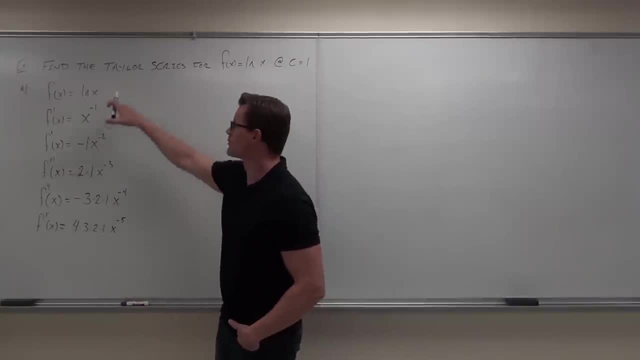 Also, do you notice something? Our pattern does not start with our first term. This is not part of our pattern. This doesn't even work with it. It has no exponent at all. So we're going to. We can start our pattern after the first term. 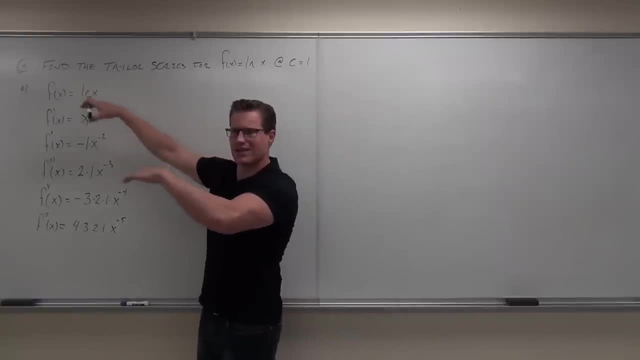 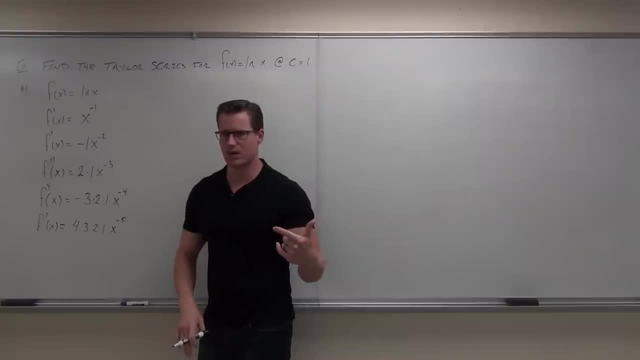 That's going to be something and it's going to be alternating. Do you guys see the alternating I'm talking about? Secondly, tell me something about my exponent: Decreases by 1.. Decreases by 1, that's right. 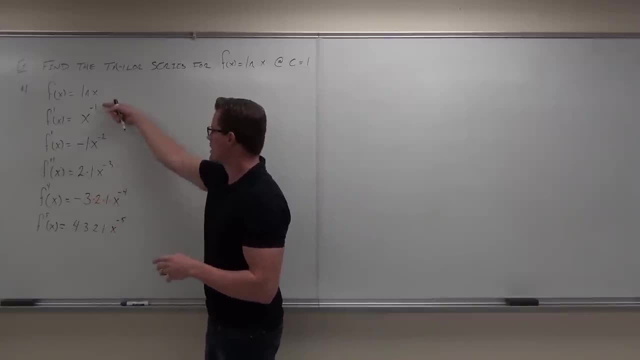 So it's negative if you want to see the absolute value increases, sure, So negative 1, negative 2, negative 3, negative 4, negative 5.. Now tell me how it relates to the derivative that we are taking. 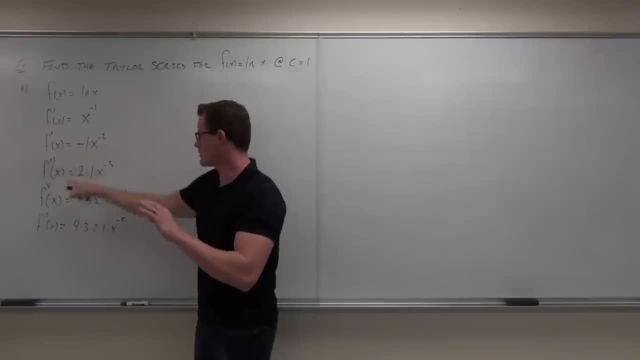 To the derivative that we're taking here is 3, negative 3, 4, negative 4, 5, negative 5, the same one. Next one will be 6, negative 6.. Does that make sense? Yes, 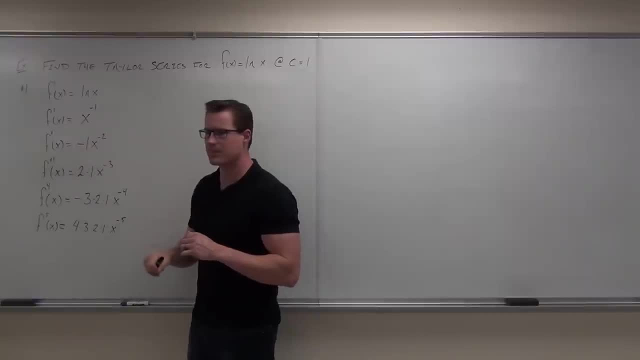 OK, Tell me something about the coefficient of my x's. What's it doing? It's a factorial. That's right Now. is it n factorial? Is it the power factorial? Is this 4,, 3, 2, 1?? 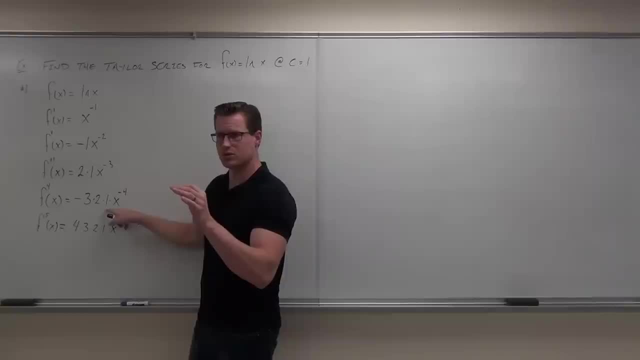 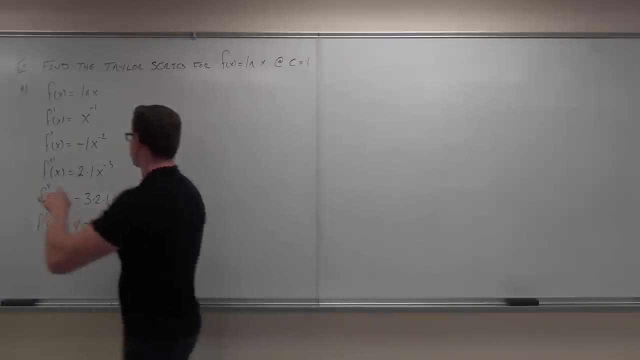 Oh yeah, It's n minus 1.. Right, So it's really close, but it's still a factorial, but it's 1 less than the power we have. Does that make sense? Yeah, Let's check it out. 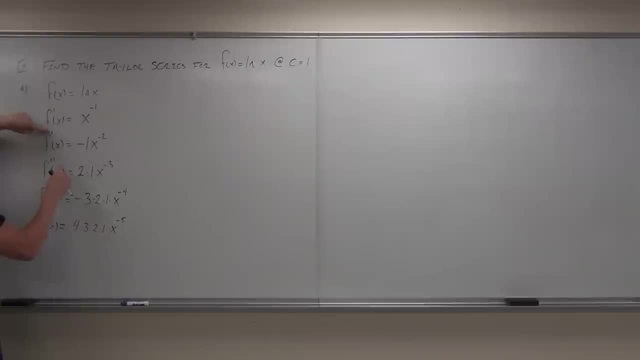 If I omit the negatives and positives, this is 2 minus 1 factorial. Sure, Is this 3 minus 1 factorial? Is this 4 minus 1 factorial And 5 minus 1 factorial And 1 minus 1 factorial. 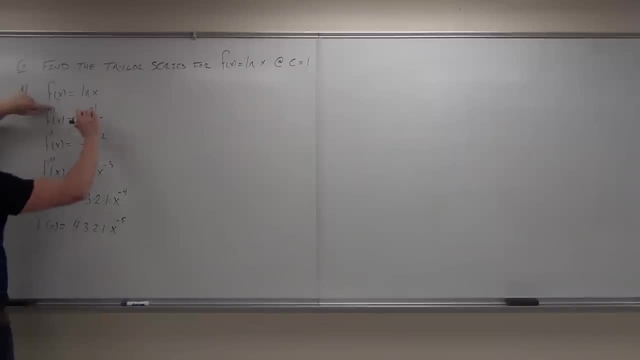 Zero factorial. Yeah, Zero factorial is 1.. Zero, Zero. OK, So we could do the nth derivative right now. What we know is that it's alternating, Yeah, it's alternating. It says it's going to be negative. 1 to some power. 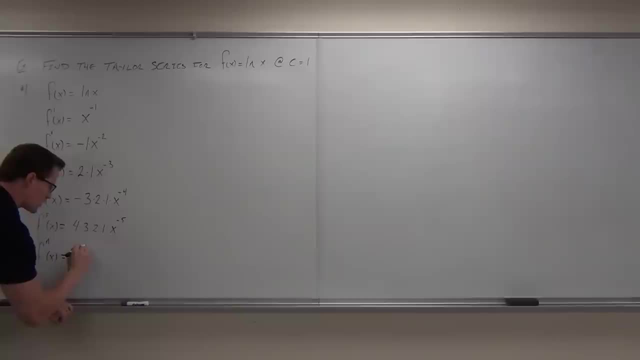 We just got to make sure it starts correctly for us. So we're going to have n or n minus 1 up here somewhere. We'll deal with that in just a second. OK, Next up: well, we're going to have: 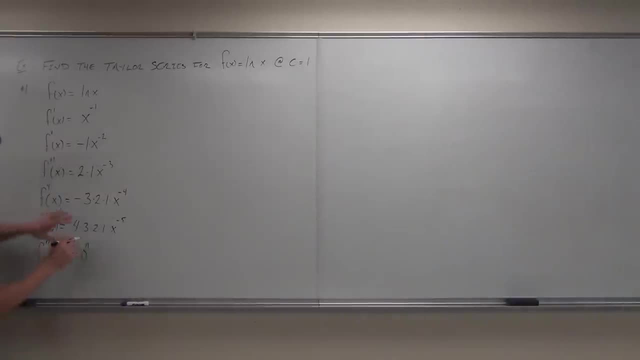 How do I represent this? n minus 1- factorial. OK, So if I get rid of all the negatives today, I don't even care about those. we're going to have an n minus 1 factorial. Yeah, We're going to have an n minus 1, factorial, for sure. and then x to the negative n power. 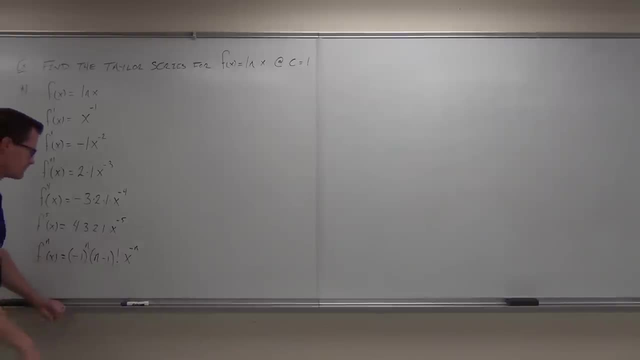 Does that make sense to you? Yeah, You're sure. Uh-huh. Okay, Now this part's what I'm worried about. How can I represent? because right here it goes positive, positive. so let's just let's. 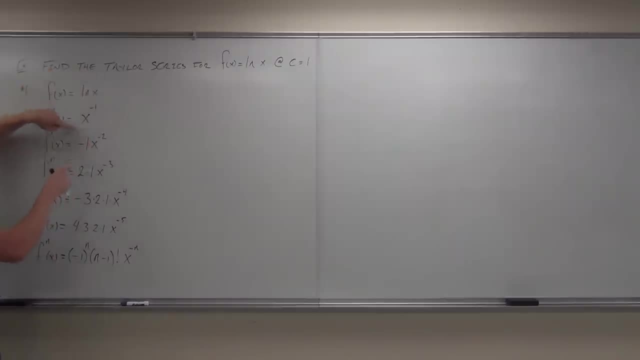 forget about this one. Let's look just here. So I don't want positive, positive, negative, positive, positive. that doesn't really work for us, That's not our pattern. So our pattern doesn't really start until our first derivative term. 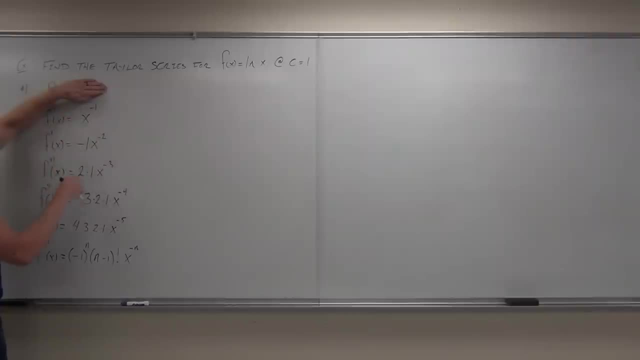 So omit that. How can I make it positive, negative, positive, negative, positive, negative. How can I start that off? Is it negative 1 to the n or negative 1 to the n minus 1, if I start at, n equals 1?. 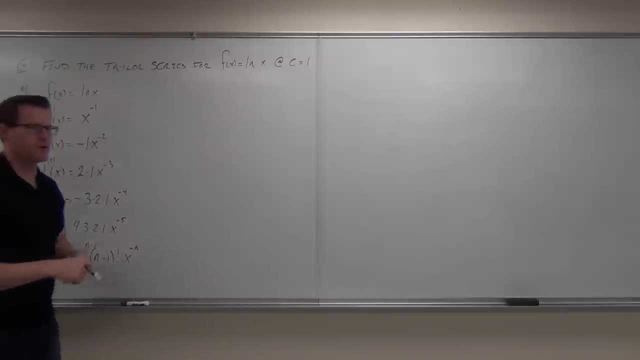 N minus 1.. N minus 1.. That's right. And you know what, If you're not good at thinking, man, I don't really, I don't know. well, if you can't find a pattern here, that's okay. 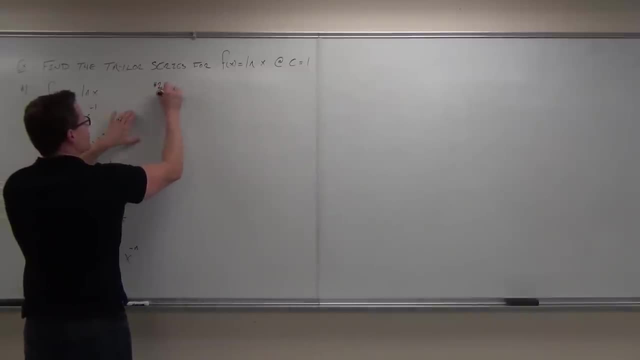 What you're really looking for. What you're looking for is step number 2, plug in the numbers. Here's f of. I'm sorry, what are we plugging in? even 1.. Plugging in 1.. Okay, so, f of 1, and f prime of 1, and f double prime of 1, and plug them all in for. 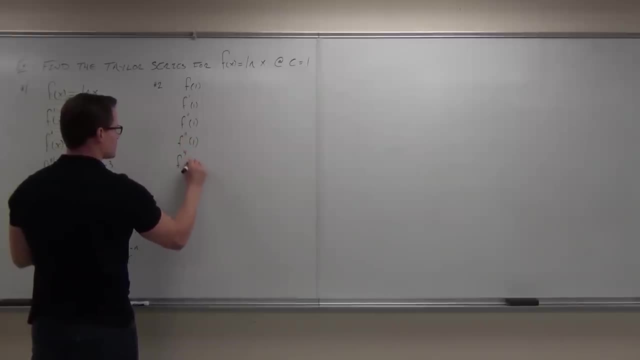 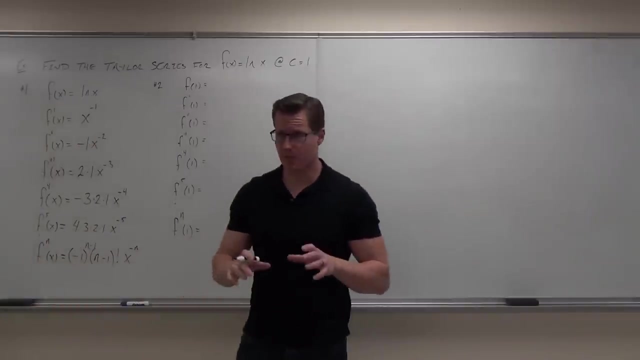 1. It's got to follow the same pattern. Okay, So it's got to be alternating. It's still going to have a factorial somewhere in there. That's why we did this is to look for the pattern and make sure it's still the same. 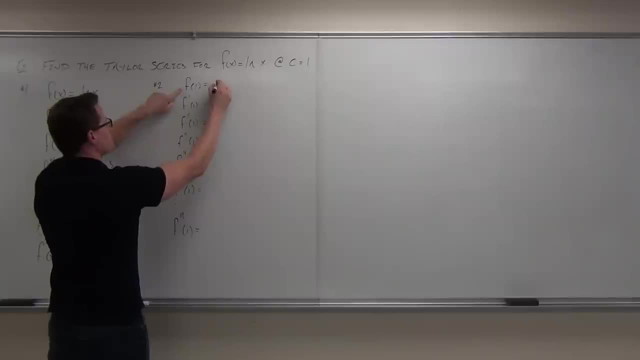 Okay, So check it out. f of 1 is what is it? 0. 0. Good, Because if I plug in 1, I get 0.. Now we just determined that's not going to be part of our pattern, so we're going to. 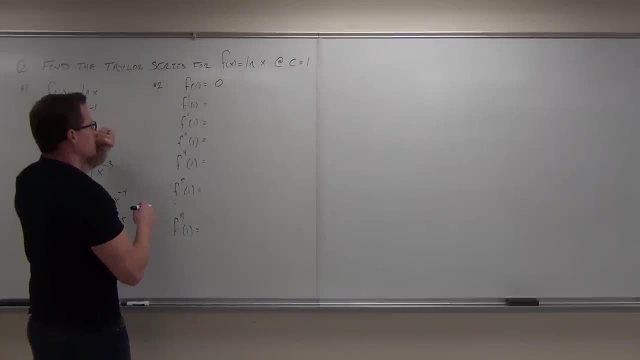 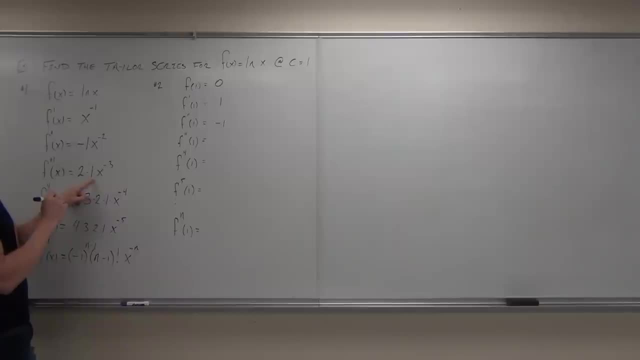 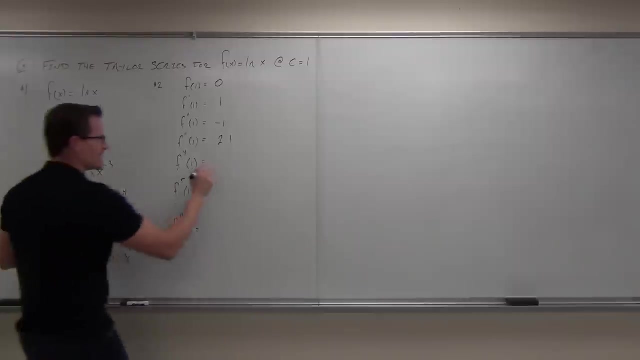 Negative 1. Negative 1. Negative 1. Plus 1. And then we're going to get 2 times 1.. If I plug in 1, you're going to get 2 times 1.. Plug in 1, you're going to get negative 3 times, 2 times 1.. 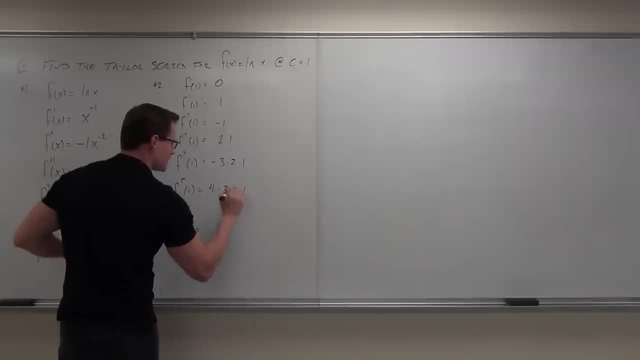 Plug in 1, you're going to get positive 4 times, 3 times, 2 times 1.. Do you guys see that all we're getting here is this series of numbers that are being multiplied together? We don't have any more x's, because 1 to any power is still 1, so, basically, if you just 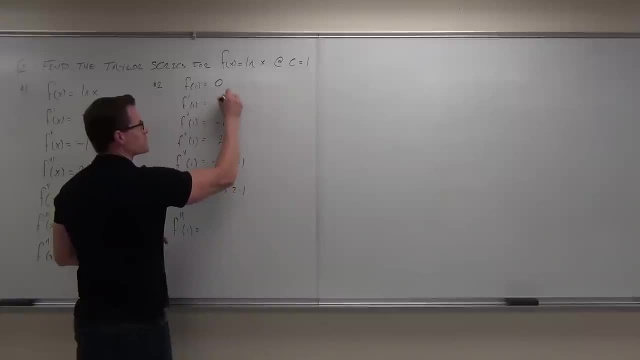 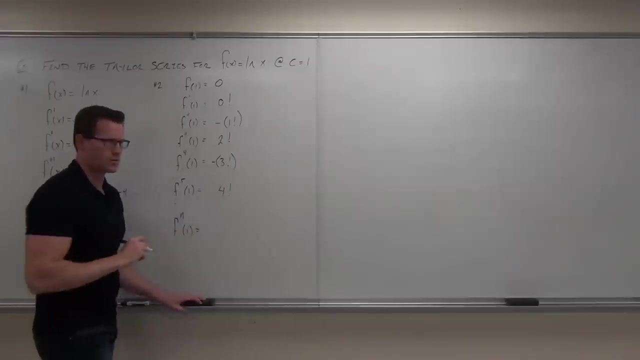 omit your x's, this will be good Again. this happens to be zero factorial. This happens to be negative one factorial. This is positive two factorial. This is negative three factorial. This is positive four factorial. You with me still, Is it still alternating? 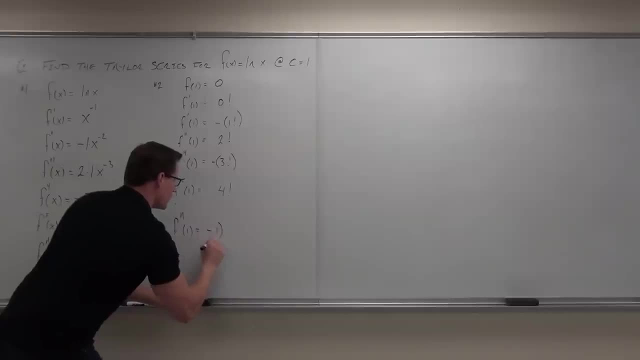 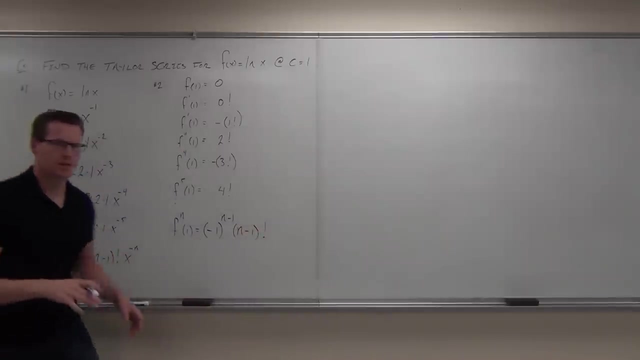 Does it still have a factorial? In fact, this is gonna be negative one to the n minus one and then n minus one factorial. You can see something here as well. Check this out If you're good enough to find a pattern, which some of you are and some of you. 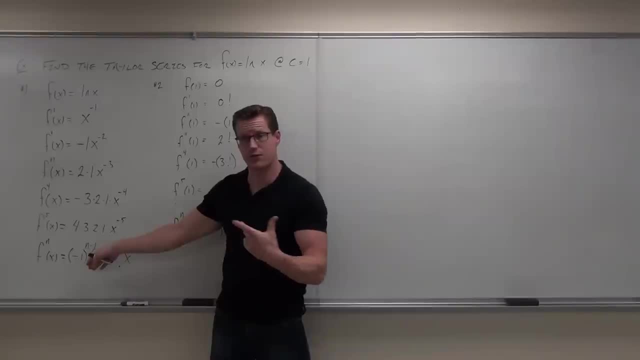 maybe are gonna struggle with this. this is kinda hard to do in general, If you follow the steps I've given you. try not to get just the numbers. Try to find your pattern. This becomes a lot easier. okay, But look at this. 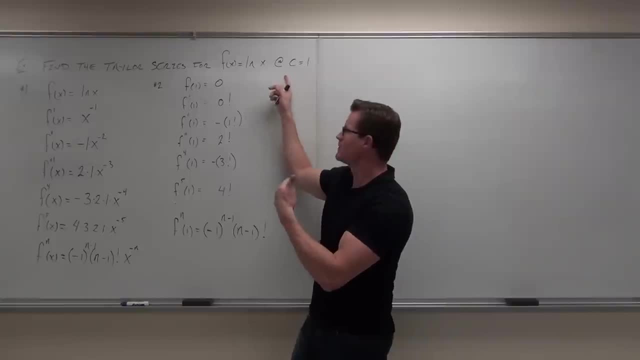 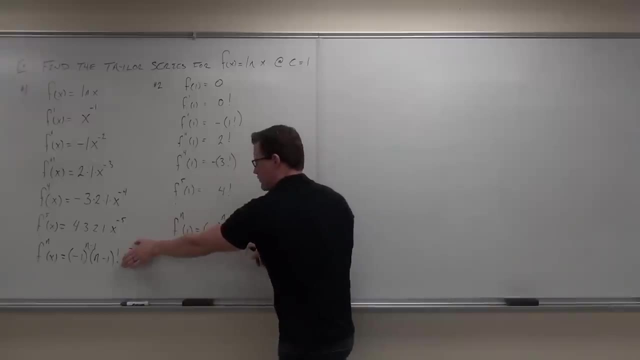 If I take my x equals one, that's my c. okay, Take my x equals c, which in this case is one, and I plug it in. Do you see that if I plug in one here, I get exactly what we found over here? 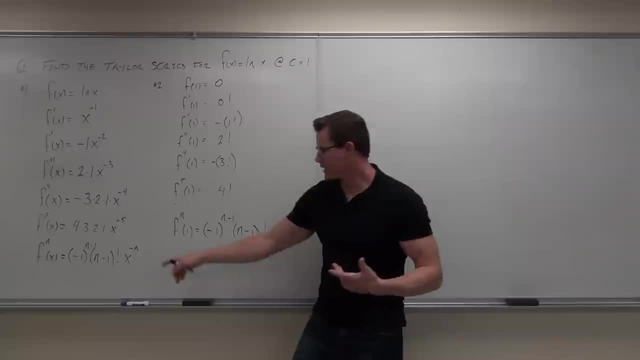 Hello, do you see that It's gotta be the same. So if I plug in one, if I plug in one, I'm still gonna get the same thing, if I found my pattern correctly. Now, if that's our n power of f at one, 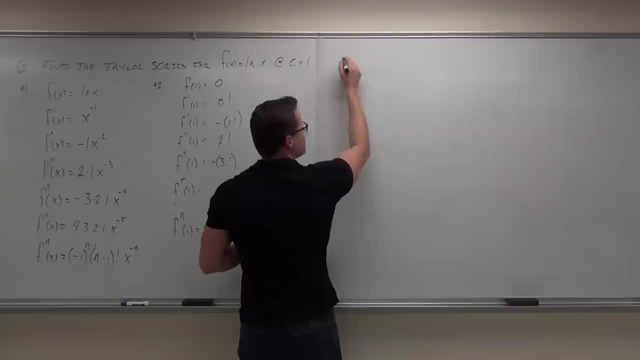 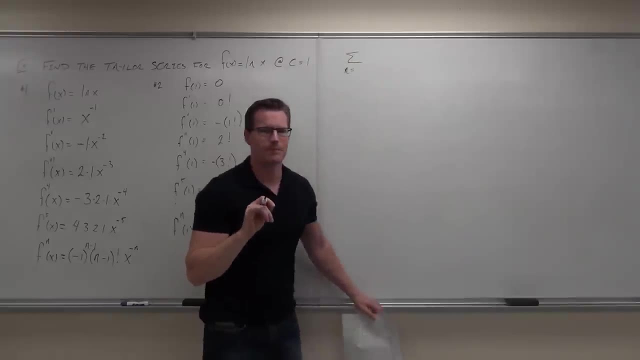 then here's what we're looking for. What we know is that a Taylor series must look like this. Our Taylor series has to be n equals. in this case- listen, in this case, we're not gonna start at the zero term. 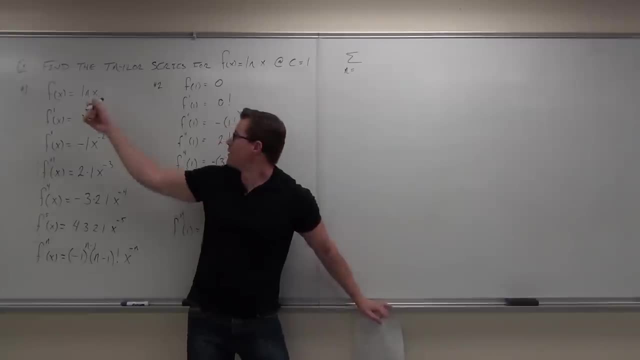 Are you listening? We're not gonna start at the zero term, because if I start at the zero term, that's this guy and that's not following our pattern. So we're gonna change to n equals one. You're gonna see another reason why in just a minute. 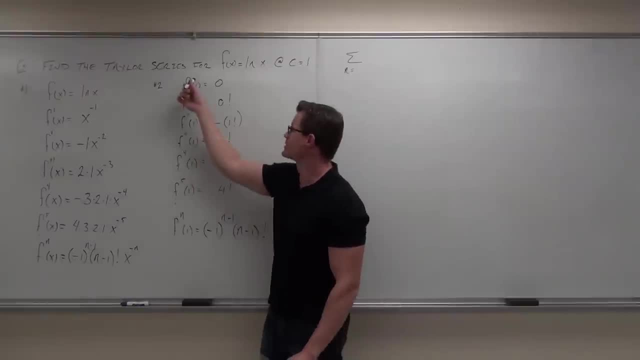 So we're not gonna start at zero, We're gonna start at one, because our pattern doesn't start until our n equals one. Does that make sense to you? Not n equals zero, not the zero derivative, not the function itself, but at n equals one. 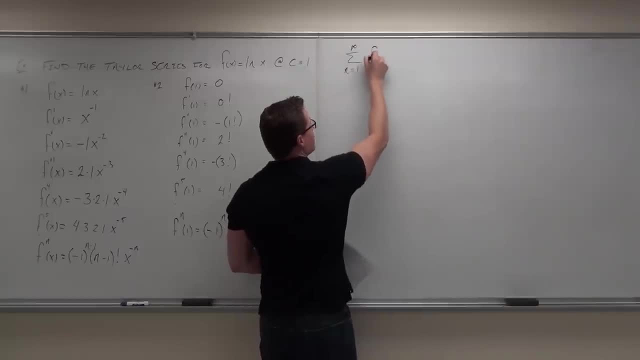 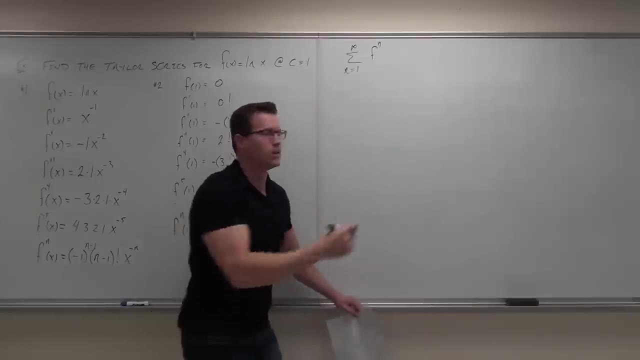 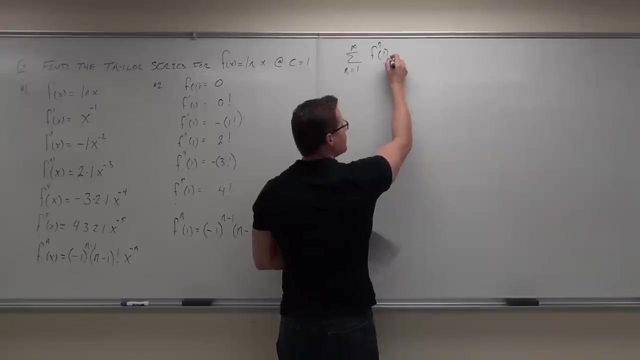 So one to infinity. we've gotta look like okay, the nth derivative at remember Taylor series C At C. Oh, what's our C right now? One, Okay, and then say what Times, x minus C to the n. 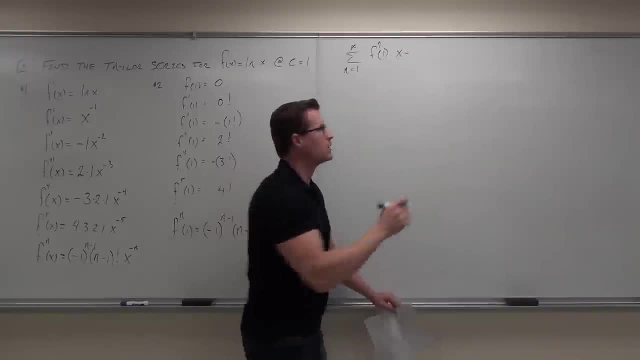 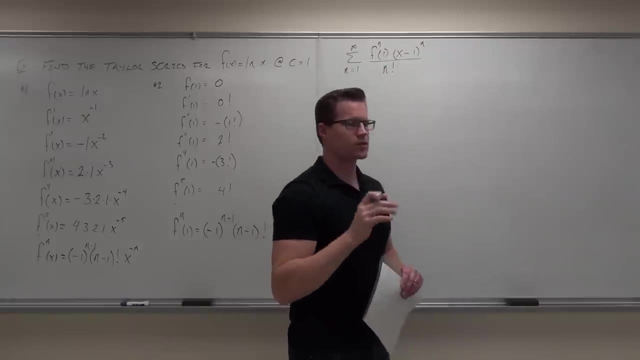 X minus okay. x minus C, very good. X minus One, Two of them And n Over And factorial- Perfect Show of hands. let's see what we can do with that. so far, So we found our derivatives. 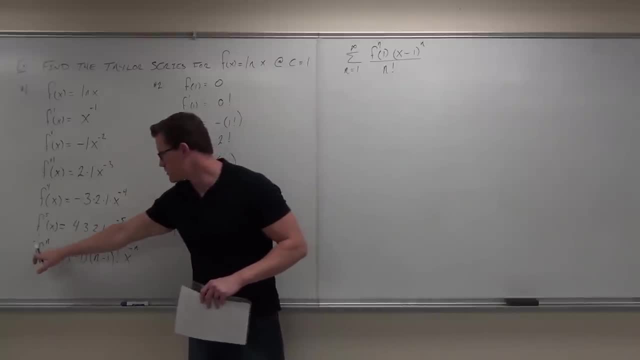 We actually found a pattern to it. If you find a pattern, if you find the nth derivative of f at x, then all you need to do, all you need to do, is plug in your center. If it's zero, plug in zero. 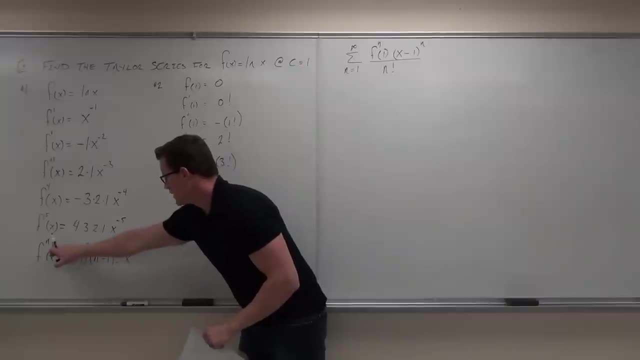 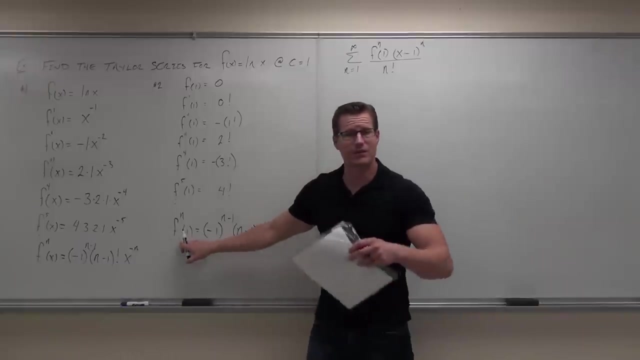 If it's one, plug in one And you automatically get the nth derivative of f at one if you simply plug in one. That's literally what this means. Now I've given you both these steps, because if you can't do this, 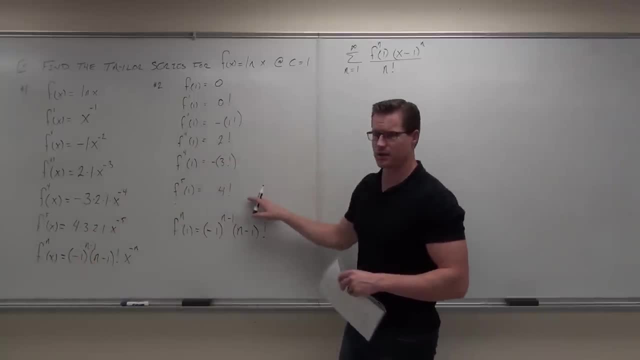 if you can't find the pattern, sometimes you will find a pattern just from plugging in the number. This is really what we're looking for anyway. So if you can't find the pattern here, use this to plug in your numbers and then find a pattern from these numbers. 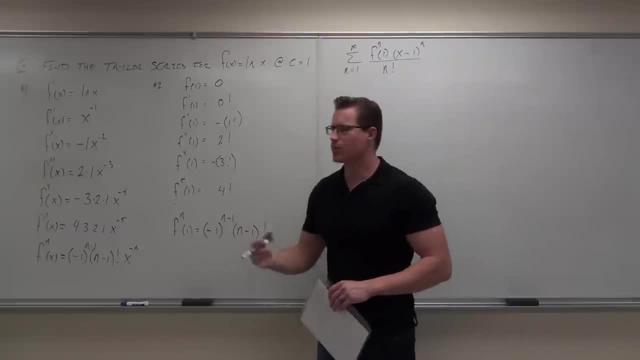 Show of hands, feel okay with that idea. Once you do that, understand that what we're trying to do here is do a Taylor series or a Maclaurin. if we're centered at zero, Taylor series are always. nth derivative of f. 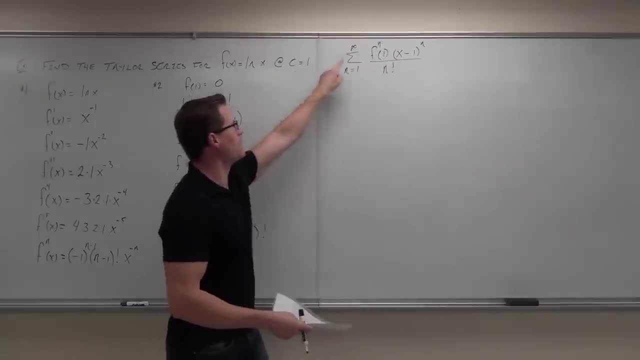 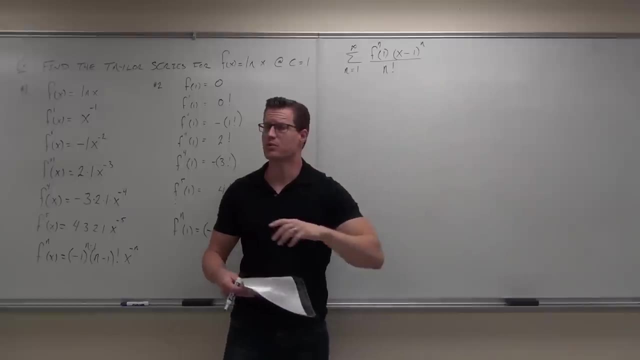 at your point C, at your center. Well, that would be at one. Hey, we already found that. Then it's x minus your center, x minus one to the nth power over n factorial. We proved it last time, So all we gotta do now is what. 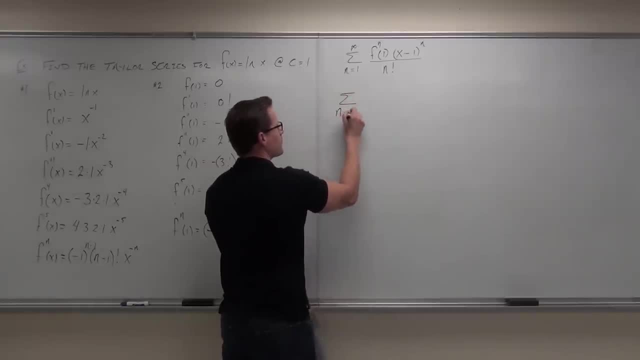 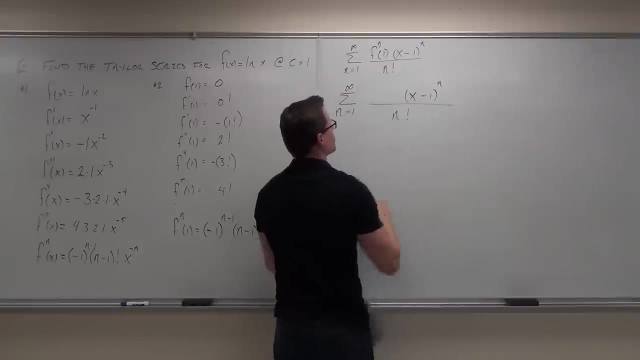 Let's make a substitution. So our Taylor series, therefore, is gonna be: n equals one to infinity. I know I'm gonna have an x minus one to the n over n factorial. Can you please tell me what goes here? Have I lost you? 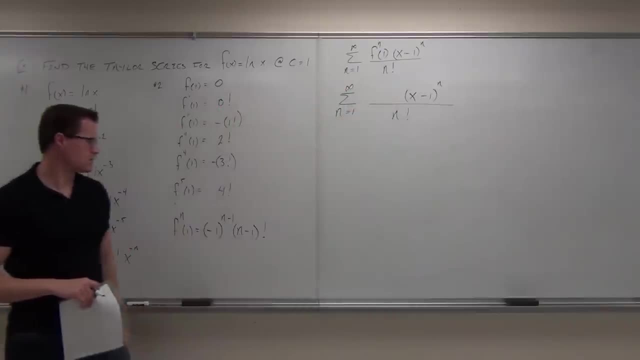 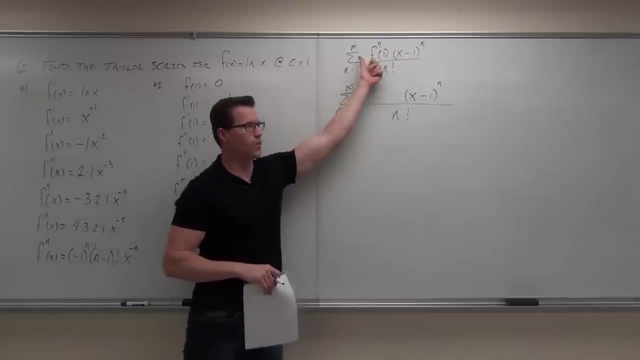 No, What goes there then? Negative one to the power, n minus one. Perfect, That's exactly right. It's literally this thing If the nth derivative of f, evaluated at one, is this, which we found in two different ways really. 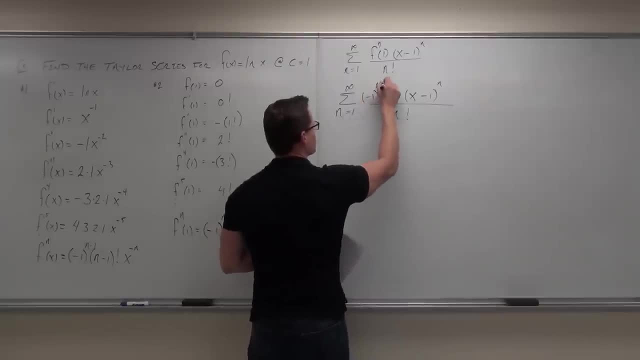 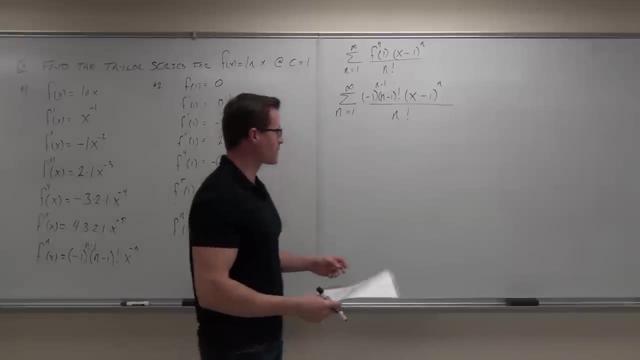 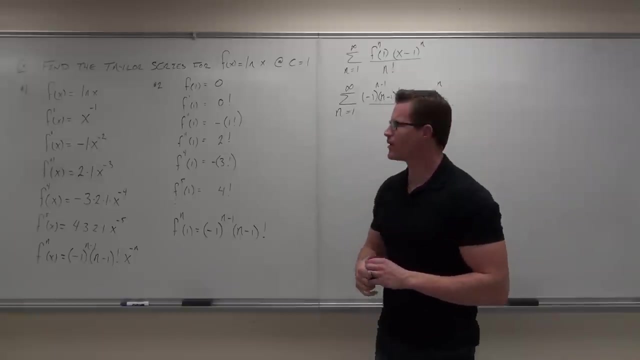 then we're gonna plug that in. So negative one to the n minus one times n minus one factorial. Okay, I really do need to make sure that you're okay with this. so far, I don't think I'm gonna give you any sort of recap. 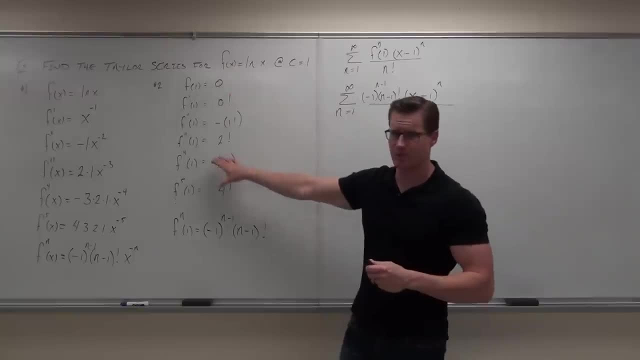 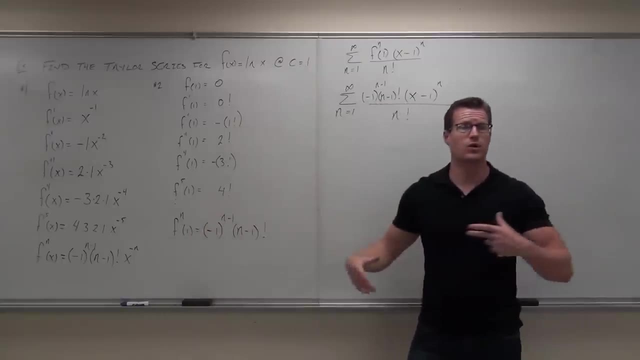 I've done it a couple times here: Derivatives- Find a pattern. plug in numbers- find a pattern. This is what you're looking for. The reason why you're looking for this, evaluated at this point, is because that is what a Taylor polynomial is all about. 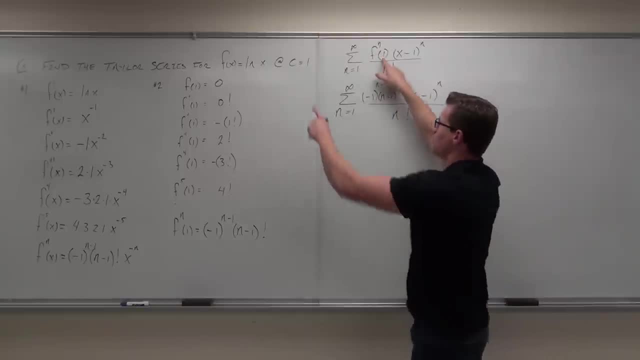 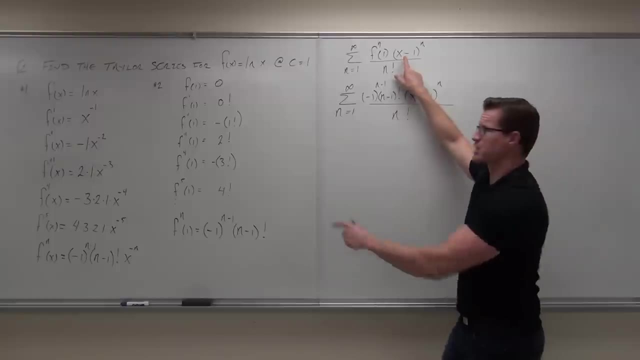 It says: find your nth derivative, evaluated at whatever your c is equal to. We have that. Make your substitution. These guys are always the same: It's x minus your center, x minus your c, evaluated at some power n over n. factorial. 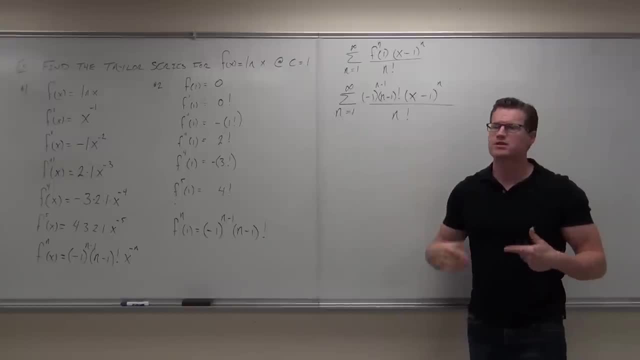 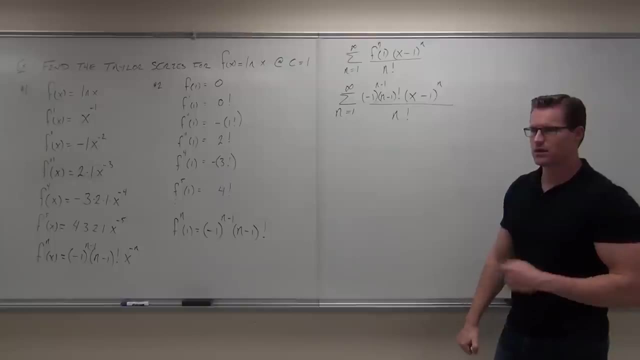 Do you really feel okay, getting that far? Now, before you go any farther, simplify it if you can. For instance, I've got an n minus one factorial over an n. I should be able to simplify that. Can you simplify n minus one factorial over n? 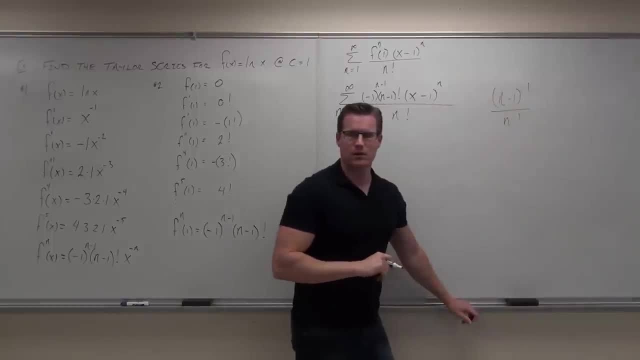 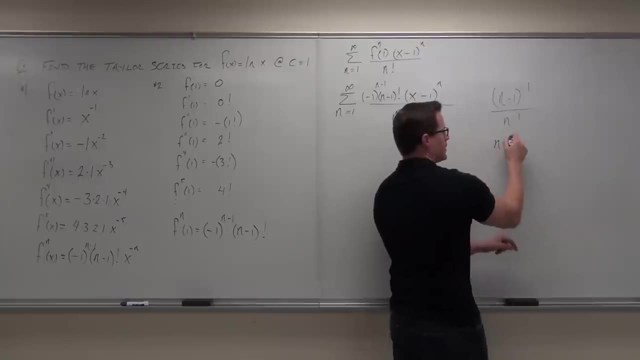 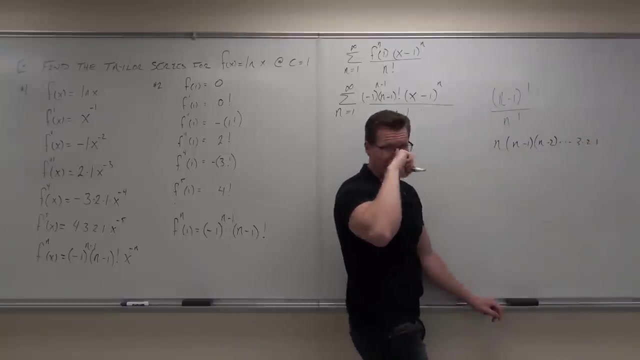 Factorial. You're left with n minus one. You're not left with n minus one. You're left with n? n. factorial is n times n minus one times n minus two times, all the way down to three two one. Are you with me? 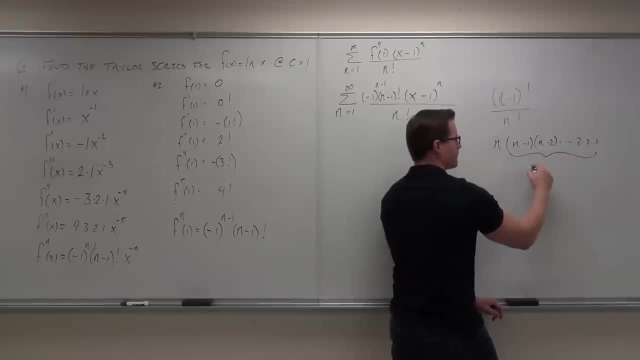 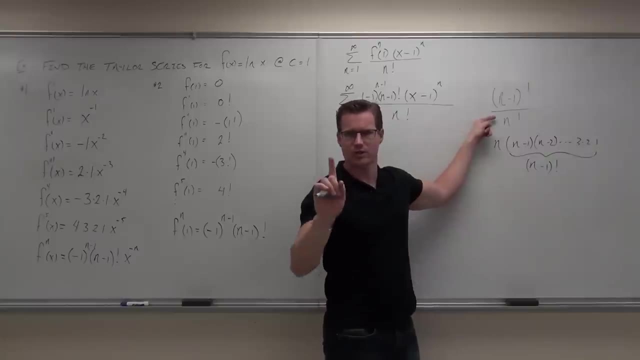 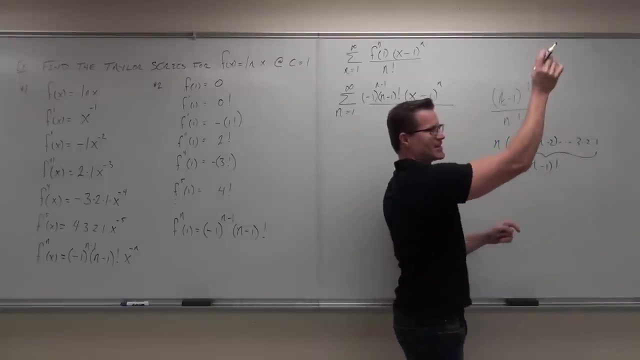 Look at this, Look at this. What's that? n factorial, n minus one factorial. So n factorial is bigger than n minus one factorial by one term, by multiplication by n. Does that make sense to you? So don't jump the gun and go. phew, phew, n minus one. 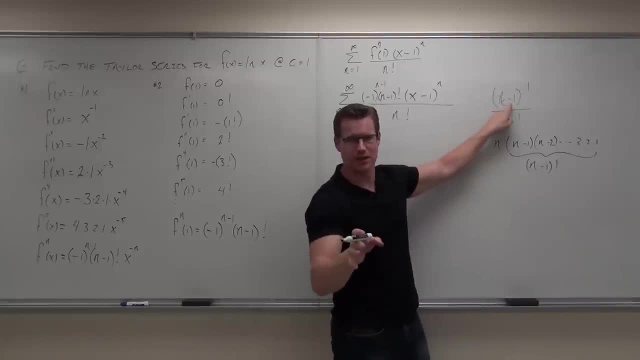 No, this is less than that. If this would have been n plus one, then yes, n plus one would be up here, But it's not. This is n minus one factorial. This is n minus one factorial times n. Therefore this: 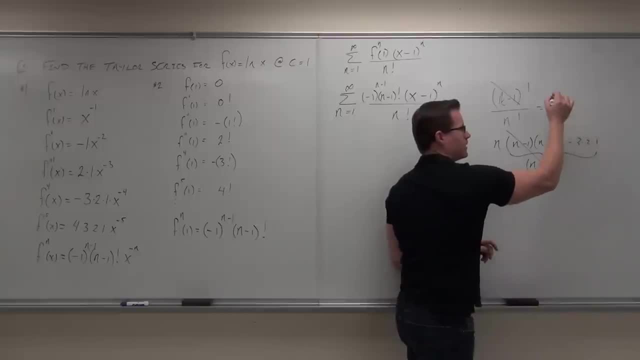 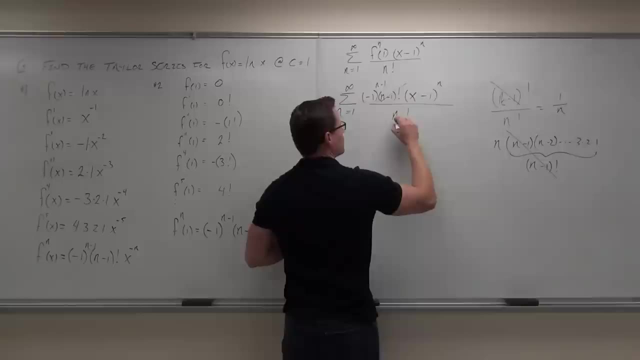 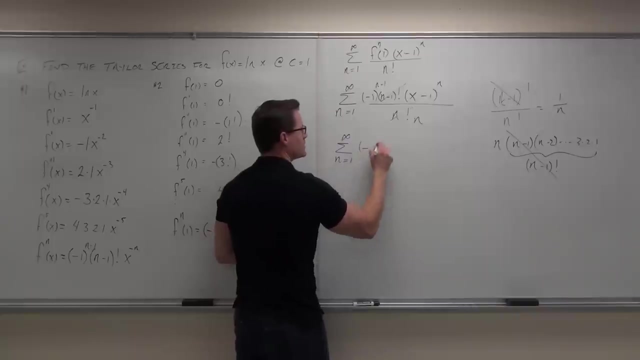 Get simplified with all this and we get one over n. That's what we get. So this goes boom, boom n. So our Taylor series becomes one to infinity of negative. one to the n minus one times x. minus one to the n: all over n. 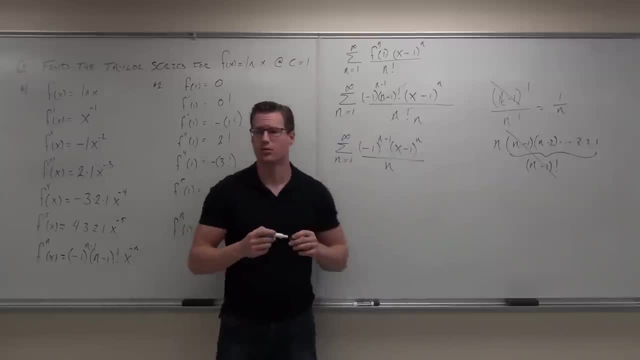 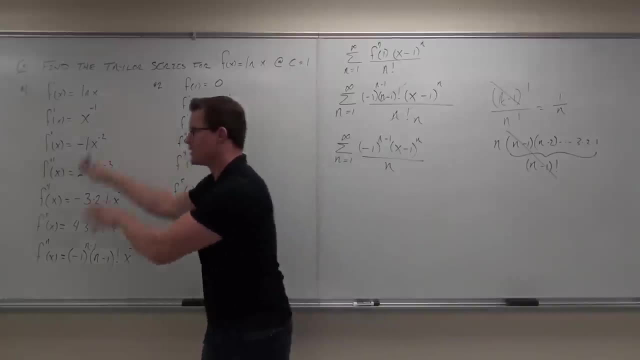 That's what we really want to work with. That's going to be nicer than working with this thing, for us for sure. Are we OK with this? Are we OK with that one? Yes, Are you sure? OK, so we've done derivatives, got it step one. 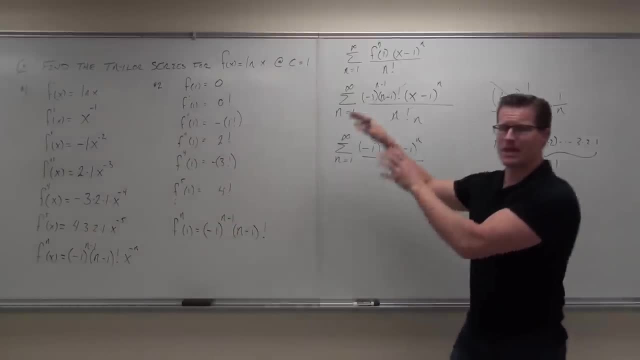 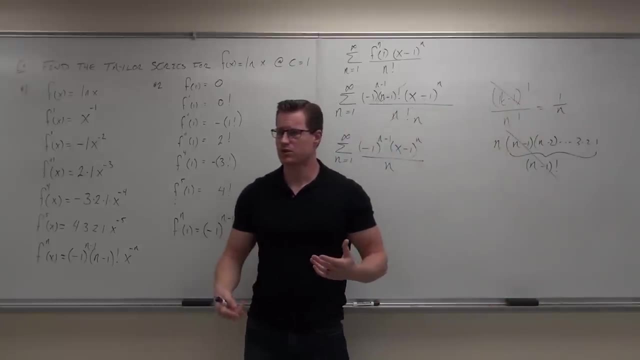 We've done plugging the numbers. step two: We've found a pattern, We've made our Taylor series. This is what we wanted to do. This was step number three. Now step number four: are we done with this? You've got to tell me where this thing converges. 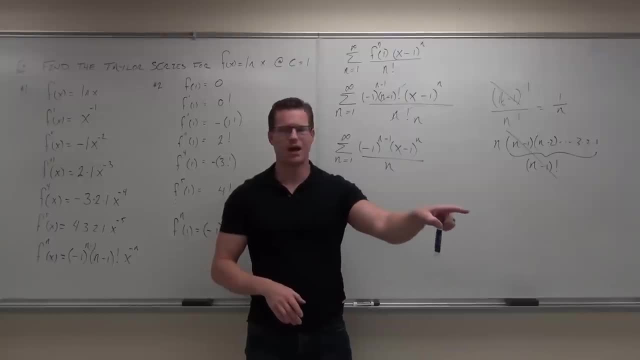 So what's the next step? Interval of convergence, very good. How, right side people, how are we going to do the interval of convergence? What would you use here? Absolutely the ratio test. For sure it's got well. it had a factorial. 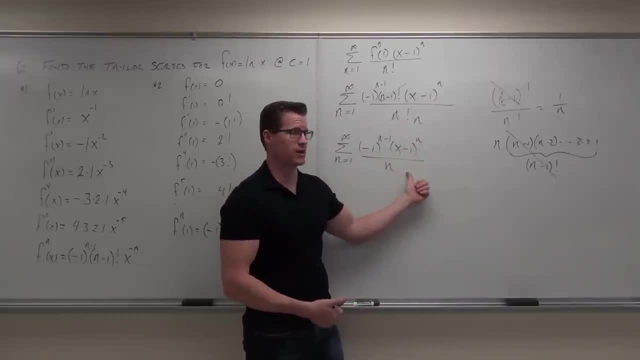 It's got a factorial, but it's got a power of n and something that doesn't have a power of n. You're not going to want to do a root test here. Do a ratio test Also. ratio test gives us a nice interval here. 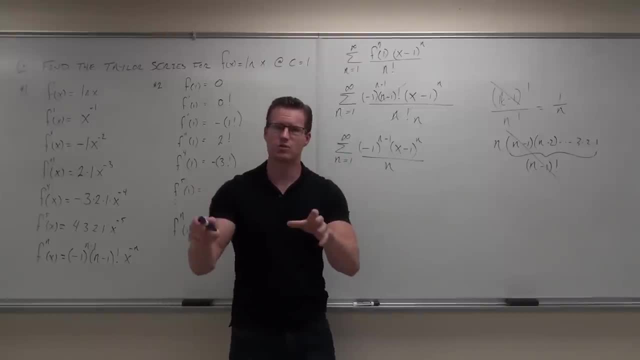 If we know that the limit is less than 1, we have convergence. Do the ratio test for me right now, please. Oh, by the way, one more reason why you can't start at n equals 0 here. Let me have your eyes on the board real fast. 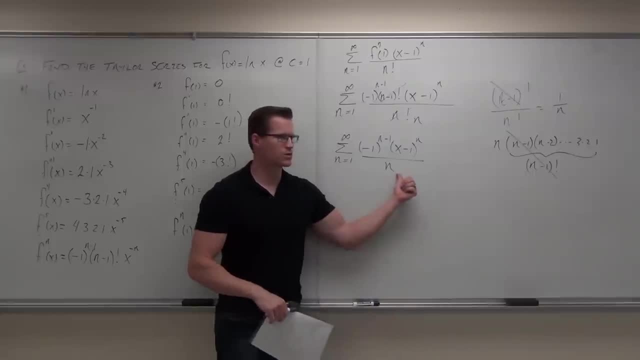 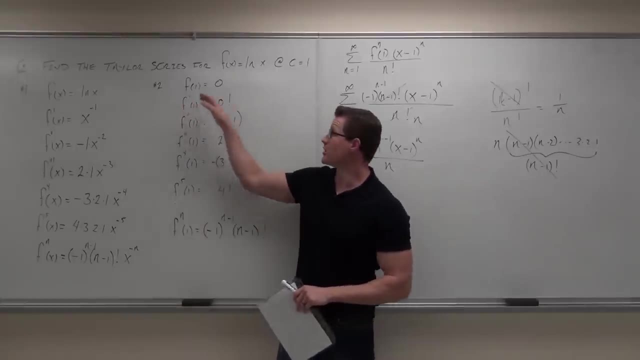 If you started at n equals 0,. what's wrong with this picture? You couldn't even do it all right, So we start at n equals 1,. firstly, because the pattern doesn't even start until the first derivative: n equals 1 derivative. 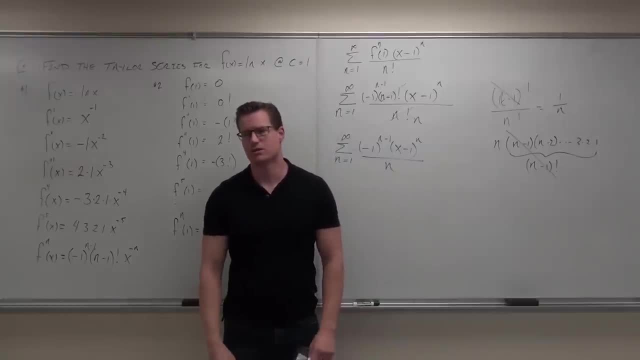 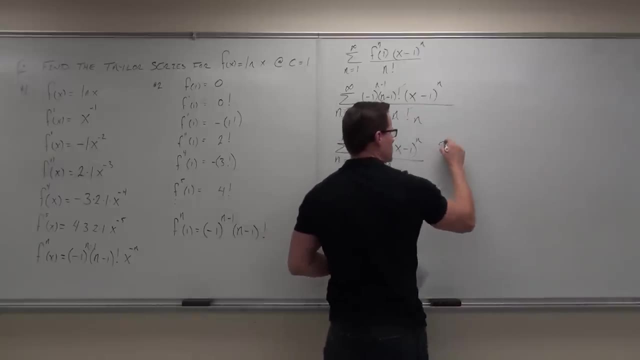 And also for the definition of having a defined series. here you can't even start at 0.. OK, so continue your ratio test. I'm going to go to my board here real quick, So we're going to do the ratio test. 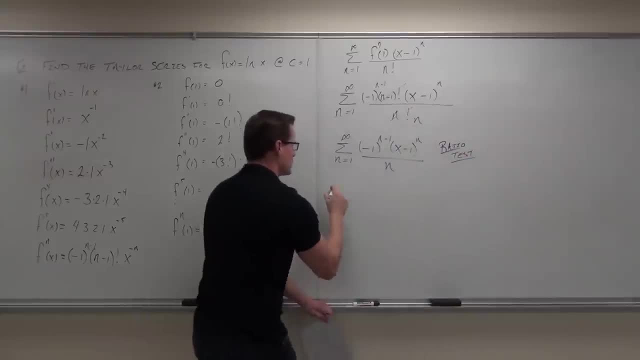 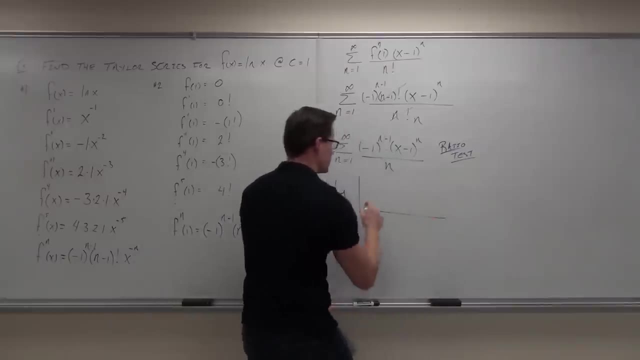 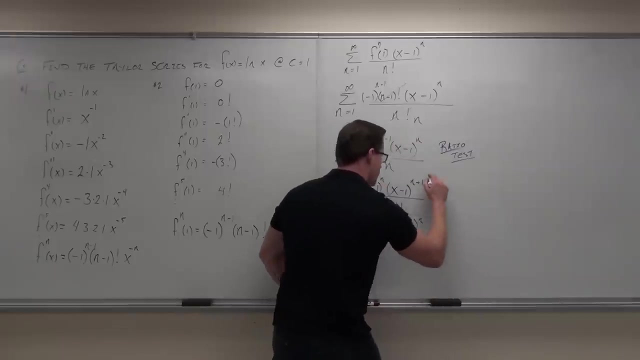 But I definitely want you to do it on your own, please. OK, We should be pretty much pros at doing the ratio test. I want to make sure you get the same thing I got. So can I have your eyes on the board here real quick? 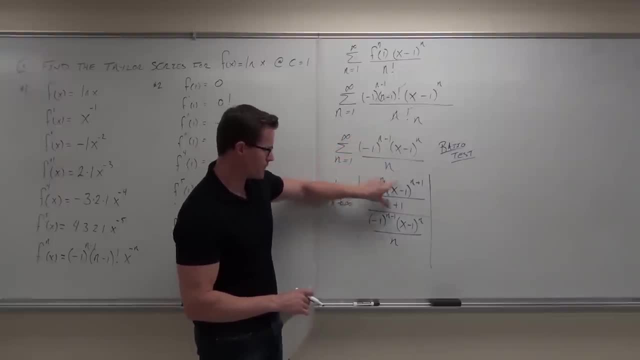 How many people did the AC? A sub n plus 1 term here, and you got this. And over a sub n term here, you got that Show of hands. if you got exactly that, Cool, What's the next step? What should you do? 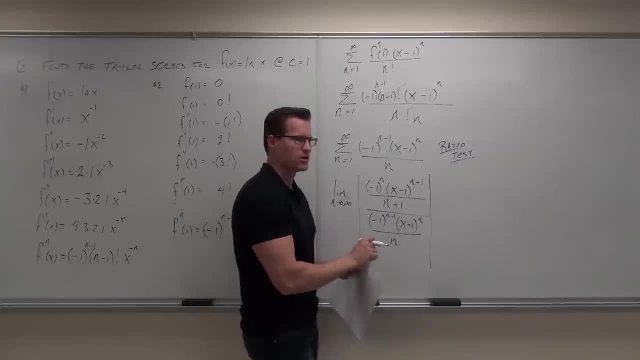 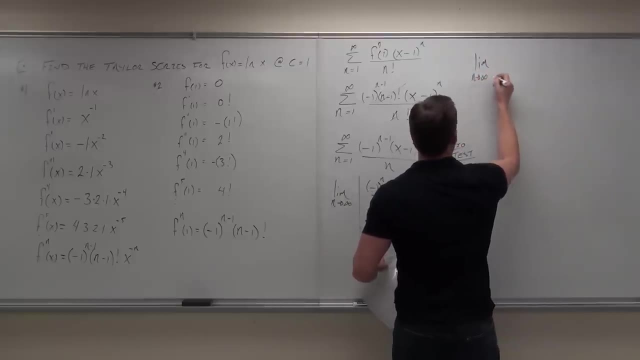 Simplify as much as you can. What's going to happen to my negative 1's They gone? So we're going to get a limit. n approaches infinity. Do we get rid of the absolute value, ladies and gentlemen? No. 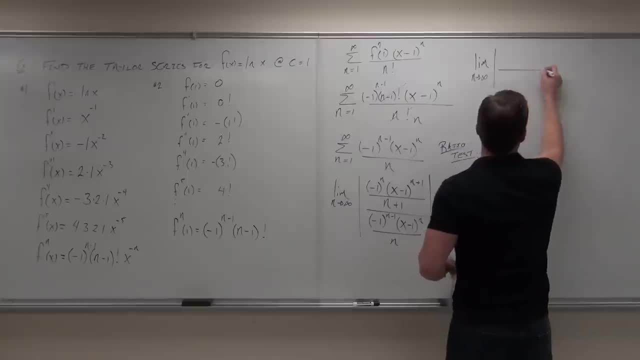 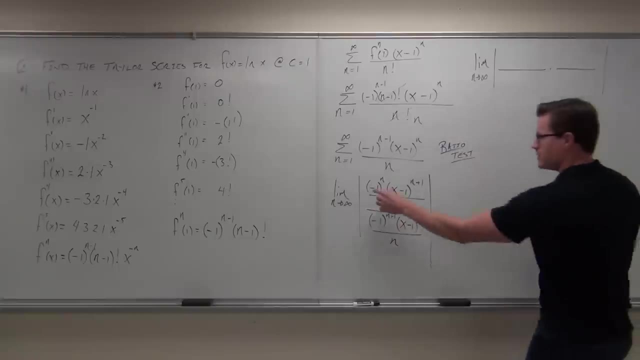 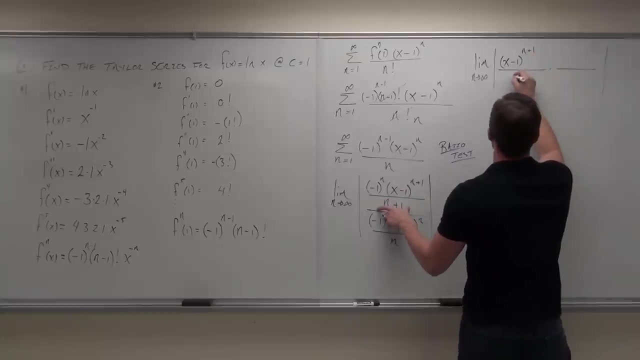 No, we really don't do that. when we have x's in here, We are going to multiply by the reciprocal of our main denominator. So here we're going to have our this piece gone, still have this piece. still have this piece. 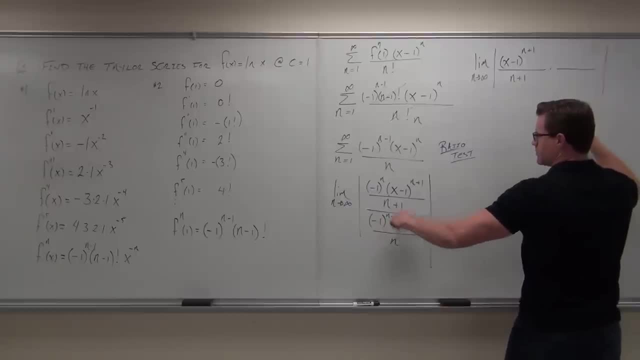 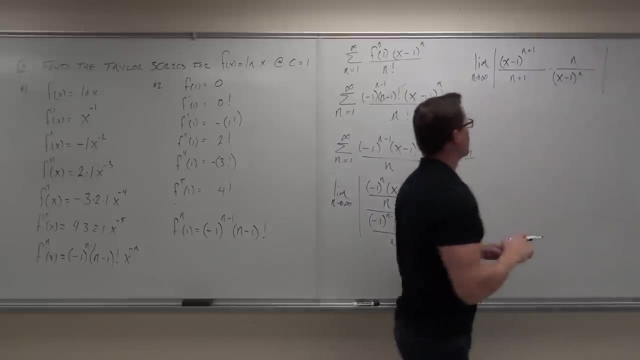 Then we're going to well, this piece is gone. Absolute value takes care of that for us. Multiply by reciprocal. we have n over x, minus 1 to the n. What's the next thing that we can do here? Can we simplify? 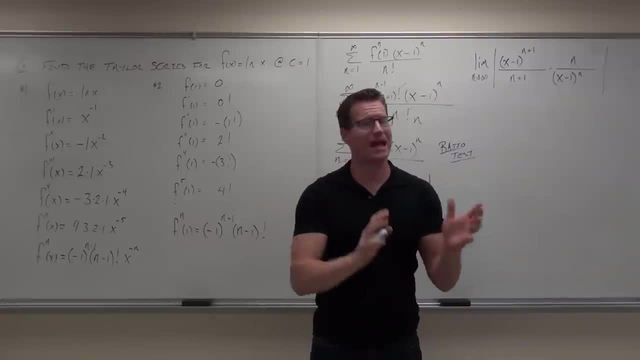 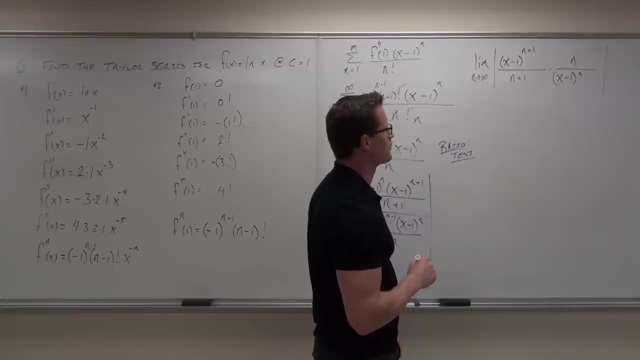 We're going to simplify it. Then we're going to collect our n terms and collect the remaining x term. Everything else is simplified here. So what do we get? You're going to get n over n times n minus 1.. OK, I'm going to get a n. 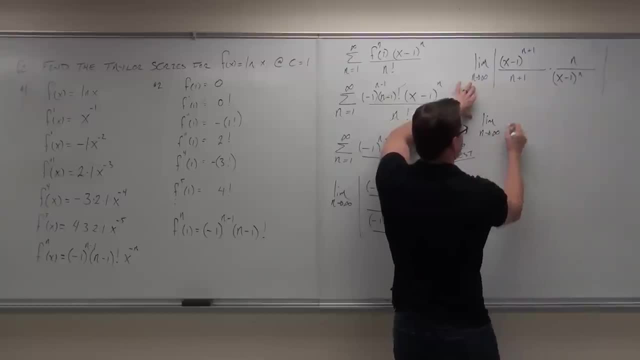 I like that. I'm going to get a limit- n approaches infinity- of n over n plus 1.. Absolute value: I'm going to get an absolute value. Very good, Why can't I pull out the n over n plus 1? 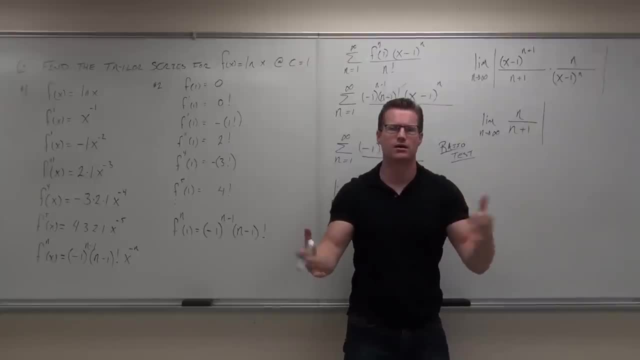 and not have an absolute value. Tell me, explain to me why I can do that. It's always positive. Very good. n over n plus 1 is always positive. I'm going to go to infinity, So this is always positive. 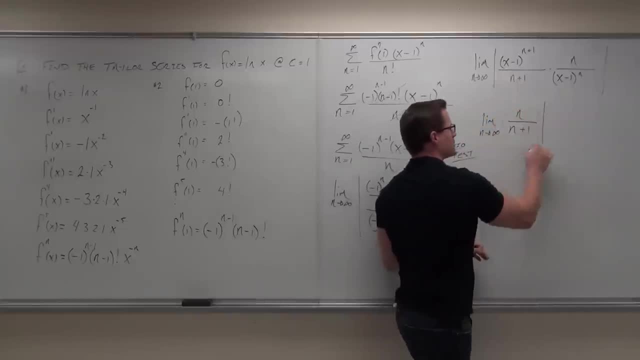 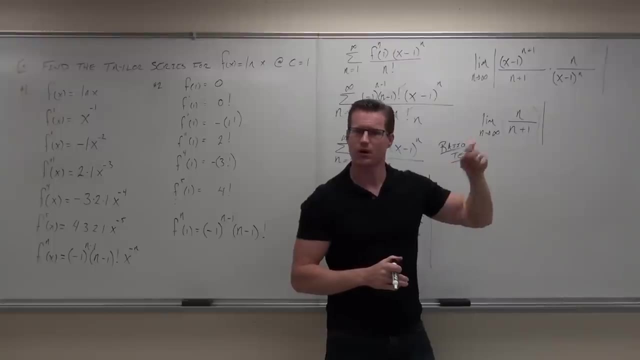 We collect our n terms. No absolute value, Maybe parentheses. if you really want to be technical about that, Put parentheses around it. What's going to be inside of our absolute value x minus 1.. Under 1 or over 1?? 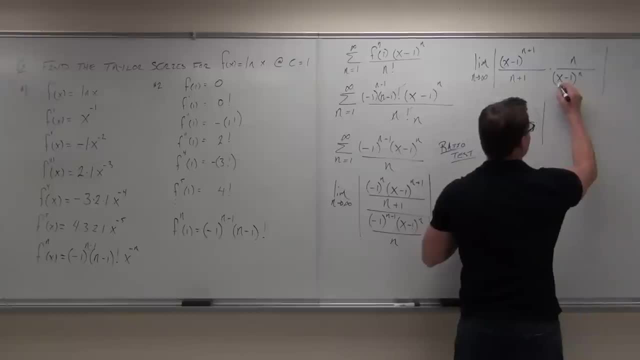 Where is the x minus 1 on the numerator? Very good, because this simplifies all of this. That little plus 1, that says that you have one power of x minus 1 more than you have here. Therefore our x minus 1.. 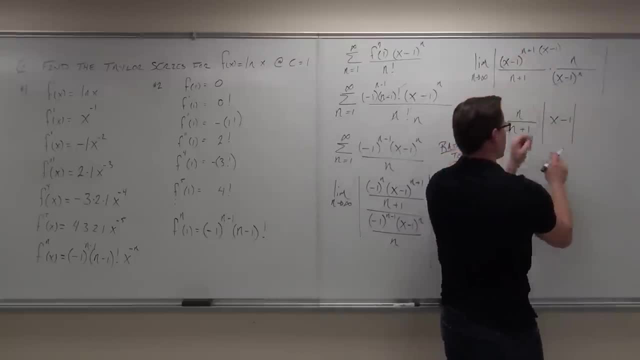 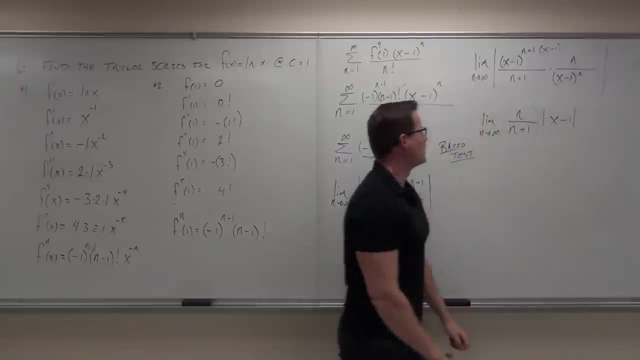 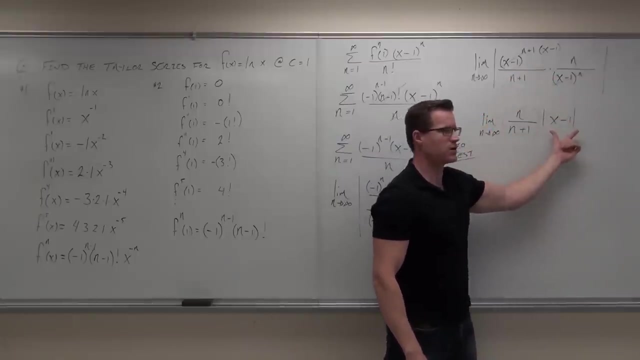 x minus 1 is still on the numerator. Absolute value is a little bit big here, So we get our n over n plus 1, no problem. Collect our n terms. We simplify, We get x minus 1.. Still an absolute value. 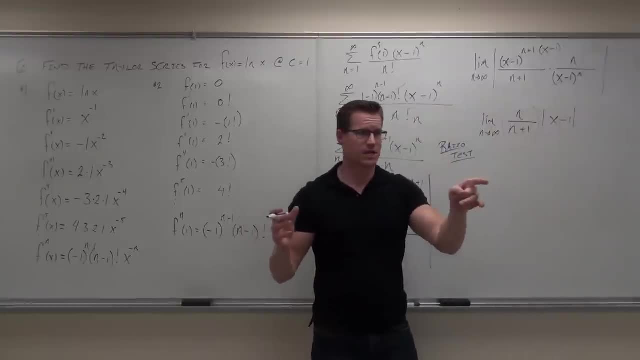 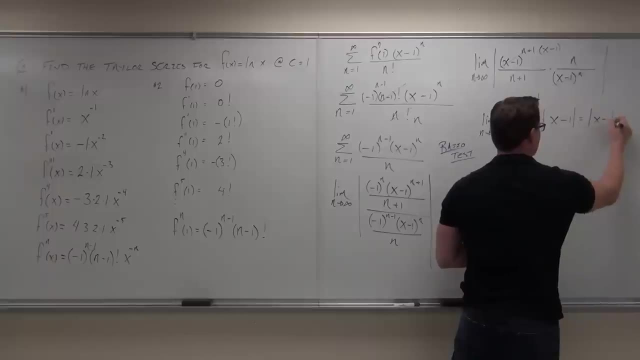 Now what do we do? Take a limit. Take a limit, Very good. What's the limit of n over n plus 1? 1. Very good, So this thing is equal to the absolute value of x minus 1.. Now tell me something about the test we used. 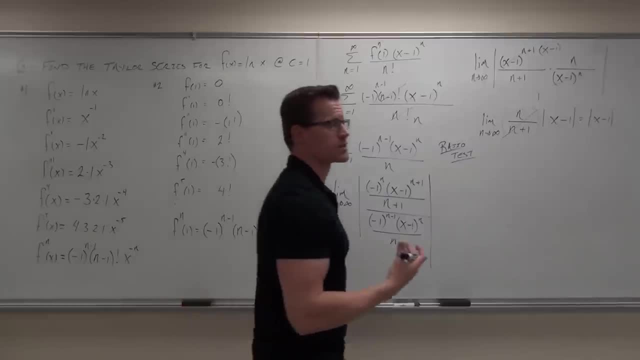 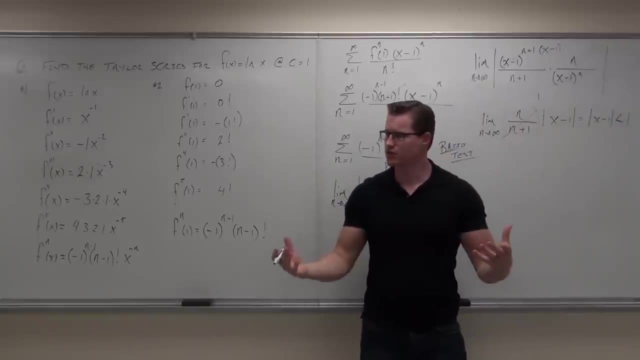 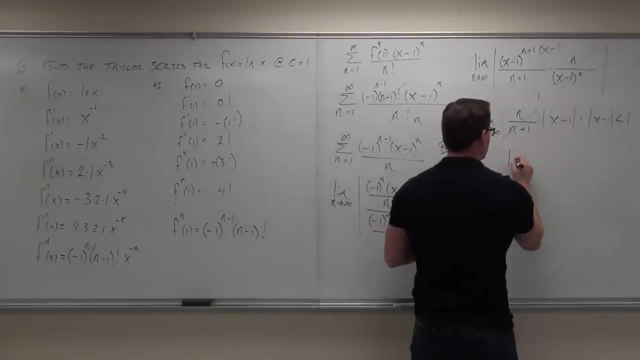 What test did we use? What's it tell us about convergence of a series. So whatever we have here must be less than 1 for convergence. Are you with me? Yes, That gives us our interval. That's great. So right now, we know that this series is going to converge when the absolute value of x 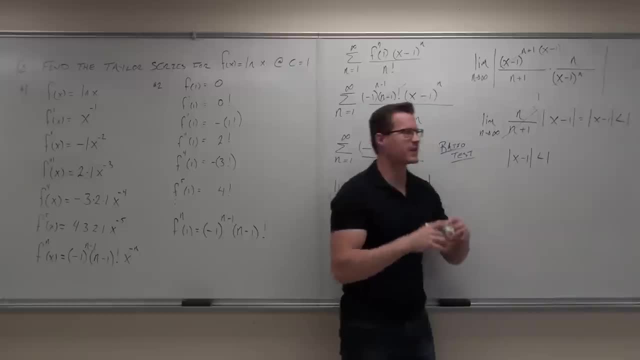 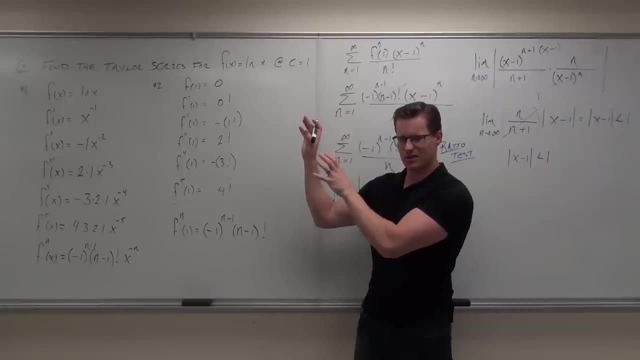 minus 1 is less than 1.. That's when we know this is going to converge. That's when we know that this Taylor series will represent our function ln of x, You with me. That's when we know, because it only works if the series is going to converge. 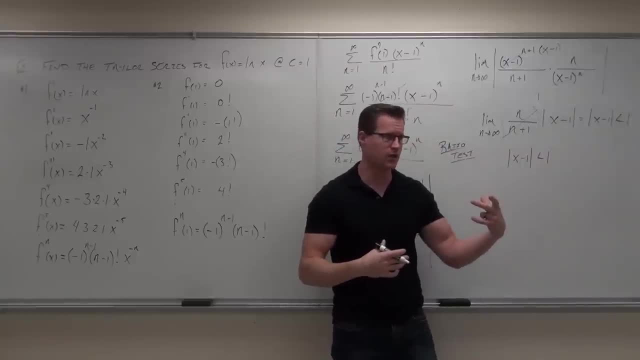 That's the only time we get an output for our function, which is the only time we can actually get a function here. Now, from here, can you tell me my radius of convergence? What is it? 1. As soon as you find whatever's being raised to the nth power right here, as soon. 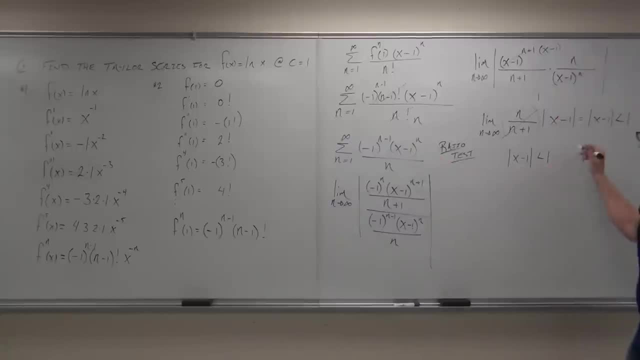 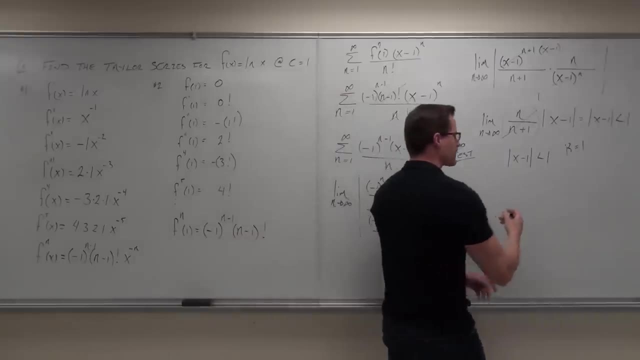 as you find that in your absolute value, that right, there is your radius of convergence. So the r is 1.. Now let's go ahead and do the interval of convergence From here. What we know by the definition of the absolute value to create a series is that it's going. 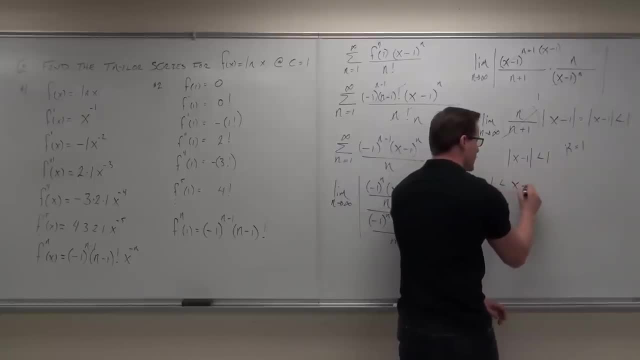 to have a negative 1 minus 1.. So what we know from this is that the absolute value of the integral is that the negative 1 must be less than x minus 1 must be less than 1.. You following me on that one. 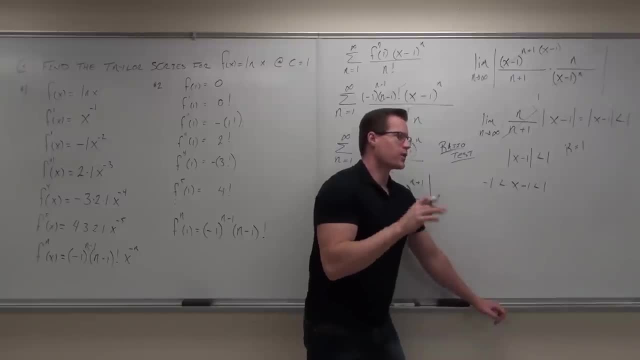 That's what the definition of the absolute value of the integral is. Now we're looking for the interval. so we don't stop here. We want to get x by itself. So when we get x by itself, we have to add 1 to all three of our zones. 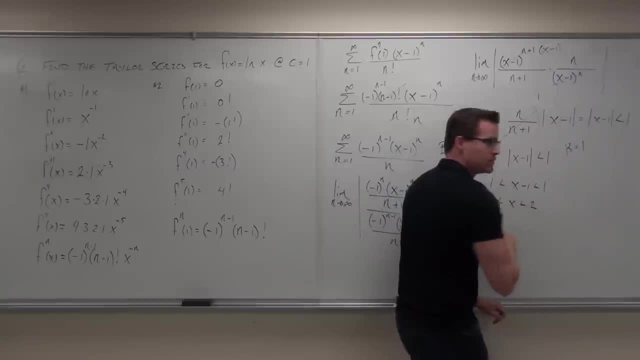 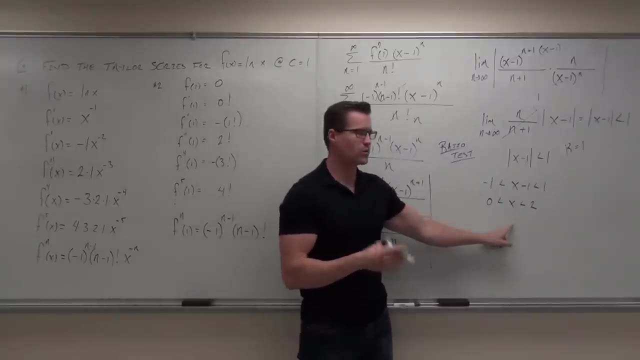 We get. 0 is less than x is less than 2.. You okay with that. So notice, it Is 1 in the center of our integral Right, in the center it's supposed to be there. Is the radius still 1?? 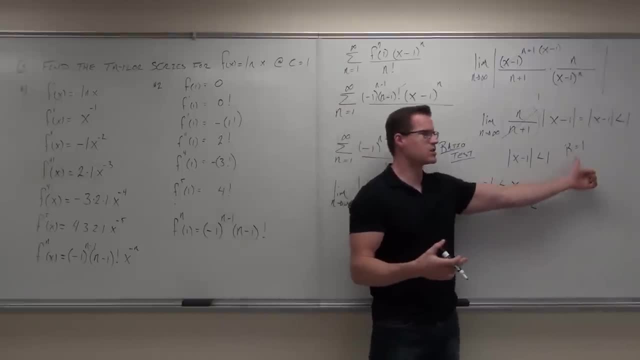 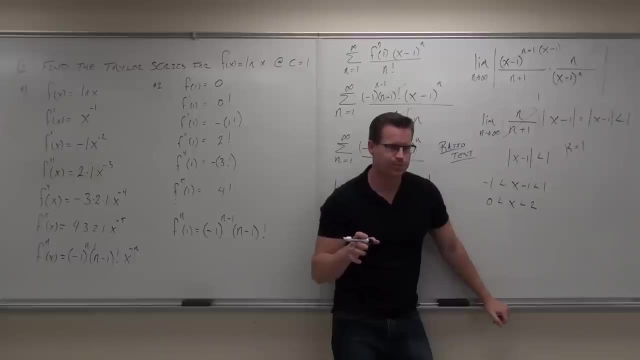 Can I add 1 and subtract 1 to get these two numbers? That's why we get our radius here first and then we get our interval. Now here's the issue: What about 0 and 2? Endpoints- We've got to check our endpoints. 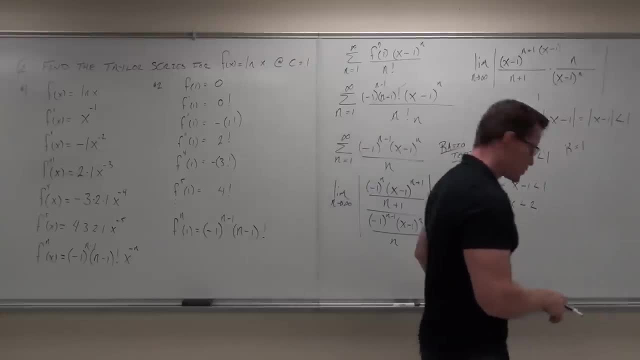 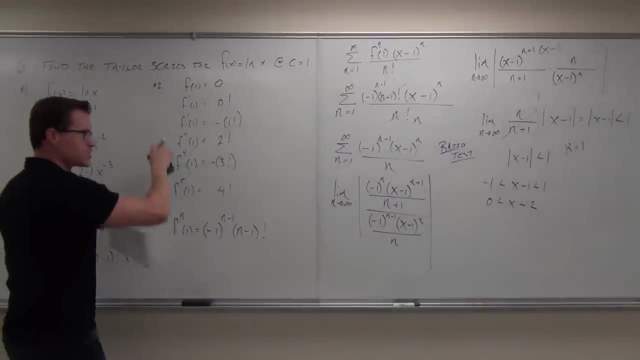 Check your endpoints. Actually, you know what. We'll do it together. I want to be a little bit quicker about this. Let's check our endpoints. Any questions on the pattern at all? Is there any? So this was just to find our pattern, just basically just to find this piece right there. 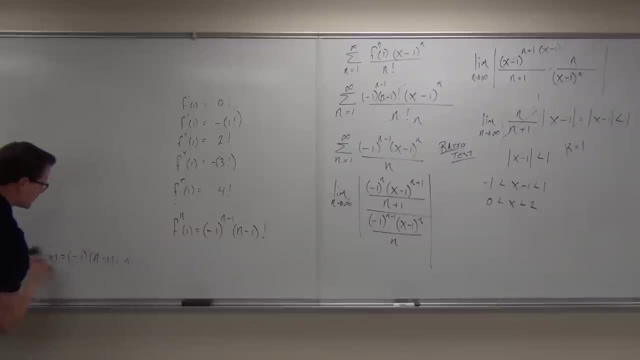 Everything else we already know. So here we go. Here's our endpoints. What are our endpoints right now? 0.. So 0.. If my original Taylor series goes from 1 to infinity of negative, 1 to the n minus 1, x, 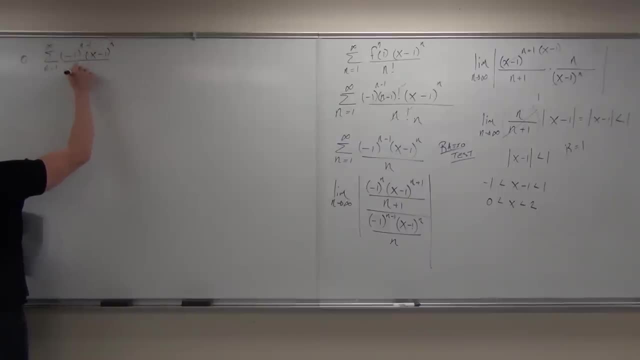 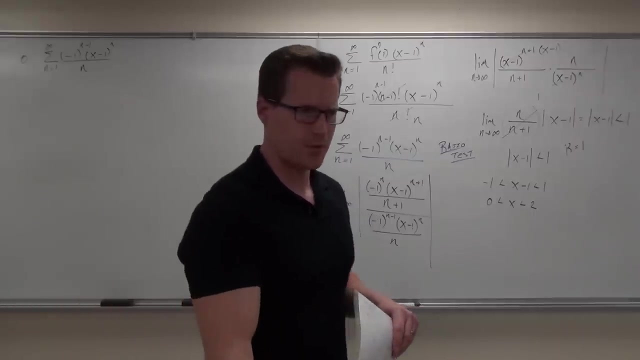 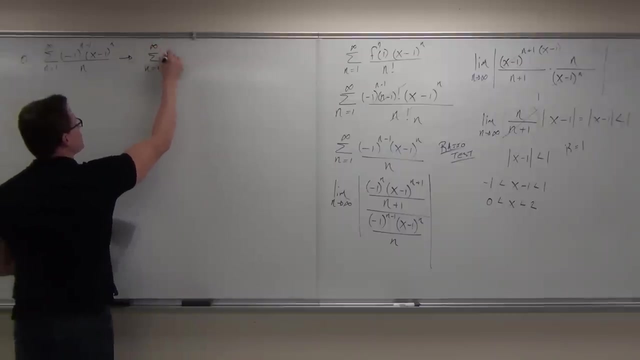 minus 1 to the n over n. Okay, And I say I want to plug what number? am I plugging in? 0. And where am I substituting that for x? So this becomes the series: n equals 1 to infinity, negative 1 to the n minus 1 times what. 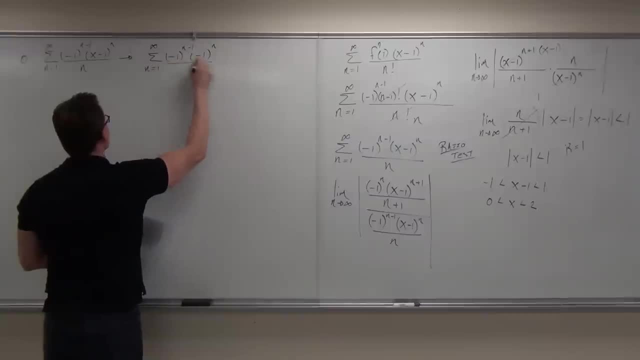 Negative 1 to the n. Oh, negative 1 to the n. That's right Over n. You all okay with where that's coming from. Mm-hmm, If you plug in 0 for x, you're going to get 0 minus. oh yeah, that's negative 1.. 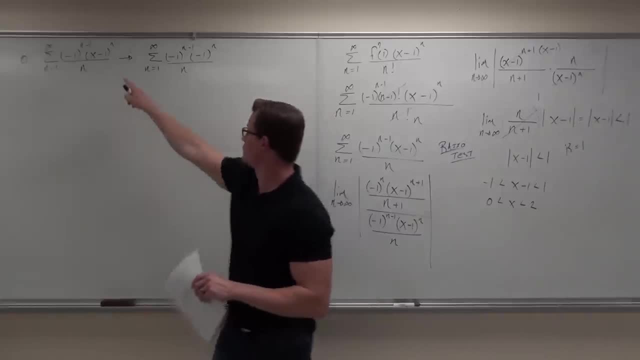 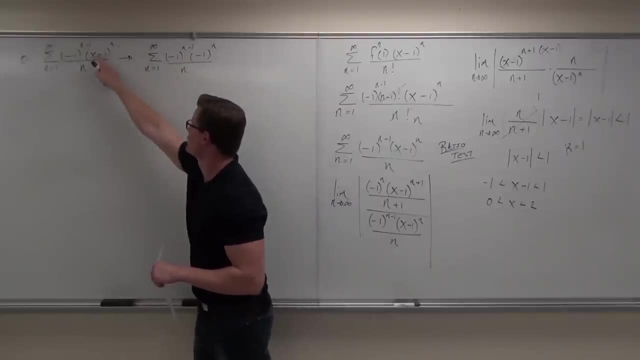 Yeah, Okay, Okay, Okay, Okay, Okay Okay. Negative 1 to the n. here We got our first little piece: negative 1 to the n minus 1.. We got the second little piece. when we plug in 0 for x, we get negative 1 to the n. 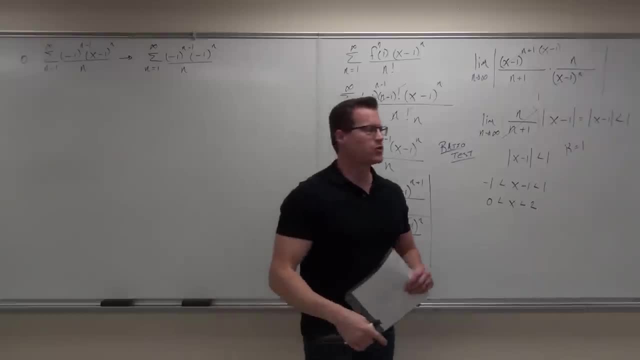 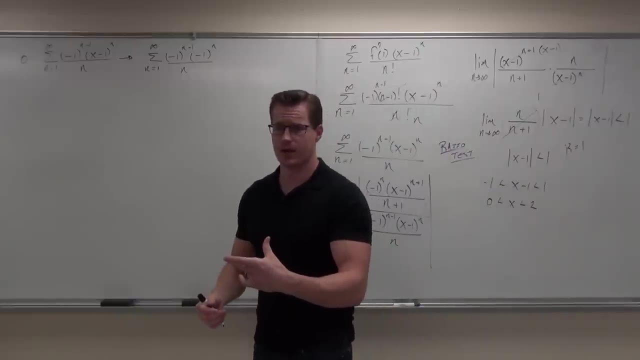 Now simplify this before you try to do any tests on it. The negative 1 to the n minus 1 times negative 1 to the n does not look very good right now. So what we're going to do is because we have these common bases being multiplied together. 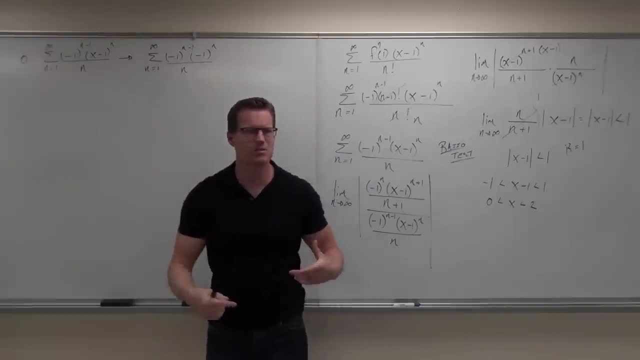 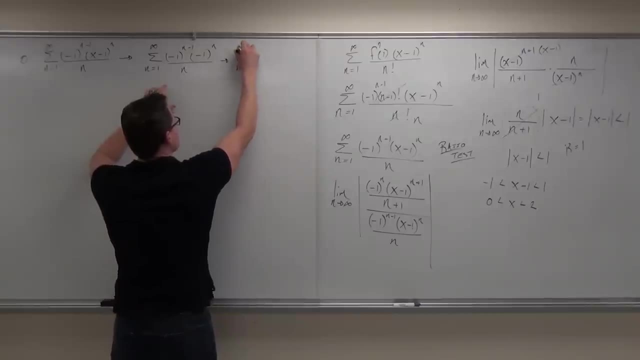 what are you supposed to do with your exponents when you have common bases being multiplied together? Add them, This comes series and equals 1 to infinity. of what over m? 1 to infinity? I'll tell you. it's going to be negative 1, negative 1 to the. 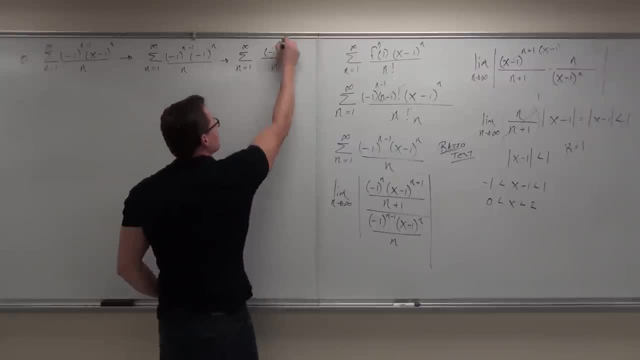 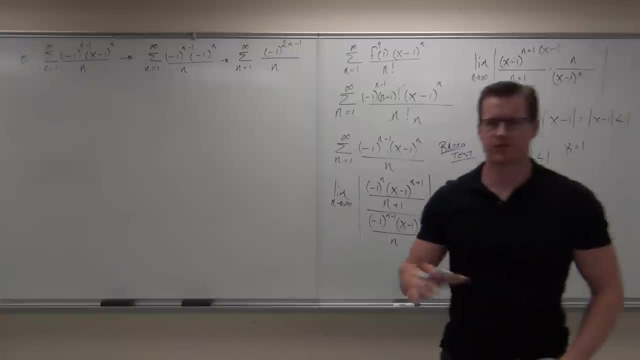 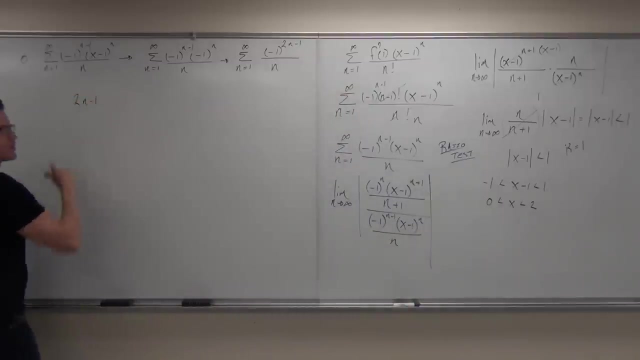 2n minus 1, 2n minus 1.. Now, where you can see this for a second, What does 2n minus 1 always give you? Plug in n's. What's it? always give you Odd number. 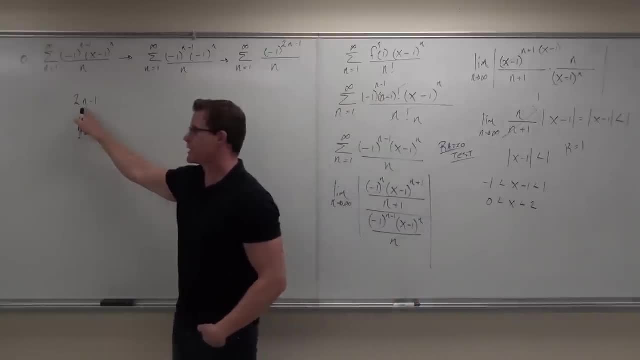 It gives you odd numbers. It's very good. So we're starting at 1, right? So you plug in 1, we get 2 minus 1, that's 1.. Then you plug in 2, we get 4 minus 1, that's 3.. 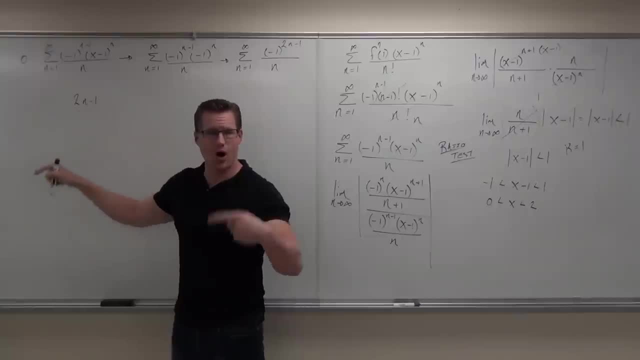 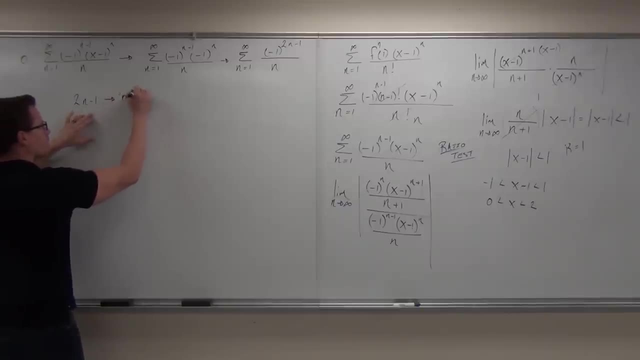 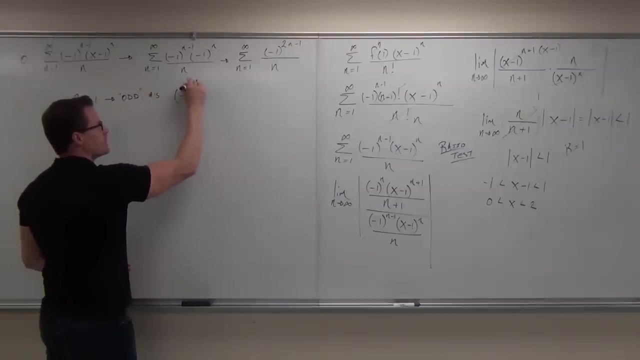 Plug in 3, we get 6 minus 1,, that's 5.. We get odd numbers, The expression 2n minus 1, this gives you odd numbers. Now how much is negative 1 to the 2n minus 1 then? 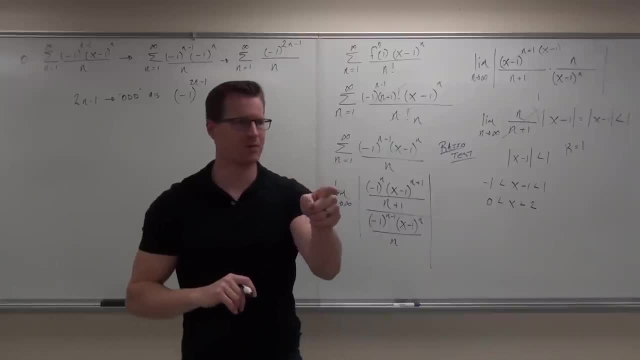 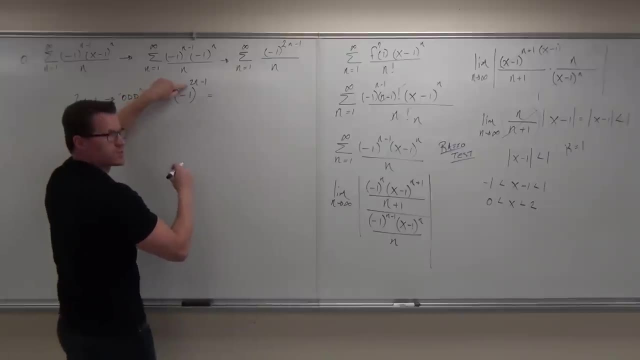 What is it? Always negative? It's always negative. Very good, Because it's always going to be to the 1st, 3rd, 5th, 7th, 9th, whatever, always odd. Then negative 1 to the 2n minus 1, you know what, guys. 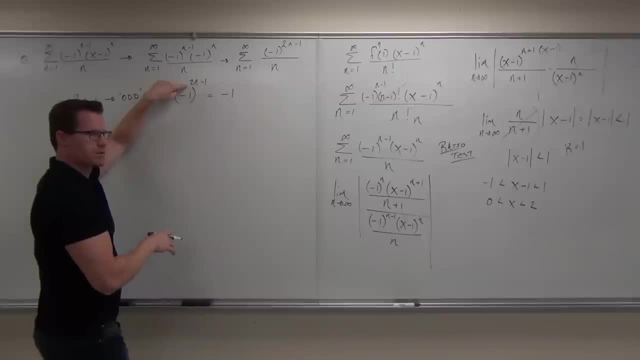 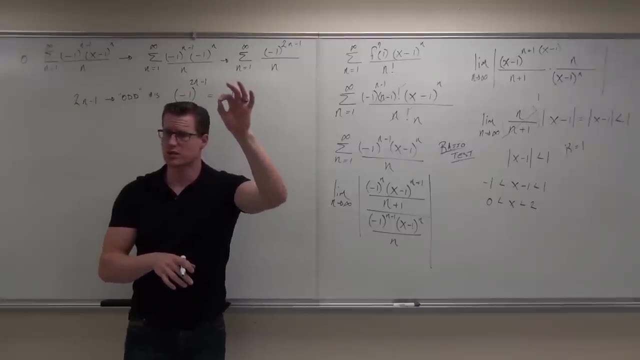 This is just equal to negative 1.. That's all it is. Does that make sense to you? Because it's always going to be negative 1 to an odd number. Negative 1 to an odd number is always going to give you negative 1.. 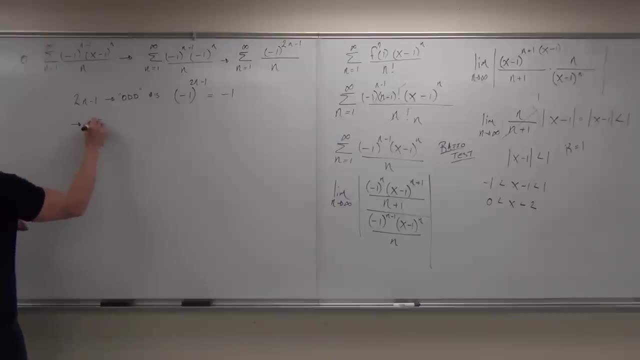 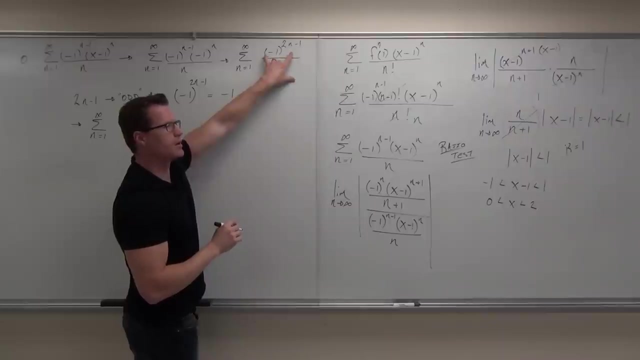 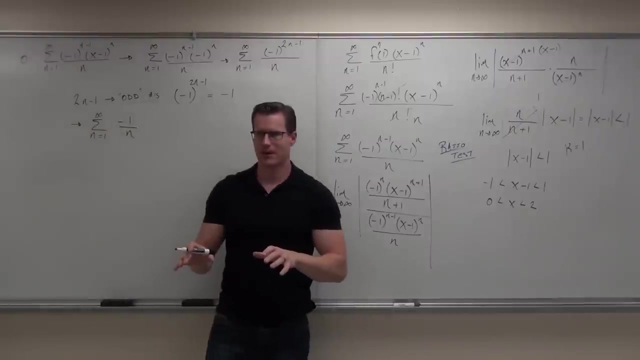 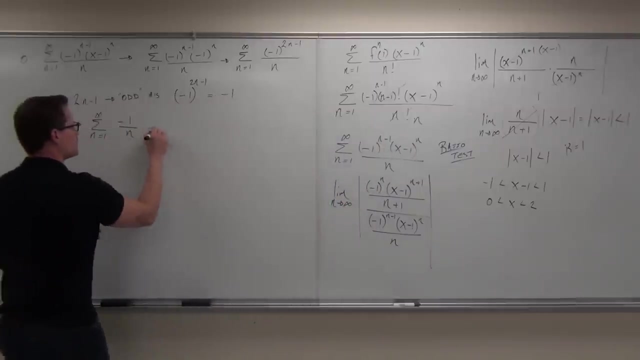 Therefore, this series becomes: how much is this whole piece? Do you understand why? Yes, If this is always odds, this whole piece becomes negative. 1 over n. You sure you're okay with it? Now, do you remember that we can pull constants out of our series? 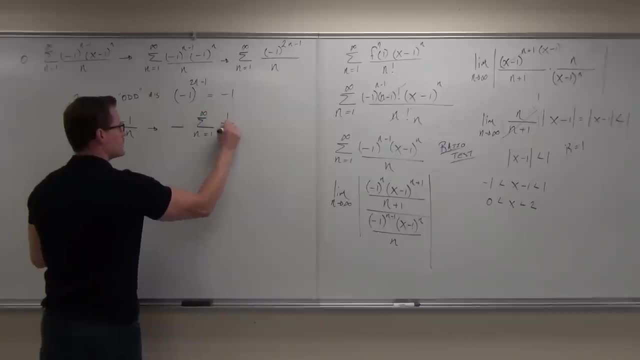 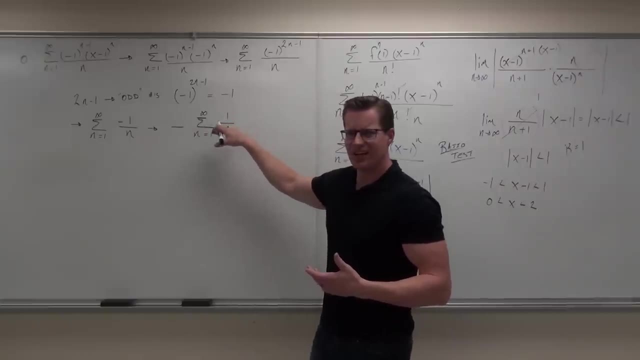 Negative sum from 1 to infinity of 1 over n. Oh my gosh, We finally have it. Tell me something about the sum from 1 to infinity of 1 over n. What is that Harmonic? That's harmonic. 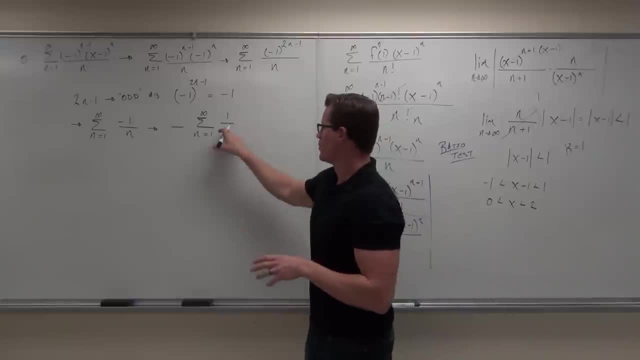 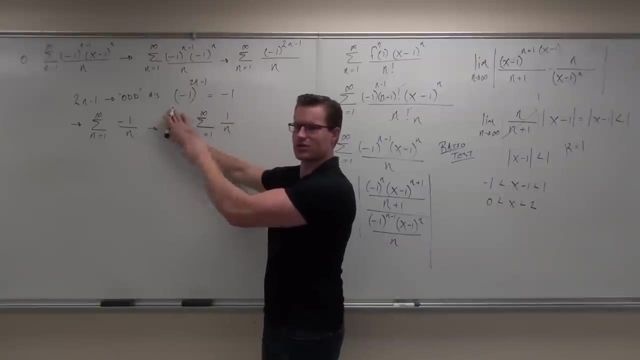 Or it's a p-series with p equals 1. Either way you say this: what happens in this series? Divergence. I don't care about the negative. What happens in this series? Divergence. Negative divergence is still divergence. 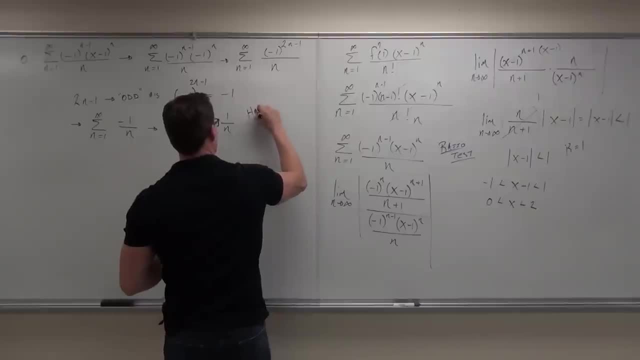 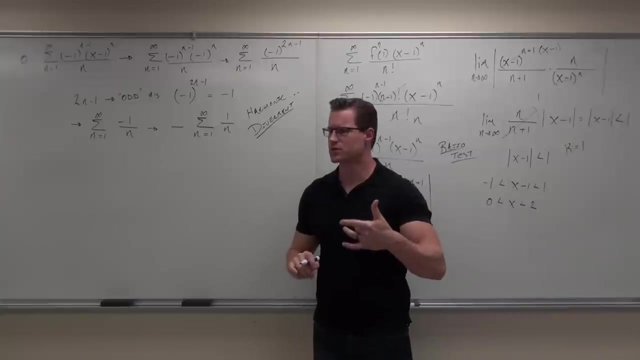 So this thing diverges. So harmonic, therefore divergent. That's it, Thank you. Tell me something about the endpoint of 0.. Is that going to be included in my interval of convergence? No, Therefore, is that going to be in the domain of my function as represented by my Taylor? 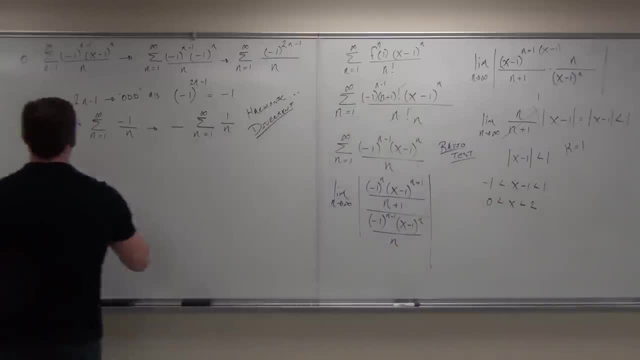 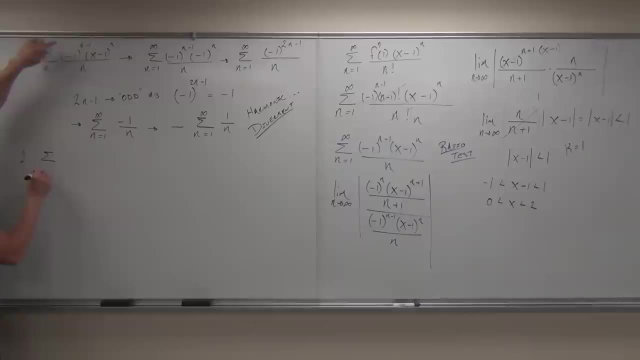 series. No, It's not going to be in my domain. Okay, The next endpoint we've got to check is the 2.. So let's plug in the 2.. If we plug in 2, this series goes from 1 to infinity of negative, 1 to the n minus 1.. 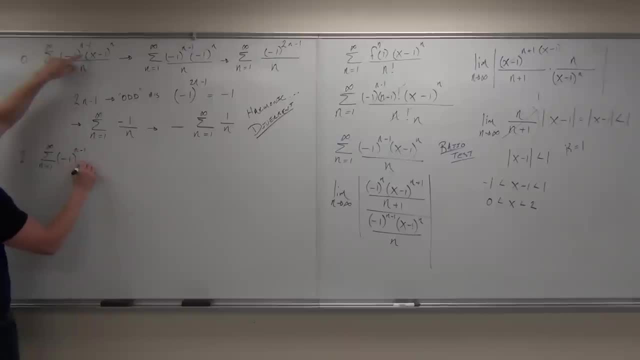 If I plug in 2, how much do I get? 1.. Yeah, 2 minus 1 gives you 1 to the n all over n. Now this one's going to be much more straightforward. We're not going to have any fancy pants math to do up here, okay. 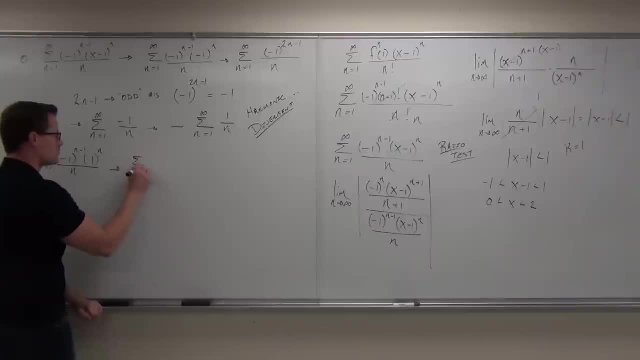 How much is 1 to the n? 1.. That's easier. I guess this wasn't too hard. anyway, You just got another 2a minus 1 as odd numbers, So this becomes negative: 1 to the n minus 1 all over n. 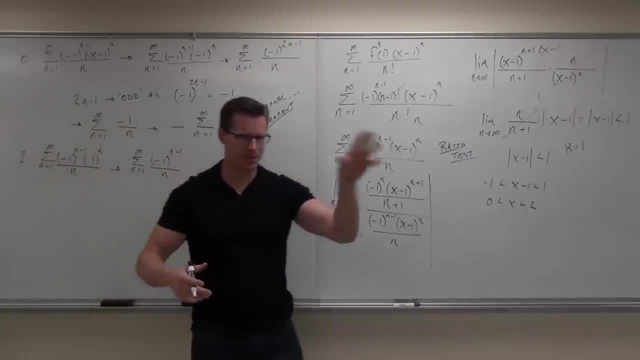 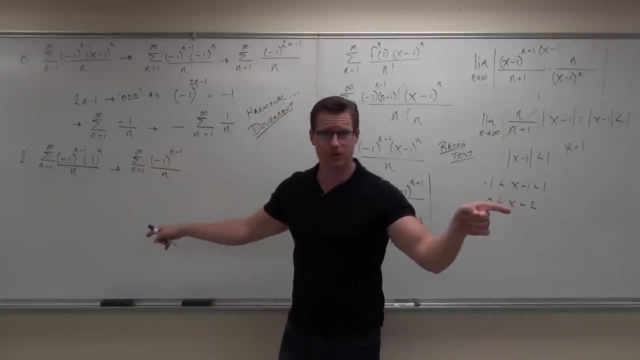 This whole thing is 1.. 1 to the n is always just 1.. 1 times anything. 1 times anything gives you the anything. Hey, tell me about this series. What do you know about it? Alternating, It's alternating. 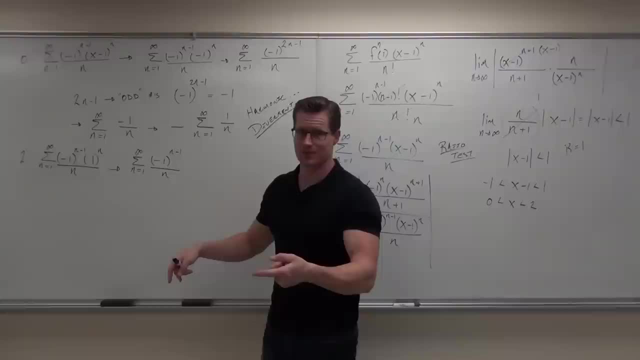 It's alternating Harmonic Harmonic. What do you know about the alternating harmonic series? Could you do a different test to show that you forgot it? Alternating Alternating series: test You got it. Don't do absolute convergence, because this does not converge absolutely. 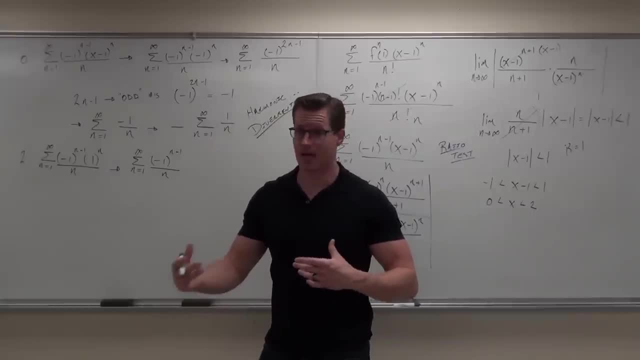 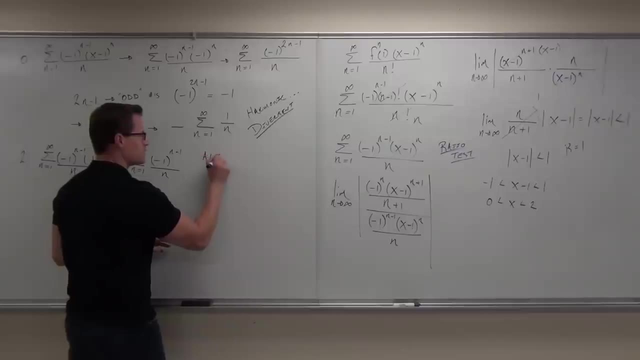 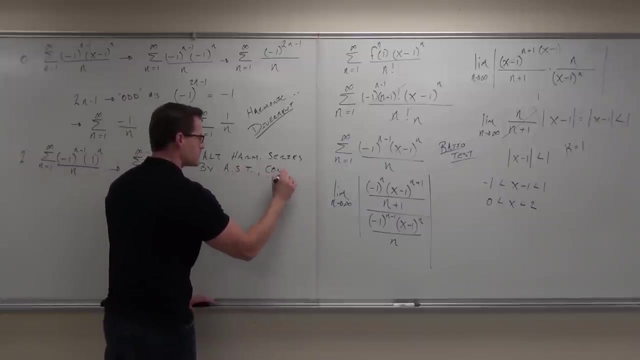 If you do absolute convergence, you get harmonic, And that says divergent. It says not absolutely convergent, It's conditionally convergent by the alternating series. So this is the alternating harmonic series. By the alternating series test, this thing converges. 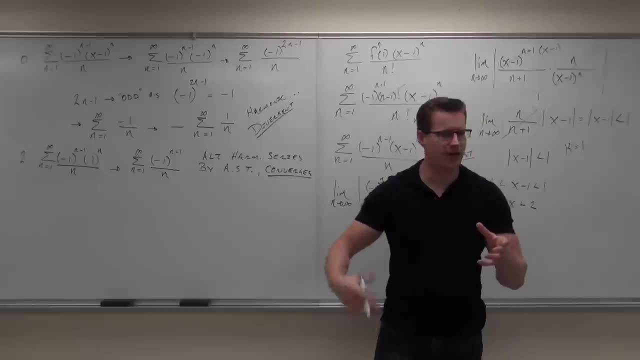 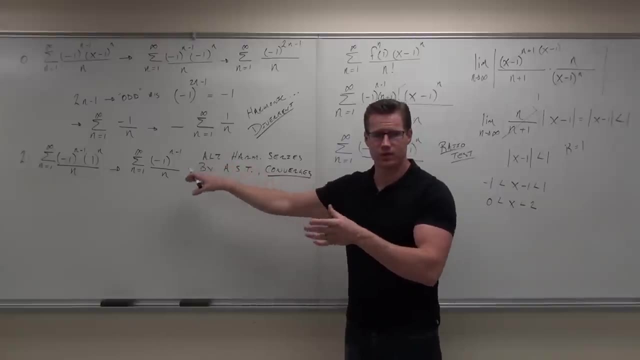 You state all these things, You tell me what it is. You tell me what you're using to find out: convergence or divergence. Is it harmonic? Hey, divergent, No problem. Alternating harmonic series- I know this conversion already- Or by alternating series test. 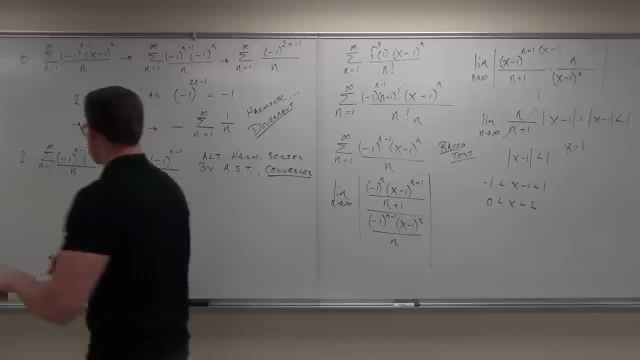 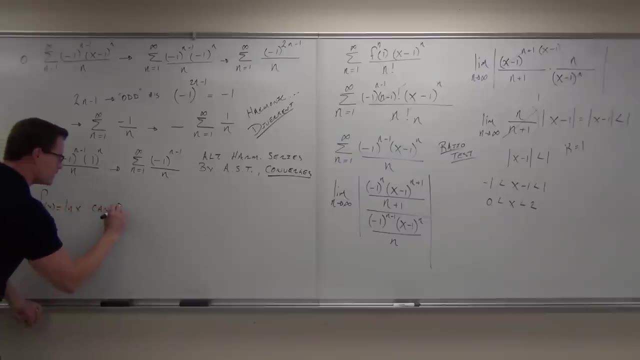 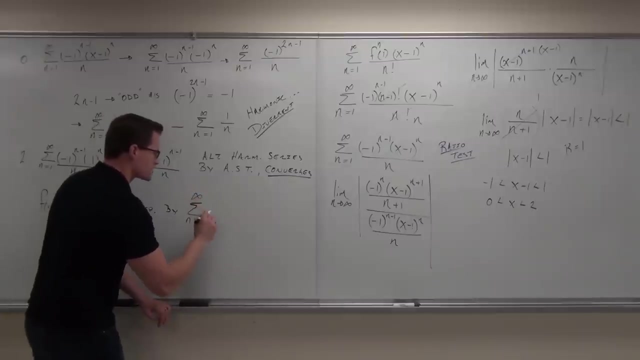 Alternating series test, It converges. So here's what we know. We know that the function f of x equals ln. x can be represented by the Taylor series. And then you show the Taylor series. You say it's negative: 1 to the n minus 1, x minus 1 to the n, all over n factorial. 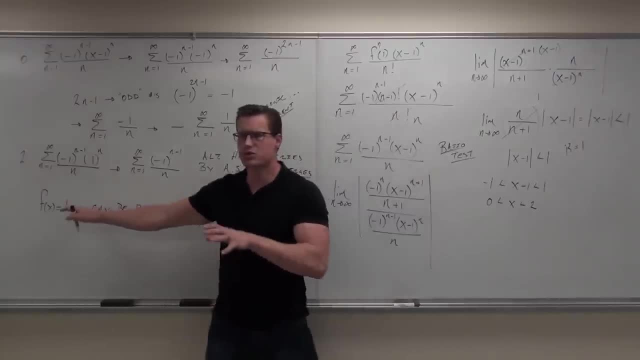 You show me what the Taylor series is, You say, hey, look at this, This is what we're doing here. folks, Don't lose track of what we're doing. Don't just miss the forest for the trees and go through this process and don't understand. 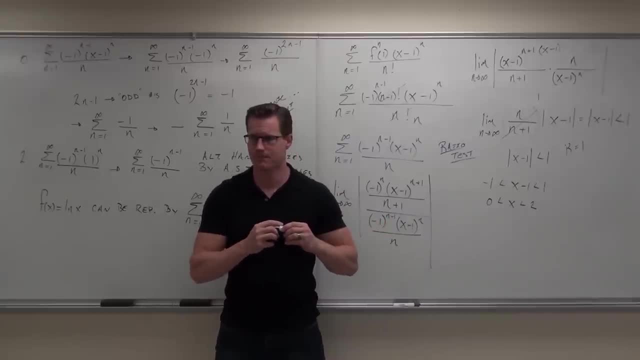 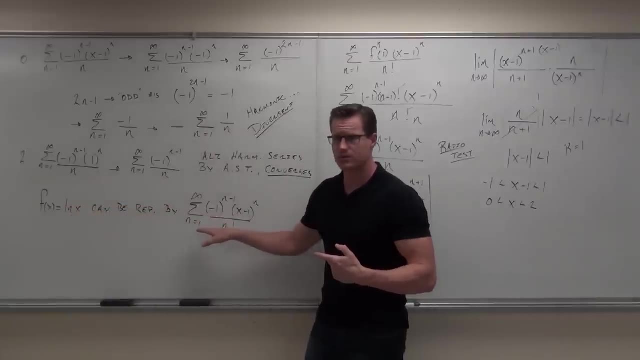 what we're doing, What we're saying is this: You ready, This function is represented by the Taylor series right here, centered around 1, on the interval, And then you tell me what the domain of this function is. Question No. 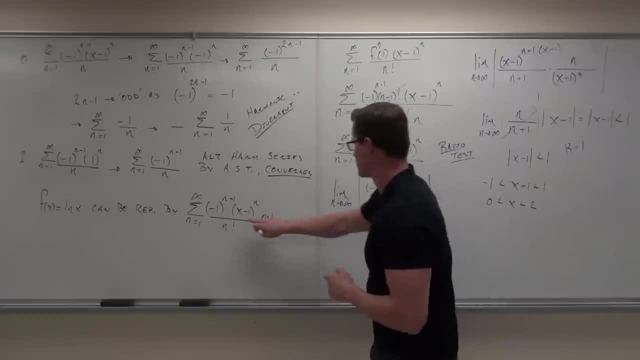 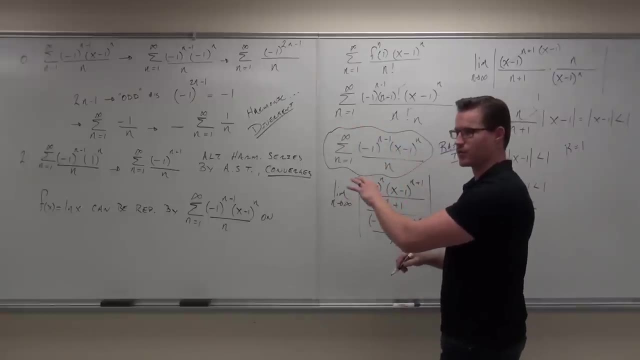 Do we need the n minus 1 factorial in there? Sorry, It should be n, Just n. It's this. Do you want to simplify it, This simplified form? So let me make sure I got it right. We got negative 1 to the n minus 1, x minus 1 to the n, all over n. 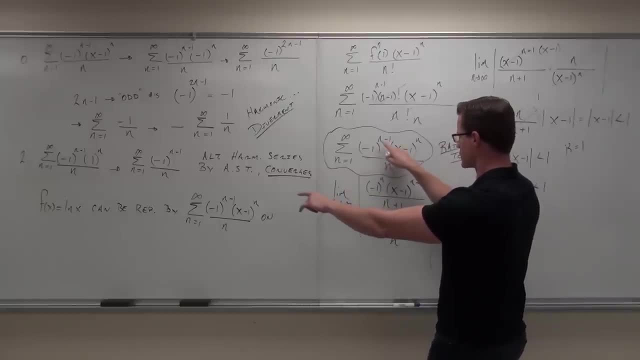 Yeah, give me this, Give me the simplified form. This is the easiest one. OK, You don't want to do this. if you can do this and get the same numbers, So do this. So our function can be represented by our Taylor series. 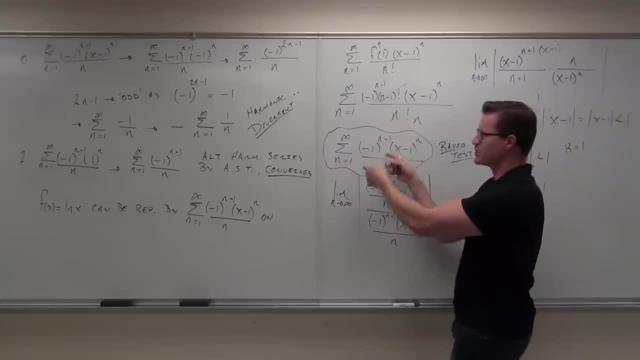 We've got it right here, But only on the given interval that you've just found. This is the only time that this series will converge. Therefore, it's the only time that this series will represent this function. It's on what interval. 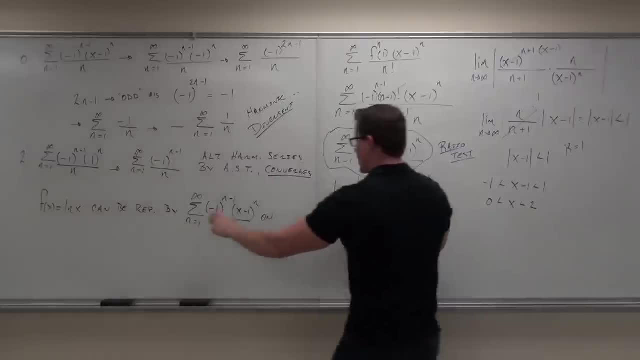 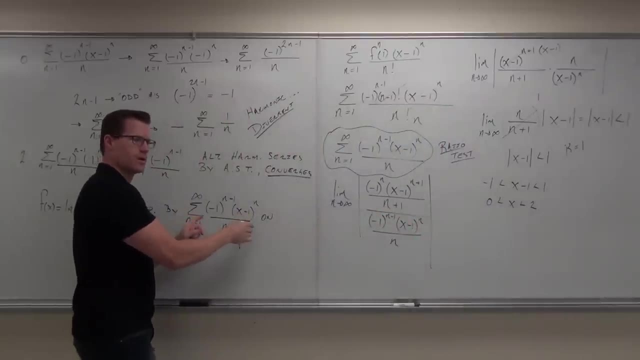 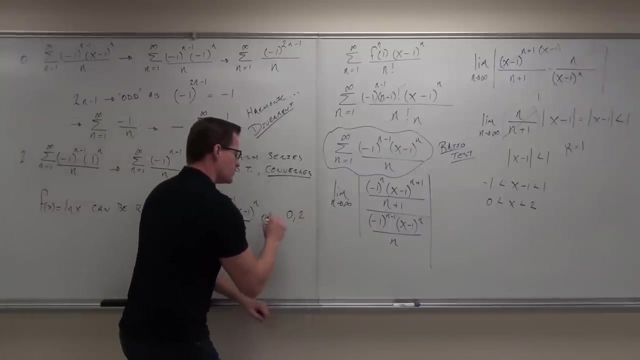 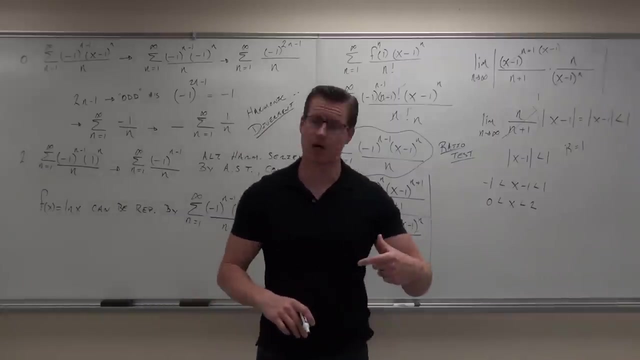 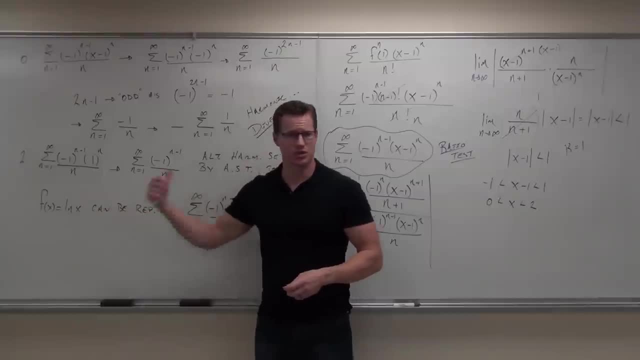 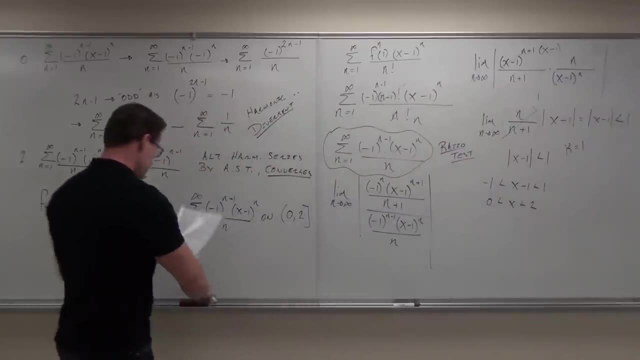 And what you plug in is going to represent that function. if you do this series to infinity, Show your hands. if you understand that one, OK, Cool, Tell you what I'm going to show you a couple other problems to do to get you really good at this. 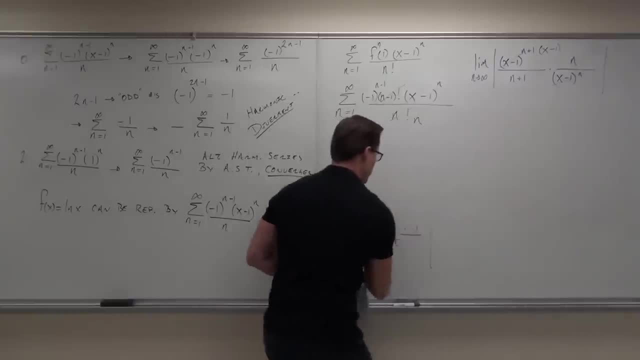 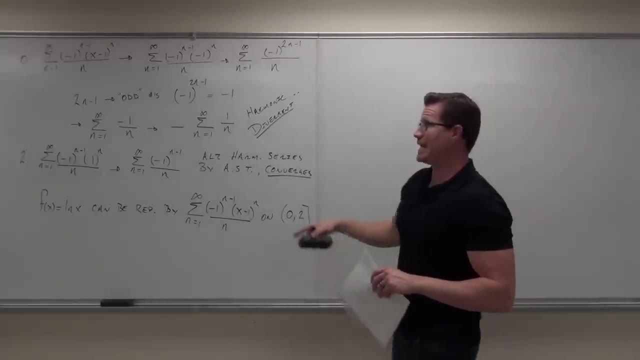 Because there's some other techniques that you're gonna have to learn here in order to be successful at doing your Taylor series and the Thorne series. Okay, last chance for any questions. I want to start fresh. Do you have any questions on this one? 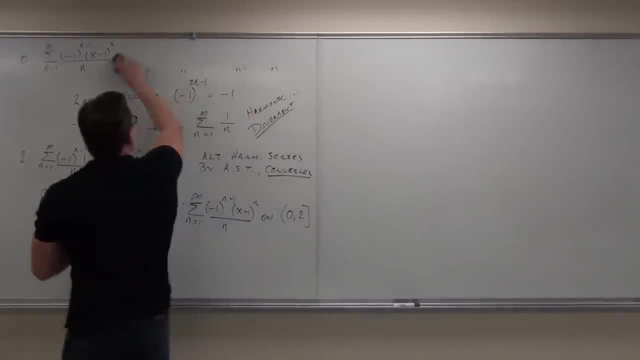 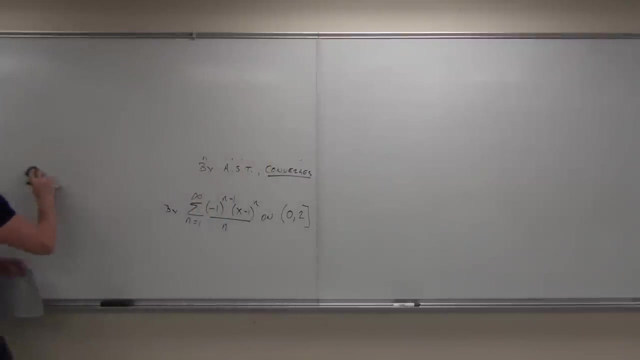 Have I explained it well enough for y'all to understand it? Cool. So our next example: write down: f of x equals sine, x equals zero. Yes, we're gonna do trigonometric Taylor series. Don't pee your pants, it's fine. 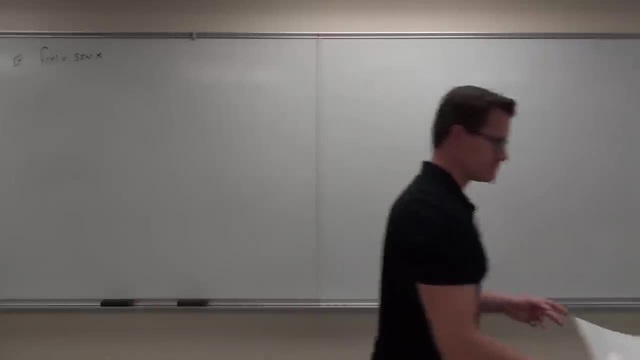 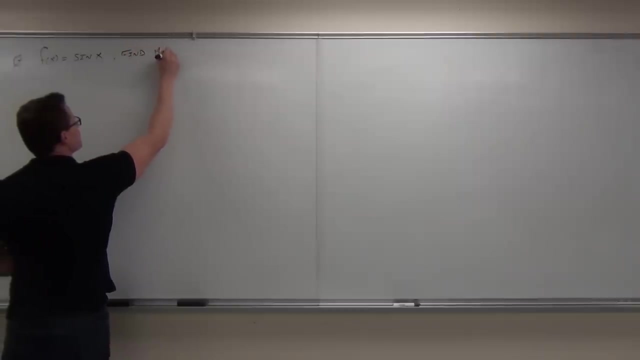 And what I want to do right now. I want to find the Maclaurin series. What's that mean? Take the d and x zero. find the Taylor series. That's right, Maclaurin series is a Taylor series. 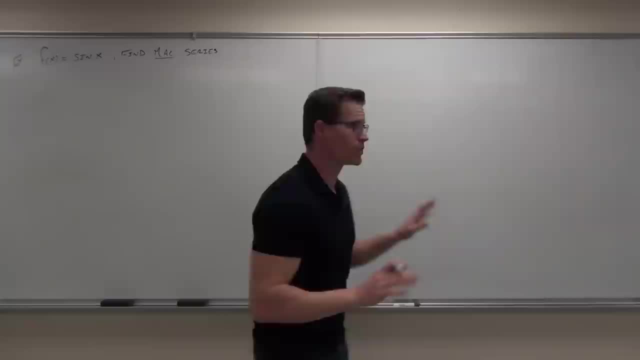 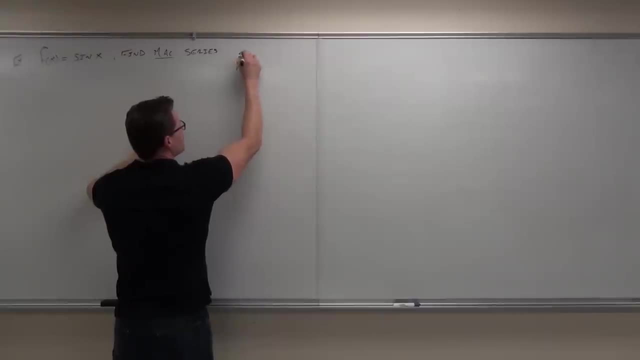 with c equals to zero, Not a problem. So what we're looking for ultimately is this. Excuse me, what we know is we want a series that has the nth derivative at zero, x to the n over n factorial. Does that make sense to you? 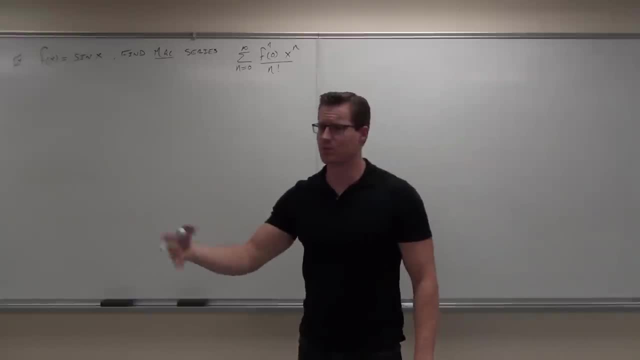 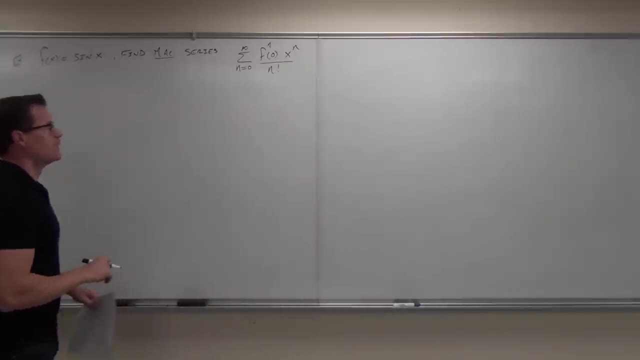 Hello, yes, no, yeah, That's a Taylor series, right. It just so happens that c would be zero, making it a a Maclaurin series. That's what our goal is is to find that thing. Now, where do we start? 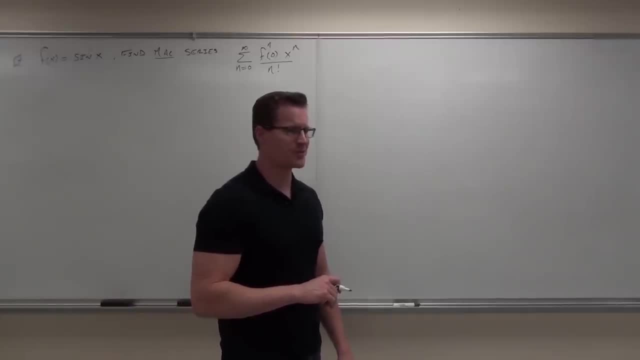 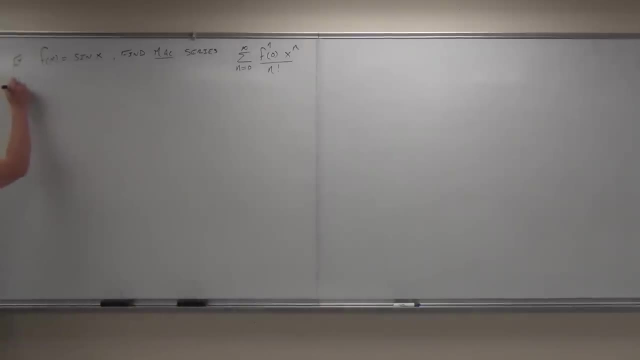 See what? now? The nth derivative of f. that's hard to say. The nth derivative of f, that's what we want. So we start doing derivatives. that's step number one. So okay, we'll start with our function. 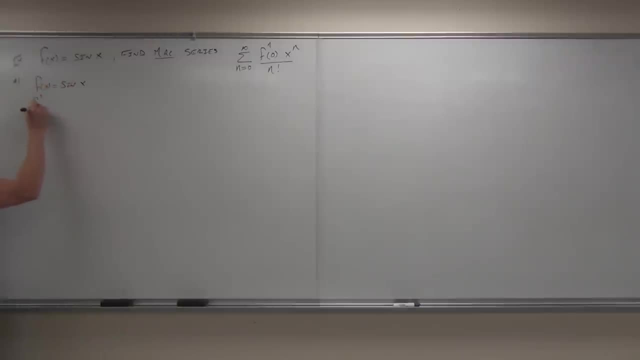 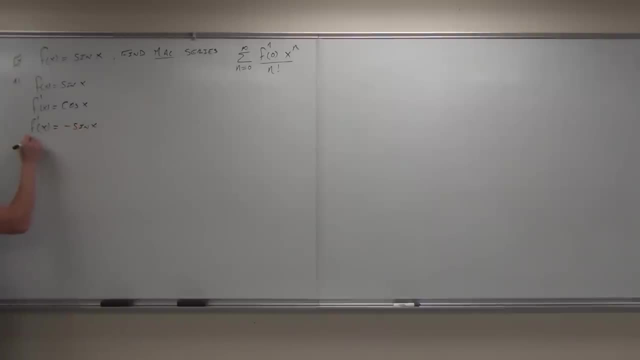 Sine x, Sine x. What's our third derivative? Negative cosine, cosine x. What's our fourth derivative? Sine x, Sine x. Is there a need to go any further? No, Okay, I hope not. Sine cosine negative, sine negative, cosine sine. 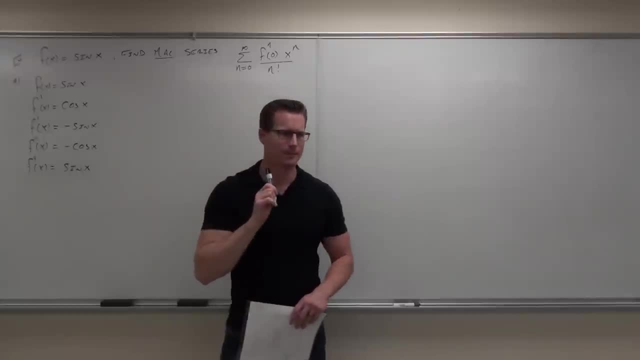 cosine negative sine negative, cosine sine cosine. Here's the problem. Here's the problem. Oops, What's this? What is that? Because I don't know. Because it depends on where you stop, doesn't it? It depends on whether you stop on a remainder. 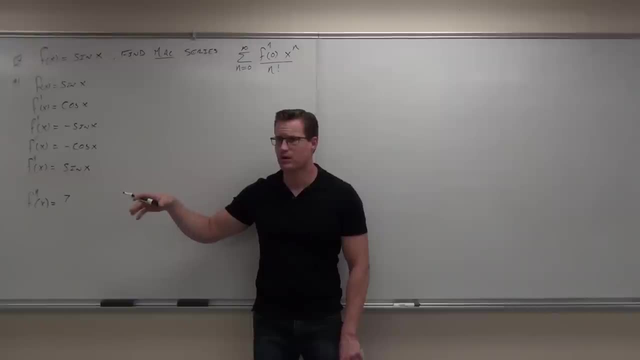 of when you divide your derivative by four. If you divide it by four and it's zero, cool, One two, Three, Zero. One, two, Three, Zero. It's gonna be a cyclical pattern. It's like number theory, okay. 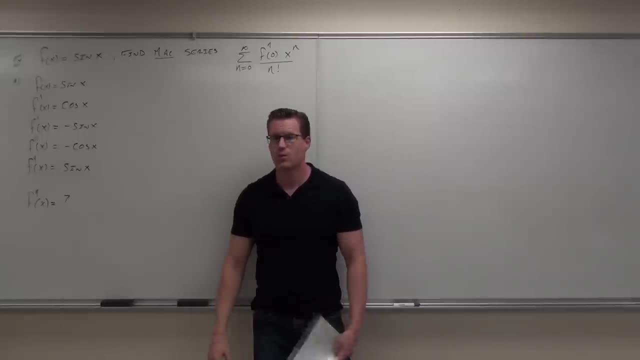 So, yeah, you don't know what that's gonna be. So this one, we can't do it this way. Sometimes we can't find an nth derivative of f explicitly, because it's gonna depend on what remainder of four that we're in on our cycle. 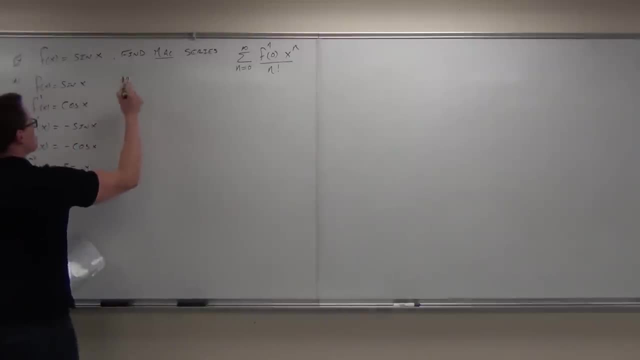 Well, you can even see it clear here. number two, Step number two says: okay, start plugging in. Oh, I'm sorry, what number is just a plug in here? Zero, Very good, Our c is zero And the first derivative at zero and the second derivative. 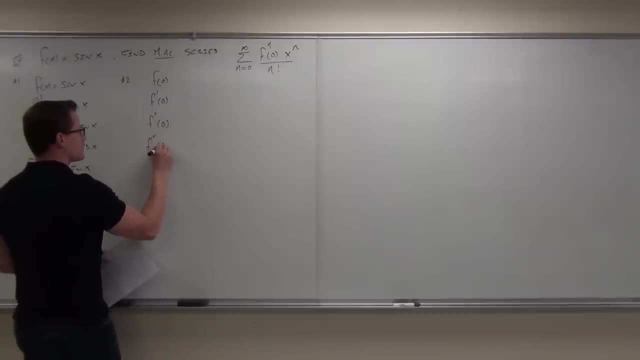 at zero, and so forth and so on. Let's see if you can give this a try. What's the function itself? at zero? Yep, What's the first derivative? at zero, One, And then One, Two, Zero. 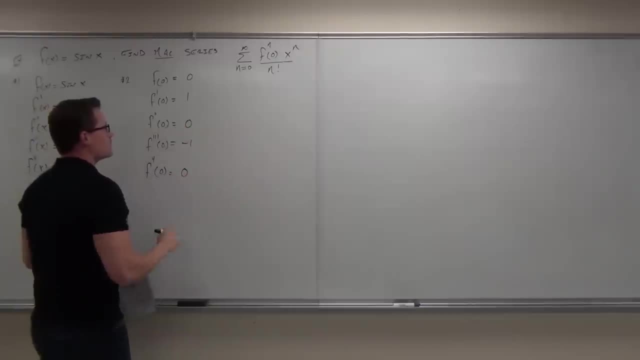 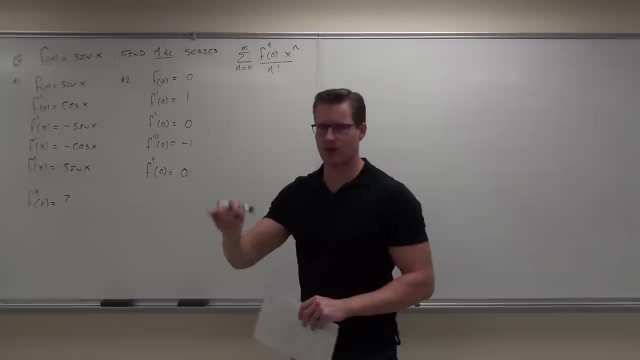 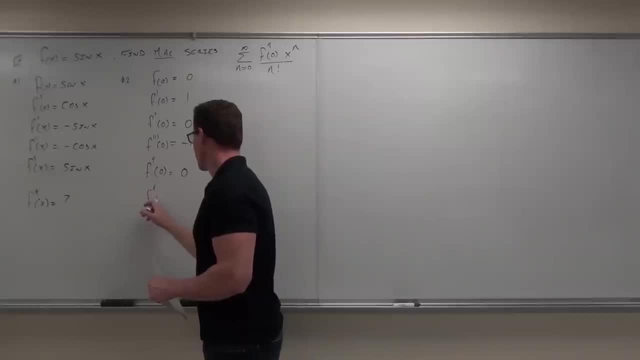 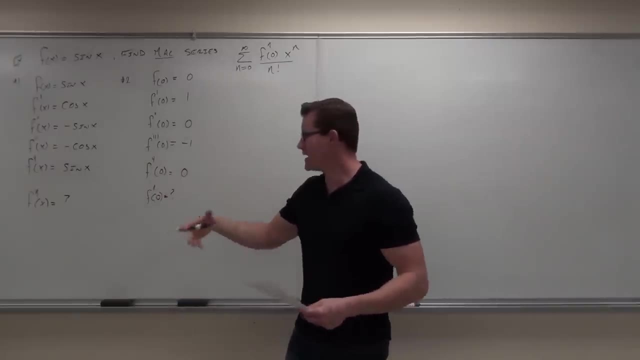 What is the nth derivative at zero? Again, I don't know. It's one of these three choices. It's either zero one or negative one, but I don't know what it is. We're gonna have to go a different way around this. 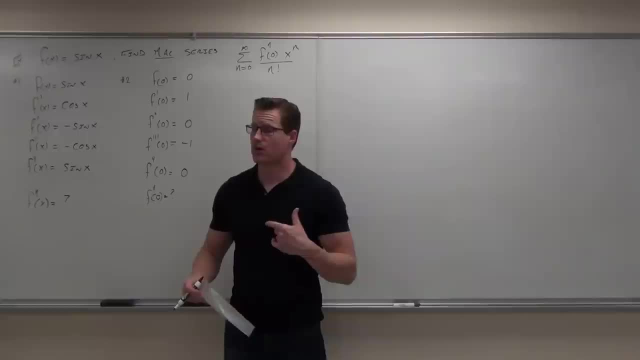 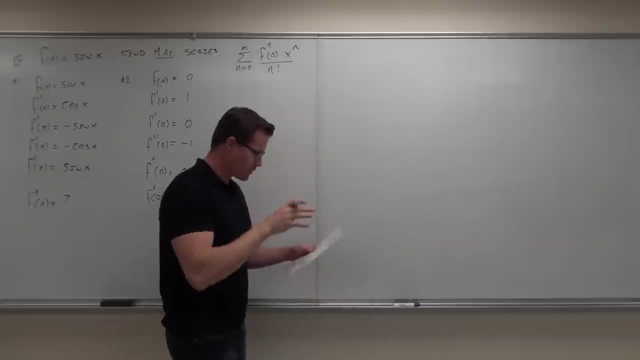 all right. So when you come up with this and you can't find a pattern, start listing out the terms of your Maclaurin series or your Taylor series. Start listing them out. So we're gonna start there. So if we really list this out, our Maclaurin series from 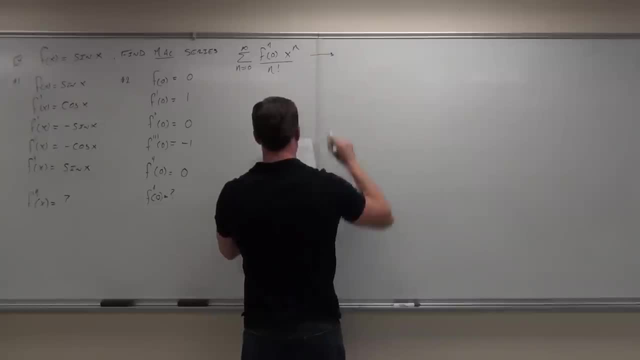 yeah, we'll do it over here, our Maclaurin series. what's our very first term? Well, this would say that you start at zero, right, You have x to the zero, that's one over zero factorial. 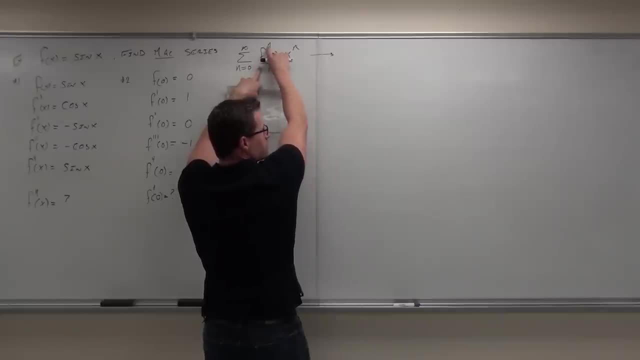 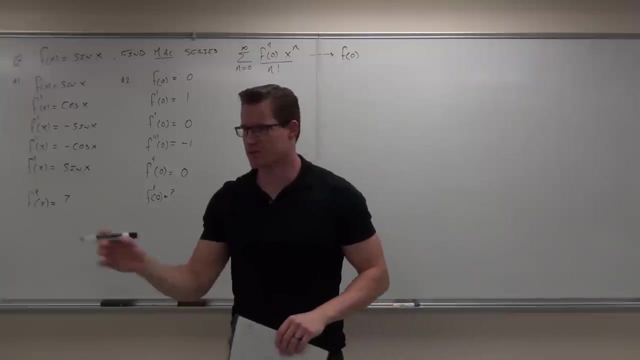 that's one. You take zero, Zero derivatives. that's basically just f of zero. Remember doing this. like the first day we did our Maclaurin or our Taylor series, we started listing out the terms for it. You start off with f of zero. do you follow me? 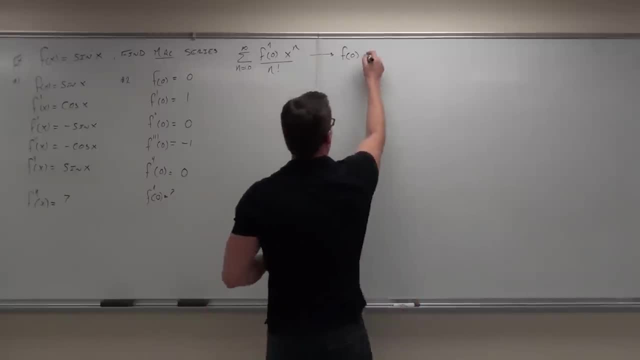 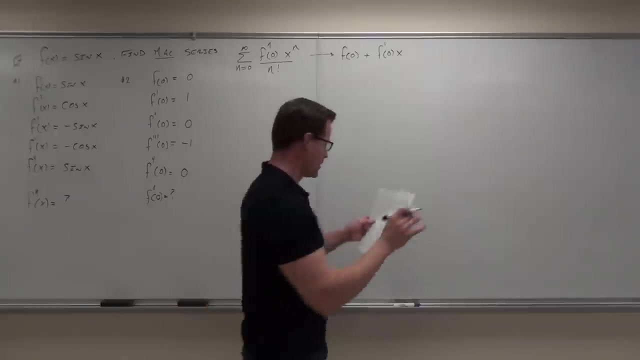 Taylor would be f of c, no problem. Then we go: okay, cool, we add to it the first derivative at zero times, x to the first all over one factorial. That would simply be one. We'd be okay with that one. 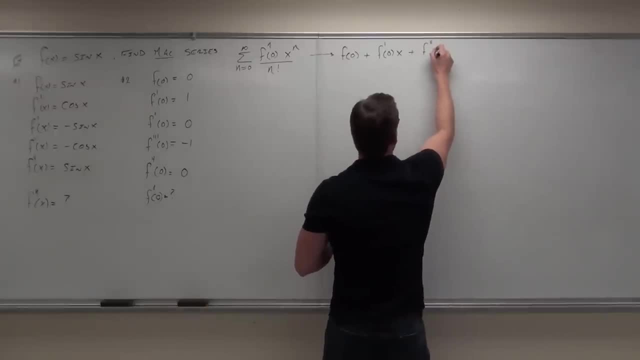 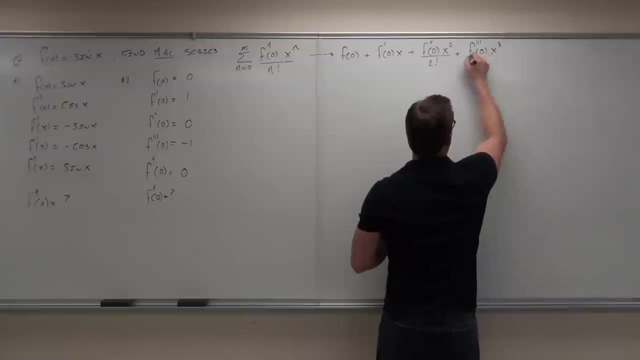 Then we'd have the second derivative at zero. We would have x squared over two factorial, no problem. Then we'd have the third derivative at zero. We'd have x to the third, all over three factorial. Then we'd have the fourth derivative at zero. 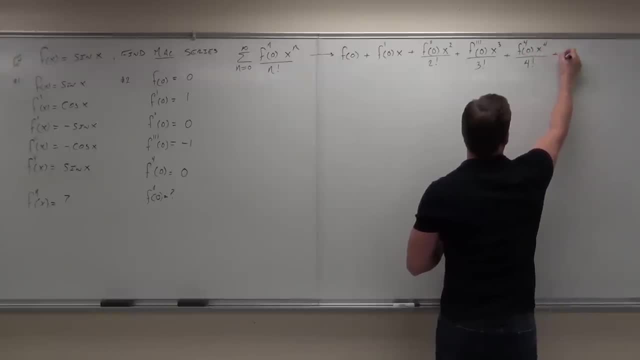 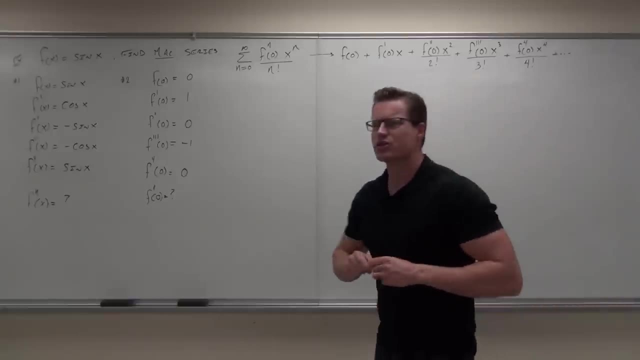 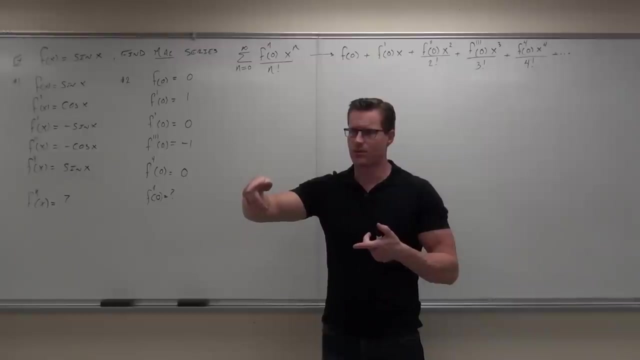 x to the fourth power, all over four factorial, and we would not stop. I want to show of hands if you can get from here to here and you understand what I'm doing. Show of hands if you do that, Okay. so our Maclaurin series says: when you plug in zero. 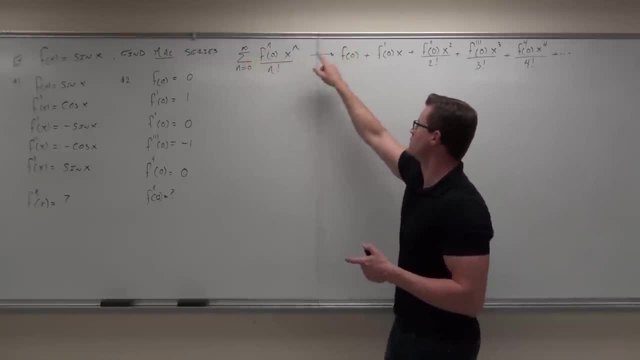 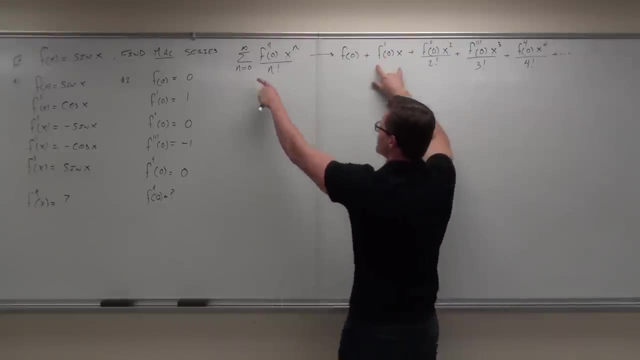 you get no derivatives. bam, no derivatives. add zero X to the zero is one, zero factorial is one. Then you plug in one. so our first n equals zero term, n equals one term. Plug in one, you get a first derivative, no problem. 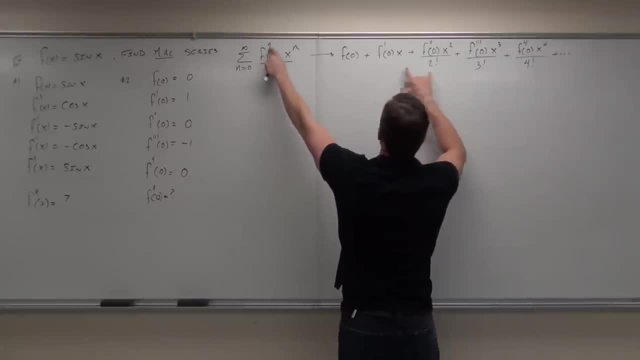 X to the first, all over one. One factorial. plug in now two, you get a second derivative. You get x to the second, all over two factorial. Now plug in three, you get a third derivative. X to the third, all over three factorial. 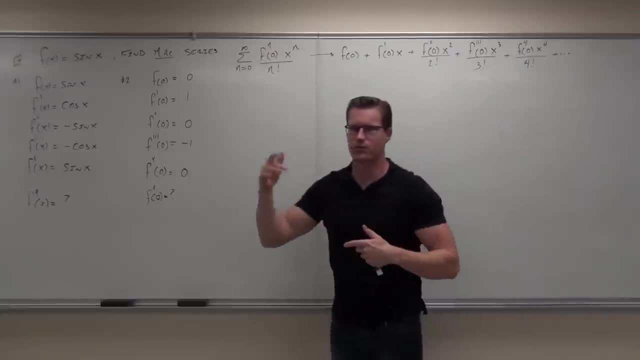 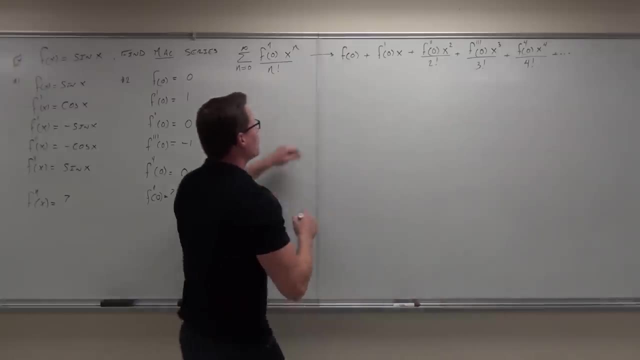 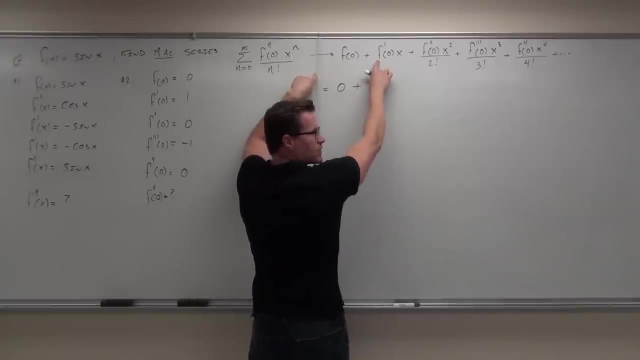 You plug in four: fourth derivative of zero. X to the fourth over four, factorial. Are you paying attention? Does it make sense to you? Let's plug in the numbers: What's f of zero? What's f- prime of zero? 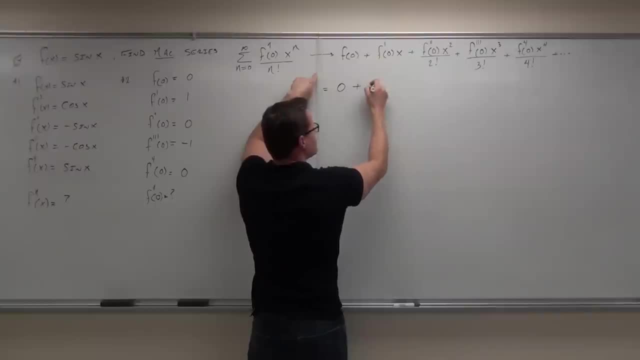 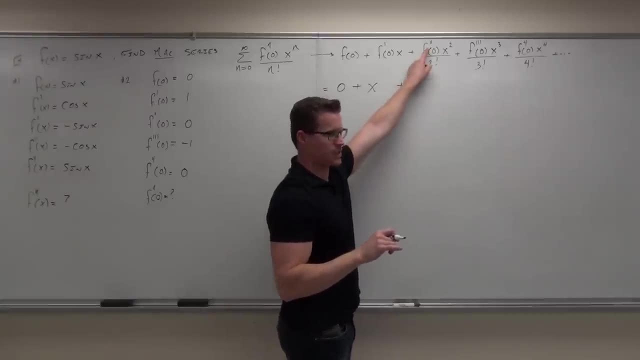 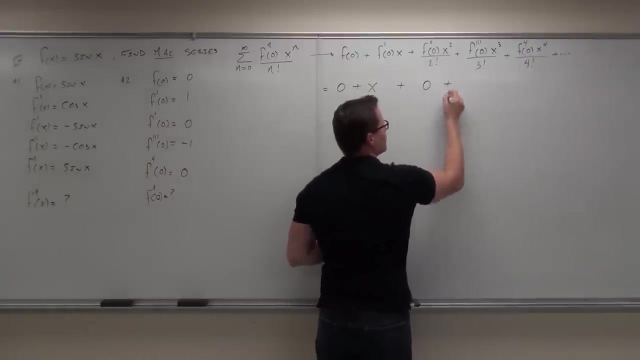 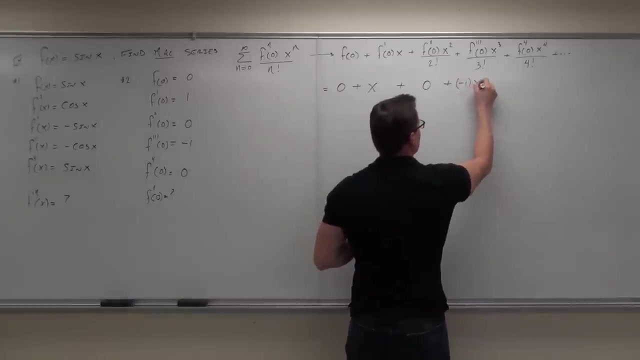 One. One. X is x. Does that make sense? Watch carefully. What's the second derivative at zero? Zero. This is why we did this, So this whole thing becomes zero. What's the third derivative, One? What's the fourth derivative? 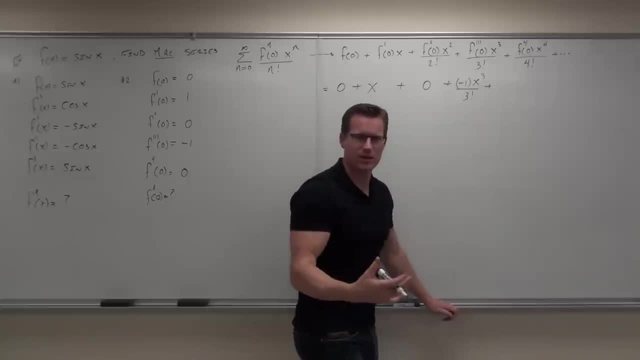 Zero, Zero. do you guys see what I'm talking about? Are you with me? You know, I don't want to lose you here, but I want you to be with me. But I've gotta move too. So do you get the function at zero, zero? 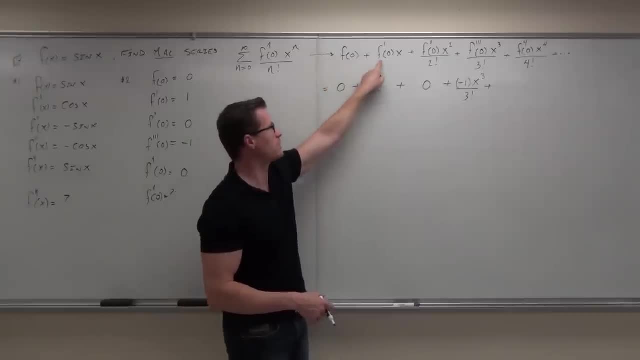 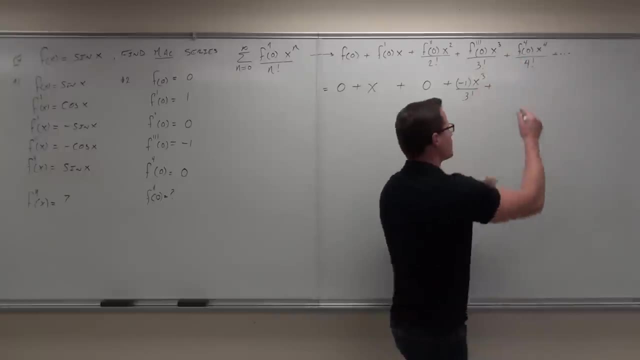 Yes, No. First derivative at zero is one. Second derivative at zero is zero. Third derivative at zero is negative. one. Fourth derivative at zero is Zero. Zero times anything is zero Plus. how about the fifth derivative? Is it gonna be zero or one, or negative one? 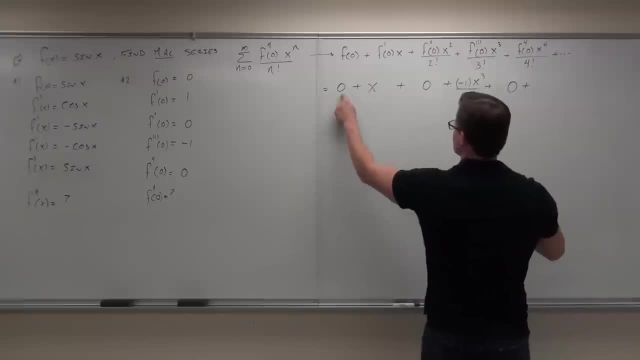 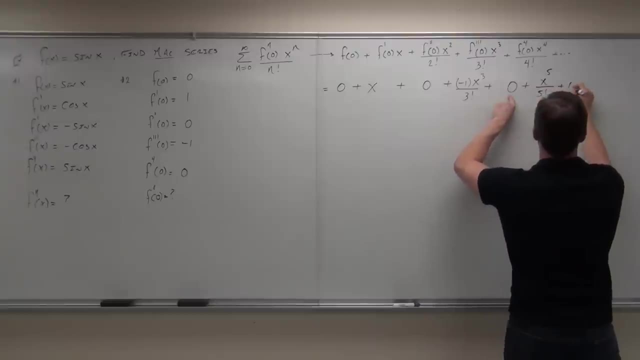 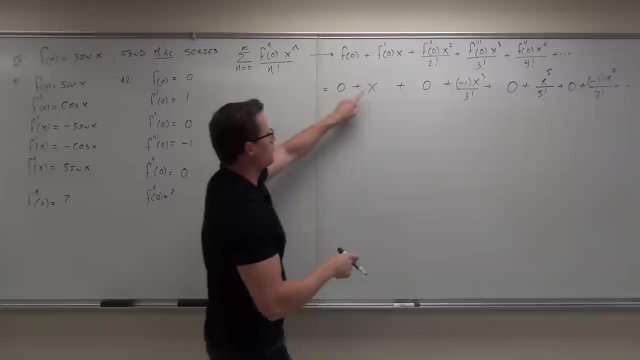 One. It's gonna be one Zero, one zero negative one zero: 1, 0, negative 1, 0, 1, 0, negative 1, 0, 1, 0, 1, 0, negative 1, 0, 1, 0, negative 1, 0, 1, 0, negative 1.. 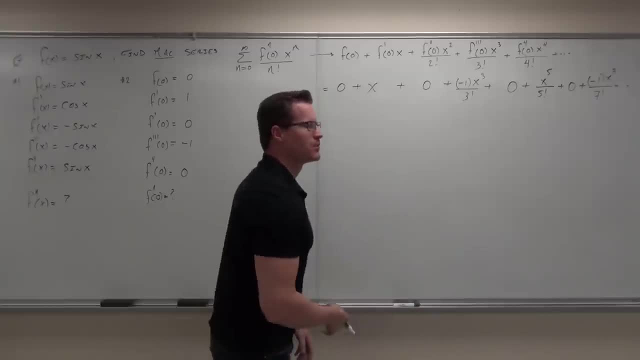 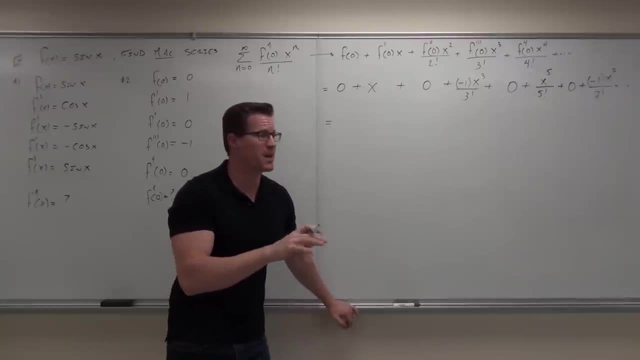 It's like a song Having fun, right, This is cool. Well, now let's simplify this a little bit. Do I really need to include all my zeros? No, Now we come to a fine point that maybe it makes a difference, maybe it doesn't. 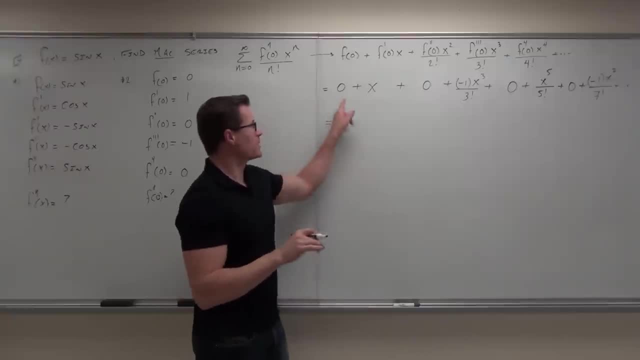 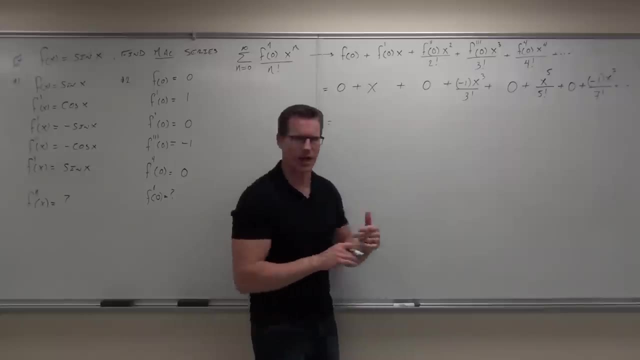 I like to think that it does. okay. We're going to come to a fine point. This really is the first term, Second term, third term, fourth term, fifth term. We're going to redefine our series here, because what's going to happen is, if I omit my first and my third. 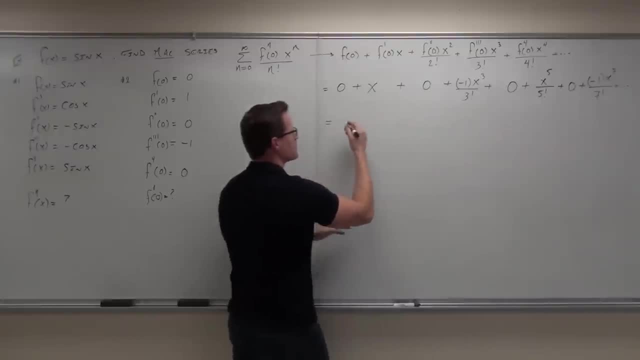 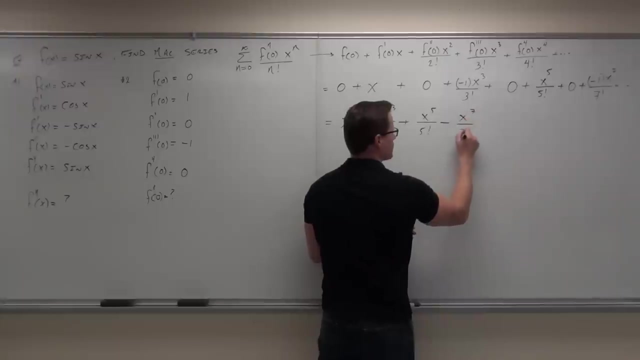 my zeroth and my second term, and my n equals 3 and 2 and 4, I'm going to get x minus x cubed over 3.. 3 factorial plus x to the 5th over 5. factorial minus x to the 7th over 7 factorial plus blah, blah, blah, blah, blah, blah, blah. 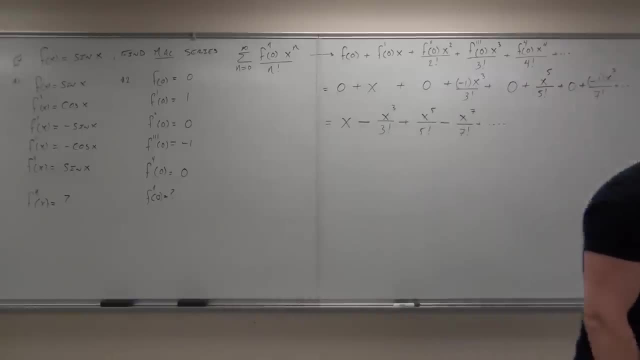 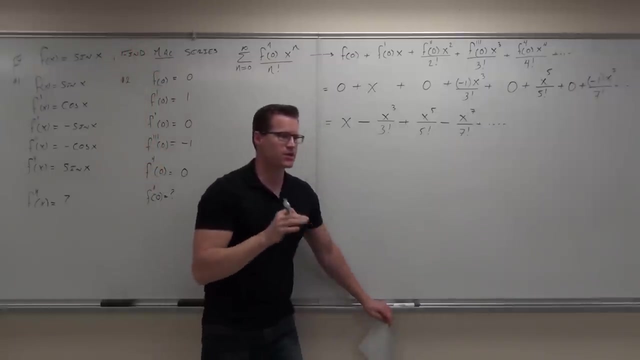 forever and ever and ever and ever. okay, Any quick show of hands, if that makes sense to you. Now, if I try to define this as a series in terms of n, my n's are going to compete. For instance, my n's are stemming from here, aren't they? 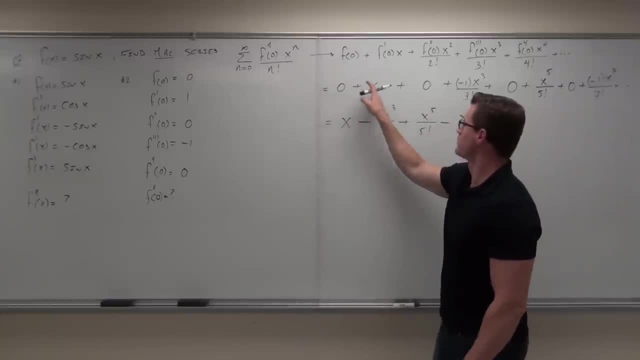 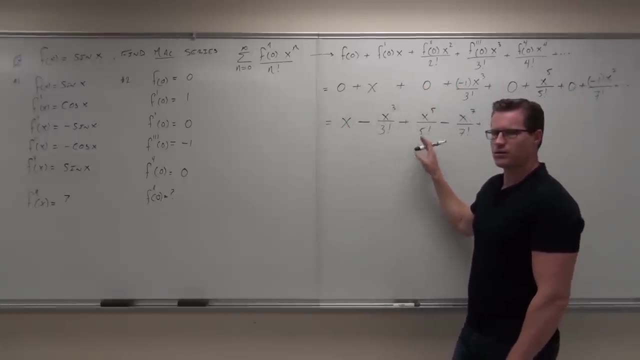 Are you with me? Which means that this is going to be my zeroth, first, second, third, fourth, fifth, sixth, seventh, But this I want to consider my first, second, third, fourth. So can I define a series in terms of n? 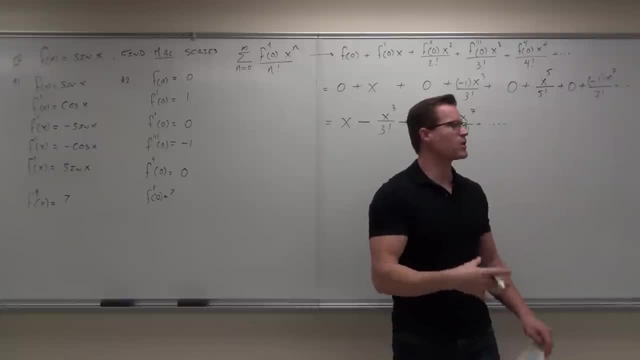 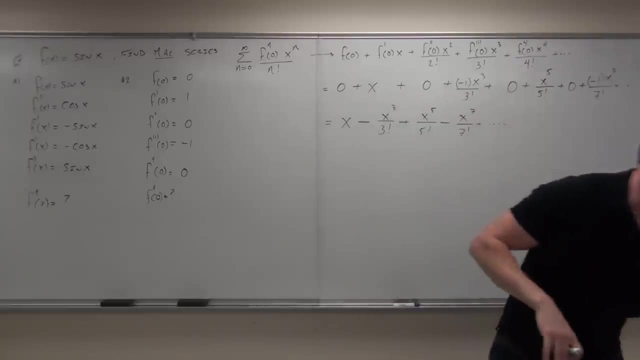 Yes, but understand, it's a different n, It's a different series. So what I'm going to do right now, I'm going to use the letter k, so we have no ambiguity as to what's going on. okay, We're going to define this thing right here as a different series. 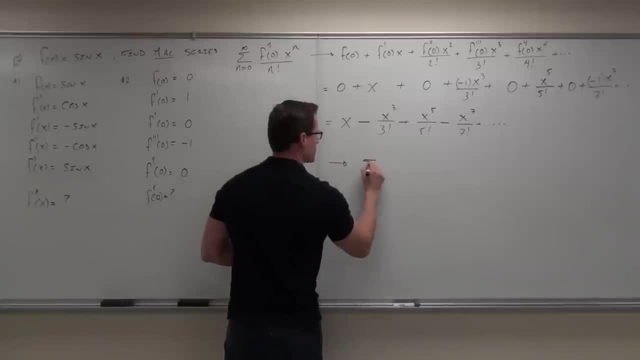 So tell me, on this series from k- k equals 1- to infinity, Tell me what's going on. Tell me something about that that you guys see: Alternate, It's alternating. Okay, that's easy, Let's start with that. 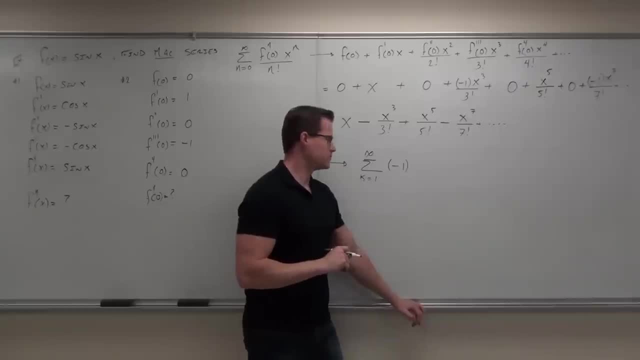 Negative. 1 to the. is the first term positive or is the first term Positive? Oh, you know what? let's start at zero, actually Start at zero, just to keep our, our, the corn series in mind here. 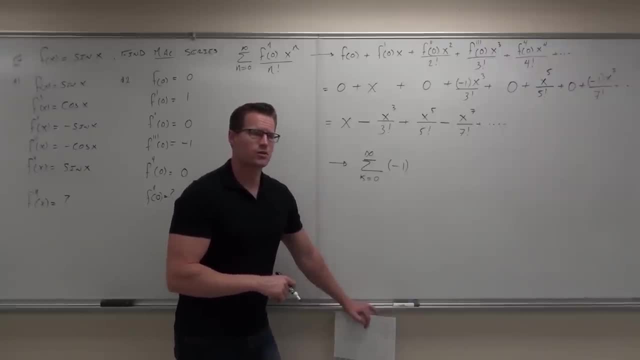 Start at zero. First term positive. first term negative, Positive. So the only way that we're going to do that is if we do N? K minus 1.. Oh, which one K N minus 1 would give us zero. that'd be negative 1.. 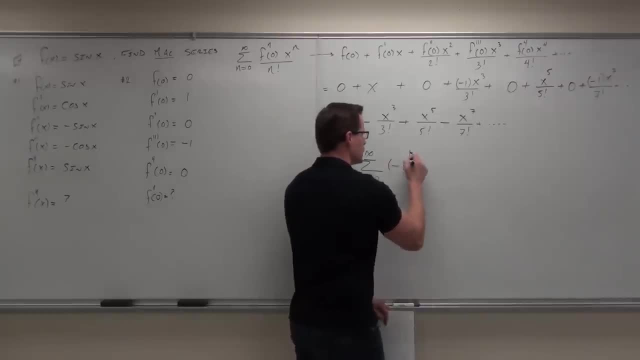 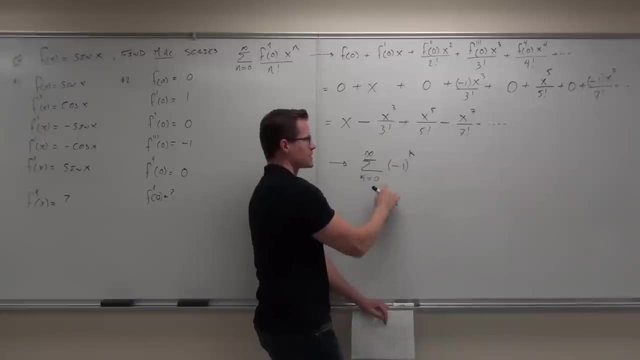 K, just k. It'd just be k, Because if I do negative 1 to the zero, I get positive 1.. Does that make sense? Yeah, If I do negative 1 to the first, I get negative. Second, I get positive. 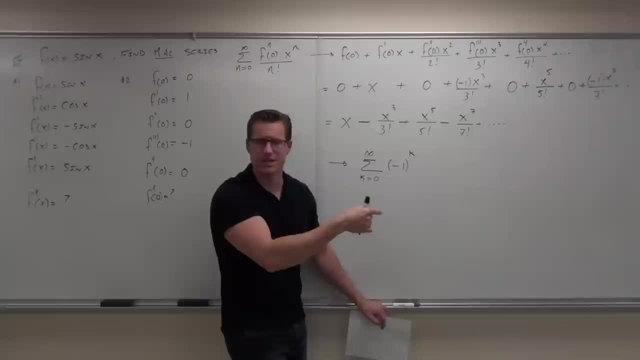 Third, I get this is going to work for us. That's where we're getting our alternating from- is negative 1 to the k. Are you sure you're okay with it? A-okay, A-okay, okay, You get an A because you're not a problem. 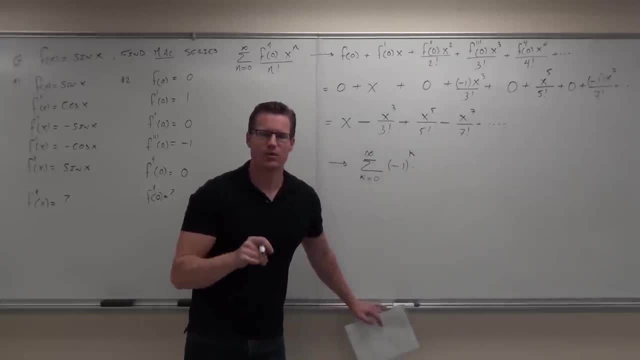 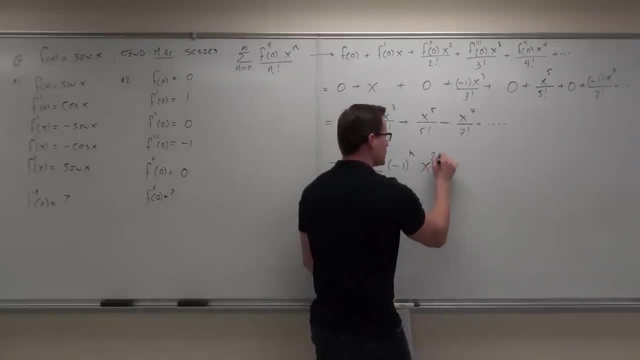 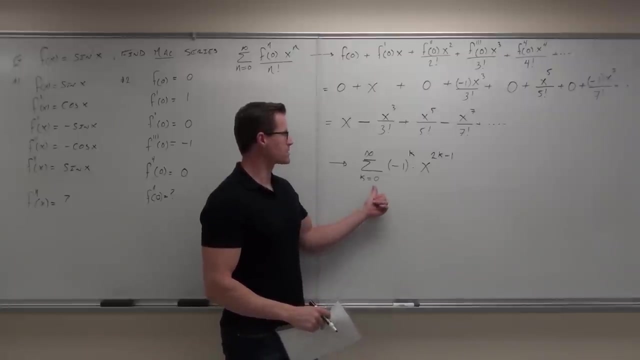 Now multiply. Tell me what our x's are doing. What are the powers of x doing? Odds, Odds, Odds. Hey, we just dealt with odds. We just dealt with odds. Well, let's see if that works. If I plug in zero, wait a minute- I'm going to get negative. 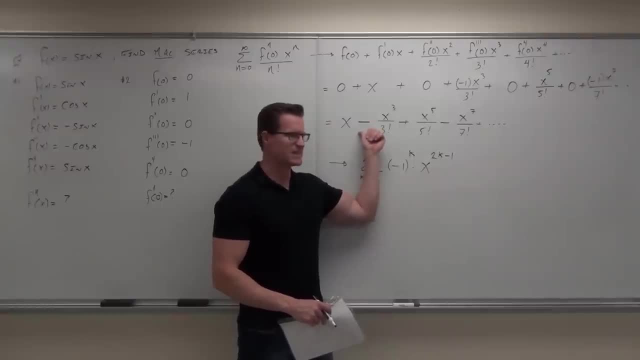 I'm going to get is this: x to the negative 1 power. How can I change it to make it work? That'll work, That'll work. So if I do zero, okay, what's 2 times zero, Zero. 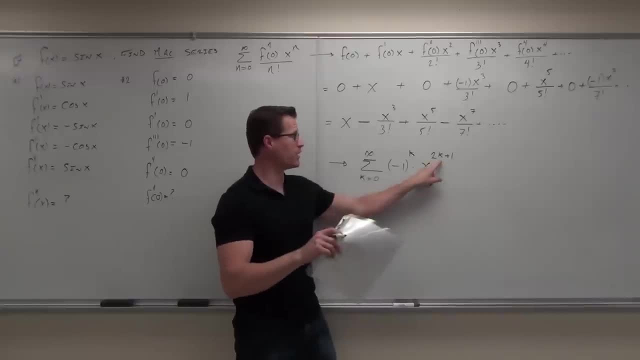 Plus 1? One One. Let's do the plug-in 1, now plug-in 1.. So remember, zero should be my very first technical term. The plug-in 1 should give me this term. Are you with me? 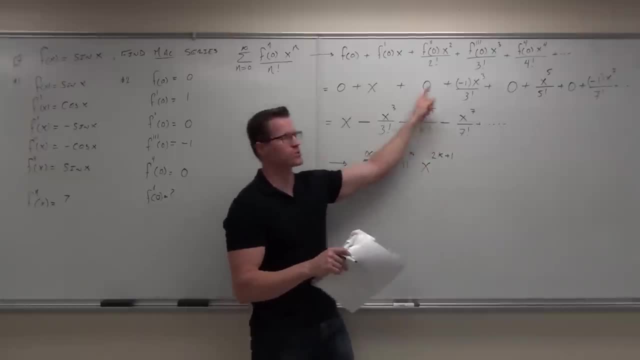 Plug-in 2 should give me this term. That's why we redefined our k's, so we don't get ambiguous with that. So plug in your plug-in 1.. 2 times 1 is Plus 1. Plus 1.. 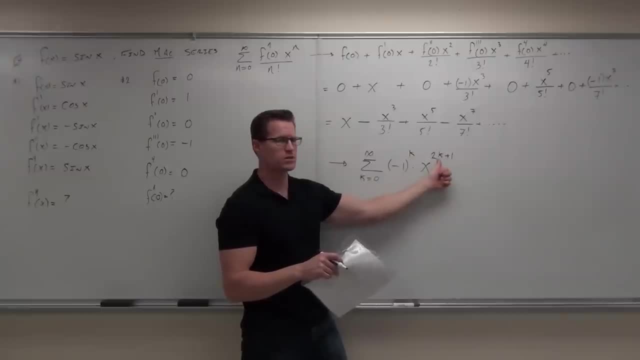 Plus 1.. Hey, plug-in, let's plug-in. 2.. 2 times 2 is 4. Plus 1? 5.. Boom. Now what's the denominator? doing 2k plus 1.? It's exactly the same, but with a factorial. 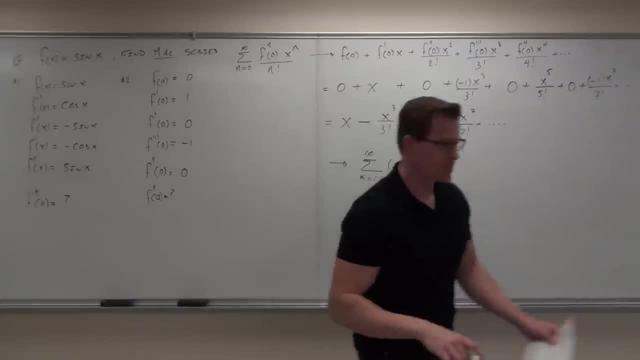 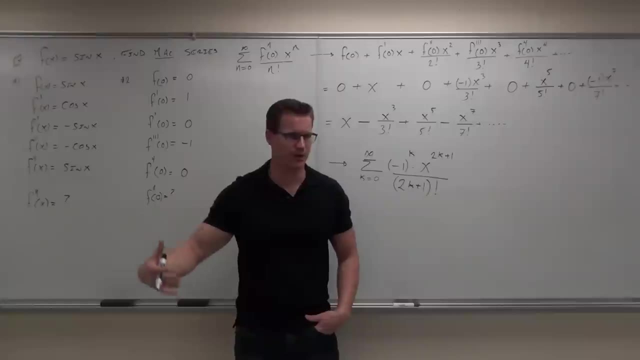 You better make sure this is accurate before we go any further. okay, So we start off. derivatives are really easy, Our pattern is really easy, but there's no way for us to explicitly define it, because we don't know what this is going to be. 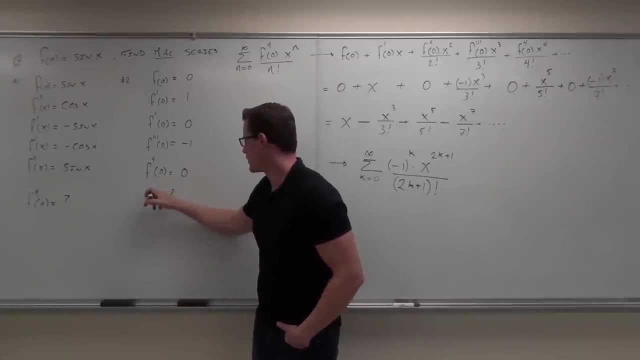 the nth derivative of f. I don't know. It's supposed to be a little n, by the way. I don't know what that's going to be. So we write out the terms. Maclaurin's series says, you know what? 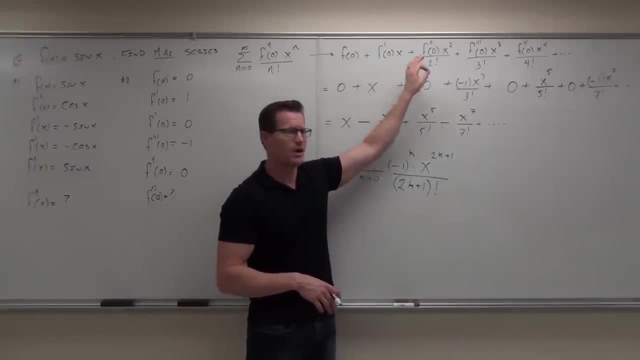 You're going to have. f is 0, f prime is 0 times x. f double prime is 0, x to the second over 2 factorial, x triple prime of 0, x to the third over 3 factorial, and so forth and so on. 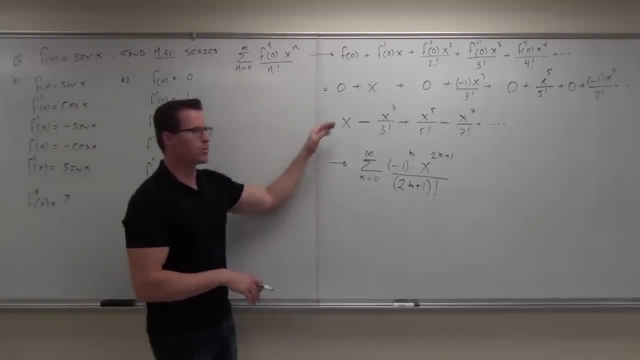 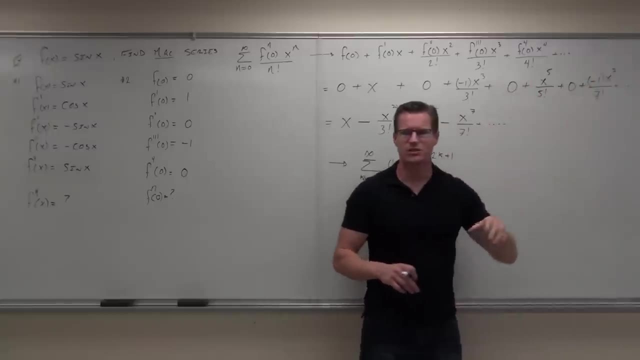 Except with our pattern that we just found. we know we're going to go coefficients-wise: 0, 1, 0, negative 1, 0, 1, 0, negative 1.. That's going to basically omit half our terms. 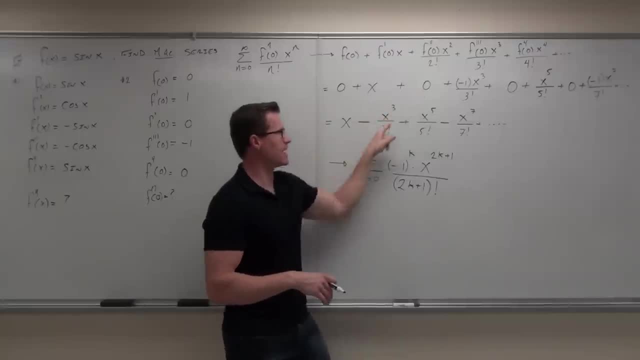 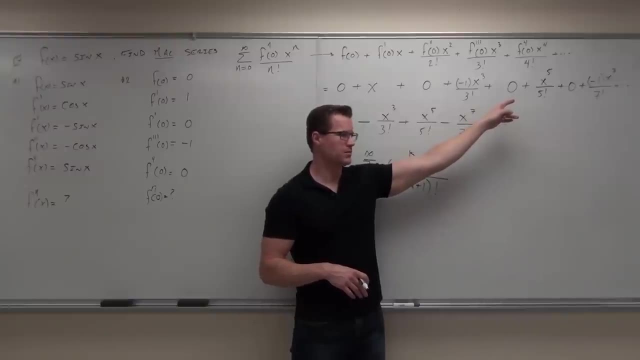 They're all gone. So we just take the terms that actually have something, and what that does is it takes a series with like 2 n terms and gives us a series with n terms, Or practically we have a series with n terms. 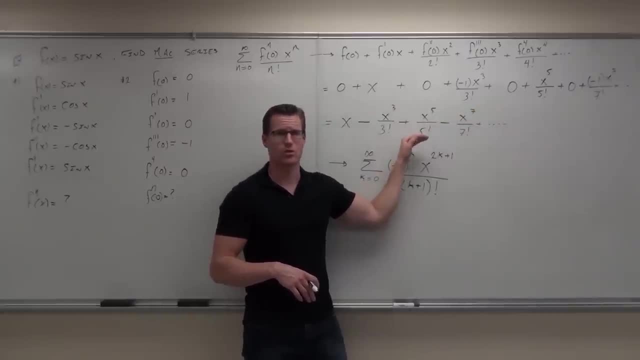 and we get a series with n divided by 2 terms, or k terms, where k equals n divided by 2.. Well, if that's the case, let's redefine it So we don't get confused. on the terms themselves, We say, OK, let's start: k equals to 0 and go to infinity. 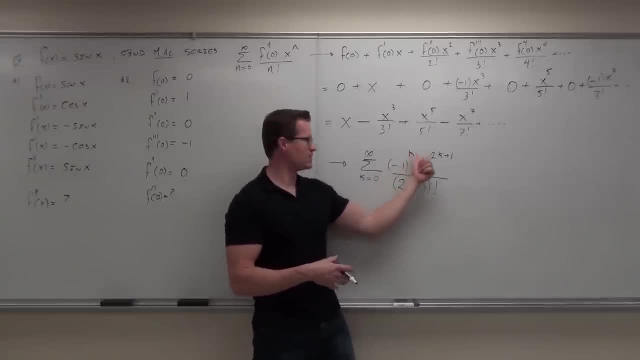 Then we have: what's that say? What's this part say for your series? Alternating? It's alternating. So this says we're alternating, No problem. This says we're taking x to the odd powers over odd numbers: factorial. This is our Maclaurin series. 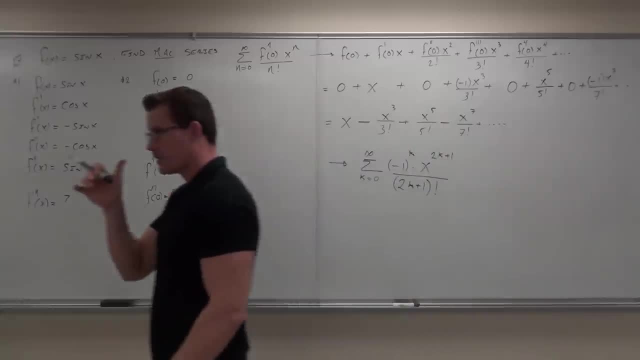 Now what are we going to do with our Maclaurin series? Say it again: Ratio, Definitely ratio test- It's got a factorial in it, right? We're not done here. You see, what we've done is we've defined. 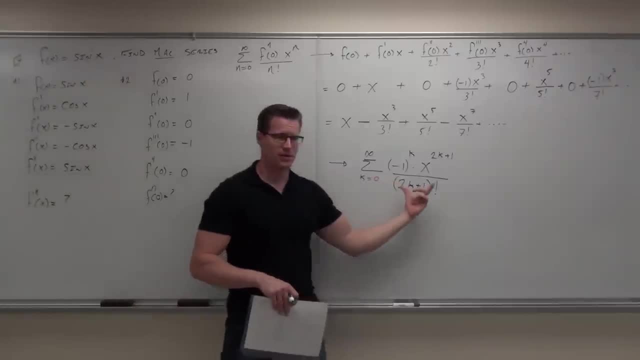 we know that f of x equals sine can be defined by this Maclaurin series. It can be defined by it, But we've got to have an interval of convergence. so do the ratio test. Notice we're in k, So your limit should go from k approaches, not n. 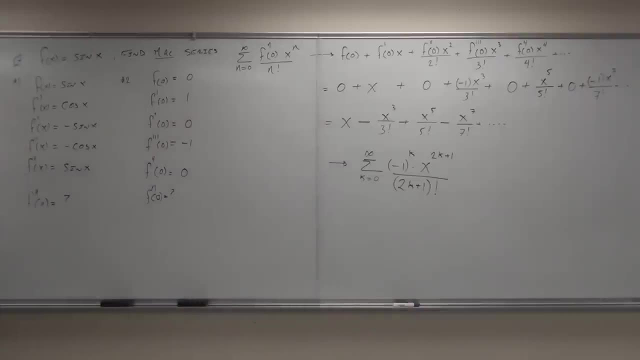 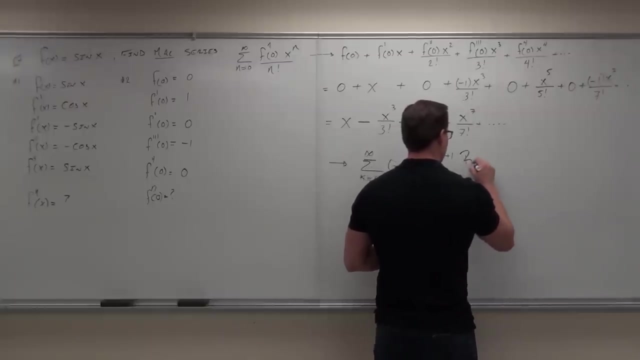 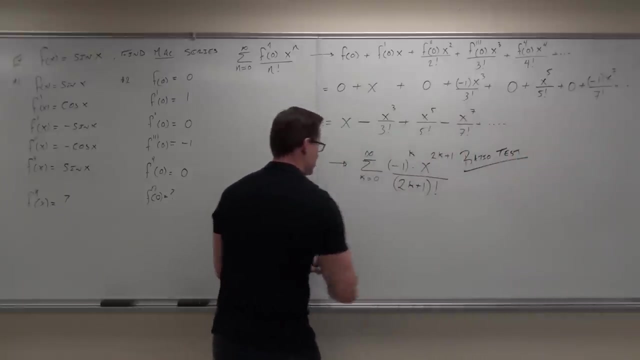 but k approaches infinity, So go for it. Go for it. This one should be quite easy for us. The simplification is going to be a little bit crazy, but it won't be too too hard. Oh my gosh. 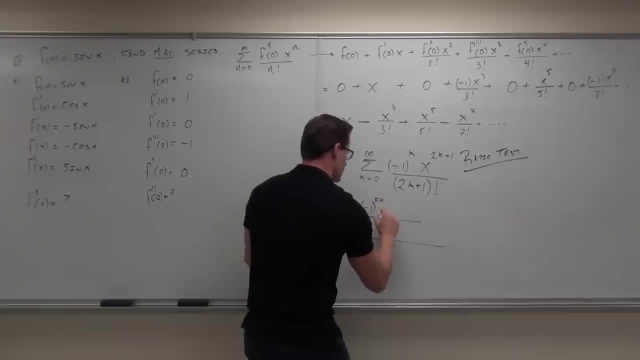 Negative 1 to the k plus 1 times x to the. You know what, If we do k plus 1 here, do you see that it's going to be 2 times k plus 1 plus 1?? Do you see that? 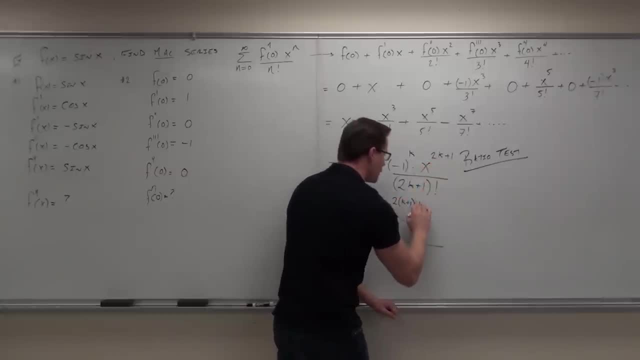 2 times k plus 1 plus 1.. Okay, And this is going to be the same thing: 2k plus 1 plus 1. factorial Sounds like we have a stutter, doesn't it? Plus 1 plus 1?? 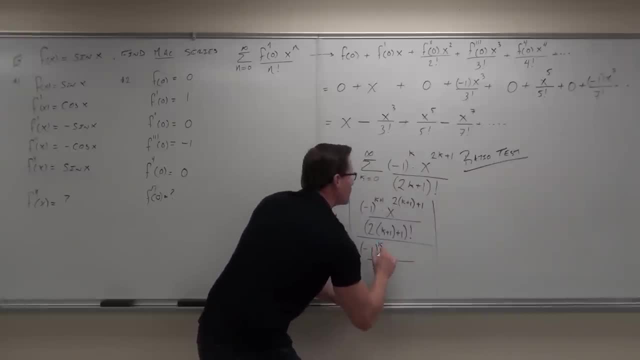 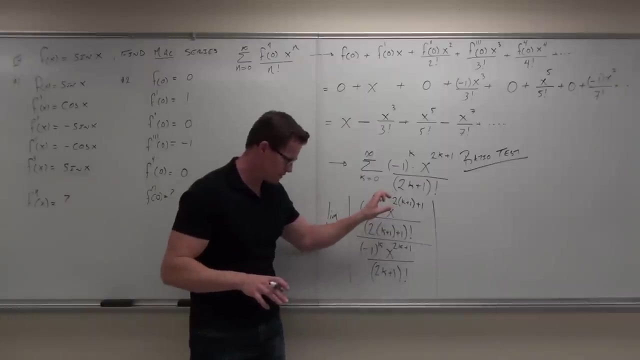 No, no, no. Negative: 1 to the k, x to the 2k plus 1, all over 2k plus 1 factorial. No problem, But I want to make sure you guys have exactly the same thing that I have. 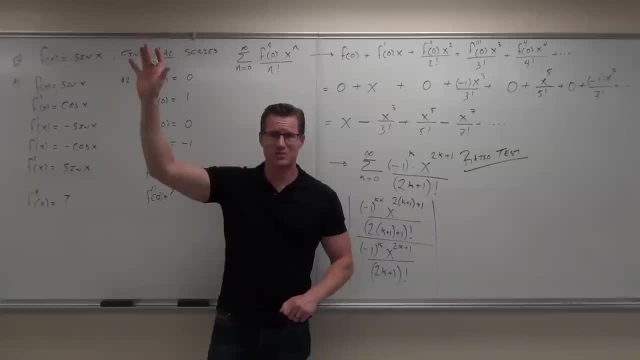 Here show of hands. if you do have exactly that, Is the ratio test getting pretty easy for you. Yes, It should be right. We've done it like 50 million times. What's going to happen to my negative 1s? 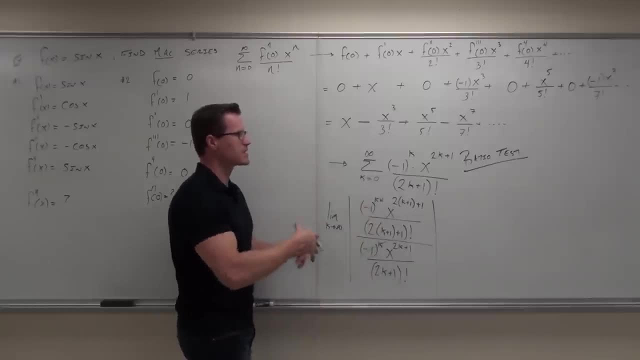 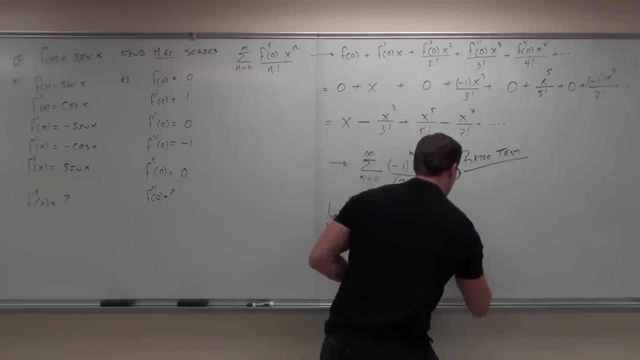 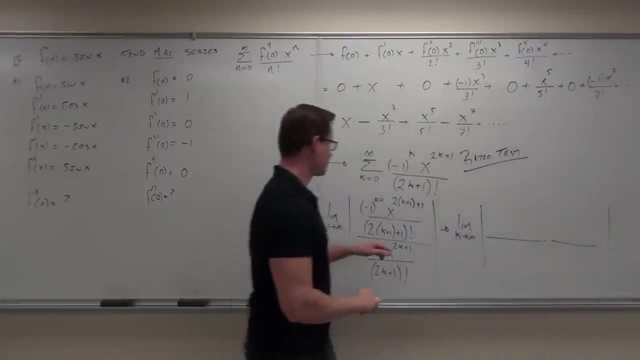 Cancel. I mean they don't matter. Absolute value takes care of our negative 180 power. Now, of course, we have a complex fraction. We'll write this as a limit. Don't change your k to an n- Absolute value. don't lose that. 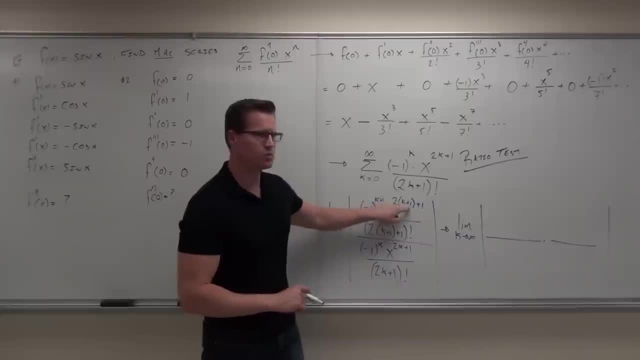 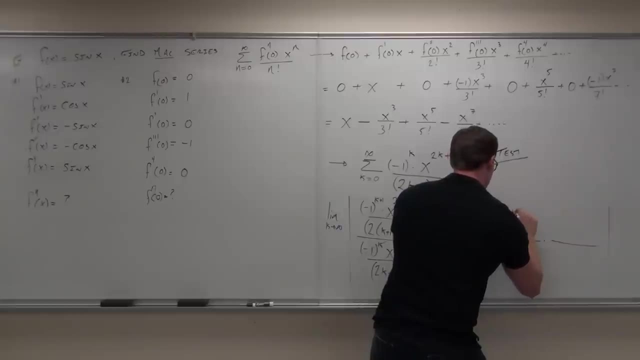 On our main numerator. let's distribute. Notice this: You're going to have 2k plus 2 plus 1. That's 2k plus 3.. Do you guys get that one? Yeah, 2k plus 3, all over 2k plus 3. factorial. 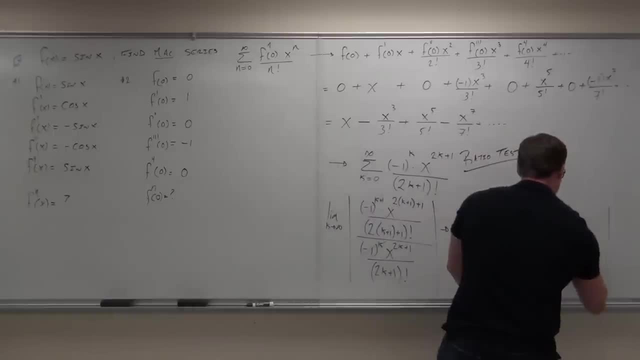 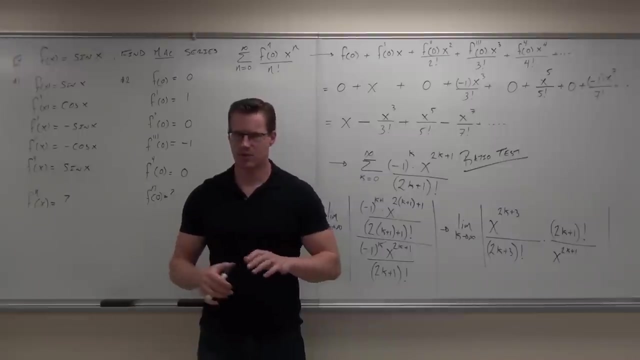 Here we're going to get 2k plus 1 factorial, And then here x to the 2k plus 1.. You all still all right with that one. Just some algebra. We've multiplied by the reciprocal. What should you do now? 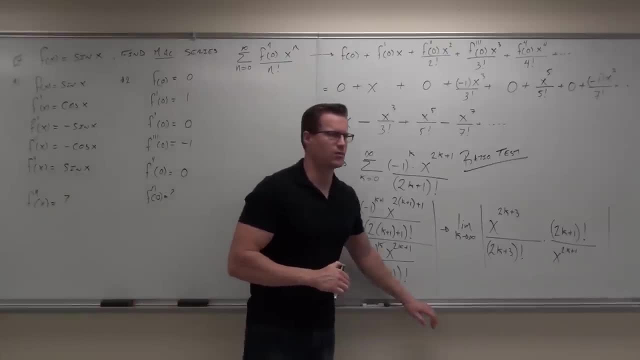 Simplify as much as you can. Now be careful with this. Can you simplify x to the 2k plus 3 and x to the 2k plus 1?? I want to say yeah, Yeah, I want to say yeah too. 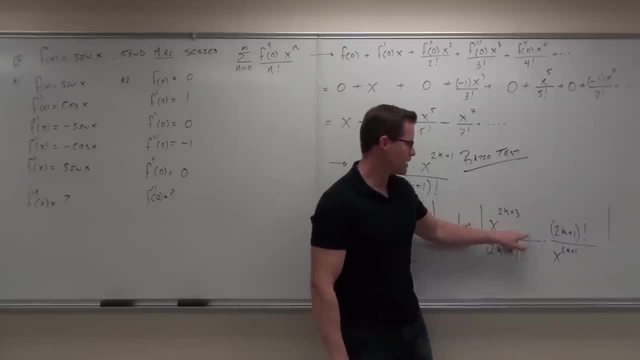 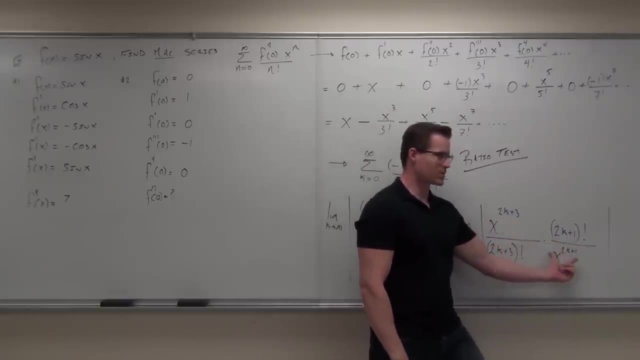 So if this is x to the 2k plus 1, this is x to the 2k plus 1 plus 2.. Do you see the plus 2 in there? This is x to the 2k plus 1 plus 2.. 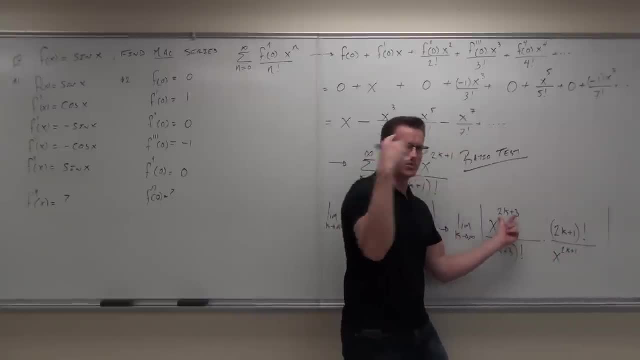 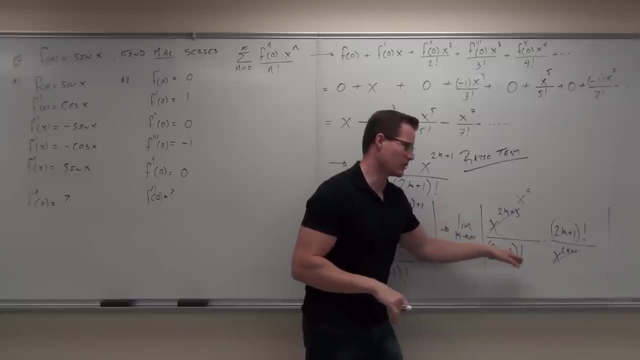 That plus 2 is really just an x squared. That's just an x squared, just an x squared. Do you get that? Yes, Then you get the whole thing. okay, Now, this one's a little weird. We've got factorials. We've done this only one time before. If this is, 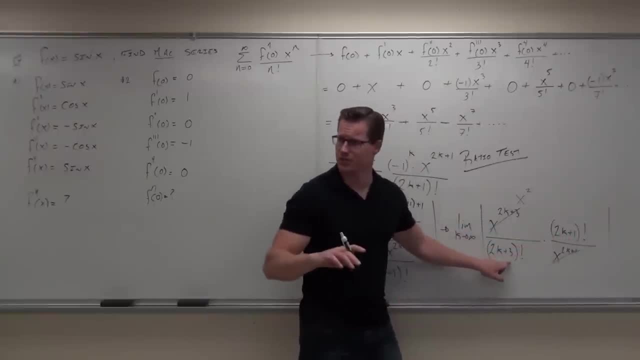 2k plus 1 factorial. this is 2k plus 3 factorial. Think about this for a second. 2k plus 3 factorial means: listen carefully, I'm not going to write it again, I've already done it This. 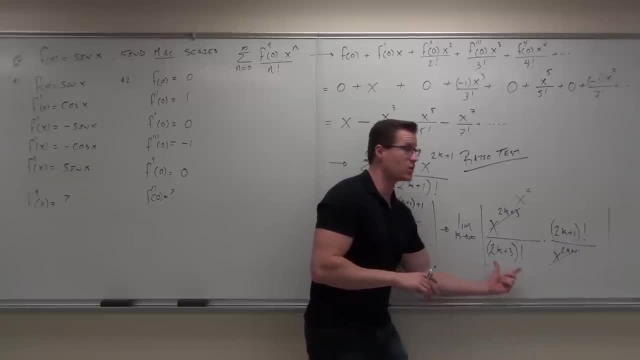 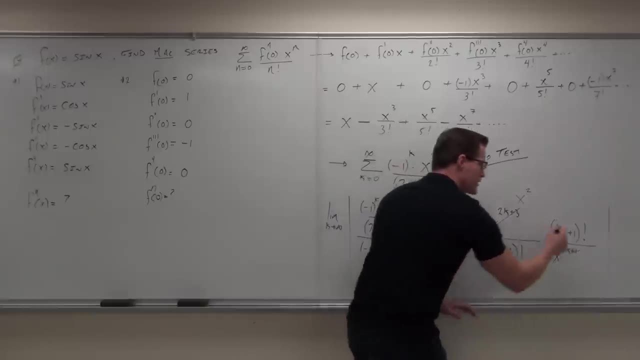 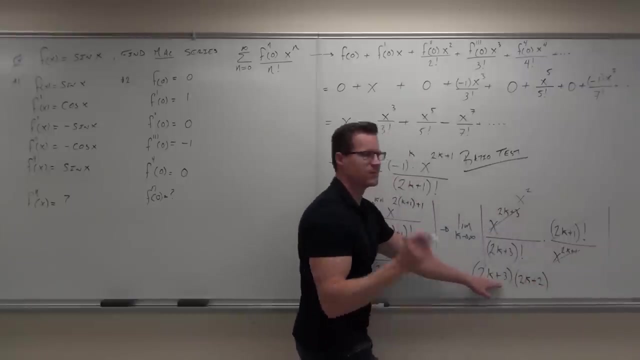 means 2k plus 3 times 2k plus 2 times 2k plus 1 times everything below it. So what you simplify this. this is completely gone. You with me, This one. you have the terms until you subtract down to 2k plus 1.. So you have 2k plus 3, no problem, You have the term. 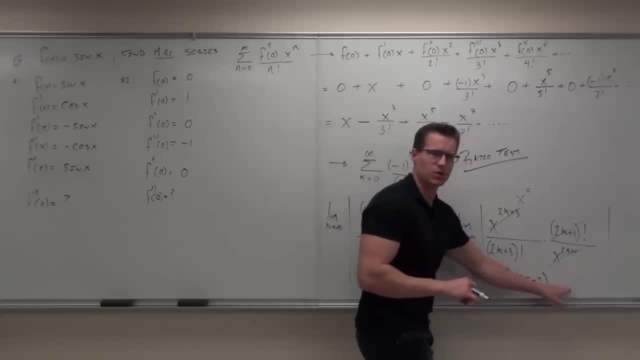 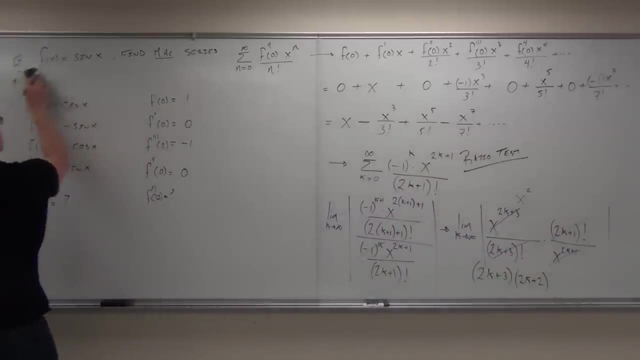 2k plus 2,. no problem. The next term would be 2k plus 1,, would it not? Yes, That's going to simplify term by term with this one. So our limit therefore becomes the limit as k approaches infinity. What do we got? 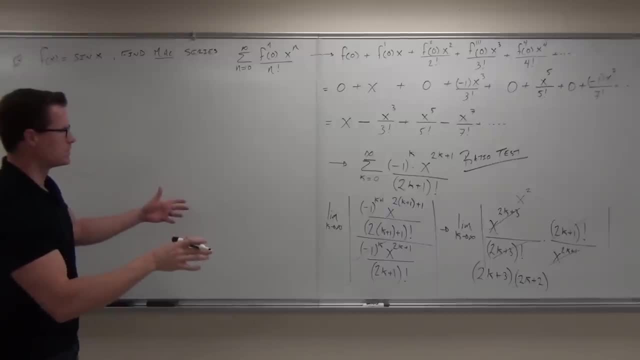 1 over 2k plus 3.. Do we need an absolute value here? No, You actually don't. You have an x squared, don't you? Or x Positive. These are all going to be positive, Just make sure. 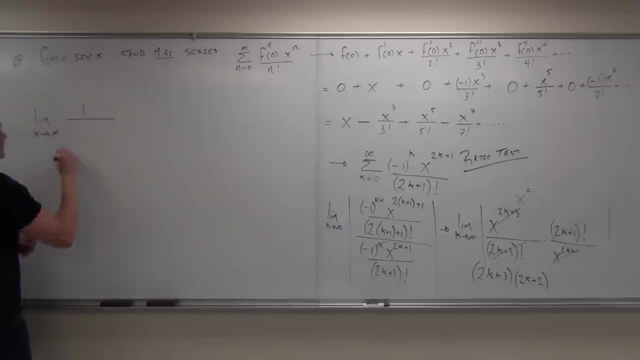 you put them in the right place, We're going to have a 1 over what's going to be on our denominator, 2k plus 3, 2k plus 3.. Times 1 over 2k plus 3.. 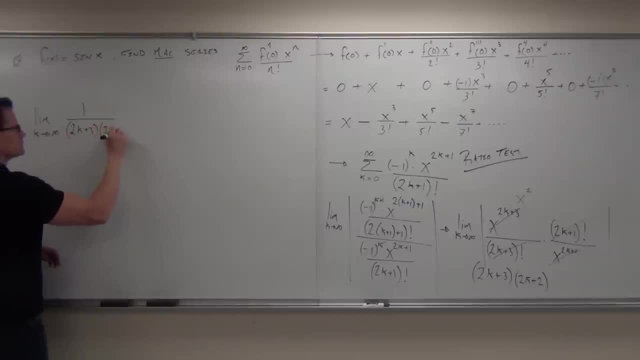 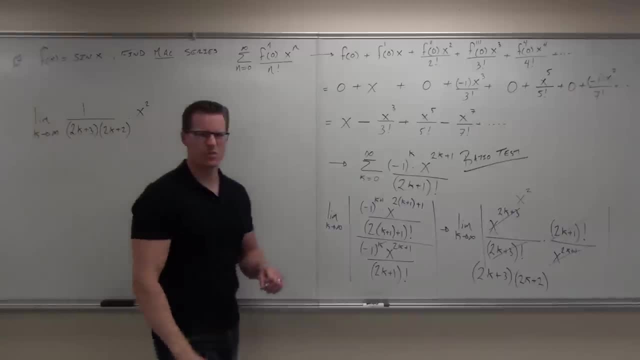 Times 1 over 2k plus 3.. Times 1 over 2k plus 3.. Times x squared. See where our x squared is coming from: 2k plus 3, 2k plus 1.. Now let's. 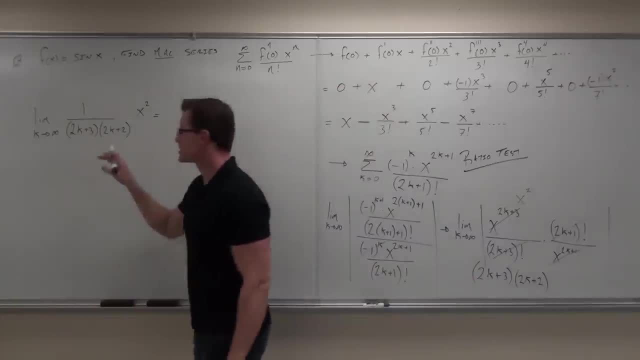 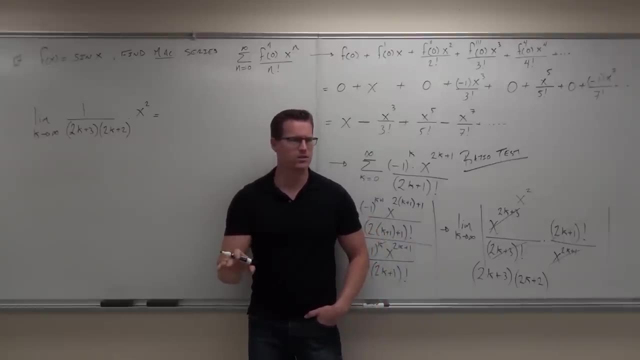 do this. Somebody have to tell me how much is this limit always going to be equal to as k approaches infinity? 0. 0. Always For any x. Yes, Remember you. tell me the x first right. You say x is blank. I say okay, pick a k. 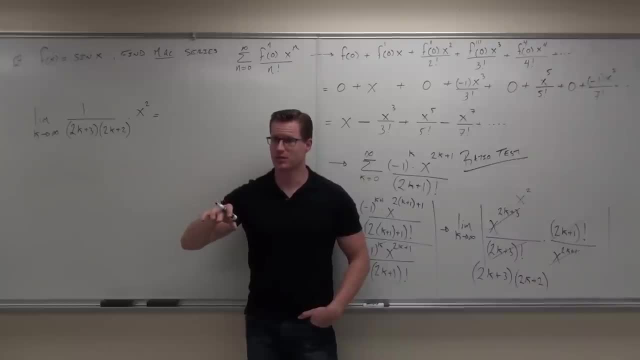 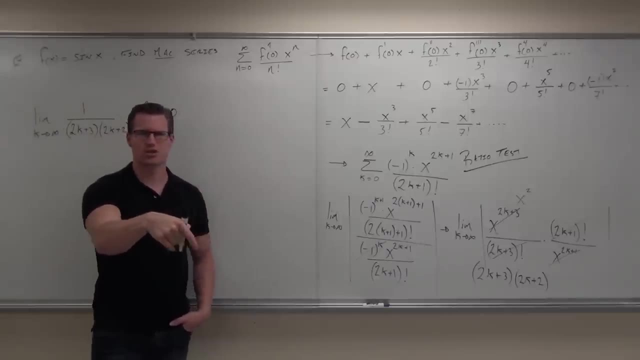 that goes to infinity. and now we take 1 divided by infinity, That's 0. 0 times any number that you've already told me is 0.. 0.. 0.. This is 0, and this is onlywhy. is this zero important, Tell me, in relationship with? 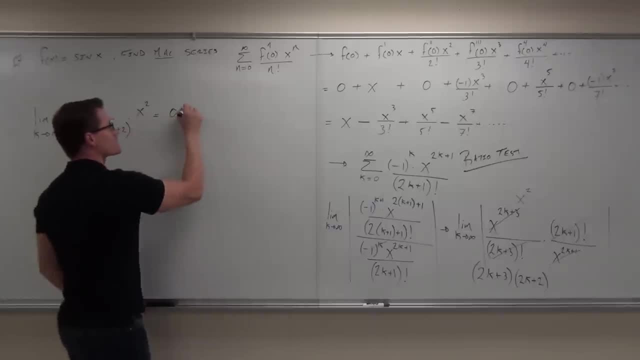 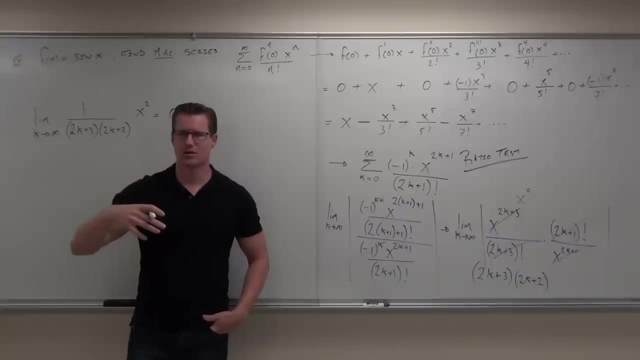 the ratio test why that's important: Less than 1.. Less than 1 says that it converges. right Now, does it matter the x for which we plug in to get our 0? No, we're going to get 0, no matter what x we plug in. So this thing equals 0 for all. 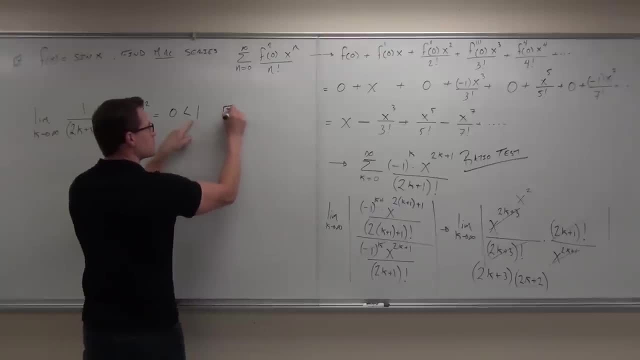 x. That means 0 is less than 1 for all x. No, Can you tell me my radius of convergence? 5 meters. The greatest convergence is infinity. What's my center? Does it really matter if we go to infinity? 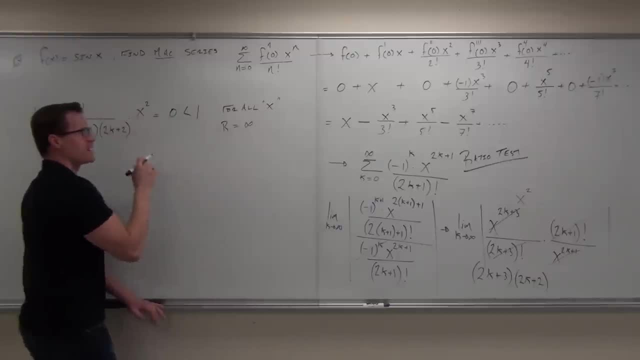 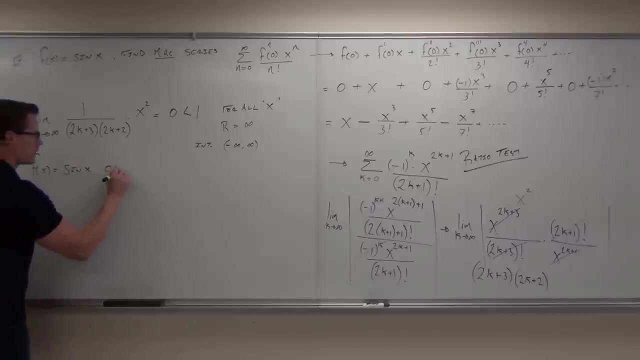 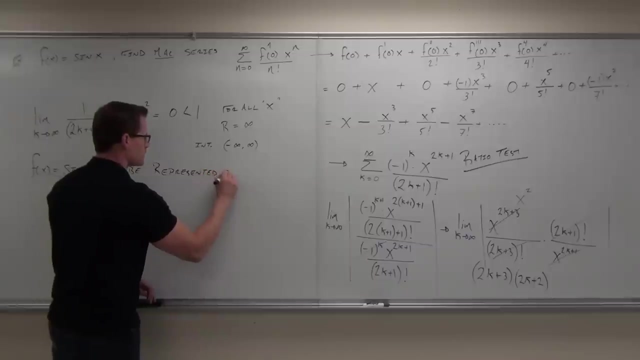 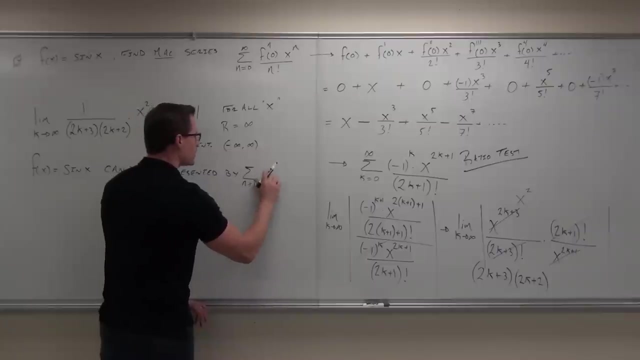 No, Not really, but the center is zero. What's my interval of convergence? The infinity of infinity. So here's what we say and you write this out: f of x equals sine. x can be represented by the series. n equals 0 to infinity. 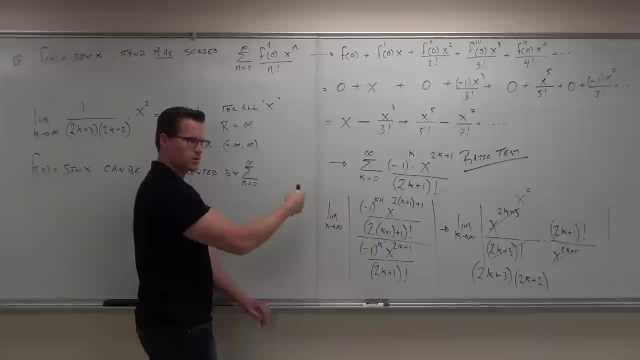 I'm going to use this series, okay, but I'm going to change it back to n's, just so we're our formats, Okay. Negative 1 to infinity: It's a dummy variable. It's a dummy k. It doesn't really matter what we use. 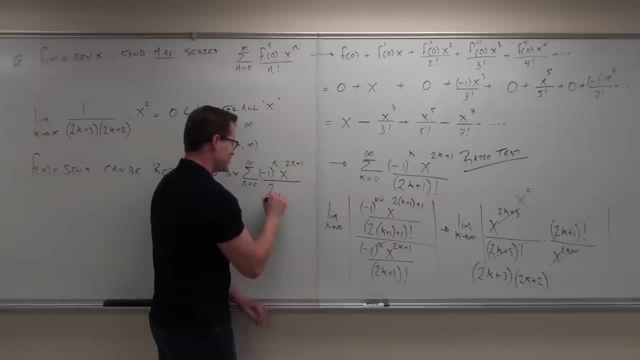 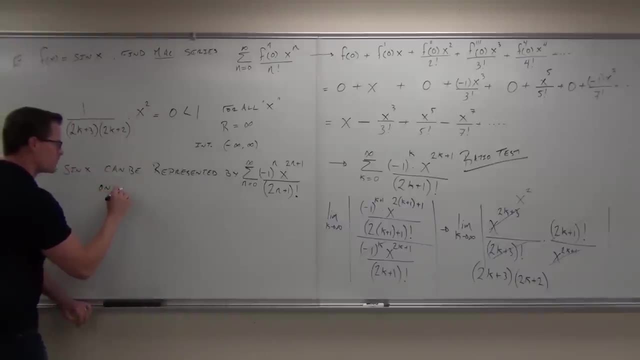 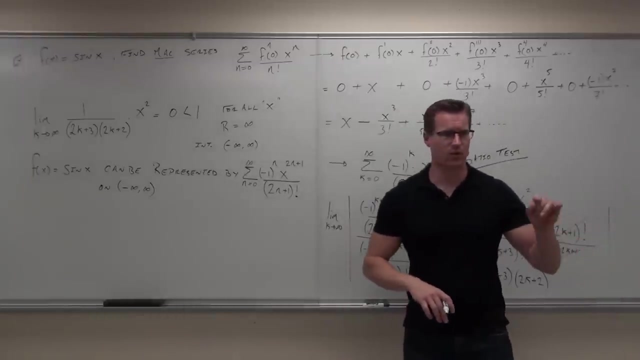 Dummy Plus 1.. 2n plus 1 factorial On the interval negative infinity to infinity, as we just showed. Hang on for one second. I know I'm going to go a couple minutes over here, but I want to show you one more thing. 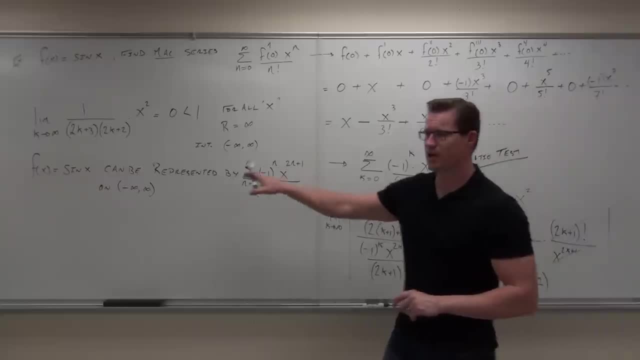 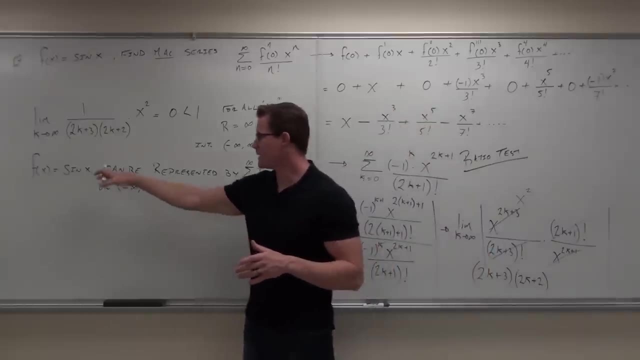 It's quite interesting. A quick show of hands if you feel okay with this so far. Now this is pretty fast Okay, Pretty freaking rad Okay. Which means if you want to find out sine of, I don't care what you want to plug in. 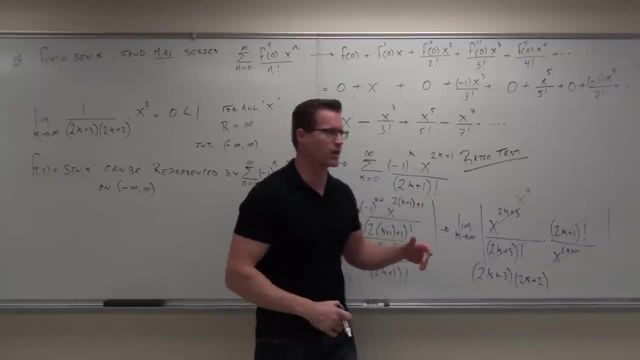 Sine of 3.. Sine of pi. Sine of pi over 2.. I don't care what you want to plug in. All you got to do is plug it in here. Remember, this is the series, right? This is where we got. 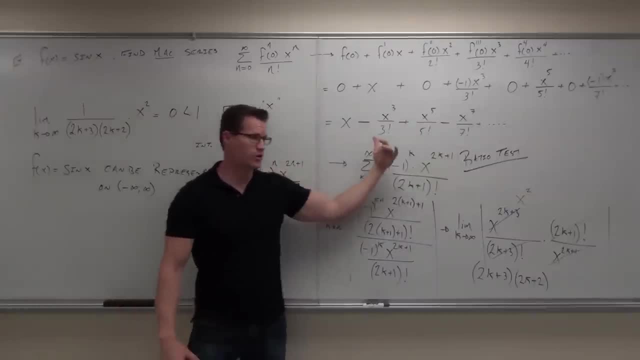 This is the same thing. This is the same exact thing. So you want to find sine of 3. Sine of negative 2. Sine of 1.846.. I don't care, Plug it in here And here. 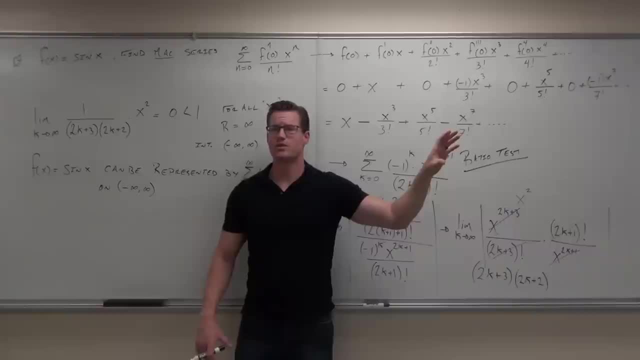 And here And here, Add up those 4nov Oh, and figure it out first however many times you want to, and you can be as accurate as you want. That's what the power series will do. Now the last thing. 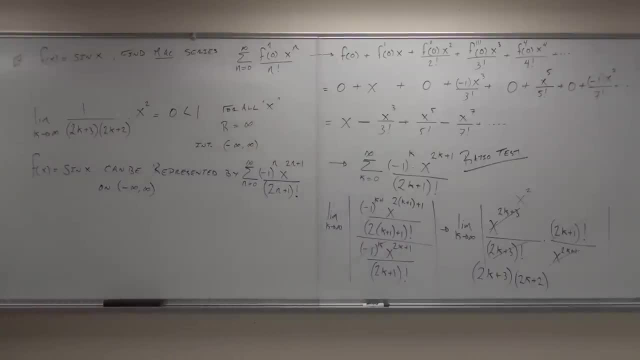 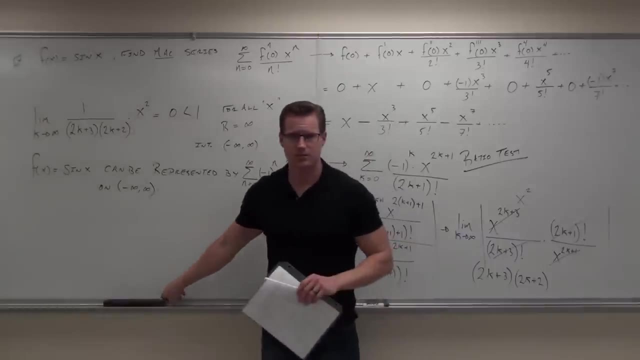 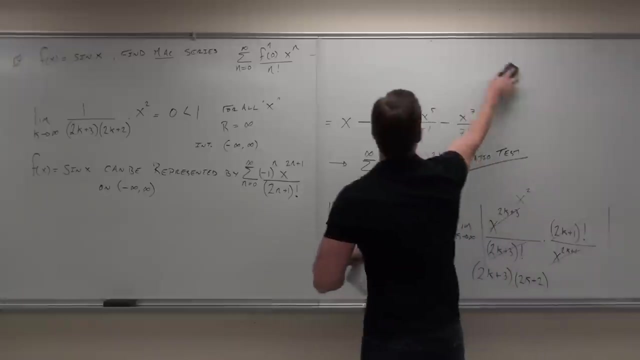 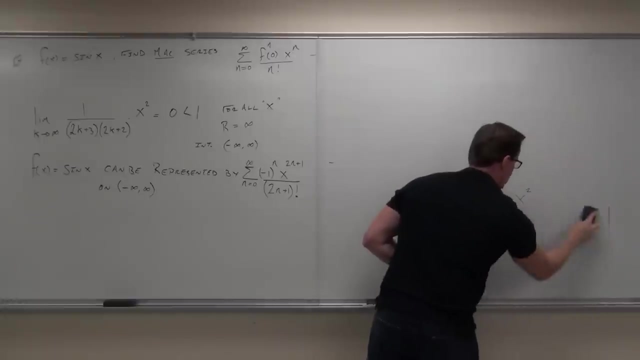 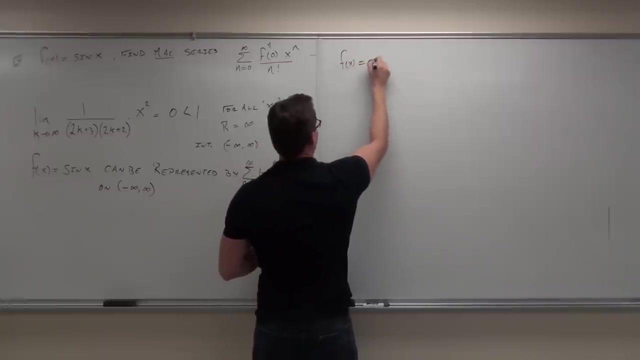 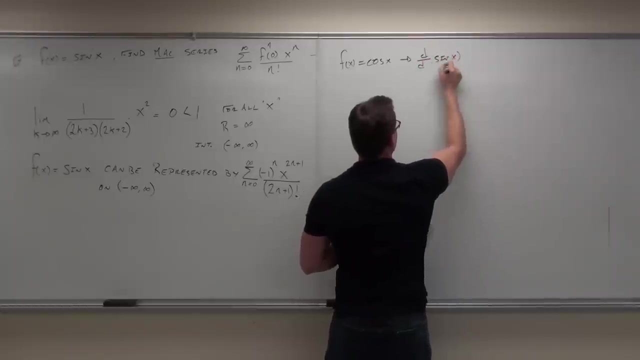 Very, very fast. This is interesting. Remember when I was telling you something about how we can take derivatives and integrals of power series? Remember we were doing that. We did it in the very end of our last session. Well, If f of x equals cosine x and cosine x is the derivative of sine x and sine x is x. 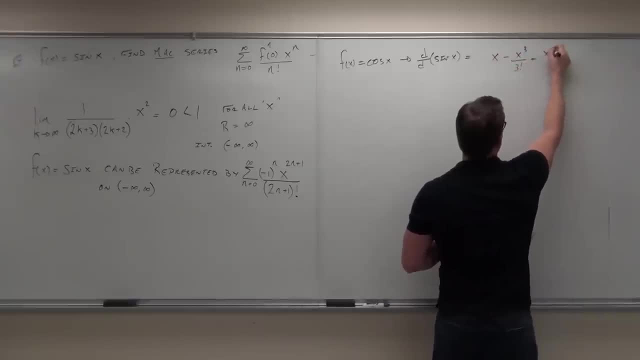 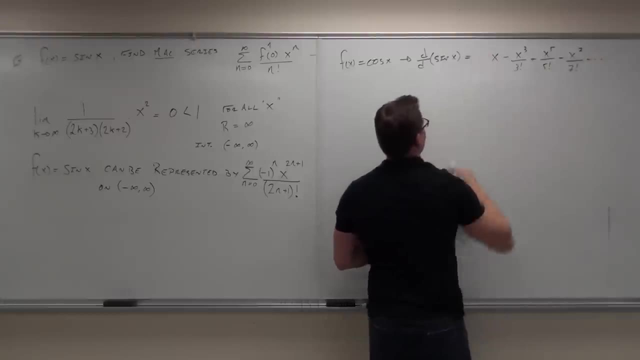 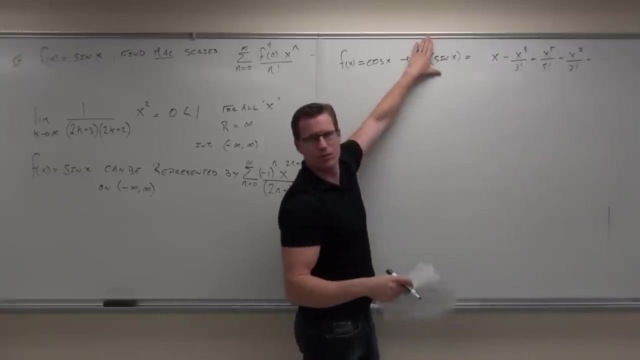 minus x to the third over three. factorial plus x to the fifth over five. factorial minus x to the seventh over seven. factorial plus blah, blah, blah, blah. check it out. Do you agree that sine x can be represented by this on any interval? 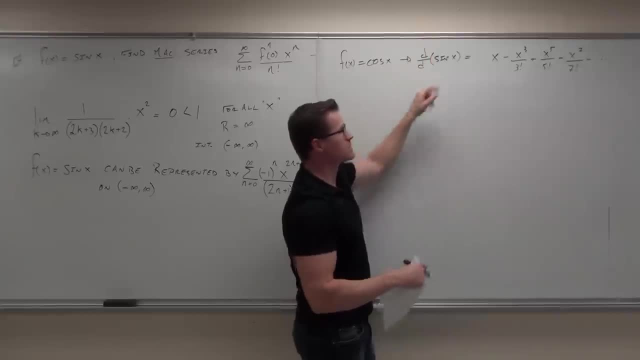 We just proved it. We just showed it. Then, if I take a derivative of sine and I take a derivative of all this crap, what I get, hey, what's the derivative of sine? I'm sorry, what's the derivative of sine? 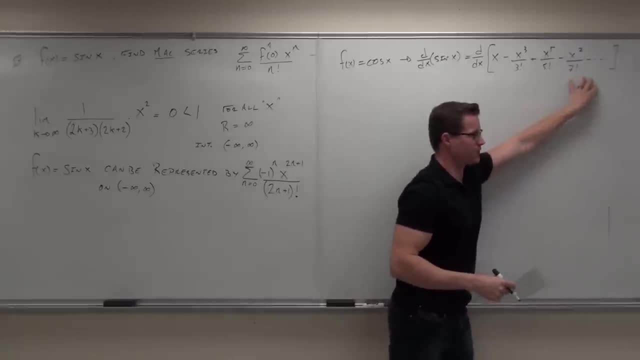 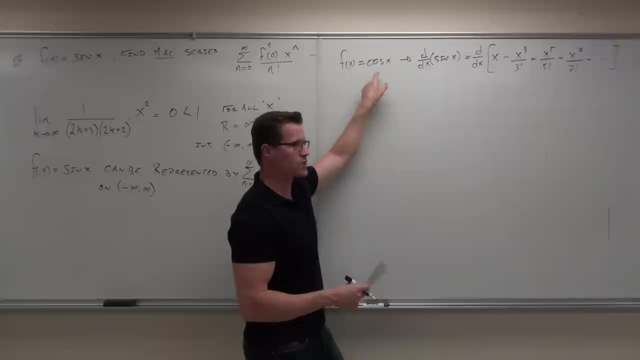 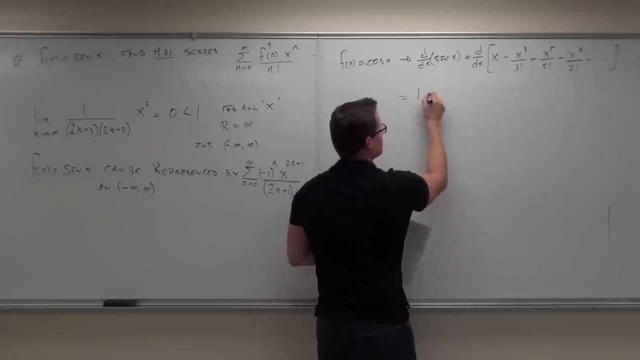 Cosine. So if sine's represented by this stuff, if I take a derivative of sine and I take a derivative of this stuff, the derivative of sine is cosine. Cosine can be represented by the derivative of this stuff, which means one minus x to. 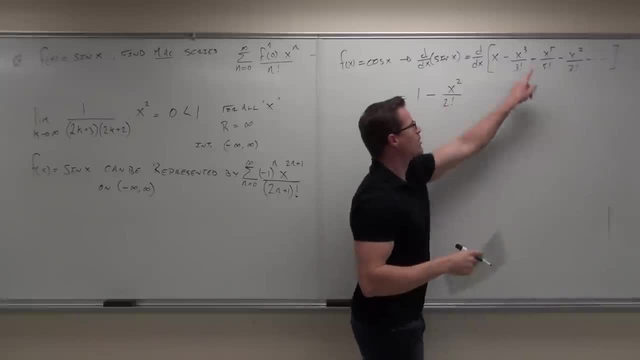 the second over two factorial. look what will happen: Bring down the three- The three's going to cross out with this three- and give me two factorial One minus x to the fourth over four factorial minus x to the sixth over six factorial plus. 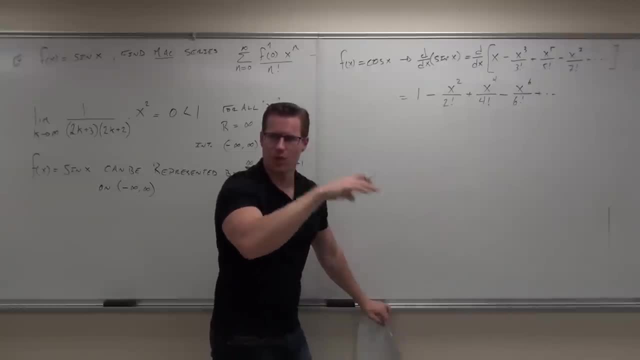 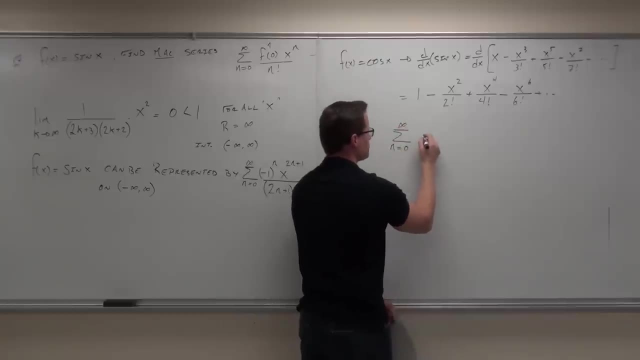 Do you see what happens? It just lowers everything by one power, and one factorial Specifically. we get a Maclaurin series. It's still alternating. It's still alternating. It's still x to a power, but it's only even powers. 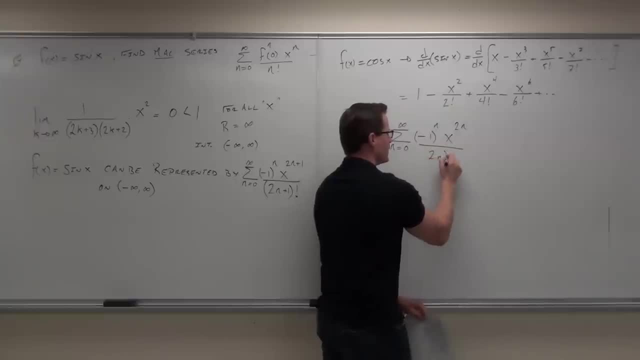 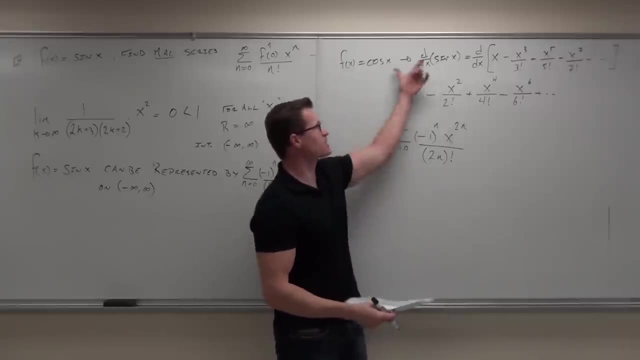 You don't get the plus one Over x to the fourth over four factorial. Minus x to the sixth over six factorial, Minus x to the sixth over zero and minus x and negative two n factorial. Do you guys get that? So we didn't have to do any work for it. we took a derivative of sine. derivative of sine. 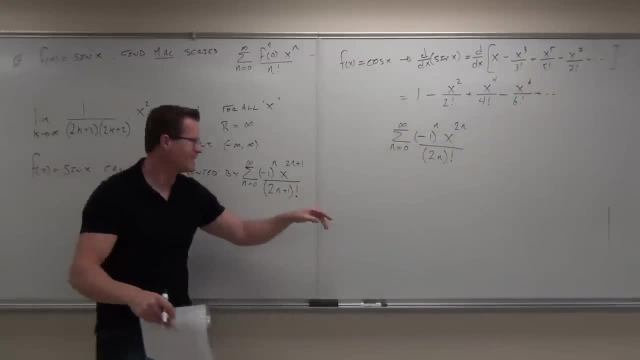 is cosine, no problem. Take a derivative of a term by term. basically, look at this. This is really cool, Check this out. Could you have done it right from here? Take a derivative. This goes here: cross it out with two n minus plus one, you get two n. 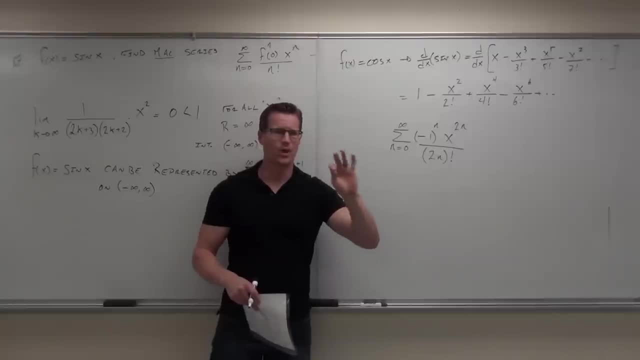 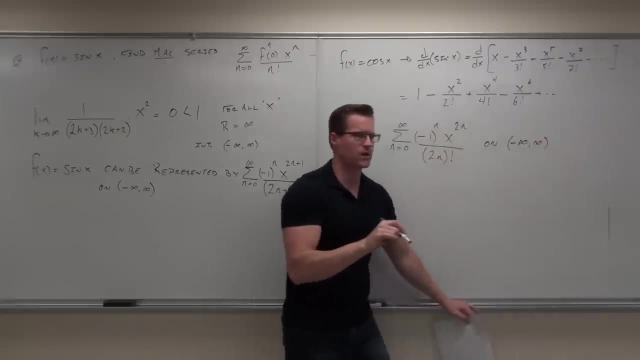 Subtract one from x minus x, we get this Last little bit. what's the interval? ührenve Phil, Huawei, Delhi, I'm telling you that when you take derivatives and integrals, your interval of convergence does not change, only the end points. 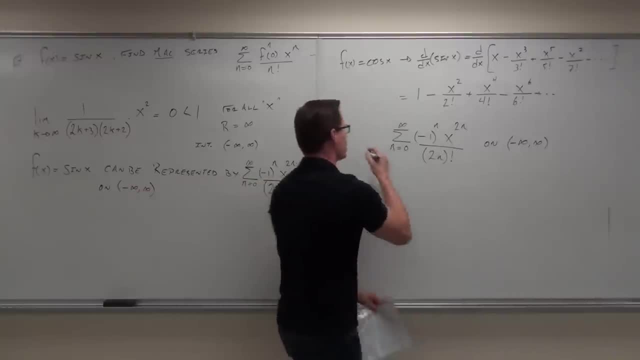 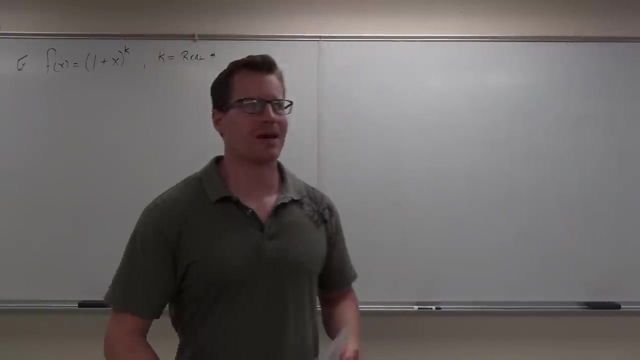 Since we don't have any end points, our interval is exactly the same. So cosine x can be represented by this thing on that interval. So if you guys feel okay with that one, okay, Okay. so getting to our last example, 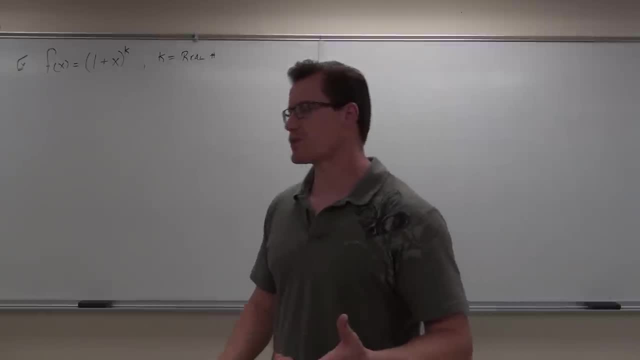 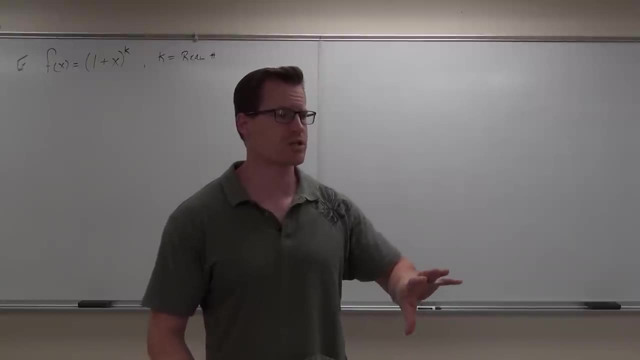 of how to do a Taylor or Maclaurin series from scratch. From scratch means that we invent our own series. After this, what we're gonna be doing is using known Taylor-Maclaurin series to fit our function to it. You see, that's a lot easier. 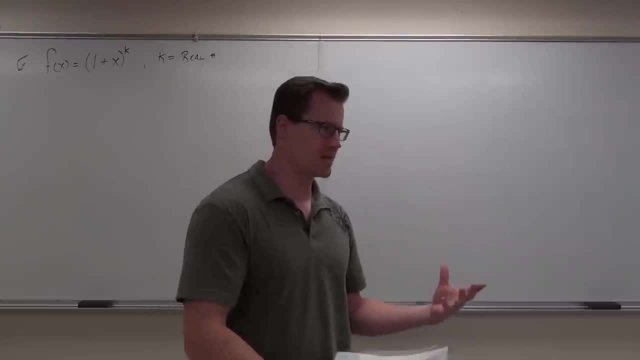 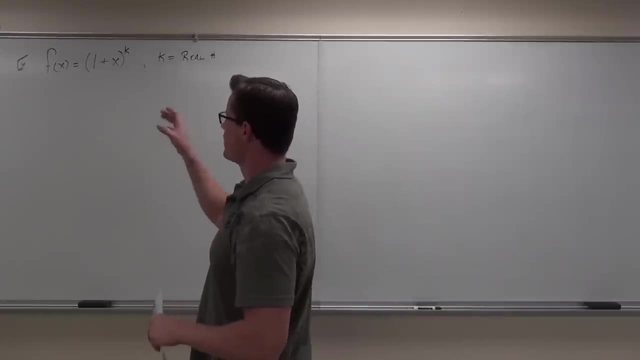 And so a lot of times we can manipulate what we have into what we've already made. Does that make sense to you? So this is the last thing we're actually gonna make, And what it is. it's a polynomial one plus x to some power. 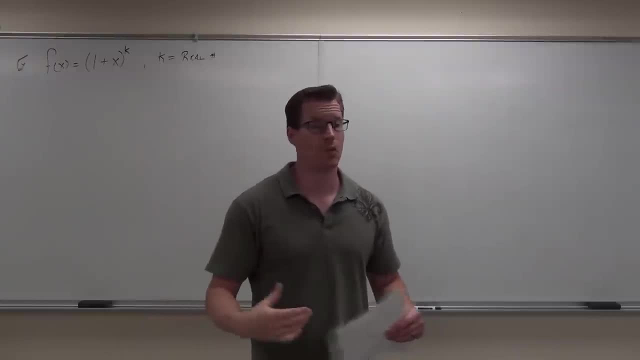 k, where k is a real number. So k could be like 1: 1⁄2, k could be negative, k could be positive, like two or three, in which we would get like a binomial expansion. That's actually what we're gonna get anyway. 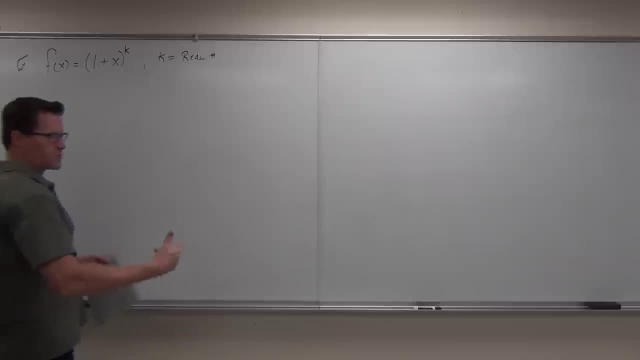 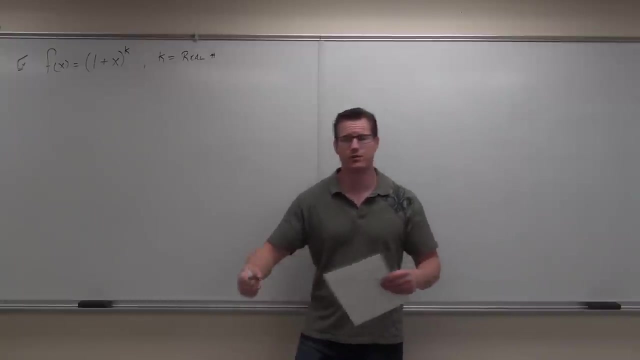 So I'll show that to you right now. So once we start, do you remember the first step? when we start any Taylor or Maclaurin series? What do we do? Do your derivative Good? so we're gonna find a series of derivatives here. 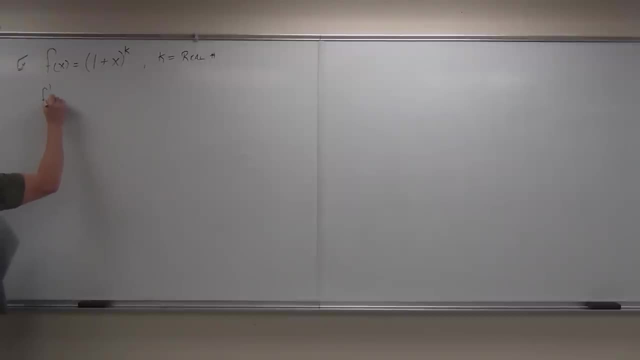 We always start with the function of self, f, of x, and we find our first derivative. First derivative is gonna be well, if you notice this, it's gonna be the chain rule, over and over, and over and over again. So practically we bring down the k. 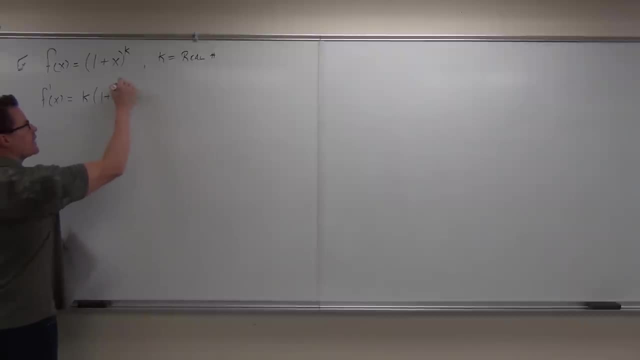 we get one plus x, the chain rule gives us one, and then we get k minus one. Very good, that's right, And we keep on going. The second derivative would give us k times k minus one, times one plus x to the k minus two. 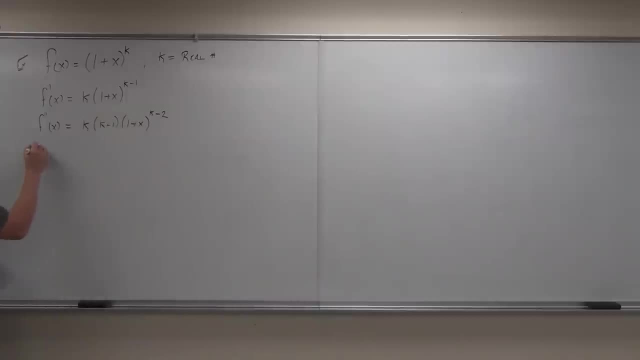 Are you hanging on with me here, Mm-hmm? The third derivative would give us k, and then it would give us k minus one, and then it would give us k minus two, and then it would be one plus x, and then it would be k minus three. 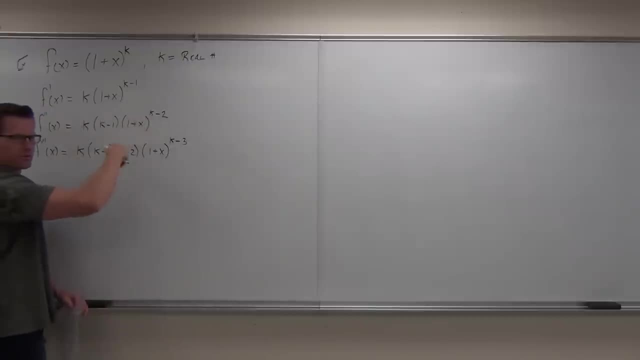 You still okay? Yeah, We're just doing a general power rule or a chain rule, whatever you want to call that. We'll do one more. A fourth derivative would be: tell me One plus x to the k minus two, then one plus x to the k minus three. 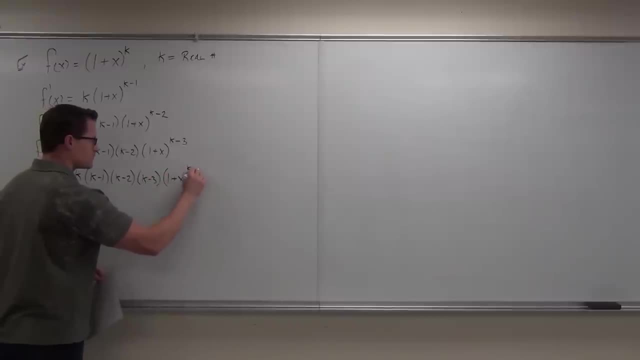 One plus x to the k minus three. Very good, One plus x to the k minus three. Now we want to make the jump. How about the nth derivative of f? The nth derivative? Let's look at this for a second. 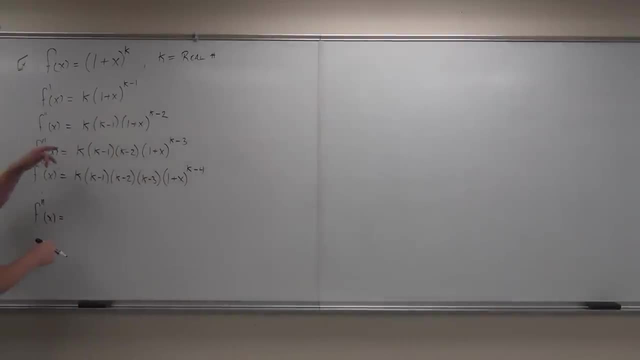 Think about what's going on. What's going on is that I'm multiplying, but it's not quite k factorial. What's happened is: I'm doing k, then I'm doing k minus one, I'm doing k minus two, I'm doing k minus three. 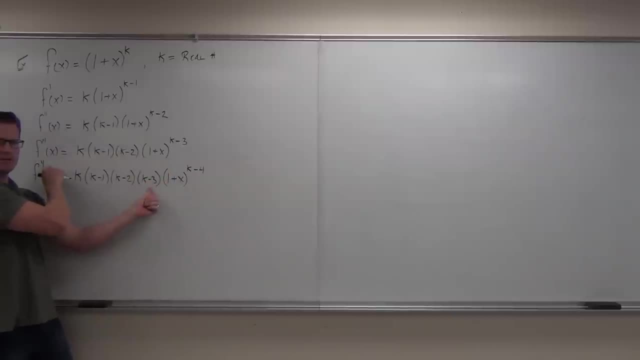 but I don't get to the k minus n. Do you see it? I get to the k minus n plus one, The k minus one more before that n. Does that make sense to you? Okay, Also, I'm doing my k. 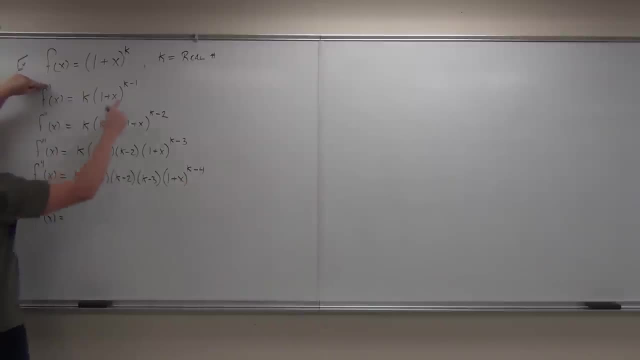 well, this is to the k minus n, so let's check it out. First derivative minus one. Second derivative minus two. Third derivative minus three. Fourth derivative minus four. Nth derivative: k minus. let's wrap it up. 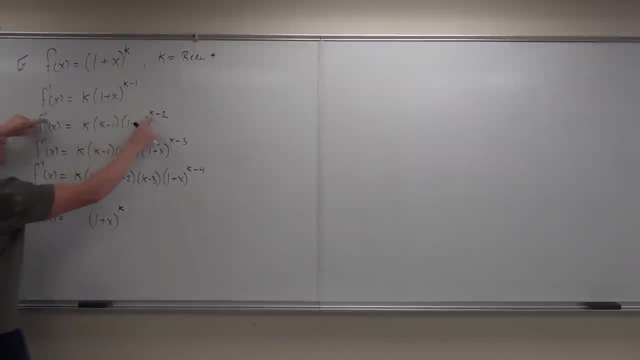 First derivative k minus one. Second derivative k minus two. Third derivative k minus three. Fourth derivative k minus four. Nth derivative k minus perfect. That's exactly right. Now, all this stuff. I gotta rewrite this. I don't have any more room. 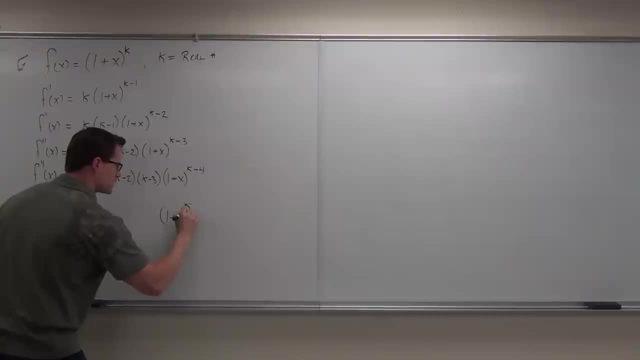 So nth derivative one plus x to the. you just said it k minus n. Are you guys all right with that one? Yeah, Now here, we'd have k. we'd have k minus one, we'd have k minus one. 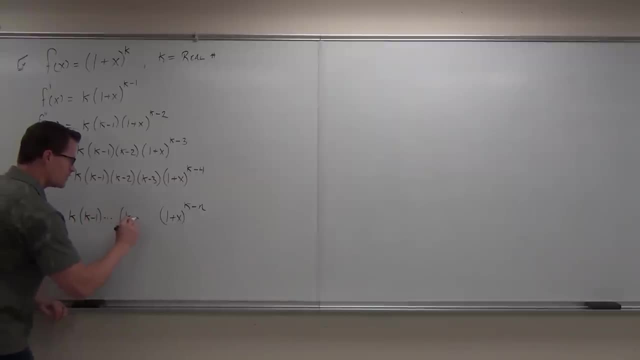 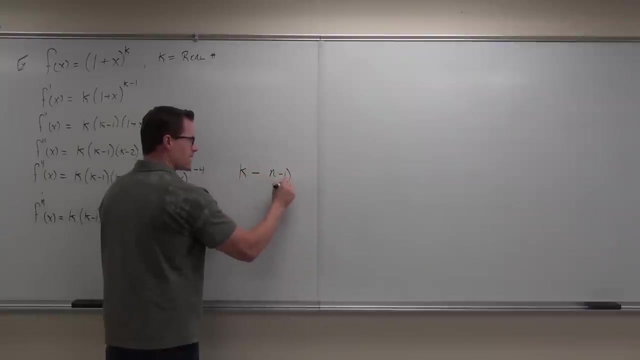 we'd have all the way down to k minus. what's this number in relation to my n? One minus one. Like one less N minus one. It is n minus one. that's right. but check this out. We'd have k minus n minus one. 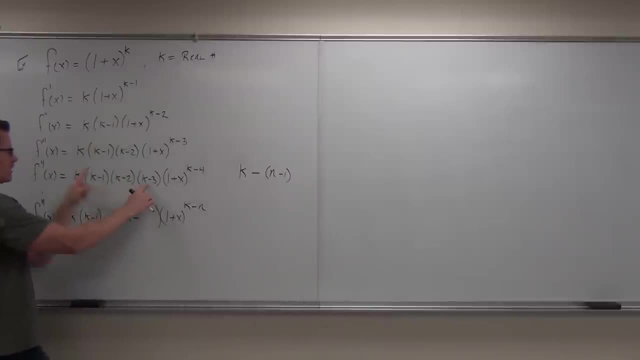 Do you guys see what I'm talking about here? This would be k minus oh n minus one K minus oh. three minus one Oh k minus two minus one K. well, where'd I go? K minus one minus one, just k. 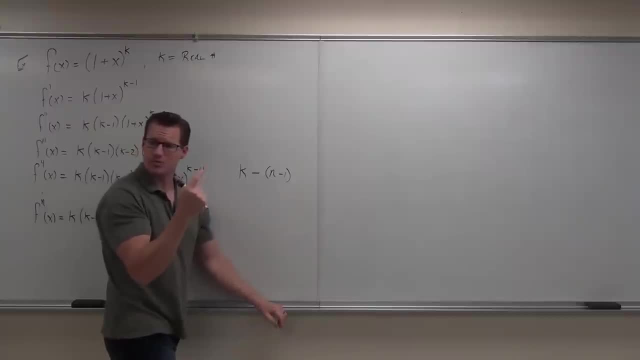 So if I had k minus n minus one, the n minus one's gotta be in parentheses. do you understand what I'm talking about? Yeah, Well, if I am to distribute this and make it a little nicer, this is k minus n plus one. 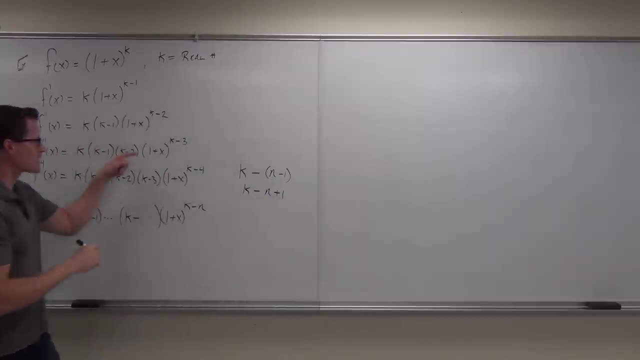 K minus n plus one. let's see if it works. We got our k, sure we got our k. Let's see how this works. Is this k minus two plus one? K plus one? Yeah, yeah, Minus two would be well negative two. 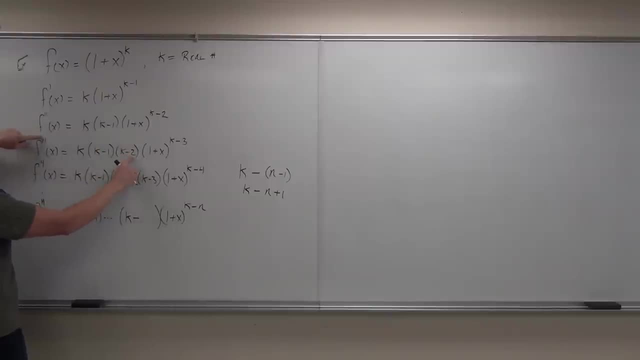 then plus one gives us minus one. Here would be three: Three minus two plus one got it, And then we'd have minus four plus one, that's three. I think I said that one backwards. I said minus three and then plus one, that's minus two. 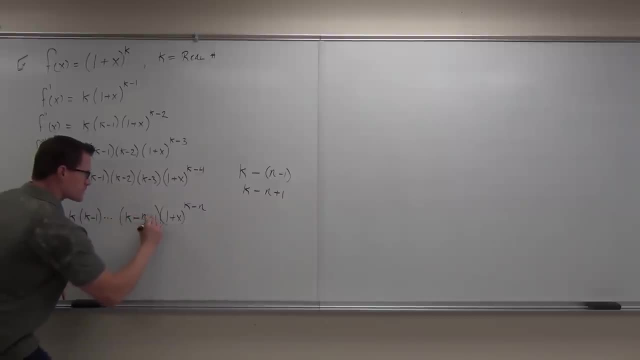 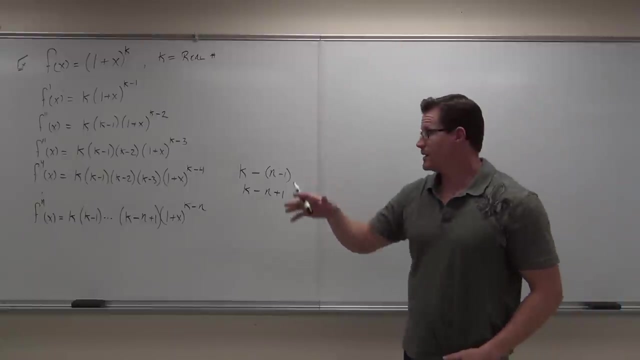 Minus four plus one, that's three Minus n plus one, and that's where we would stop. It should make us feel okay with that. so far. Now we actually have a pattern for our nth derivative of f, which means that if I want to find 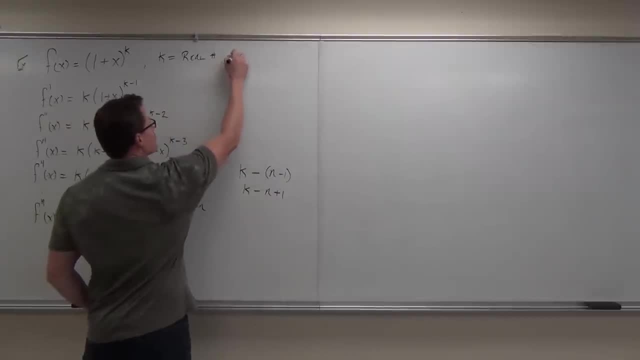 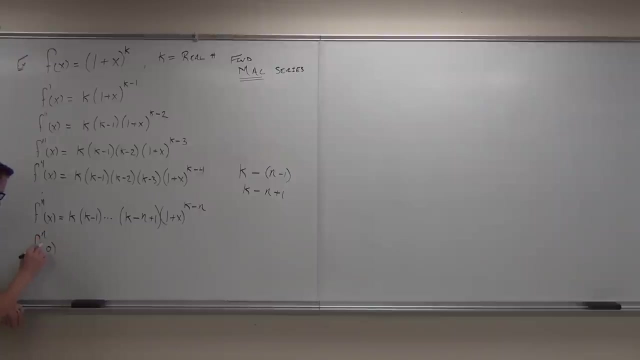 what I want to do here is find the Maclaurin series. So if I want to find the Maclaurin series, what I want is the nth derivative of f at zero. What I want is the nth derivative of f at zero. 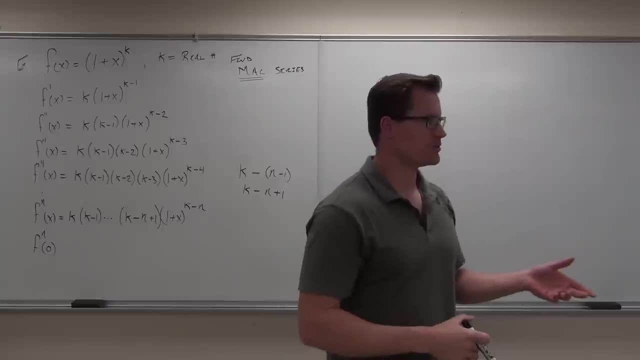 What I want is the nth derivative of f at zero. The Maclaurin series says it's centered at zero. You with me on this one? Well, let's do that. What number am I going to plug in and where am I going to plug it in? 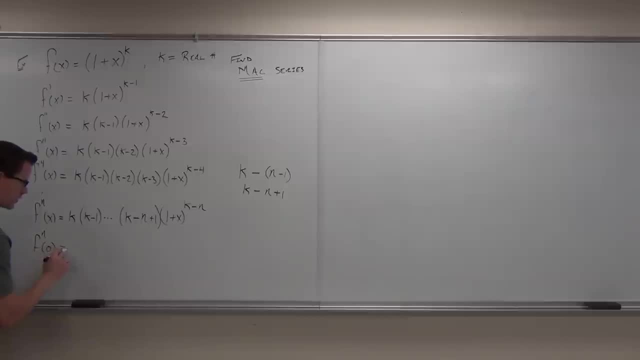 Zero for x. So that's what it says right here. So if I plug in zero for x, what's one plus zero One, One to any power One. So this whole thing is going to become one. Essentially, I'm just going to get this piece back again. 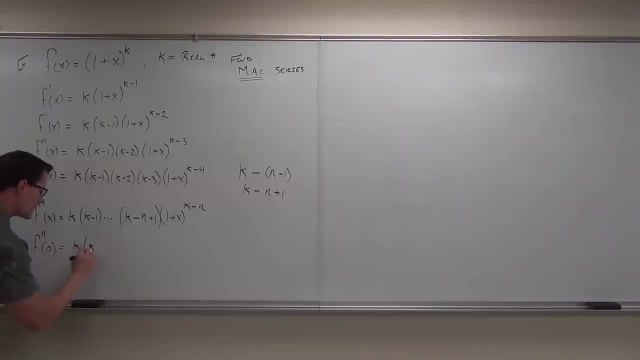 Do you see it? Yeah, So k, and then k minus one, and then all the way down to k minus n plus one. So k minus n plus one. So k minus n plus one. Okay, show of hands if you're okay with that so far. 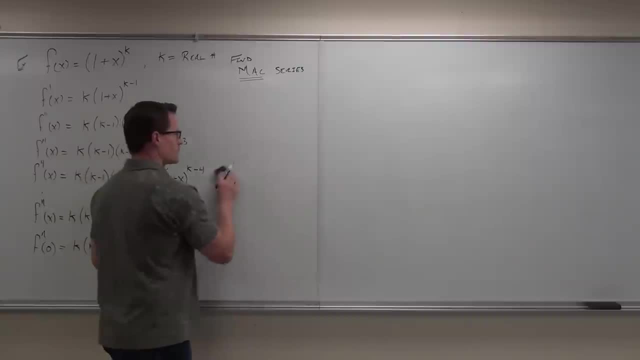 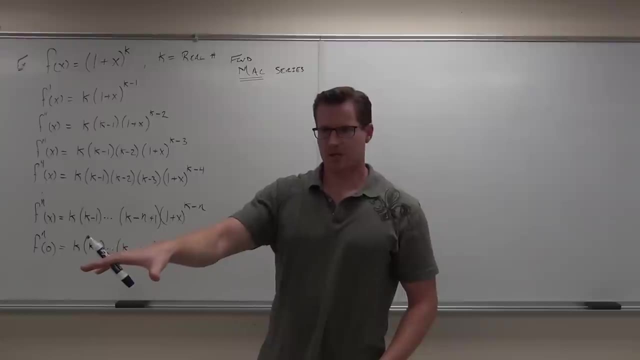 Okay, show of hands if you're okay with that so far. Okay show of hands if you're okay with that. so far. You guys over here, are we? yes, no, All right. so if we're looking for the Maclaurin series, 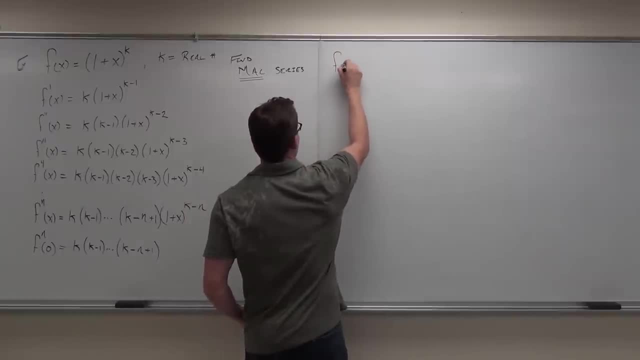 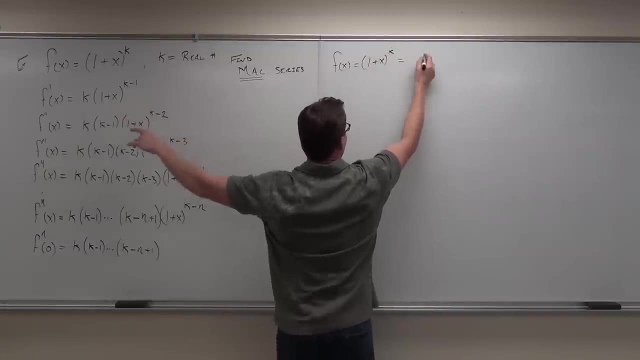 here's what we're saying. We're saying the Maclaurin series should represent a function f of x. in this case, one plus x to the k by doing this. in this case, one plus x to the k. by doing this. 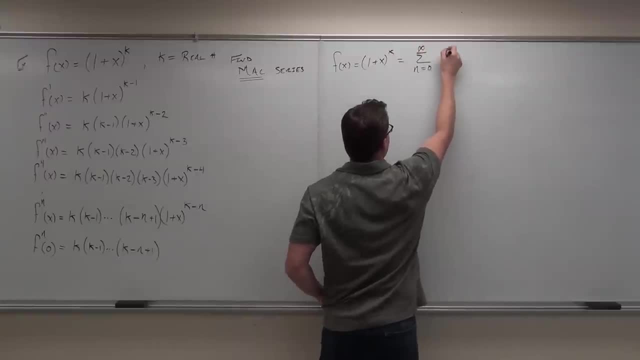 It should be a series that starts at zero and ends at infinity. It should be the nth derivative at zero. It should be over n factorial times, x to the nth. If that's a Maclaurin series, Does that look familiar to you? 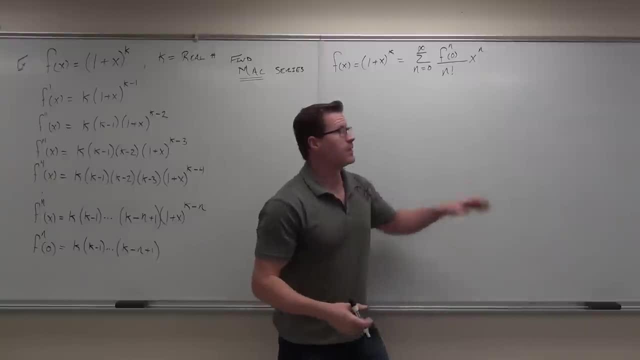 Yeah, That's our Maclaurin series. All right, cool. Well, hey, you know what This part is going to be there, no matter what, It's centered at zero. yeah, That's why we have Maclaurin series. 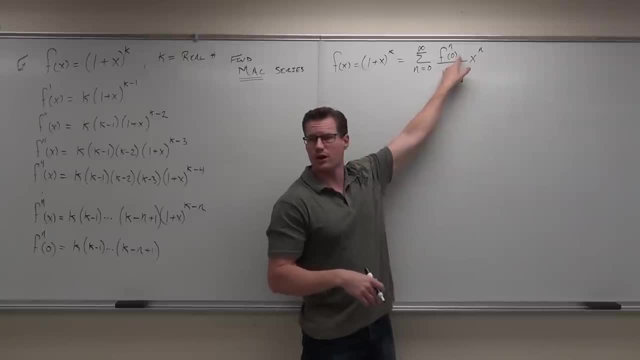 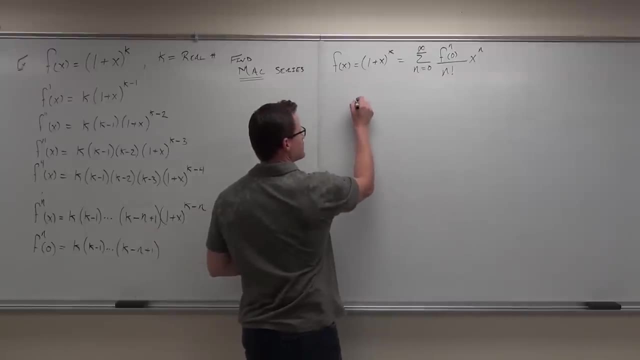 This is over n, factorial, not a problem, This one. do we know our expression for the nth derivative of f at zero? Yes, you do, In fact, we just found it, It's right there. So now we say, OK, this series is: n equals zero to infinity. 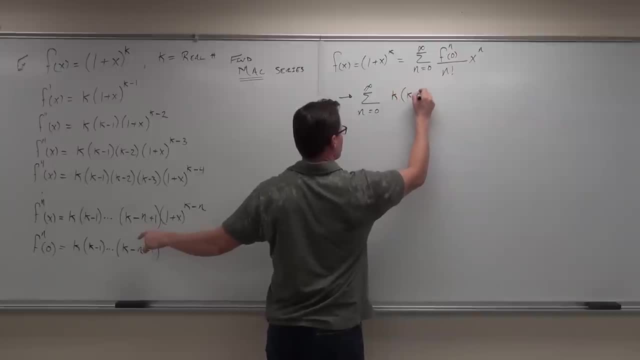 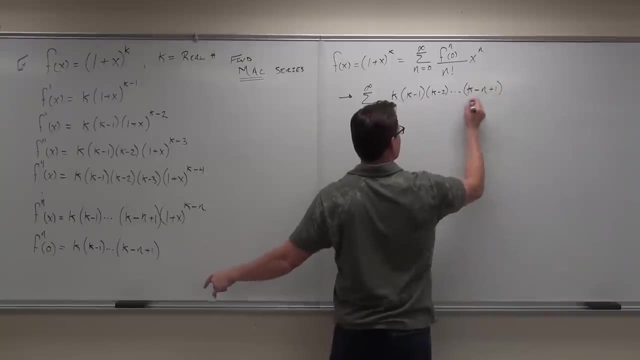 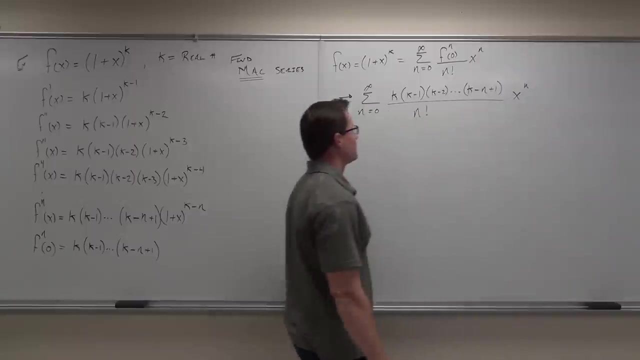 We've got, oh my gosh, k, k minus 1, k minus 2,, all the way down to k minus n plus 1, all over n factorial times, x to the nth. Goodness gracious me, that's a lot of stuff. 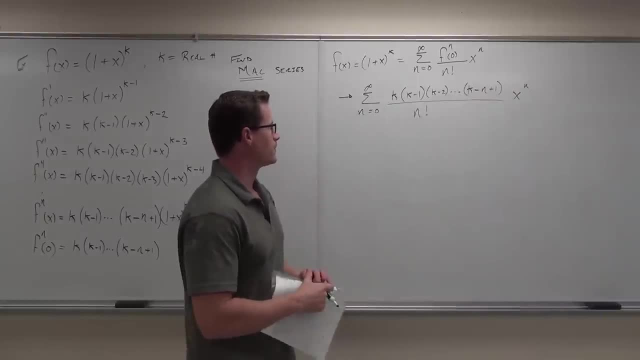 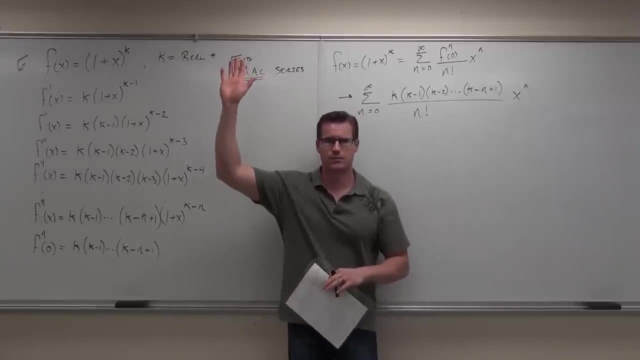 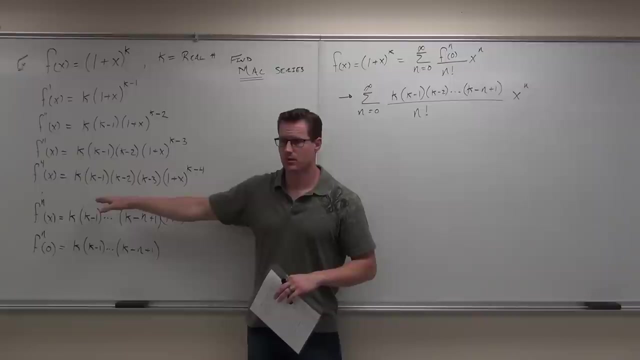 OK. what I want to know is: by a show of hands, do you feel OK getting that far? Do you? Do you see where it's coming from? Do you see where all our derivatives are coming from? Yes, no, Why we stop at n minus, sorry, k minus n plus 1.. 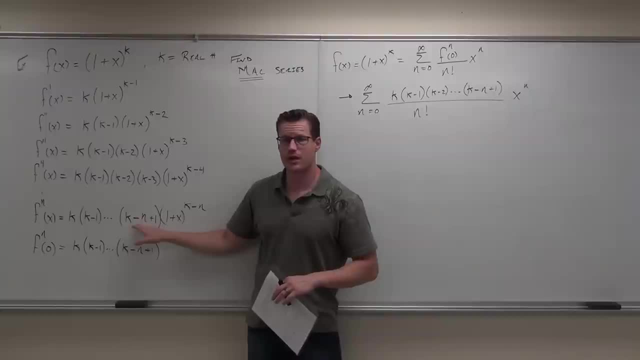 Do you see where that's coming from? All right, well, if we plug in zero for x, which is our center, it's a Maclaurin series. it says c equals zero. No problem, Sure, Let's plug that in. 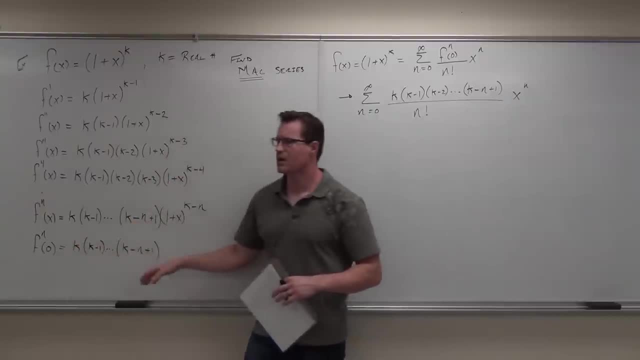 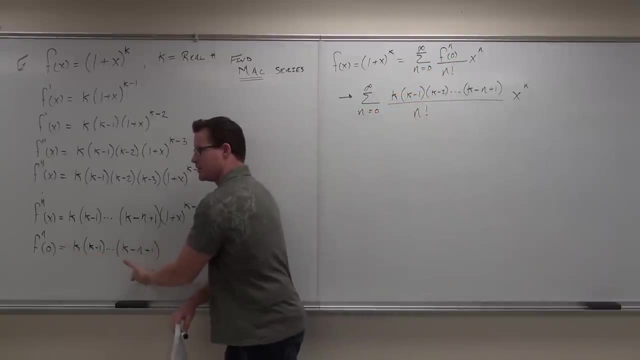 So at zero, we get this thing's gone, We get just this piece. By definition, a Maclaurin series is the nth derivative of f. at zero, Hey, that's right here. Times x to the nth. OK, that's right here. all over n factorial. 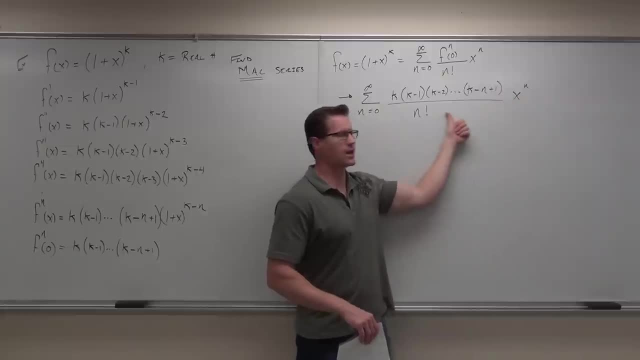 So we have the nth derivative of f at zero. We've got x to the nth, we've got n- factorial. Hopefully it's clear for you. it's just a Maclaurin series. You guys are with me on it. Now let's do the first few terms of this to see what it really looks like. 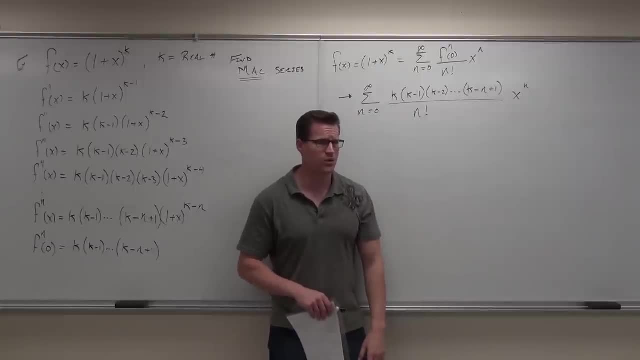 Because many of you are probably going: how in the world am I going to do that series? What in the world does that look like? Here's what it looks like. This series looks like this. So really, you could represent one plus x to the k by doing these terms: 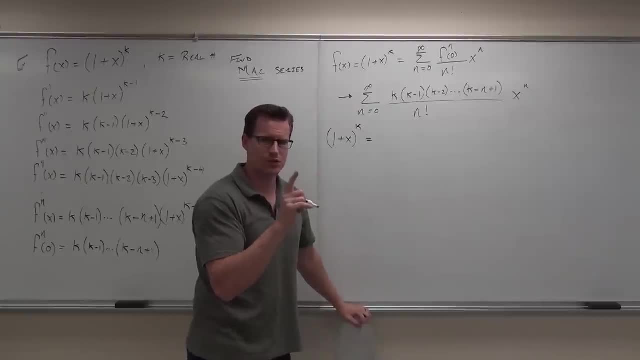 The first term is going to be one. The first term is going to be one because remember what the Maclaurin series represents. Are you listening? The Maclaurin series represents f of zero. first F of zero says I just plug in zero. 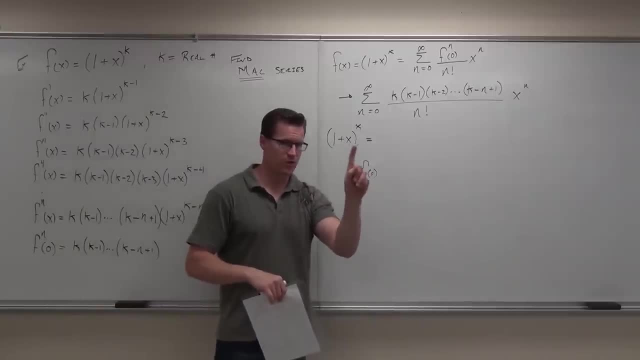 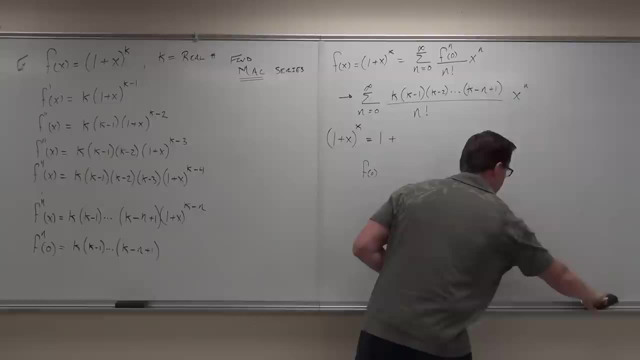 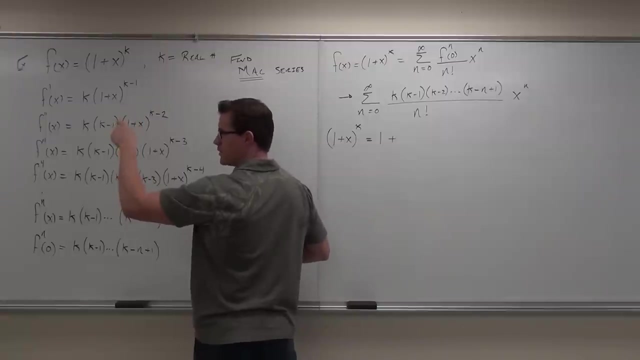 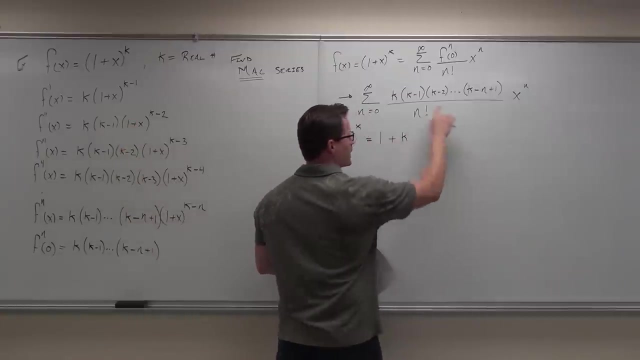 I would get one. One plus zero is one Too many. power gives you one. That would be my first term. Then I would get the first derivative at zero. The first derivative at zero would give me k, But then I'd have my x from my power series. 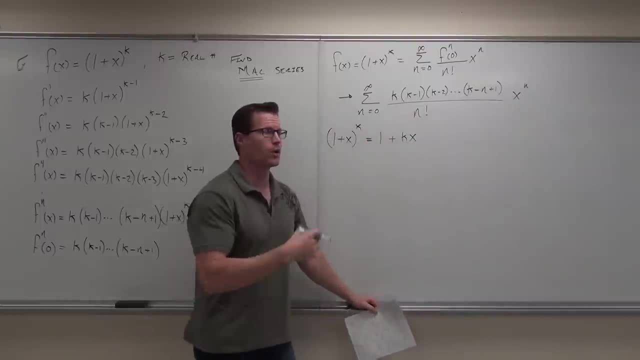 I'd get kx All over one factorial because it would be my first term. Are you guys alright with that so far? So this, practically speaking, just represents these guys right here. Then we multiply by x to whatever our n is and divide by n- factorial. 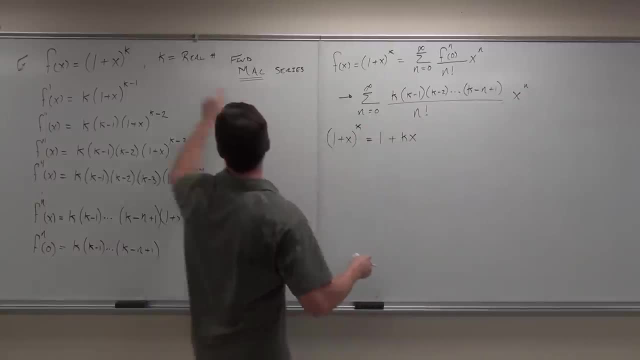 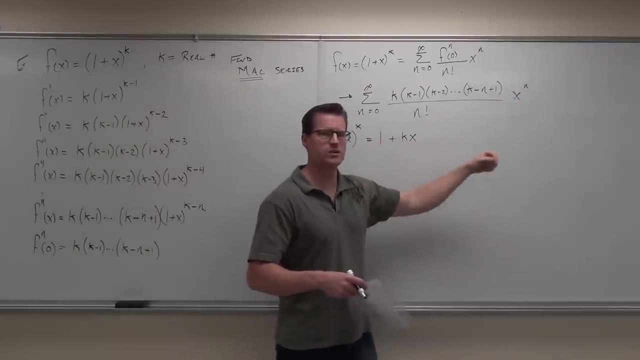 So here we go. Okay, At zero term, I'd get f of zero, that's one times x to the zeroth power, That's one. Divided by zero factorial, that's one. So we get one. The next term says: okay, cool. 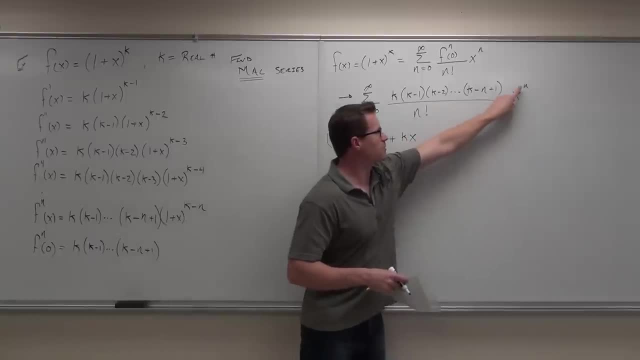 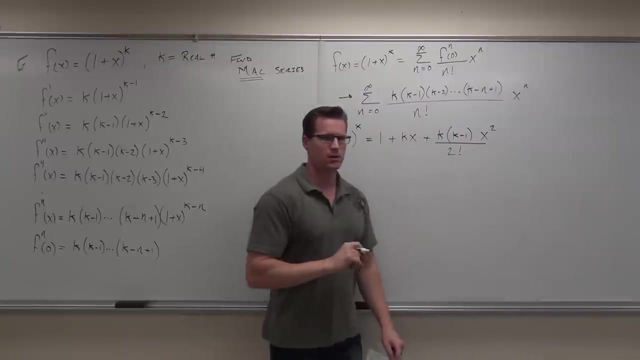 Well, we get k times x to the zero, X to the first over one factorial, that's kx. Then we would get k times k minus one times x to the second, all over two factorial. Are you starting to see the pattern at work now? 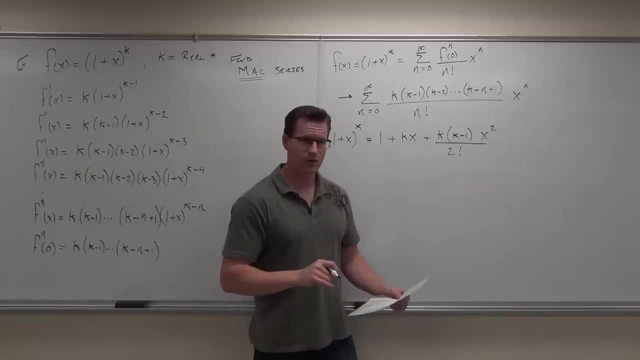 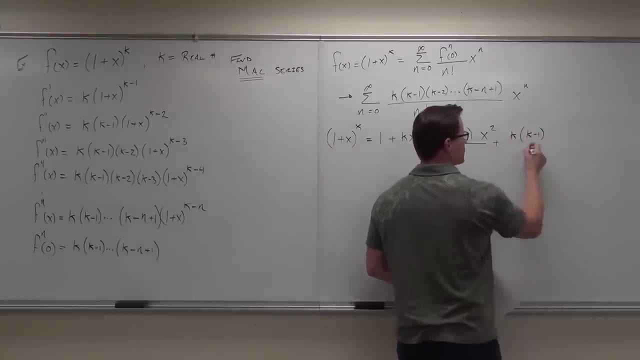 Yes, No, You sure, Mm-hmm. Okay, Then we keep going. We get k. We get k minus one. What's the next term? k minus two. What's the next term k minus two. Actually, the factors would be. 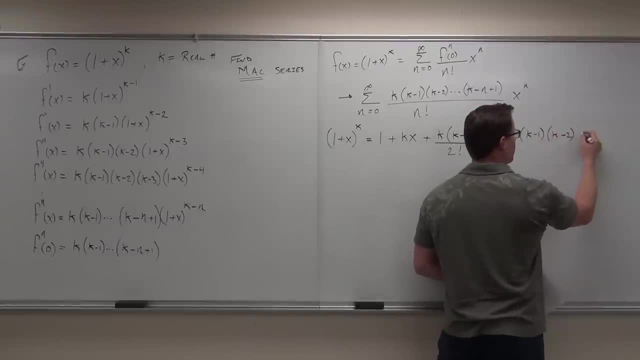 And then what? x to the third, x to the third, all over, Perfect. That's what this thing looks like. You go, okay. cool, It starts at one, because the Maclaurin series says you start at the function evaluated at. 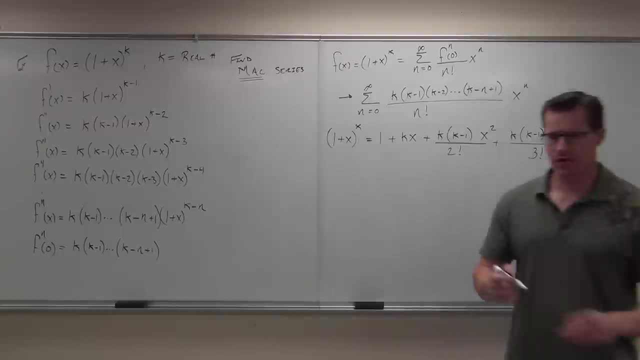 your center. Are you listening? Mm-hmm? You start at your function evaluated at your center In a Maclaurin series. that center is zero, So you start at f of zero. That would be one, two, I don't care what it is. One, two. Any power is wrong. One, two, three, four, five, six, seven, eight, nine, 10,, 11,, 12,, 13,, 12,, 13,, 14,, 15,. 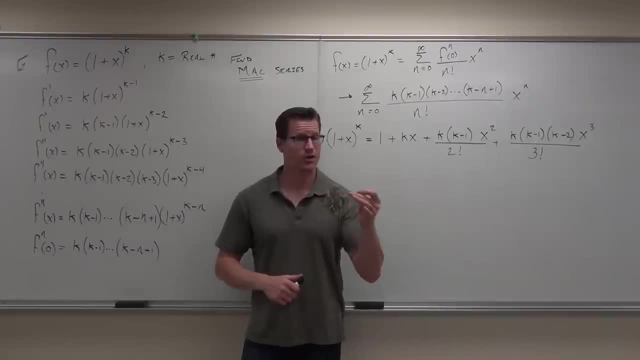 16,, 17,, 18,, 19,, 20,, 21,, 22,, 23,, 24, 25.. You start at one And multiply it by x to the zeroth over zero. factorial, That would be one over one. 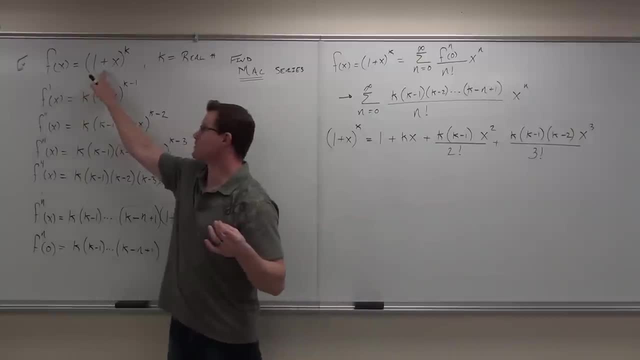 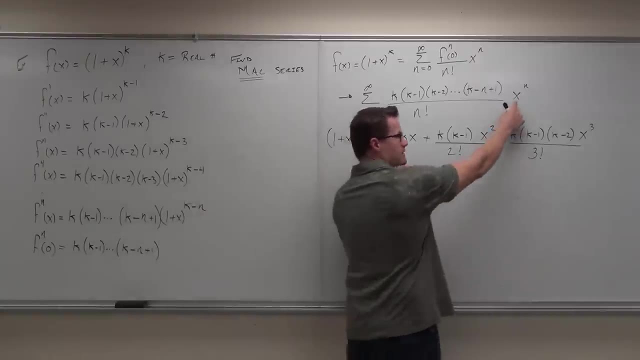 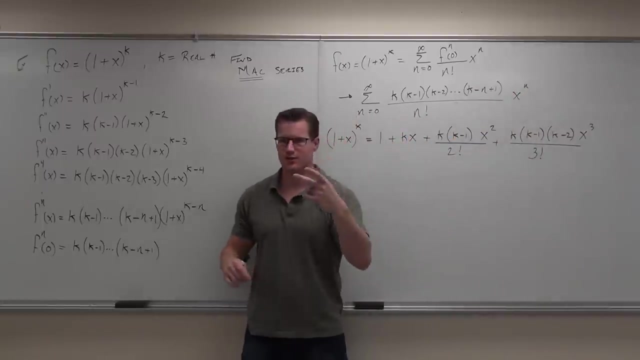 That's giving you one. Then you do the first derivative evaluated at your center. The first derivative Evaluate your center is one times k, So it's k. Now, that is the best you can do. All right, That's what this is. 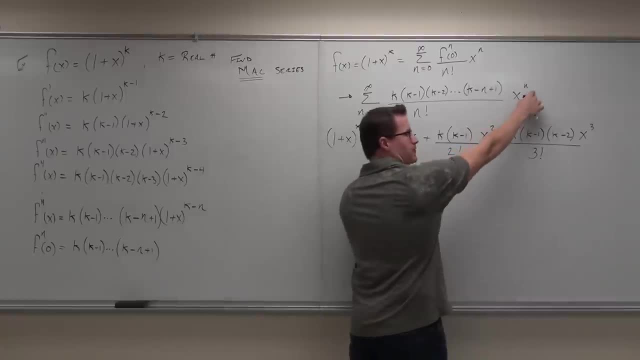 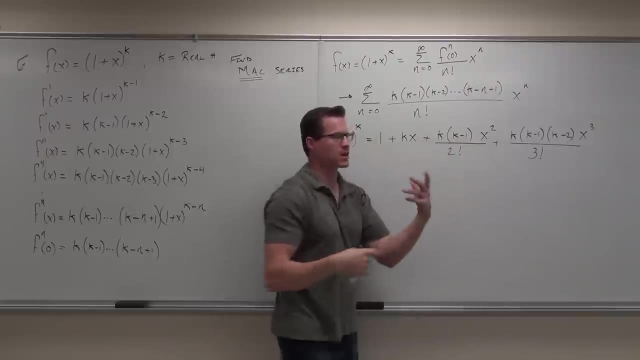 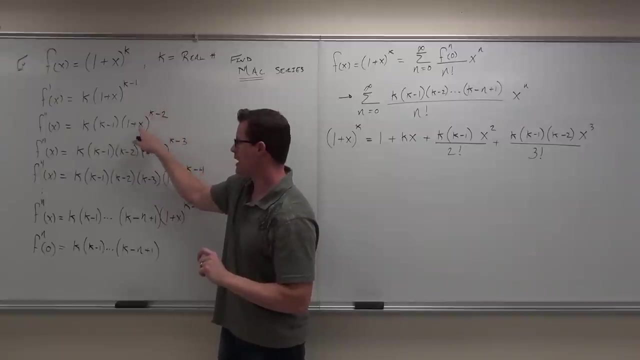 That's what you do. times x to the first, all over one factorial, That just gives you k times x. does that make sense? Then you do your second derivative: evaluate it at your center. x equals zero. Okay, well, that's one times k. 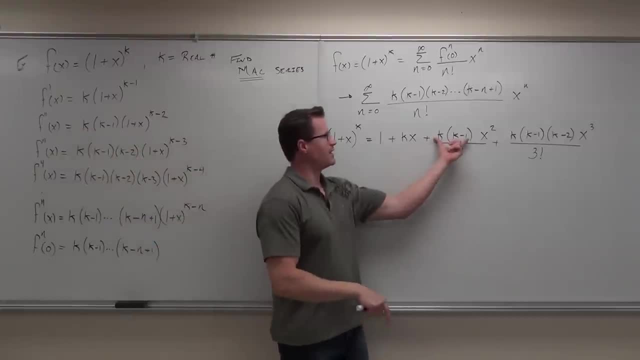 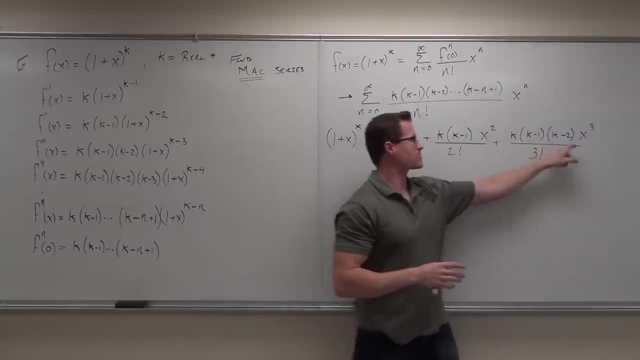 okay, so we have k times k minus one. hey times x to the second over two factorial. that's where these things are coming from. that's where they're coming from. The next one would be k times k minus one times k minus two times k minus three. 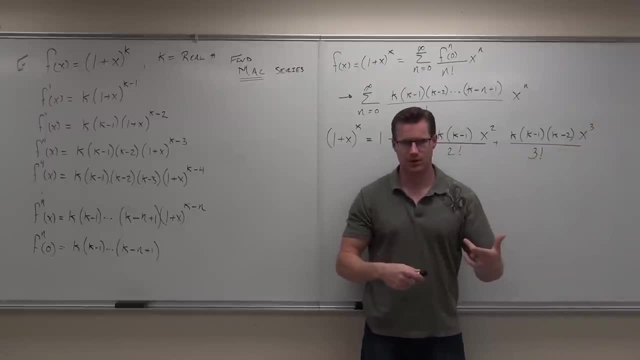 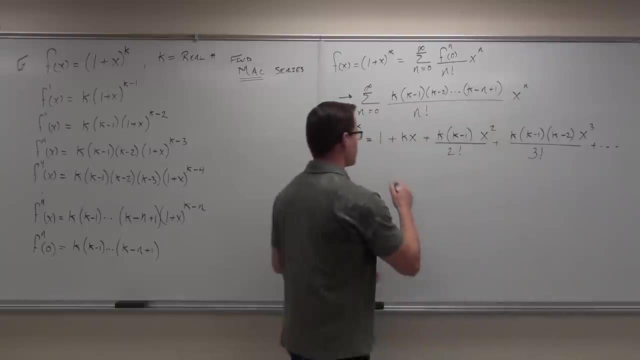 x to the fourth, over four, factorial, and you'd continue forever. Does that make sense to you? What this is called is the binomial series. Binomial, two terms being expanded. So this is the binomial series, And we can make this series look a little bit different. 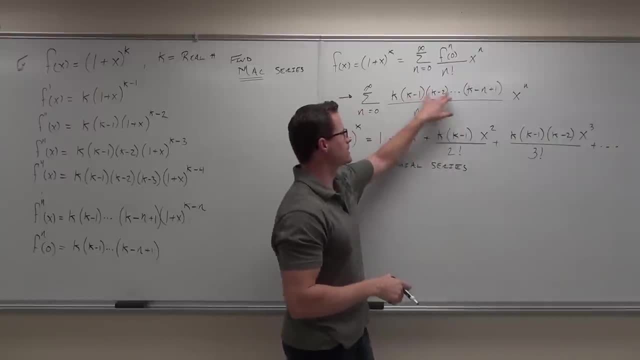 What this actually gives you here. these things give you the binomial coefficients. Do you know what the binomial coefficients are? Have you ever heard of Pascal's triangle? If you took me back to this one, you have heard of that. Pascal's triangle goes one, one, one. 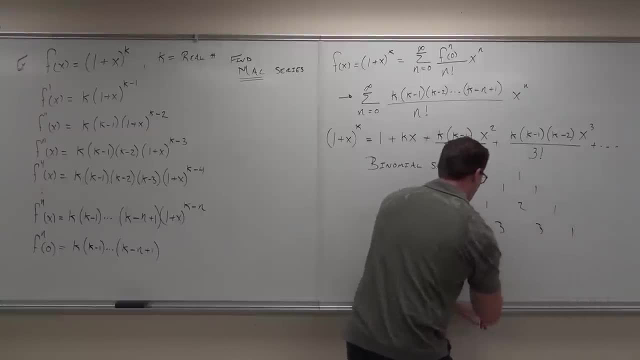 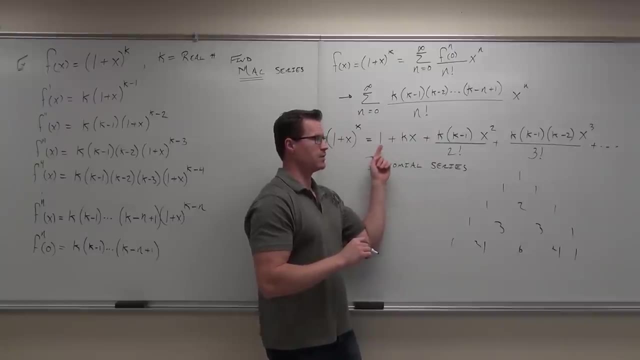 one, two, one one three, three. one one four, six, four, one. have you ever seen that before? Yes, That's what these numbers are. one And then well, whatever k you have, it would depend on that. 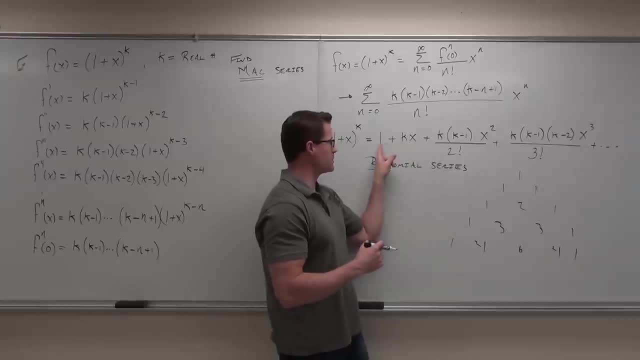 But that's what the binomial coefficients are. So this thing- this gives you this one k, this gives you the binomial coefficients for whatever k you actually have- Isn't that kind of interesting. It's gonna give you a line of Pascal's triangle. 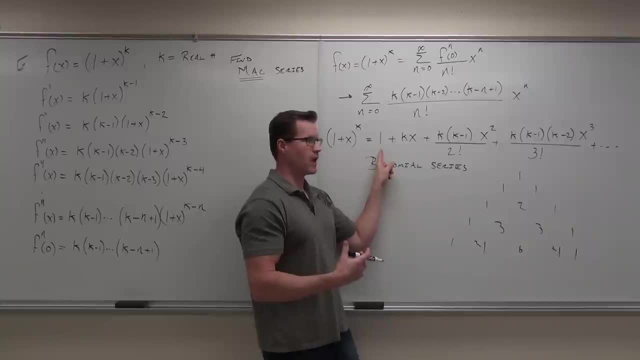 What does Pascal's triangle always start with One, And then it depends. It's gonna either do, well, one, two and then one, three, one, oh, look at that. Whatever your power would be, That's weird. that's kind of cool. 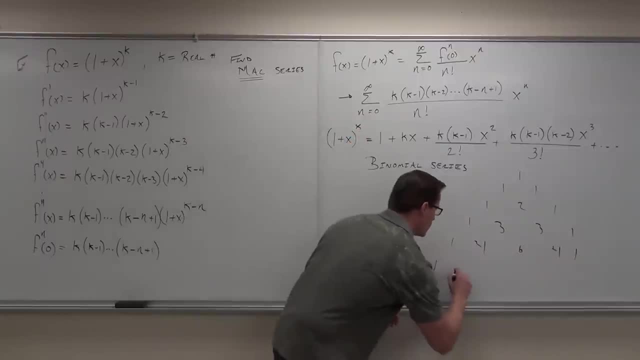 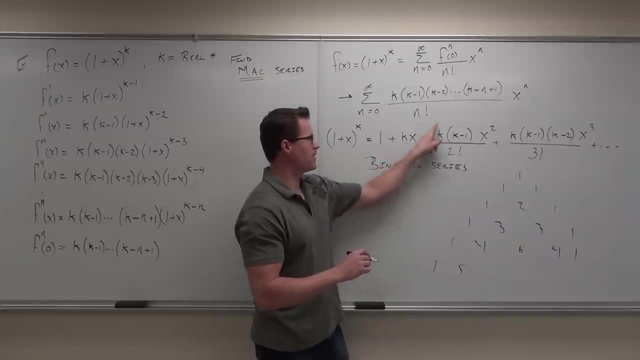 So if you have a power of the fifth, I'd be down here. One five, It'd be one five, 10, 10, five, one. That's interesting. So this would be one five. this would give me 10,. 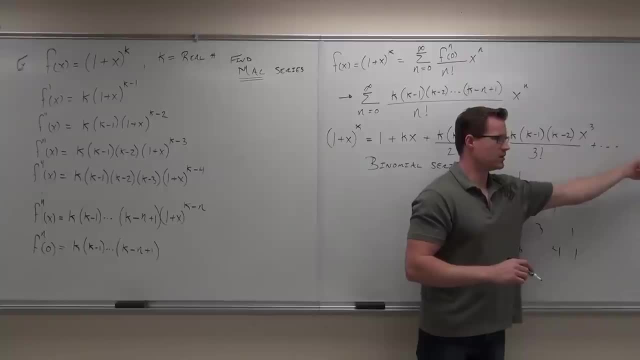 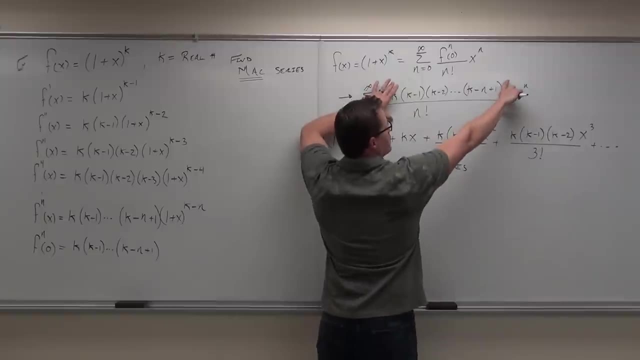 this would give me 10, five and then one. That would be my binomial coefficients. So the way that we write that, actually, since these only represent your binomial coefficients, we can write it this way: This series is represented by. 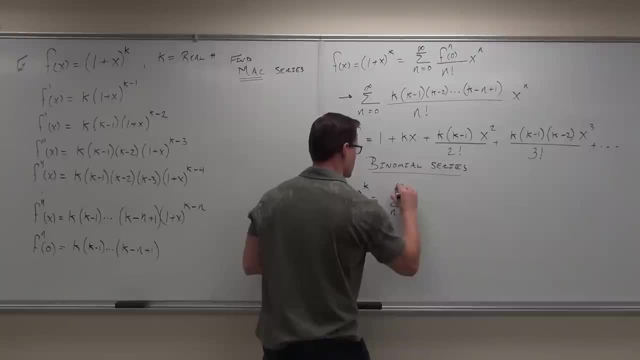 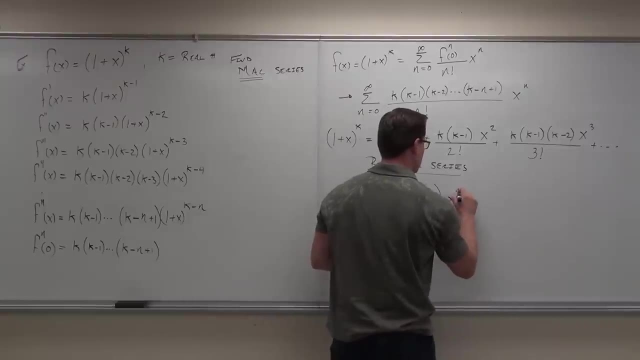 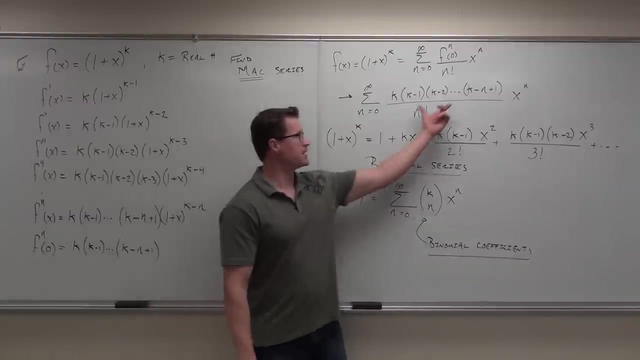 k? n. this stands for binomial coefficients, Like that. So what I want you guys to know about this thing is that this idea, this whole thing, from here to here, all they give you are the terms of Pascal's triangle. Those are the binomial coefficients. 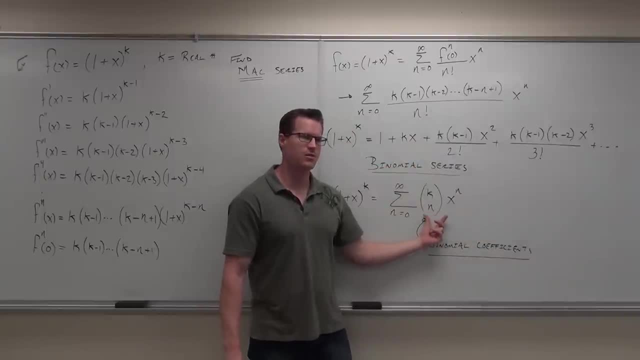 This is represented by that, just to make it look nicer. So if you've ever seen that before, that's what that is: Quick head nod. if you're okay with this so far, Would you like an example to see how this actually works? 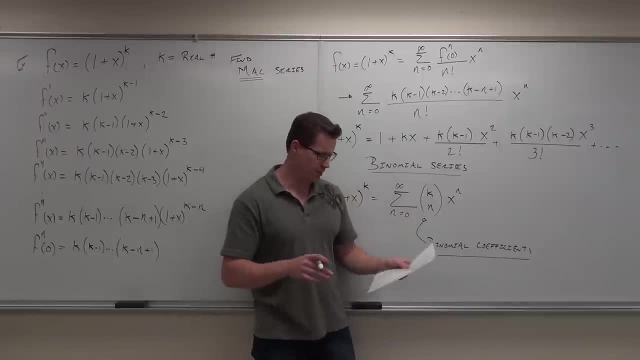 in practicality. Okay, before we do this, I want to give you a couple notes. Here's your notes. If k, do you have this written down, Because I'm gonna erase this for some room? So these are binomial coefficients. 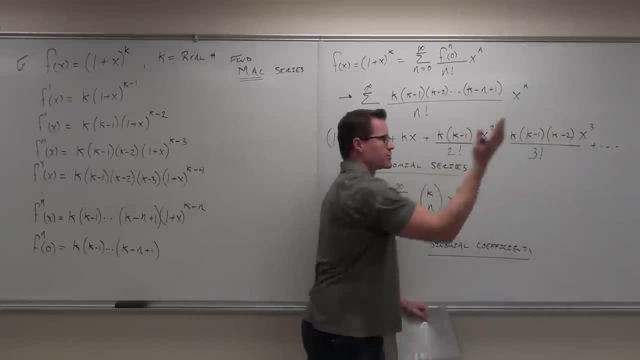 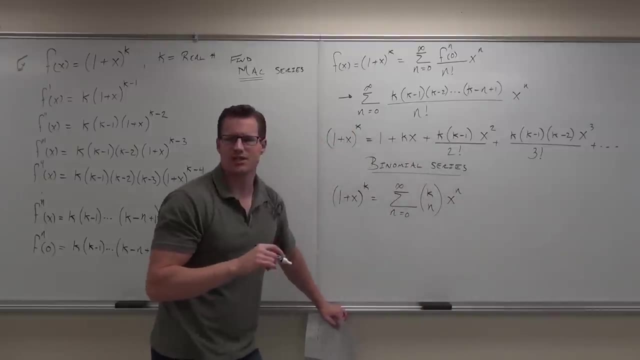 These are binomial coefficients. These are binomial coefficients. That's it If k is a positive integer. if give me an example of a positive integer, please. Four, Good, what else? Two, One and Ten, a hundred. 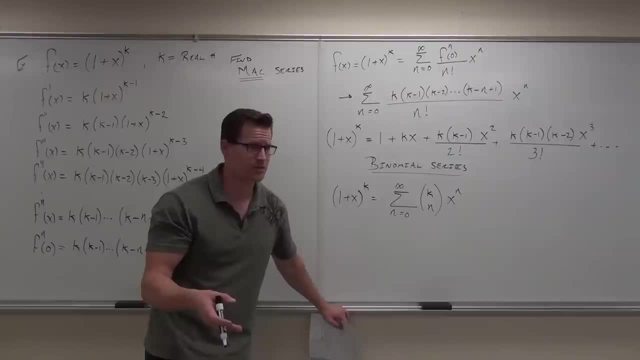 Not any positive number. no 1.3 is not a positive integer. Well, integers of what Positive whole numbers? Very good, A positive whole number is a well, whole numbers are inherently positive. So a positive integer are whole numbers. 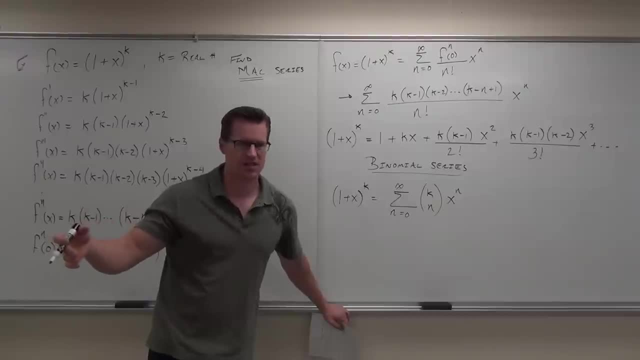 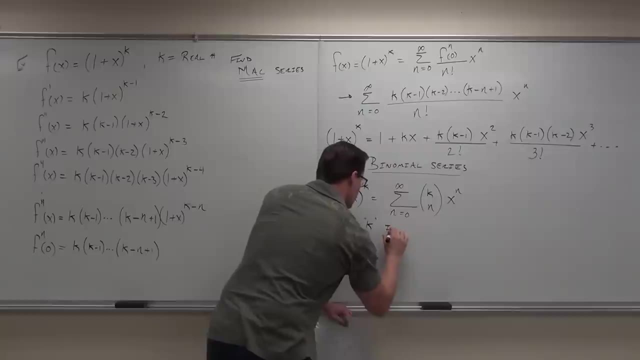 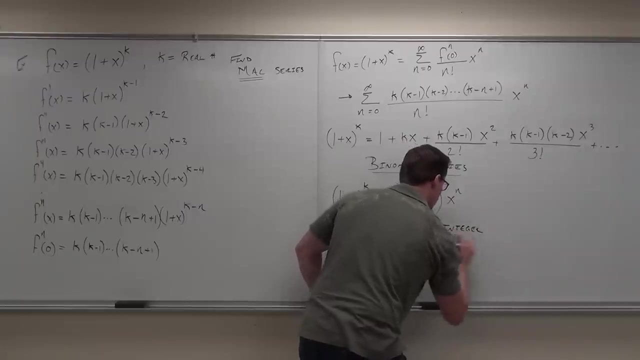 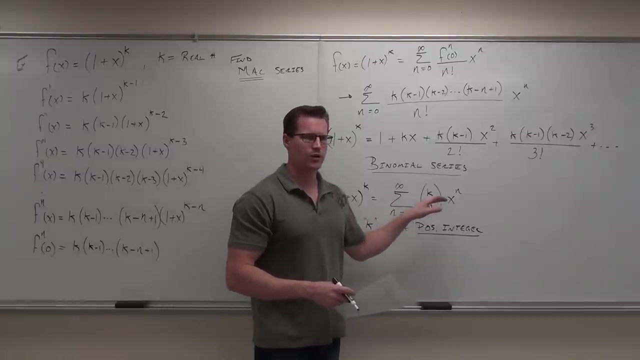 One, two, three, four, five, six, seven, eight, nine, ten, not zero. Does that make sense to you? Yeah, Well, k is one of those. If k is a positive integer, then this series will converge for all values of x. 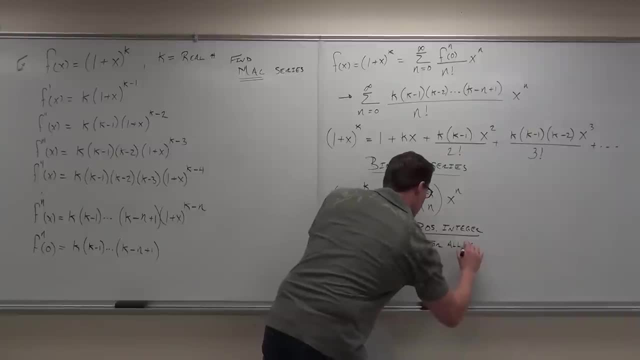 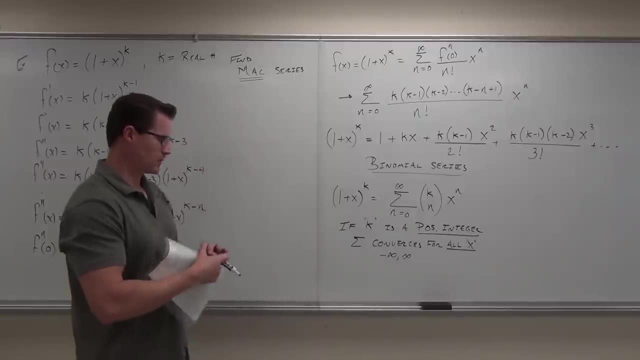 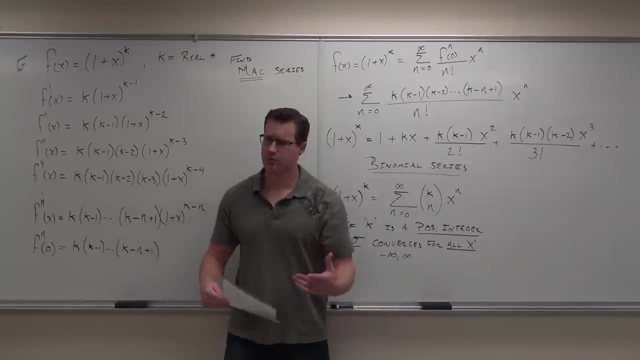 Okay. so let me put this in other words for you. okay, Let's say that your function was one plus x to the third. Is that a positive? is three a positive integer? Then this series is going to represent this function for any x to the third. 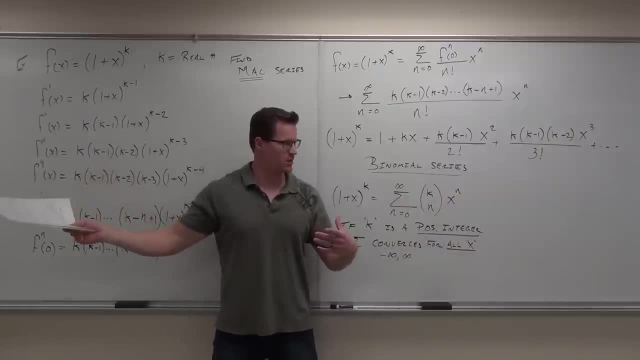 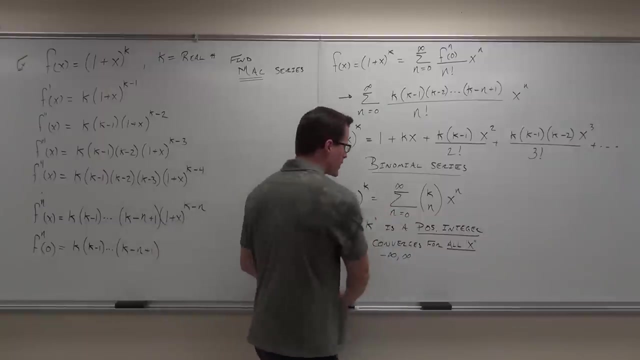 Any x. Does that make sense to you? If this was, if the k was now negative? four, is this series going to represent that for any x? No, No, but it will represent for a different set of numbers. okay, So here's the other choice, I guess. 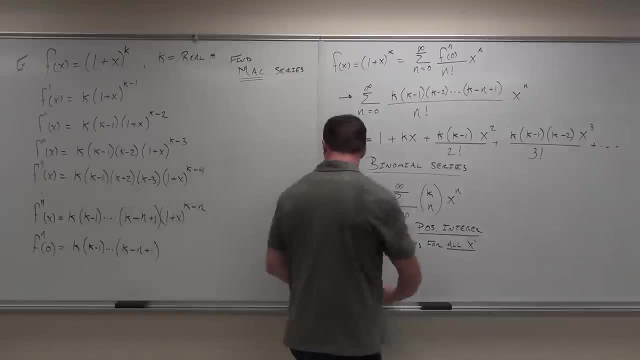 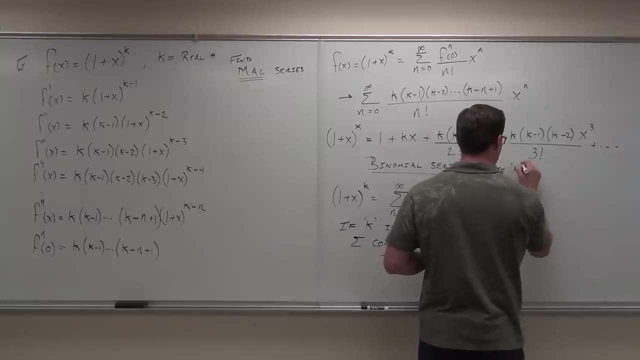 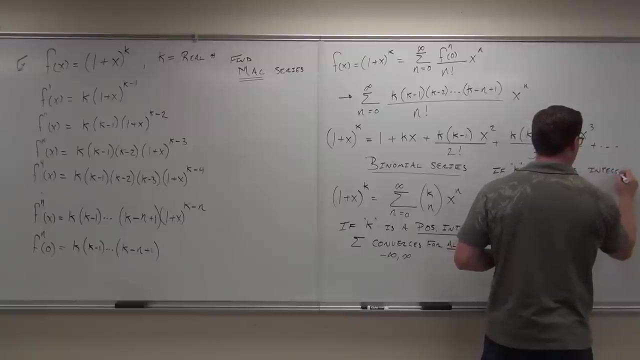 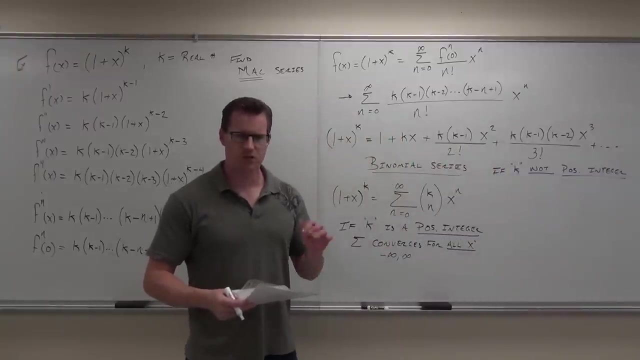 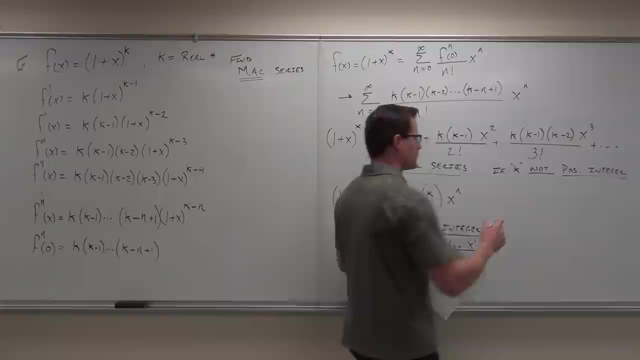 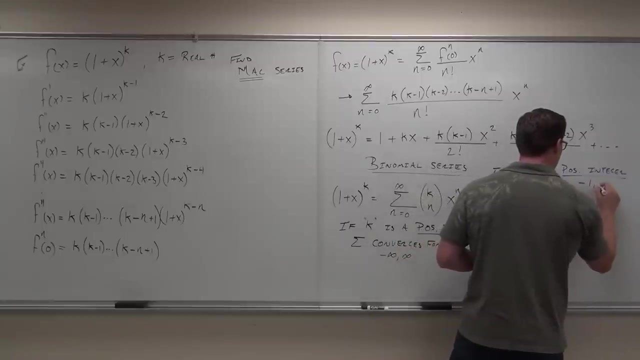 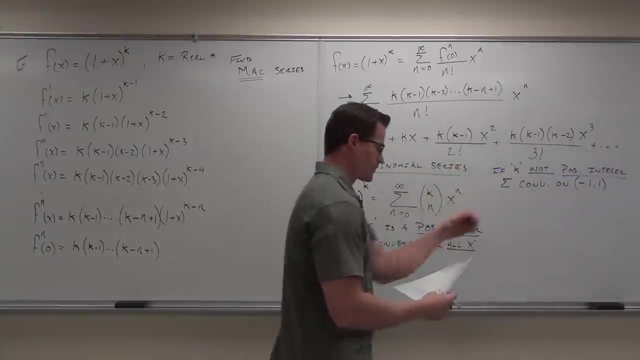 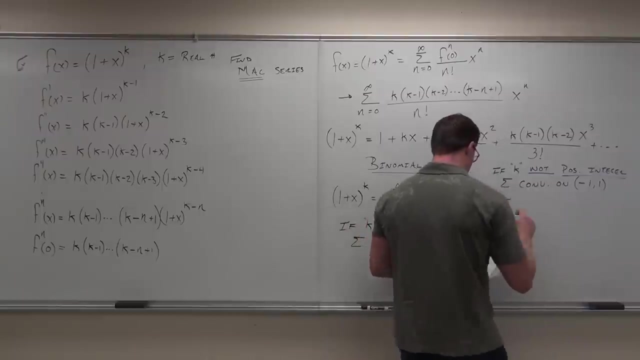 If k is not a positive integer. If k is not a positive integer, this series will converge, but it's only going to converge if x is between negative 1 and 1.. More specifically, if k is between negative 1 and 1,. 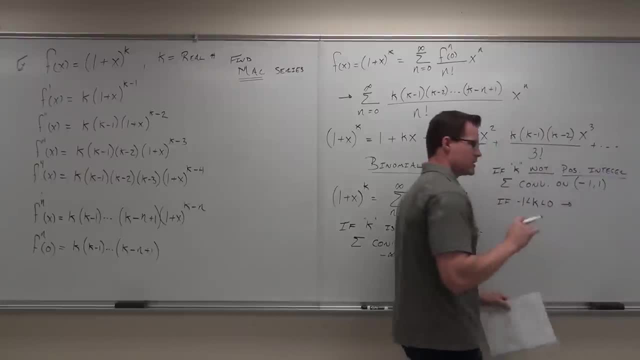 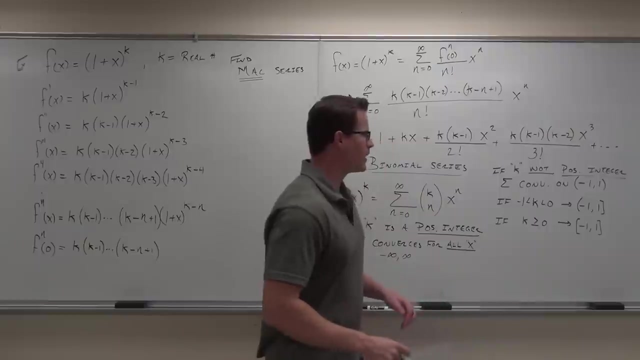 and 0,, we get to include the endpoint positive 1.. If k is greater than or equal to 0,, we get to include both endpoints. If not, we don't include any endpoints And that would be by the ratio test. 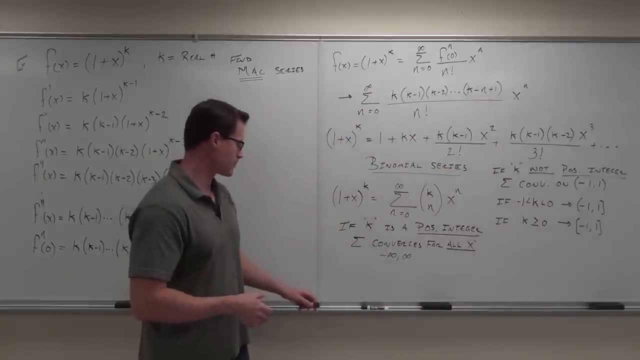 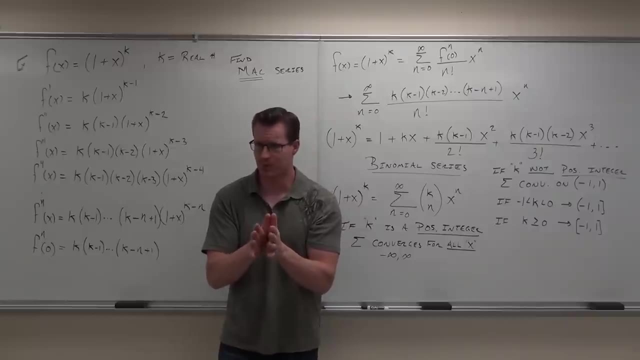 So let me go through it one time. as far as all this conversion stuff goes, You ready? I'll give you an example in just a minute. We'll go through it pretty quickly, but we'll give you an example here. So binomial series: no problem, those are binomial coefficients. 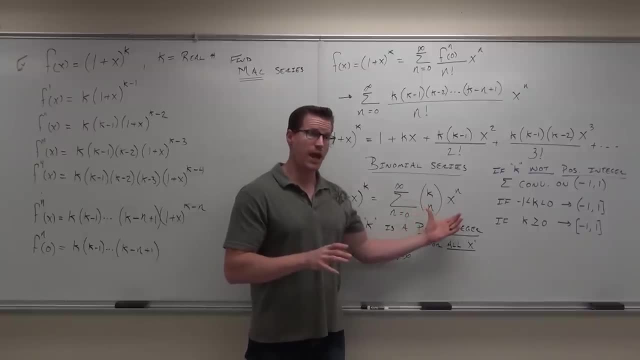 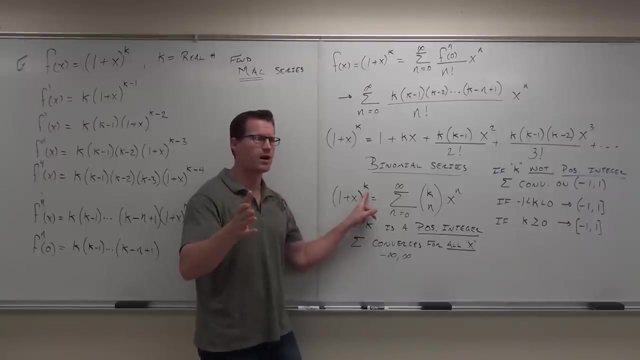 What this series will do. this series will converge and represent this function if k is a positive integer anywhere- 1,, 2,, 3,, 4,, 5,, 6,, 7,, 8, if k is sorry, if k is 1,, 2,, 3,, 4,, 5,, 6,, 7,, 8,, 9,, 10,, 11,, 12,, forever, no problem. 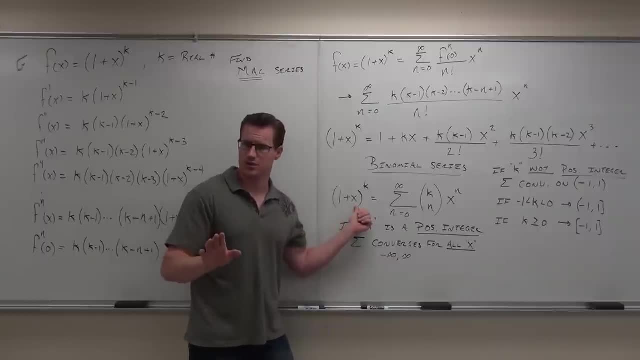 then this series will converge before any value of x that you want to put in there. Do you grasp that Your interval of convergence is negative? infinity to infinity. not a problem, It will always converge. Now, if k is not a positive integer, that would be 1 half. negative 4, negative 3 half. 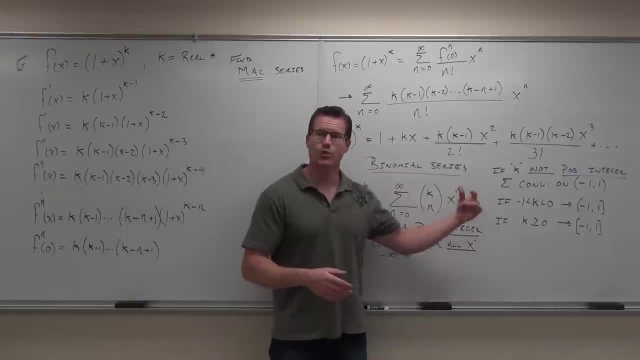 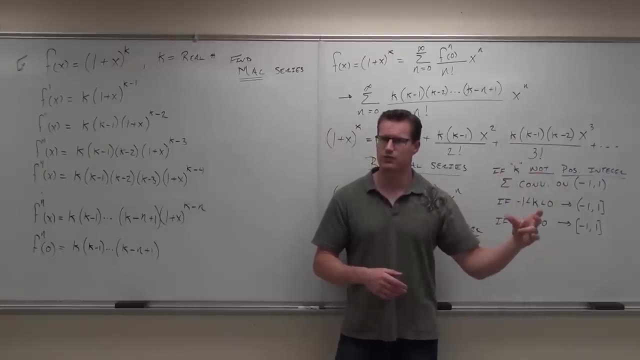 whatever it happens to be, this series will converge. it will represent your function, but only on the positive side, But only on the interval of negative 1 to 1, x equals negative 1 to 1. Those values of x will make the series converge if k is not a positive integer. 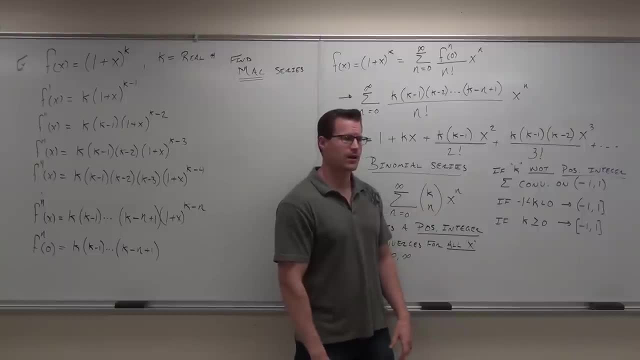 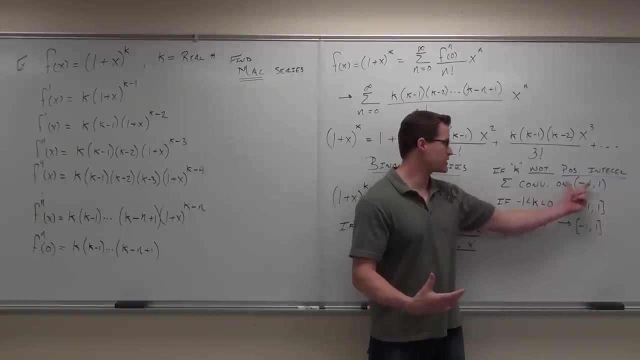 Have I explained that well enough for you? Now there's more specifics to it. If k happens to be between negative 1 and 0, you get to include the end point of this interval, 1.. If k happens to be between- well, not between, sorry- positive, so greater than or equal to 0,. 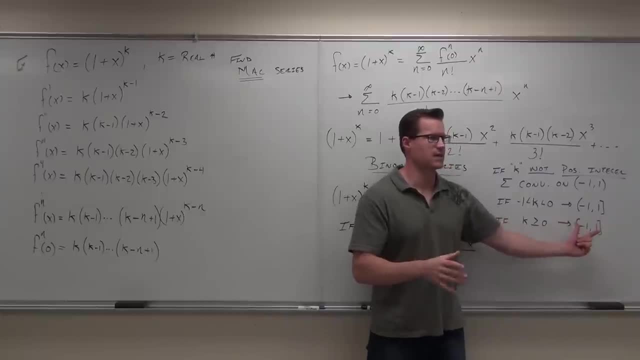 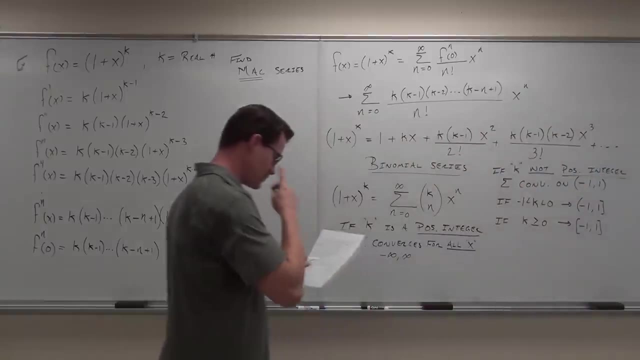 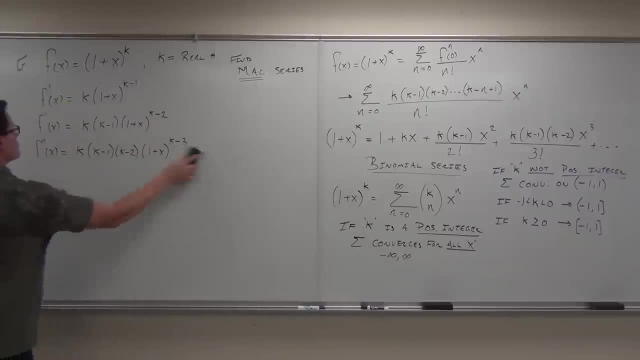 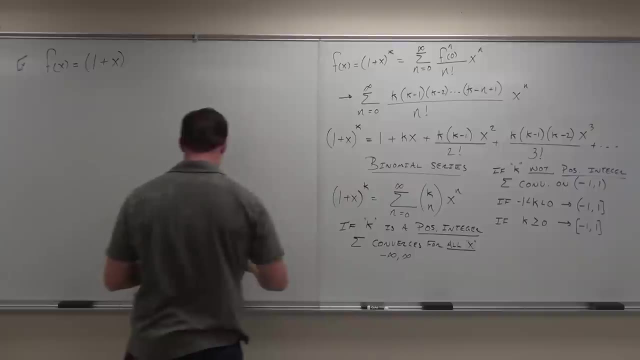 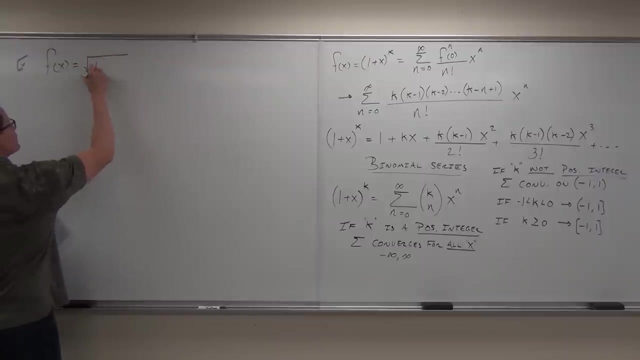 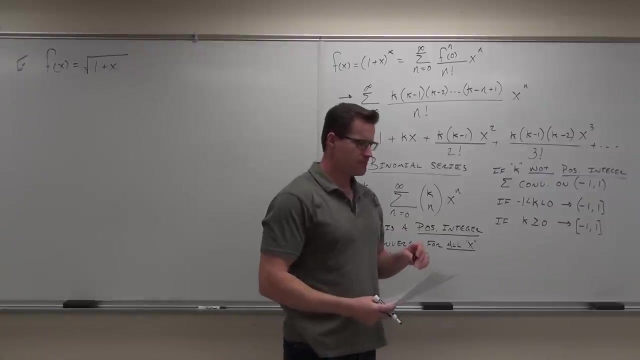 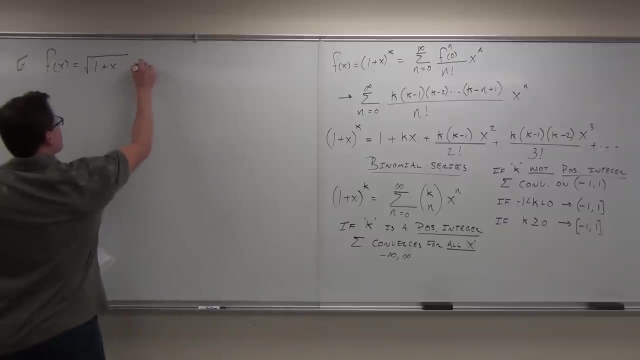 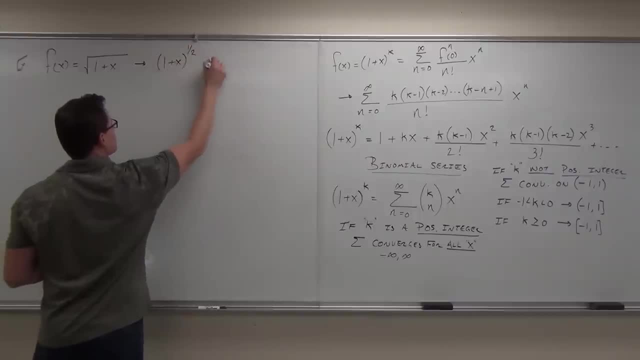 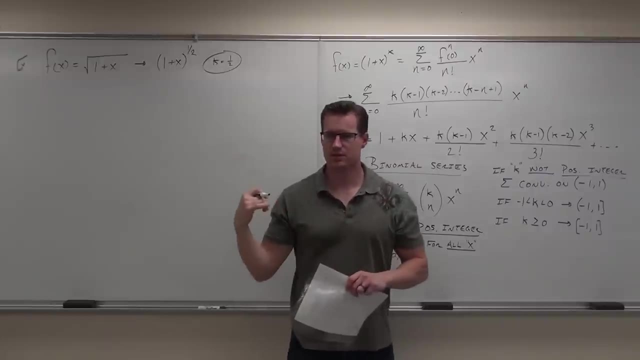 Do we currently have something? No, No Good. One and a half, OK, Good, Now can we represent this with a Taylor series or a Maclaurin series? Yeah, Yes, we can. And tell me something. 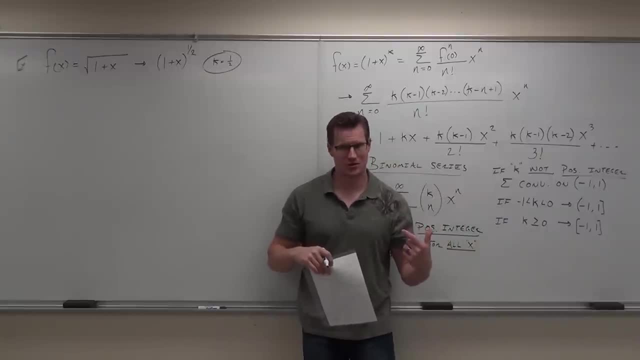 Will the series that we get converge? They all converge? Where will it converge For all x? or between negative 1 and 1? Negative 1 and 0.. OK, now let's think carefully. So we're not here, right. 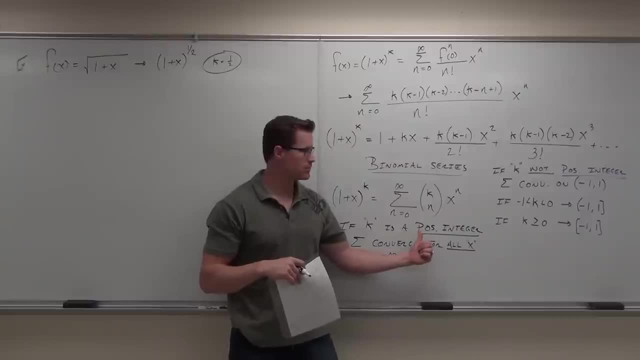 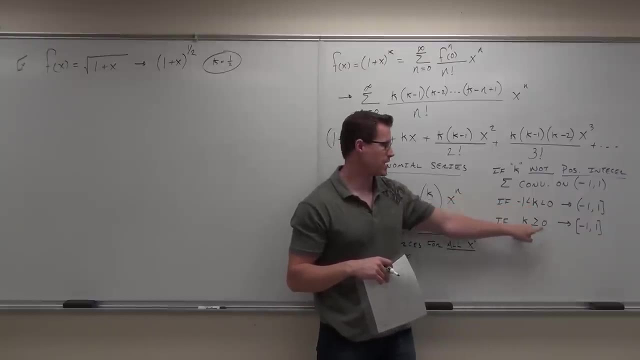 k is not a positive integer. k is positive. Is k between negative 1 and 0? No. Is k between negative 1 and 0? No. Is k bigger than 0?? Yes, We're here. If we weren't here and k was negative. 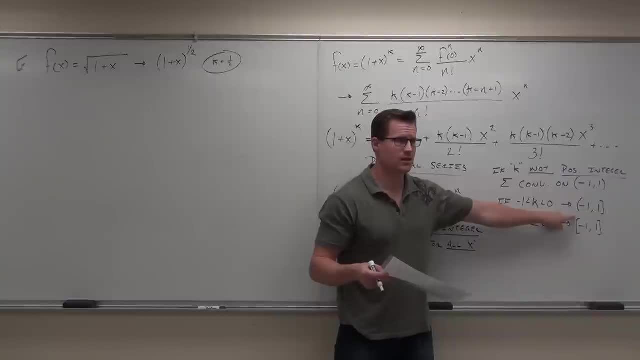 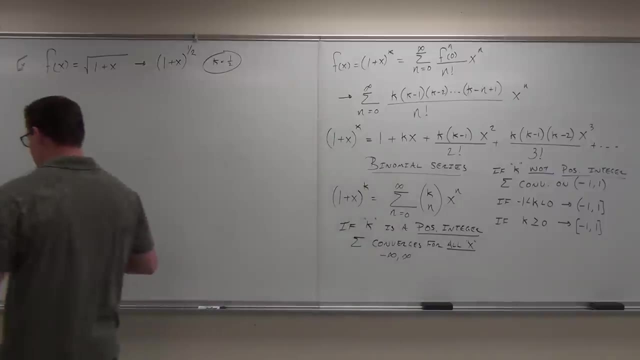 let's say k was negative 1, half we'd be here. Let's say that k was negative 2, we'd be here. Does that make sense to you? OK, so here's the deal. We can represent 1 plus x to the 1. 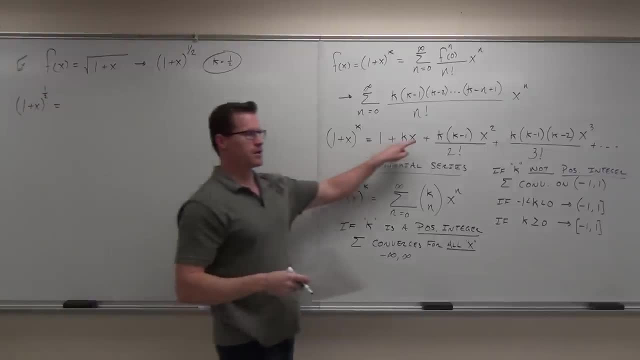 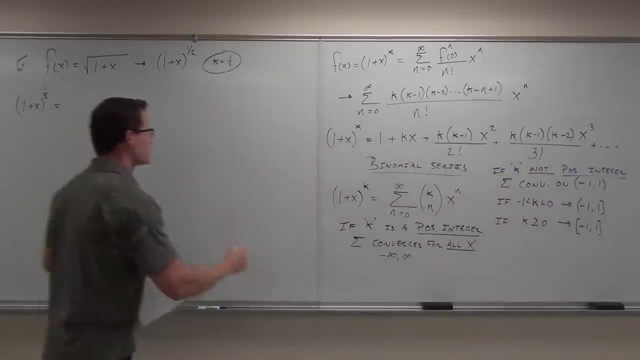 half. We can represent the power by listing out these terms, these binomial terms. So what we'd do is we'd say: all right, let's just follow this for right now. So we're going to start with what? Good? 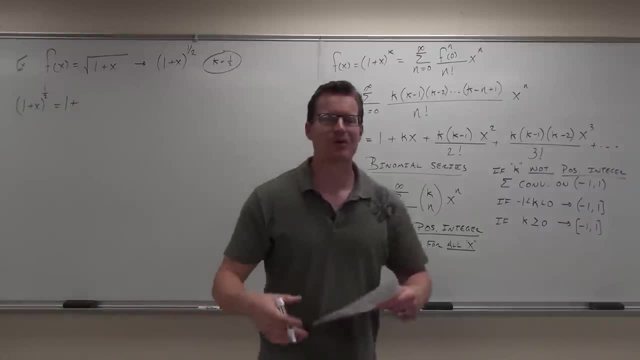 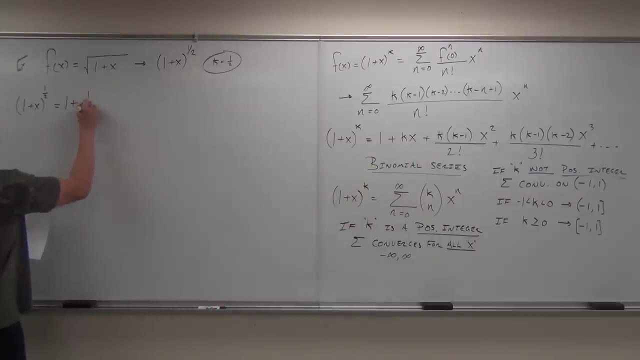 1. We always start with 1.. That was the easy one. OK, let's continue. What's the next term? What's our k? So we would have 1 half x plus. What's our k? again, 1 half. 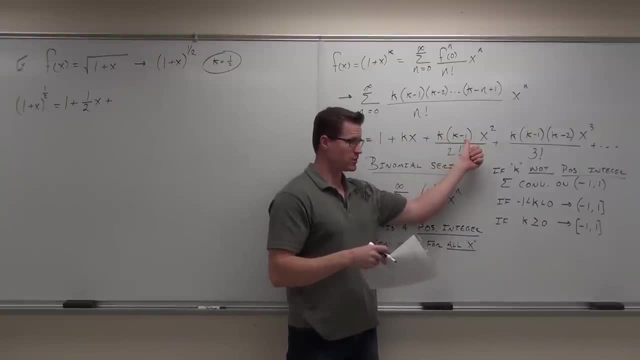 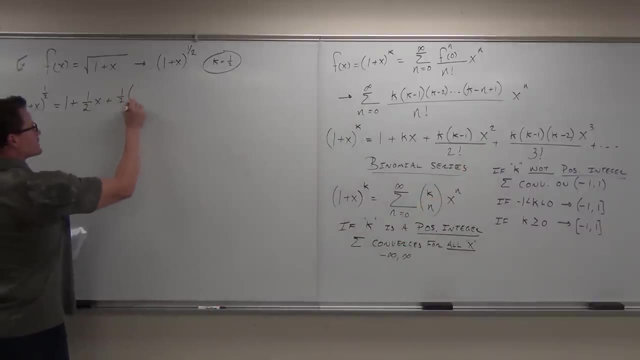 So we'd have 1 half times 1 half minus 1 times x, squared all over 2 factorial. So 1 half times 1 half minus 1 times x, squared all over 2 factorial, Then we have what? 1 half. 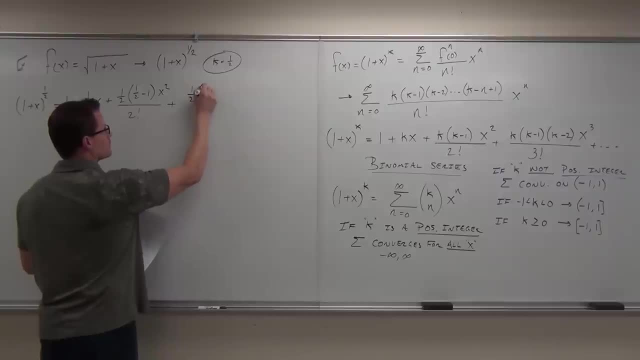 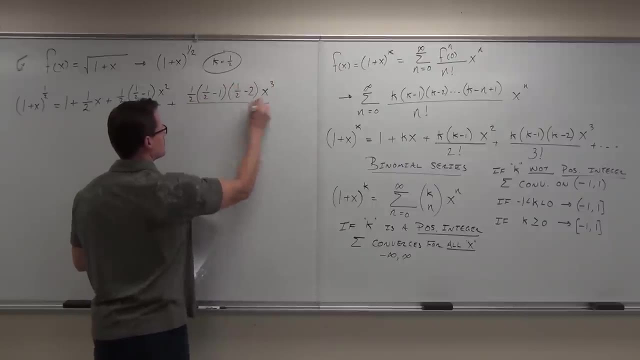 1 half. very good, Keep going. Times: 1 half minus 1 times 1 half minus 2.. Times: x squared: x squared from 2 factorial to 3 factorial 1 half. Could you do the next terms if I asked you to? 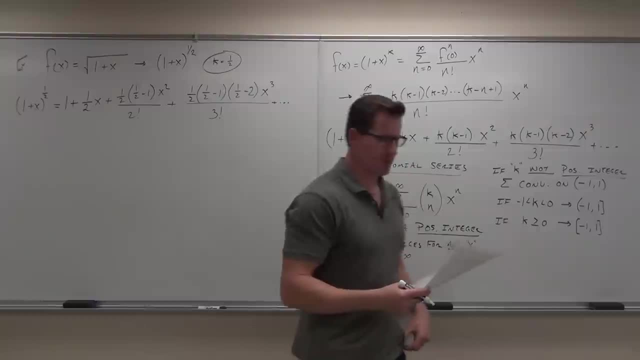 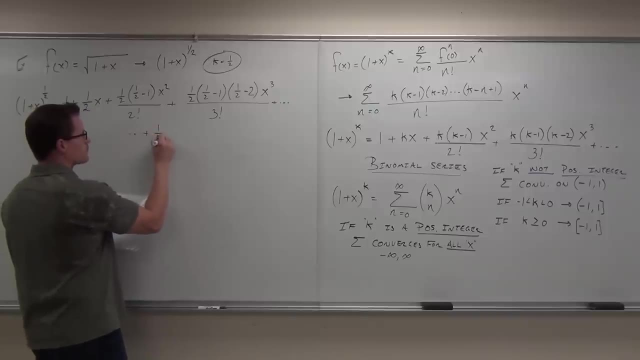 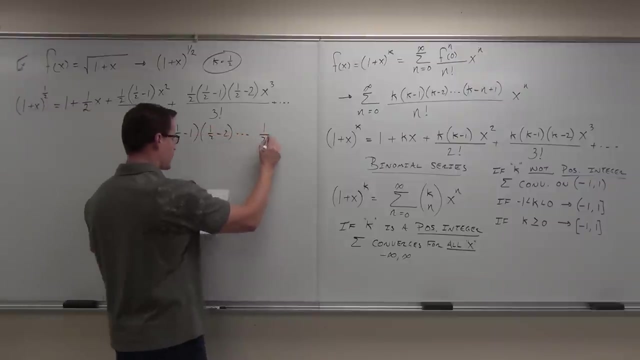 Yes, Very good. Now, ultimately, what we're going to get down to is: we're going to get this. We're going to get down to 1 half, 1 half minus 1, 1 half minus 2, 1 half minus n plus 1.. 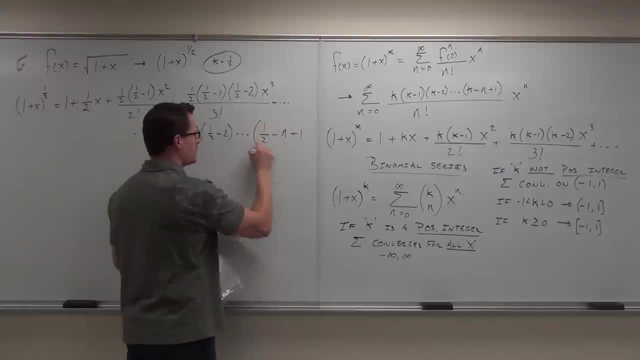 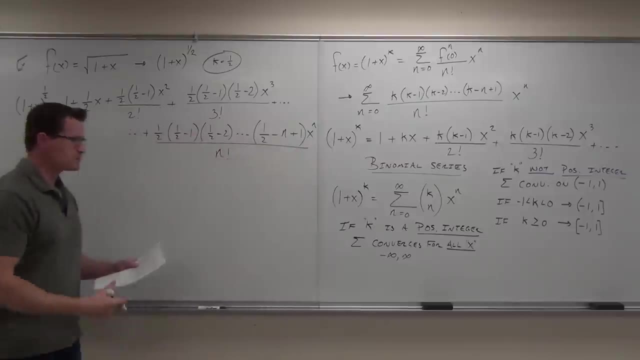 Remember that term: k minus n plus 1.. Okay, And we would have x to the nth all over n factorial. That's where we would end. Now we're going to simplify this a lot, a lot, a lot. So we've got to look at what these things are actually doing, these fractions. 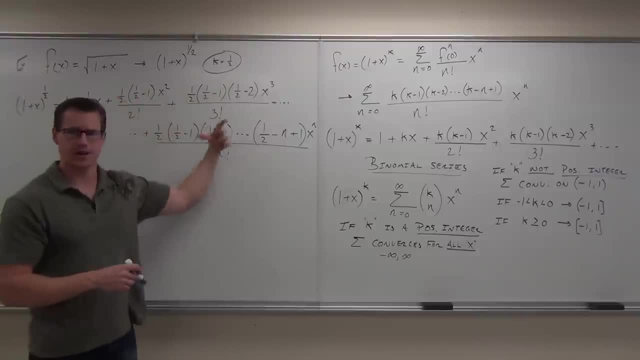 What we're going to do is we're going to take these fractions, simplify them and look how that affects our problem. Are you with me? Are you sure you're with me? Okay, Let's think about 1 half times, Whatever this happens to be, 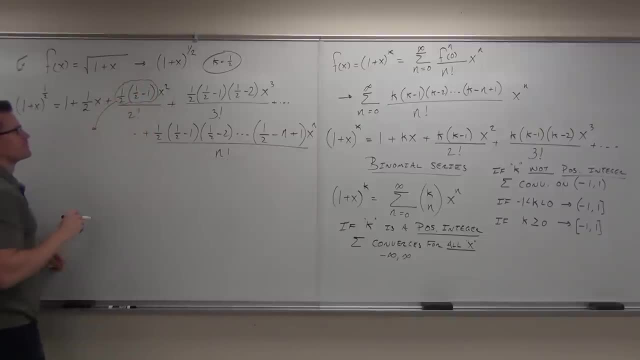 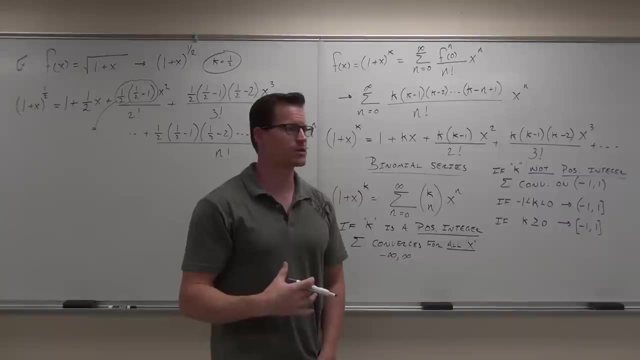 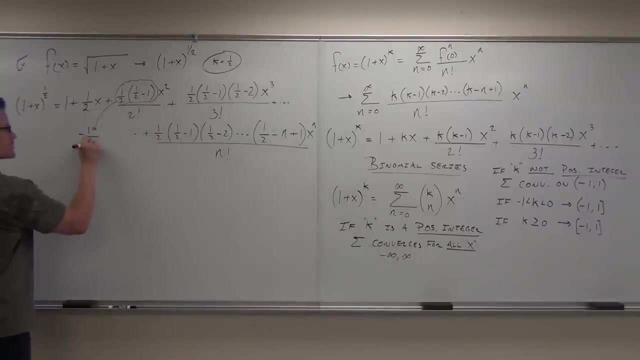 What's this going to give you? Okay, Remember what we do with patterns. What we do with patterns is we don't really multiply things. I know it's negative 4.. But what I want you to see is that this is really negative: 1 over 2 times 2.. 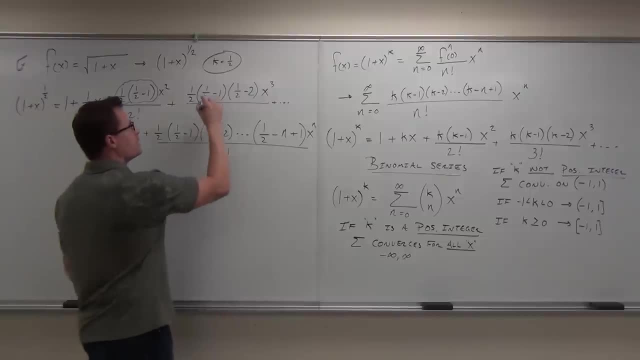 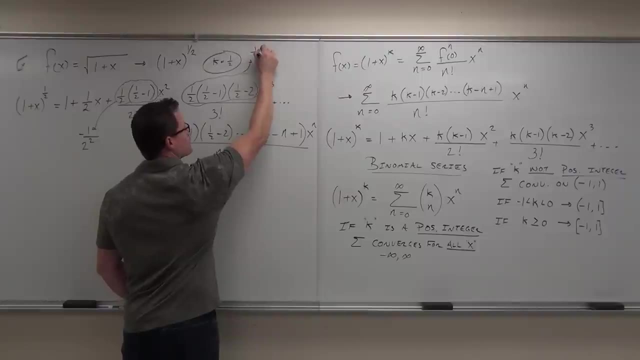 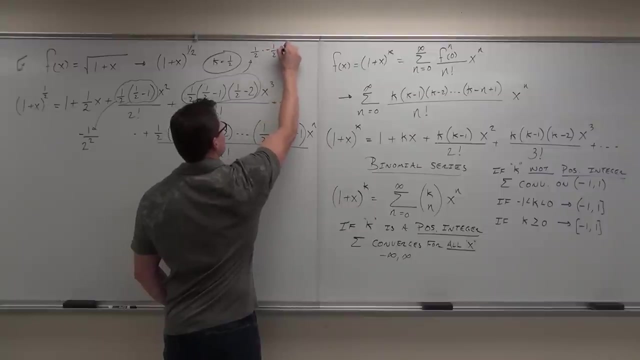 Do you see it? 2 squared, This one Would be 1 half times 1 half. negative times, negative, 3 halves. Am I right? Or would it be positive or negative? Positive, Positive, And you would get 3 over 2 cubed. 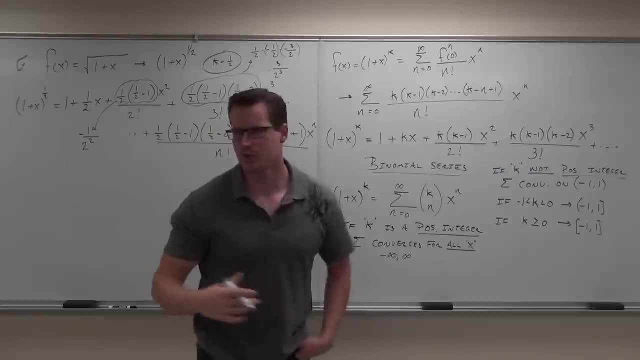 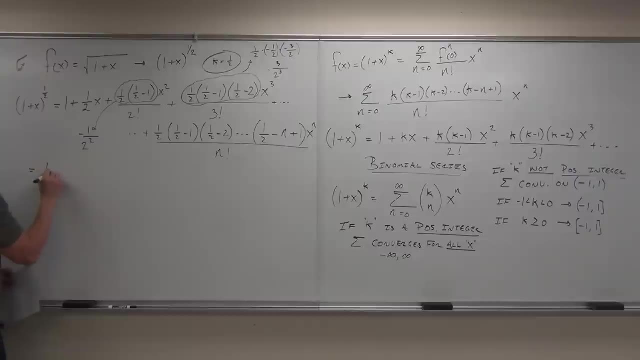 Are you with me? Yes, Okay, Let's put this together then. So what this becomes. We'd start with 1. We'd have 1 half x, but then the next one. Check this out. This is where the pattern actually starts. 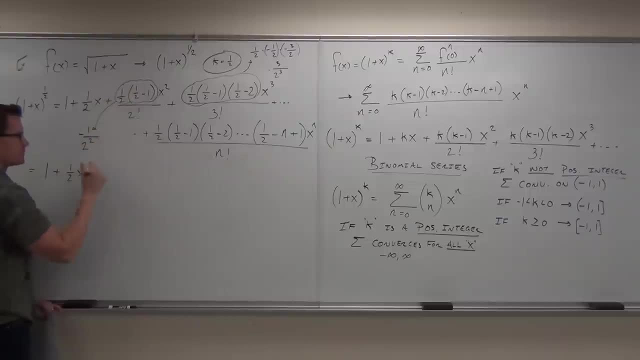 So positive, positive. What's the next term going to become? We're going to have x squared all over 2 factorial times 2 squared. This, right here, is negative: one over two squared. If I take this, this goes on my denominator. 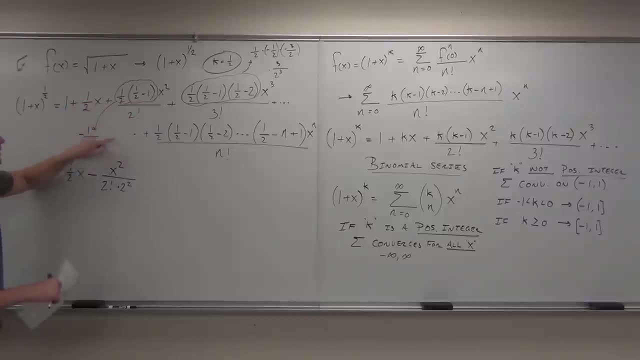 this negative changes that to a minus. I have an x squared on my numerator. I have a two factorial on my denominator and now the two squared on my denominator. The algebra can be a little tricky if you're not super good at algebra. 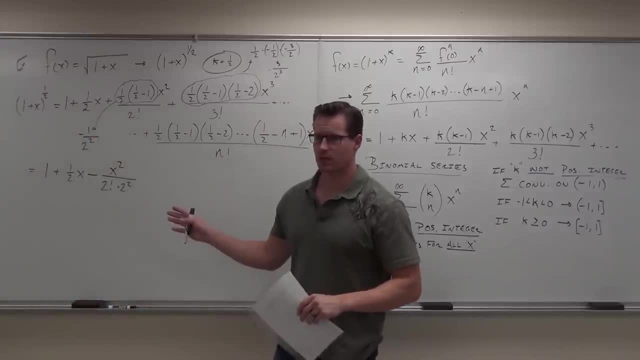 Do you see what I'm talking about here? Yeah, Are you sure? Have I lost you? I don't wanna lose you. Okay, let's go to the next term. Come on, stick with me here, folks, Do I have a plus or a minus? 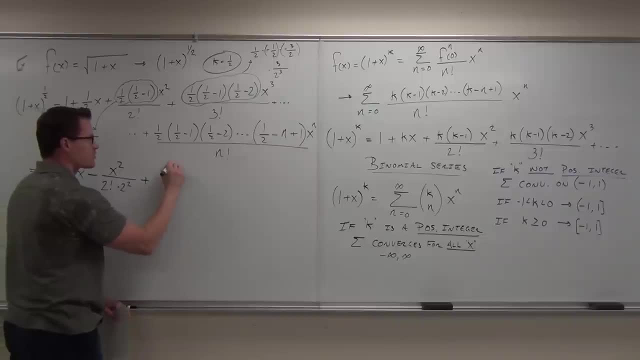 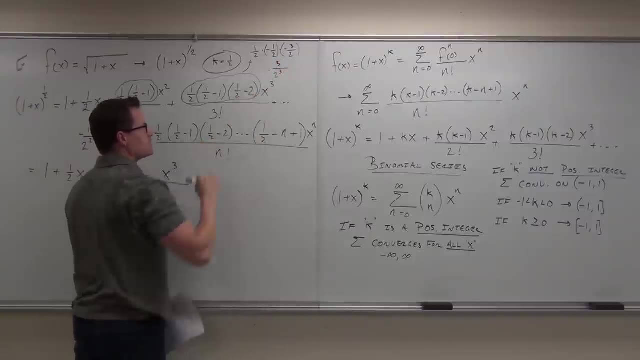 Plus. It's gonna be a plus because it's positive. I'm gonna have an x to the third on my numerator. Do you see why? Now, this was three over two cubed. So what I get is: where would the three be? 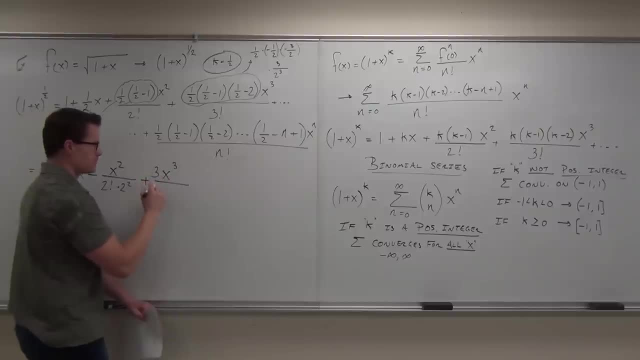 The three would be on the numerator. Where would the two cubed be? Three factorial times two to the third. Does that make sense to you? Okay, now the next one. Let's see about the next one. Do you suppose the next one's gonna be positive or negative? 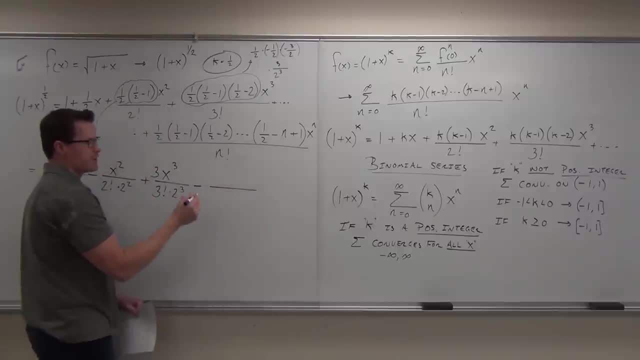 Negative. Okay, On the numerator. do you understand? I'm gonna have an x to the fourth. Yes, Do you understand that I'm gonna have a four factorial somewhere? Yeah, Do you understand? I'm gonna get a two to the fourth. 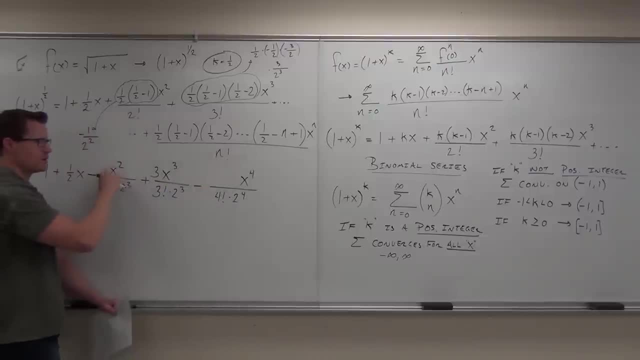 Yeah, Now these numbers are interesting. This goes one, See where the one's coming from. Five, Three, Five, See, actually it's one times three, isn't it? This is one times three times five. The next one would be plus. 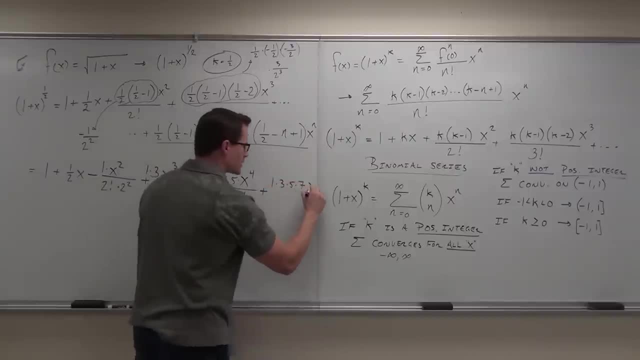 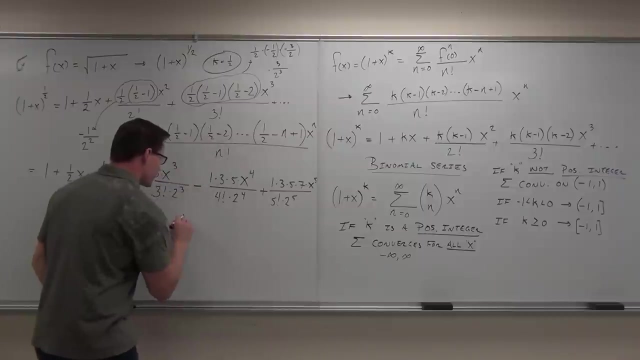 One times, three times, five times seven, X to the fifth over five, factorial to the fifth, And that's the pattern we're looking for. The last term, the last term as we end this it's gonna be. there's actually no really good way. 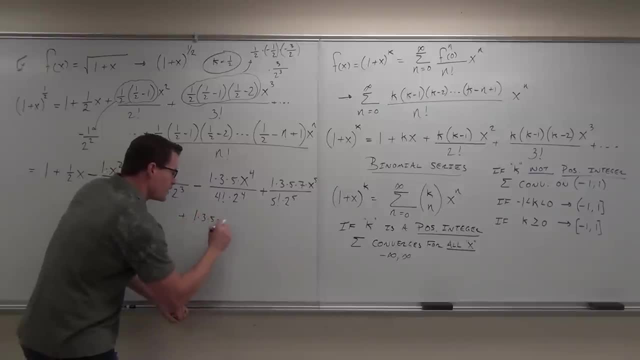 to write this pattern. It's one times three times five. You've gotta write that out and then go. okay, well, where's it ending? It's ending at two n minus one. It's ending at an odd number: Two n minus one. 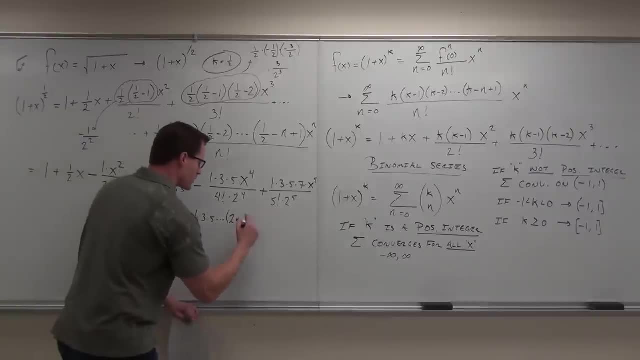 I'm sorry, two n minus three, because the minus one would give us too much bigger. oh, one bigger minus two. X to the n all over. let's see if it matches. This is our n matches our factorial. 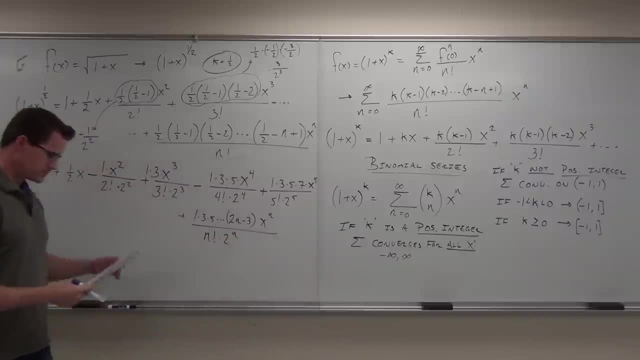 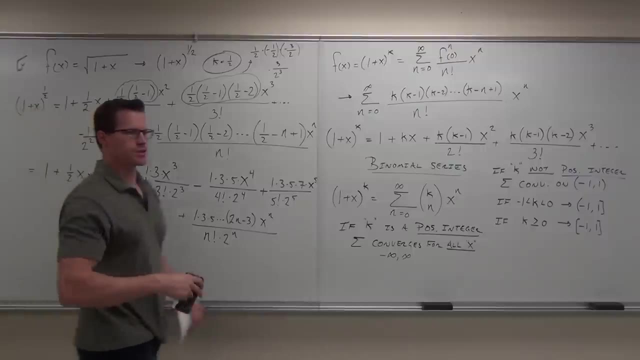 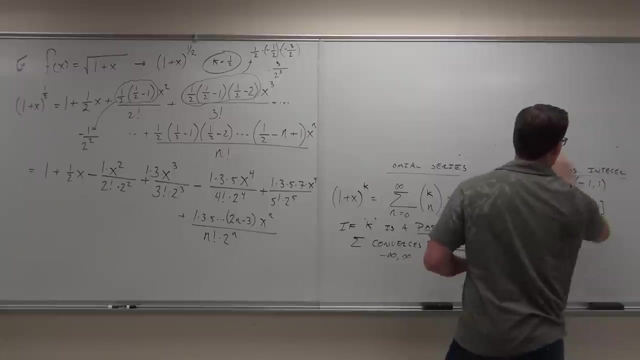 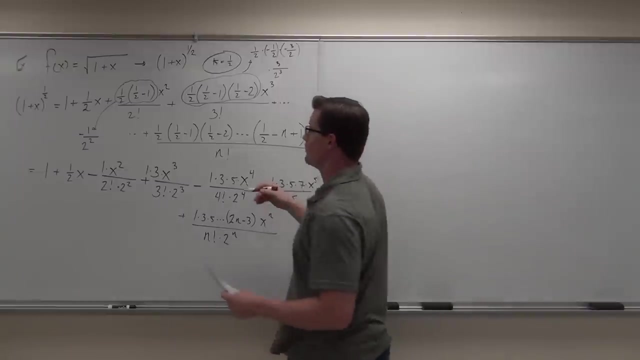 n, factorial two to the n. Now, because this pattern starts at the second term, we're gonna define it this way. So what we know, we can represent this function one plus X to the one half by doing this. Do you guys see what I mean about the pattern starts? 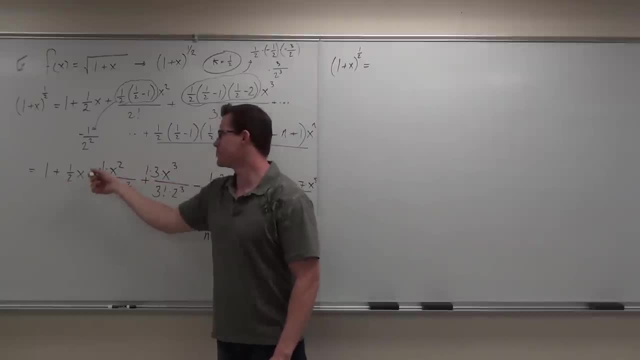 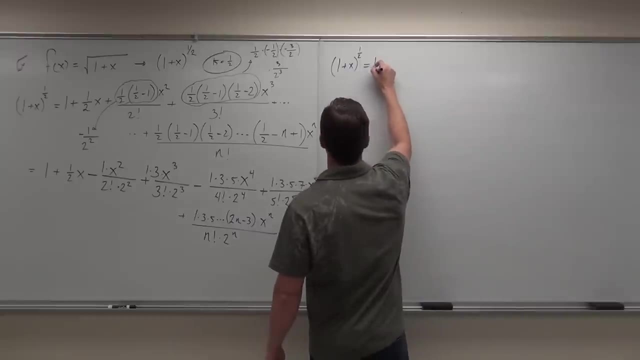 at the second term. This pattern doesn't really start right here. This is positive, positive, and then we go negative. The pattern starts here, So you can define a series like this or a function like this. Define it like: okay, well, we got one plus one half X. 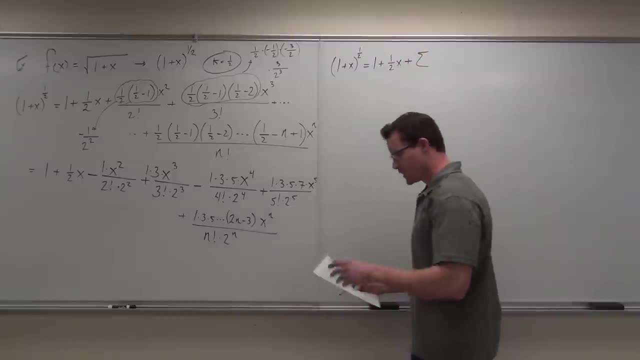 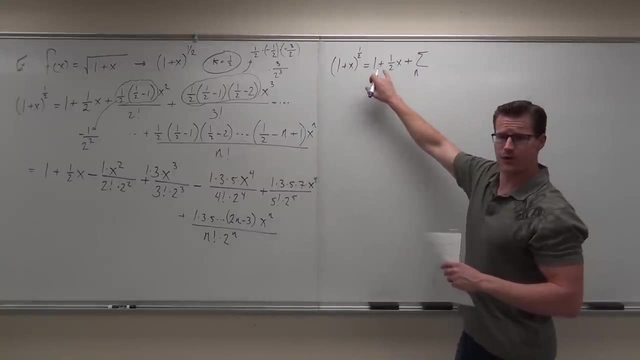 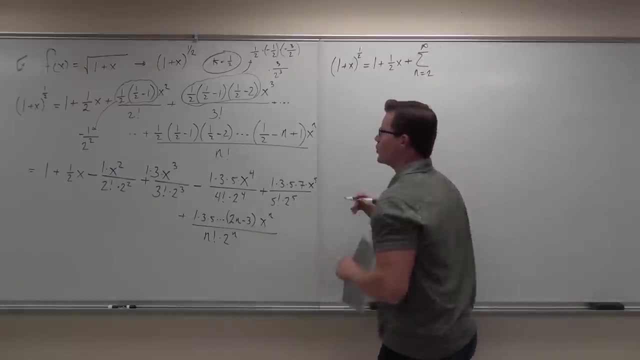 plus, and then we're gonna start with our series. The series does this: It starts at the. if this is the zeroth term and this is the first term, our n would be starting at the two To infinity. We gotta start with. look at this. 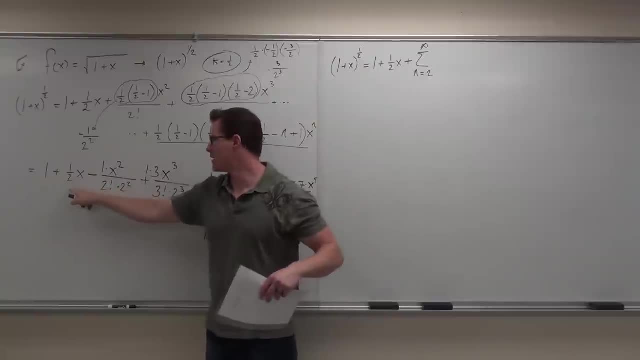 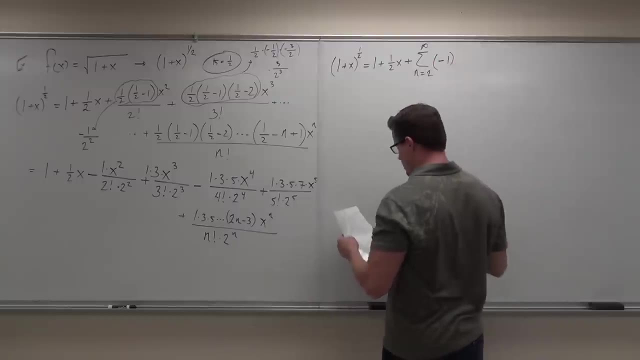 Do you guys see that? I have the same one, I get the same one half, and then I have a minus. I get to start with a negative term. So what we're gonna do is say I want this negative one to start by being negative. 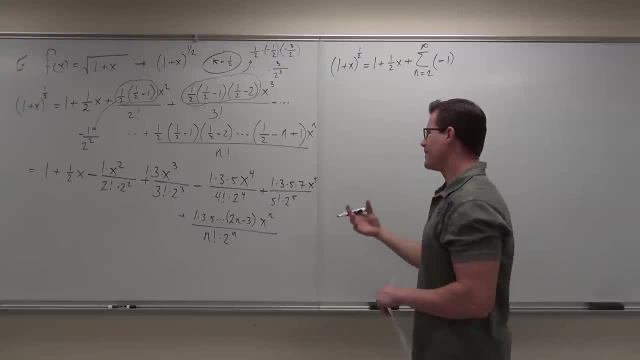 How can I do it? N minus one? I can do n minus one. We're gonna use n plus one, just so we don't have any problems with it. We can do n minus. I think n minus one will work as well. 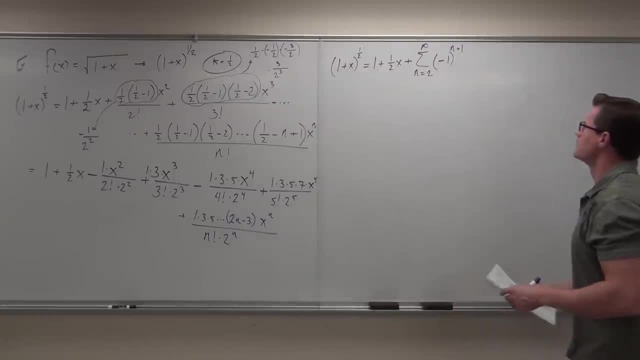 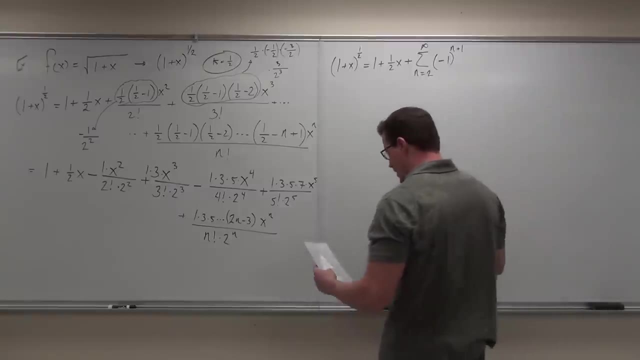 So n plus one, did you see? it's gonna be the same exact thing. It's gonna be a negative plus one. okay, cool, After that. well, we have man. the pattern starts. The pattern does this Omit these first two terms? that's what this does. 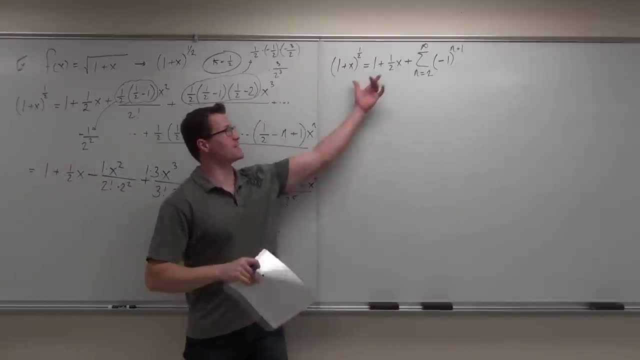 It says: hey, put the first two terms, Then start your series. this is like where we start our series. Start your series with a negative, then make it a positive, then a negative, then a positive. That's what this is doing. 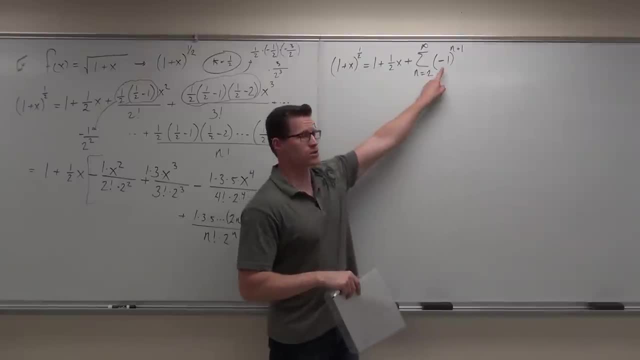 Start with a negative, then a negative, then a positive, then a negative, then a positive. That's what this is doing: Then doing positive, then negative, then positive. Are you with me still so far? Yeah, The numerator of your series does this. 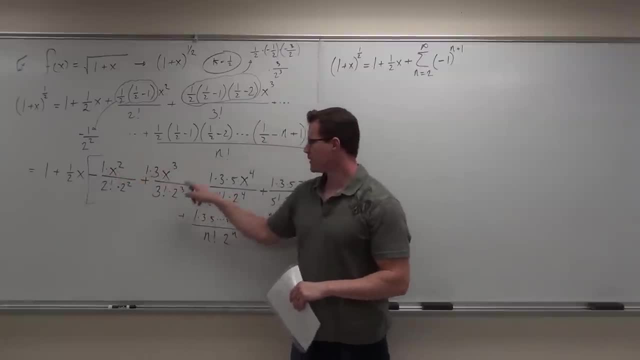 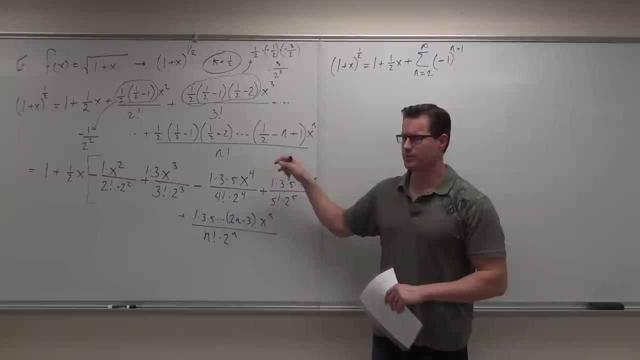 The numerator goes: one, one, three, one, three, five, one three, five, seven, one, three, five, seven, nine, blah, blah, blah, blah, multiplying by all the previous odd numbers. It's not a factorial. 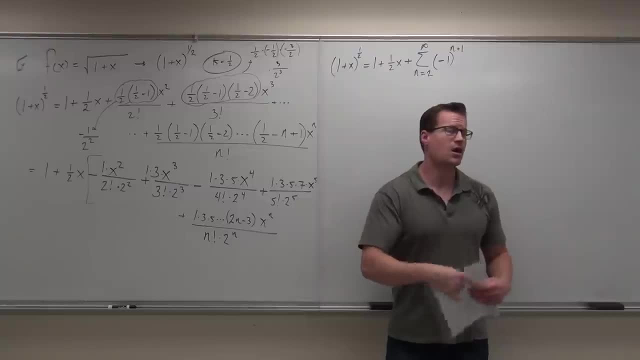 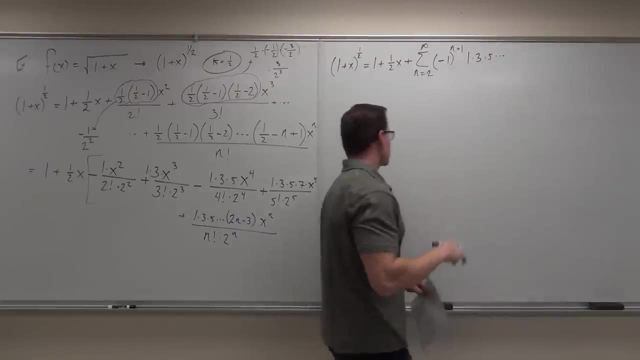 because you're not multiplying every single number, You're multiplying only the odd numbers. The only way we represent that is by showing it. Then we do one times three times five, and then you say you're gonna stop at. well, what we want to stop at is: 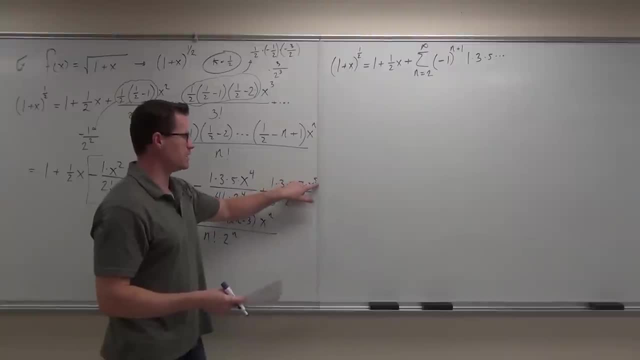 let's see this would be compared to this n. this would be two times five minus what. to get this Two times five? because we want to be some n right And it's gotta be odd. so it's two times something. 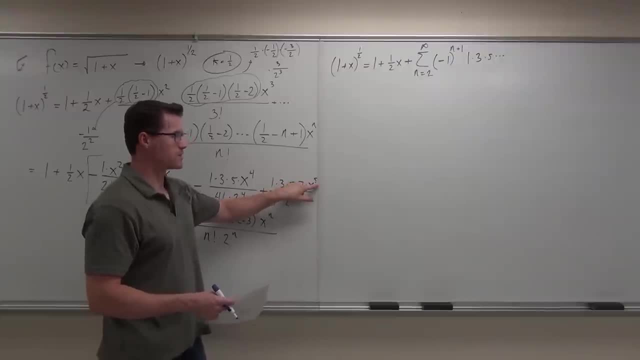 minus one, or minus three, or minus five. Well, to get this number, it's two times five, which is 10, three, not one. It's not stopping at nine, it's stopping at seven, One odd number before. 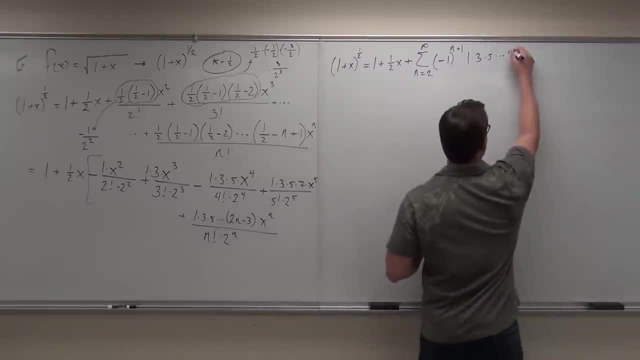 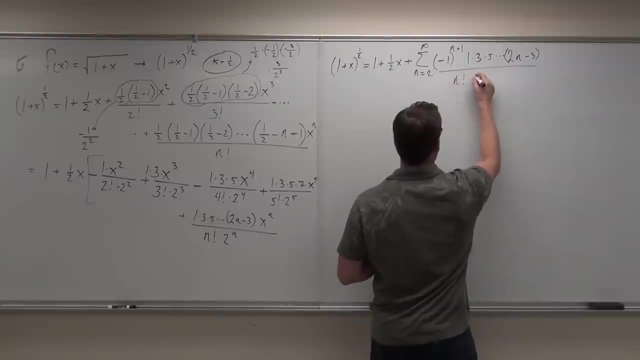 Two n minus three That. So we're gonna stop at two n minus three. That's our numerator. Our denominator is only n, factorial, no problem. Two to the n, got it. And then we have x to the n. 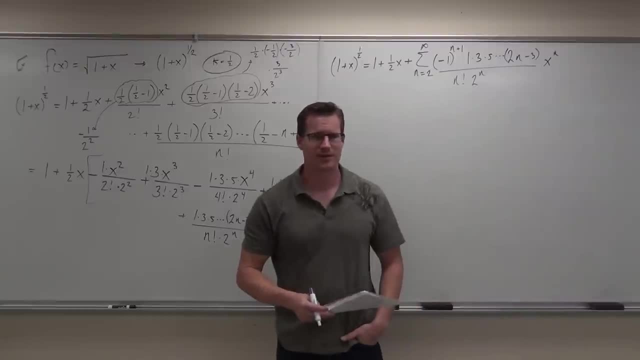 And that's about the nastiest freaking thing that you've probably ever seen. yeah, Yeah, Crazy A little bit. Do we have to check for convergence? Yes, No, No, no, because we already did it. I would have proved it to you. 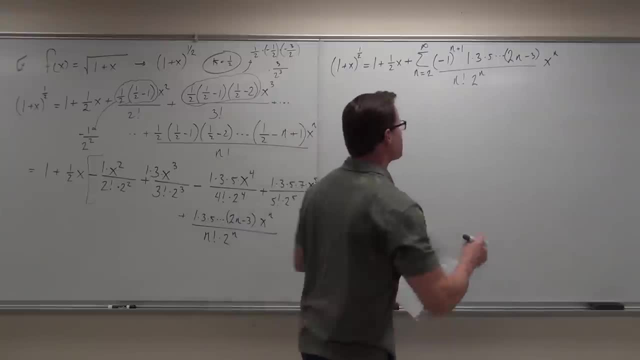 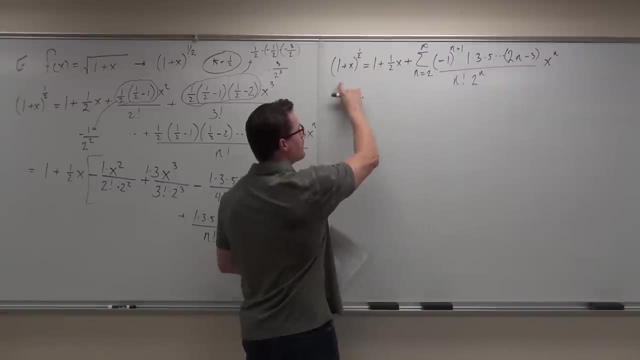 in the very first example we did today. So what we'd say is that so f of x can be represented. that's what this means. f of x can be represented by this series on the interval. What's our interval? 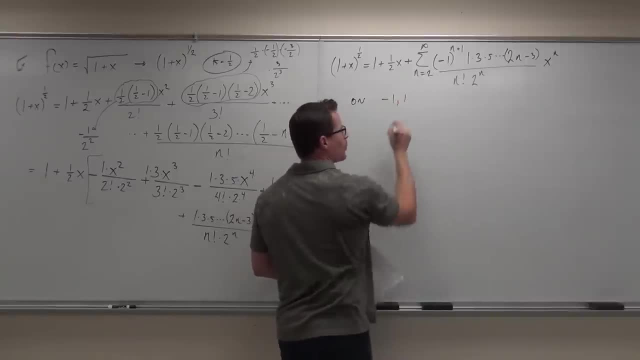 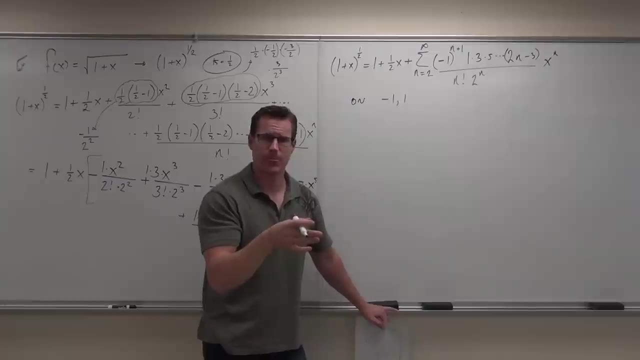 Negative one to one, including both. Why including both? Because it's greater than zero. That x is Good. yeah, x is the k. the k is greater than zero. It's not between negative one and zero. Also, this would be all real numbers if k had been what. 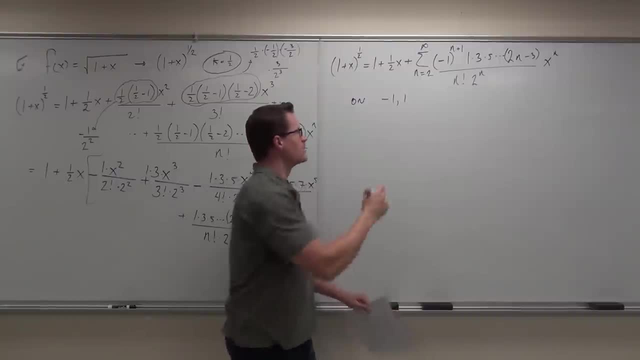 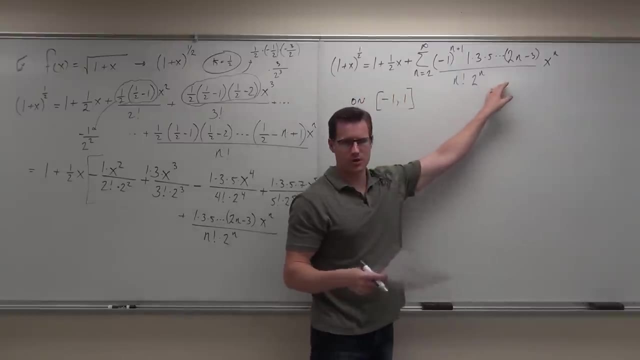 Positive integer. Positive integer, that's exactly right. So we'd say this: we'd say that our function can be represented by this really nasty series. We know it's gonna be convergent, because we already proved y we already showed that. 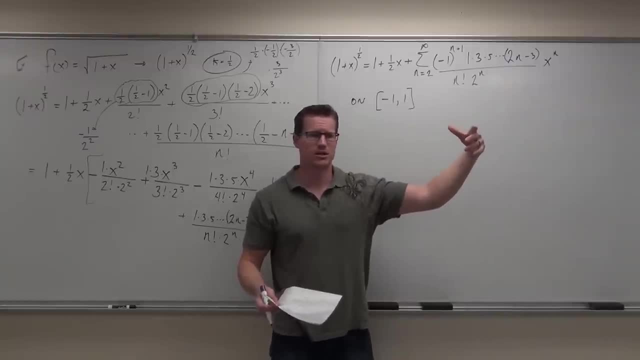 If k is positive integer for all real numbers, x. If k is between negative one and zero, then it's for x equals negative one to one, but only including the endpoint one. If it's outside of that range, if it's less than one, less than negative one. 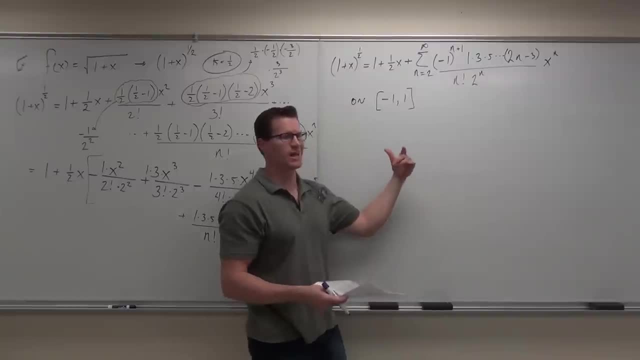 then it's only for negative one to one, not including any endpoints For us. we say, hey, look at that, our k is not a positive integer, but it is positive. If our k is not a positive integer, but it is positive. 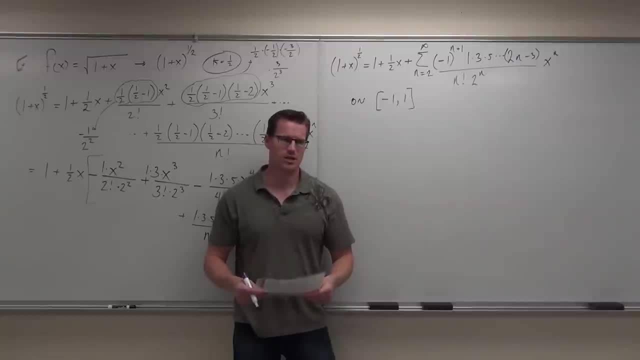 we include both of our endpoints. it goes from negative one to one. That was a crazy example. Show of hands if you hung with me, or okay on it. It's a little weird, right? Is it gonna take some maybe thinking about later? 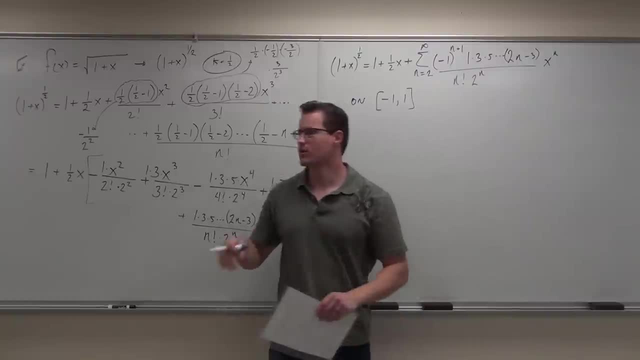 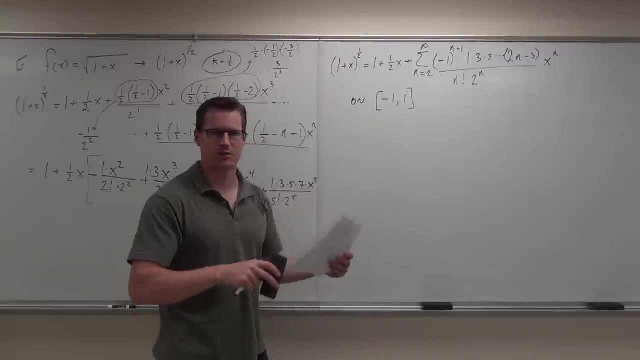 Maybe, maybe, watch this part again. Now, what we're gonna do from here on out. I'm gonna show you how to make your given function fit a series we've already done. I'm gonna list out some series. Most of them we've done already. 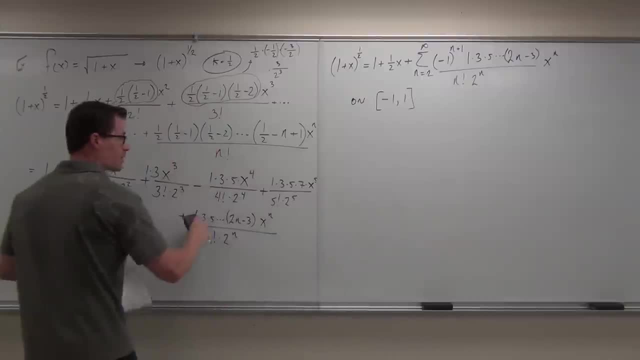 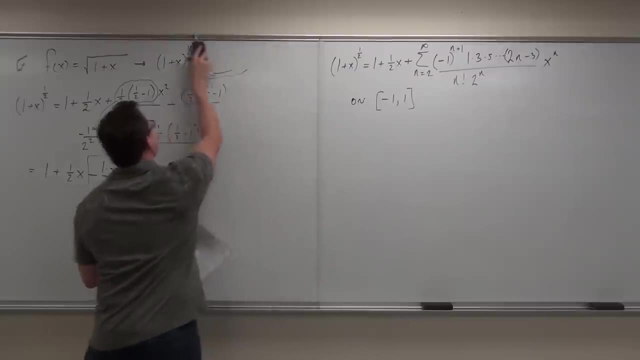 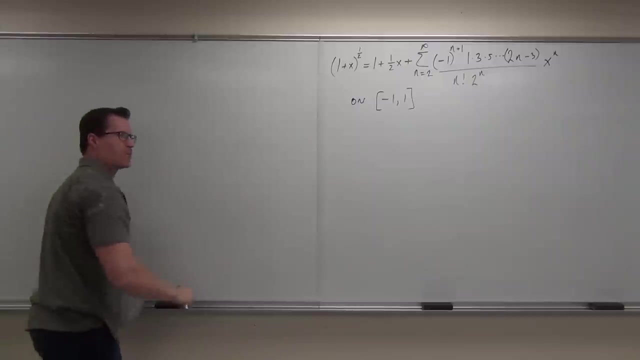 The last two. well, there's two or three of them that we haven't. Are there any questions? No, thank goodness. okay, That's great. Okay, I need you to write this quickly. We've already done. they are in your notes. 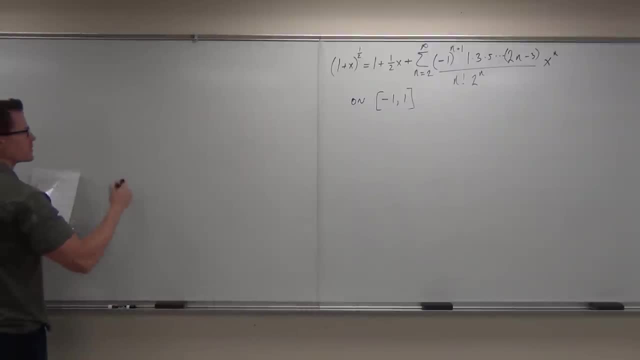 I'm just recapping here. So here's some common Maclaurin series That's smaller, I think. Okay, okay, all right, So we're gonna go back, and then we're gonna take one first and then, and we're gonna 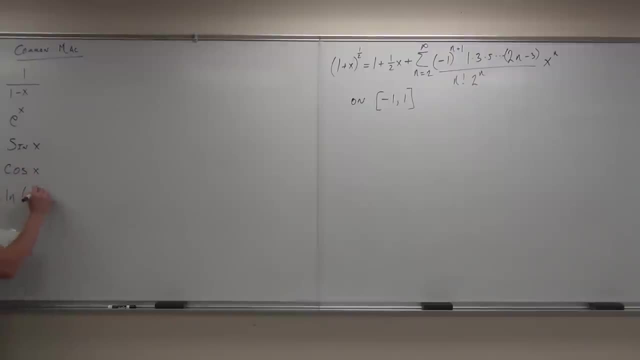 All right. So we're going to take a little bit and we're gonna use the hand written by the master. All right? Okay, All right. So what I'm going to do for you is I'm going to give you what these series look like. 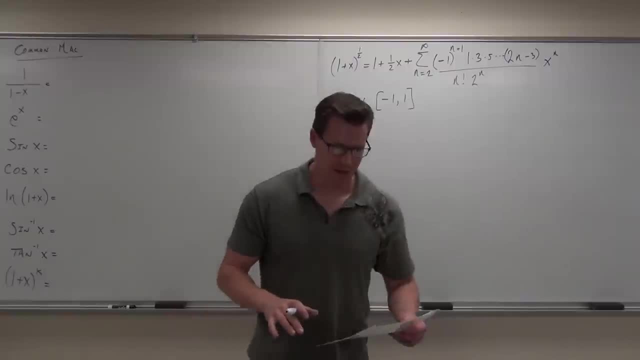 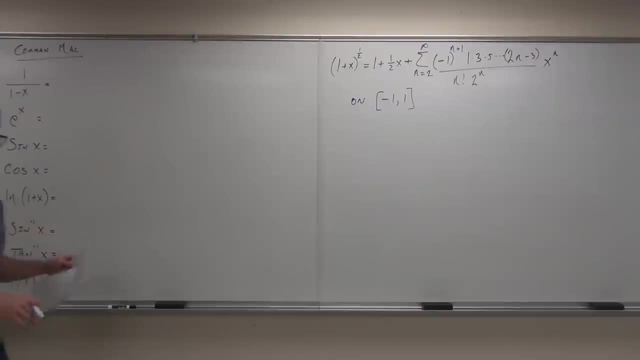 I'm going to give you the actual series notation for it And I'll show you how to work with it, because it's going to be really nice. I promise You're going to like this better than what we just did. Well, that's not saying much anyway. 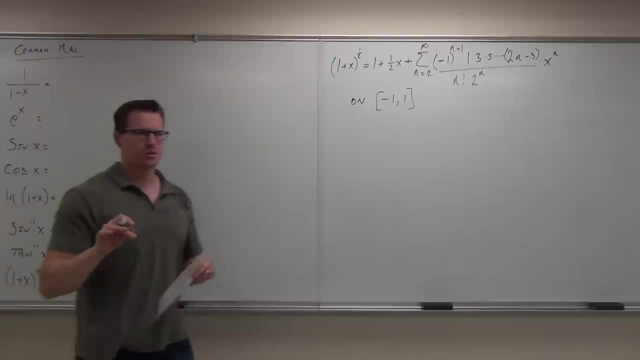 So here we go. What this series is. do you remember doing that? It's one of the first ones we did. We took an integral of this. It became negative ln of 1 minus x, and then we divide it and we got this: 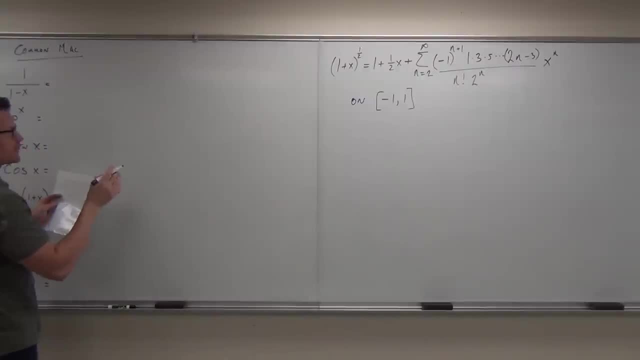 We got. well, that represented ln, But this series is represented by 1 plus x plus x squared, because what it really is is simply a geometric series. Remember that a was 1, r was x. Bam, this is our geometric series. 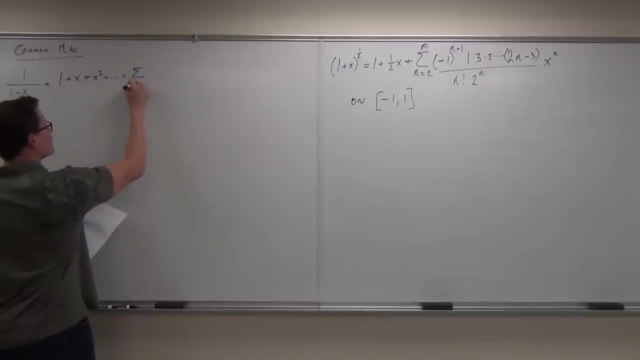 And it was simply represented by this, And the interval of convergence was negative 1.. It was negative 1.. e to the x was a nice one, It was 1 plus x plus x squared over 2 factorial plus x to the third, over 3 factorial plus. 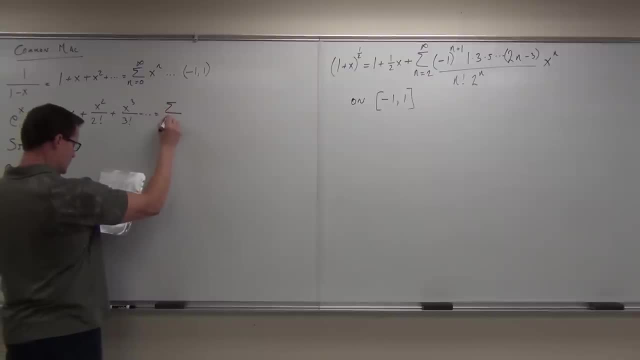 and that's the series from n equals 0 to infinity, of x to the n over n factorial. So we got the real numbers for all, real numbers, Sine. Do you guys remember doing sine? Remember doing some of these ones? We worked through them. 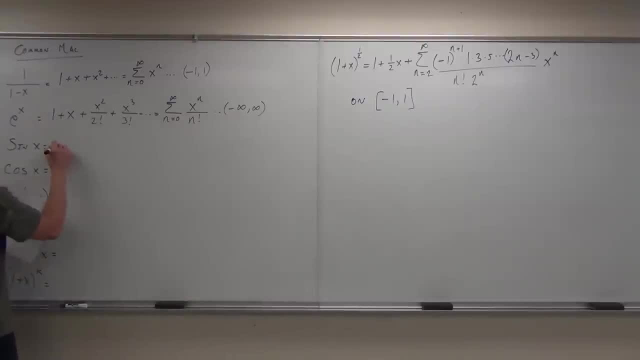 This is all of our examples. We made them from scratch. Sine was this: It was x minus, x to the third over 3 factorial plus, x to the fifth over 5 factorial Over 5 factorial minus, And that created the series for us from n equals 0 to infinity negative 1.. 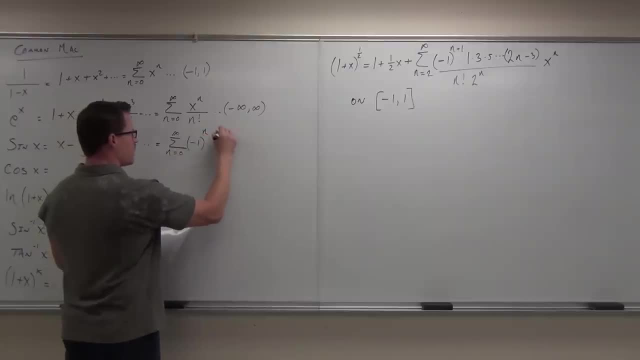 It was alternating obviously x to the odd 2n plus 1, over 2n plus 1 factorial And it converged for all real numbers x. Does that one look familiar to you? Yeah, We did it yesterday. 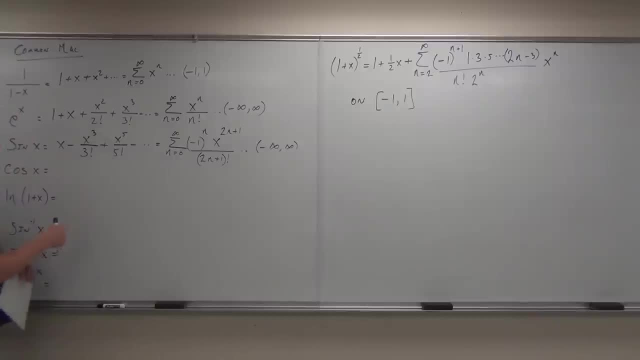 We did, Oh, perfect, So it looks familiar. Cosine. This one was really easy. Cosine was just the derivative of sine. 1 minus x, squared over 2 factorial plus x to the fourth over 4 factorial minus blah. 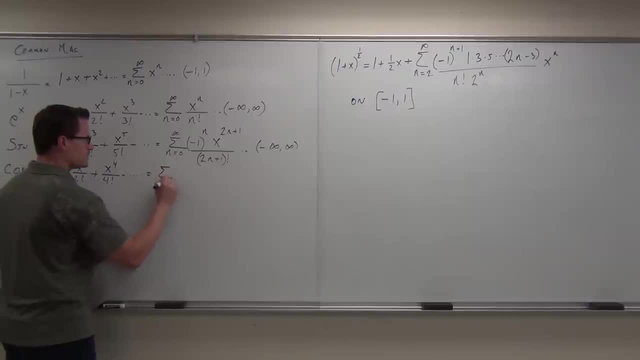 blah, blah blah. We said: hey, it's still alternating. It's now x to the even numbers, Even numbers over even numbers, factorial, And it converged from negative infinity to infinity. Oh, that's the last thing we did. 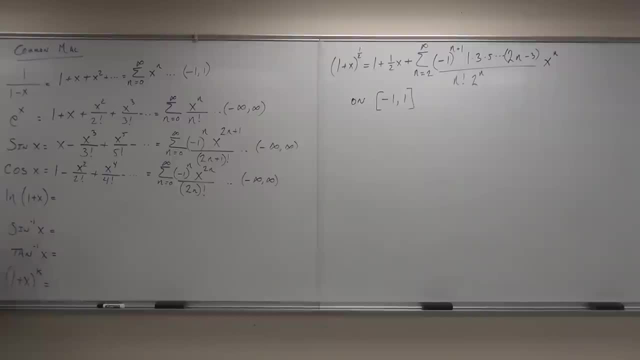 That's right, OK. ln of 1 plus x. ln of 1 plus x. We have x minus x squared over 2 plus x to the third over 3, minus x to the fourth over 4.. I don't remember if we did this one or not. 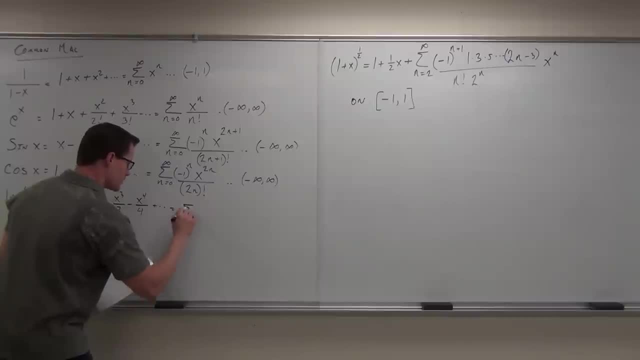 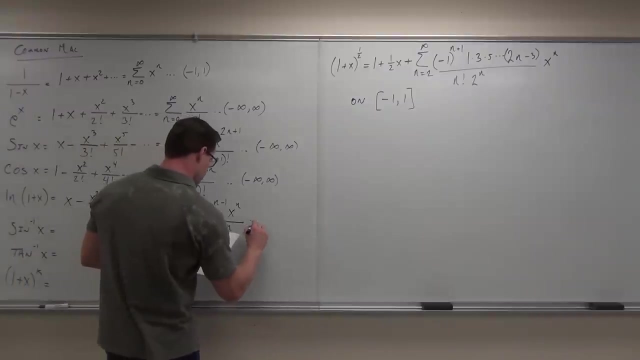 This is the series from n equals 0 to infinity. Negative 1 to the n minus 1.. x over n, all over n, And you can see that right here. It's kind of a nice one. This converged on negative 1 to 1.. 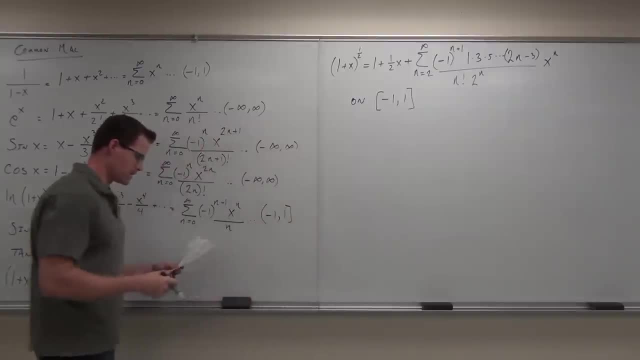 Positive 1 was included. Negative 1 is not included. You know, I'm probably going to do the last two over there, just to be clearer. Sine inverse of x- We would have, x We would have. no, we have not done this one, OK. 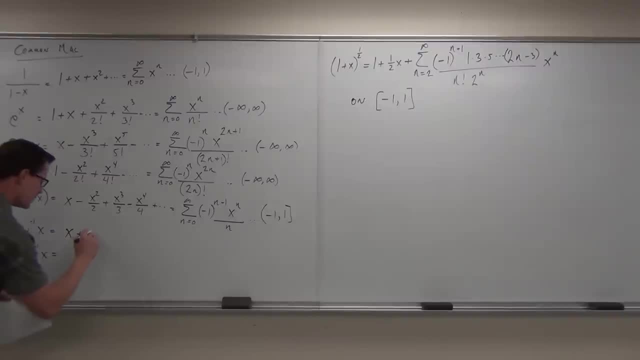 I'm just giving this to you, so you have it. We actually do x cubed over 2 times 3.. We would do 1 times 3 x to the fifth over 2 times 4 times 5.. And what this ends up being is a series which is quite interesting. 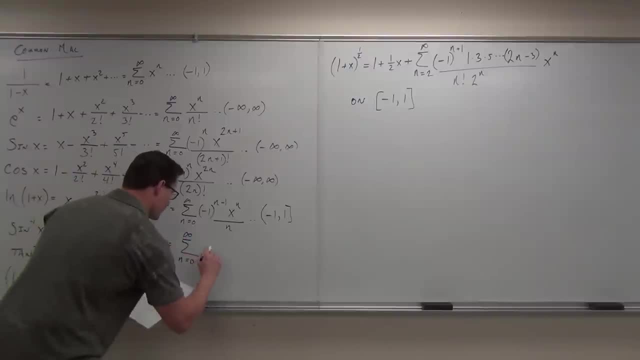 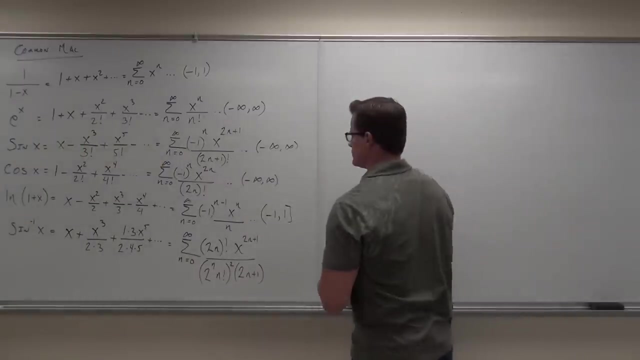 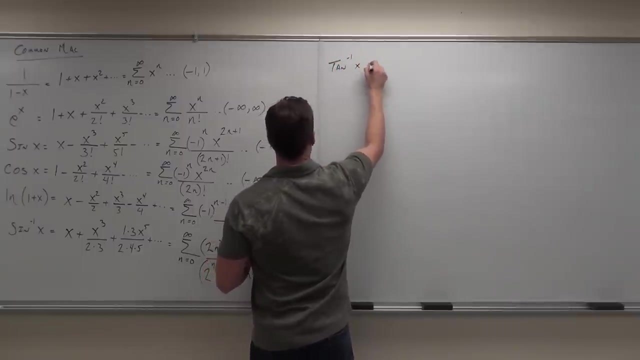 We start at 0.. We go to infinity. We have 2 to the n factorial, x to the 2n plus 1, all over 2 to the n n factorial. squared times odd numbers, These ones are going to be 10. inverse of x is this: 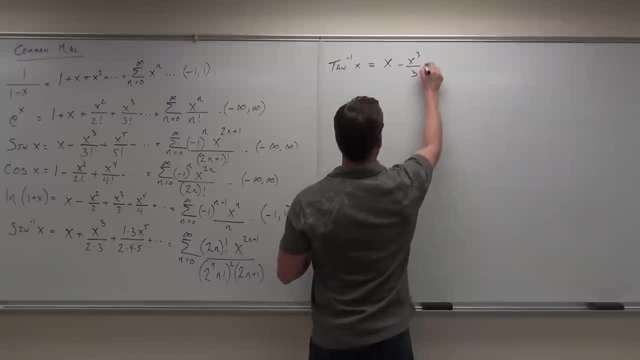 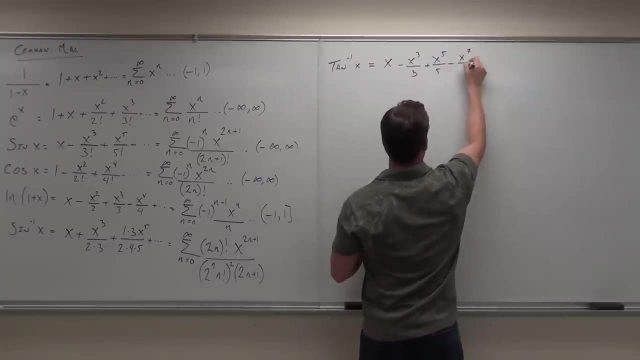 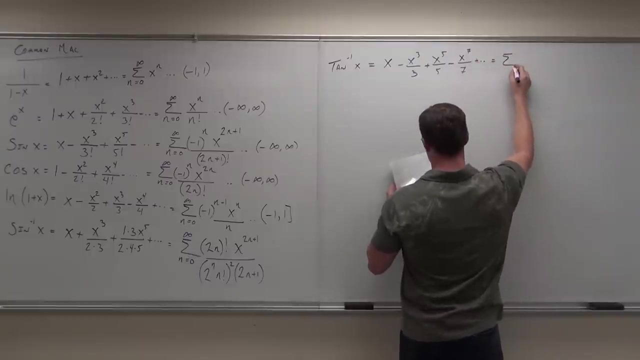 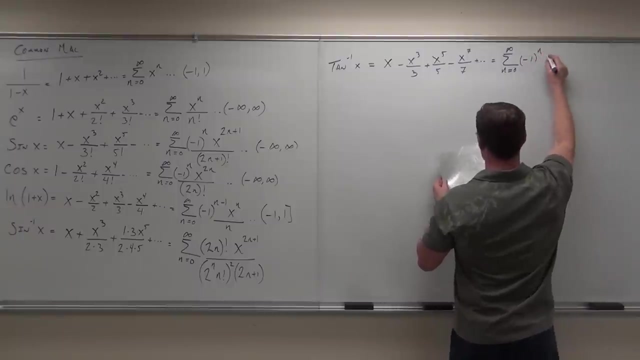 x minus x cubed over 3, plus x to the fifth over 5, minus x to the seventh over 7.. Or in other words, it's an easy one, Looks nice, at least We get alternating. We get x to the odds over odds. 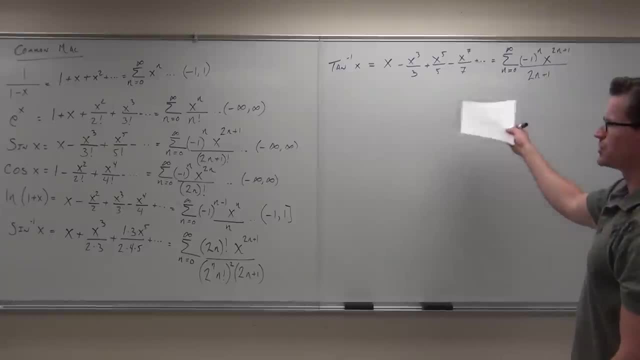 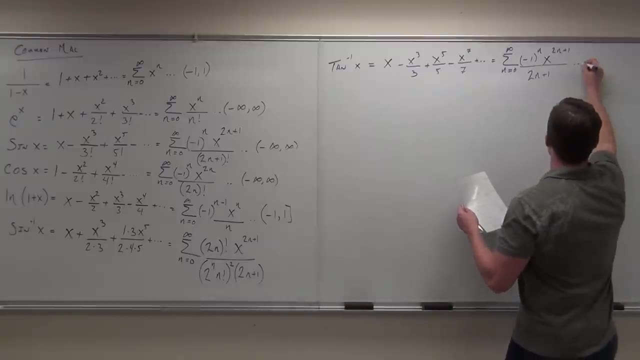 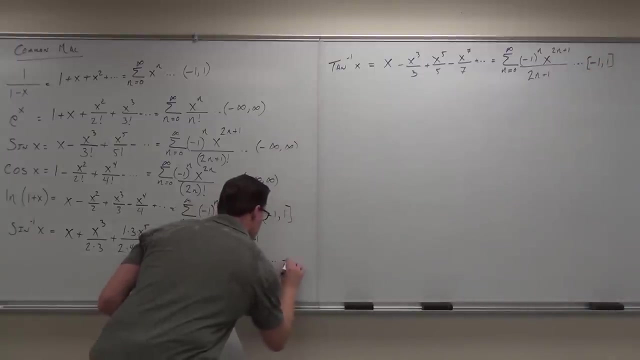 Do you see how similar tangent inverse is to sine inverse? It's really similar, except that's a factorial. Really similar, though It's interesting. And tangent inverse only converges on negative 1 to 1. Inclusive, And so does sine inverse. 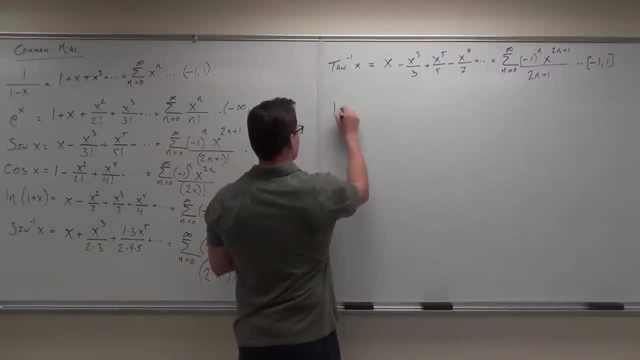 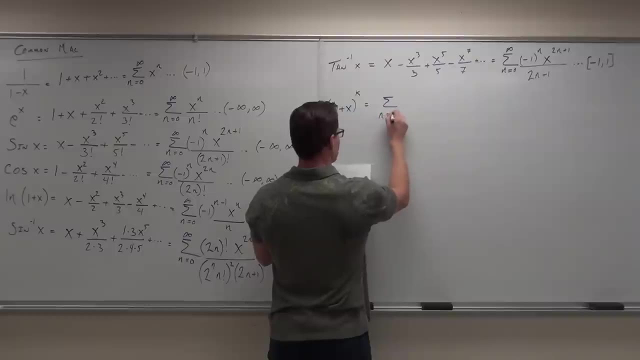 OK, Last one. We just did it. If you have 1 plus x to the k, this thing is equal to the series. We just showed it. n equals 0 to infinity. I'm not going to go through it again. 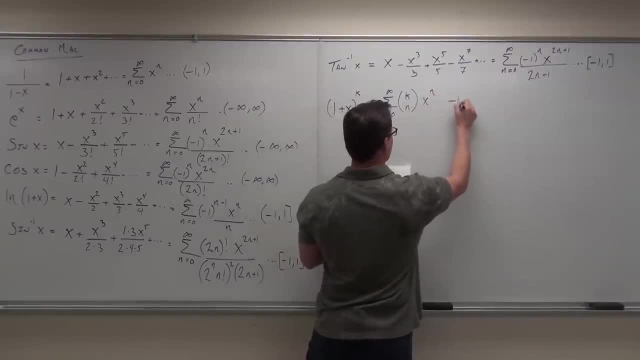 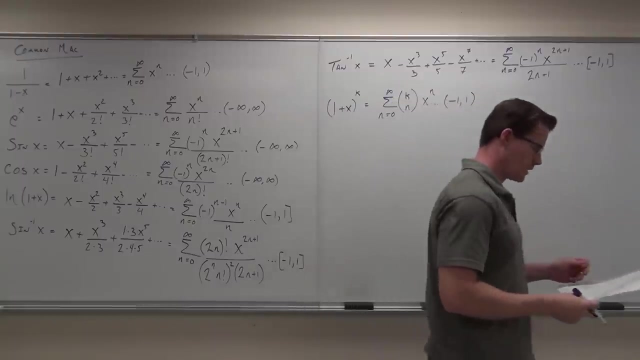 Binomial coefficients times x to the n And it converges on negative 1 to 1.. Converges on negative 1 to 1.. If k is- and there's special cases- If k is a positive integer, it's all real numbers. 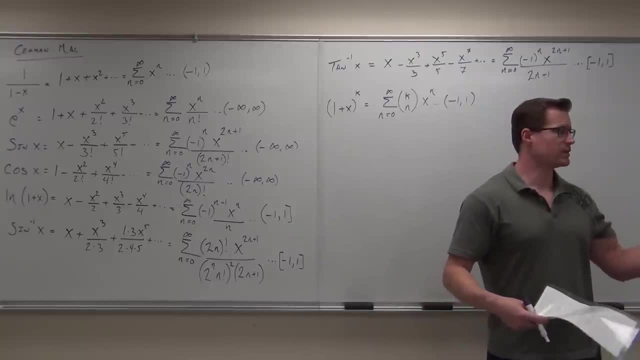 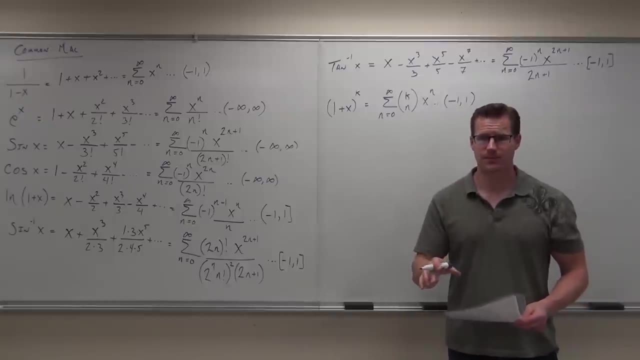 If k is between 0 and negative 1, then we get 1 included. If we get above 0, then we get both n points included. So there's special cases there. Now here's the point. Let me make sure I got all these right. 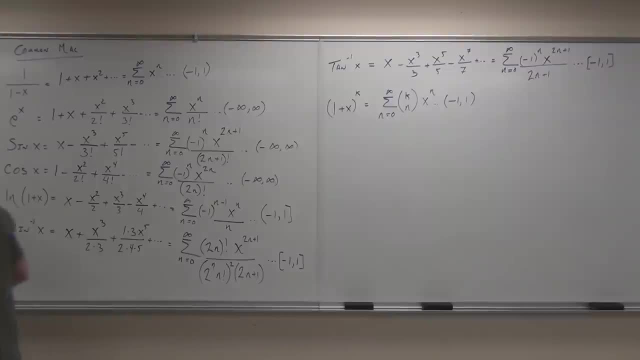 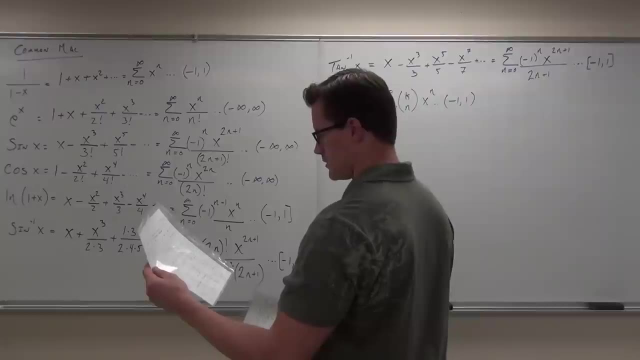 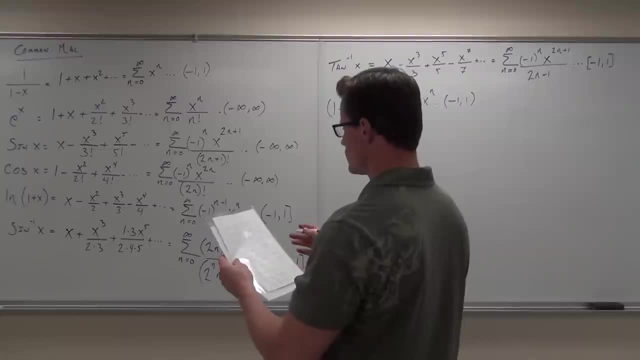 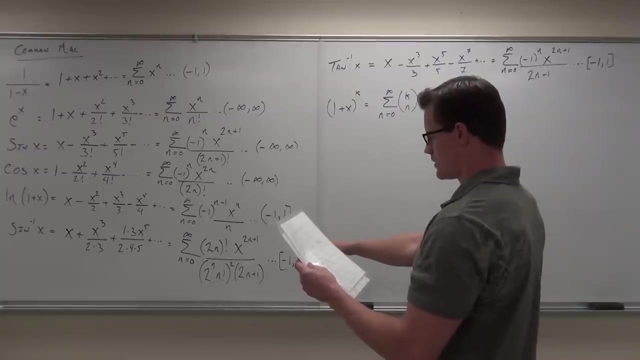 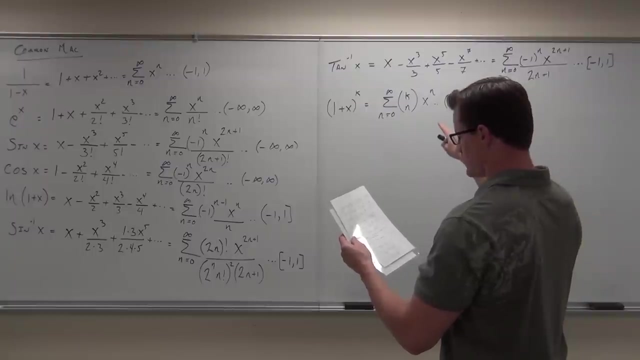 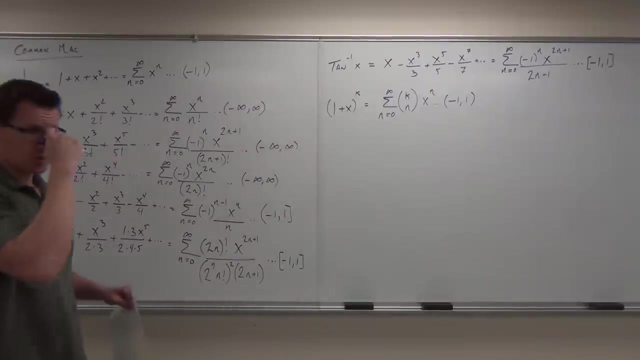 Cosine inverse. That looks good. Perfect, Got it. Thank you, That one's so nasty. All right, Now here's the whole point. The point that I'm going to make here is that you can manipulate functions that you're given to fit these forms. 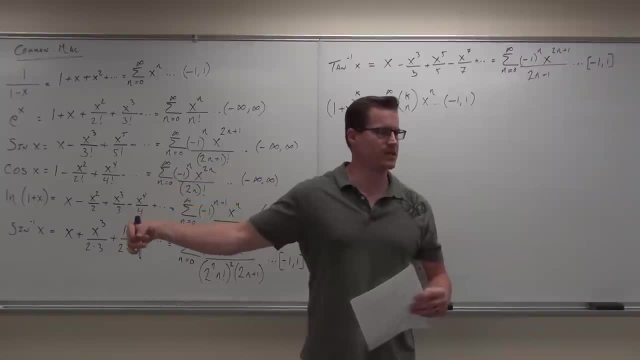 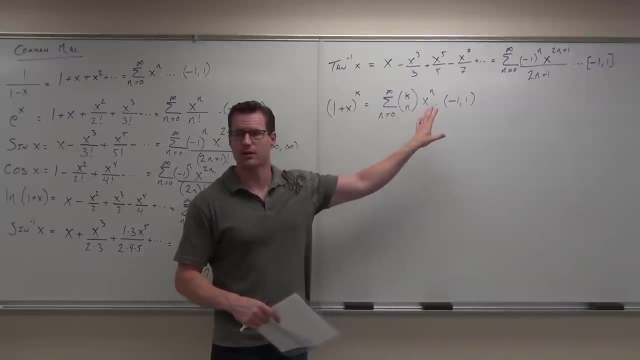 And if you can do that, then you don't have to reinvent the wheel. basically, You don't have to start from scratch on these problems. Have you written this down? Because I'm going to erase it here real quick, Because I need to start here. 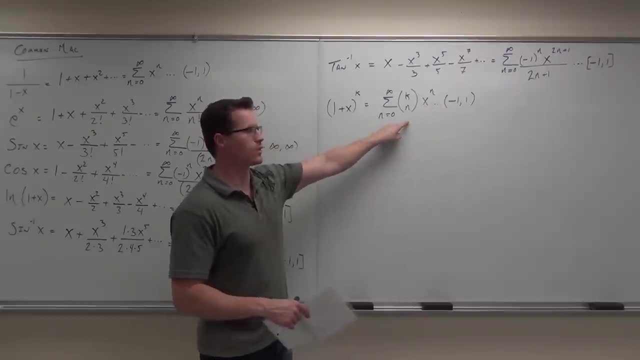 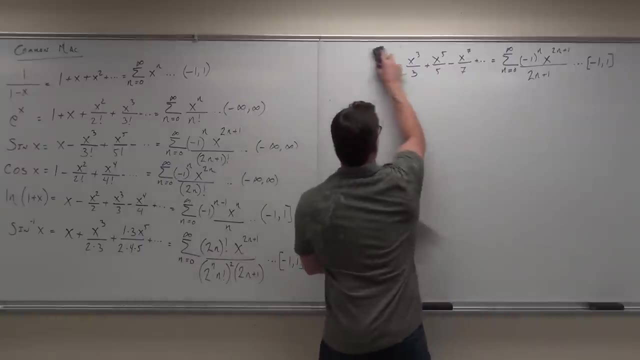 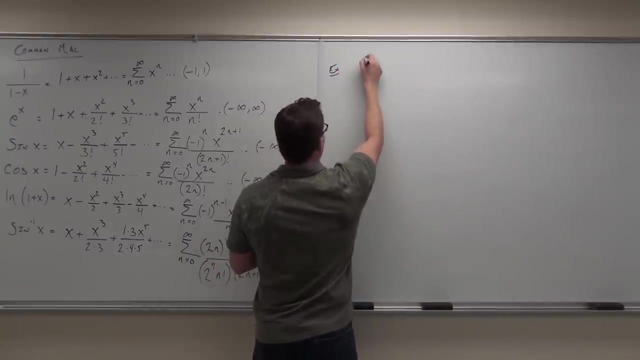 Do you have it? Yeah, This one you already have, So just worry about that one. Can I erase it? Yes, No, Yes, OK, Good, For example, let's say, I give you this function on your test, which I'm going to do. 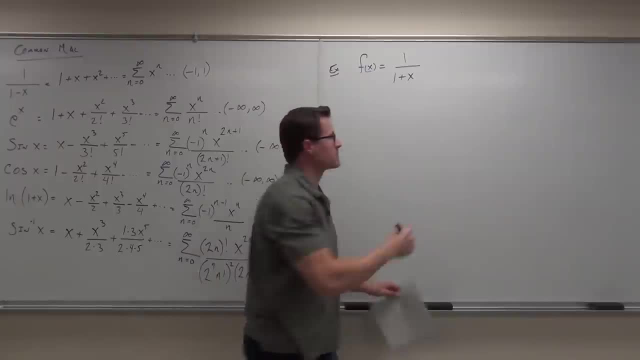 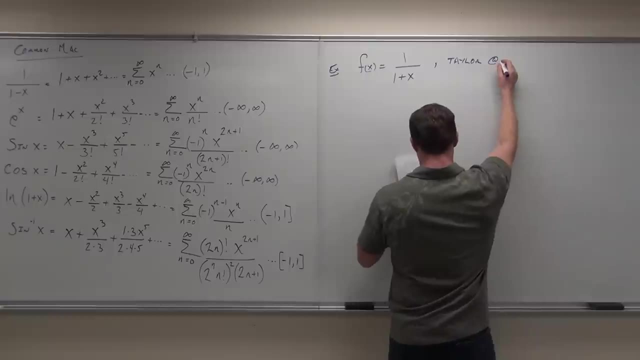 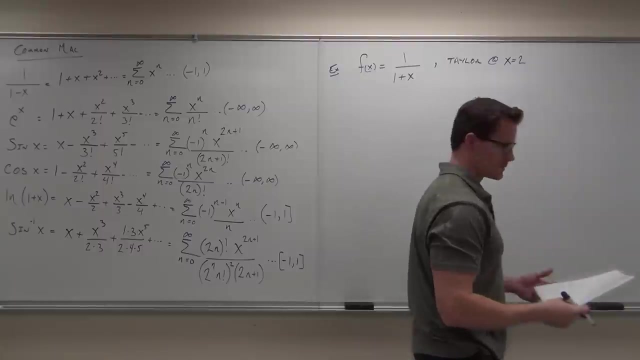 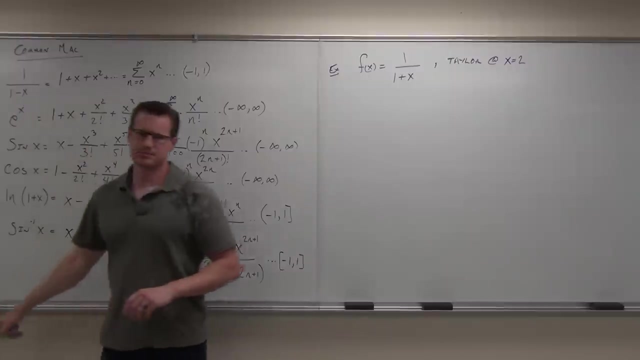 And I say I want you to find the Taylor series at this point. So I want Taylor at x equals 2 or c equals 2.. And we'll go for it. Now here's how to diagnose the problem: If you're going to have a Taylor polynomial or not a Taylor polynomial. 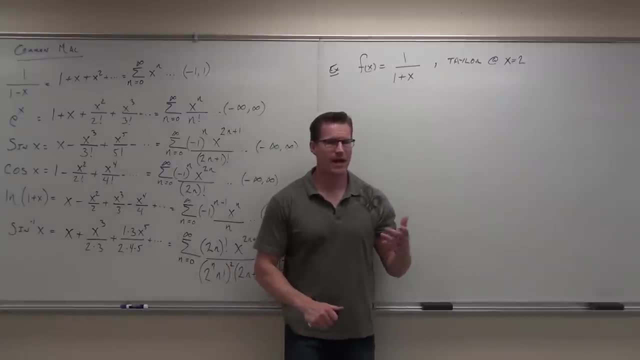 I'm sorry I'm skipping ahead. You're going to have a Taylor series at the point x equals 2 or c equals 2.. What that means is that somewhere in your series you are going to have x minus 2.. Does that make sense to you? 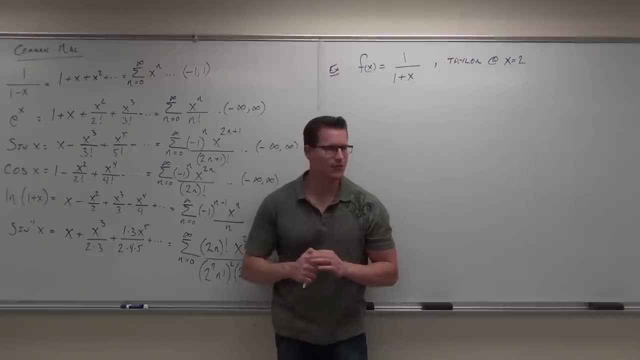 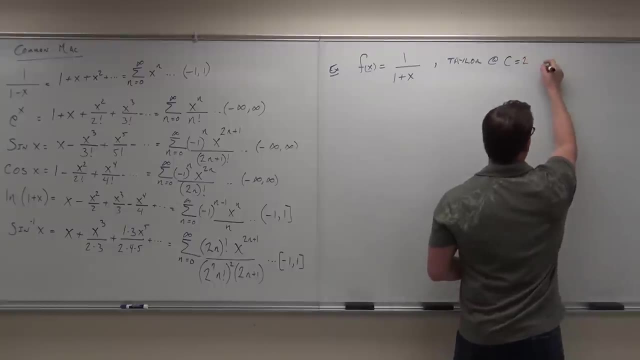 No, I can tell by the blank looks on your faces that you're like what? If you're going to have x equals 2 or c equals 2, whatever I want to say there- then you're going to have x minus 2 somewhere in your Taylor series. 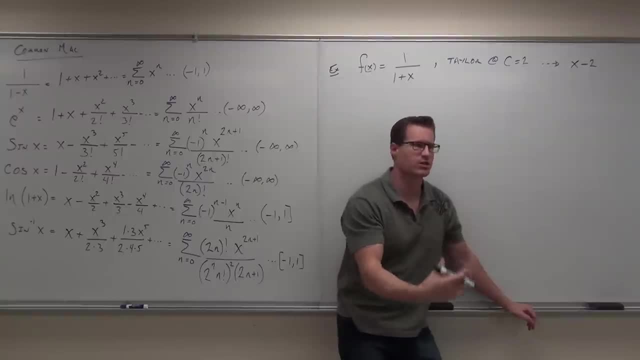 Your Taylor series says x minus c. Yes, You're going to have x minus 2 here if your c is equal to 2.. Show of hands, if you're OK with that one. OK, Here's what you need to do, Whatever your center is, if you have x minus 2, x plus whatever, sorry, c equals 2 or c equals whatever. 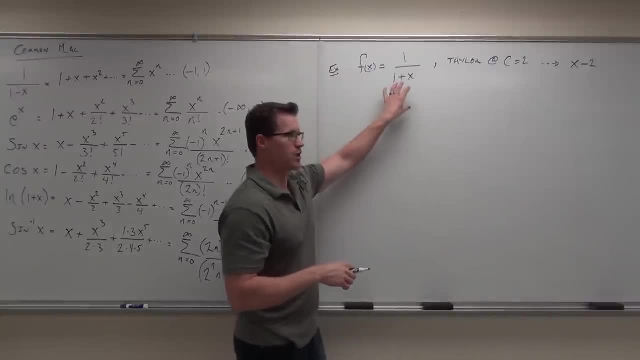 get x minus that number in your given function. You must make this up here somewhere. So what that is, what that means, is that I've got to manipulate this such that I find this, This in here. Are you listening? I'll show you. 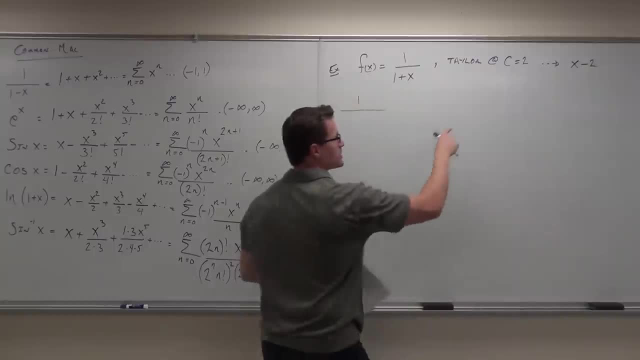 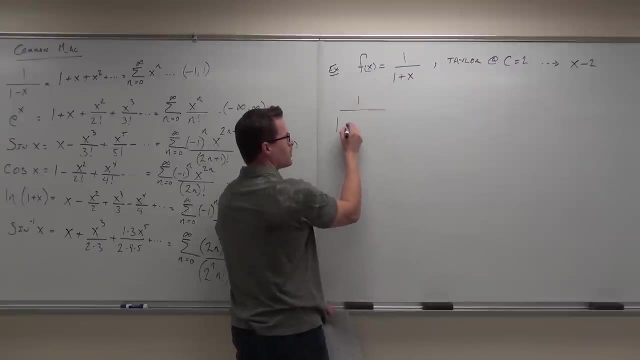 If you don't know what in the world you're talking about, I'll show you. OK, You've got to manipulate this to get my x minus 2.. So here we go, From 1 over 1 plus x. well, I think about it: 1 over 1 plus, I would do x minus 2,. 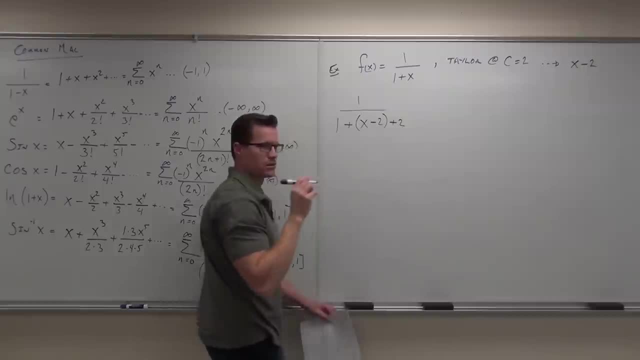 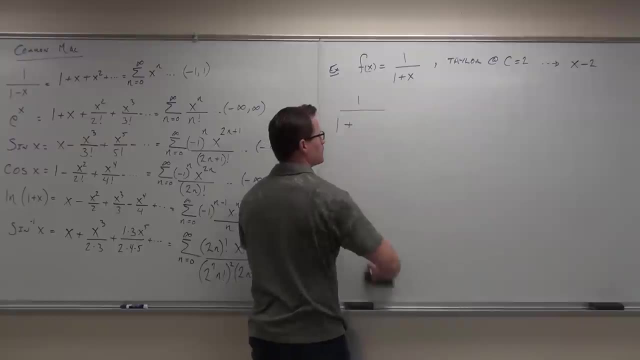 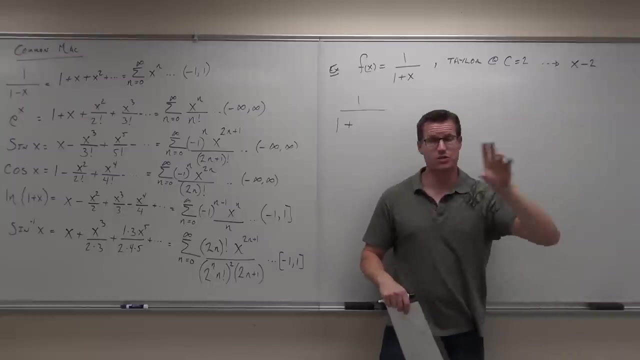 but then I have to undo it plus 2.. Can you follow that one One more time? I have this, I need this. So if I extend it to 2, I'm going to have to have an x minus 2 somewhere in my problem. 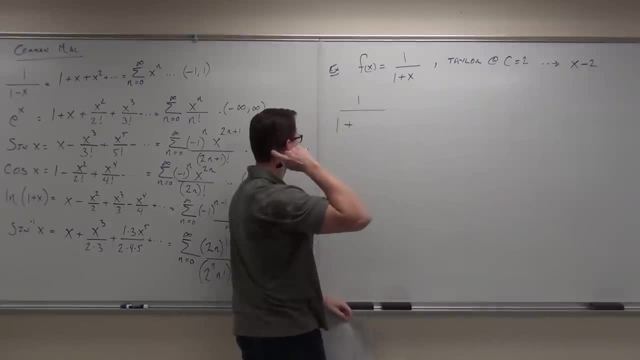 I have to have that. So my 1 over x, plus whatever. I'm going to say, all right, cool. Well, 1 plus x. no, I need an x minus 2.. That's what I need. Does that make sense to you? 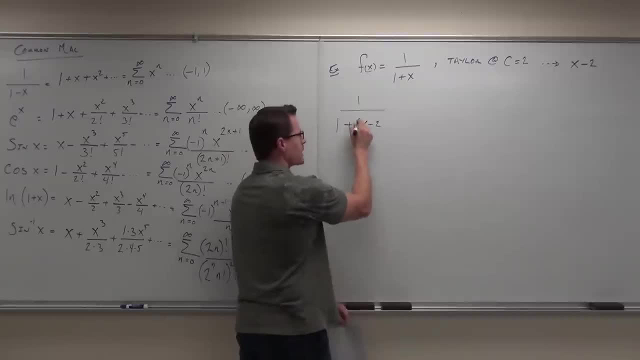 I can't just arbitrarily subtract 2 from my problem, though If I subtract 2, I'm going to have to add it back. It still has to equal this thing. Does this still equal that? Yes, Sure it does. Now let's simplify: 1 over 3 plus x minus 2.. 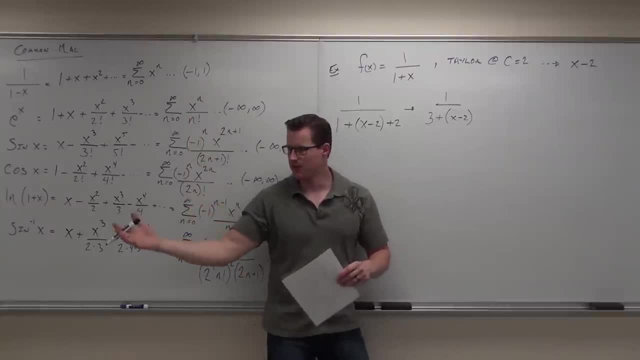 Quick show of hands, if you feel OK with that. so far Do you see that we have the same function. It's just we've made this piece in it. It's going to be Taylor series. It has to have x minus 2 up there somewhere. 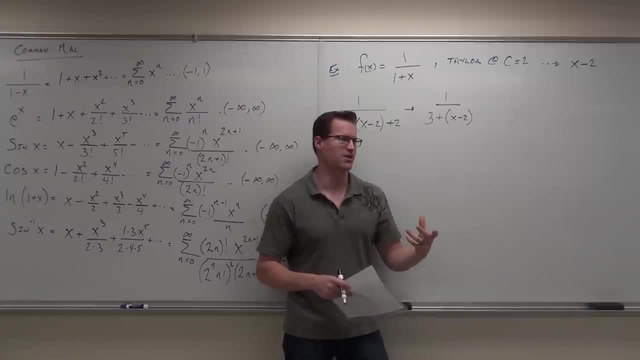 That's our center. You've got to find your center. You've got to be centered here. Now take this and actually look at this one. What does this most closely match out of all of these? Does it match sine inverse? No. 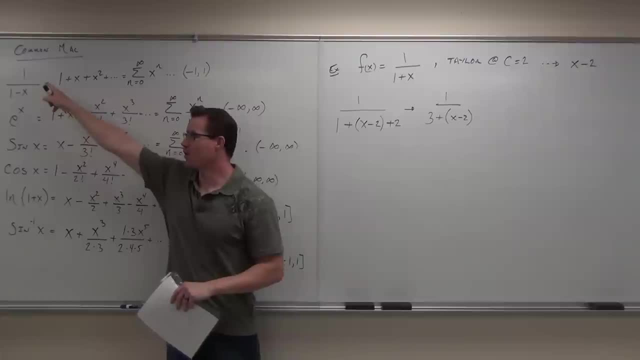 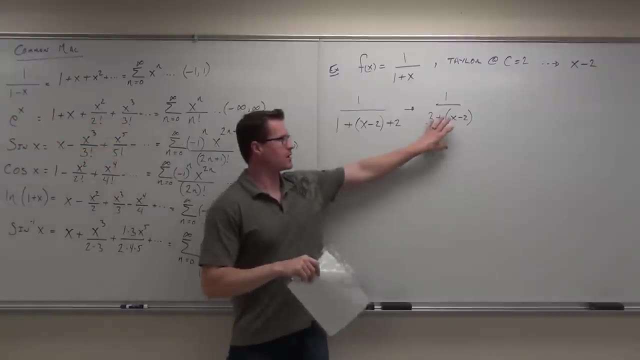 No, it doesn't. Does it match e to the x? No, Does it match 1 over 1 minus x? Yes, That's the closest. That's where we're going to try to fit it. So we need to make this thing fit, this thing. 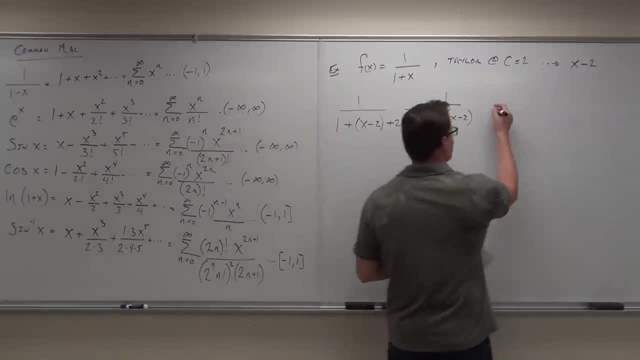 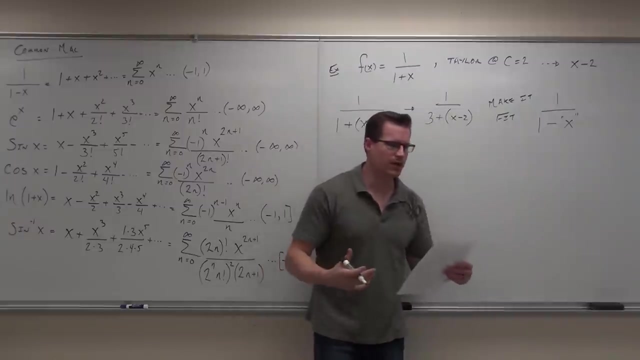 Now when I say fit this thing, we need to make it fit 1 over, 1 minus. I'm going to put x here in quotations. x. x stands for some quantity. It can be a really nasty looking thing, but it stands for x like whatever's there. 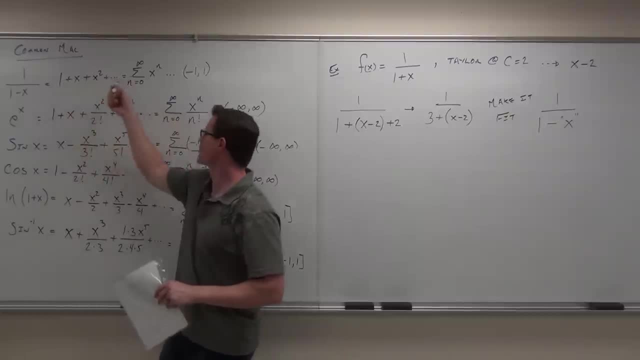 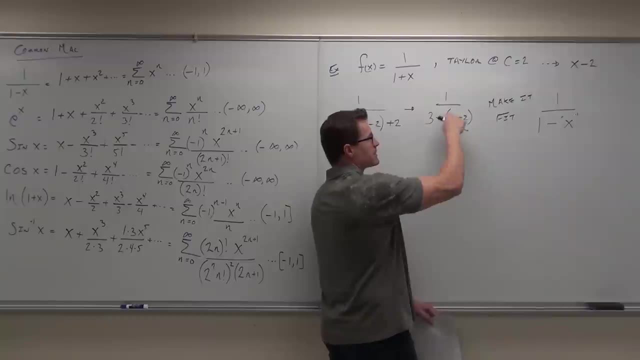 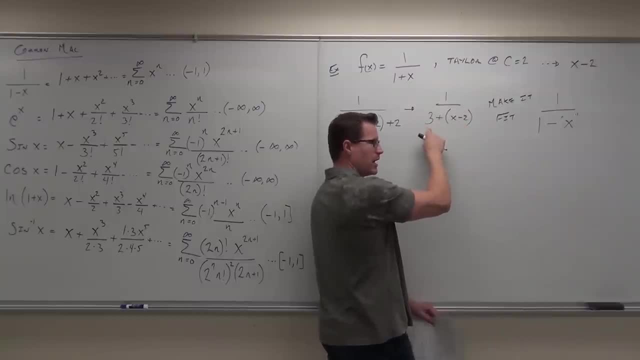 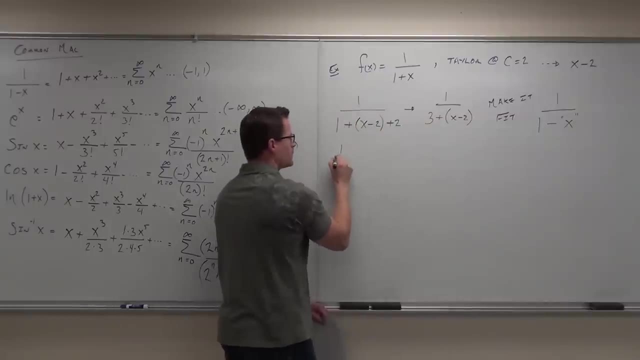 thing becomes a 1.. Can I do that? How do I do that Factor? If I factor out a 1 third? if I factor out a 1 third, I would get 1 third times 1 over 1, plus x over 2,, I'm sorry, x minus 2 over 3.. 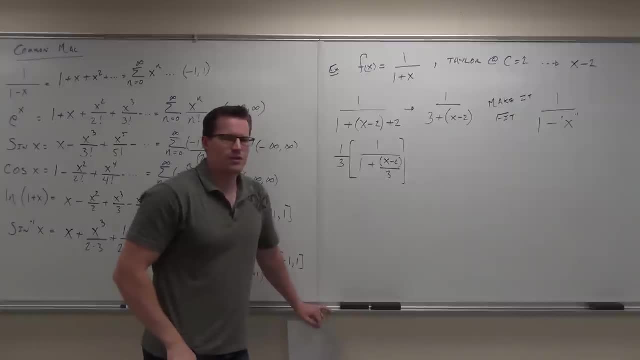 Can you do the algebra on that to make sure that that's okay with you? Yeah, Distribute the 3. Here's 3. Here's x minus 2. Do you guys follow? Yeah, Now, this is very close. 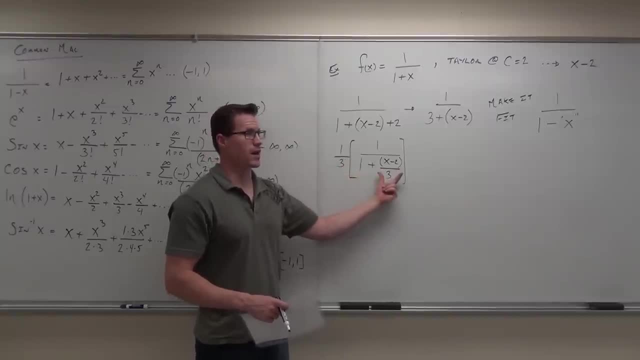 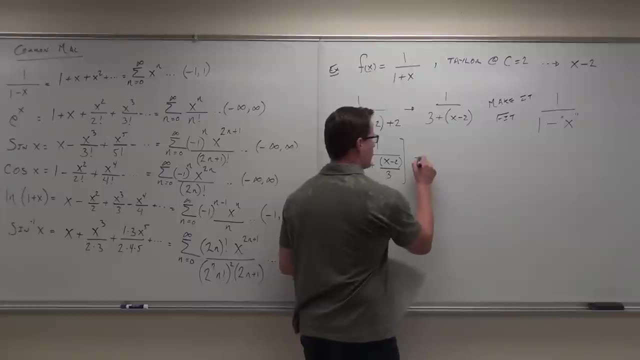 This is 1 over 1, plus something, some bunch of crap. okay, I want 1 over, 1 minus. I've got to change it to a minus. It's got to fit this. So I'll have my 1 third. 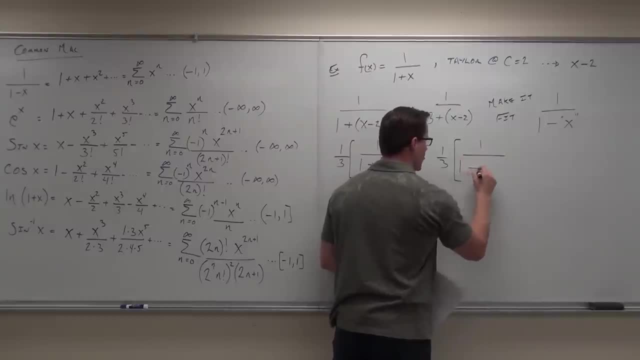 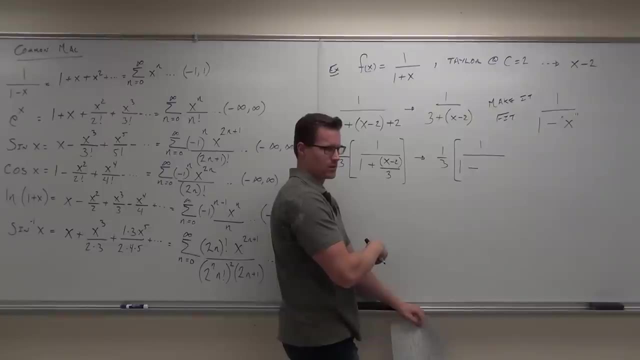 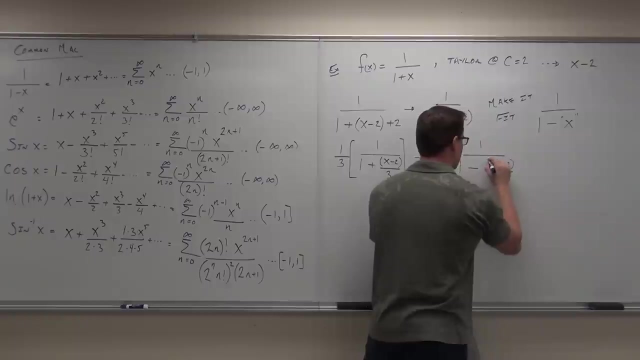 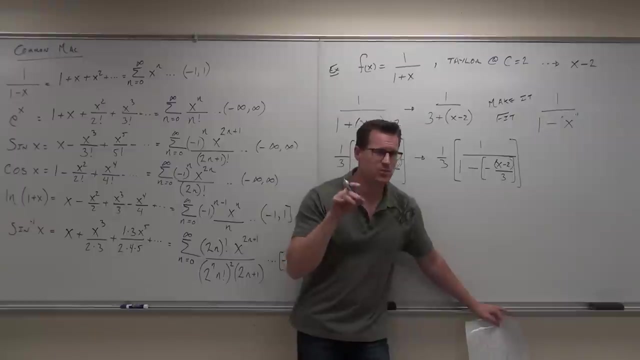 I'll have my 1 over, 1 minus, But then this: how can I make that minus? How can I make a plus equal a minus, something You can't do? negative x plus 2.. Explain me why you can't do negative x plus 2.. 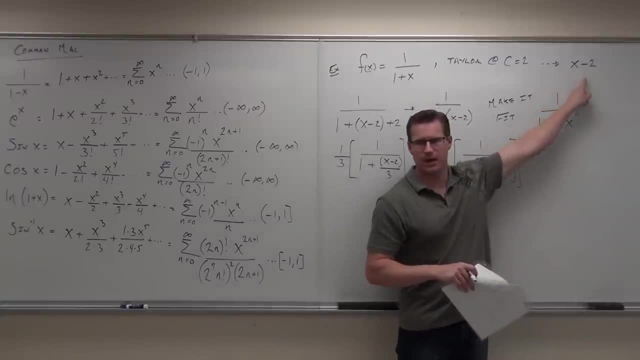 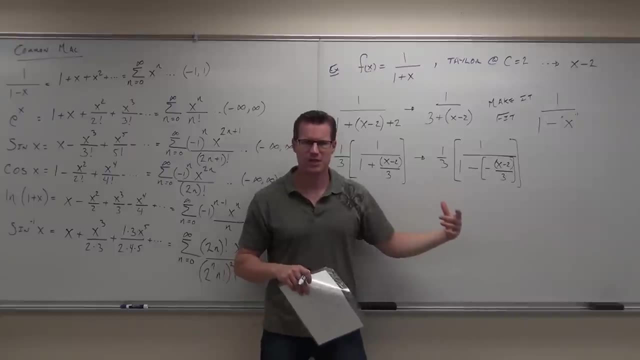 Boom, You have to have that. Does that make sense? So you've got to have that as your center. That's got to be there. It's okay. It's basic algebra. It really is basic algebra, But you feel okay with it. 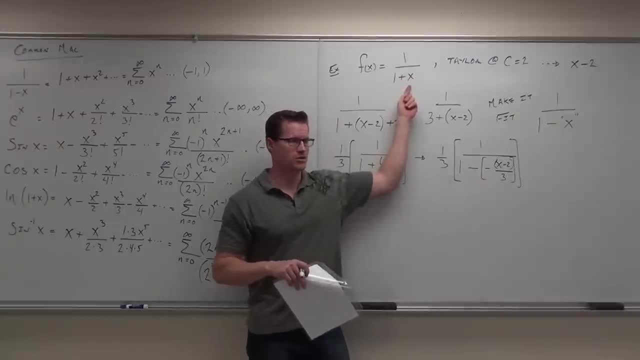 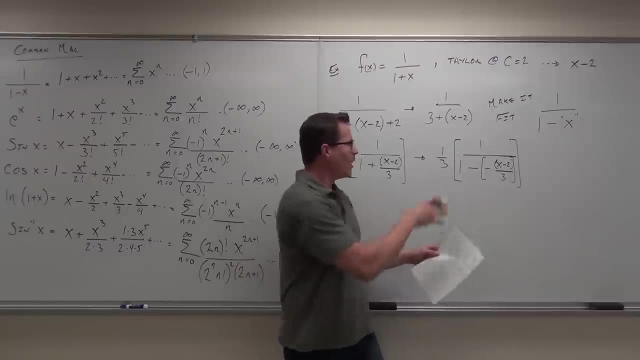 Is this thing, still this thing? Yeah, just nasty looking. Now here's the cool part. Okay, this is where the rubber hits the road. all right, This is what's awesome, What this really is. yeah, it's 1 third. 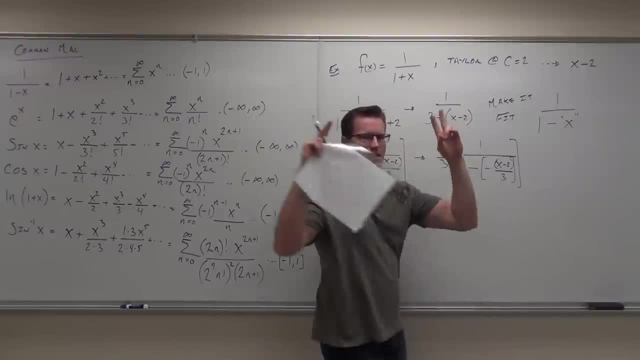 But inside here, do you see, it's 1 over 1 minus x. It's just our x, our junk. is this junk? That's our junk. Are you sure you're okay with it? Do I need a 10-second recap to go over it? 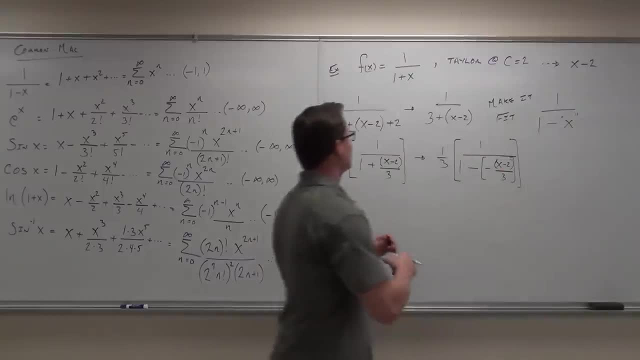 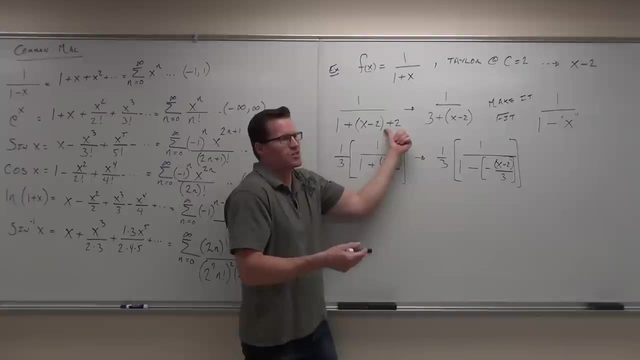 Are you sure you're okay? Yes, Some of you don't look. okay, Make this here, because that's our center. If it's 2, you've got to have x minus 2.. Put that up there. Yeah, you've got to add 2 to it. 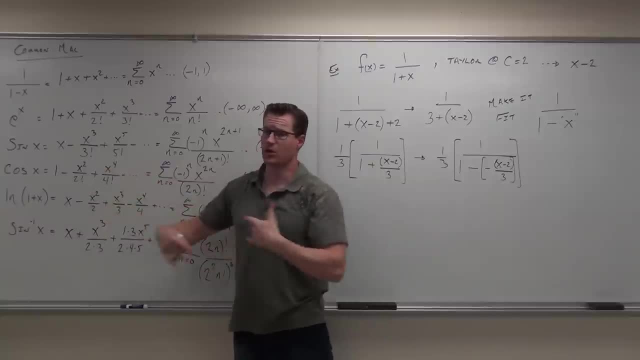 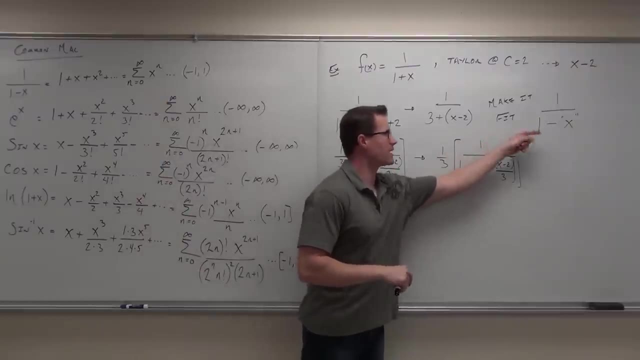 Simplify it, Make it fit one of these things. In order to do that, we need 1 over, 1 minus junk. x is your junk. Okay, if I need 1 over, 1 minus junk right now, I don't have it. 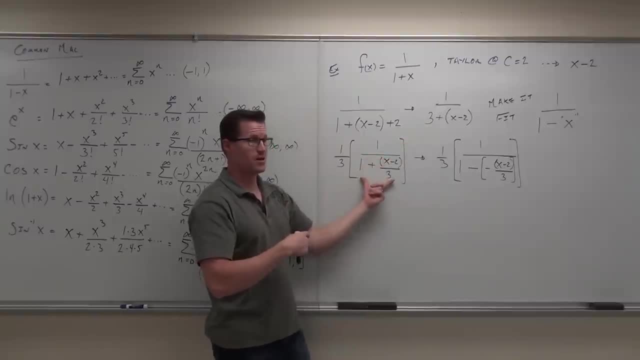 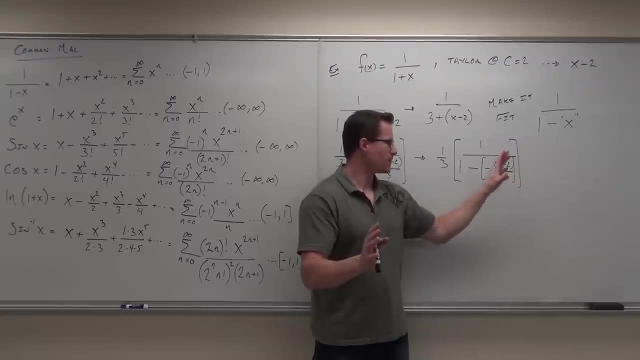 Make this a 1. Divide by 3.. Got it. Make that a minus, Split off a negative. Now, I got it. Now it's 1 over 1 minus junk. Cool, Cool. Take this thing, fit it to this stuff and then see what happens. 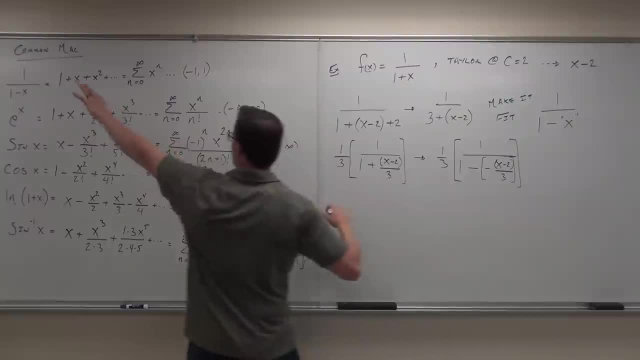 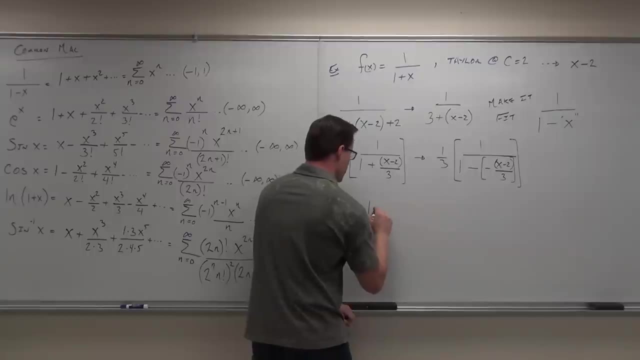 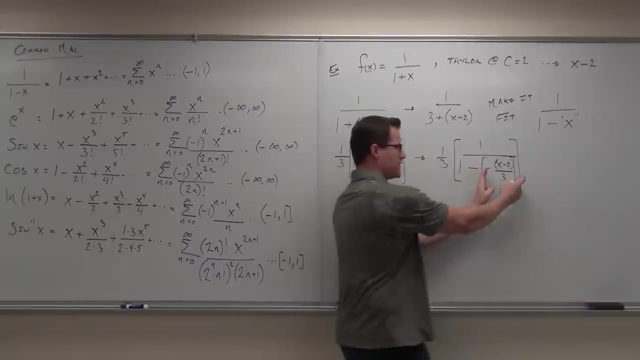 So if we see what happens here, we're going to fit it to this formula. What's our formula? start with 1.. Yep, The next thing we have in our formula is what x. Notice how x is the junk, This is the junk. 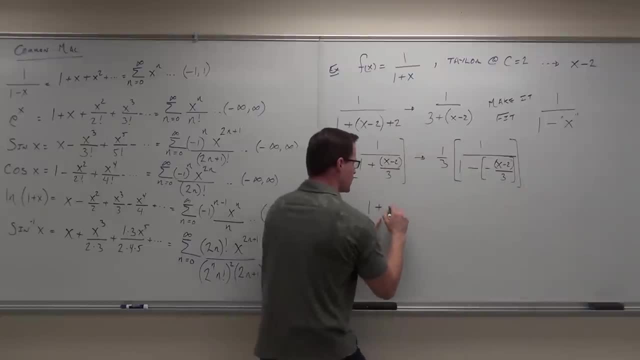 You sure You okay with that? Yes, So 1 plus, we have negative x minus 2 over 3.. So far, so good. Are you sure you're okay? I don't want to leave you behind here, because this is very important for us to know. 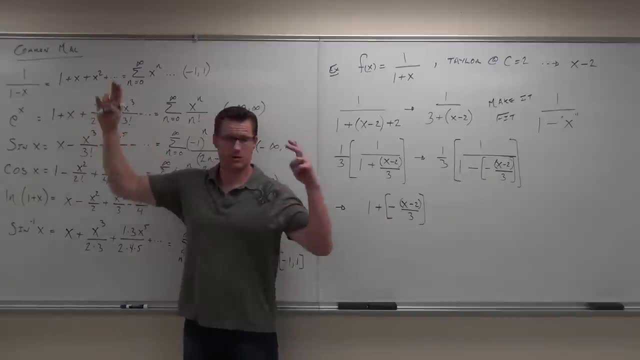 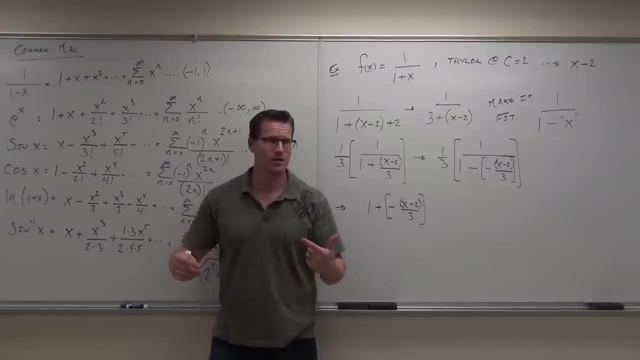 We have 1.. We've got 1.. We've got junk. Here's junk. Put your junk. Next thing we do: Junk squared, Junk squared. Yeah, junk squared. What's in between there? Junk squared, What's in between there. 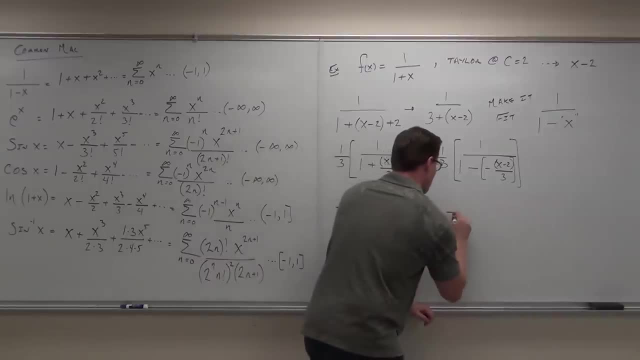 Plus What's in between there, Plus, Okay plus. I don't like to say the whole thing. So yeah, junk squared Minus 2 over 3. Whole thing Squared Plus. Let's do the next one and then we'll stop. 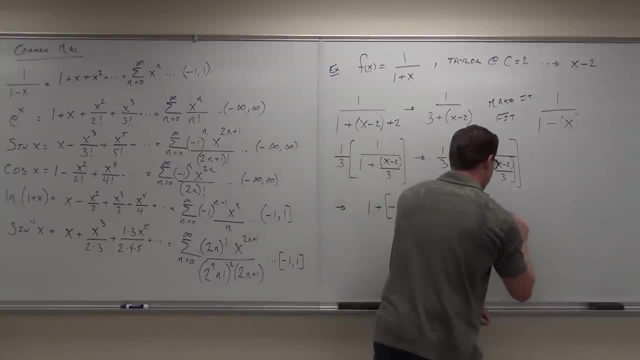 What's the next one? Plus Junk, Plus Junk Q, Q, Plus Blah, blah, blah blah. We're going to go forever and ever and ever. Okay, I need a show of hands If you think that you can make it from here to here. 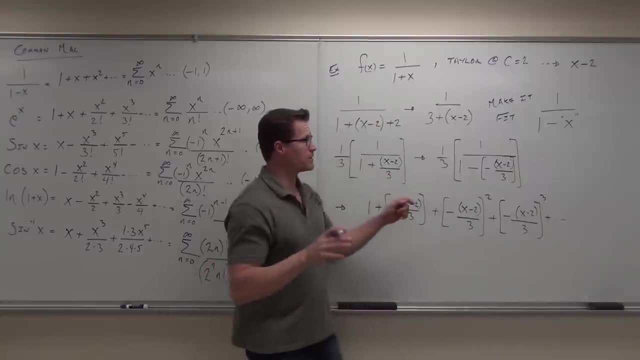 Okay, Okay, Okay Okay. If you think that you can make it from here to there, Show of hands. if you can do that, It's not that bad right. You just put the whatever your x is. This is the important part. 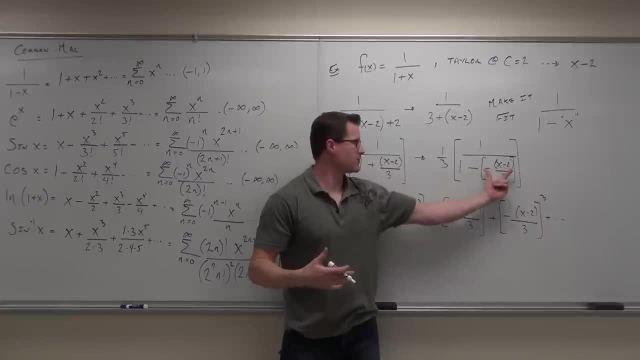 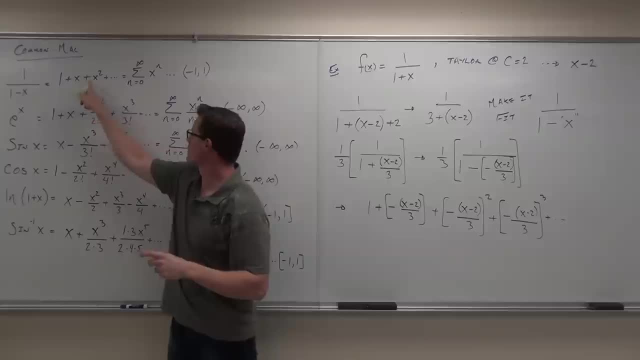 and then see what happens with your series. Now, there's one thing that we're forgetting. What are we forgetting? The one-third. The one-third is multiplied by all your stuff. Wowee, Don't worry about that, right? I forgot about that. 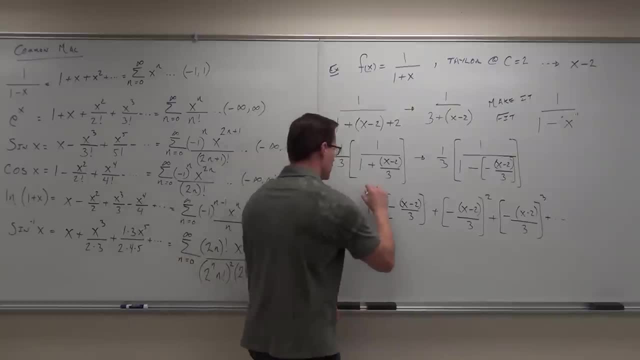 Don't worry about that, Okay, Okay, The one-third is multiplied by all your stuff. Wowee, Don't worry about that right now. I forgot about that. Don't worry about that right now. Anything wrong on the test? Yeah, 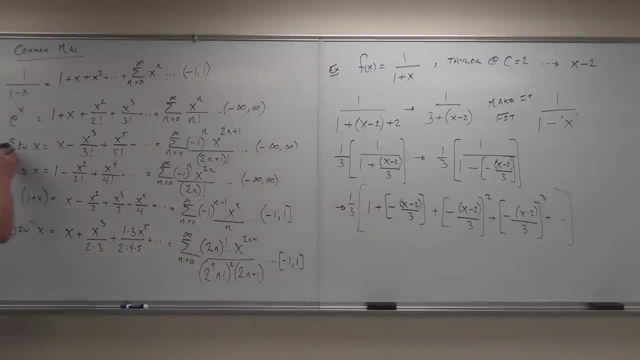 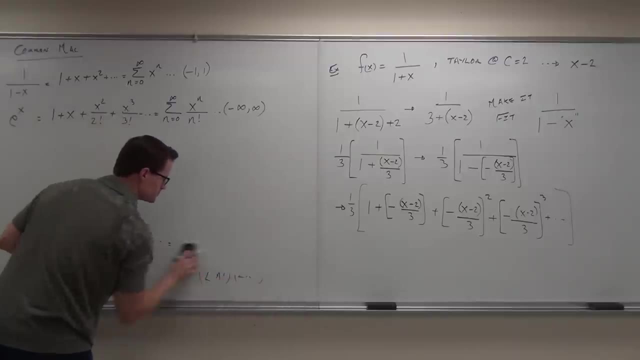 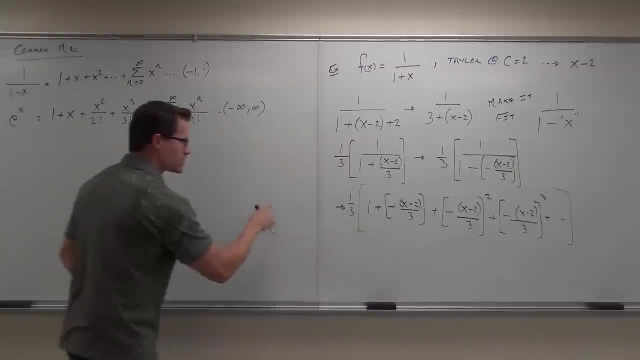 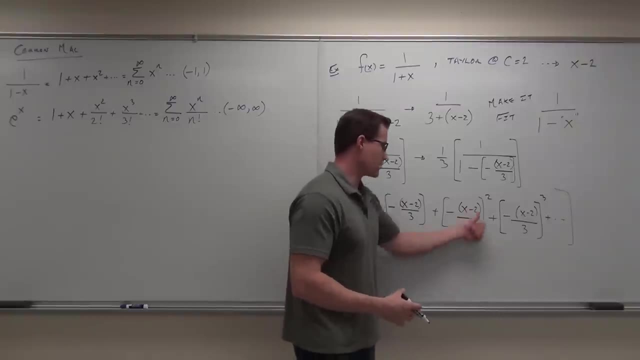 Okay, Okay, Let's keep on going. Let's take this, Let's simplify it. So if I take that and remember …. Oh man, remember, We are looking for patterns here, We're looking for patterns. So what I'm not going to do, I'm not going to go 9 and 27.. 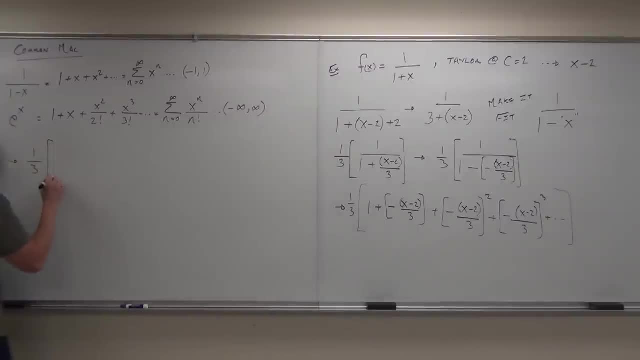 What I'm going to do is I'm going to keep the one-third. I'm going to do a 1.. I'm going to do a minus. So notice how that's a minus. We got x minus 2 over 3.. 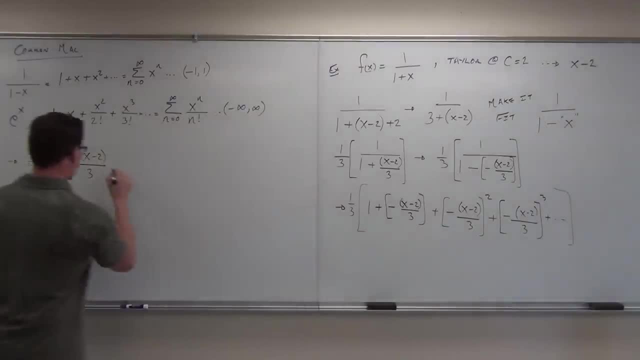 What's the next thing? we're going to have a plus or a minus Plus, we're going to have x minus 2 squared over 3 squared Yes, no, No, We're going to have a minus x minus 2 to the 3rd over 3 to the 3rd. 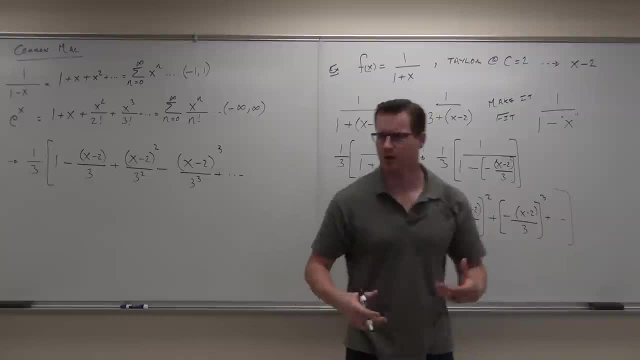 That is going to be a plus, And then so forth and so on. Can you make it down that far with me? Yeah, You see where we're getting the x minus 2 to the 1st and do the 2nd and do the 3rd. yeah, 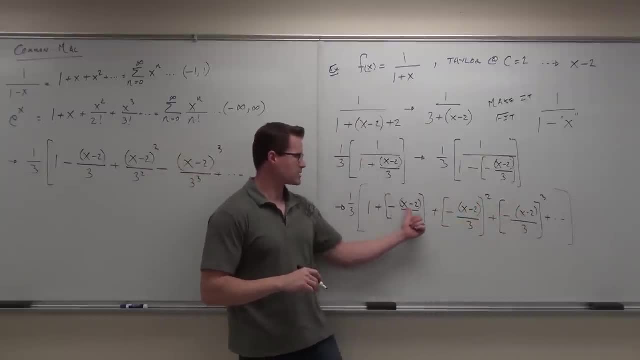 Yeah, We get to the 1st and do the 2nd and do the 3rd. We're doing positive- oh, I'm sorry- negative and then positive and then negative and then positive, And we have 3 to the 1st and 2nd and 3rd and 4th. 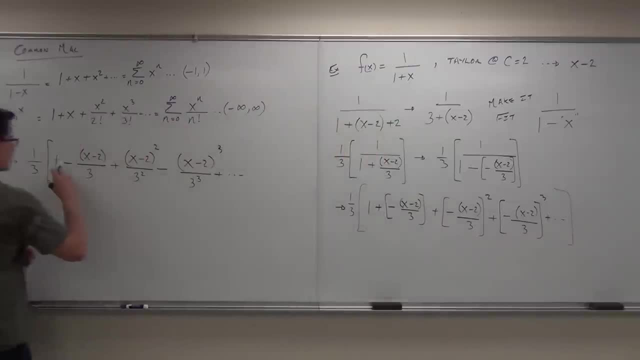 Now we're looking for a pattern here, So check it out. Let's fit this to our pattern. This is 3 to the what power Nope. this is 3 to the 1st. This is 3 to the aha that's going to give us our 1.. 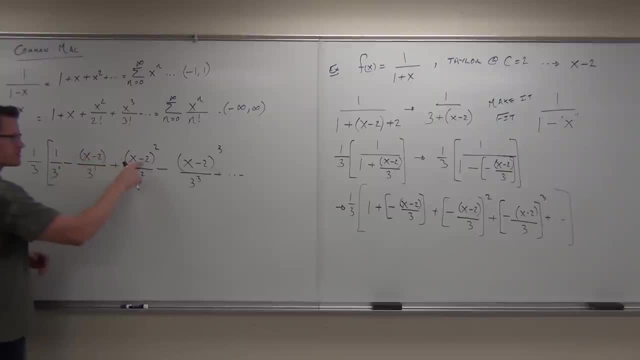 So we start with 1, x minus 2 to the 1st, x minus 2 to the 2nd, and then 3rd, We get 3 to the 0.. 1,, 2, 3.. 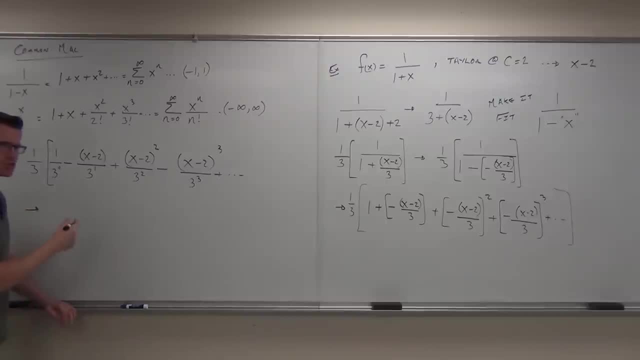 Can we go ahead and make a series out of this in series notation Sure, Here's how you do it. The 1- 3rd starts out front and you multiply it. Make this your series. Our series starts at n equals Zero. 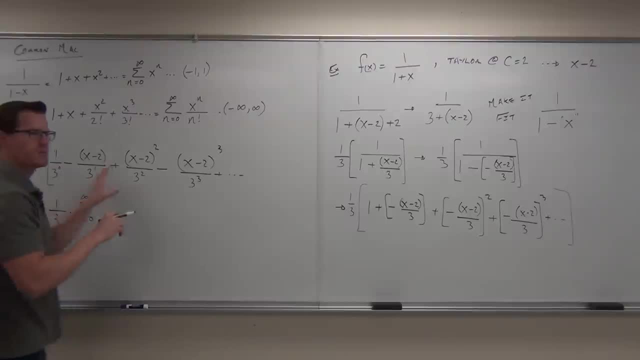 Good zero, It goes to infinity. Tell me something about this series that we know Alternating. Alternating: It starts with a positive, So we're going to have negative 1 to the n, Because that's going to start positive. 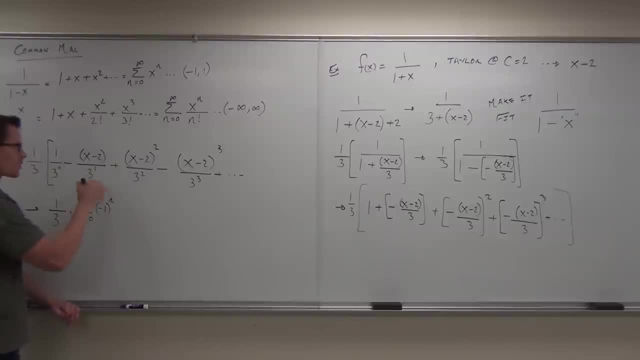 The next one would be negative, The next one would be positive. Does that make sense to you? Yeah, We're going to have x minus 2 to the n. Very good, All over. 3 to the n, 3 to the n. 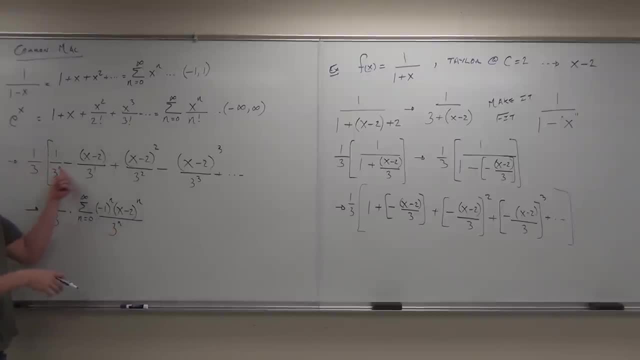 Perfect, You guys are getting it. Yeah, this is 3 to the n Hey, 0,, 1,, 2, 3.. Here's x minus 2 to the n 1,, 2,, 3.. 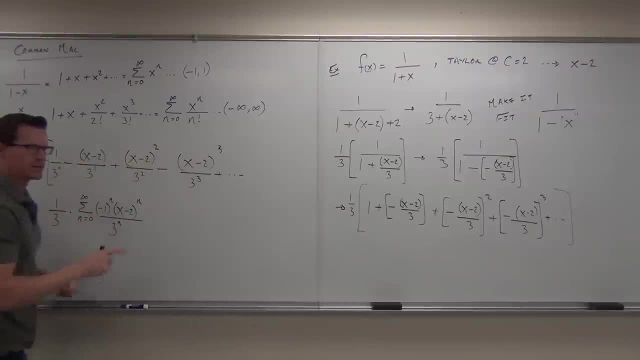 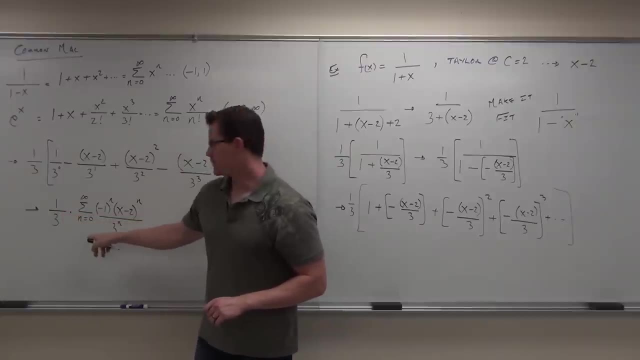 Here's starting positive and going alternating, No problem. There's one more thing we've got to do. It's very easy: Close, Take the 1- 3rd and move it inside. So if you have 1 3rd times this, do you understand? this is 3 to the 1st. 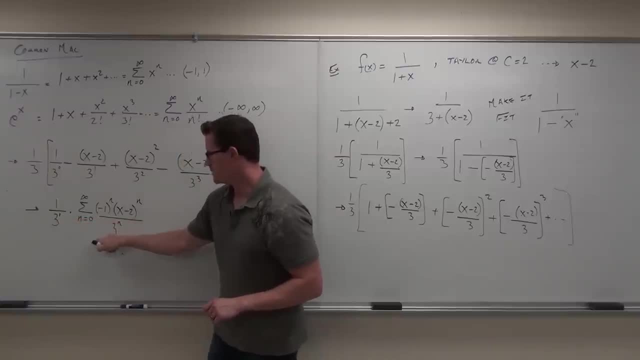 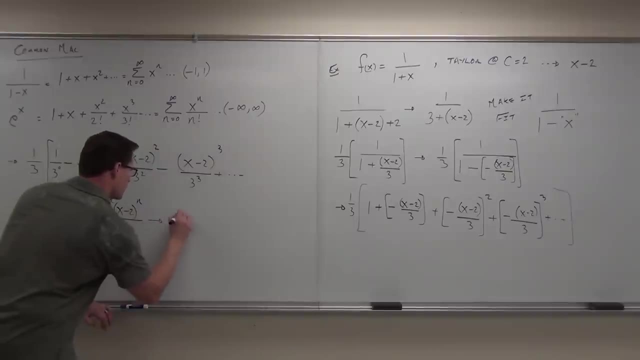 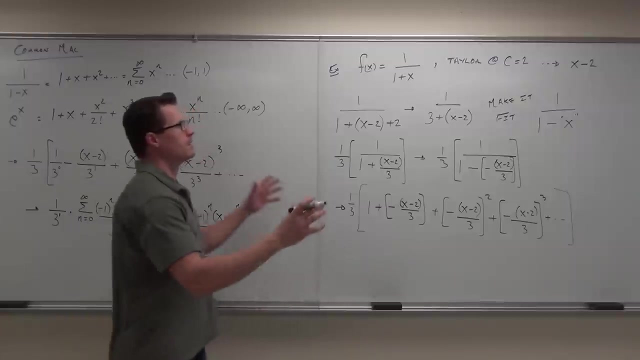 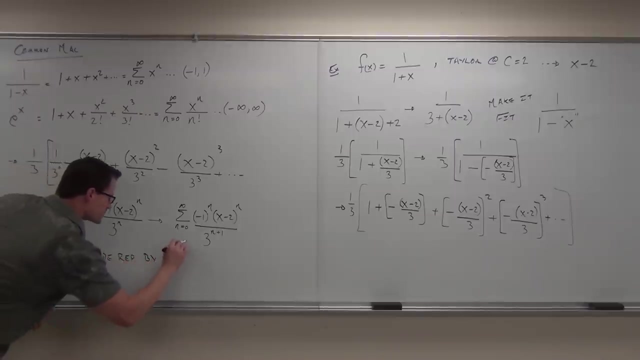 Yeah, If you have 3 to the 1st times, 3 to the n, you get 3 to the n plus 1.. Okay, Now wrap it all up. F of x equals 1 over 1 plus x can be represented by this on the interval. 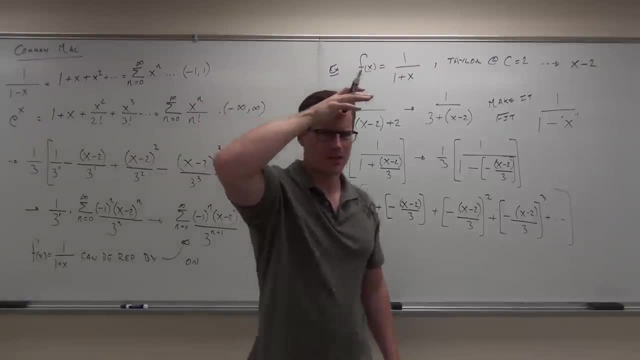 Oh, wait a minute. We've got all about the interval, didn't we? Do we have to check the interval? No, No, It's already been done for you, which is why we use these things: No ratio test, No end point test. 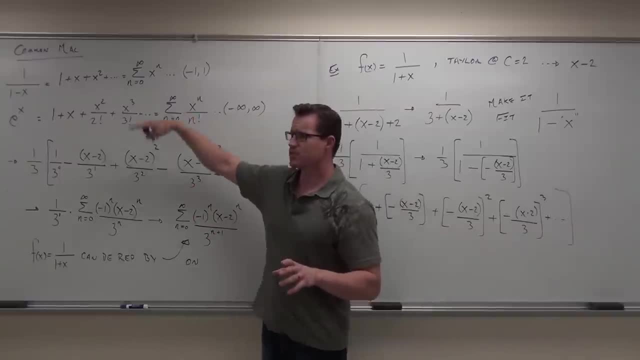 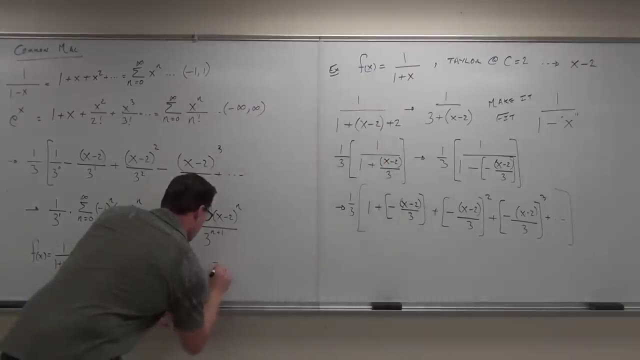 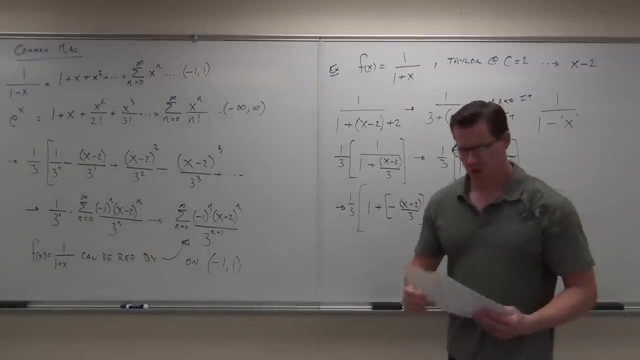 No, nothing. Look at the board. Which series did we use? What's the interval of convergence? The 1 to 1.. Same thing here. Pretty cool, right, You can make them fit. This is one of the harder ones that you're going to do. 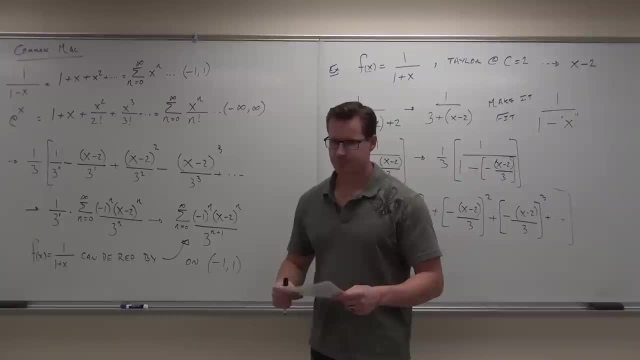 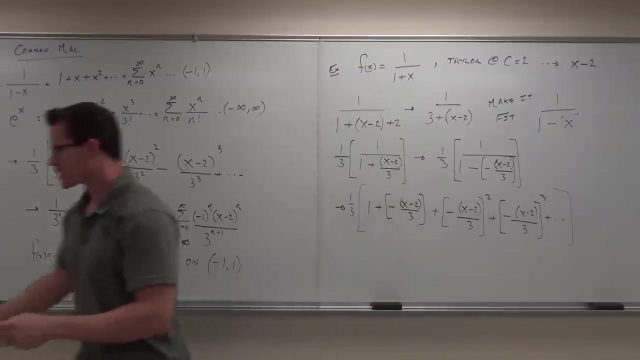 Now we're almost done with it. Almost. I kind of lied a little bit. This would work if your x was just x, but keep in mind, don't stick with me here for just a second. okay, This would work if your x was just x, but your x that you used here is your junk, okay. 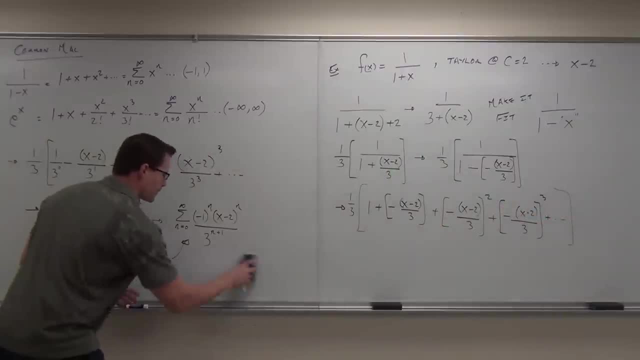 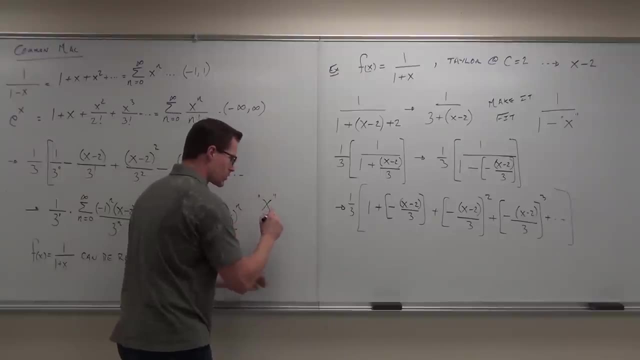 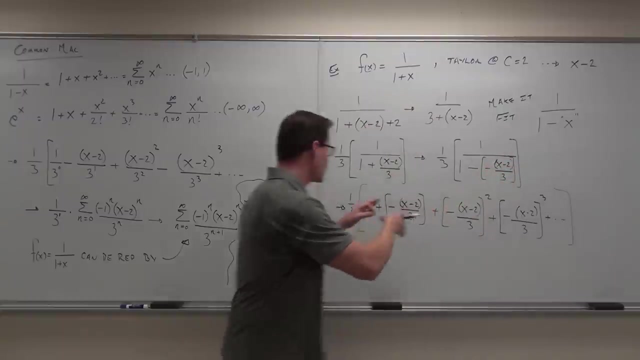 So we have one more thing to do: Remember that your x, Your x, works between negative and positive, Negative and positive, Negative 1 and 1.. Do you follow? Yeah, Okay, Just put your junk into where this junk is. 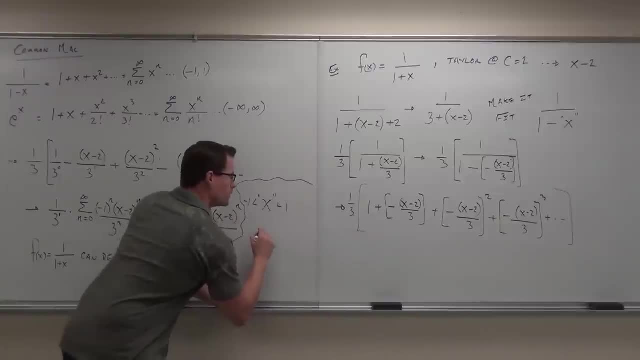 So what's your junk? Negative X minus 2 over 3.. Negative Negative. Okay, So negative x minus 2 over 3.. That's your junk. Multiply by 3.. Oh, wait a minute. What's negative? due to inequalities? 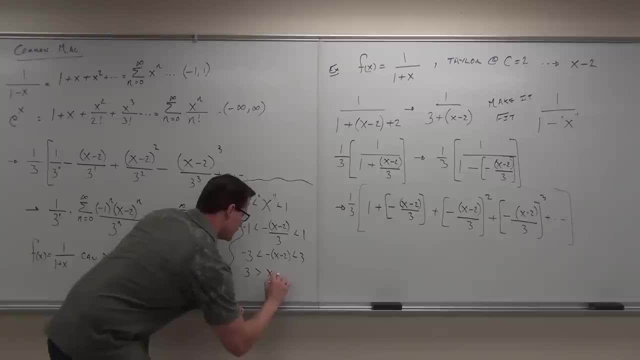 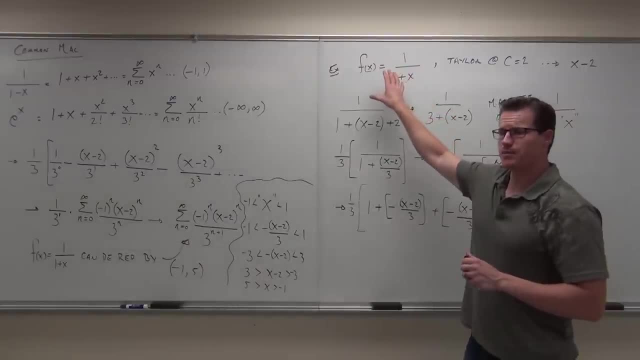 We get the interval negative 1 to 5.. We get the interval negative 1 to 5.. We get the interval negative 1 to 5.. Take your function, Make your center fit. After you make your center fit, manipulate it so it fits one of your series you already know. 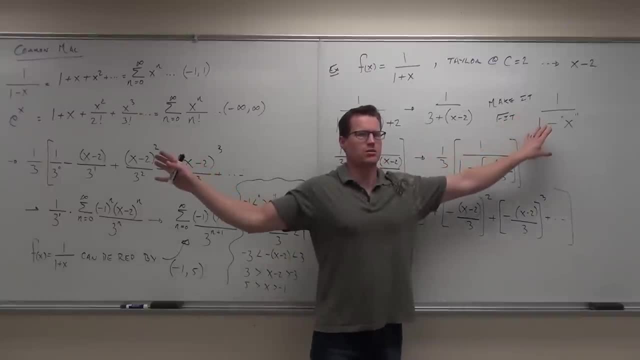 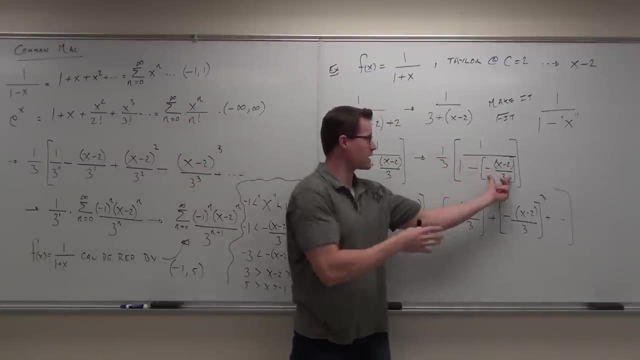 After that, use it. Whatever your x is up here is, whatever your junk is here, whatever we made it fit as okay. So this right here, this becomes your x. So this right here, this becomes your x. Just don't forget that at the very end, when you get all this stuff done, when you find your pattern, 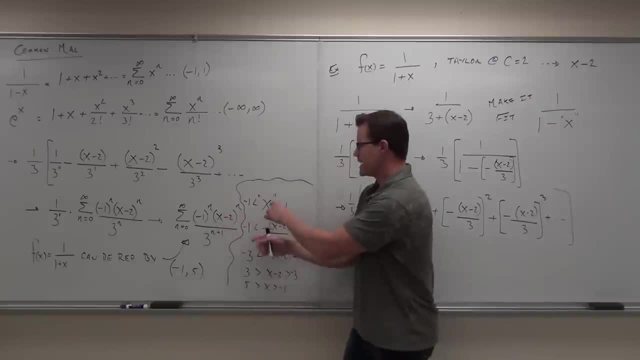 when you make your pattern work. it's not going to be that hard. When you make your pattern work, take your junk. take your junk and just use it. Good, All right, Great job. Thanks man, Thanks man. 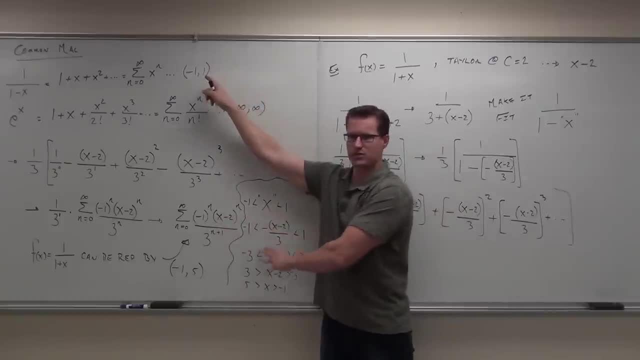 Good job, junk. put it back into your interval and then solve for it. solve for what that interval is. Does that make sense to you? Yeah, Okay, now I'm going to pause the tape here real quick. If you need to go, you may go. I'm going to stay here for another 30 minutes. 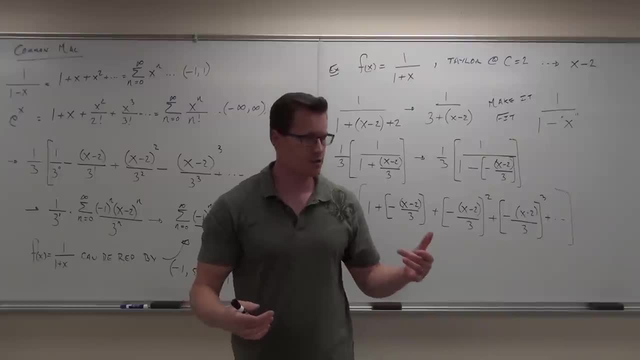 or so- and lecture. I'm going to put this on videotape, so if you want to just do this later, you can. So if you need to go, go. I don't want to make you any later than you are for whatever you want. So I'm going to give you about 30 seconds, If you want to. 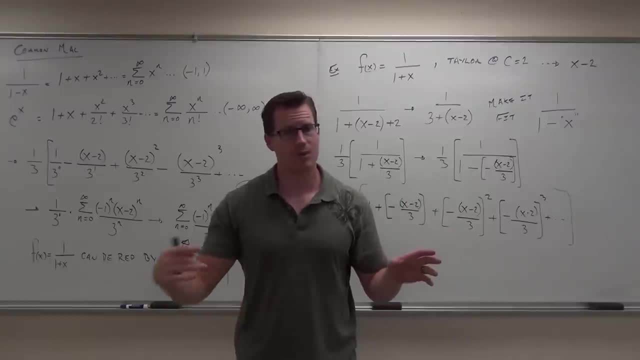 head out, head out. You're not going to offend me, okay, If you want to stay, I'm going to be lecturing. I think you're going to enjoy it if you do stay, but if not, have a great spring break. Okay, 30 seconds, Go or stay. 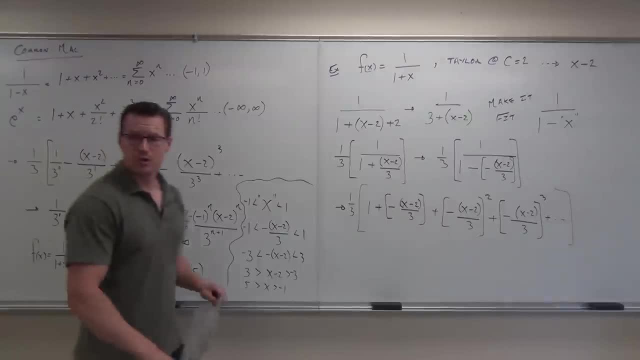 This doesn't look like something I can afford to miss. You can watch it. It's going to be the same. It's not the same. It's not the same. Oh, I don't want to do this to you guys. If you really need to go, 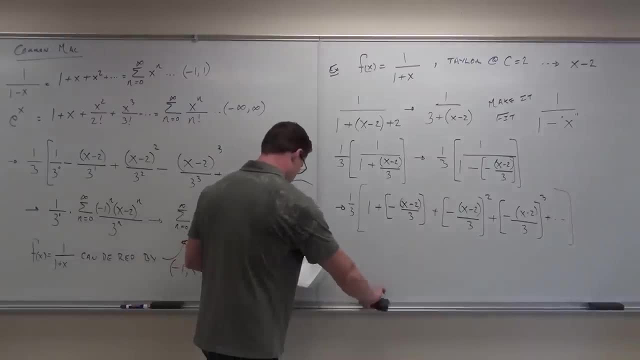 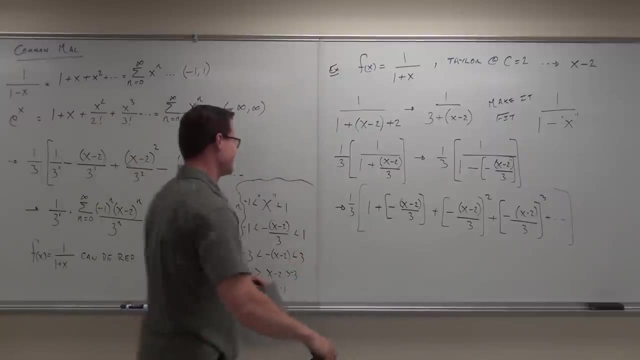 No, Oh no, it's fine, Okay, All right. So now we're going to continue. That's all I'm saying. Did this make sense to you? Did you grasp that You go? okay, take your junk, plug it in, no problem, Just don't forget. 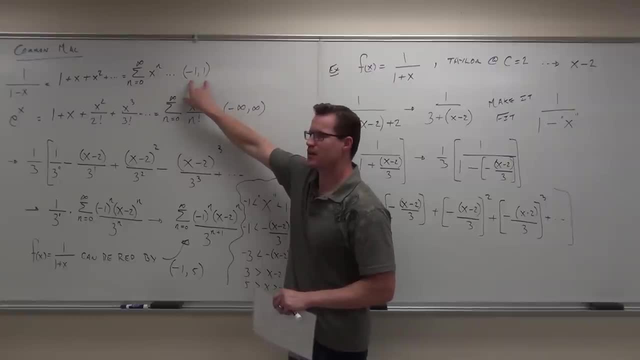 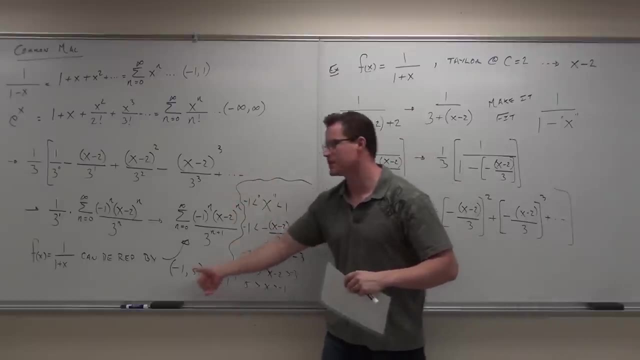 about your interval. Your interval, yeah, it's going to be based on this, but this says that your x, your stuff, is going to be between negative 1 and 1. Solve for your actual x and you get here between negative 1 and 5.. Now we're going to continue. We have about. 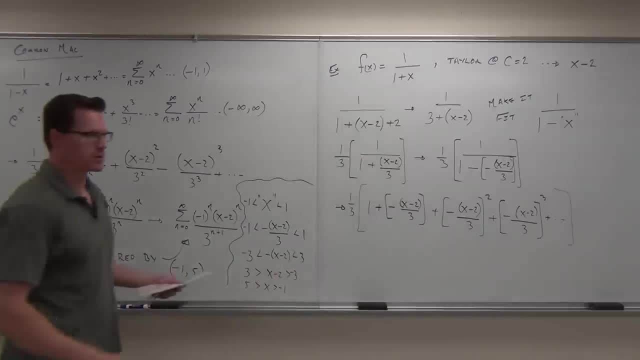 two and a half more examples. They're going to go quicker now that we have this idea. So what I'm going to do is I'm going to put up the example We're going to talk about what series we're going to base. 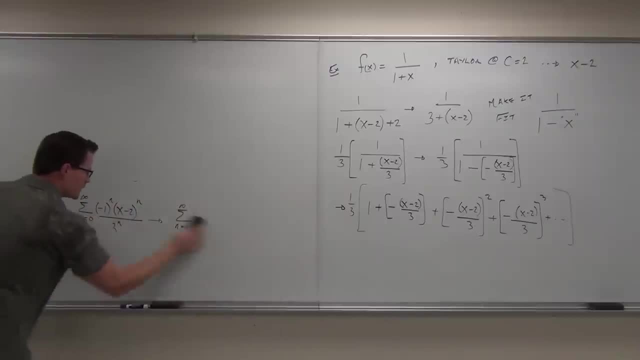 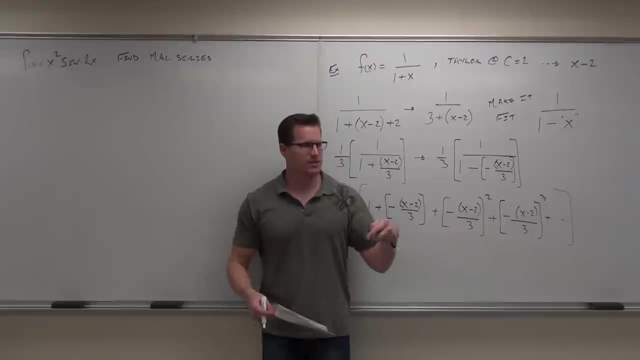 it on. I'm going to show you the things that we can do and we'll end it. So next example, What I want to do with this. I want to find the Maclaurin series. You'll notice that in the previous example we based it on a Maclaurin series, didn't we? 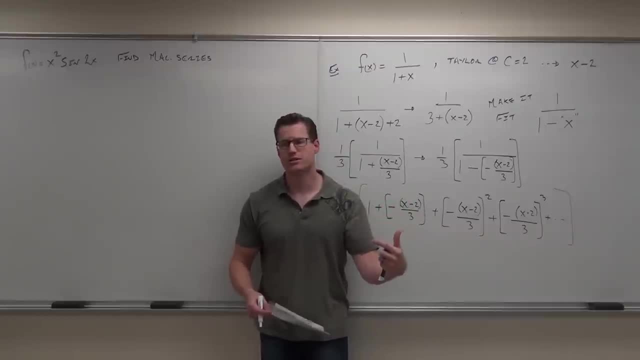 Because I gave you common Maclaurin series. If you need a Taylor series, you have to fit the x minus the center in there, Not a problem. If you want a Maclaurin series, it's even easier. So if I have x squared sine of 2x, well, what series are we going to base that? 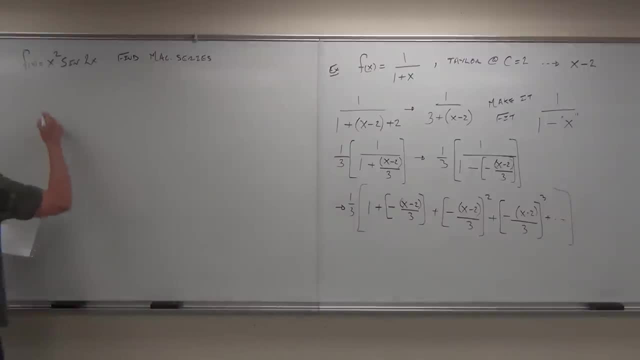 on Sine x, Sine x. So what we know is that if sine x is equal to x minus x cubed over 3 factorial plus x to the 5th over 5 factorial minus, blah, blah, blah, blah, If that's the case, look. 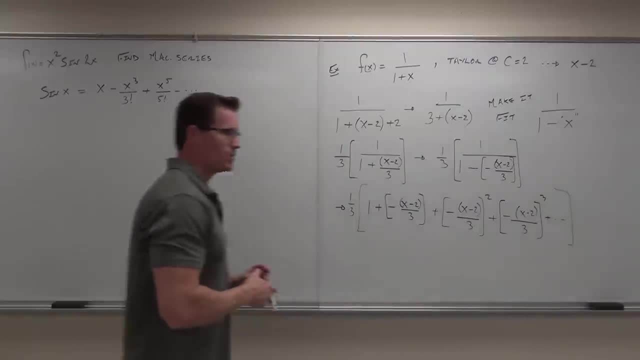 at what we can do. It's so nice, All we've got to do, all we've got to do. well, is this exactly like this? No, Is this exactly like this? No, It says sine x. it says sine 2x. Don't fret, don't worry. If sine x equals this, then sine. 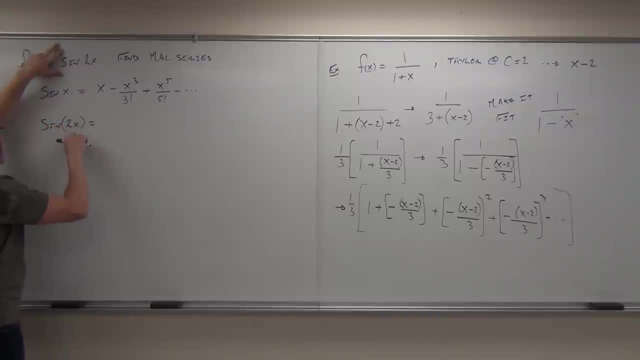 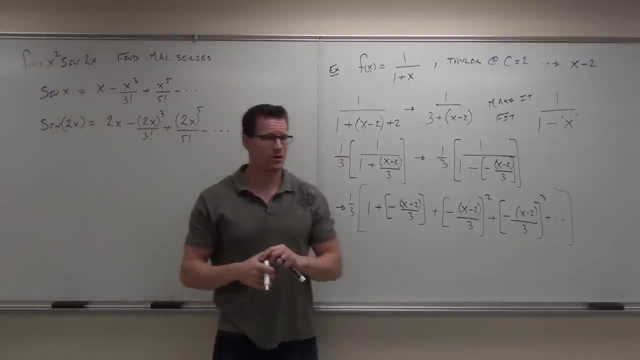 2x equals. plug it in: 2x minus, 2x to the 3rd over 3 factorial plus, 2x to the 5th over 5 factorial minus, and you keep going like that. Notice how here I keep using the word. 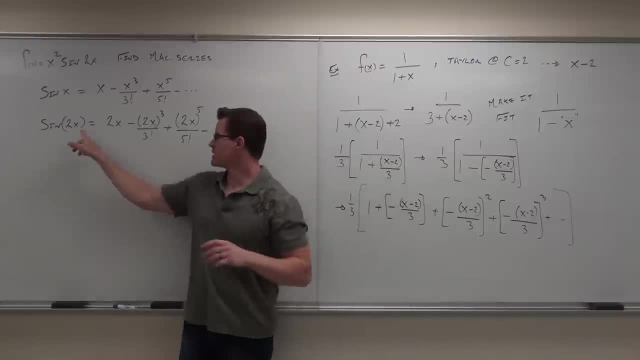 junk. I'm going to still Your x. your junk is now 2x, So you just plug it in Now. fortunately for us, because we have a Maclaurin series, you don't have to fit an x minus anything. 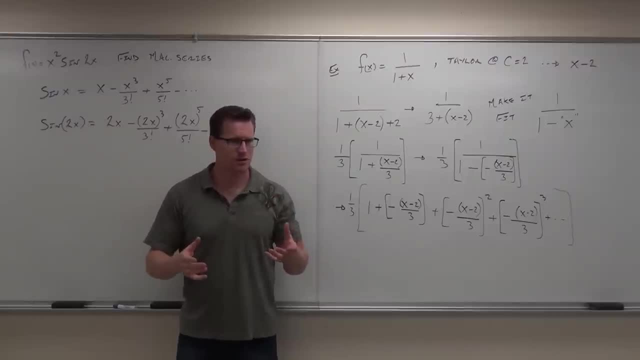 It would be 0.. It would just be x. Does that make sense to you? So cool, all right. Well, your junk is 2x. Just put it in here. We've got 2x. We've got 2x, cubed, We'd have 2x to. 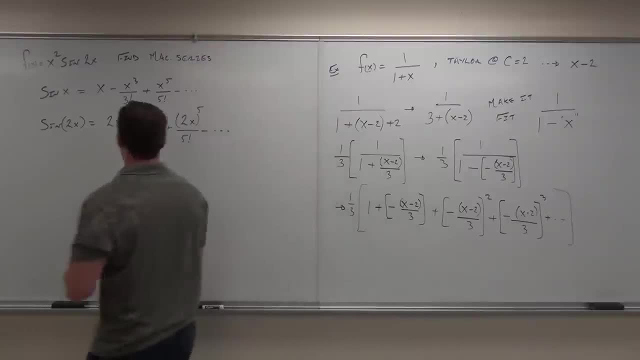 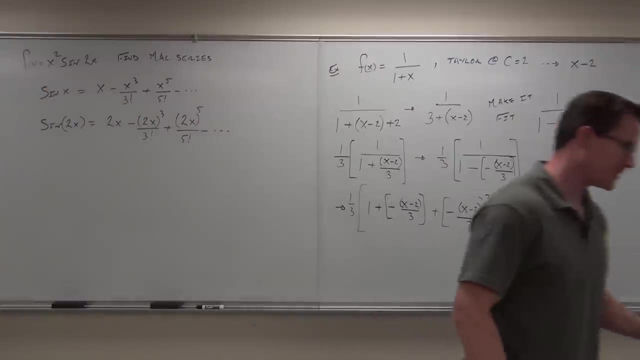 the 5th. So you can just feel all right with that one. All right Now. oh man, Is this the same as that? No, but it's really close. So if that's not the same, what else could? 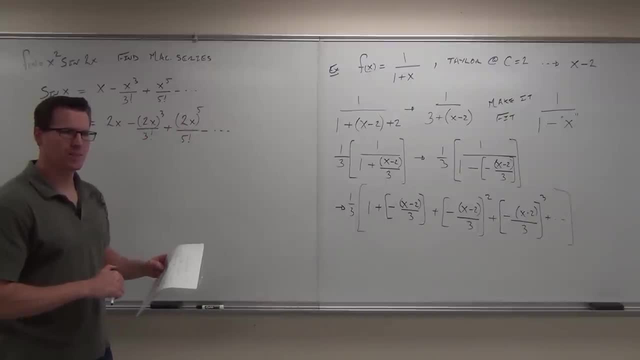 we do Say: what now? How do I make this look like this? You can actually do that right now if you want. I'm going to show you how to do it later. It's really easy, So I prefer doing it this way. but you could multiply by x, squared everywhere. You could do that. 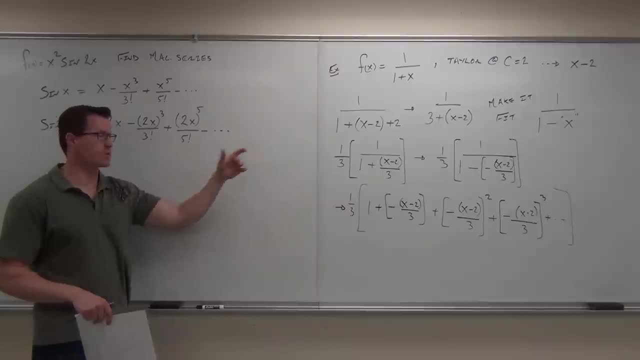 It's going to come out exactly the same, It's just the pattern's a little harder to find. So we're going to start finding this pattern right now. So, working on the pattern, let's see what it actually does. What this is is. this would be 2x, No problem, Remember I'm 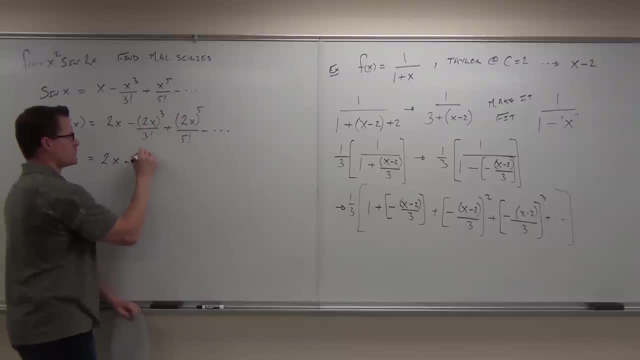 looking for patterns here. So I'm going to have 2 to the 5th. No, I'm not. I'm going to have 2 to the 3rd, x to the 3rd, over 3 factorial. I'm going to have 2 to the 5th. 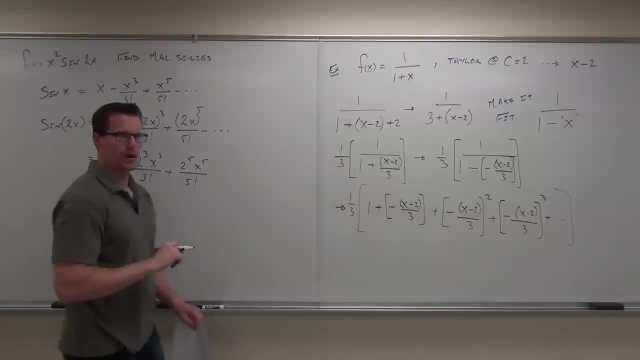 x to the 5th over 5 factorial. I'm splitting this up for a reason. The reason why I'm splitting them up is because I'm going to have 2 to the 5th- x to the 5th over 5 factorial. I'm. 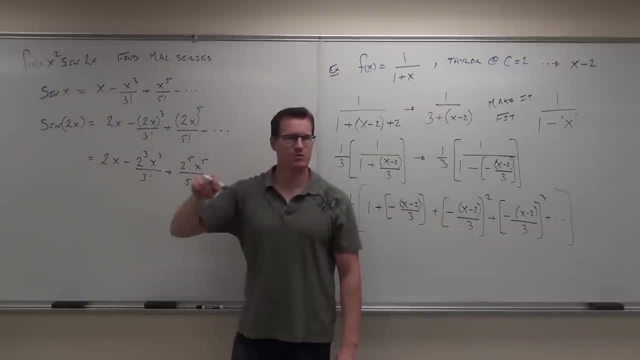 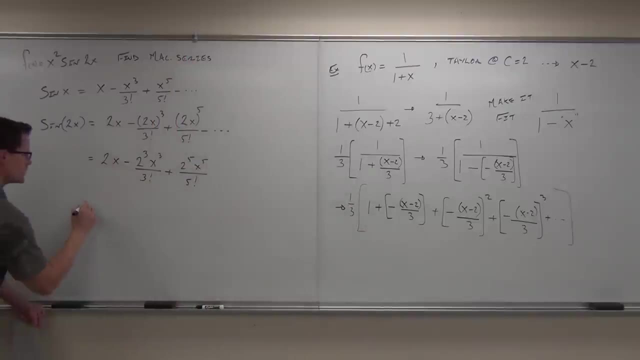 going to be multiplying by x squared later, And so I'm going to have to split them up at some point or another. I'm going to split them up right now. Show of hands, if that makes sense to you. Now let's make our series. We're about good to go on this, So our series. 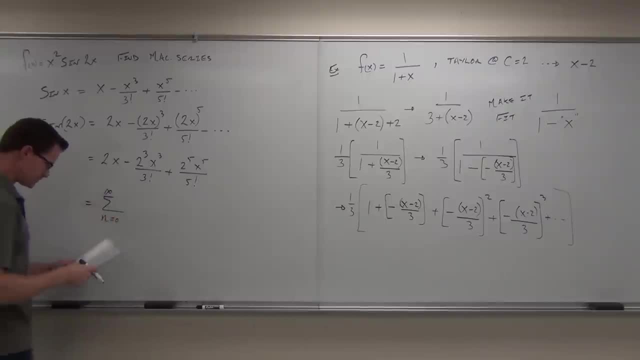 starts at 0. It goes to infinity. Tell me something about this series that you know. Yeah, it's alternating And it starts off with a positive. So that would be n, That's right. Tell me something else about this series. 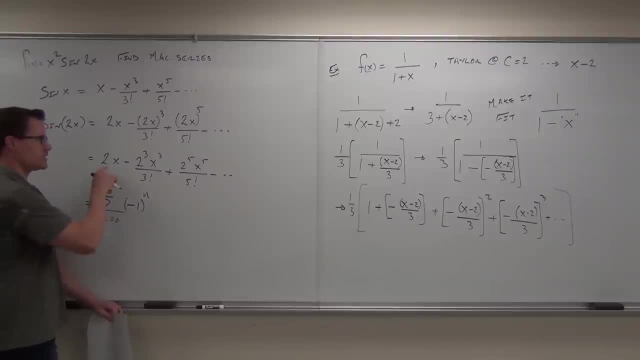 It's odd numbers. It's odd numbers, That's right. It's taking 2 odd numbers. It's taking x 2 odd numbers, All over odd numbers, factorial. We have to use a plus 1 here for our odd numbers, because 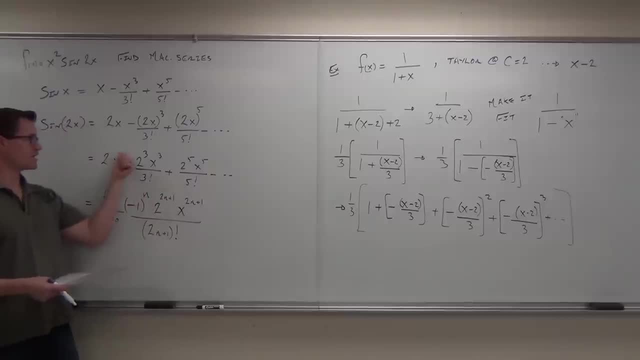 we're starting at 0.. Do you guys see what I'm talking about? We start at 0 and we get a 1 and a 1.. This is well, and you're 0 with a term, you're actually getting 1.. So you're. 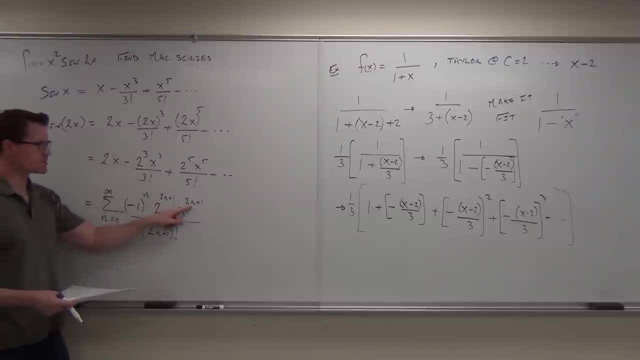 getting 1.. So 2 times 0 plus 1 gives us 1.. 2 times 0 plus 1 gives us 1.. All over 1 factorial. So we're starting. it says 0, but we have to make them odds, but we have to start at. 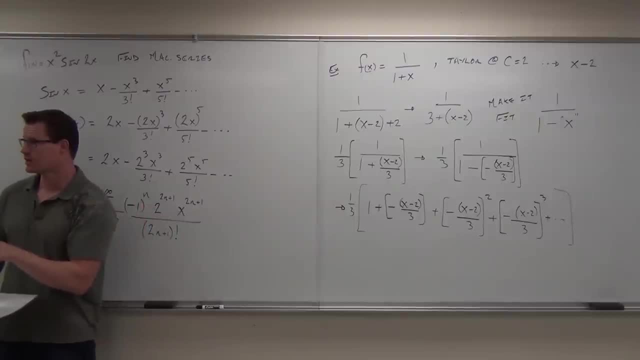 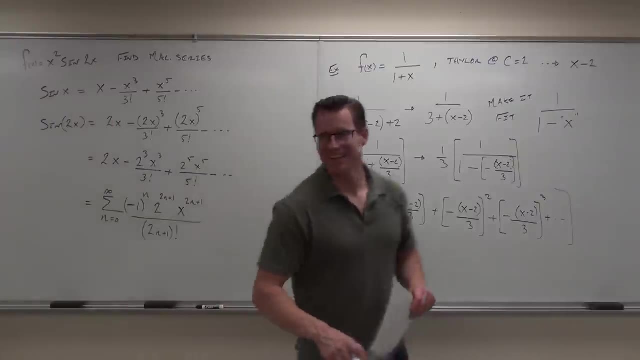 1. So it's not minus 1 this time, It's plus 1.. Do you see why Did I lose you? You're going to get in the way. Does that make sense? Okay, So here's what we know. We know that this thing sine of. 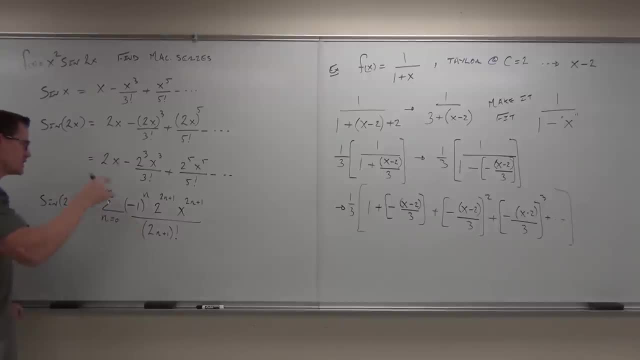 2x would equal that series with no problems. Now how do I get from sine of 2x to what I want? You can do things like that. So if I multiply by x squared and I multiply by x squared, listen, It's an equation, It's. 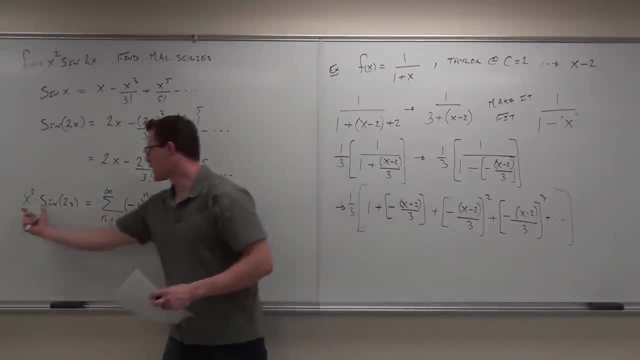 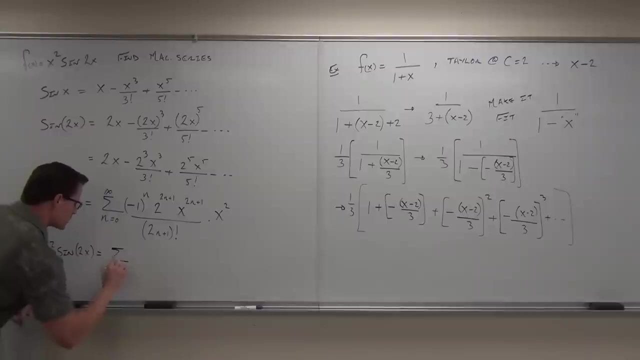 going to work. This thing is represented by this series. Therefore, x squared times. this thing is represented by this series: times x squared, Therefore x squared times. sine of 2x is equal to our series. we go from 0 to infinity, negative, 1 to the nth, 2 to the 2n plus 1.. 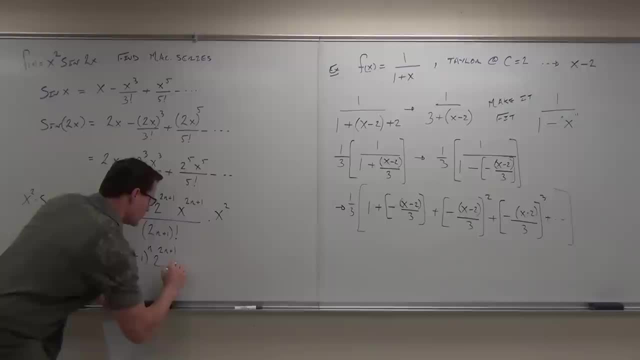 What's that going to be? 2n plus 3.. 2n, yeah, do you guys remember that You're adding x to it? so 2n plus 1 plus 2, that's 2n plus 3.. 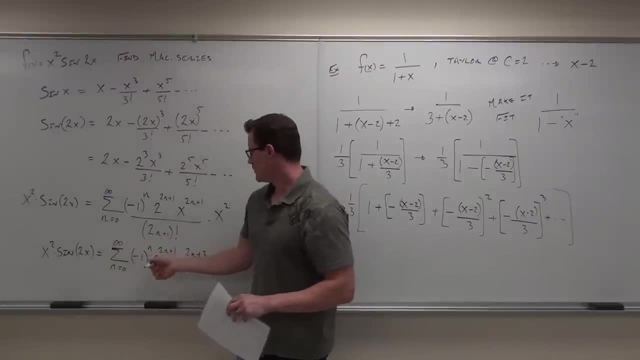 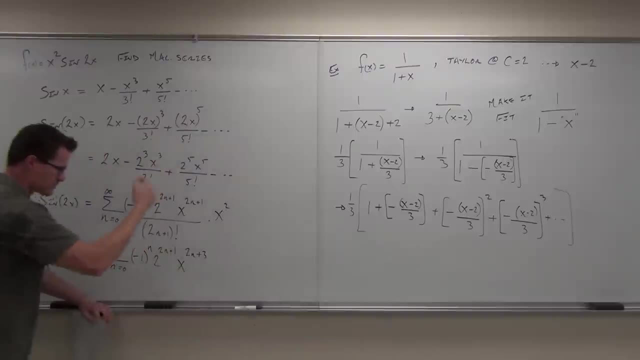 Now I'm going to stop for just a brief moment. Do you understand that you could have multiplied by x, squared here, and got the same thing? It's just your 2s would be different than your xs, so your powers of 2 would be different than your xs. 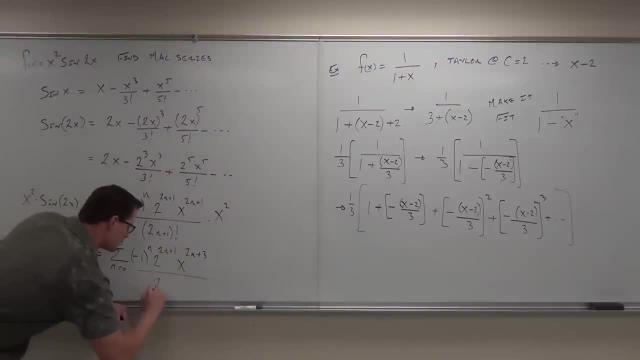 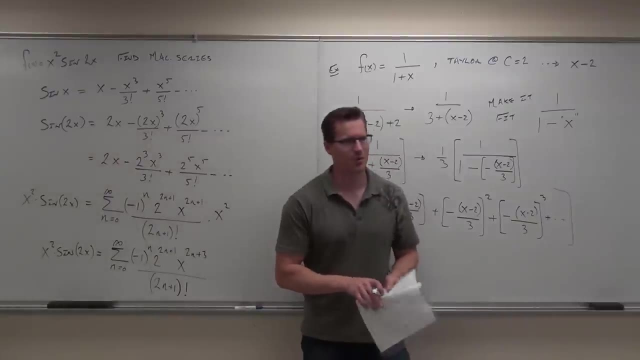 Is this going to change to 2n plus 3?? Now, we're almost done with this one too. This is going to go quicker. after this, Look back at your notes and tell me the interval of convergence for our sine, Not sine. inverse for our sine. 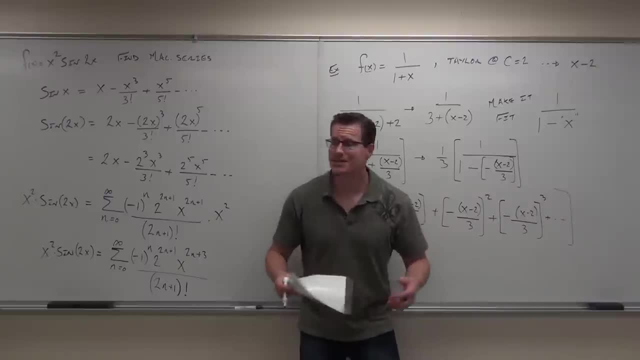 Negative infinity to infinity. What that means is that if our sine is convergent on negative infinity to infinity, our sine of 2x is also convergent on negative infinity to infinity, and even when we multiply by x squared, it's still convergent on negative infinity to infinity. 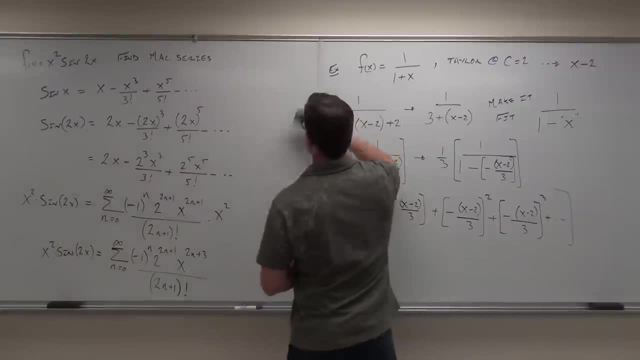 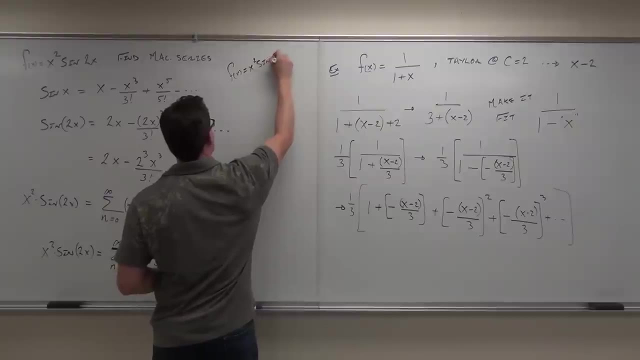 So what we say? we wrap this thing up and we would say that f of x equals x squared sine of 2x. Now this can be represented by our nasty series on negative infinity to infinity. And if you forgot what that means, here's what it means. 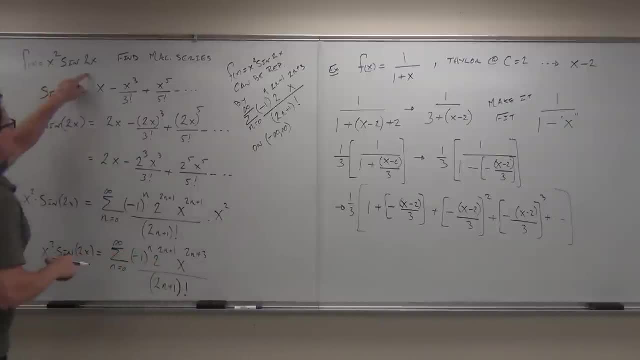 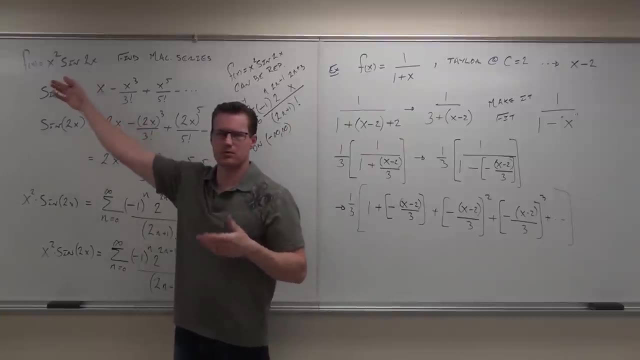 It means this: If I want to, If I want to find out this as a value at any number, I could actually do it with this series. I could plug in my Give me a number, Any number: Three, Three, Plug in three. 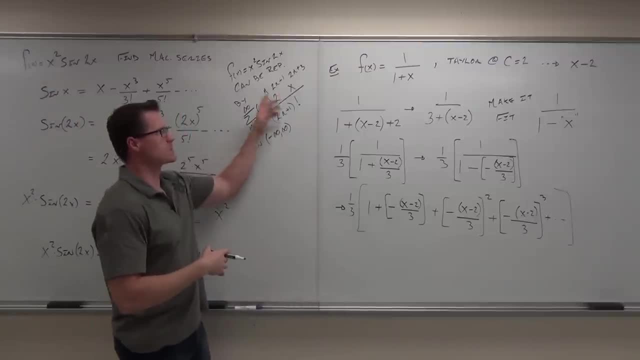 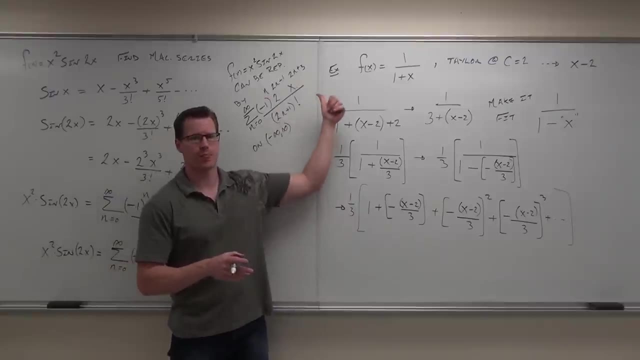 If I wanted to plug in three, I could actually represent it by plugging in three to this series, working it all out to infinity and adding it all up together, And it will work for any value. What it says is that this series will converge for any value of x. 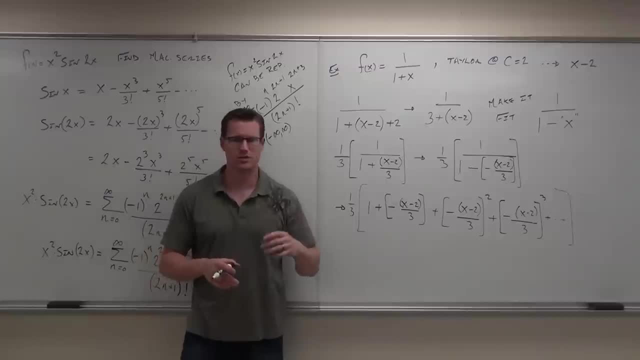 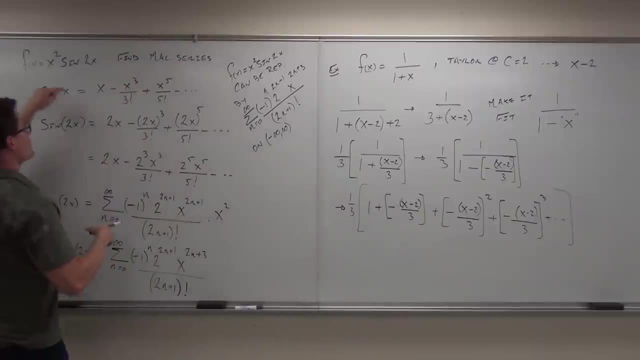 Therefore, for any value of x, this series, this power series, Taylor series, McLaurin series, will represent our given function. So, fans, if that one made sense, So can you manipulate what you have to get what you need. 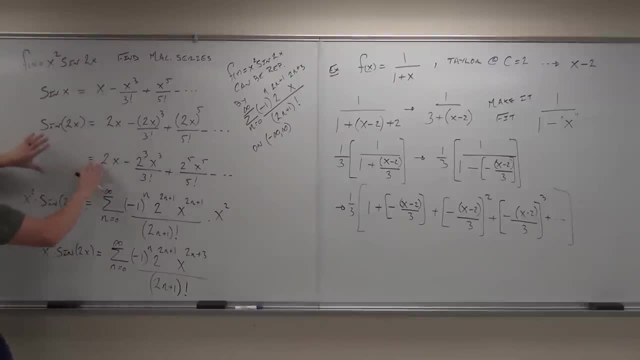 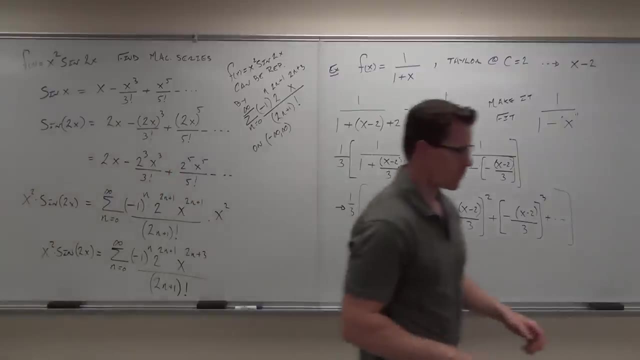 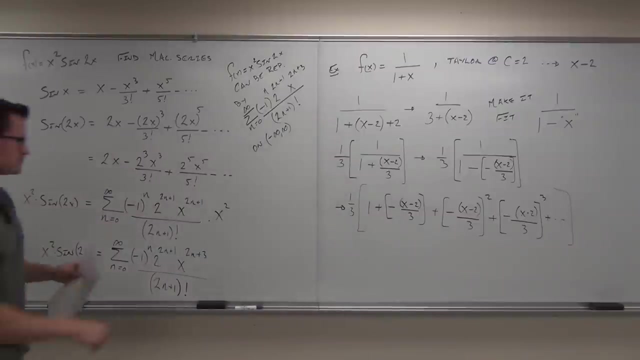 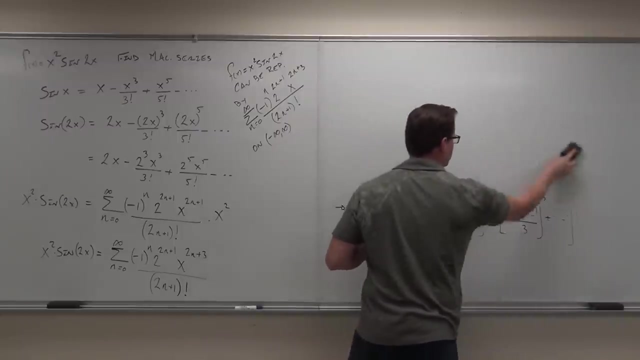 Sure, Multiply this by two, you get this. Take, find your pattern, find your series, multiply by x squared, No problem. Just a couple more. The reason why you don't have a whole bunch of other McLaurin series, why you only have a set amount of them from me. 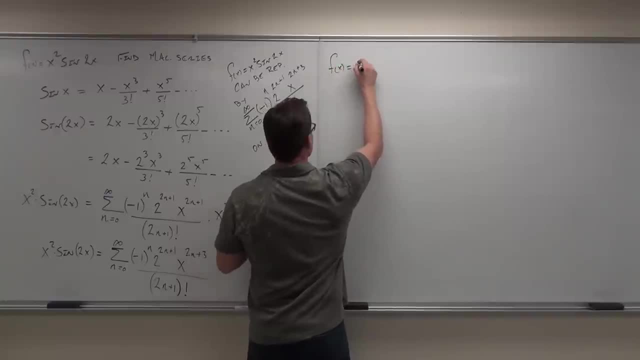 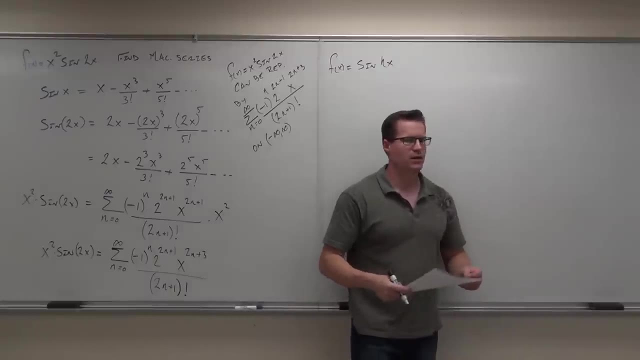 is because a lot of times you can manipulate what you're given to what you want to get. Remember cinch. Do you remember the definition for cinch? No, No, we don't. It's a. do you remember what it means? 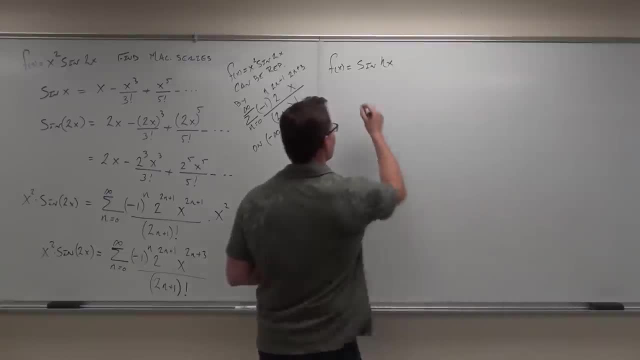 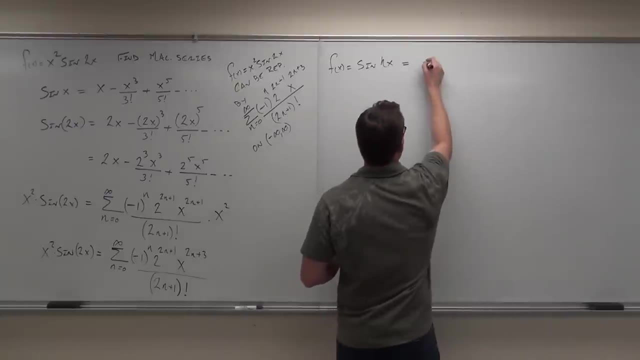 Hyperbolic. That's what it means. It's a very. at least we understand that. Okay, so well, if you don't remember it, here's what this meant. This meant e to the x minus e to the negative, x all over two. 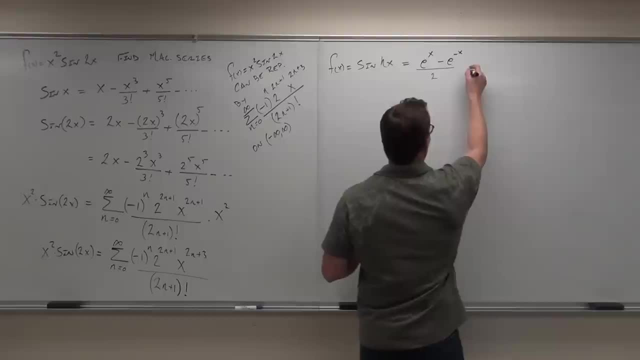 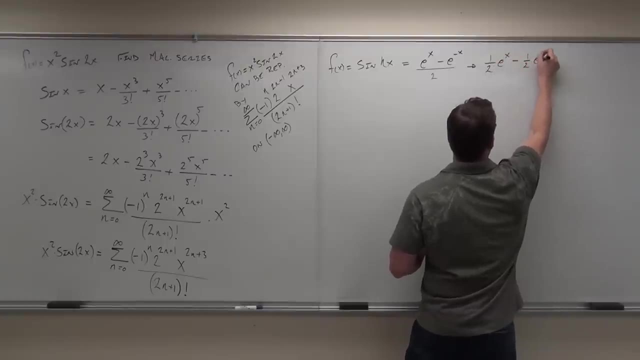 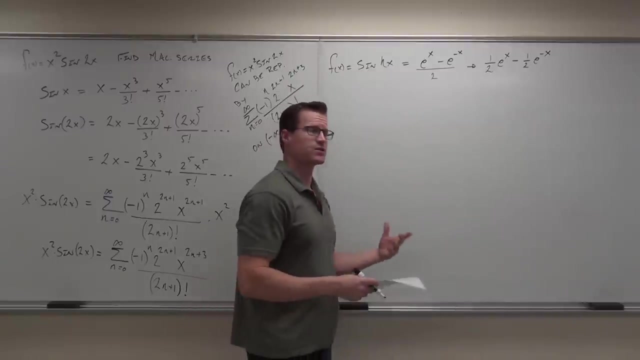 Do you remember that one? Yes, Okay, cool. Well, if you split this up, okay, Then what we really have here is a combination of two different series, which is really cool. So think about this. Look back at your notes and you tell me what e to the x equals as far as your series is. 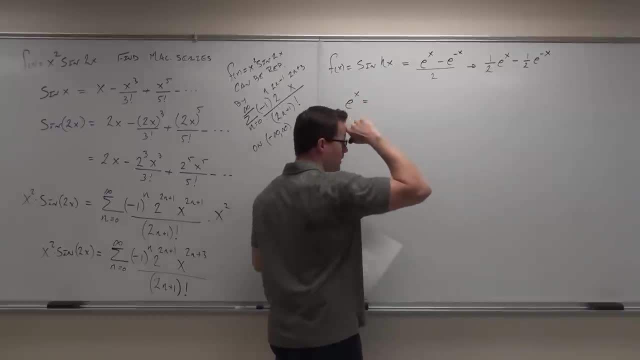 You know what? that's great, but we're going to have to do it term by term, because we're going to have to find this pattern, Because we're going to be combining two series. okay, So tell me term by term what e to the x is represented as. 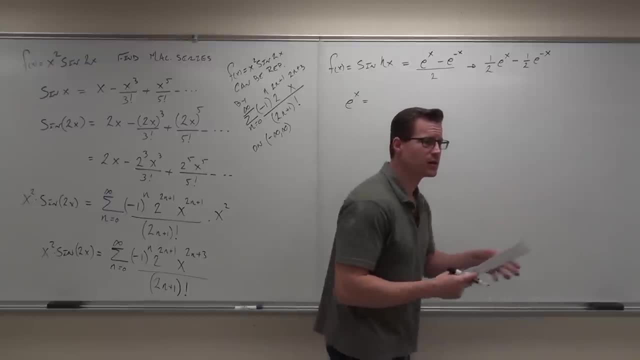 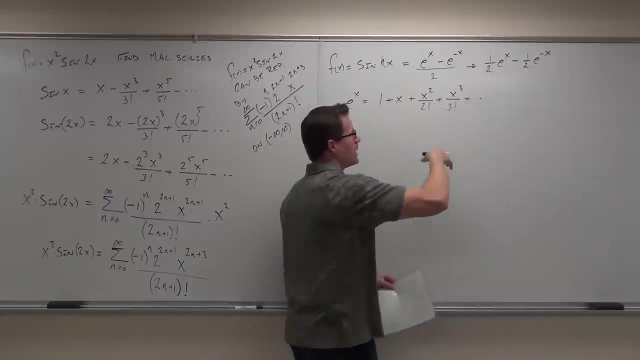 One plus x, One plus. say it again, Plus x, Keep going, Plus x. squared over two. factorial Plus x. cubed over three factorial. And Patrick's right, that would be x to the n over n factorial. Quick head nod, if you're okay with that so far. 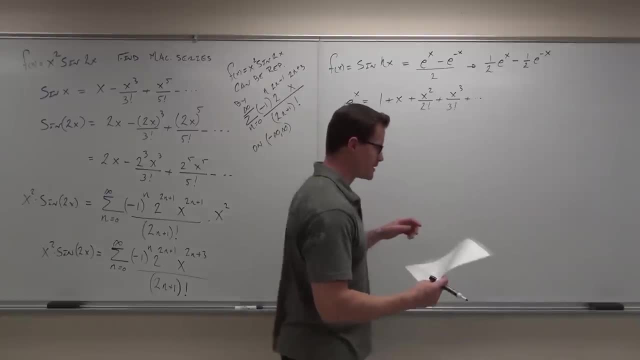 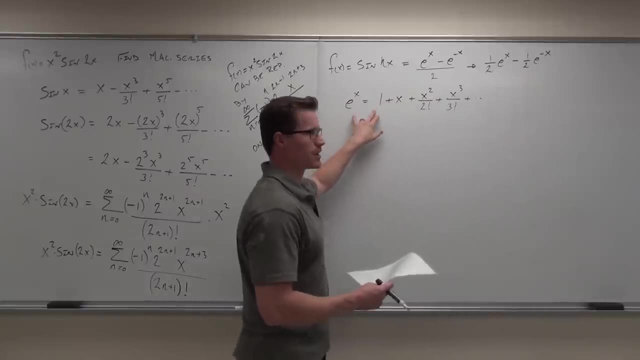 Awesome Now, If we can fit these things to this thing, this thing to this thing and then subtract them what we just find. So check this out. This is kind of interesting. So if I do, oh, wait a minute. 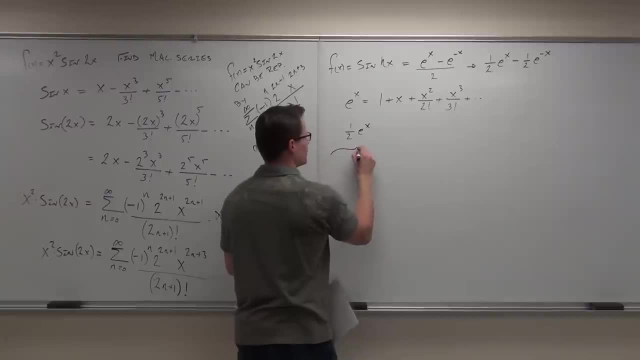 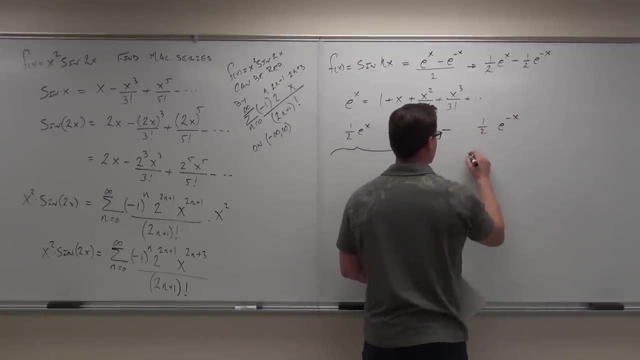 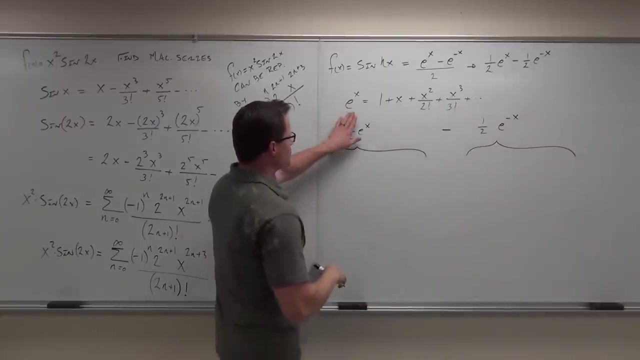 One half e to the x minus one half e to the negative x. well, if I have one, look at that, Do you see that e to the x is just going to be this bunch of junk? So this is going to be one half times one plus x plus x squared. 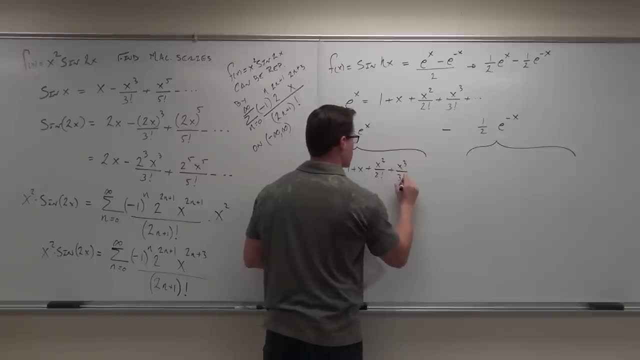 over two factorial plus x. to the third over three factorial plus blah, blah, blah, blah. minus one half times. here's our one half, here's our e to the negative x. You tell me, Does this fit? Does this fit exactly what this is? 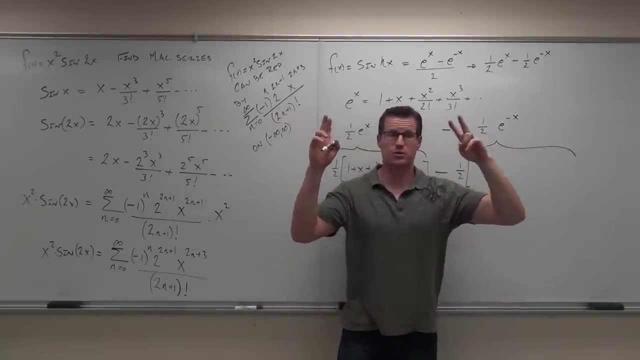 No, What's our junk here? Negative x. So negative x is what I'm plugging in. So if I plug in negative x, then I'm going to get one I'm going to get. please look carefully if I plug in a negative x. 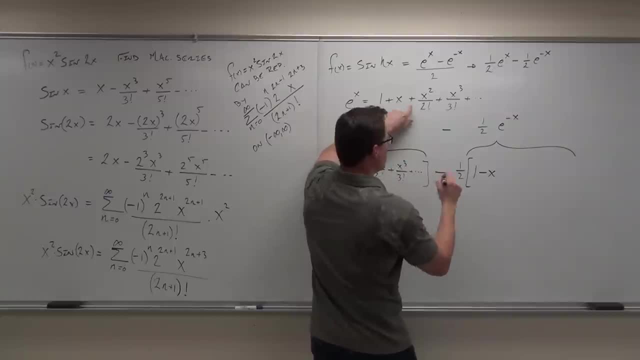 I'm going to get minus x. Do you see why I'm going to get plus x? squared over two factorial. Do you see why I'm getting plus? Yeah, Because if I plug in a negative x, I go okay, one one. 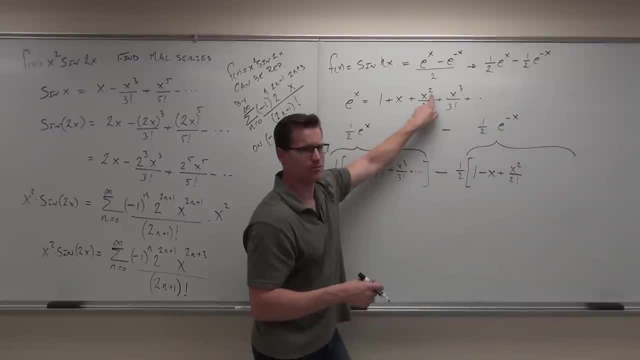 Negative x Cool. What's negative x squared? Positive x squared. okay, What's my next one? Negative x to the third. Negative x to the third is still negative x to the third. It's negative x to the third Over three factorial plus, blah, blah, blah, blah. 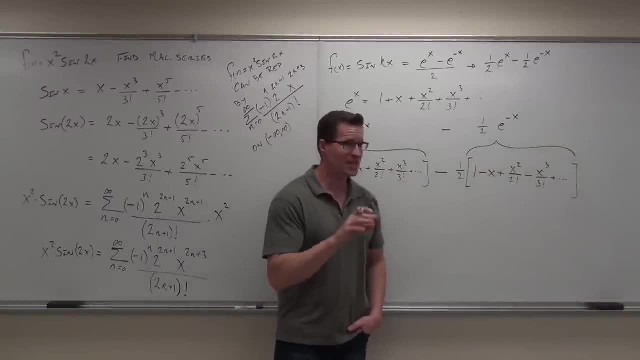 Are you sure you're okay with this? Now something really, really cool is going to happen when we do this. Check this out. Ignore the one-halves for a second, because, naturally, if I'm subtracting something multiplied by one-half, 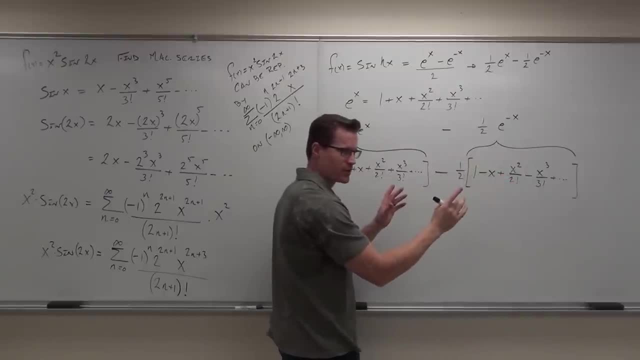 I can subtract the terms themselves and multiply the one-half later. Did you catch that? So watch What's one minus one Zero. Those are gone, Do you see it? Yep, Now this would be x minus negative x. 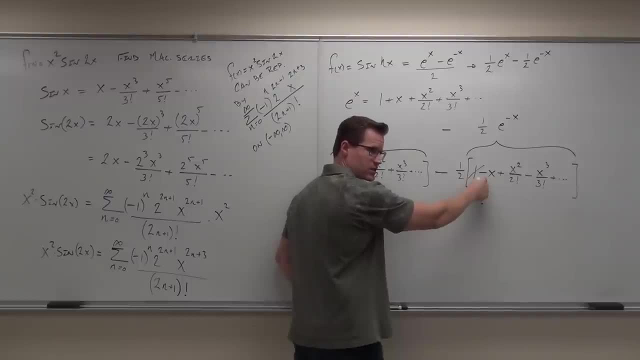 So that does not simplify, because that's going to be x plus x. That would give us 2x. But what's this? Yeah, jump, X squared over 2 factorial minus X squared over 2 factorial Zero. Do you see that every even power is gone. 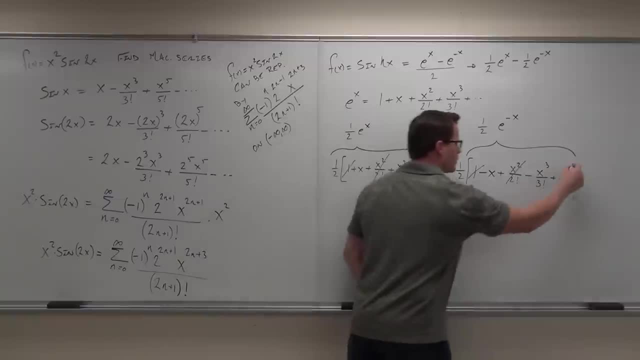 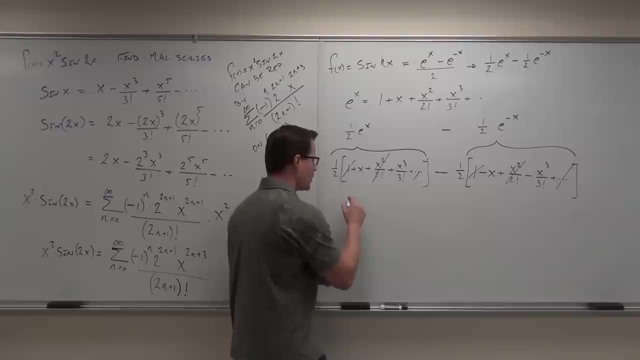 Every even power. So the squared squared, The fourth with the fourth. Let's combine what's left over. In fact, if I just factor out my one-half, we're doing some advanced elsewhere here, all kind of in our head. If I just factor out the 1 half, what I'm going to end up getting is: well, here's 2x and here's- remember, minus and negative is a plus. 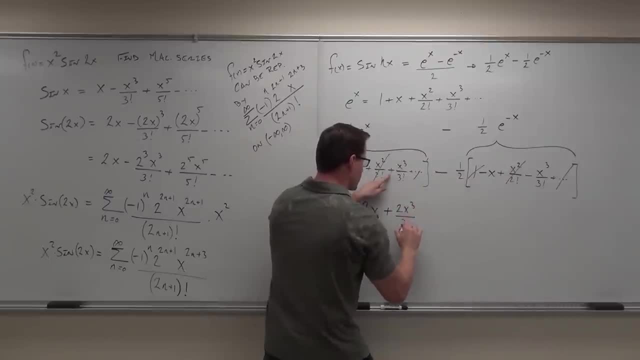 We'd get 2x cubed over 3 factorial plus 2x to the 5th over 5 factorial plus blah, blah, blah, blah, blah, blah blah. Did you catch that? We did some advanced algebra here. 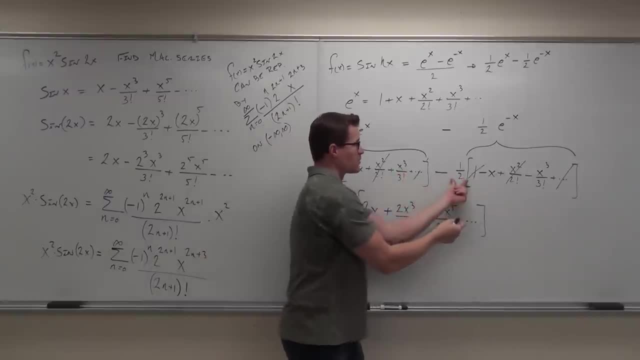 We're distributing our negative and we're combining our like terms. Basically, we're factoring out our 1 half, no problem. Our negative we distribute and then we're combining like terms. If you get that, your 1s are gone. 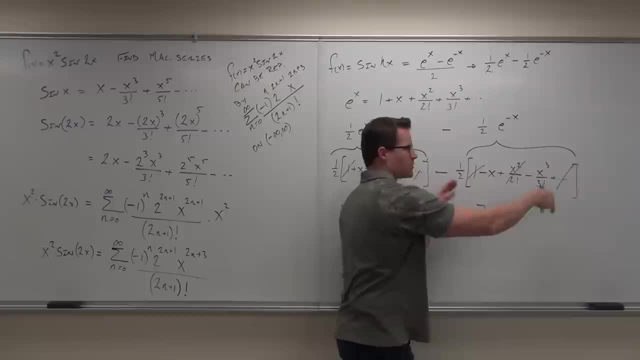 Your 2 power 2s are gone. Your power 0s are gone. Power 2s are gone. Power 4s are gone. Every even power is gone. Your odd powers will be added together: X plus X- 2x. 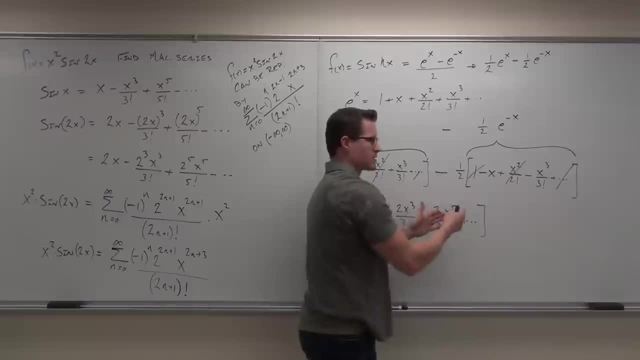 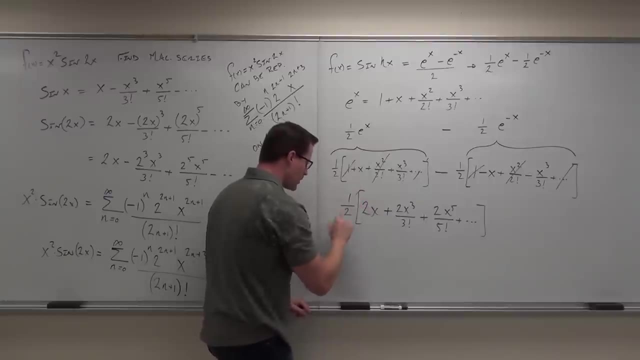 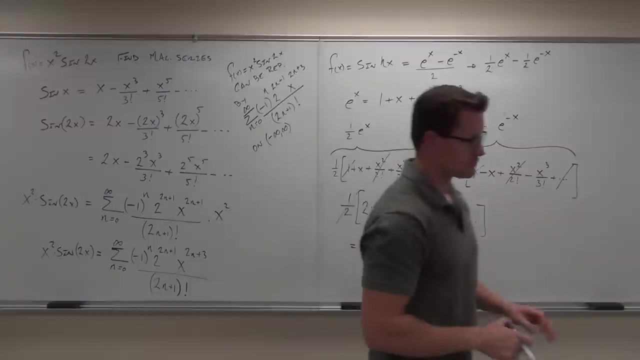 X third, X third, 2x third, X fifth, that's 2x fifth. Now, when I distribute my 1 half, what happens With this one and that one and that one and so on? So this becomes X plus X to the 3rd over 3 factorial, plus X to the 5th over 5 factorial, which makes a series. 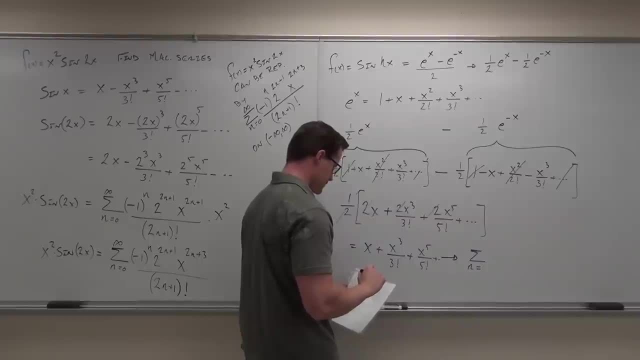 Oh, let's do this together. Where does it start? Starts at Zero. Zero Goes to infinity. Tell me about my power, The powers of X. what do I have? Odd powers, Odd powers, Remember. if I'm starting at zero, is this odd power going to be 2n minus 1 or 2n plus 1?? 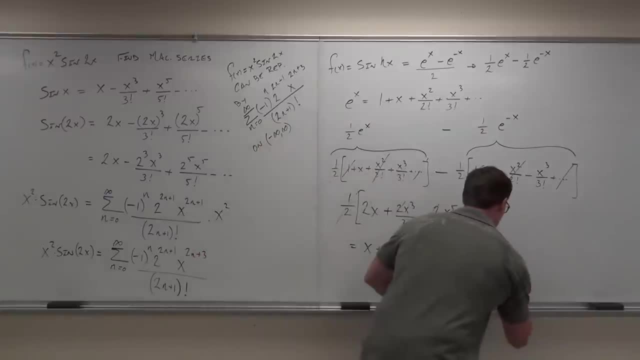 Plus 1.. Because I have to start at the 1.. So, yeah, you're right, X to the 2n plus 1, all over. tell me what I get on my denominators 1 over 1.. 1 over 1.. 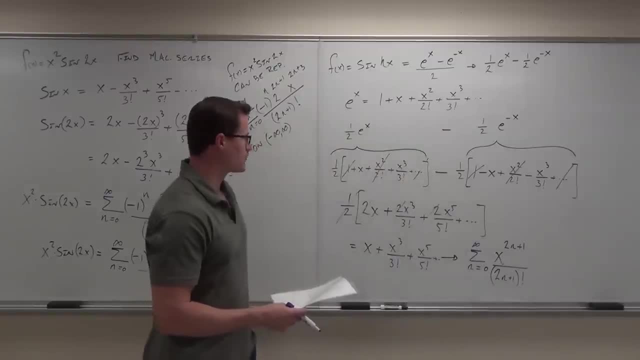 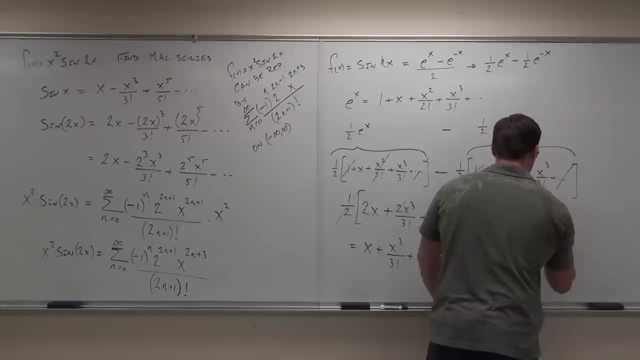 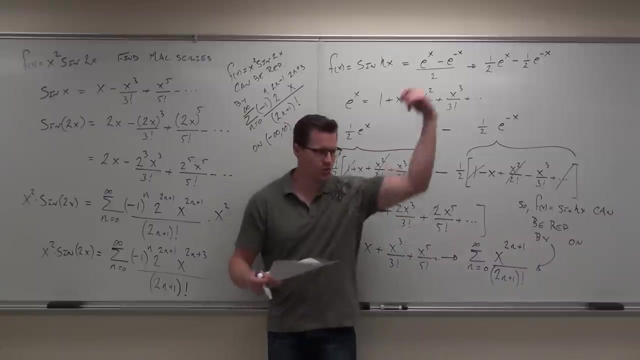 Beautiful. That's exactly right. So F of X equals sinh. X can be represented by this on. now look back. what, what Maclaurin series did we use to do our work with? E to the X, E to the X. 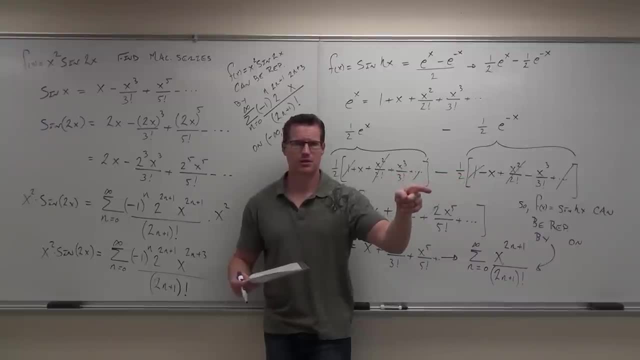 So look at the interval of convergence of E to the X- All real numbers- Negative infinity to infinity. Therefore, if we used a Maclaurin series which has a convergence of negative infinity to infinity, then this series also has convergence of negative infinity to infinity. 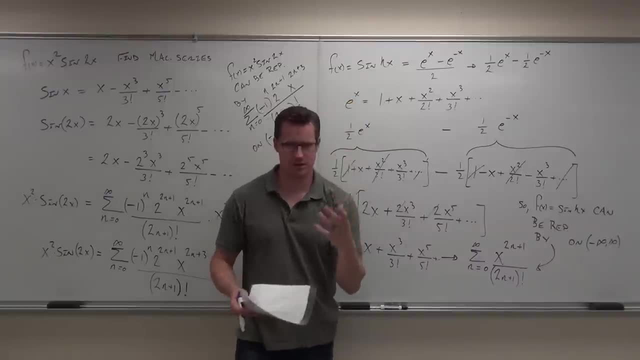 So when we get something that's not explicitly listed, we don't want to make this thing up on our own, okay, We don't want to start doing derivatives of this. It's crazy. We don't want to do that. We want to base it on something we know already. 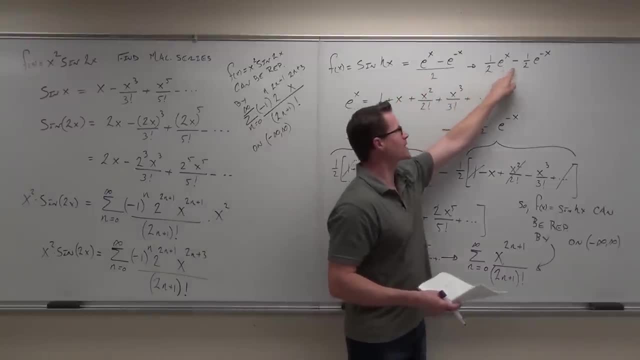 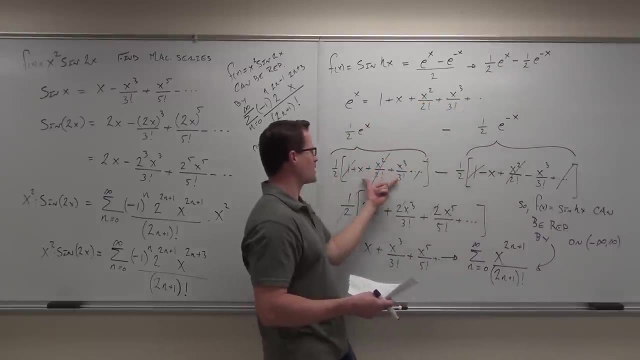 The definition is this: Well, that's 1 half E to the X minus. oh, look at that. This is exactly what this is. This is just this stuff with a negative X plugged in everywhere We get here. we get here. multiply by 1 half, no problem. factor out the 1 half, distribute your negative. lots of stuff simplifies out and we've got a very simple series to work with where we already know the convergence. 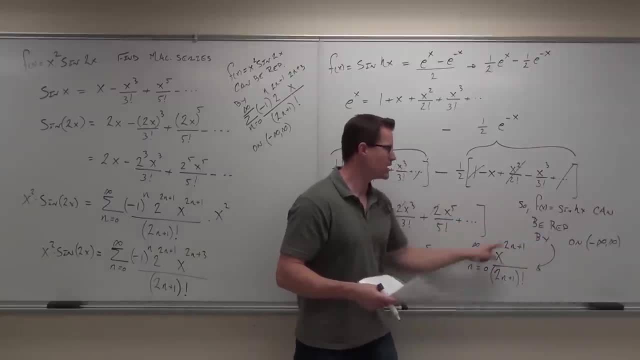 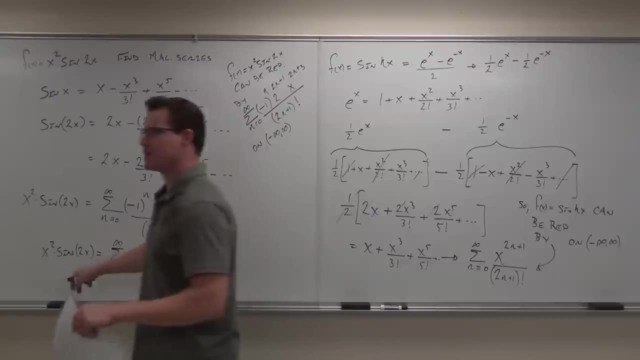 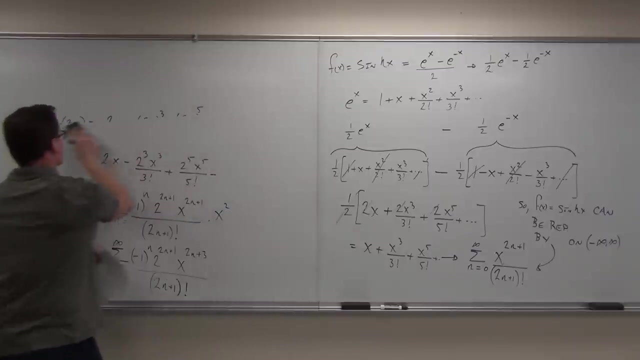 So when I say represented, that means that this series will give us this function for any number of X you plug in, and that's kind of cool. We have one more thing to do and then we're going to be done. Okay, this is the last thing. 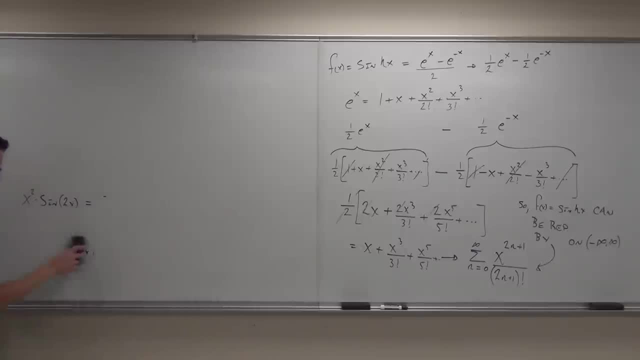 This is going to blow some of your minds right now. okay, This is what I really wanted to get to today, because it's so interesting, It's so cool. I want to lead you down this road here and I want to consider this. 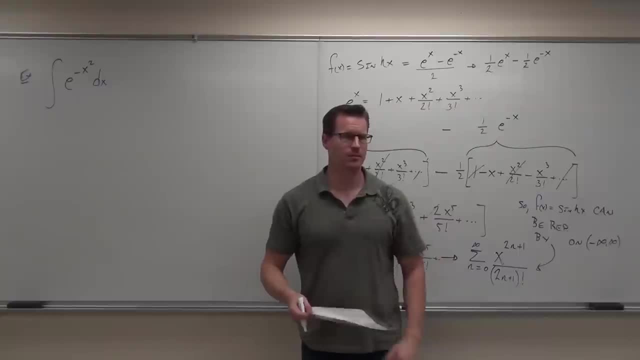 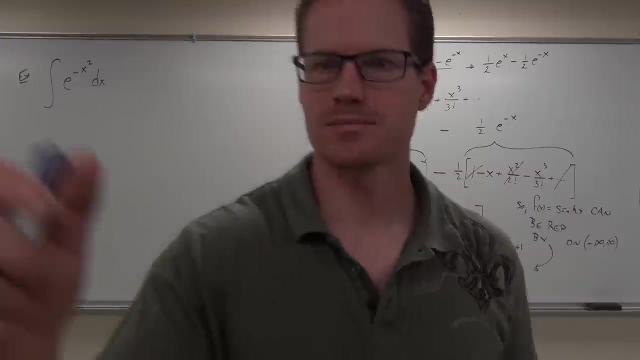 Here's my question: Do the integral? that wasn't a question, was it? Do the integral, can you do it? How do you do it? Do the integral, can you do the integral? Is a U sub going to work? 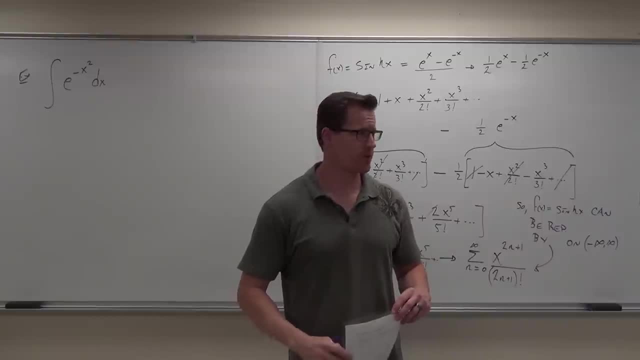 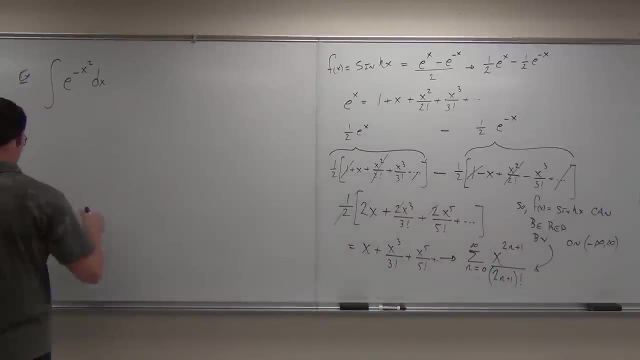 No, heck, no, It's not going to work. It's not going to work. It's not a definite integral, so I'm not going from anywhere to anywhere. Can I do the integral? that's sub all. Yeah, Here's how. 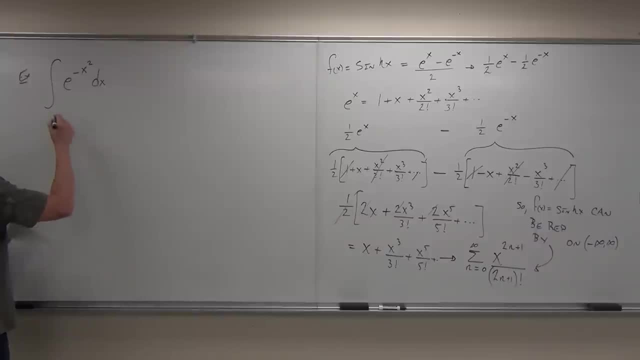 Firstly, well, you know that E to the X, we actually just work with it. One plus X plus X, squared over two. factorial plus X to the third, over three factorial plus blah, blah, blah. right, Hey, can you make this thing look like that? 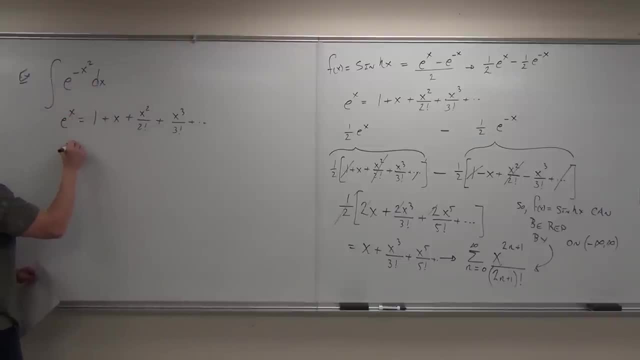 Can you make it look like that? What's your junk here? You can't even square it, X squared, So plug in your junk. If you plug in your junk, I still have one. Then I have Minus two X squared. 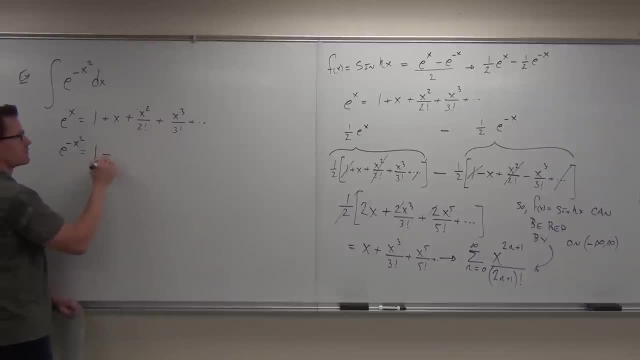 No, not minus two X squared. Oh, it's squared. It's going to be a minus, It's just going to be X squared. Are you with me on this? Here's our X right. Take this. That is now your X squared. 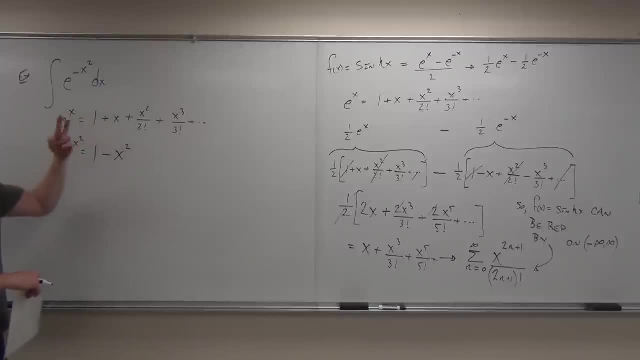 Okay, That is now your X. Does that make sense to you? This is your junk. Plus we have negative X squared, squared over two factorial plus negative X squared cubed over three factorial plus blah, blah, blah, blah, blah. Well, that's one minus X squared, plus X to the fourth over two factorial, minus X to the sixth over three factorial plus. what would the next one be? 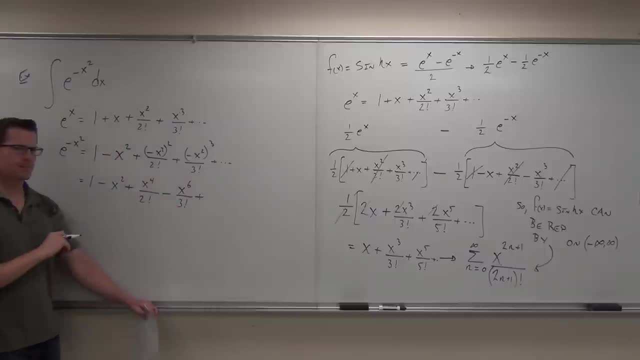 Come on, Go for it. Are you with me on that one? Yup, Are you sure you're with me? Let's write this as a series. Our series would be zero to infinity. Tell me something about our series. What would we get? 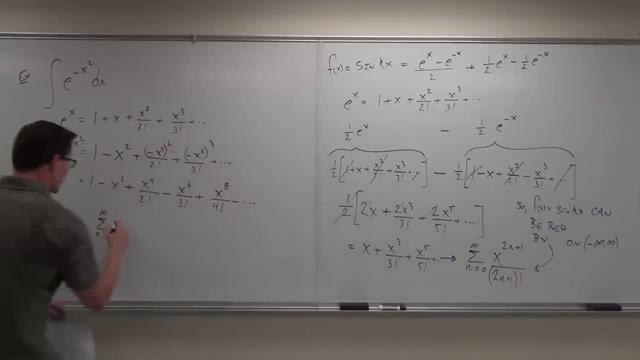 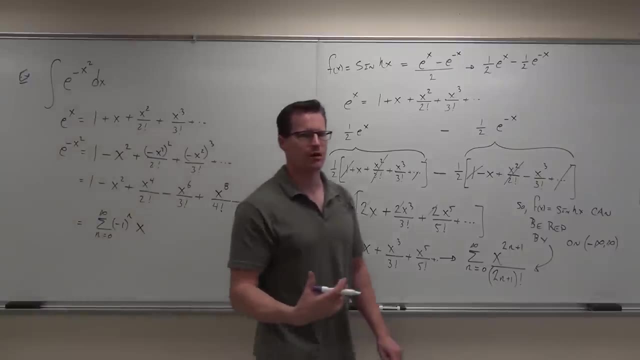 Alternating. Say what Alternating, Definitely alternating, And it's starting positive, So negative. one to the the n We'd have x to the. tell me something about our x's. what's going on? all evens. 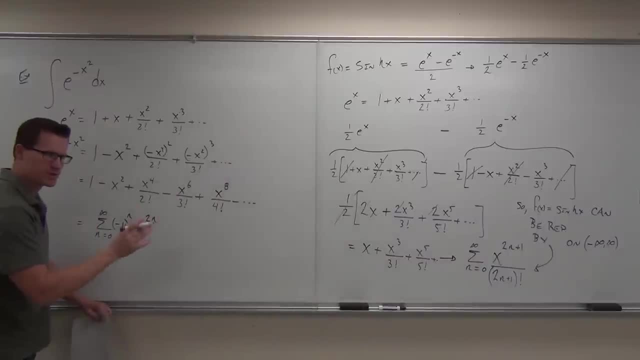 That would be 2n. No pluses, no minuses, just 2n. When we plug in 0,, we get out 1,. we plug in 1,, we get out 2, all over, what N factorial, That's right. n factorial, that's right, exactly. 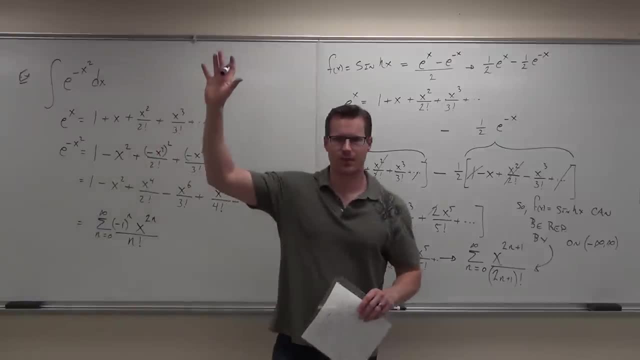 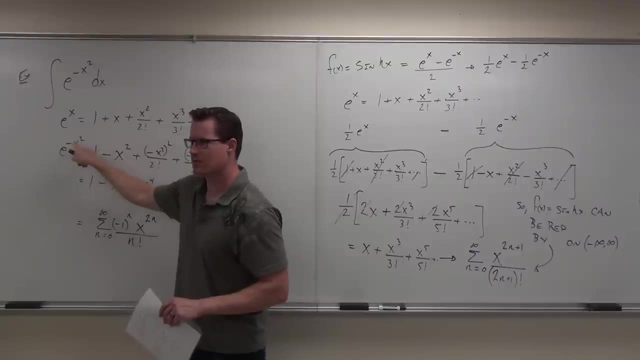 right Show of hands. if you're okay with this so far, You sure you're okay on getting from here. actually, from doing the x to the negative x squared. do you see where that's coming from? We're just taking the negative x squared and plugging it in every single place we got 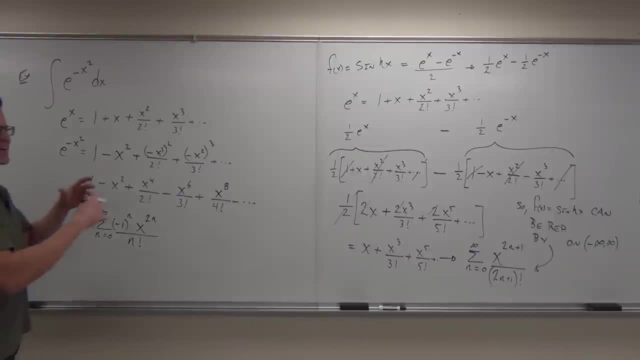 it. Now, this is so cool If we want to do the integral. if we want to do the integral, well, let's just, since we know that we're going to have to go, since we know that this equals this, since we know that this equals you believe that? right, It converges for. 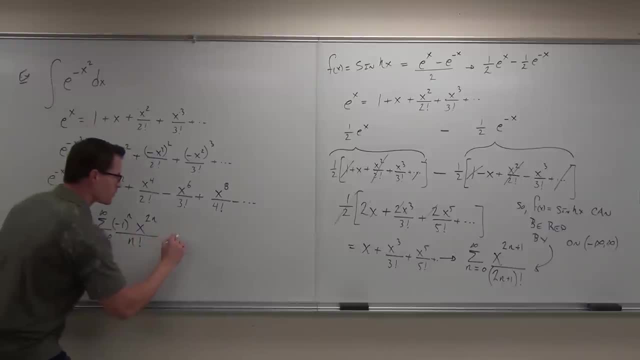 all real numbers. Since this converges all real numbers, this is for all real numbers. Well, if this equals this, and I want to find the integral, do you remember anything about calculus? You can integrate on both sides of an equation. Well then, all I need to do 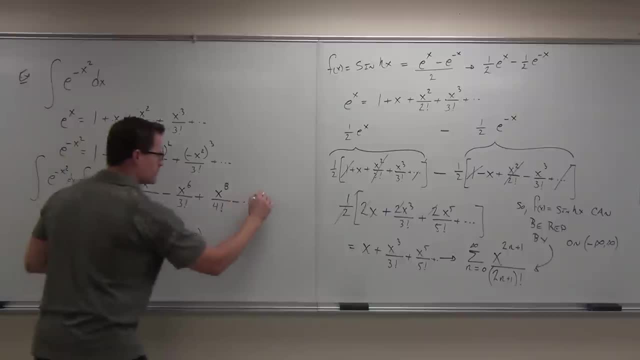 is: integrate this side and integrate this side, Integrate this side and integrate this side. What that means is that if I do my integral, I could do it from here. actually, I'd have to do it from here. Minus x cubed over three, plus x to the fifth over two factorial times. 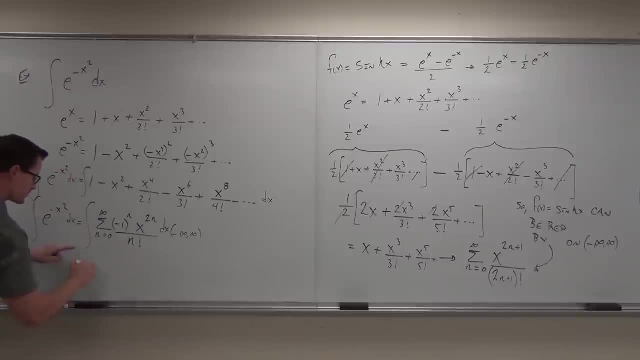 five. Well, you know what? There's an easy way to do it and I showed you this before. If I integrate this one, what's going to happen to my power? Remember doing the calculus on these things. So this is a series Negative. one is still going to alternate. I'm going to have x to 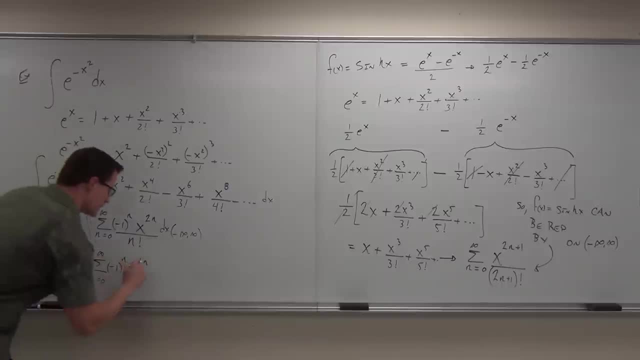 the two? What do you do with integrals? Do you add or do you subtract? I'm still going to have an n? factorial, but I'm now going to divide by my two, n plus one. You can't put them together. There's still an n? factorial, but now you're just dividing by that new power. 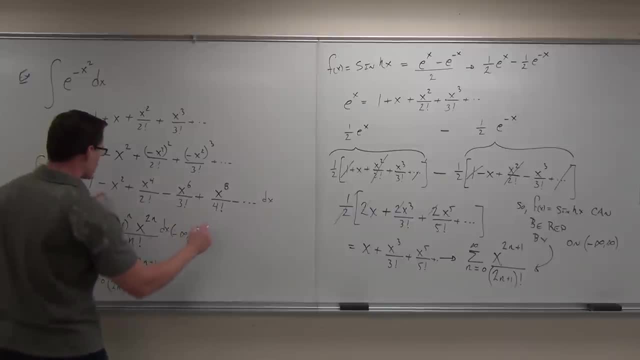 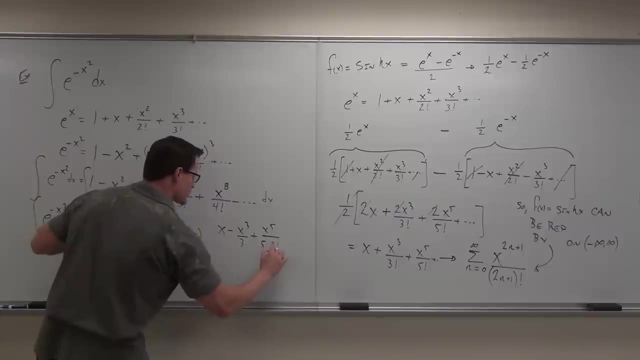 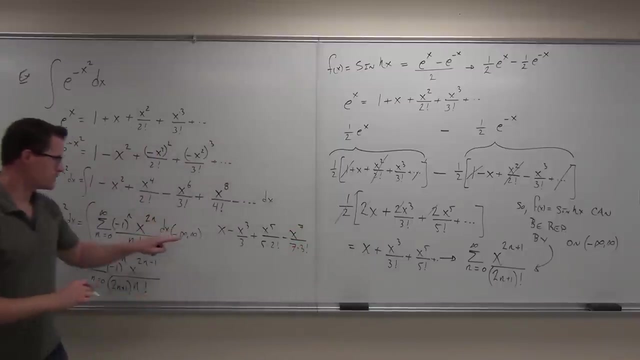 That's exactly what you want to do. What you would get if you did this term by term, Term by term, would give you x minus x cubed over three, plus x to the fifth, over five times two factorial. minus x to the seventh, over seven times three factorial. It would give you alternating, still odd x's. You. 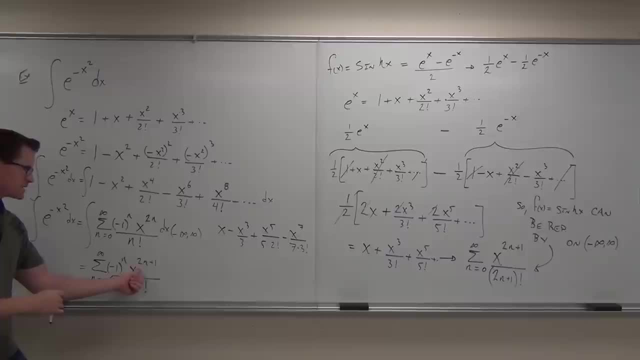 see the odd x's Odd powers of x: One, three, five, seven. No problem, It's giving you odd numbers: one, three, five, seven times your n factorial, Zero, one, two, three factorial, So you can do integrals of functions that you could not. 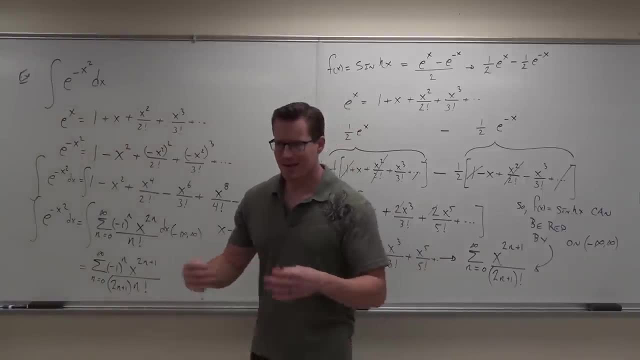 do any other way besides this. Is that not interesting to you? Isn't that kind of cool? We've done an integral of this thing. That integral will be represented by this series. If I want to find the integral of whatever I want, it's going to be on this series from.